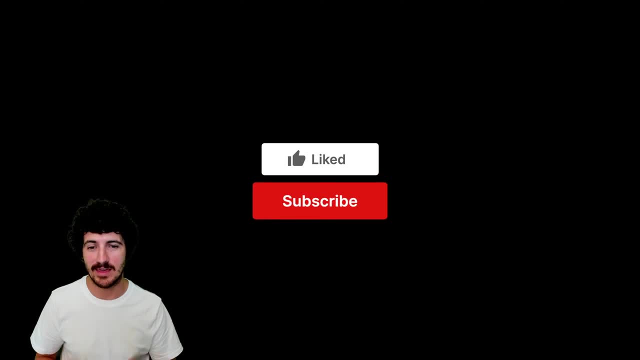 you if you want to support my channel, if you want to support the work that I'm doing here and subscribe if you think you're going to like the content I publish in the future. Click on the bell if you want to get notified when I go live next or when I upload new videos. You can also join us. 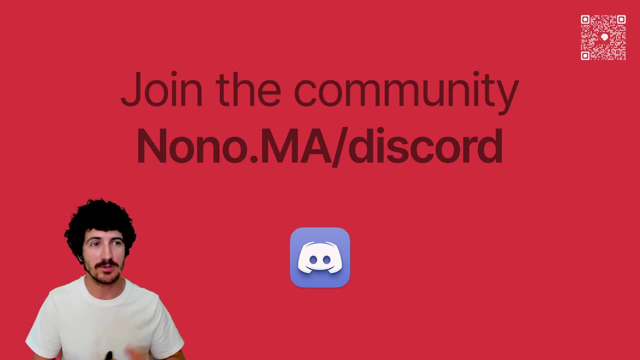 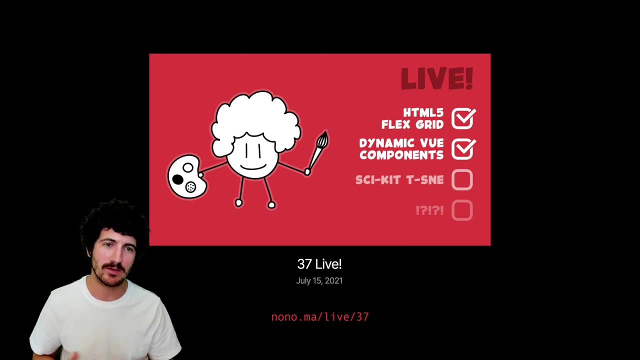 join the community. There is an invite for you at none of the mass. as discord, You can also click on that QR code up there with your phone. and a reminder: last week we didn't see machine learning and the live stream was about HTML5, JavaScript and web components. We did a flex grid with HTML5 and CSS and we also made a 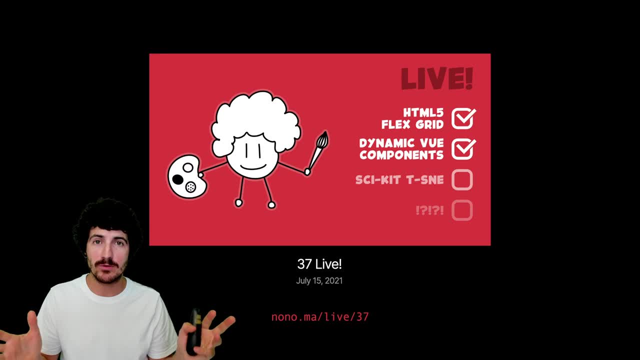 dynamic view component, which was a grid view, that turned into a list that could also be sorted by different properties, say time or name or numbers alphabetically. We didn't get to scikit-tsn and I promised that in a future live stream we would focus solely on that, So I'm going to try to do. 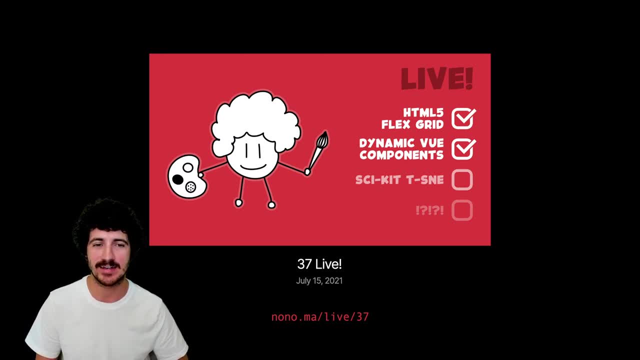 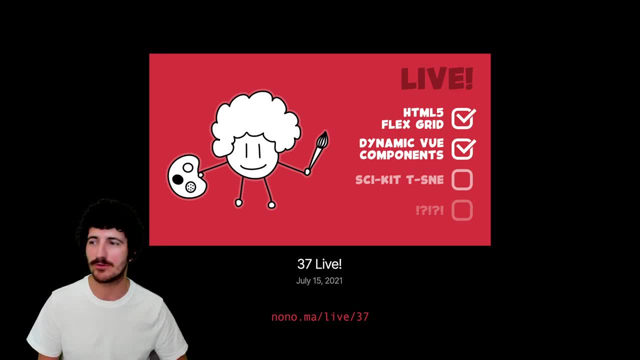 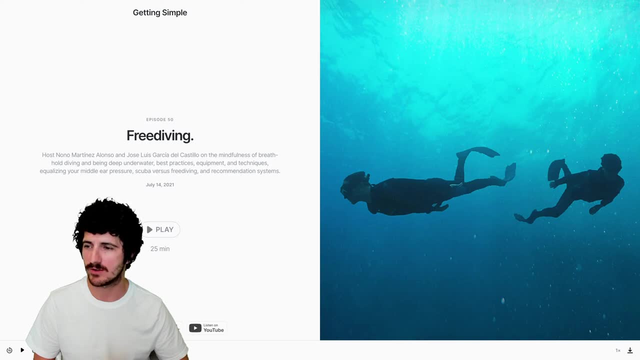 today. So thanks for confirming the audio and video is good And, uh, as a quick announcement, we released- uh, last week or two weeks ago, we released the freediving episode getting simple. So Jose Luis Castillo and George truly talk about the mindfulness of الحctority کی. 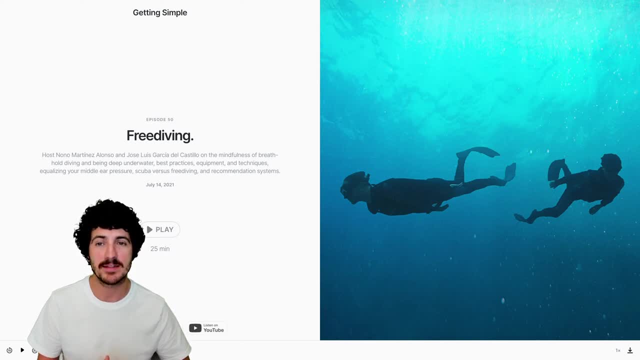 of breathe holding diving and deep being, deep underwater, best practices, equipment techniques equalizing your middle ear pressure, scuba versus free diving, and recommendation systems. i believe this is a really good sport if you're looking to train your. you know physically, your body and also your. 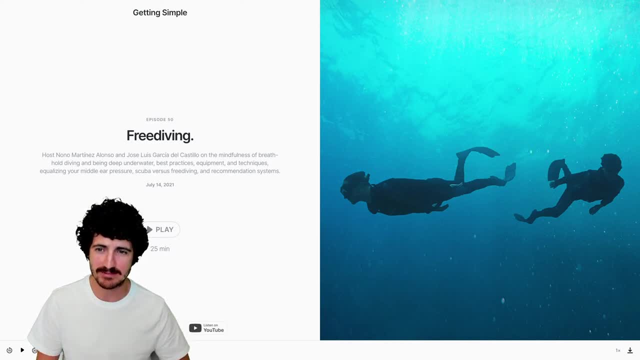 your mind. so it's mental and physical and, yeah, i'll invite you to listen and tell me what you think. it's a short one compared to others, is 25 minutes. and hello, john mark. also nice to see familiar faces online. glad that you passed by and um said hi in the chat. all right, so 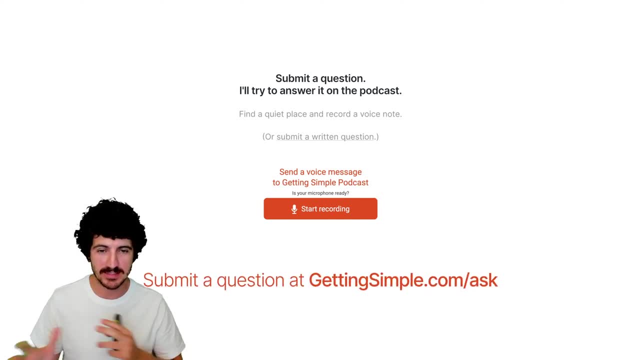 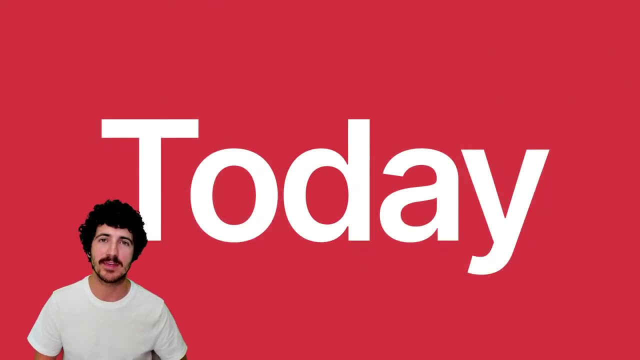 you have a door open to ask questions about this or previous episodes of the podcast at getting simplecom. ask and we're going to get writing into today. so today, as i said, i don't know if we'll have time to do this, but i'm going to do this today, so i'm going to do this today. 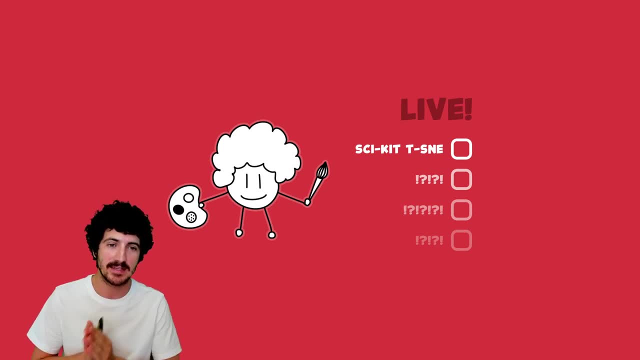 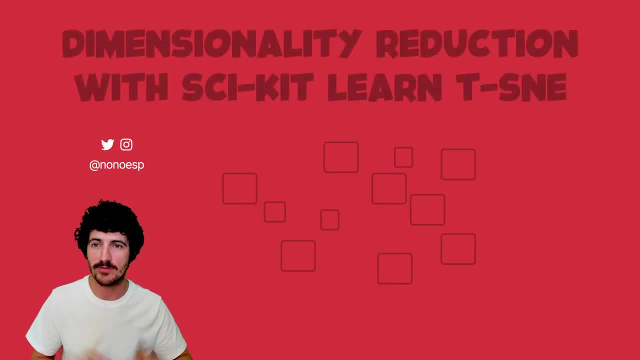 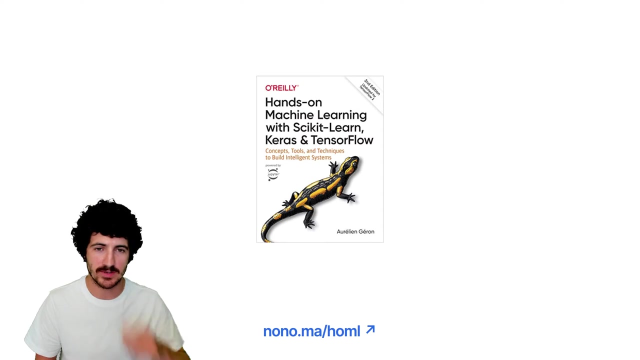 for other things, but for sure i want to get started with the psychic tisney project or or exercise. this is the cover. of this is dimension dimensionality reduction with psychic learn, tisney, and we have some material, so i am getting material from the handsome machine learning with psychic. 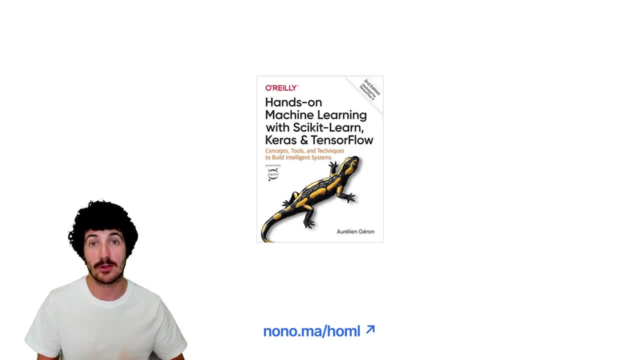 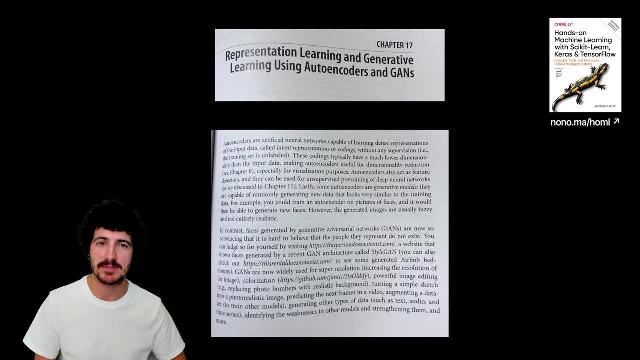 learn keras intention of a book by aureline jiron that i am encouraging you to get, or or like, learn from, if you want to get a little bit more information about psychic learning please. if you want to get into machine learning, specifically about chapter 17, that was. 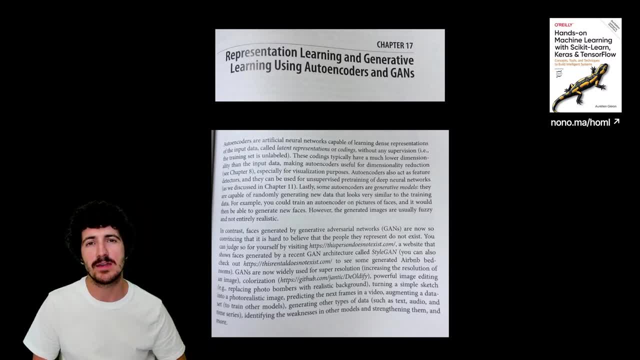 auto encoders and guns. this is something that we did on live streams- 34- i don't know if 34 and 35 or 33 and 34, but you can go back. they have. i think they have chapters and these are the ones that go through how we actually build an encoder, a decoder, and 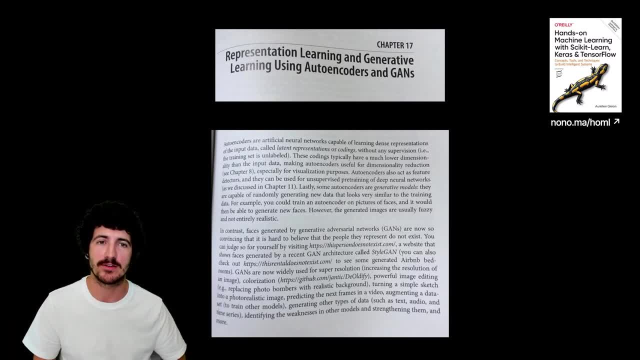 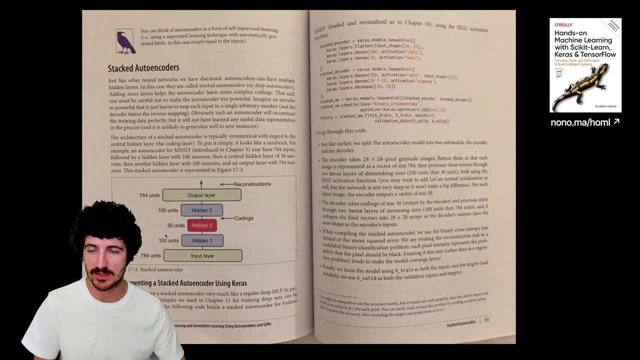 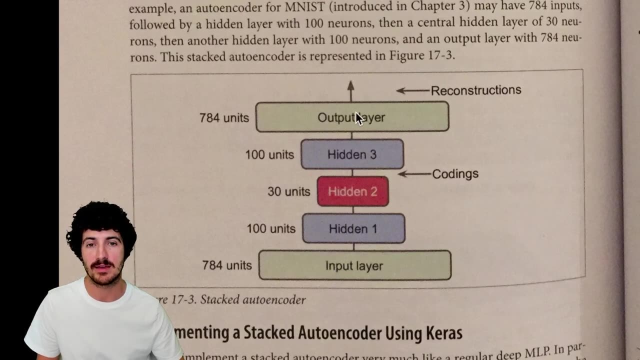 how we stack them together, and you know there is a lot of theory there. that, or or even handsome hands-on practice that we learn from this is: you know there are many ways in which you can do this- stacked out encoders. but long story short, you try to input something and get the same in the 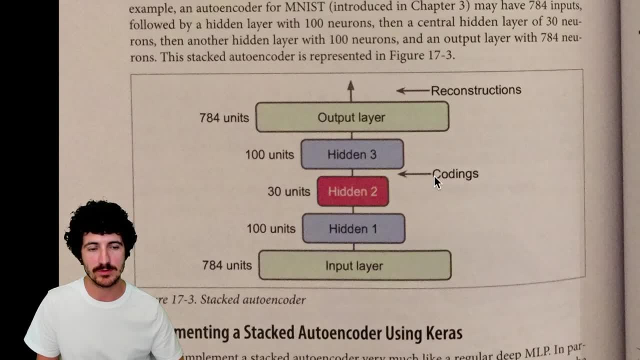 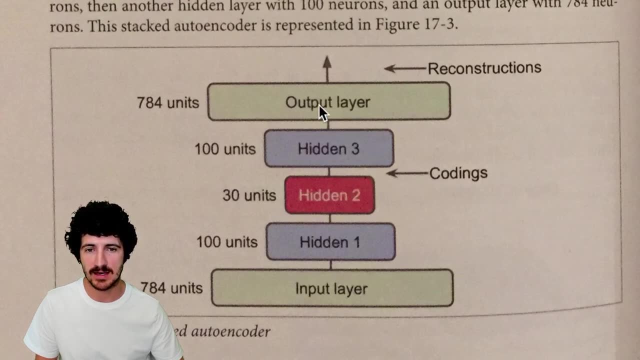 other way, but on the way you're training an encoder, so you're obtaining these codings on the right, and then you have another second part of the network, that is a decoder which from those codings, tries to regenerate the original output. these are networks that are mainly 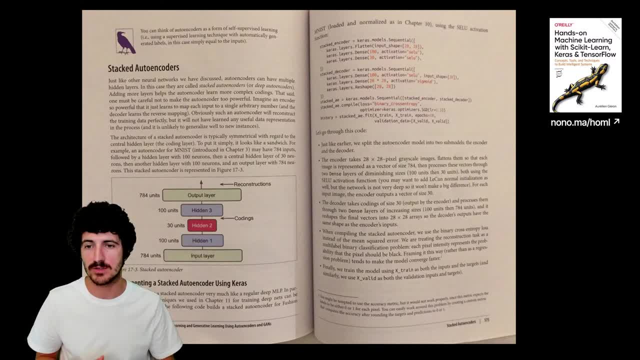 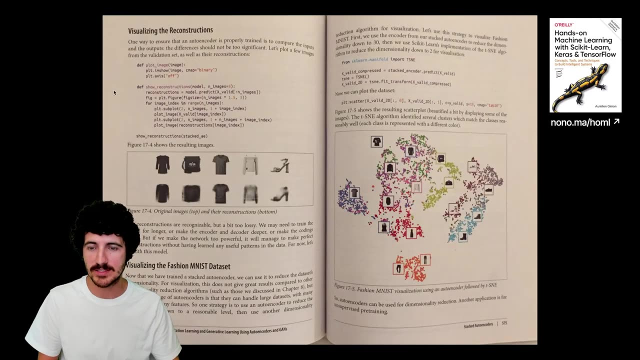 for noise removal filters, not for generation, because the the output are usually noisy. but if you get guns on the game and other types of networks, these are good architectures for generating images. we saw how to do this, i believe, in live 35 or 34, how to get a network that could. 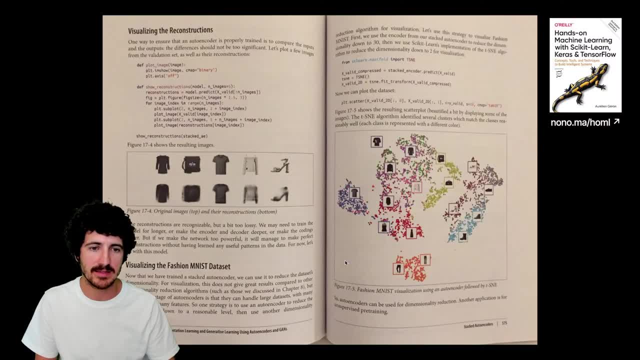 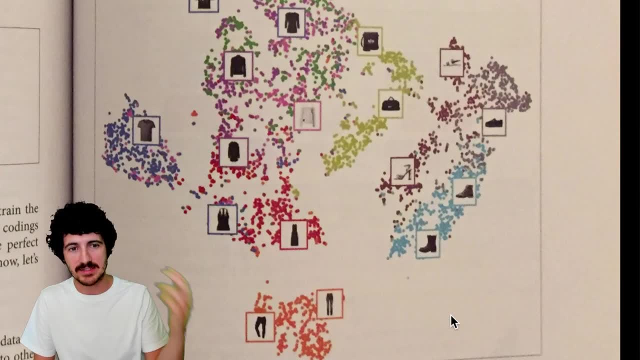 learn how to generate these images from this image, and what we want to see today is this part here. so is um, what we would imagine that we can obtain this is, uh, disney, um, flattening a highly dimensional space. we have 30 digits of 30, a coatings of 30 digits, i think, on the network that we coded back. 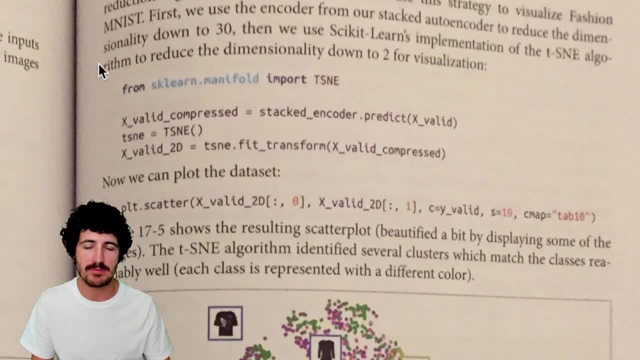 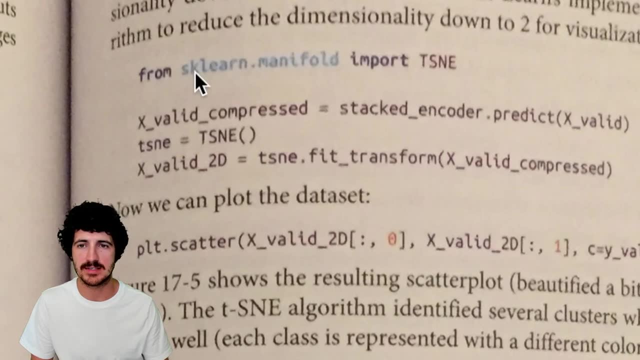 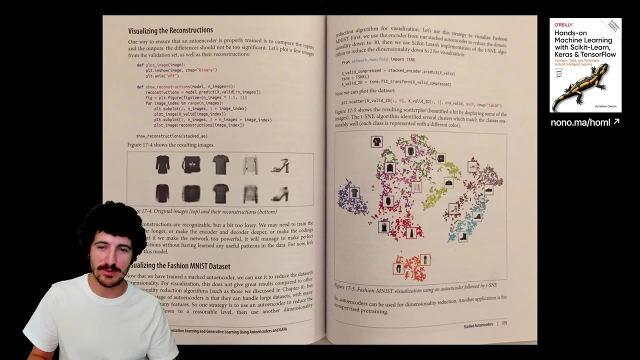 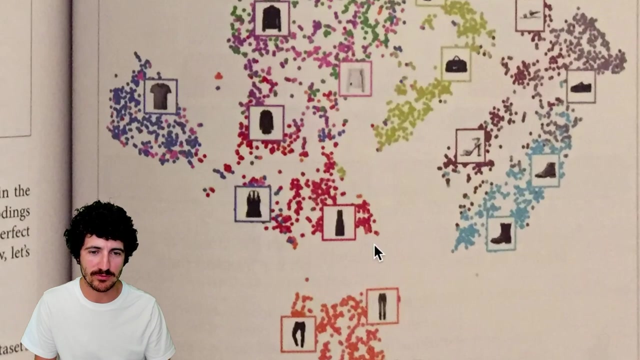 in previous live streams and with this library, so with the disney library of from sk, learn manifold, and this is really pixelated because this is a really bad image, but i have the book here with me. so, yeah, we're going to try to visualize that here and i'm not sure if we're going to be able to get. 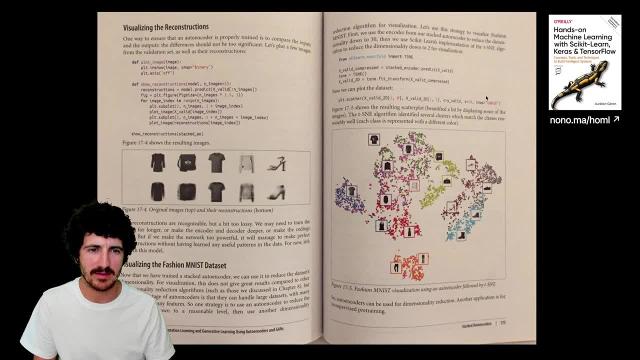 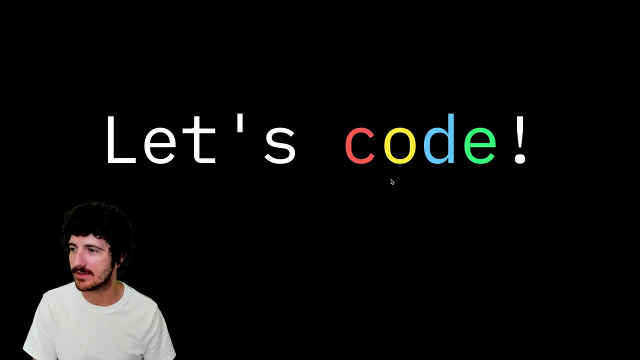 this big images here by automatically? i think maybe we are, but yeah, we'll see. so i think that's it, so we can get, uh, started with coding now and, um, one thing that i'm going to show you now. all right, so quickly turn over to the chat here. 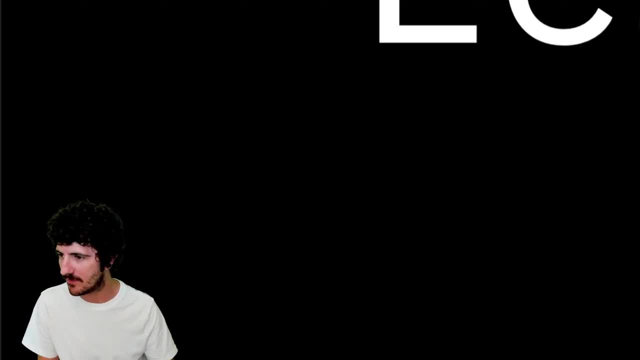 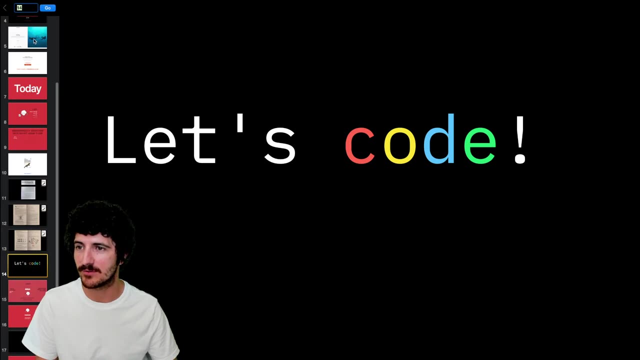 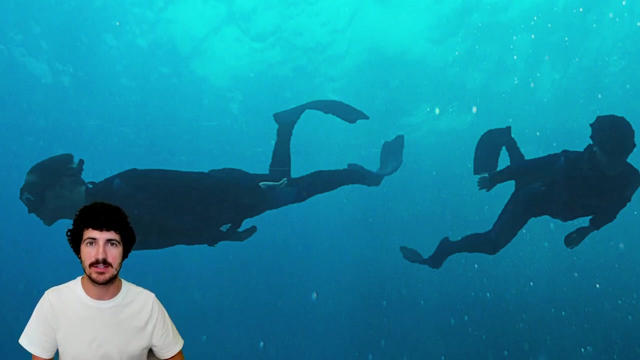 john mark says i like the free diving too. a bit far from the sea right now but compared to scuba, enjoy the liberty. yeah, i actually haven't tried. so this is kind of commenting on this. i actually haven't. uh, i haven't tried scuba diving, so actually diving underwater with an oxygen bar. 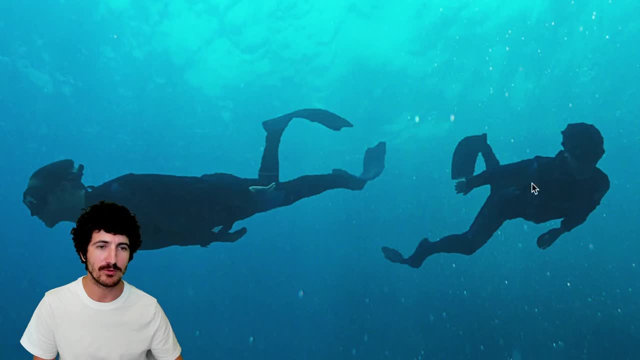 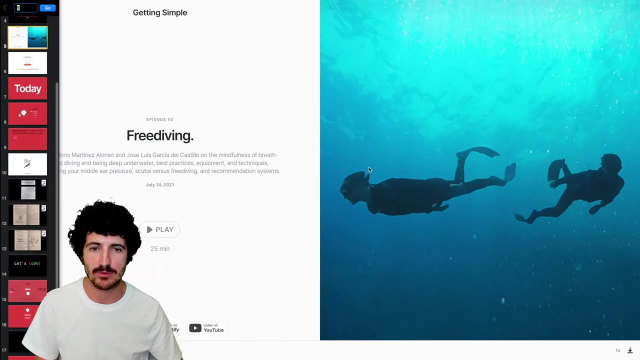 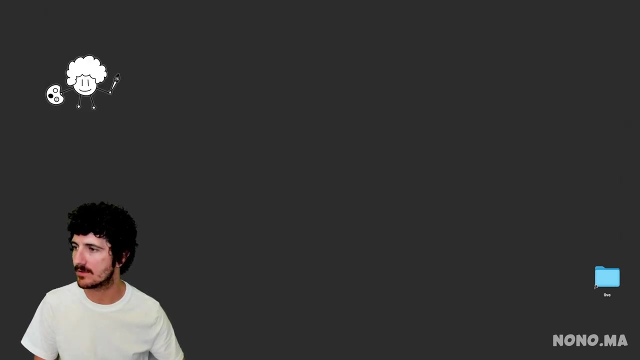 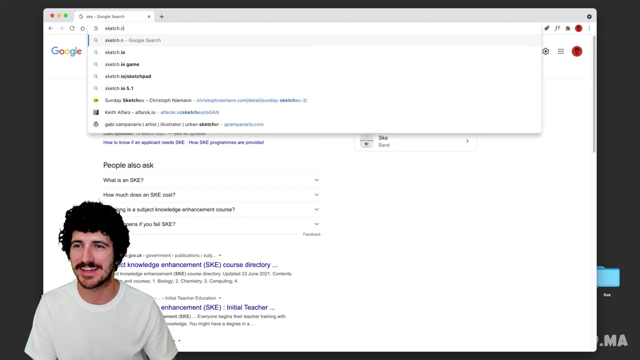 i've only done it um snorkeling or with, like you know, free diving techniques, which is uh with, uh like a lead weight, bells and and other things that let you go um deeper underwater. so the um, the one thing as a, as a pointer, that i think i showed last week on the on the sketch, ah sketch. 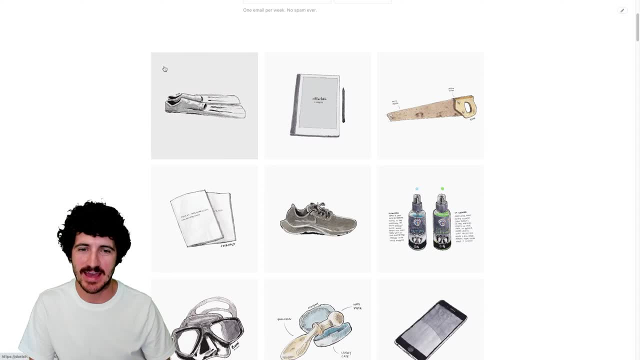 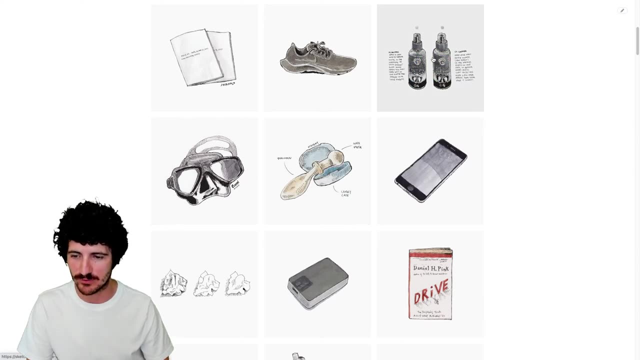 terrorism ma site if you go there i have an � a few stories. So this one that was an auto event, this one is first impressions. This one is how to prevent your diving or snorkel mask from fogging up. And then this last one that is the diving reflex. 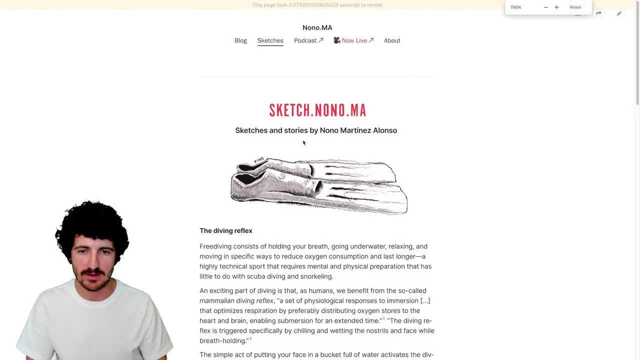 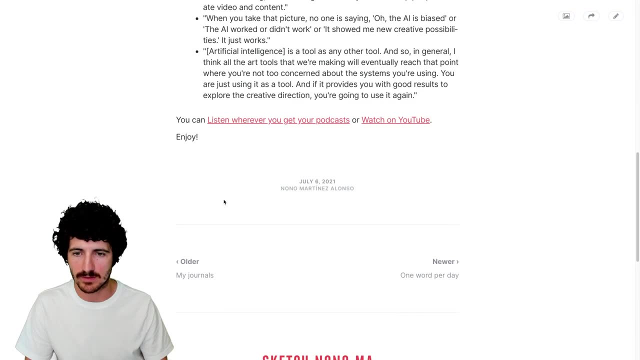 You have a few short essays or publications that talk about my experience free diving or some of the concepts that that I've learned. You can go back here, So blah, blah, blah. Yeah, There are a few back, Yeah. 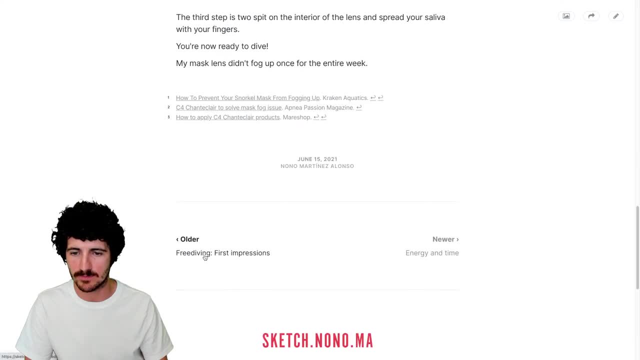 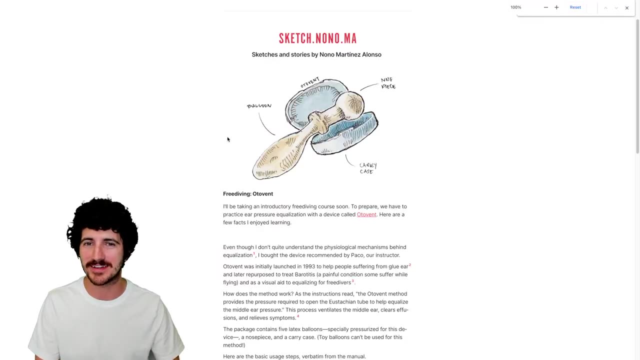 So these ones, so this is the ones that I was. You mentioned it before, All right, And uh, yeah, I think that that's it for kind of the the plug, or like showing some of the things that I've been writing lately. I see, also, class is high. 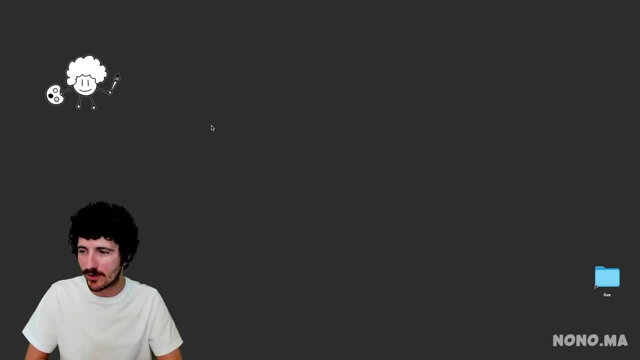 No, no, um class, I believe I haven't seen you on the live stream before. Uh, maybe you can tell us how you found the channel or why you're connecting or where you're connecting from. All right, So I said I was going to show. so we were: uh, at this, let's go slide. 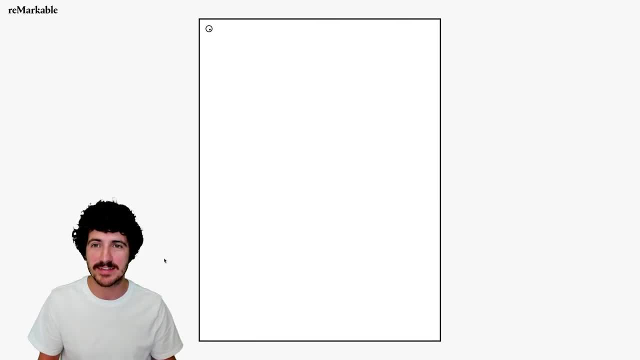 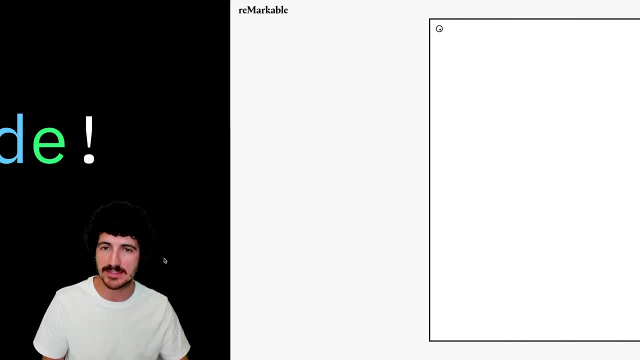 that is kind of what we're going to start doing now. I have something here on the right. This is something that I've used before on on the live stream but that I want to show today, So one of the sketches that I had on my on my site was this: uh, remarkable. 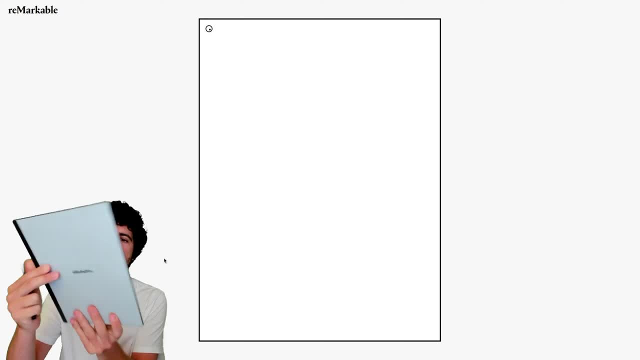 tablet that I hope you can see there Right? So this is a the remarkable two tablet and they just released a beta feature today, Like I discovered it like five minutes before going live in. Look how awesome this is. So now I can uh, sketch here and take notes on like a whiteboard style and you 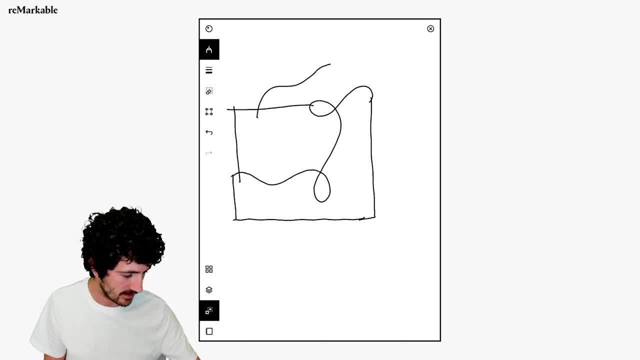 can see that light right now. I can go here and I can erase all and you can actually see. so this is a new feature that they called a screen share, which before you could just see like some sort of life uh VETA view, but now you can actually see me. 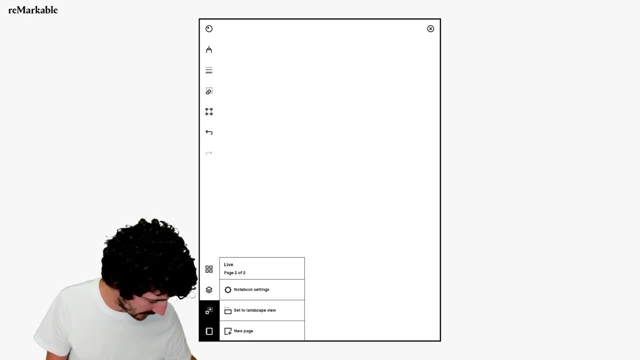 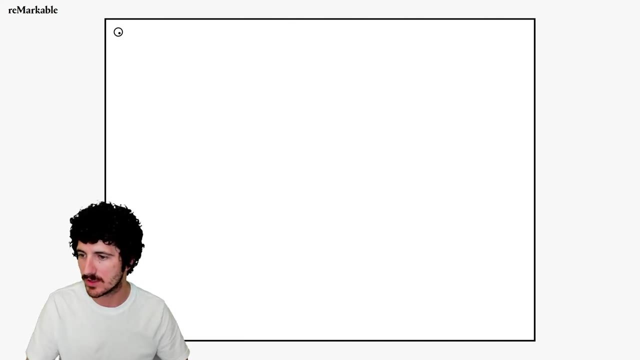 Uh, drawing life, and I haven't tested yet What would happen if I said to landscape view: Yeah, this is probably even better because we get, we get it zoomed in and I can just put it like this: and I have uh a canvas, uh a canvas board. 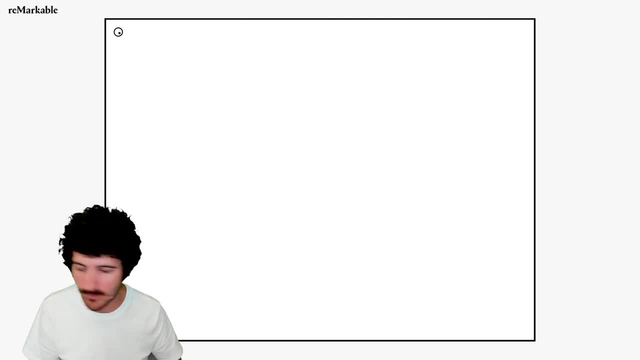 Uh, all right, So I see also. uh, I'm from India, Okay, So, um, hello, I can put here too, and we have here Class from India. So seems to be like, um, a new subscriber. 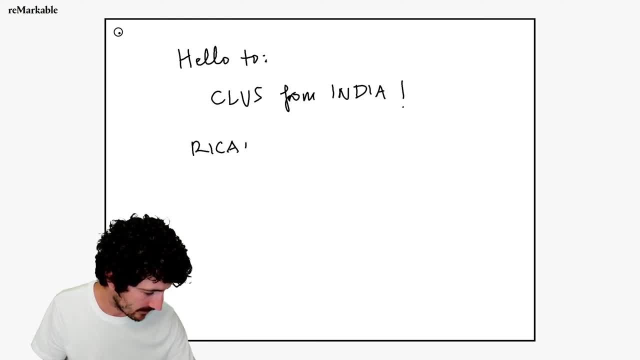 So welcome. And uh, Ricardo, from Brazil, I'm your new subscriber. Well welcome. I hope that you enjoy it. today We're going to see a lot of machine learning, or at least a bit with a Disney. So, uh, let's take a look, and you know the policy. 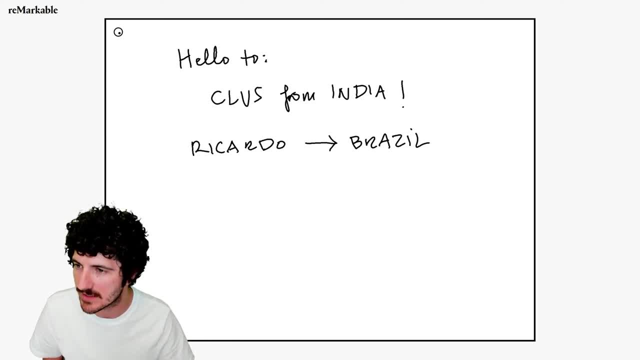 So, And I don't know how many, yeah, three people voted. It seems like everyone wants to see Disney. Um, I don't have another great alternatives, but I'll I'll try to do that. um, moving on, 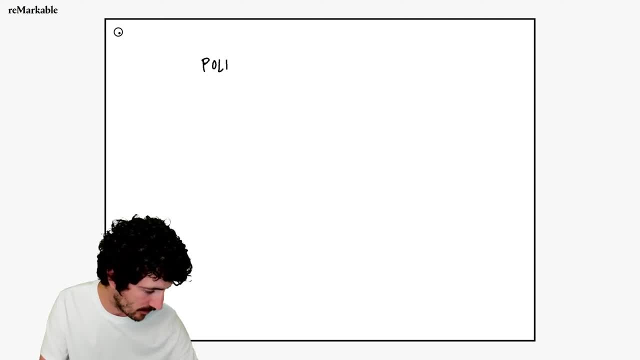 So in future, live streams, So we we get this sort of polling system where we can um go between, uh different choices and and you guys can be the ones that pick uh one on the other, in this case, the one that 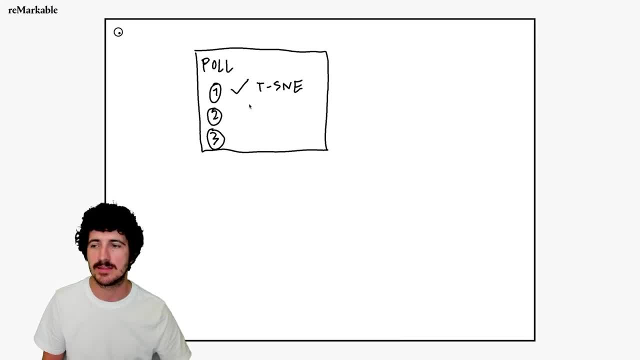 Um, one is Disney, So this is also just to encourage you to be, uh, live at the beginning of the live stream If you want to kind of um participating, choosing the topics that that we're going to discuss during. 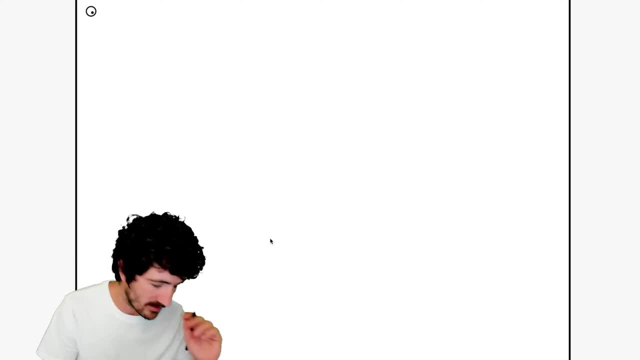 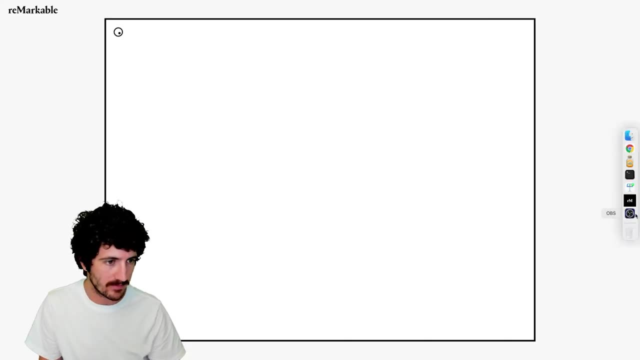 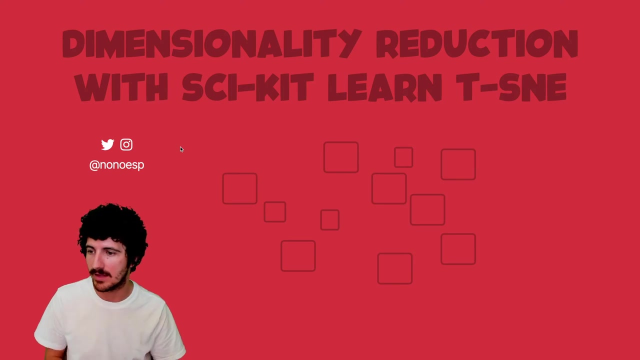 the, the live stream itself, All right. So things that we have that um, I'm going to go to the um just record a like an interest screen For this, So we have it later for in case we edit a tutorial and we'll get started. 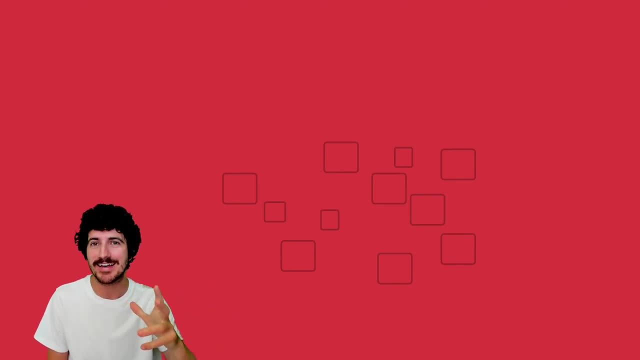 Also a question that I'll ask while I'm recording this. anyone has, uh, played with Disney already? We psychic learn with Disney, because I like to know if you have any insights or any comments that you can do there. Hmm, Okay. 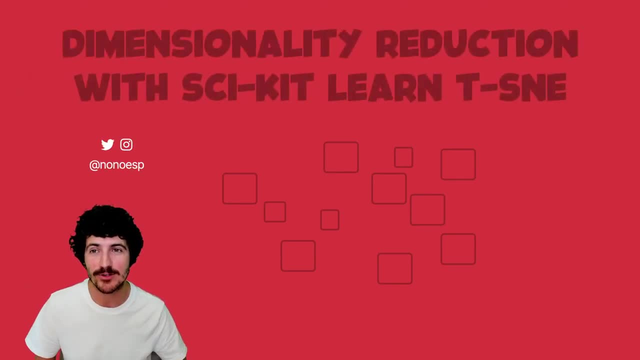 Hi everyone. It's not here And this is a hands-on tutorial on dimensionality reduction. We're going to try to do that with psychic learn and the Disney implementation that comes in this package. We'll try to get the codings that we've obtained from another neural network. 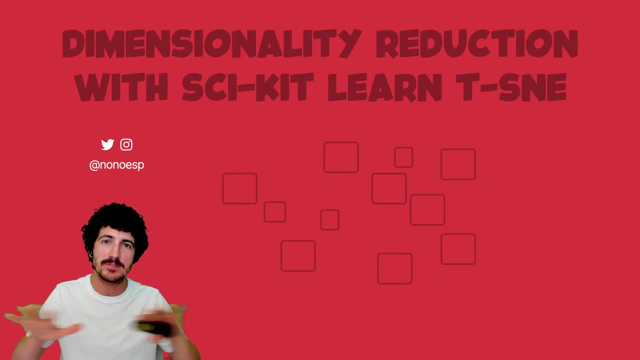 Put our data set inside of psychic learn and try to reduce the dimensions of our data set into 2d so we can plot it into a 2d map or an image and we can understand the similarities. or Howard data set. Uh, Luke's, when you compare one input to the other or one data sample to the other, it's not a marketing thoughts of here. 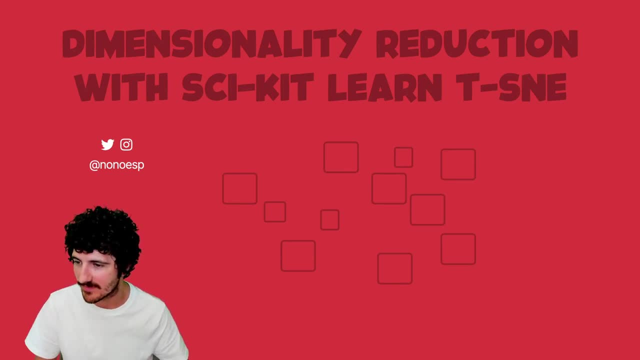 So let's get started, All right. So, uh, we're going to now record an outro, just in case I forget that as well. but yeah, I don't know how long this is going to take. So okay, Thanks a lot for watching. 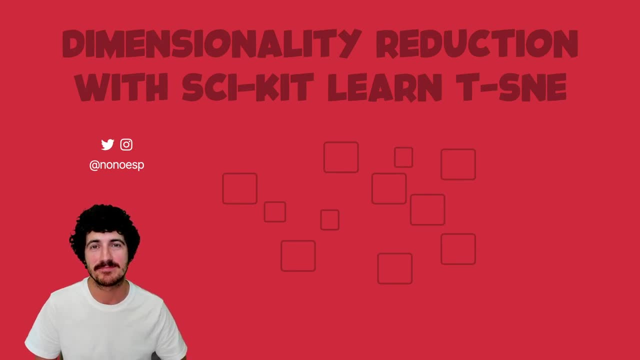 It was none of here in. We'll see you next time, All right. So I see, um, I want to know one. nothing, I'm importing cafe, but it's showing the Sarah cannot parse, Yeah. So clues for questions that have, uh, not too much to do with the topic that we're covering today. 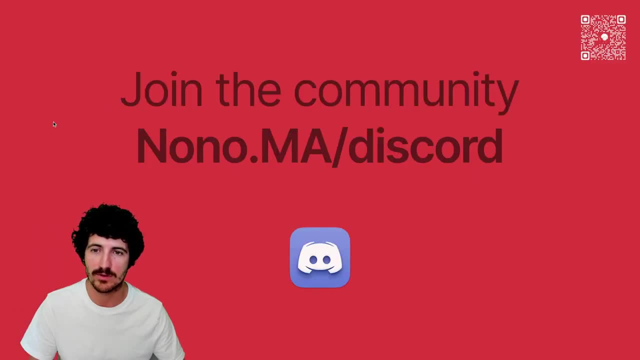 Um, I would encourage you to go to the discord server so you can join the community. Yeah, Yeah, You can ask on the. probably this is good for the coding channel, the code channel. You can go into that QR code or at none of the masters discord and you can ask those questions there. 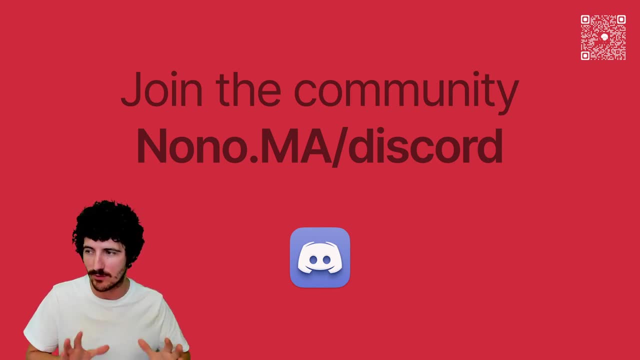 I don't think I can help you today, because we're going to focus on a different topic And, um, yeah, maybe, maybe you can do that, I'm not sure. All right, So let's get going with, uh, what we were going to do. 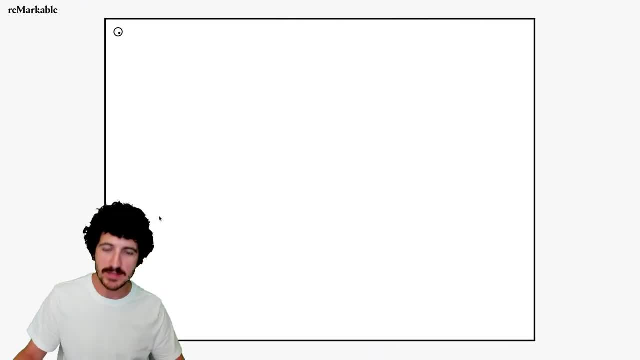 So this is the tutorial, All right. So we have this canvas here And I'm going to make, or I'm going to do, a recap of everything we know and everything that I expect to do in the next hour. So let's see if I can center this thing here. 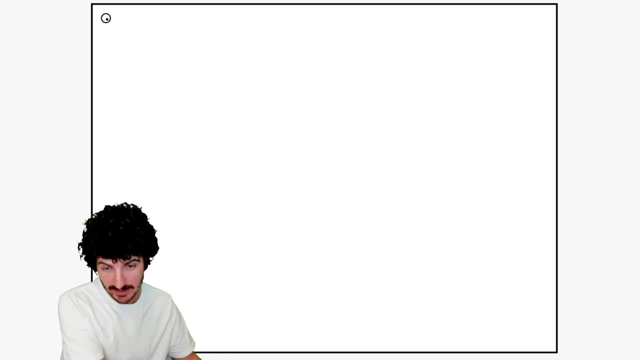 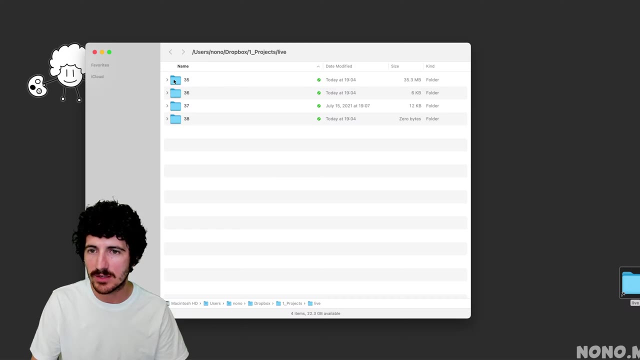 All right, cool. So things that we know or things that we already have on live stream and I have to check there, Um, how can I do that? Yeah, So, live stream 35.. Um, yeah, So we generated these, these data set and, I believe, live streams. 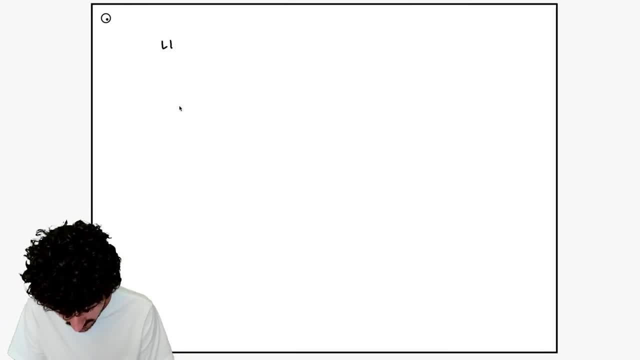 Okay, So in live stream. so life um 33 and 34, we did see Stacked, Yeah Yeah, How to encoders. we made, uh, I believe, two versions of a Colab notebook And, uh, in there we were actually having that architecture in which we were taking in an image. 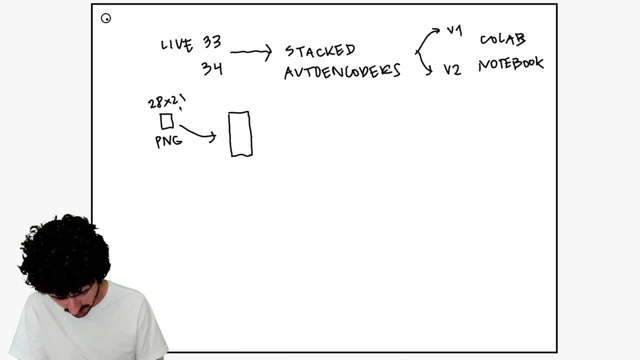 So that would be like Maybe a PNG. I think that was 20 by 28.. Uh, we were encoding that into a 30 digits, right? So these were the, the coatings of our network, And then we were getting that back into another image that is 25 by 25.. 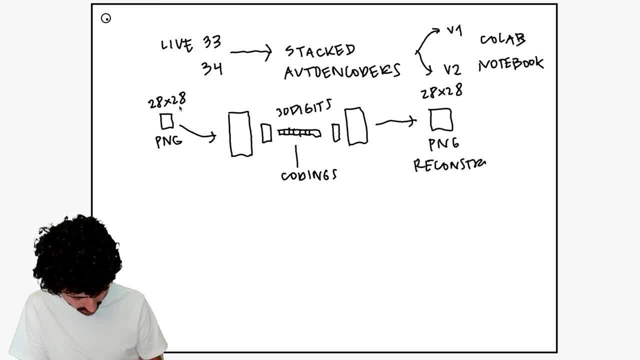 That was the reconstruction Um, and this was our input. So we uh tried to do here is to train this part, which is an encoder, And, uh, this part here that is a decoder. What did the? what the encoder learns um how to do right. 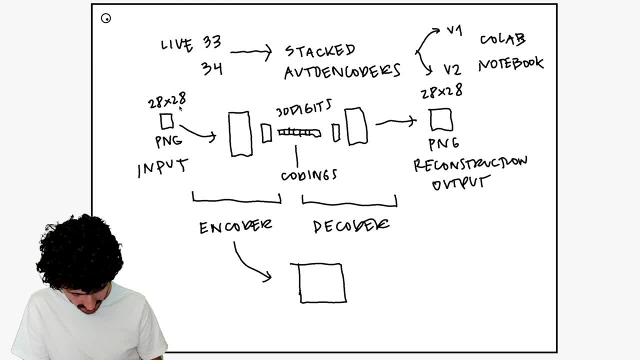 So the encoder learns how to take An email. So, whatever it is- and it's 28 by 28,, which is 768 pixels, into a one, the tensor or Ray that has just is one by 30.. So it has 30 digits, right. 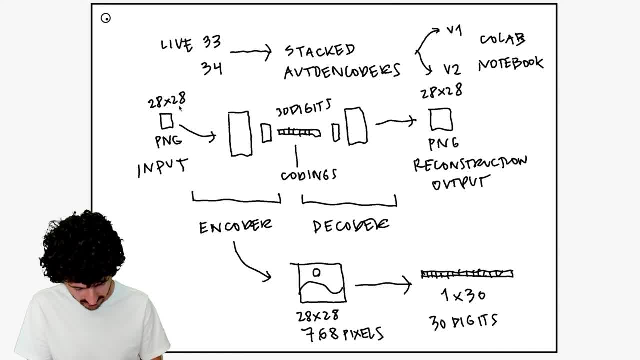 Or pixels, whatever you want to call it. It's just: 30 digits is not pixels, because here actually we have RGB, So Three channels for each of those pixels. All right, So we're trying to get, and I'm going to go to the next page now- 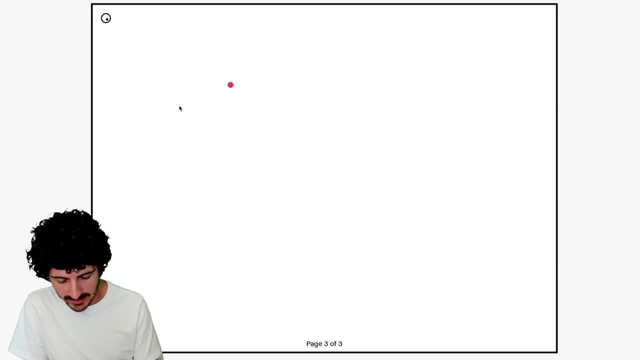 So we're trying to do is trying to get a network where we put an image right. So we have our network here, which is a decoder and we're going to get. so this is our input and this is our Okay Codeings. 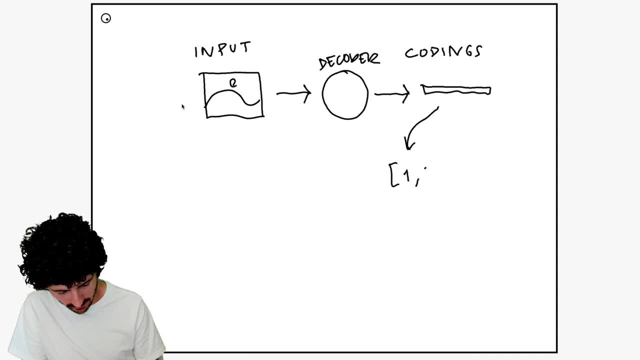 And those coatings that I mentioned are going to be 130. So three digits we'll then input into tehs knee and are going to be able to plot on a two D image And hopefully we're going to get clusters That belonged to different classes. 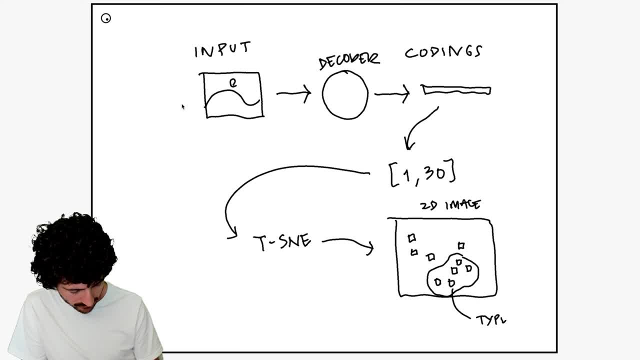 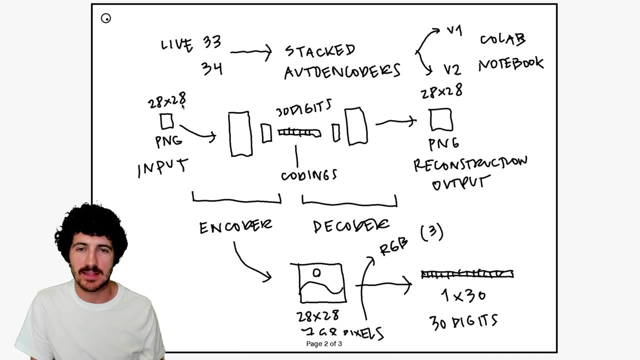 So, for example, this could be Okay, Uh, type one or type two. The problem is that my- so the data set that we're going to use those sketches that I showed before, those don't really have a like. we don't have a classifier. 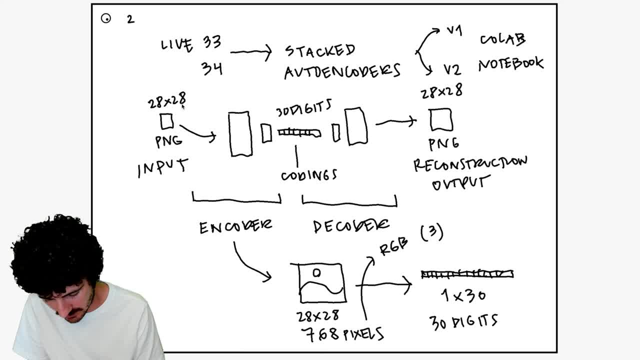 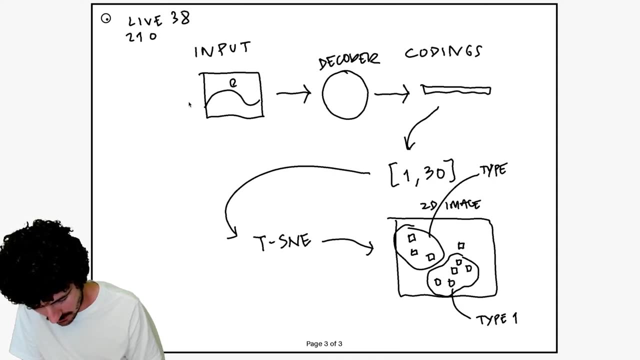 to classify them. so we'll just see how the data samples look in similarity between them. So we're just going to try to do that. Let's just add here live 38.. This is like 38 and it's 22nd of July. 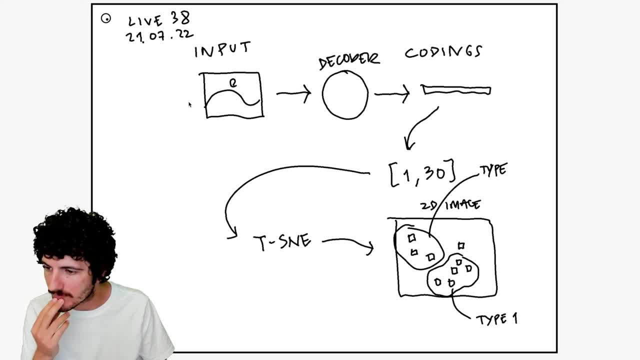 All right, So I'm going to read here the comment from Ricardo. So I've already used this knee. Let me see Oh message retracted. I was going to read it in Ricardo, but you lead it before I could do that. 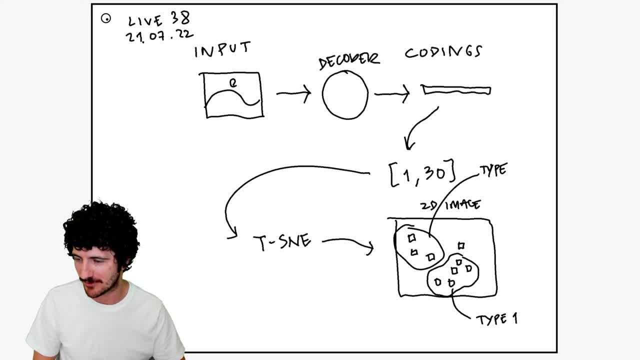 So if you want to rewrite, if not, it's fine, It's up to you. I was. now I'm curious about what you were going to say that you've already used at Disney. Okay, So let's keep going. So the first thing we're going to see is, like we're going to take a look. 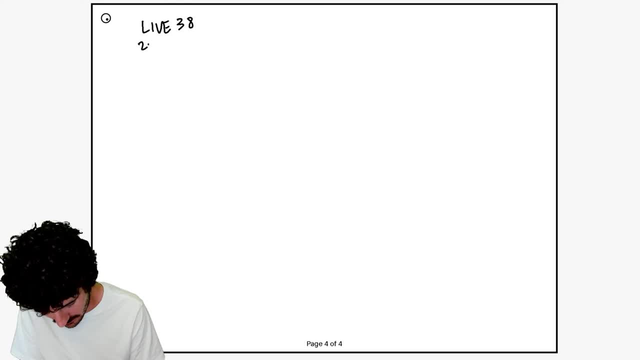 So this is again live 38.. Maybe we don't need to write the date all the time And, um, we have a set of 105 images. We need to, We need to recover our notebook and, uh, we need to, uh, make a new one, you know. 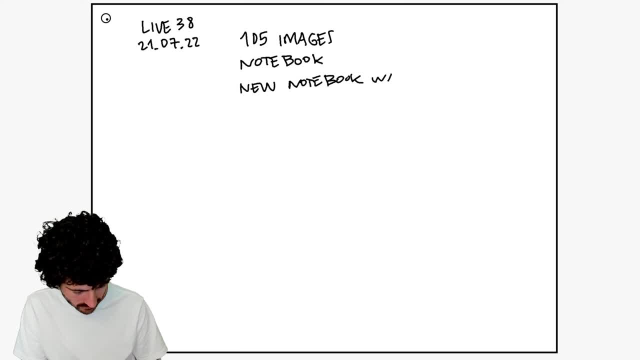 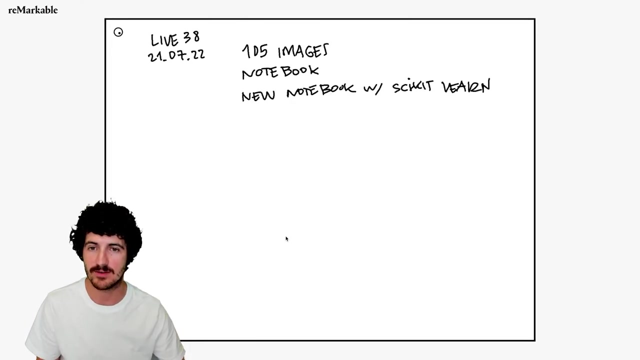 book with side kid: learn, Right. I think I can even zoom into here, Right, Awesome, Cool. So let's see, So I can. um, yeah, let's do that. If you have any questions and if your life, feel free to put them on the chat. we're going to get started right now. 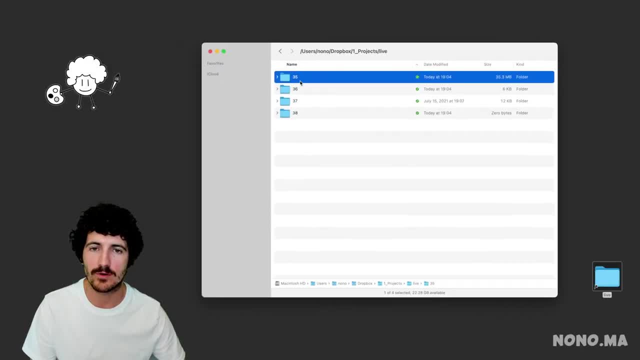 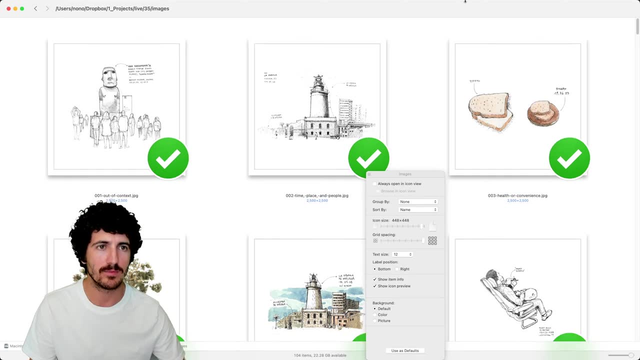 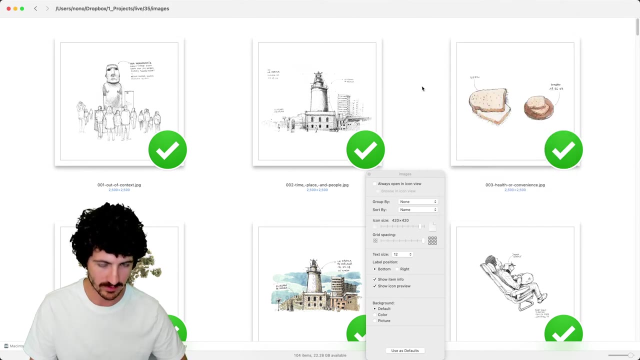 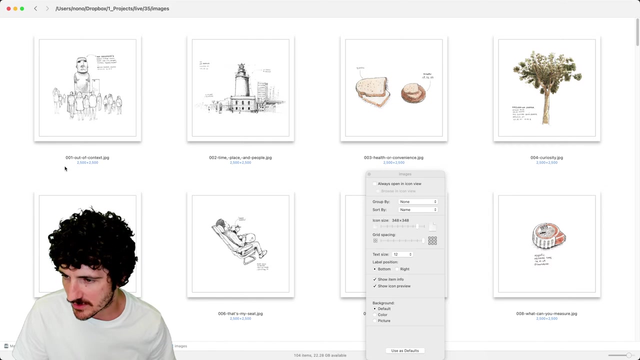 Great, Cool. So, as I said before, I have these data set, so we have 105 images from my hope. that's actually stopped Dropbox, to make sure that This doesn't slow down the computer, Right? So Ricardo was curious about using the t-SNE with convolutional neural networks and make Disney plot instead of images in the plot to plot colored data points in an unsupervised way. 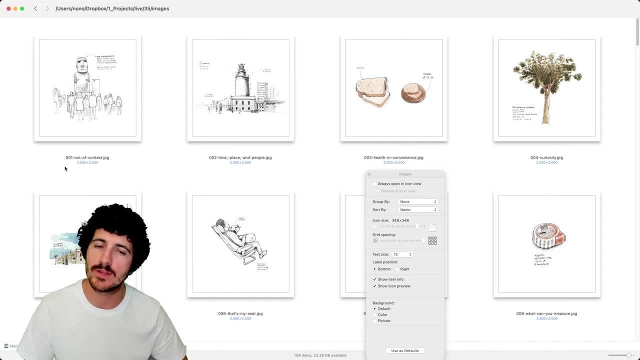 Data points in an unsupervised way. Can you elaborate a bit more? Would that be like um things that the network is learning? I'm I'm not exactly sure how that would like. I can not imagine it, And maybe that's what the the exercise you're proposing is about- about figuring out what it does. 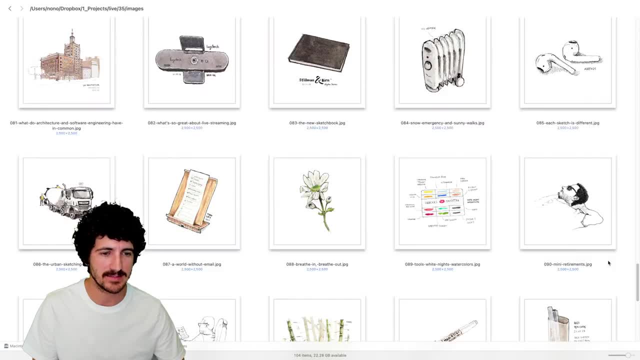 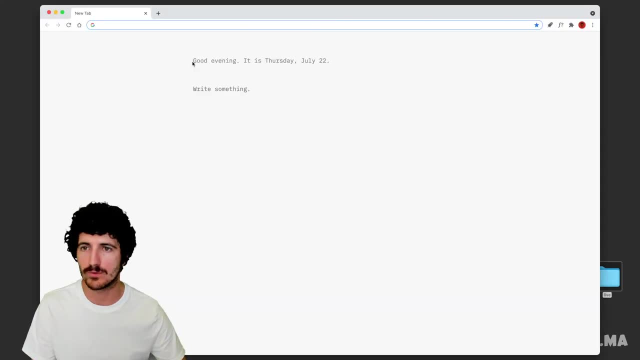 All right, So this is a data set and, uh, these has 105 sketches from the website, So we have a if you go into um the live repository, So this is the repository of the live streams in live stream. 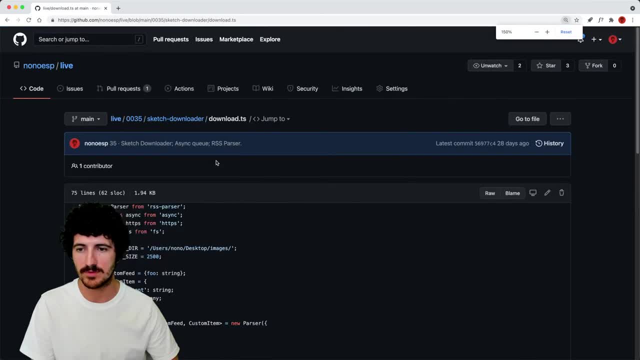 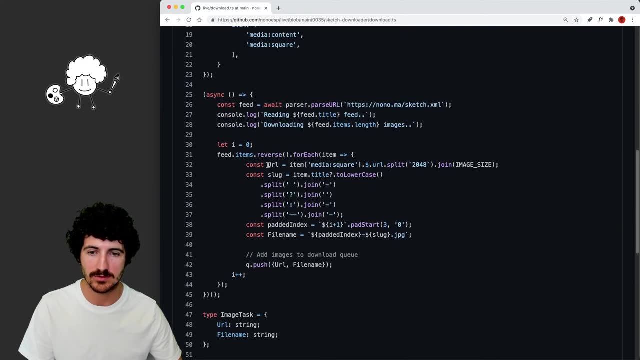 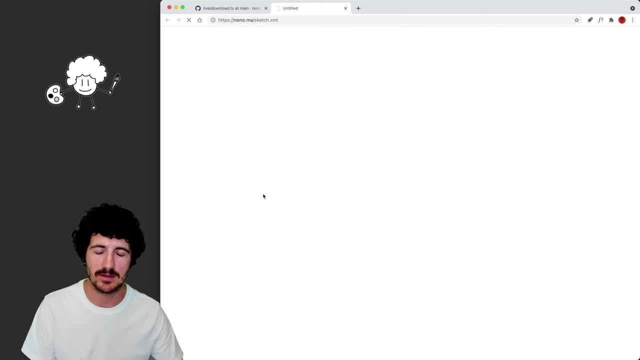 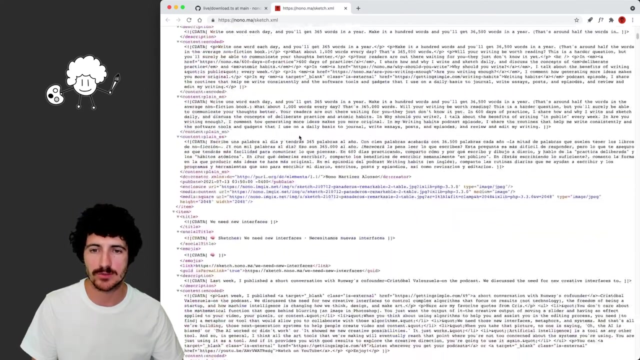 35, you have a TypeScript script that will guide you step-by-step on how to use an asynchronous pipeline to download those images from my RSS feed. That is here, but you can actually change the URL of the RSS feed and a few properties to download images from another source, right? 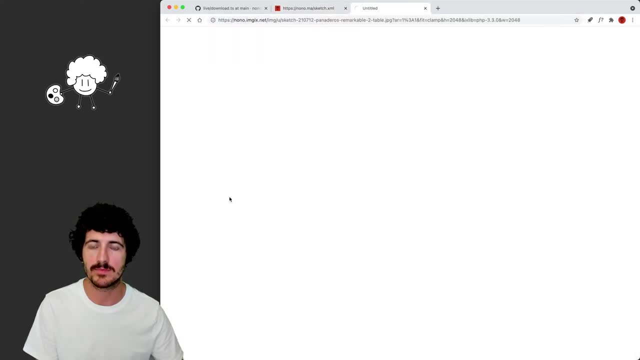 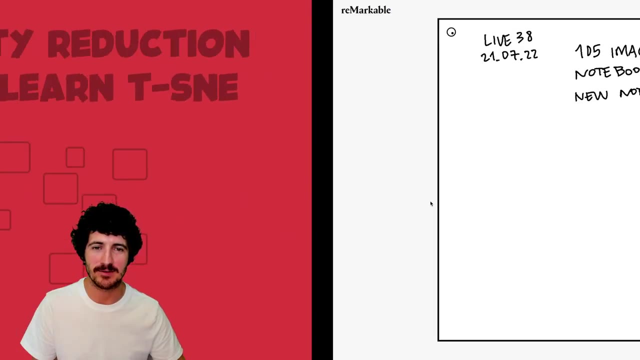 In this case, we were just getting the images from here that, Um you know, show you that here. finally, no, this is a remarkable tablet that I was using, uh with uh, this application here to share screen. 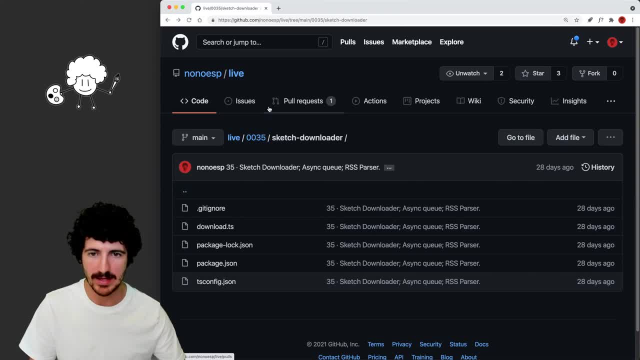 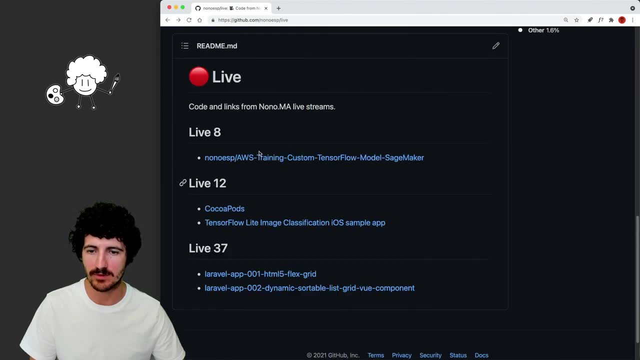 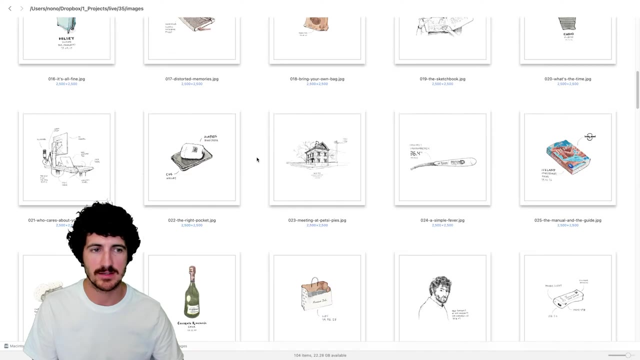 And yeah, so you can go there to take a look at that, And I don't think we have more things here on the, on the repo, the algorithm that we're going to use. uh, well, I was mentioning we have these 105 images. 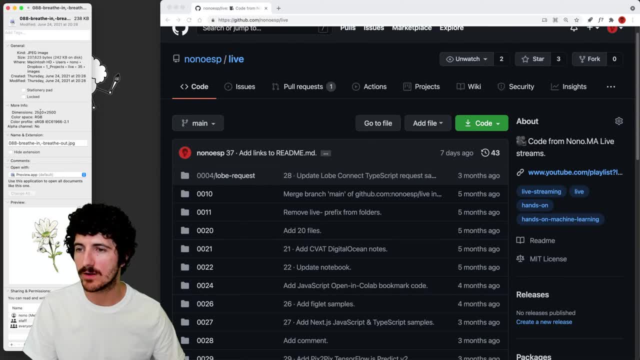 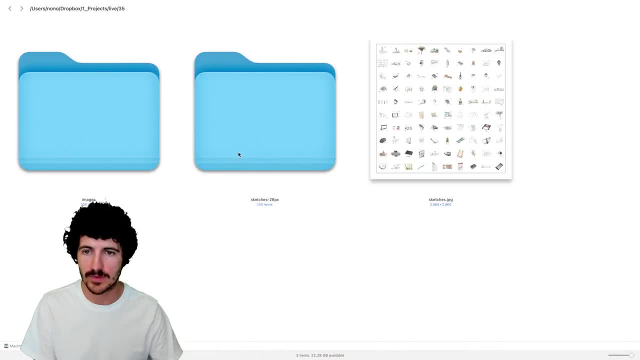 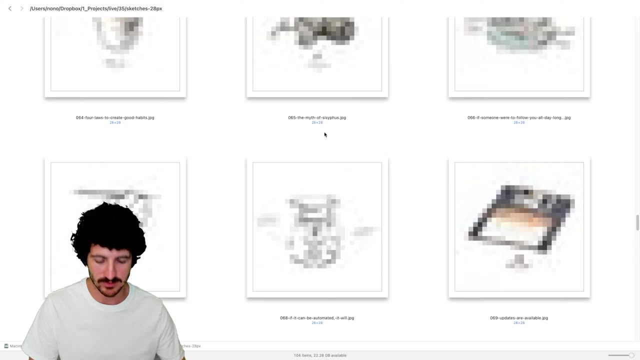 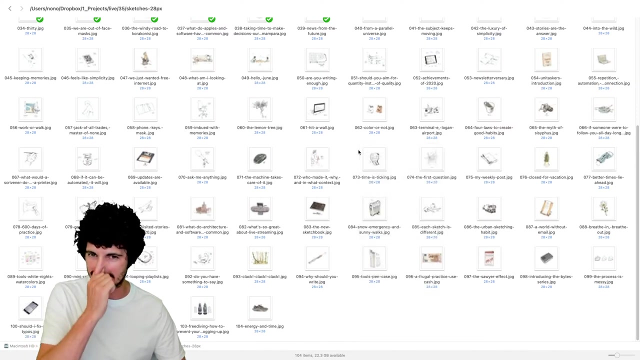 These ones are 2,500 pixels height and width And, um, if I go here to sketches, 28 pixels. right, You see that these images are super small, so much as we can not understand them by. if I make them a bit smaller, you start trying to maybe make sense of them. 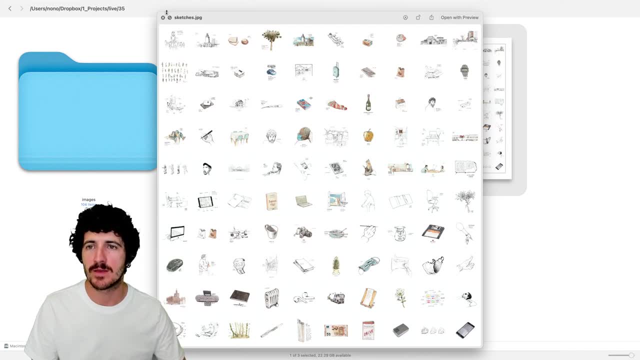 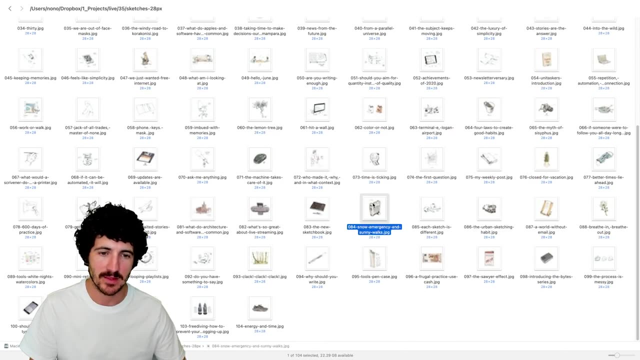 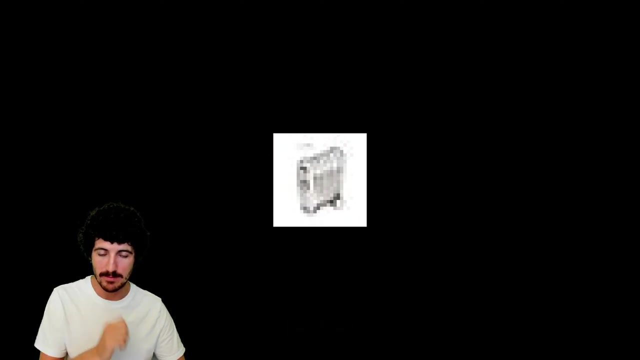 And here we have a collage of all of them, right? So the purpose of having the images down to 28 pixels is to be able to put them into the Keras model and have the training be a bit faster, And uh, yeah, so class things that. uh, what Ricardo is saying is is right. 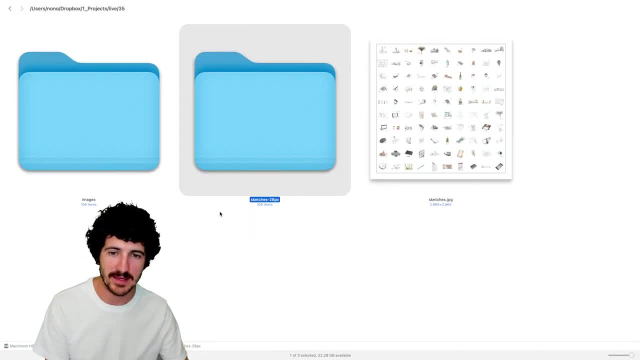 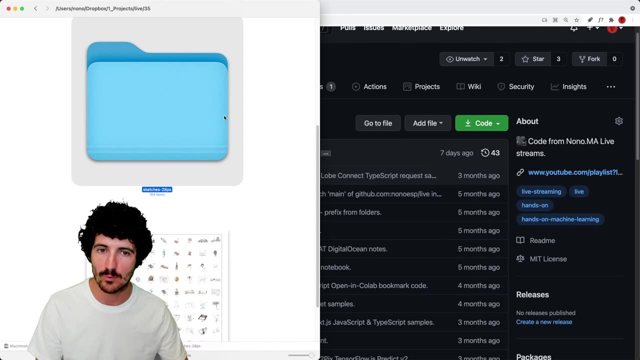 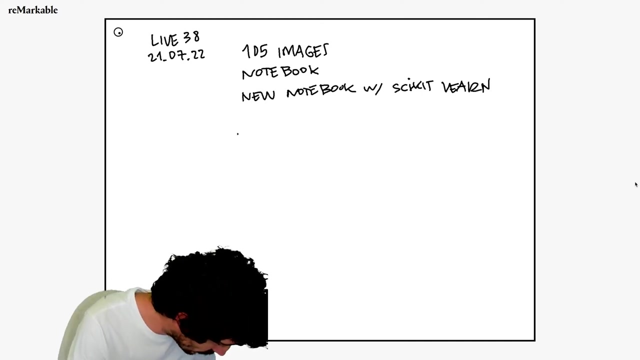 I am not understanding it fully yet, Um, but I will at some point. Um, so we have these data set and this The. this is the data set that we're going to use. Uh, we have to. you know, challenges that we're going to have to face are, um. so let's see. 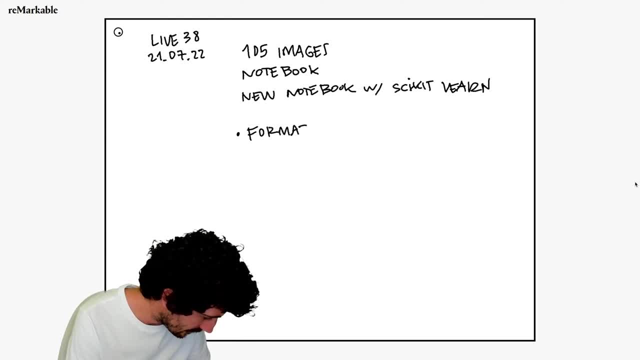 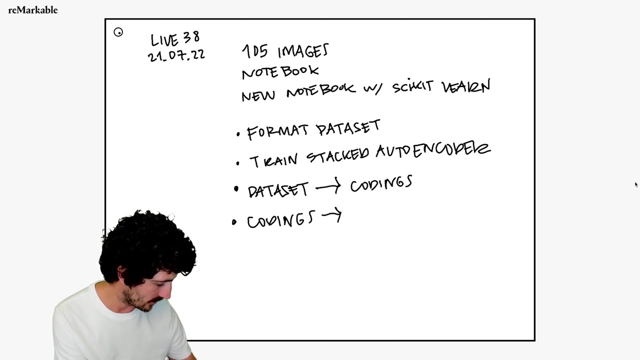 So, format: data set Train, It's that. Oh, so, Um, so we're going to go into the encoder, um data set conversion to codings, and then our codings are going to go into and then, uh, plot them. 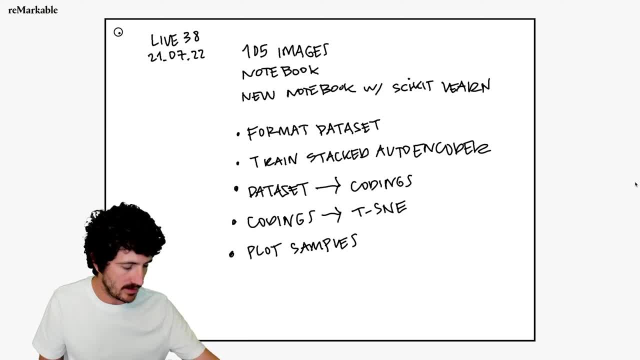 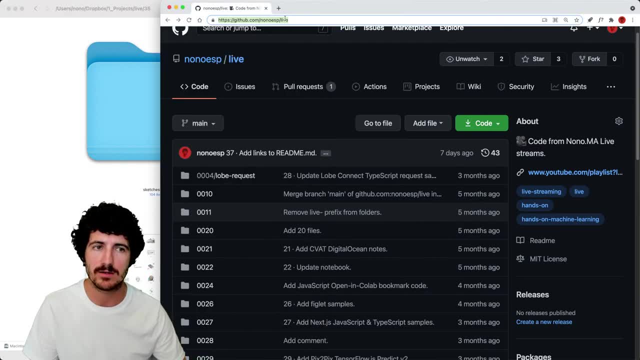 All right, All right, So let's see. let's see how fast we can do this. Okay, So let's see. let's go back to our notebooks. So for this I'm going to open call lab research to googlecom. 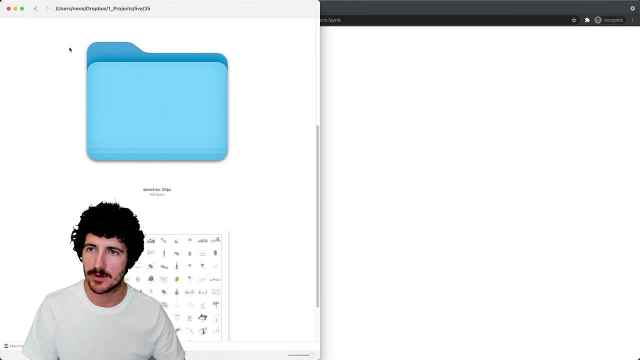 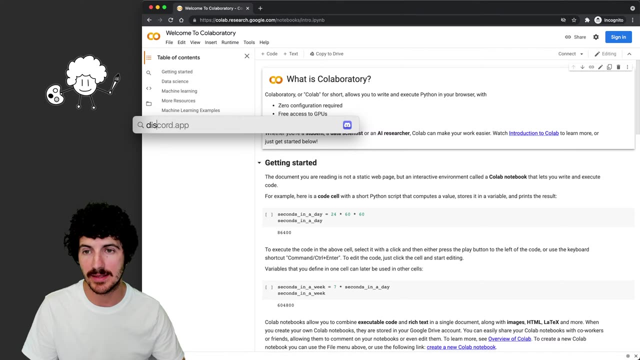 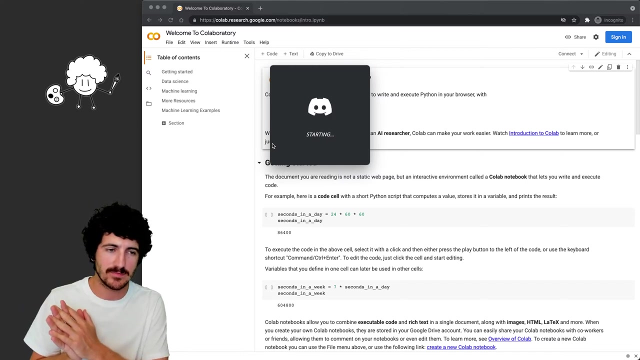 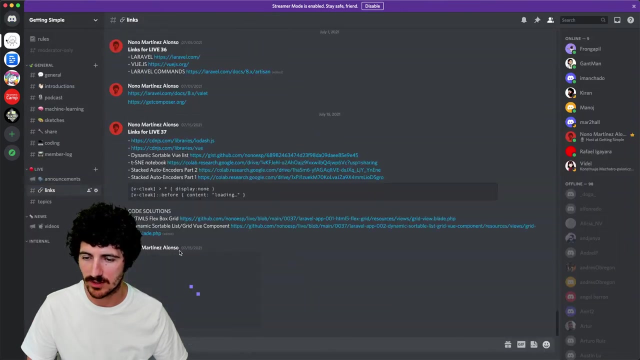 This is the website where we can access the, the um, the notebooks And to to do, I believe, On this court. we have the links for, or last um for the previous Lightroom, So we have the um, the links here, so we can maybe make here uh, links for life 38.. 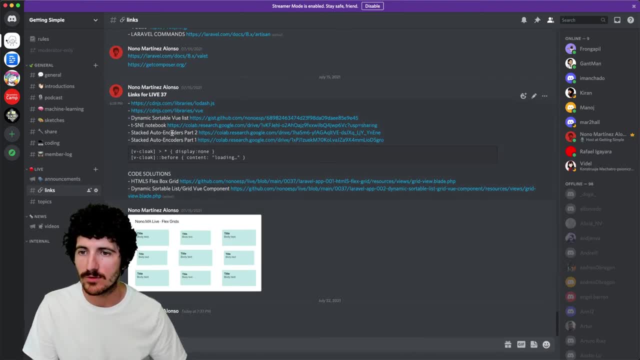 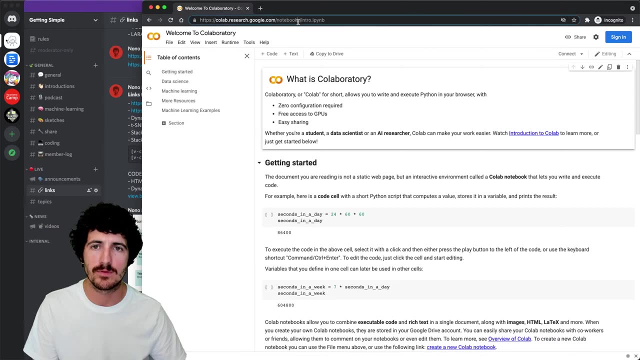 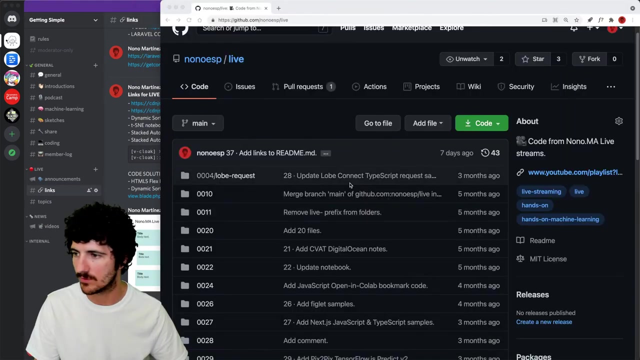 And we'll start adding things here later. So here we have the stack autoencoder part one and part two. Maybe this is part three, I'm not sure- And I'm going to sign in with the account that I created for for the live stream. 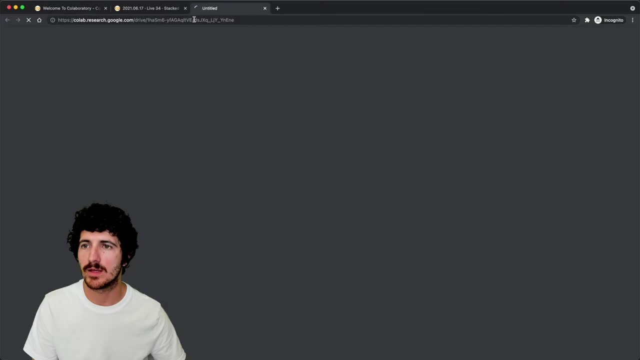 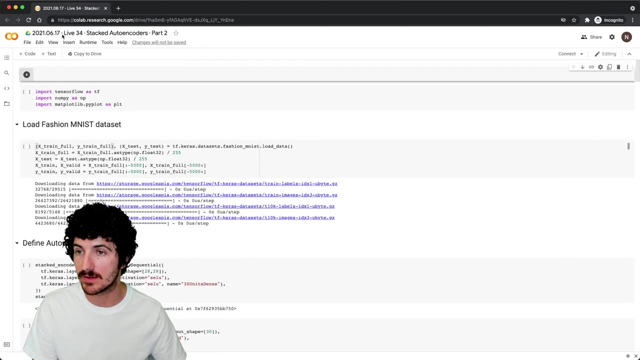 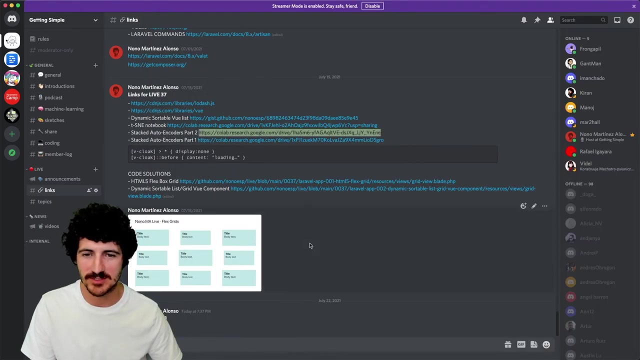 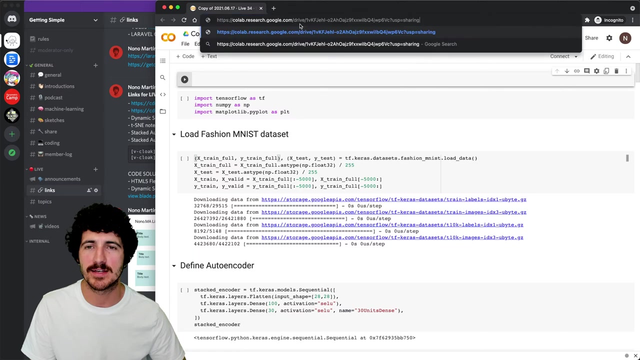 Right. So we got Google call up here and we can now access the stacked out encoders notebook. So this is going to be- Um, I'm going to make a copy, so save a copy in drive. you know, I I be Ricardo. I'd be interested in seeing some of the things that you have been working on. maybe you can share them with us at some point on the network. 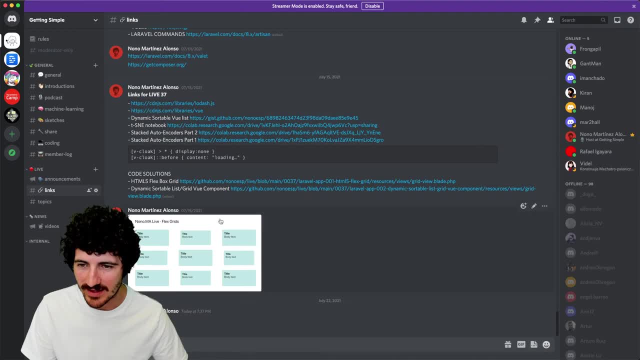 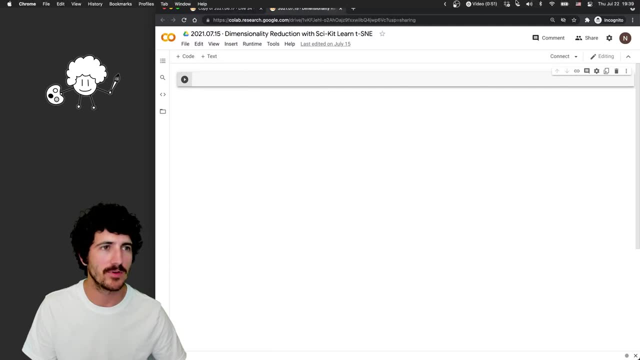 On the live stream or or in some other form. Okay, So, um, all right. So they mentioned the reduction with, uh, psychic learn. We didn't end up doing that last week, So we're going to update this notebook. 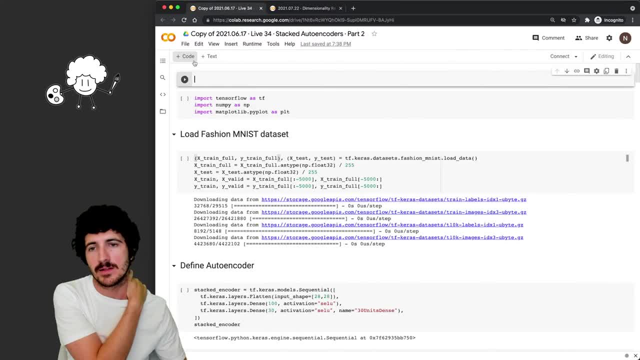 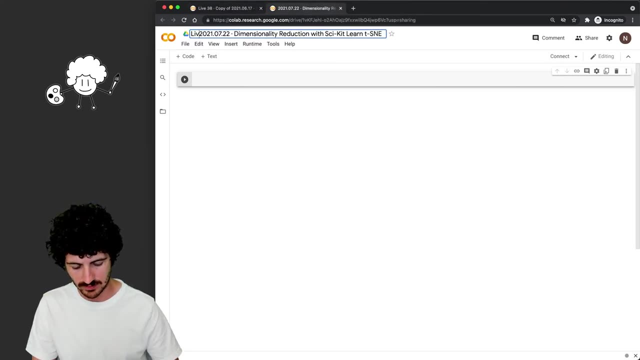 I think this is my notebook and? um. okay, so here we have the copy of the previous notebook that we might not need. Um, this is live 38 and I'm going to put the same here. So live 38. Okay. 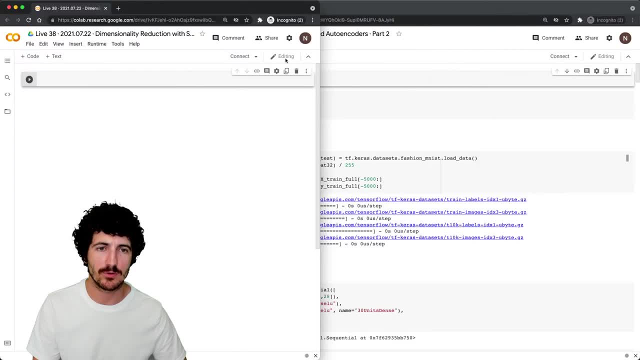 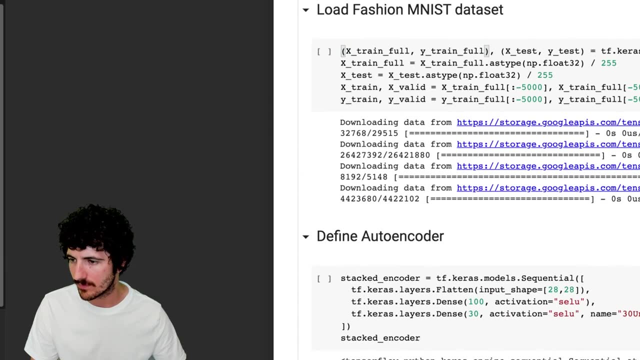 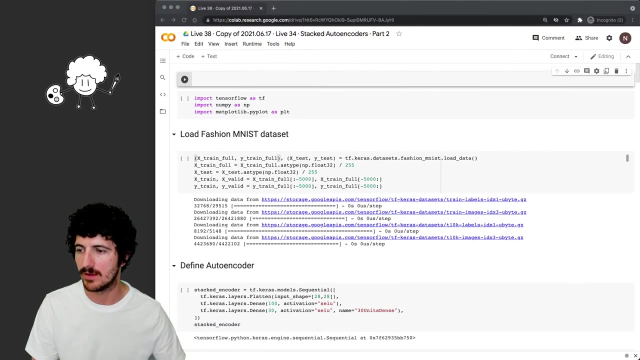 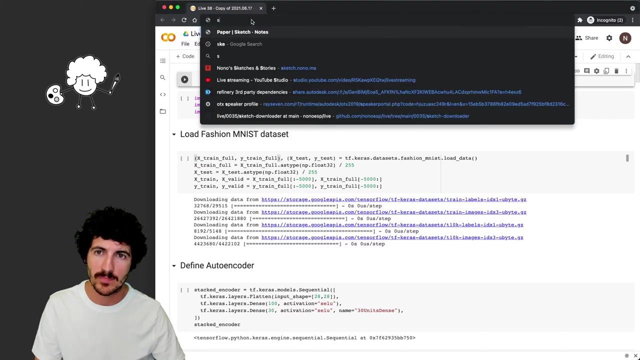 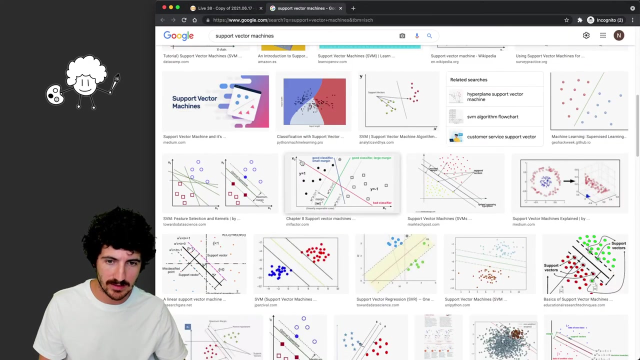 So, now that we have this, let's see what parts of the code we need from the previous notebook. So, Okay, Okay, Oh, okay, Yeah. So I think, Ricardo, I think what you're referring to, um, what you might be referring to, and I'm not too sure, right? 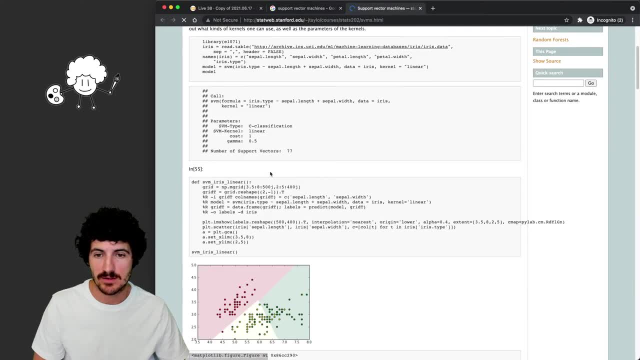 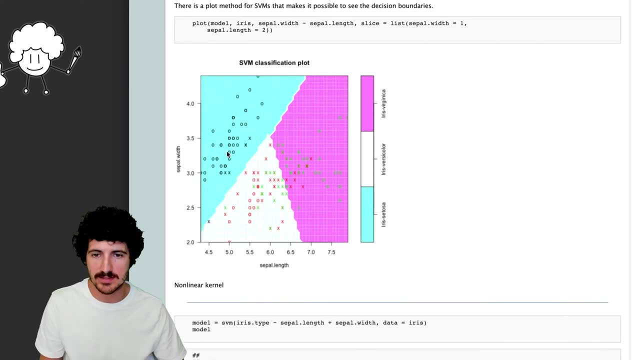 When you have data samples, some algorithms like support vector machines, for example, you have different clusters of data and, uh, these type of algorithms. So this is something that we're learning from. this is where you can actually um to say something like: okay, we, we, we need to, we need to separate this, this algorithm. 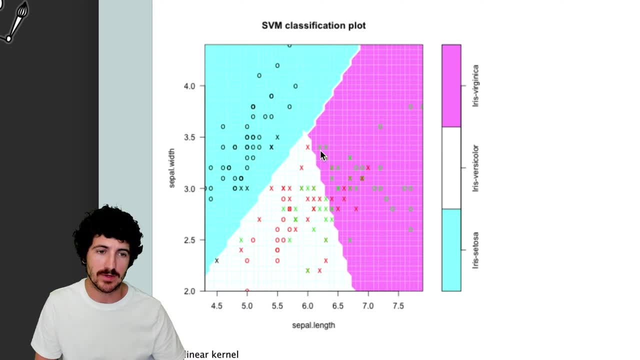 So if you, if you have a good cluster and then you have an algorithm, might, uh, automatically or in a unsupervised way- unsupervised way, as you were saying- My um separate your data into different clusters? 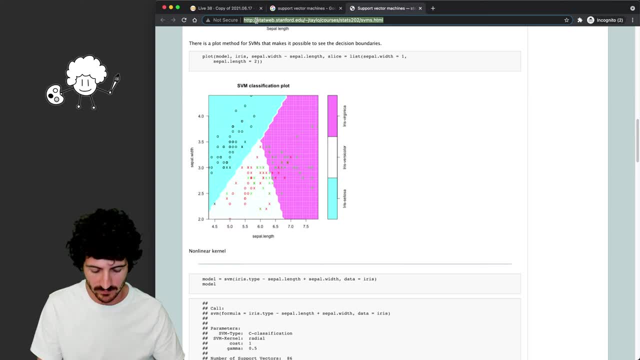 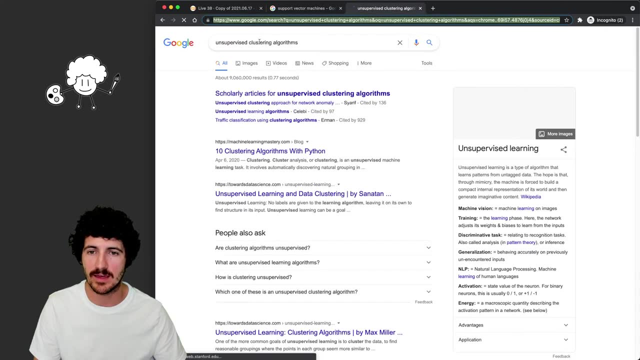 Right, So without you having to specify them. So this is like on Super Vice clustering algorithms. It's kind of like K, K and an end. Okay, Yeah, Okay Okay, Thank you, Thanks, Thank you, Thanks, Thanks. 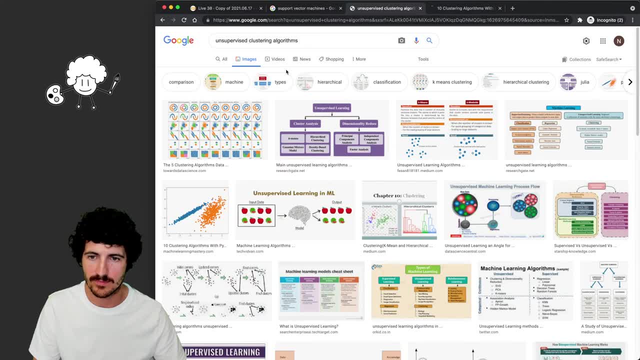 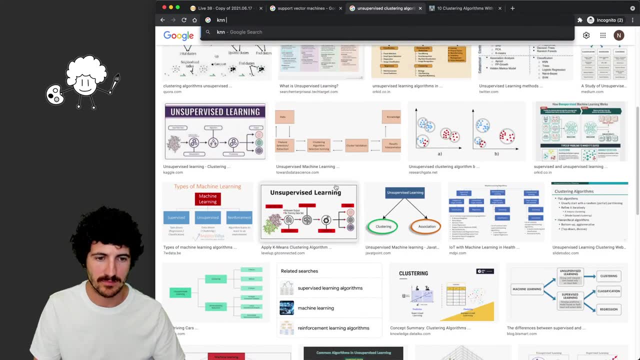 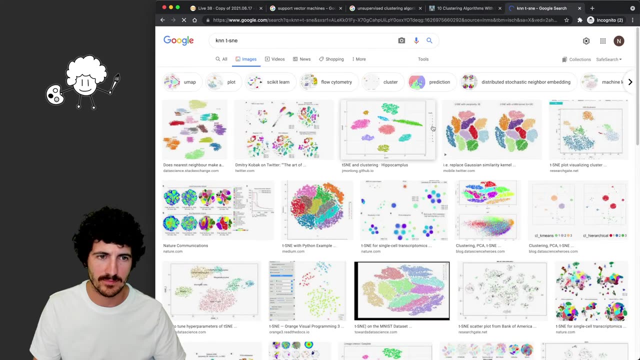 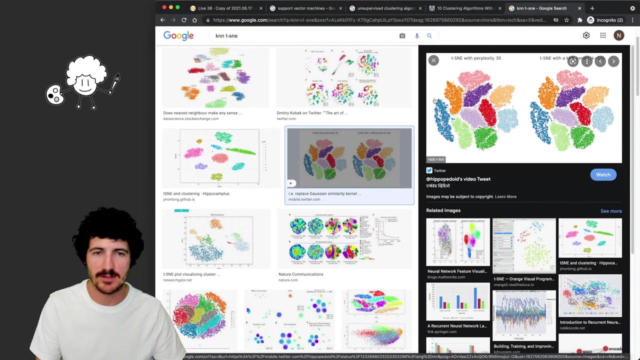 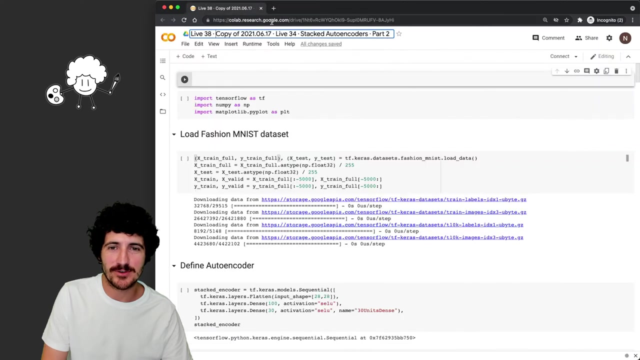 Yeah, Thanks to the two of you, It was a fun time. Thank you, Okay, Okay, Okay. But yeah, let's see, These are super interesting questions and comments, by the way. All right, let's try to continue here. 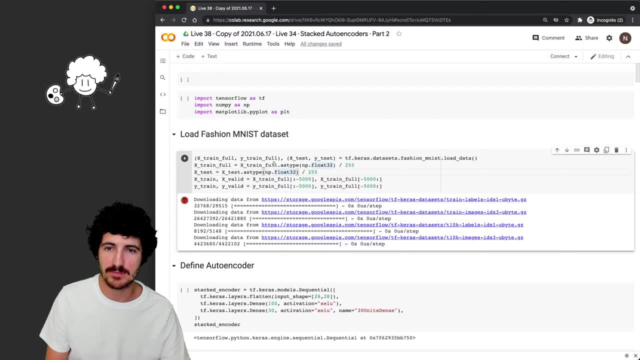 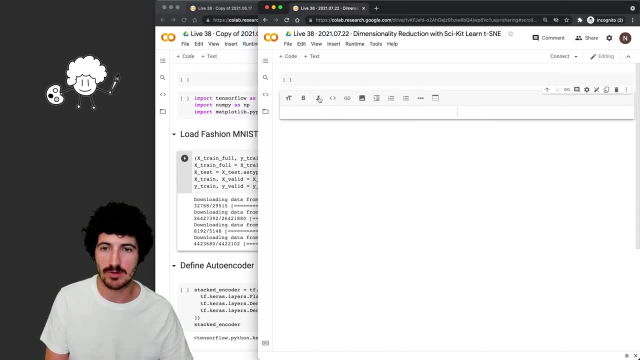 The first thing that we have is that we have the fashion MNIST dataset, and I want to do this with our own data, right? So what I'm going to do first is I'm going to add a text block here. I'm going to say: load costume dataset, and this is like: images are 28 by 28 pixels. 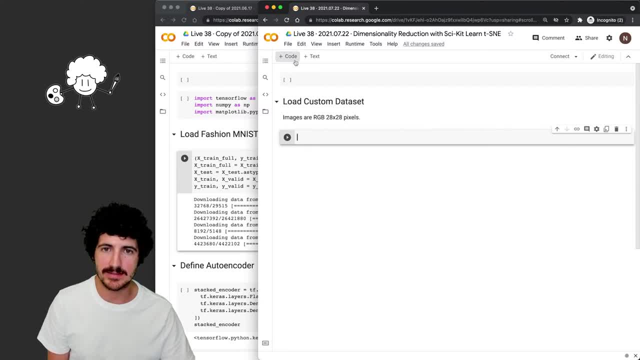 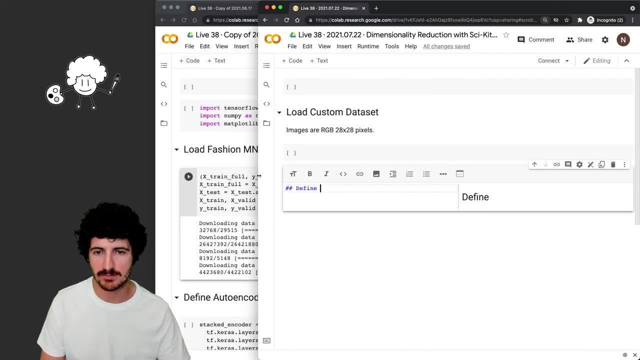 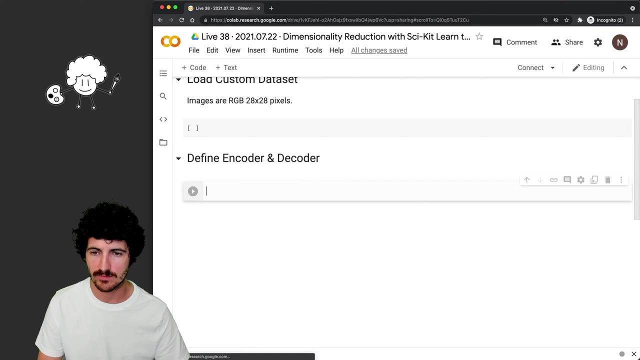 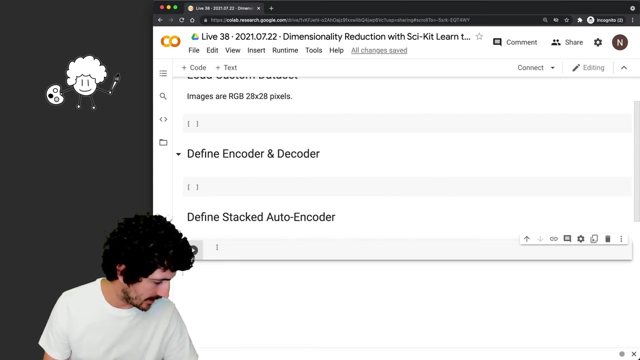 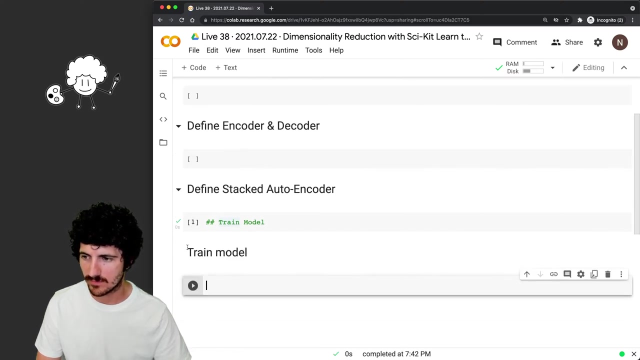 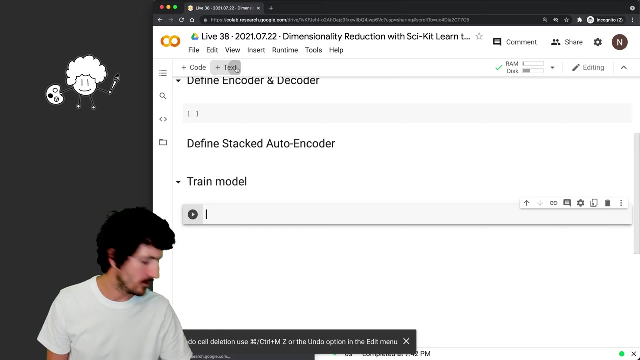 RGB. Okay, Uh, then the second thing that I said: they say we need to define our- uh- maybe let's make this bigger- Define encoder and decoder. Define a stack out to coder, Then um, train model and uh, later would have to. 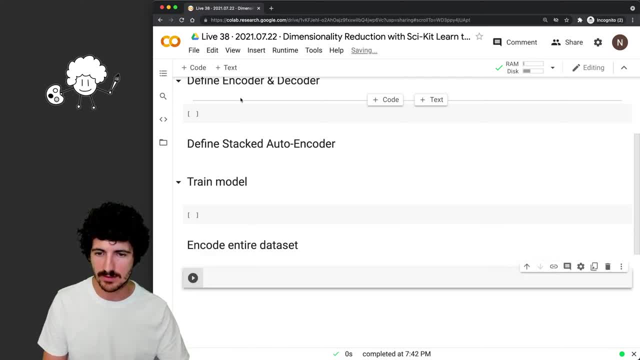 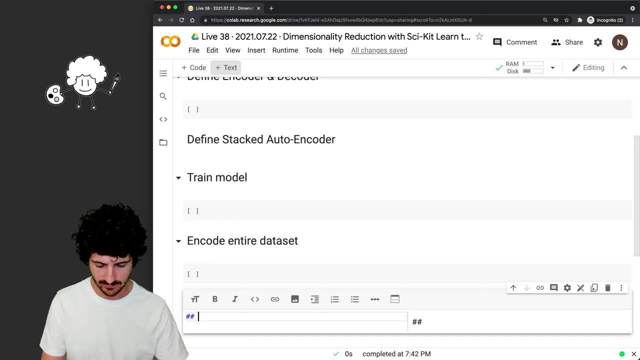 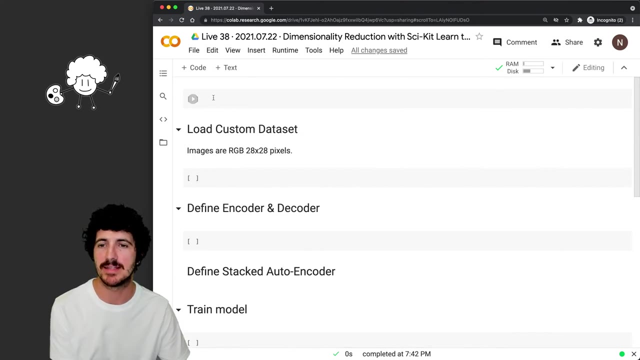 encode, Okay, That data set, And then we'll have to Well, the reduction with this, and you know, these categories might change, but at least we have placeholders here, All right. So first thing we're going to do is I'm going to import TensorFlow as 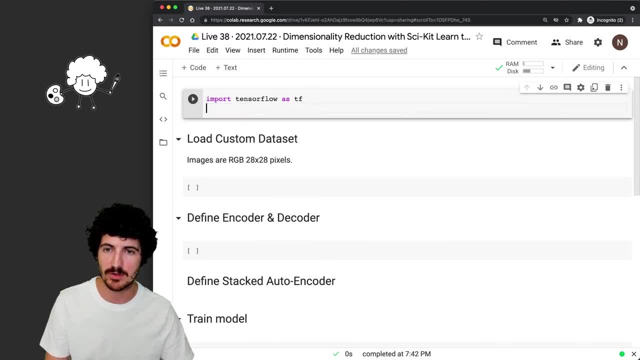 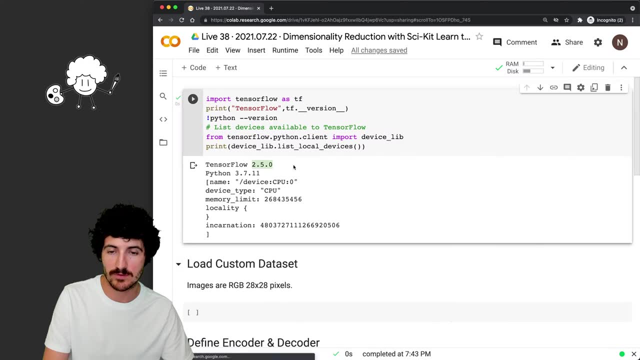 TF and I'm going to import. um well, I'm going to leave scikit-learn for later. Um uh, let's take a look at what we have. So we have TensorFlow 2.5.0.. We have Python 3.7.. 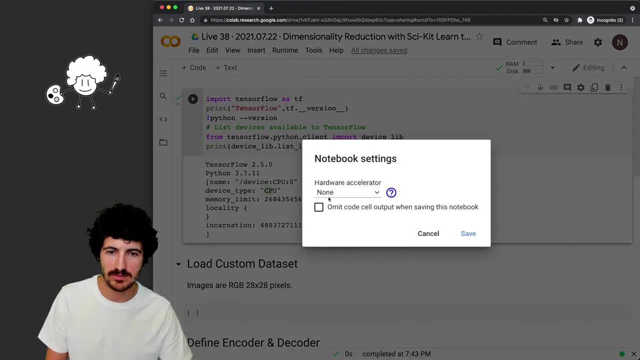 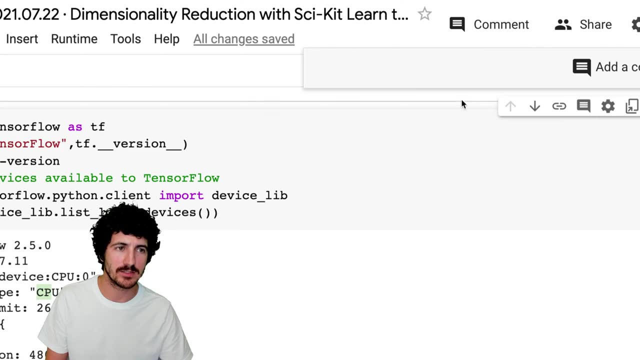 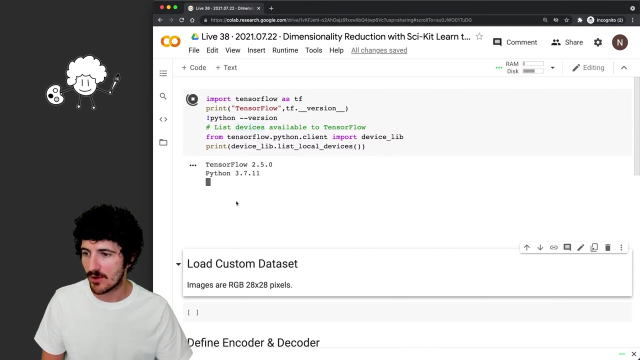 We do have a CPU and we don't have any GPUs. We can select the GPU here to make our notebook faster. So this is now going to allocate it for you and initialize a new um runtime. So now we run this again, we're going to have the same version of TensorFlow Python, but now hope. 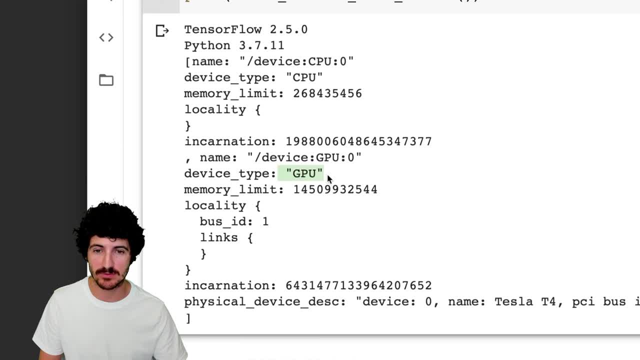 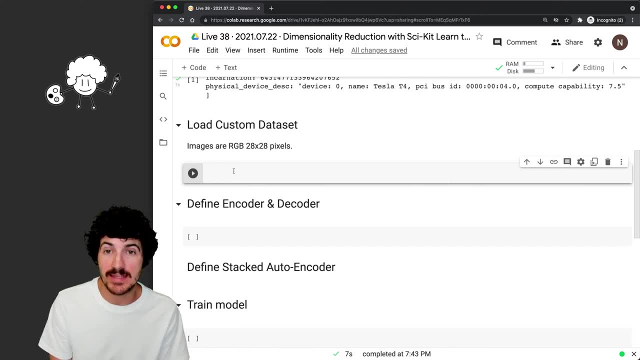 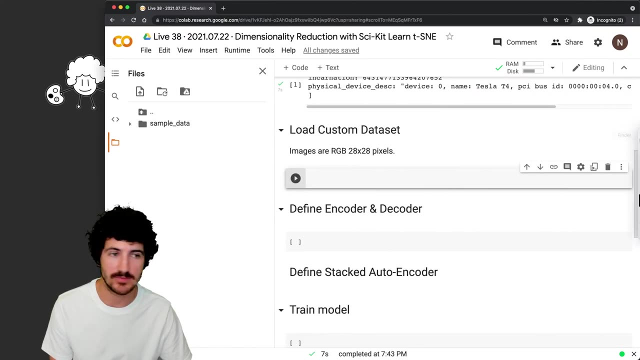 We will have a GPU. All right, So now we have a GPU. device is a Tesla T4.. Okay, Great. So where do we have our data set? How are we going to put our data set here? And maybe the easiest is that we just drag and drop, because this is a really small data set. 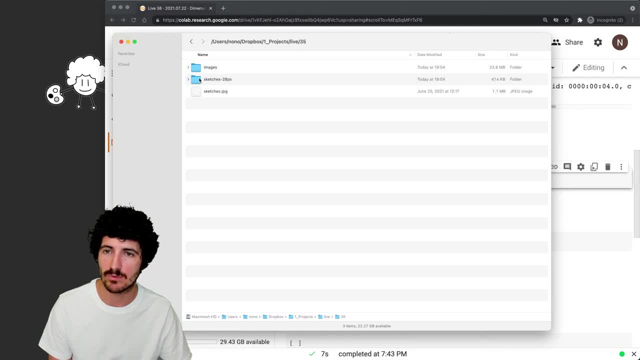 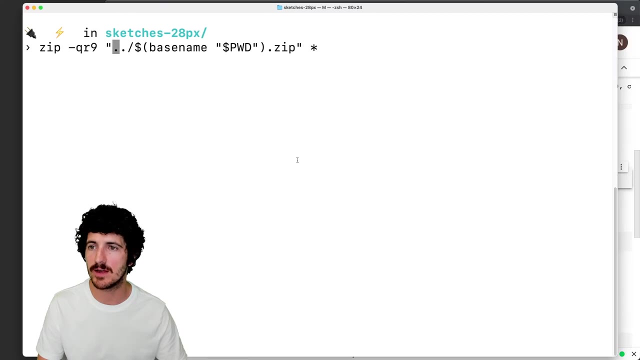 The problem is that this might require that we do that every single time that we want to do this, but I'm going to go with that route. Okay For now. So I'm going to go into this sketches folder. I'm going to use this script to see my file. 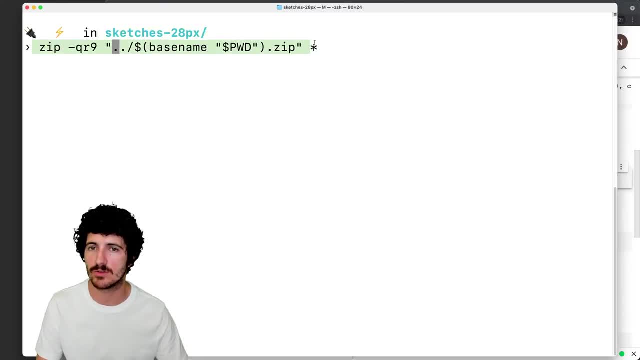 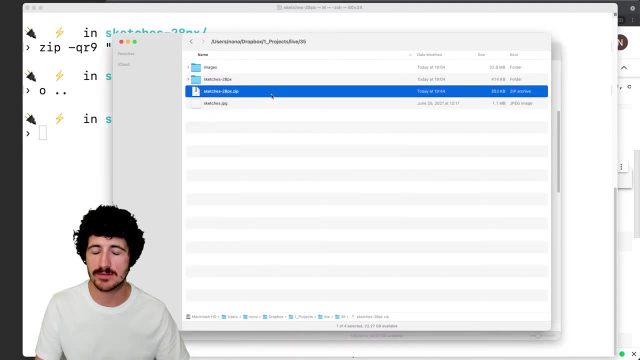 So it's just, uh, I go into the folder and I just call this, which is just zipping the file with the same name that, um the folder has. So maybe we just call it sketches, and this is 352 KBs. 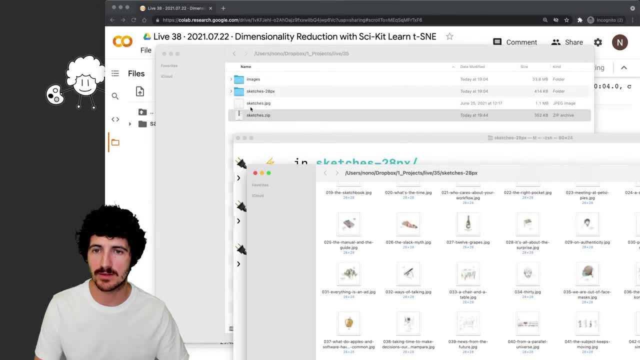 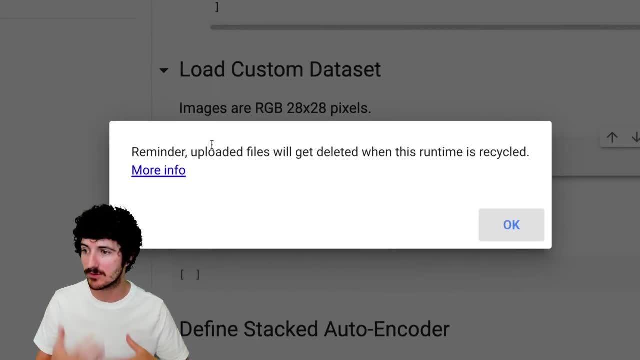 So this is super small. So we're going to simply Drag and drop that into our notebook. a reminder that files will get deleted when the runtime is recycled. So if you close your notebook, go away and then come back, the data there is not going to be there. 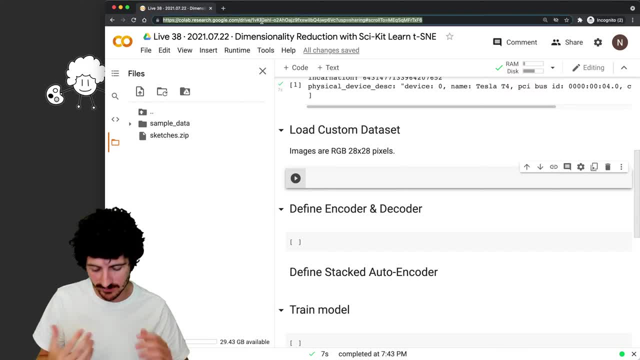 So there are ways in which you can download those files or um, maybe download them from other source or upload them somewhere. So if you look for, I think- um, I don't know if this is going to show up, Yeah, 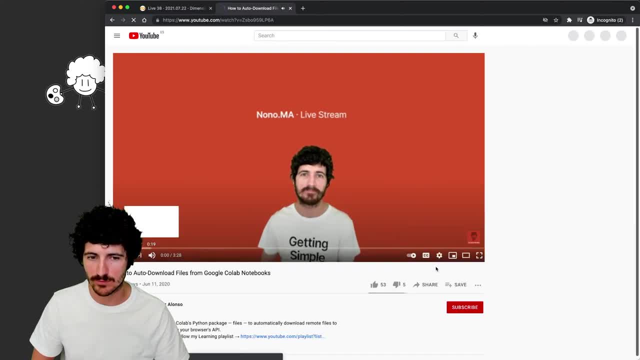 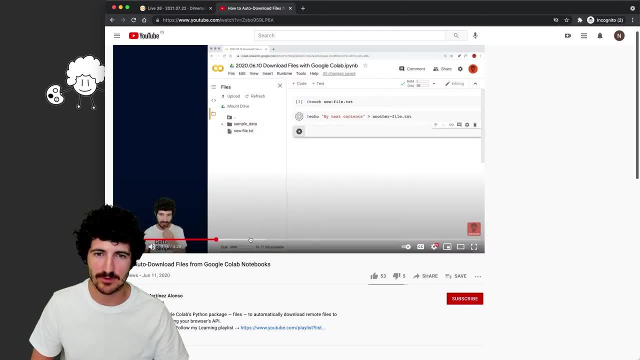 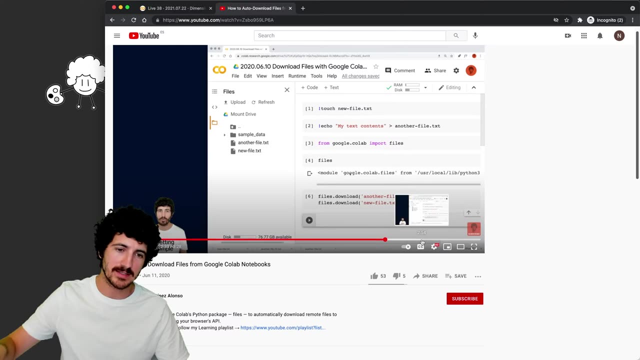 So I have a video on how to- oh, this is old man. I have a video here on how to auto download um files from from Google cold up, And this is something that I really liked, because that way you can run your notebook and then your file send up on your downloads folder. 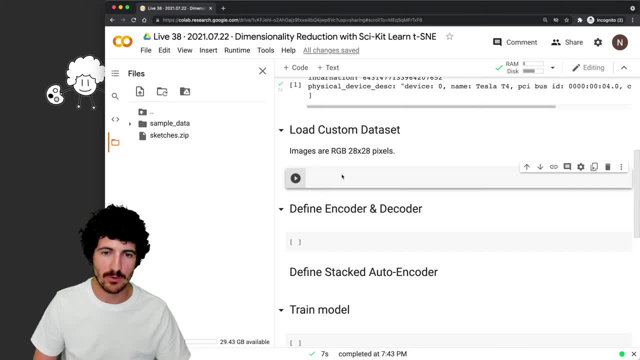 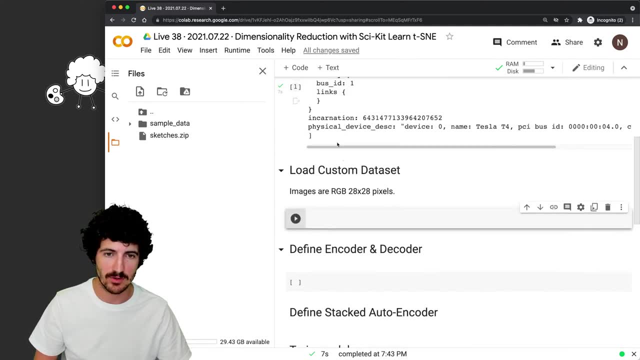 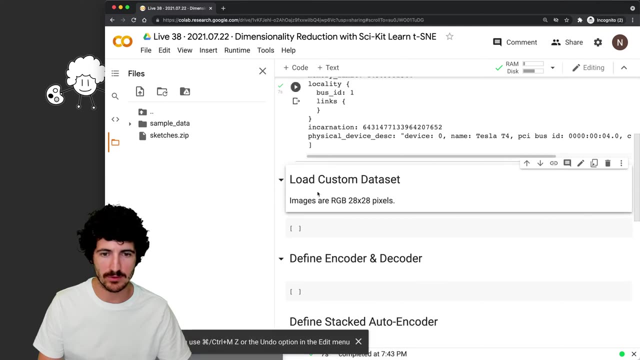 And you don't have to worry about that limitation. All right, So now we have this here and I guess we could And see them. So, uh, load custom data set So we're going to do some preparation here, or maybe load custom data so we can do here. 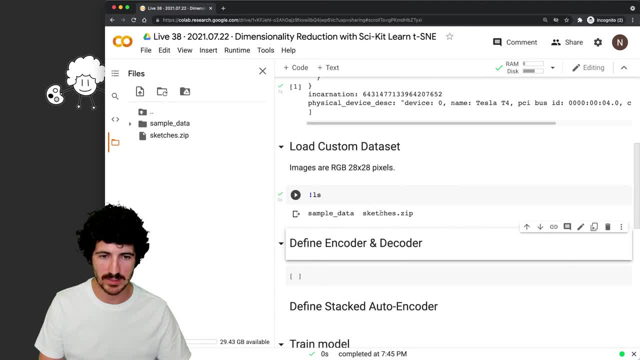 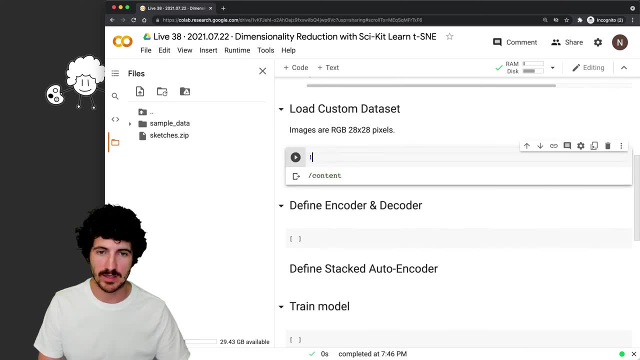 So we can, let's see what folder we're at. So we were on the folder in. we're in the content folder, which is this one here, So we can do and see sketches of SIP, Let's see. let's see what happens here. 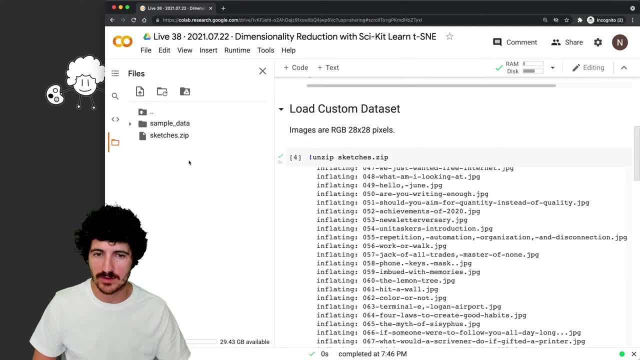 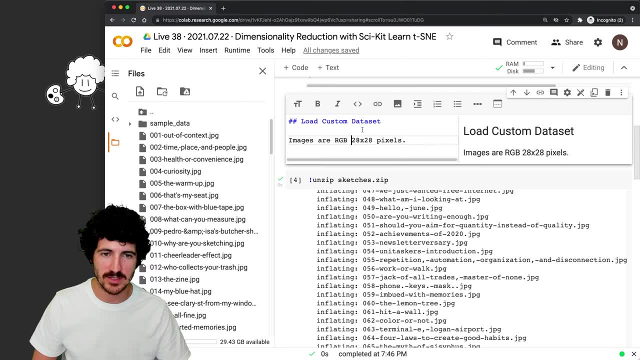 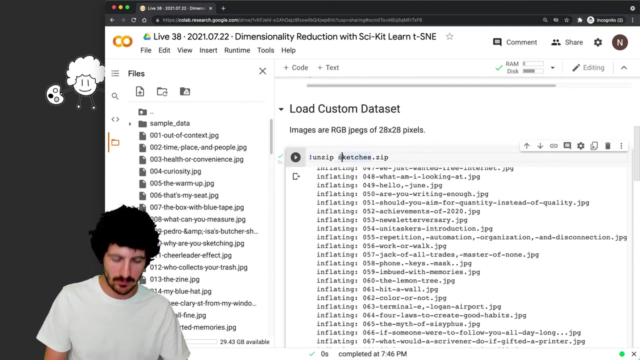 So I I think all this- Okay, This is my goal- to this folder, which is probably not the best, but yeah, I mean we, we have them all here and they're, they're JPEGs- Cool, If we put here the queue, uh, these processes silent so we don't see anything. 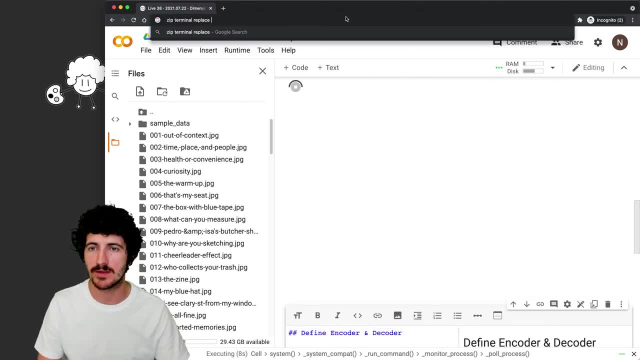 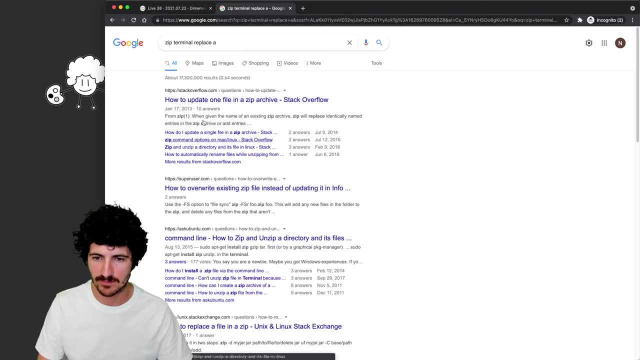 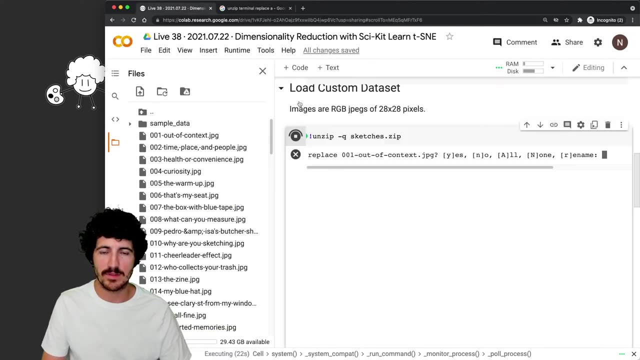 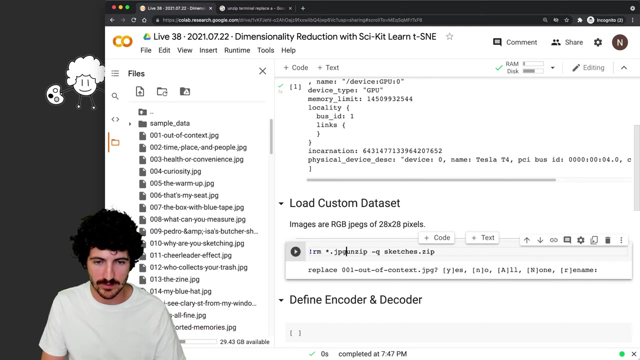 Except for that, um save terminal replace Yes. Well, one thing, one thing that we can do to avoid these sort of questions is we can just say: remove all the JPEGs in this folder and then unzip. that way, Everything gets removed. 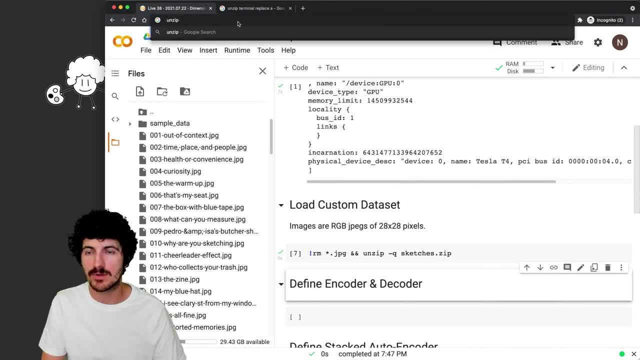 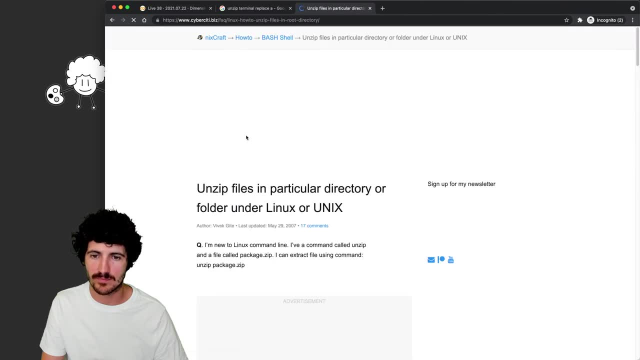 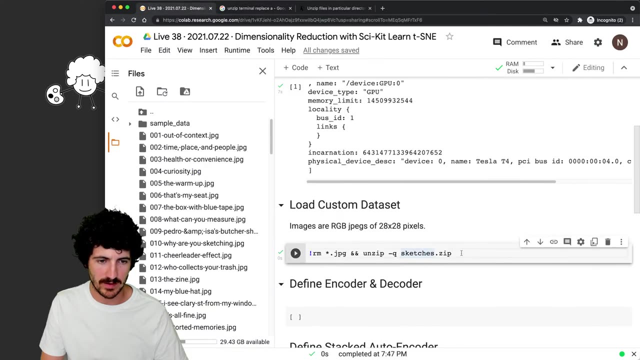 And then see again some seed terminal and SIP in folder. Right, So we can specify here to unzip on sketches. that way we unzip to a directory instead of to the main folder. All right, Okay, Okay, Okay, Okay Okay. 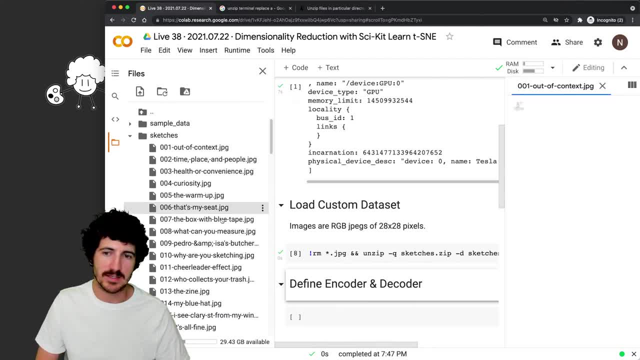 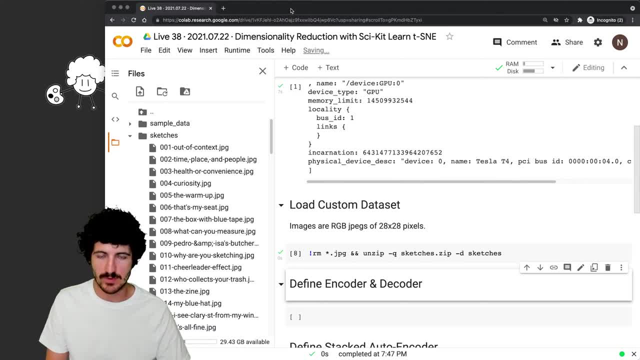 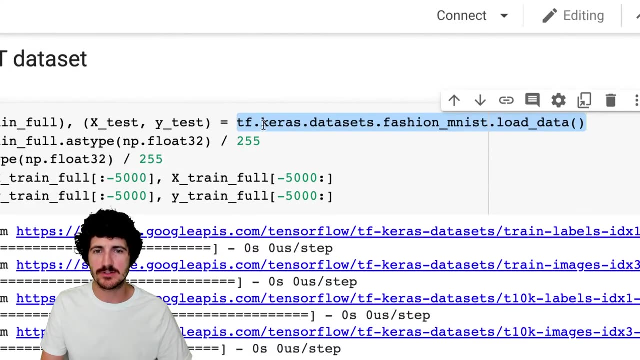 Now we need to see how to load that in the same data format that we had our data set on the the previous live stream. So these notebook here you can see we have we're downloading With this function here. So TF, dock carrots, dot data sets, fashion M&Ms- load data. 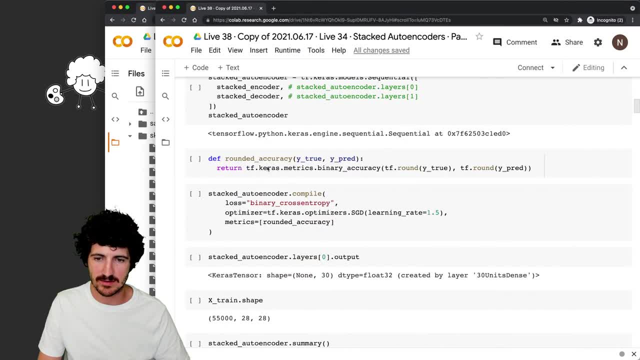 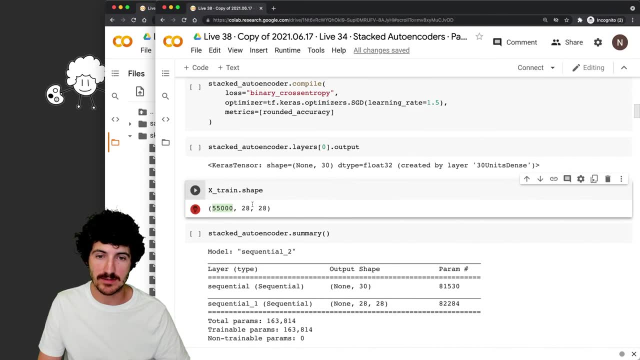 This gives us um data in a really specific format, So in this format here, so at 28 by 28 pixels, and they're 55,000.. So we want to get our data in the same format, but in um having less, less of. 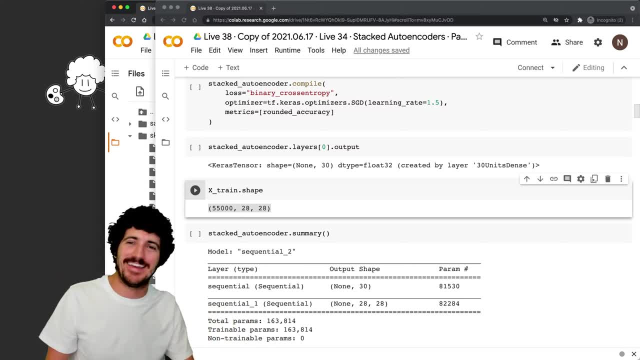 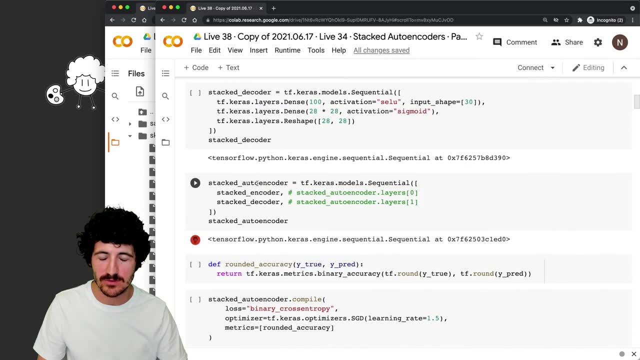 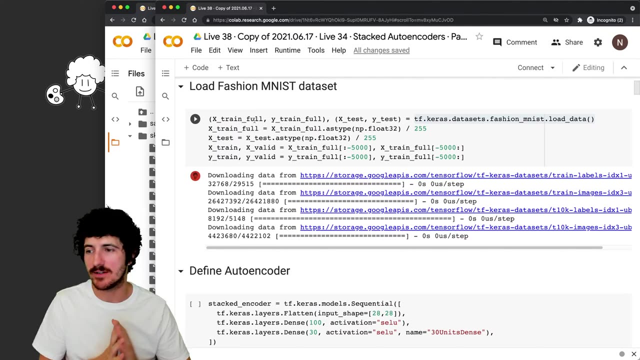 them and hello bear, uh. nice to see familiar faces, and what we have here is automatic, so we have uh. right now is: um, we only have 105 samples, which is going to overfeed a lot, and this is not something that I had thought of. 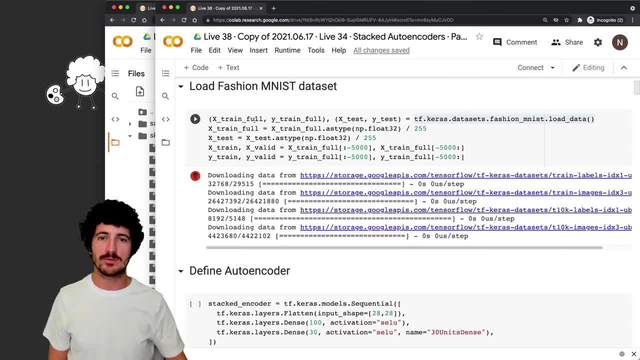 but at least we can set up this notebook and then we'll we'll use it better, So we will load all of our data. We have extreme full white rainfall And there's the test and the test. So let's just debug here the data. 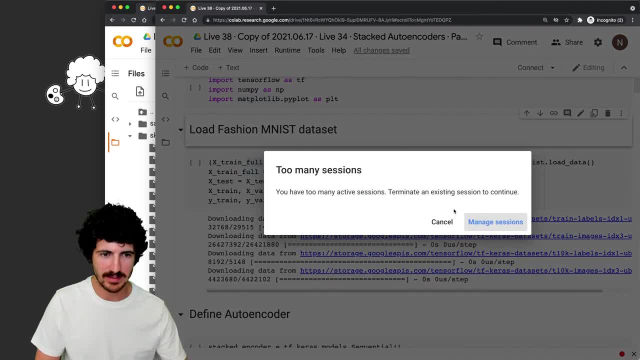 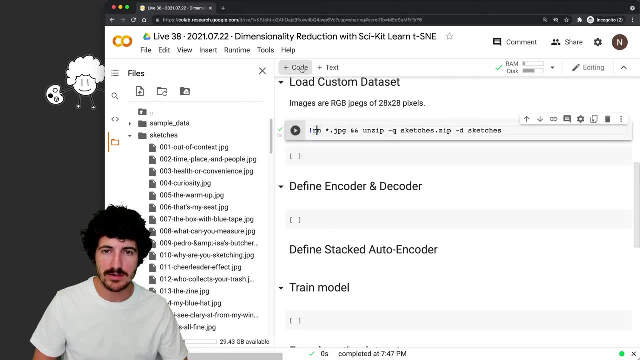 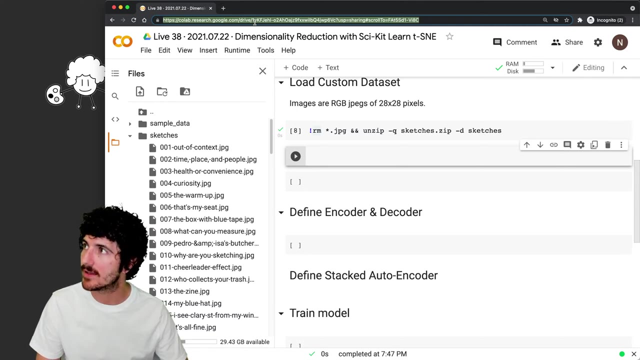 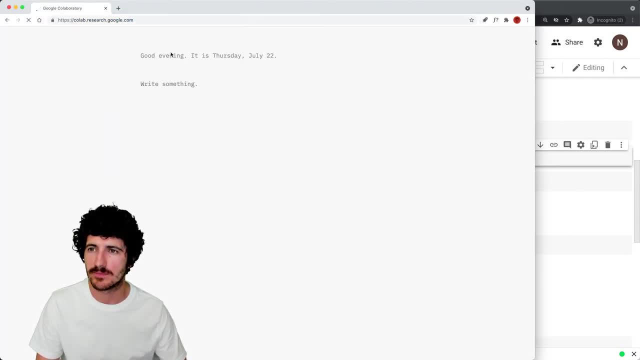 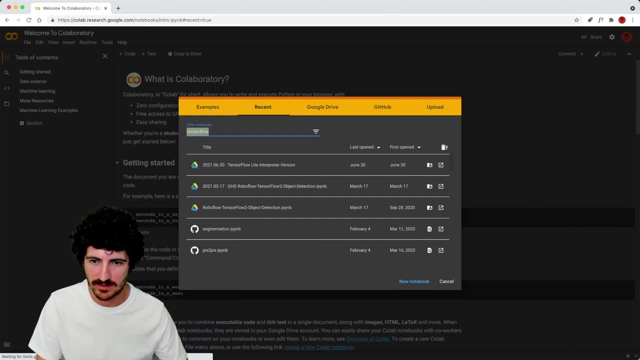 Let's see, Okay, Okay. So here, here's my data, Here's my data. Here's my data and I've got a bit of a bit of an example of how long this is going to take. So I'm going to just go ahead and click this and we'll do an example of this. 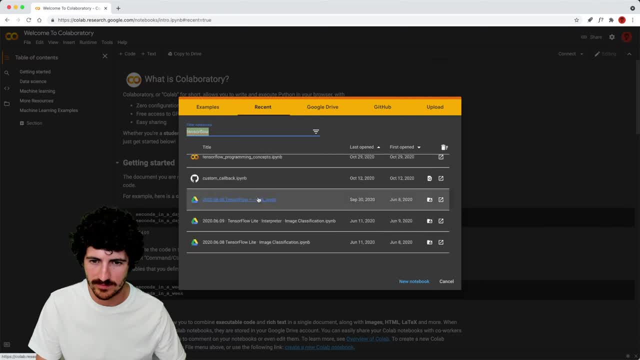 and if we could see this, it should take like 12 minutes. So I've got myself a couple of things right here. So we've got my data here. So this is my data. I'm going to drag it back out of my data for a second. 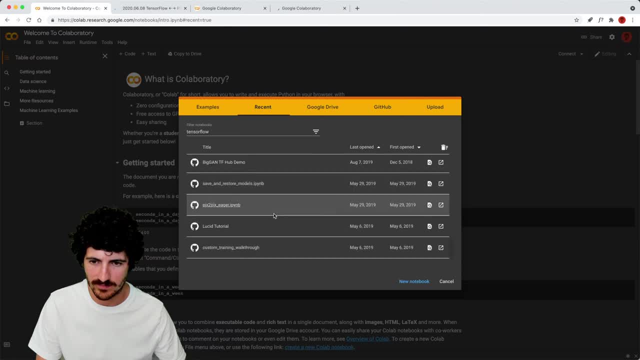 And you guys can see that I'm really, really happy with it. So this is just a jump here and there. So here goes the data. This is the data. If you see the data, I know I have the data here. 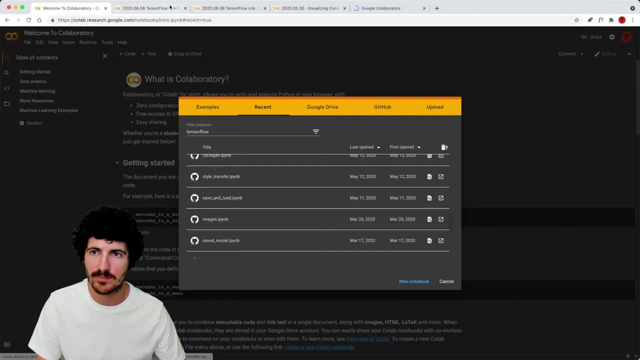 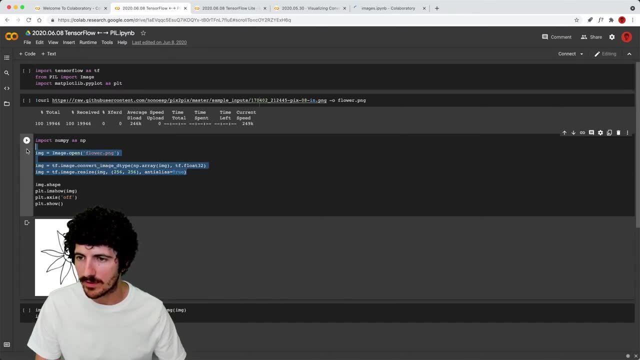 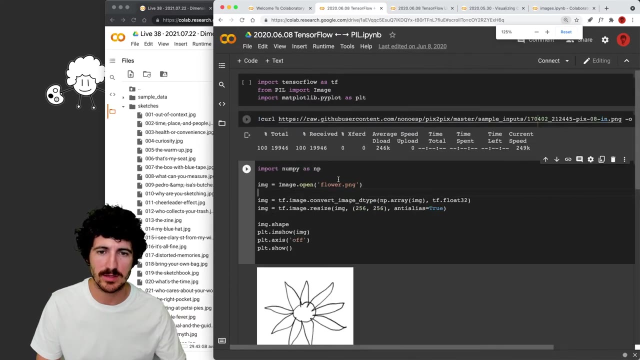 And now I'm going to go back to the sort: Um, well, this is one way, but I think there should be better ways. So we just load the. what I'm showing here is, uh, loading the images with bill, but I want to load them directly with denser flow. 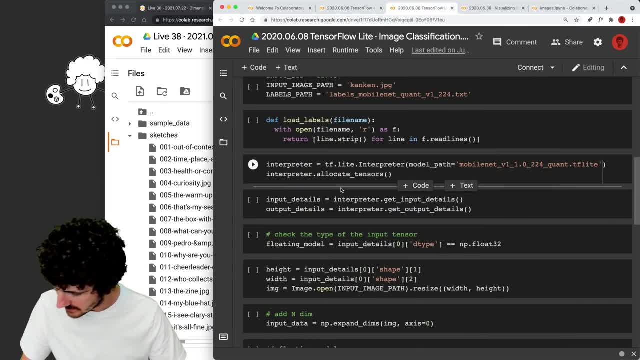 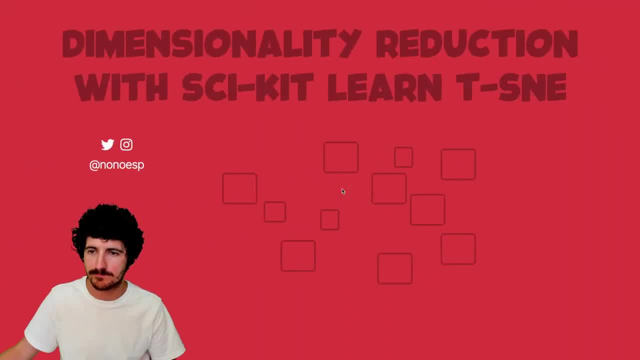 I don't want to load them with um, with bill. Uh, let me see, actually, let me just take a look at the book Just just to see if, um, if, there's something useful here that we could um. 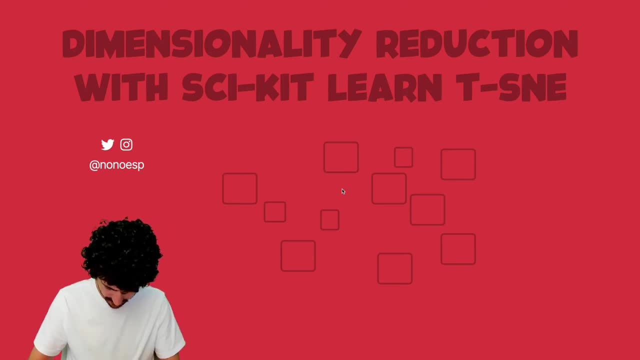 that we could use. Okay, K means. there's an algorithm here that is doing K means and actually seems to be similar to what we mentioned before. Class says: I want to know how to know how many comp to the layers should we? 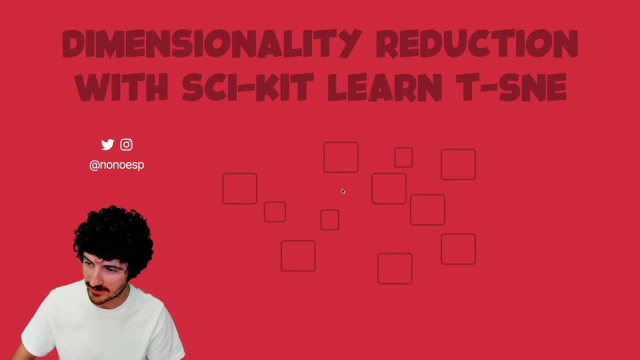 See Set without parameter. hyper-parameter optimization. That's a good question. I'm also trying to learn that. that's like neural network architecture, right, Like to try to identify. it really depends on the task you're trying to do And I'm no super expert. 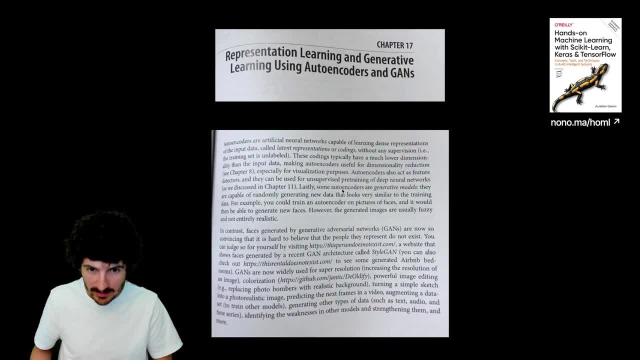 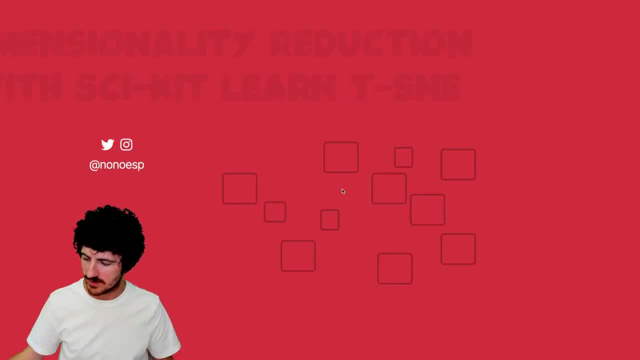 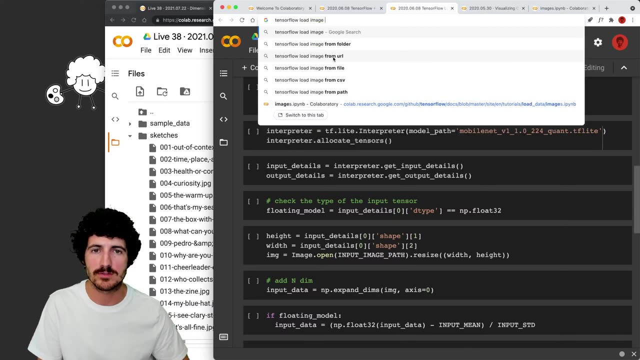 Let me check Here. I'm just trying to see if there's like, um, Oh, if there's like a section where we could uh see those things. but yeah, that might take more time, All right. So let's say here: uh, there's your flow load image. 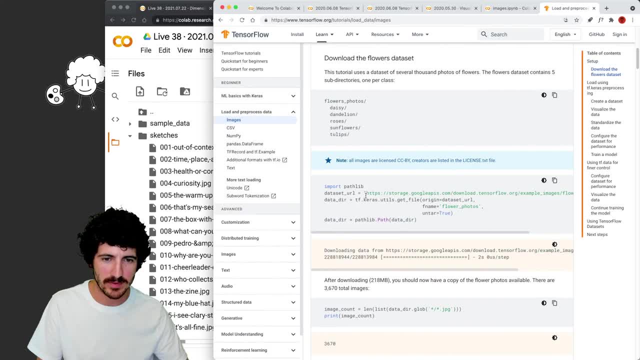 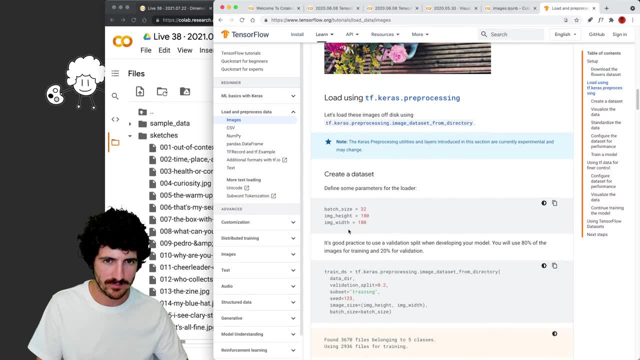 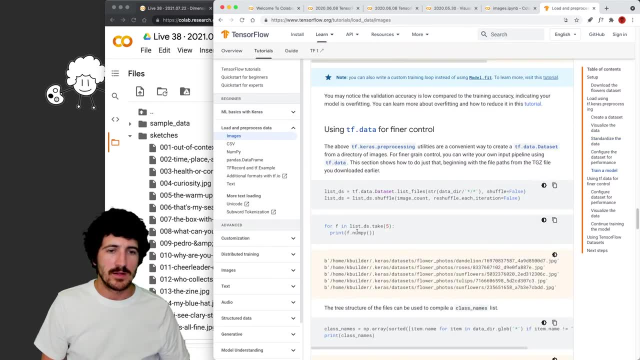 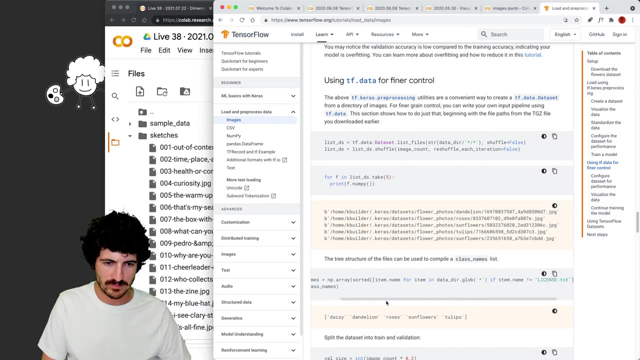 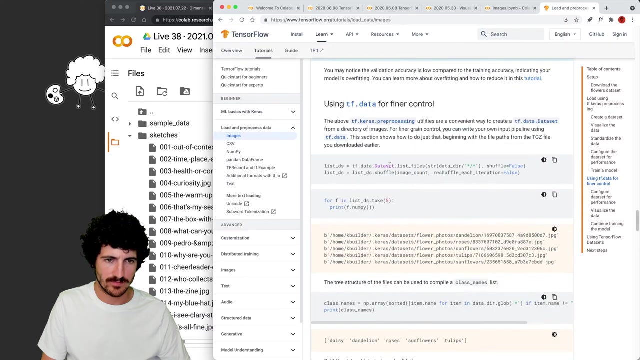 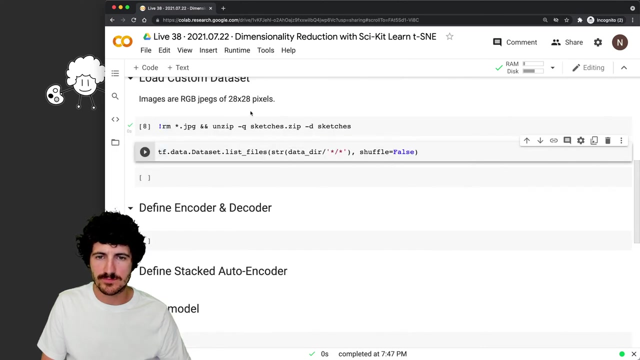 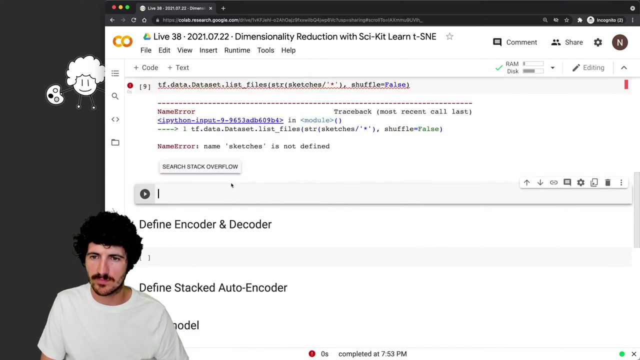 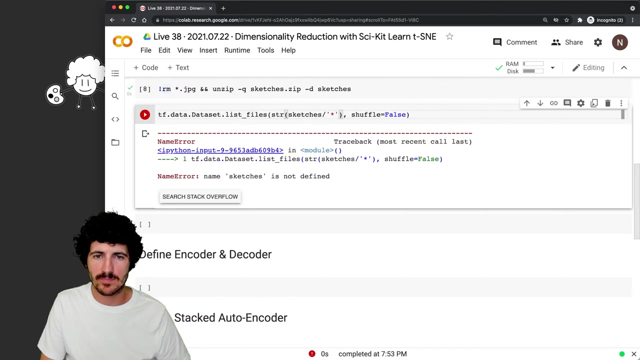 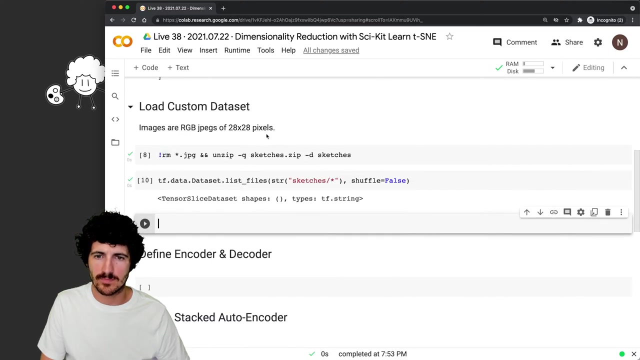 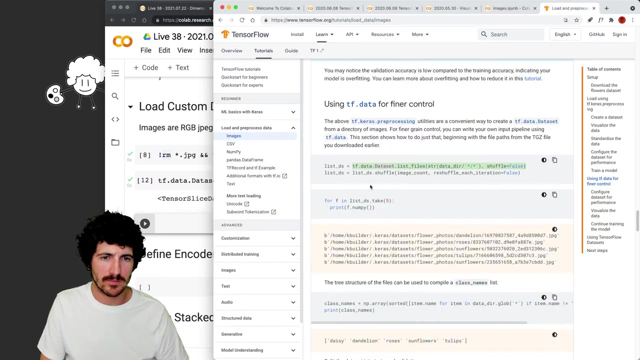 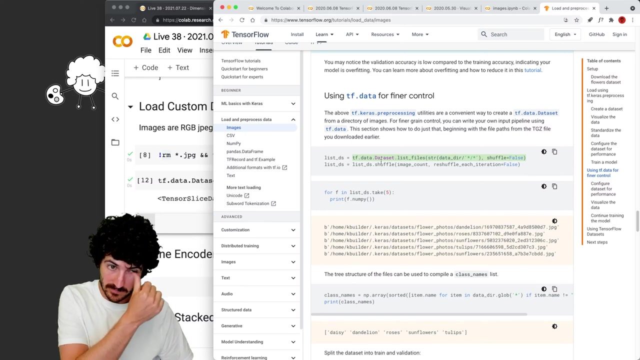 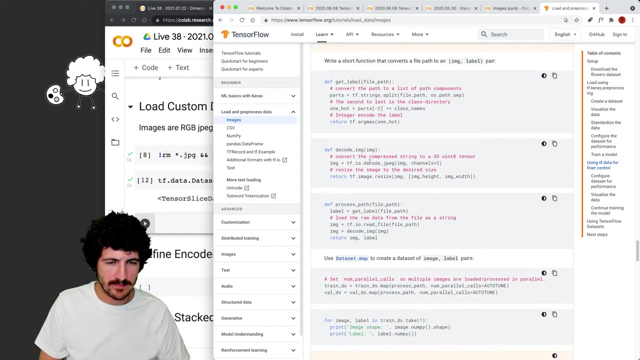 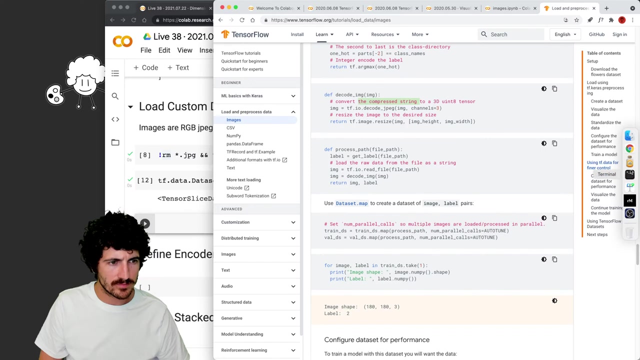 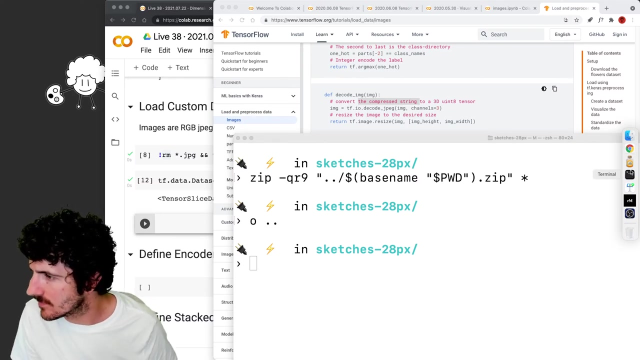 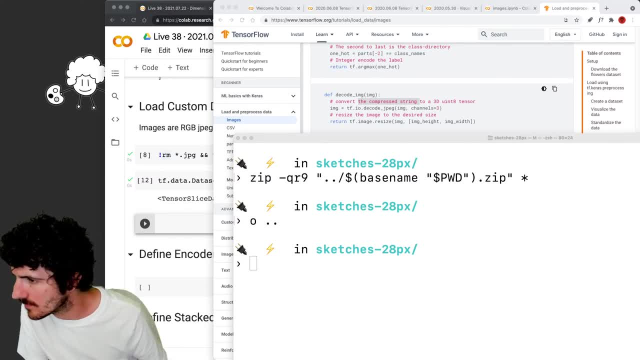 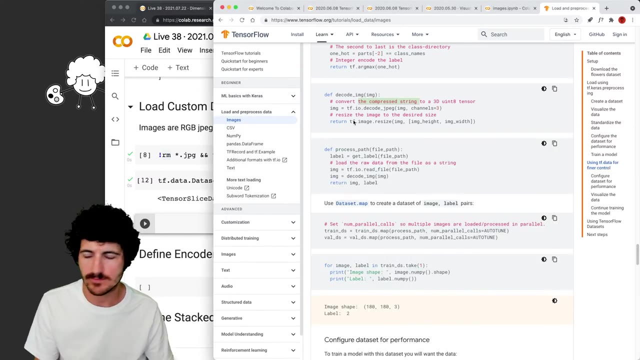 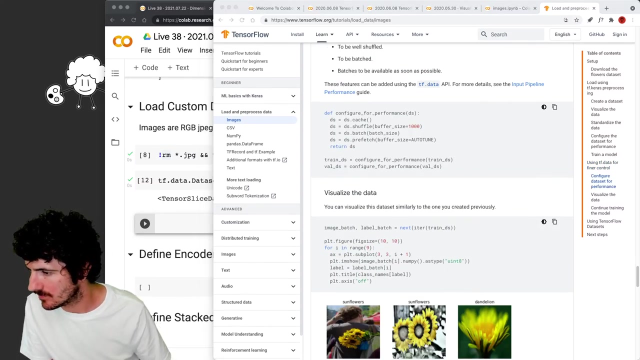 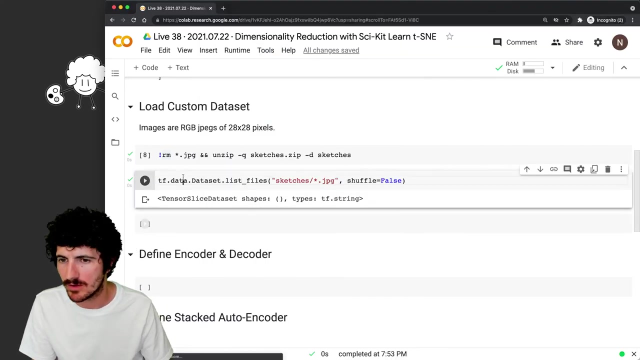 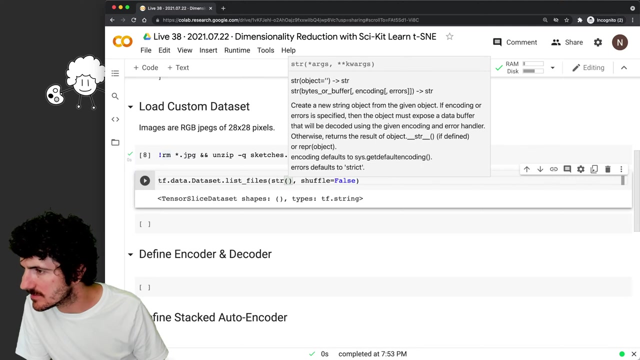 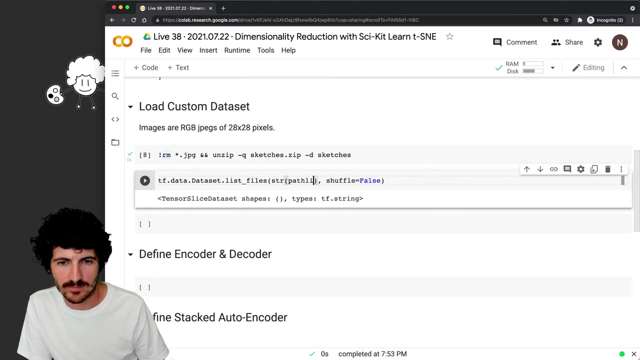 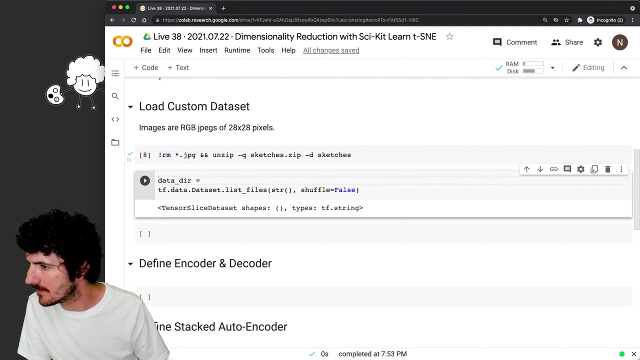 All right, Thank you. Okay, let's try this one here. So dataset, list files, string Data there. So data there. Where is data there? All right, So let's take a look here, So just to see if this works. 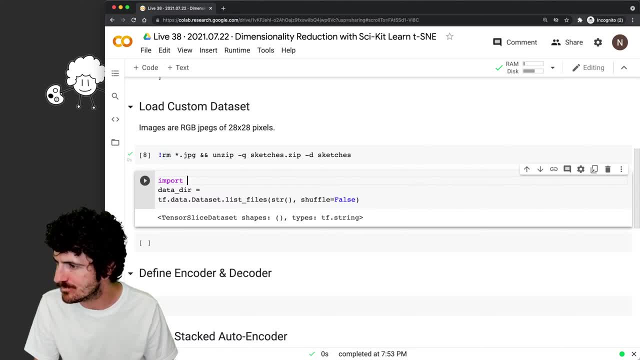 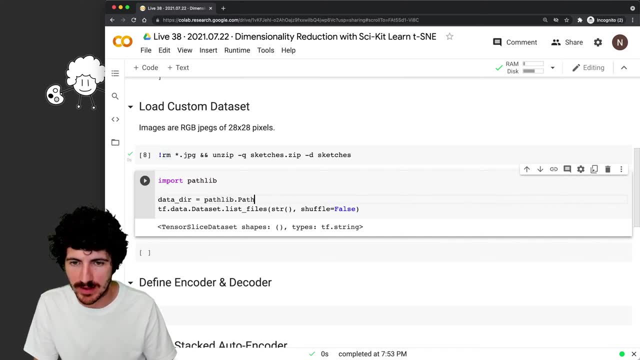 So I'm going to import pathlib and I'm going to call pathlib path sketches, and then here we're going to do data there, And, And then our pattern here is going to be: um, uh, just everything here with JPEG. 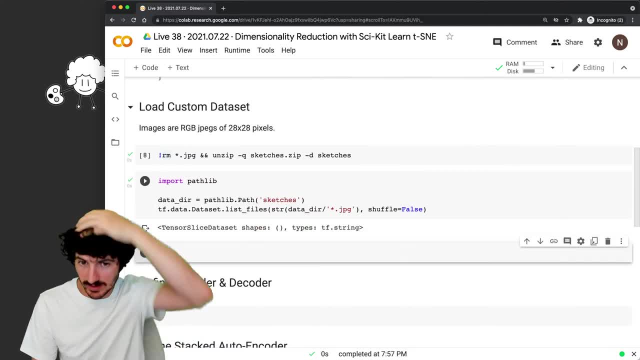 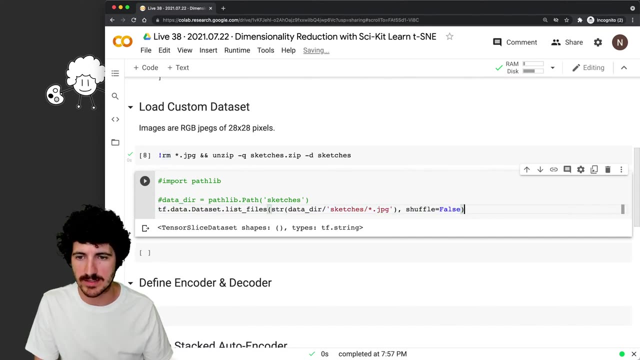 All right, Let's see if that executes. All right, So we get shapes, types, strings, and this was good before, just that. Um, I don't think we even need these things if we just put here sketches. but let's keep it for later. 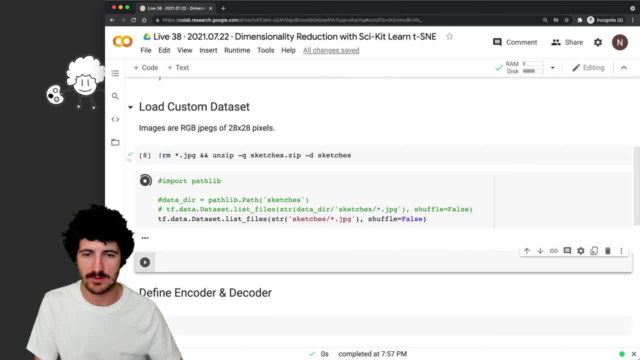 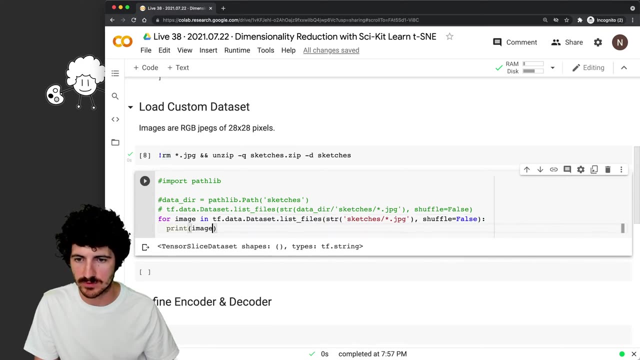 Yes, In case I think I was doing something Okay Here. Uh, the problem is that these are strings and they don't have a shape. So we could say, for image in print, image, Let's see. All right, So we're actually okay. 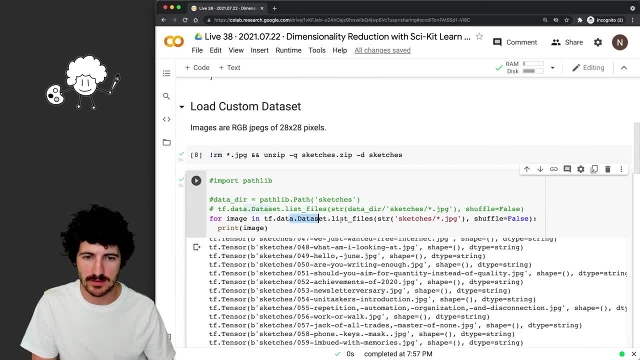 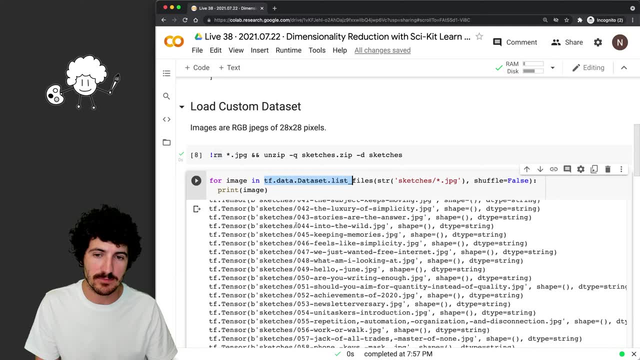 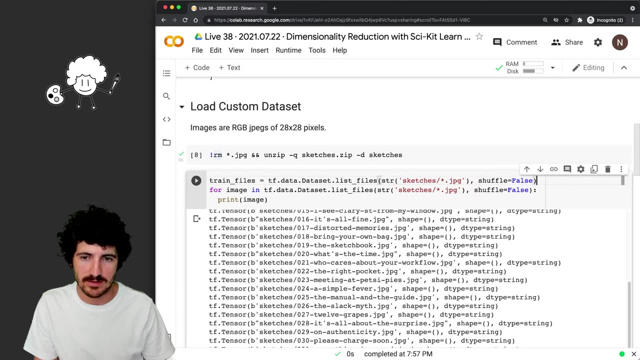 So I was a bit confused because I wasn't seeing the shapes, but this was actually working before. So what we're doing is we're least Thing. this is sort of making, well, sort not, it's actually, if I do here, uh, train files and print, so we just do this. 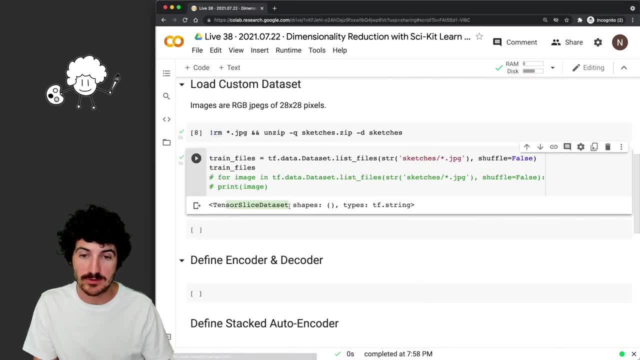 Right. So what we have here is a tensor slice data set which doesn't have any shape because the type is string and uh, with those train files. so we can say here train files and we can say Here file, we can print the file and, yeah, again we get these binary, uh, string here. 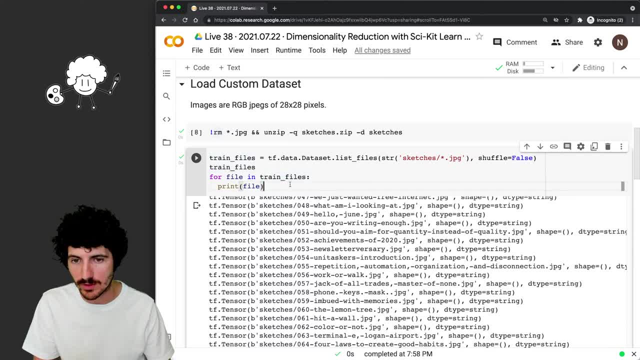 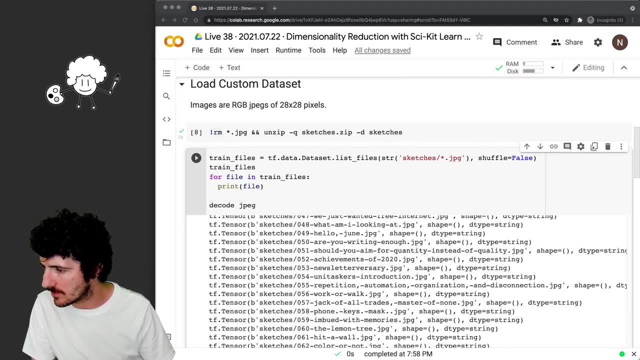 That is just the path to the string. So we need a function now to decode those uh images. right? So the code JPEG. I'm going to use a helper function that I have here, So we're going to decode, we're going to define a function that is going to decode, um, an input image. 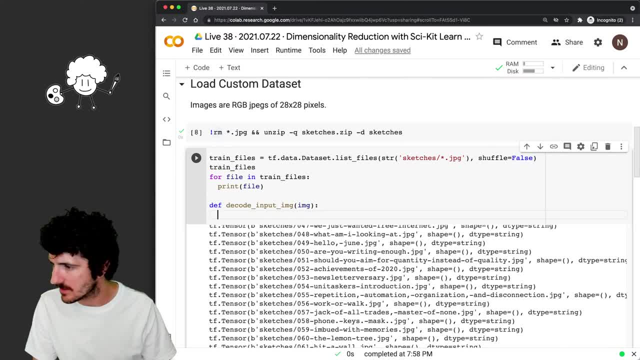 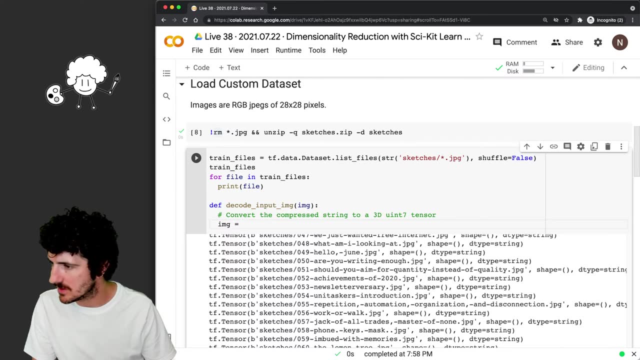 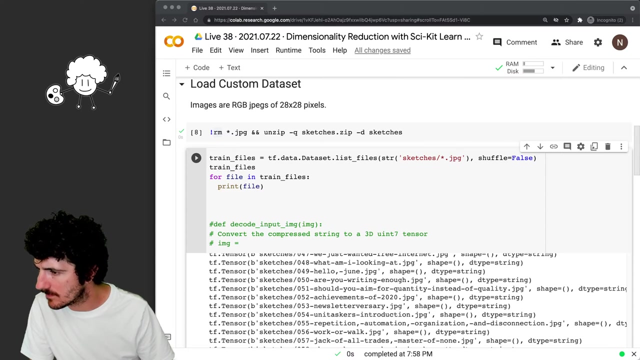 And uh, we're going to convert the compressed string to a 3d you in a denser, So image is going to be. let me see So. first we need the load image train, right, Okay, Okay, Okay. 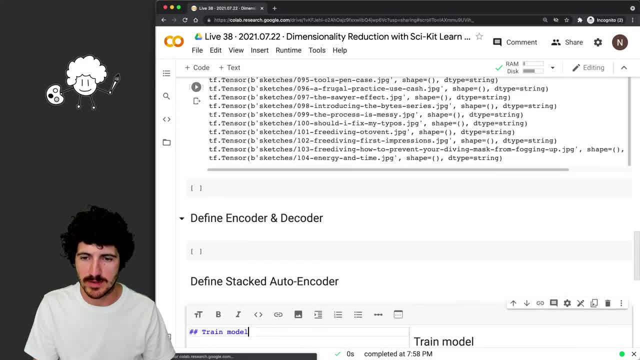 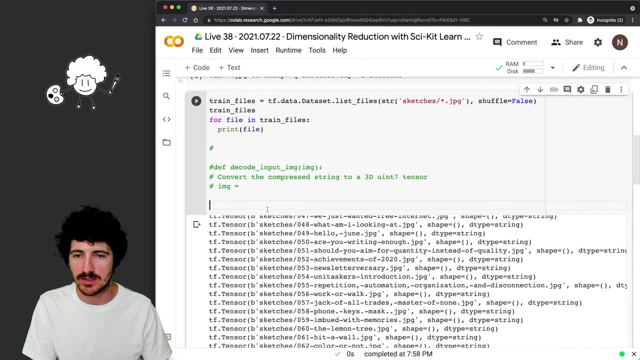 Okay, So we're going to do here to helper functions, but at the end of the day, what we'll end up doing is that we're going to need to do this. We're going to need to um call on train files. 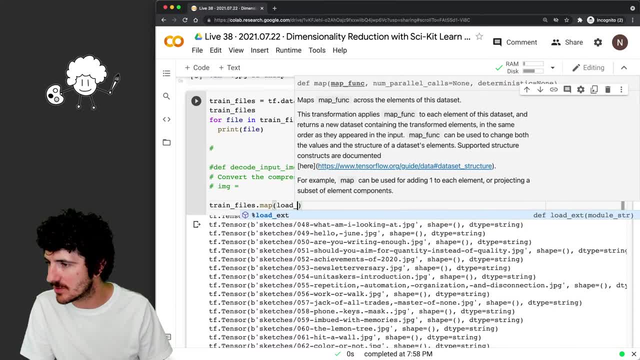 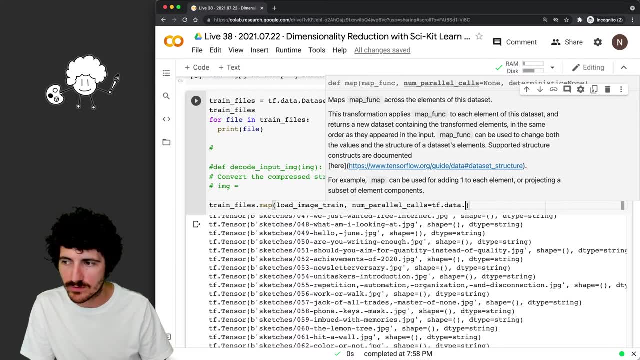 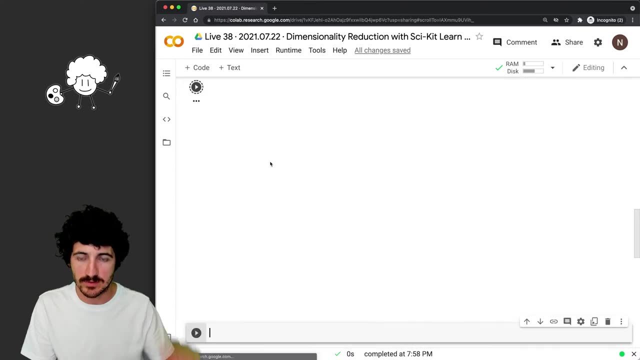 We'll map And then, um call a function. No, we haven't defined yet That is, load image, train and non-paralleling calls. We're going to use out the team, All right, And of course this is going to fail because that function doesn't exist. 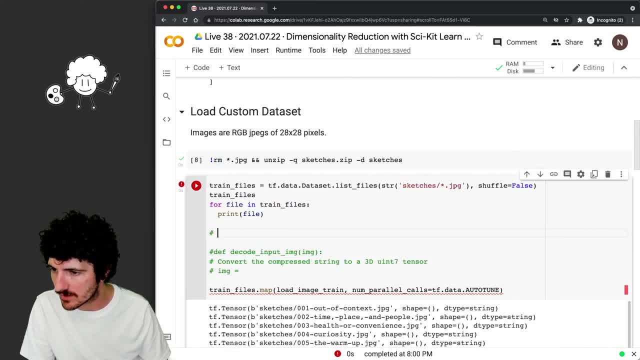 And, uh, what we can do. let me just take a look here in the chat. All right, So there are no comments, so we're going to end the poll. So we have four votes here and Great, All right. 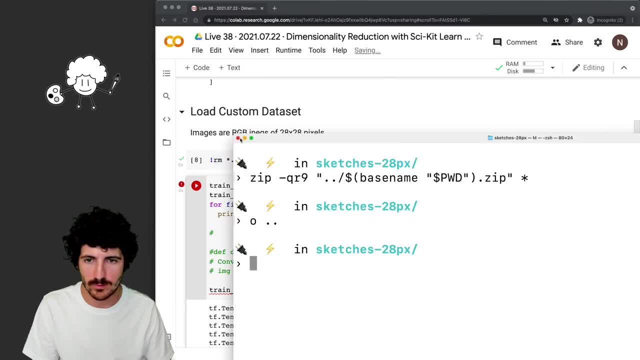 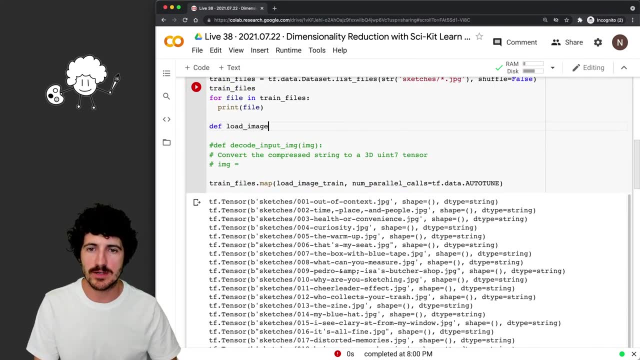 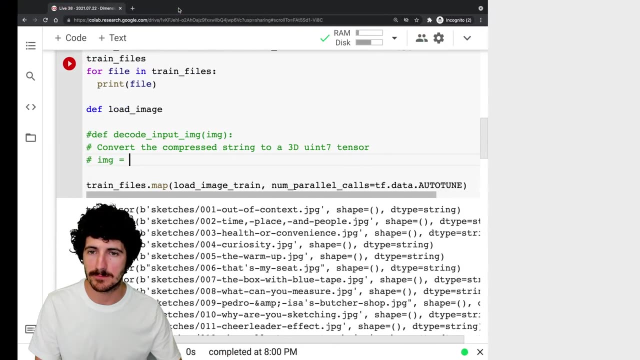 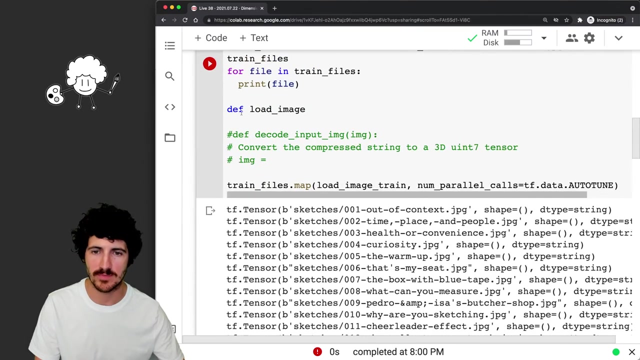 So let's keep going. So we have. so we're loading the data set and we're going to define that. load image train function. load image- Um, This is better, I'm not sure. Load image train function: Um, I'm not sure. 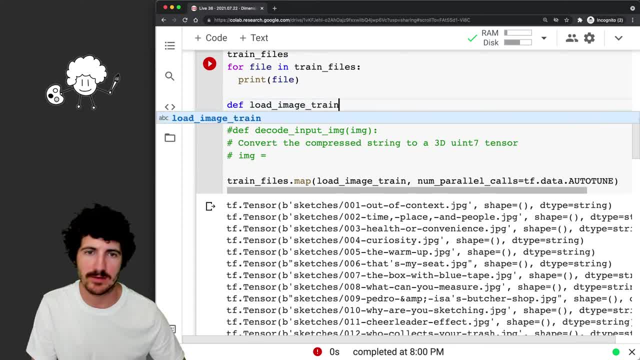 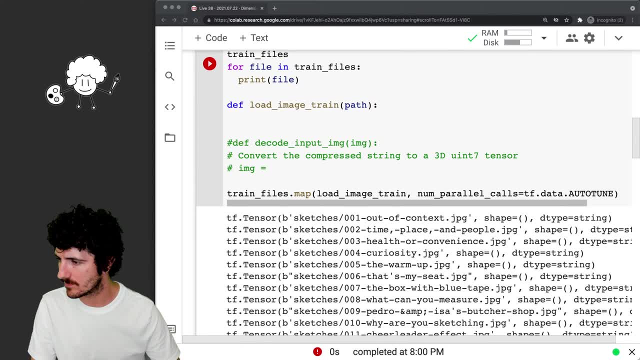 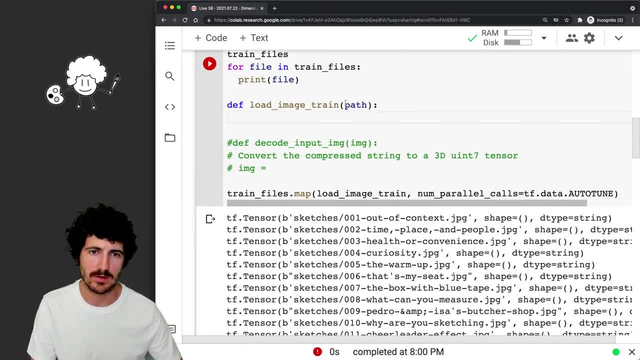 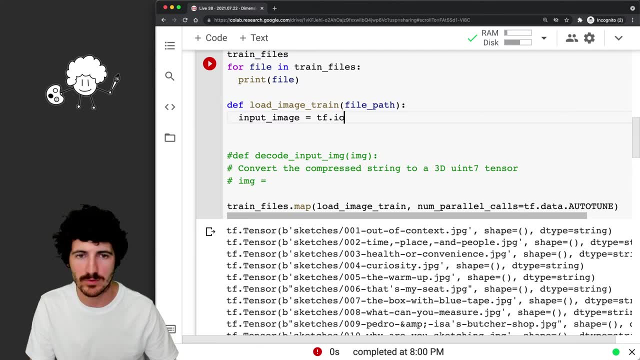 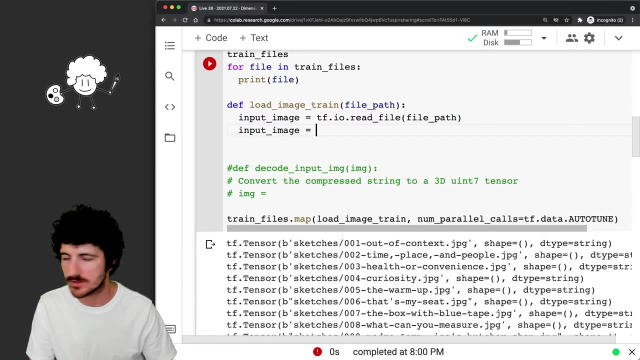 Um train and we'll get the. I think we just get the path. Yeah, Yes, We get the file path and, uh, what we do is that input image is going to be. we can do read the file. So, the file path and that input image, we're going to decode our input image. 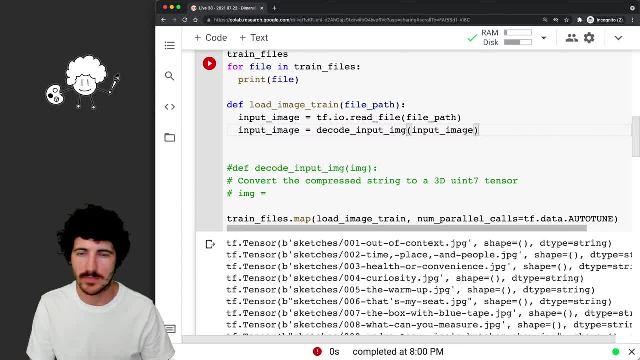 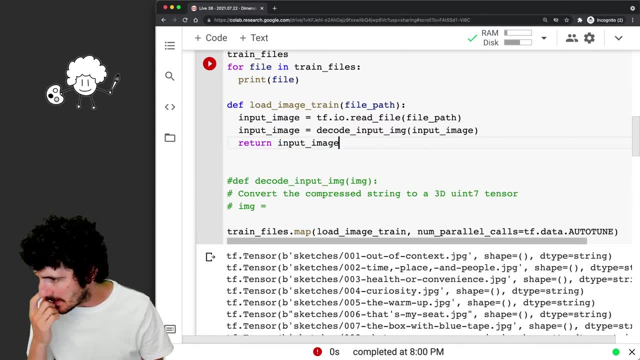 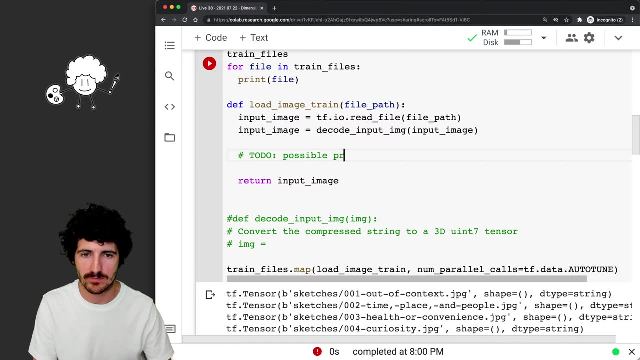 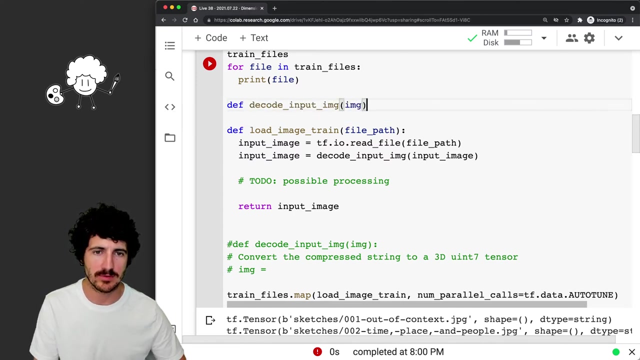 And we're just going to return that input image- and you know we could do other processing here that I'll show here, Um, and we need now that, uh, the code, input image function that I was going to define below before. 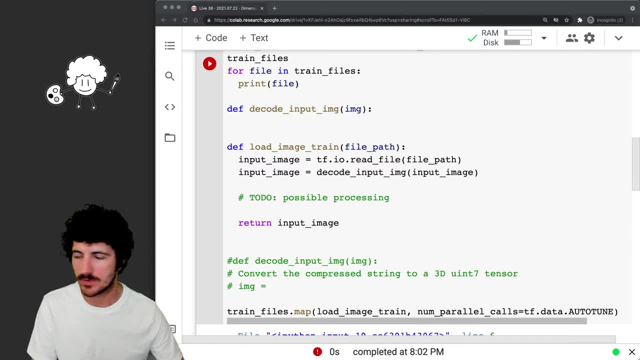 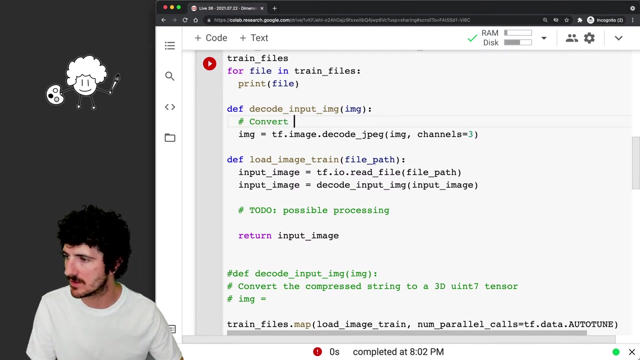 All right. So here we would: um the code, input image: Um, so we're going to get TF image decode JPEG with that image data that we've um tamed and we have three channels. What this is doing is that we're converting the compressed string to a 3d unit eight, uh tensor. 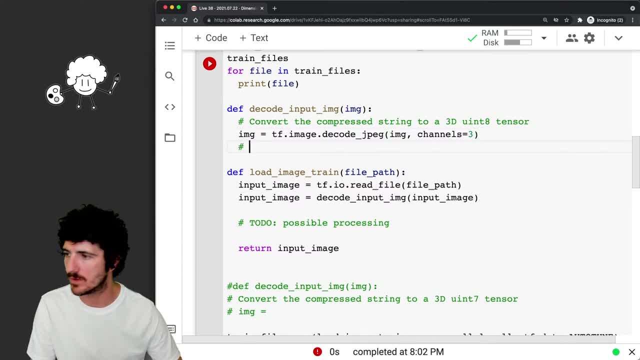 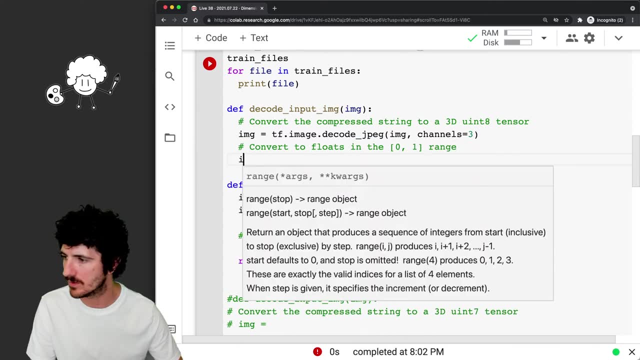 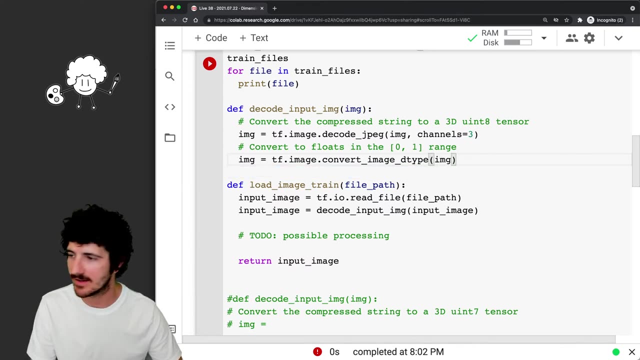 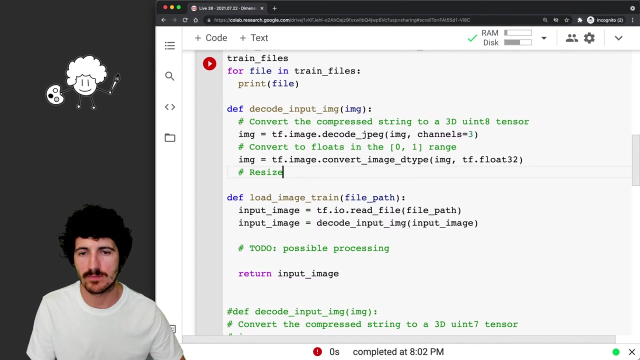 And uh, now what we do is we Convert to Floats in the zero to one range. So we use TF image, uh, convert image D type and uh, we get a TF flow 32. And now we, uh, we would maybe here resize the image, right. 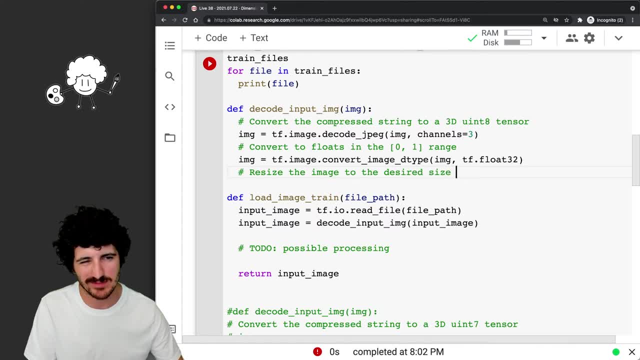 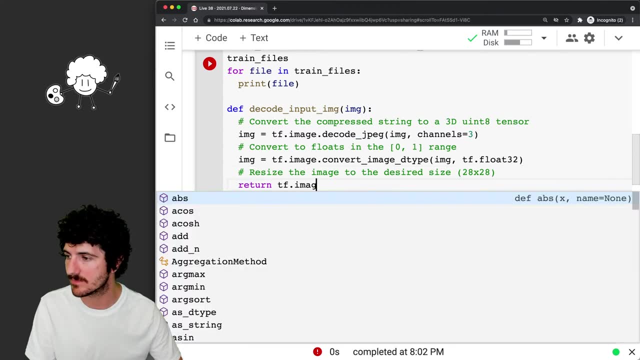 The image to the desired size, which you know it's going to be here: 28 by 28,- but the image is already that size. But if we do this, um, then uh, the the data set doesn't need to infer the image size and we can do other operations right. 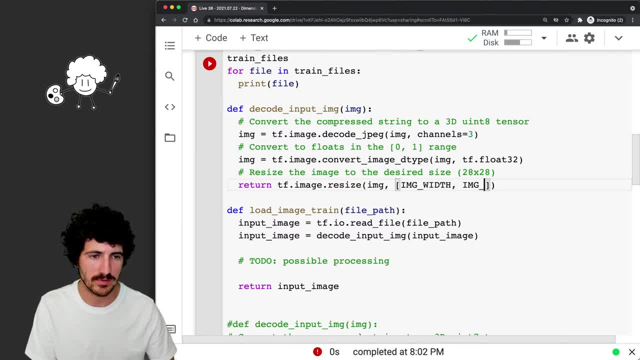 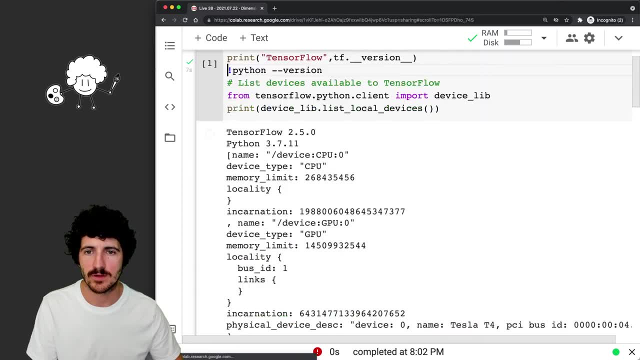 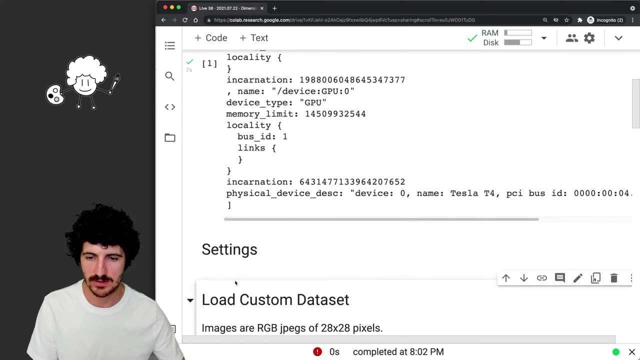 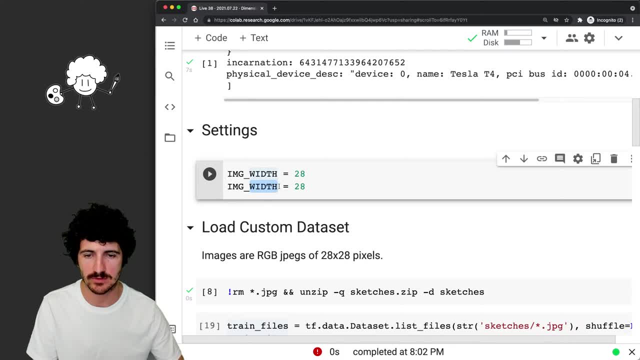 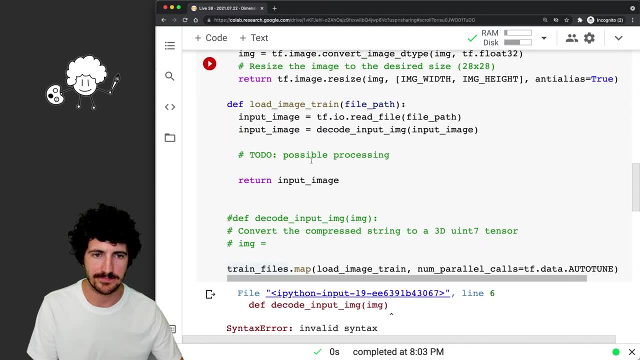 Okay, 28.. And Image height is going to also be 28. So we load that Great Cool. So, um, where are we All right? So we're here, so we're loading, and then we resize the image. 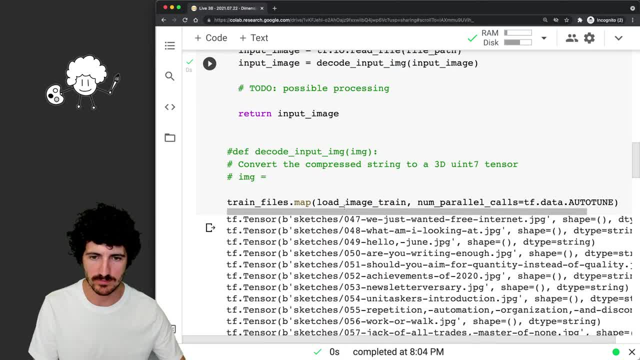 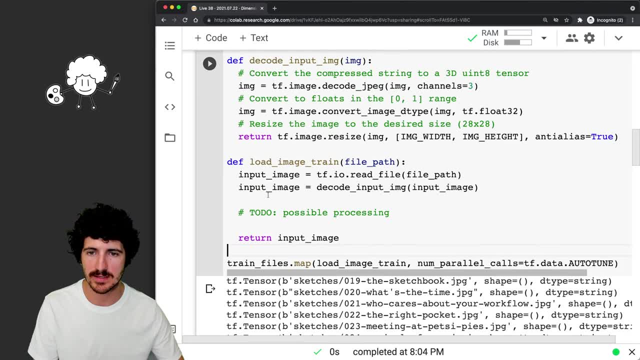 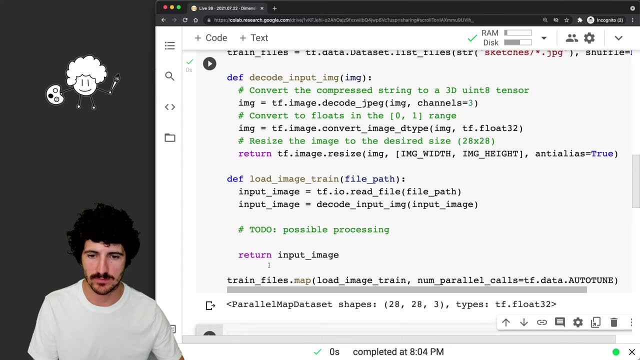 So these should already work, Right? So we're printing that, uh, which means that we're going low, to, to, to, to, we don't need this and we don't really need this Or this. all right, So, uh now. so let me go back here. 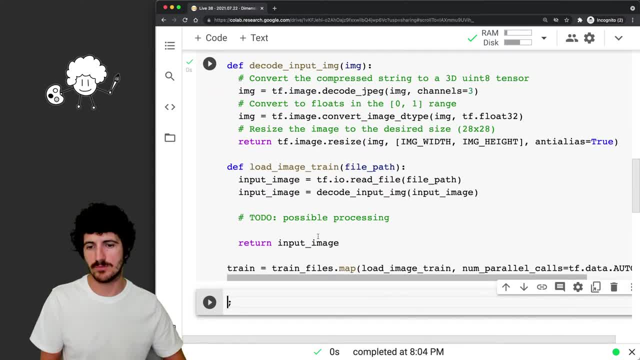 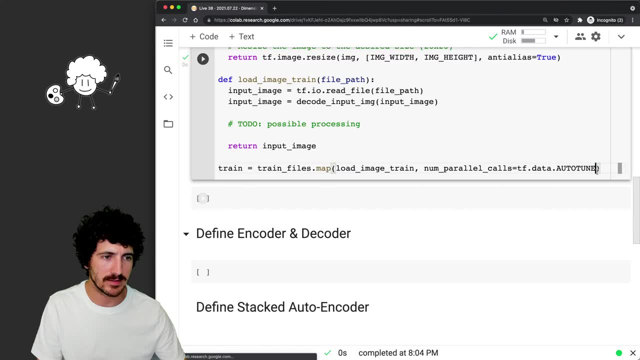 So this is going to be the train data which you know. we don't really have this data, so we might need to do some split later, but for now, let's see what we got here. so we got this train. 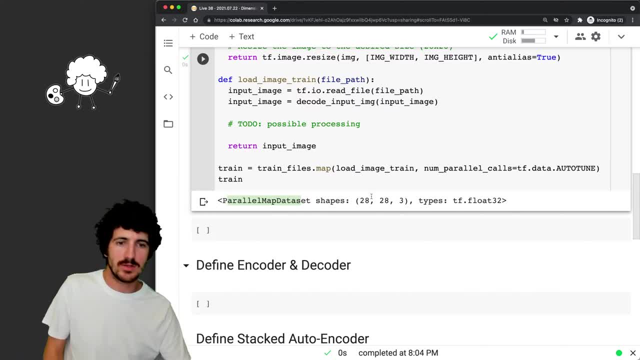 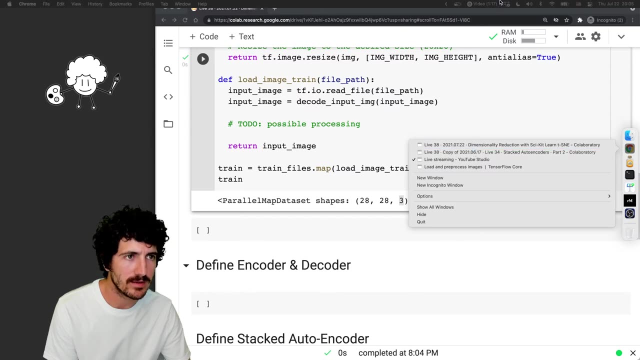 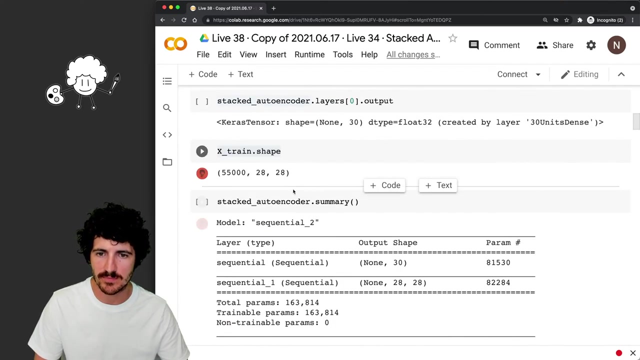 All right. So we have a parallel um data set with shapes 28 by 28, um by three. There's one thing that is different here from um the previous right. So we on the previous um live stream we were getting the shape right. 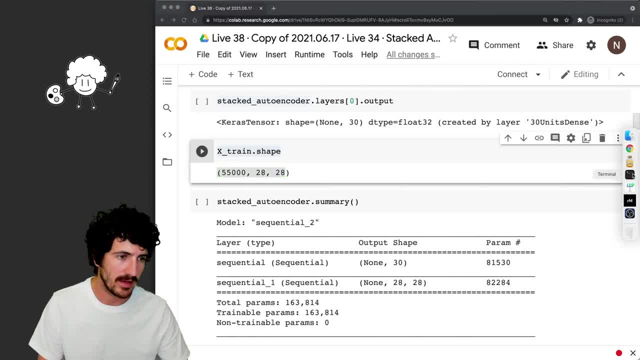 So we were actually getting just black and whites and, uh, maybe that's something that we could do here with Keras. We don't really want the images. Um, well, I mean, we do want the images to be black, uh, to be color. 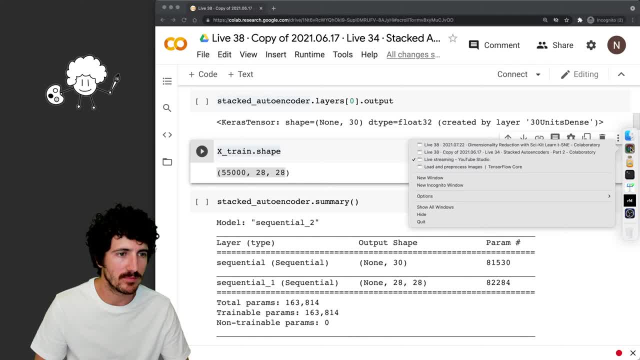 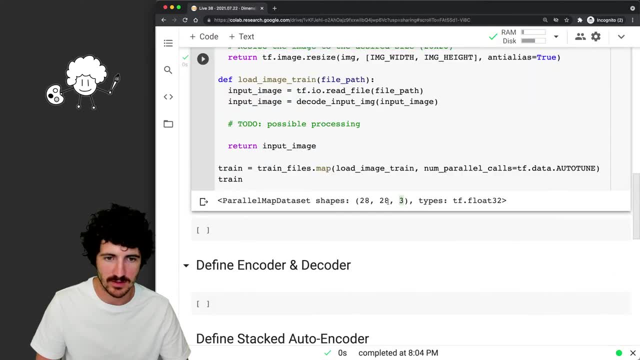 But maybe, maybe that makes this, uh, probably, a bit more complex, a bit different than what we had before, And we'll have to change the um, the neural network architecture. So we have 28.2.. Okay, Okay. 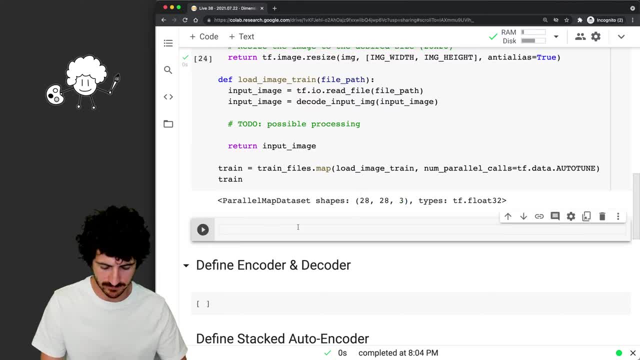 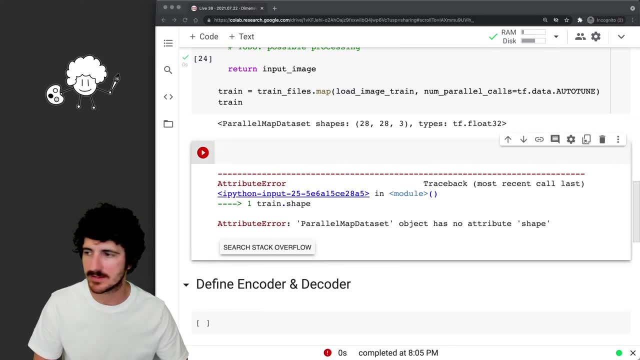 28,, 28,, three. This is, these are the shapes um train. I don't know if I can. Okay, So we'll have to get a subset of the data set. So we'll get. so let's see here. uh, uh, all right. 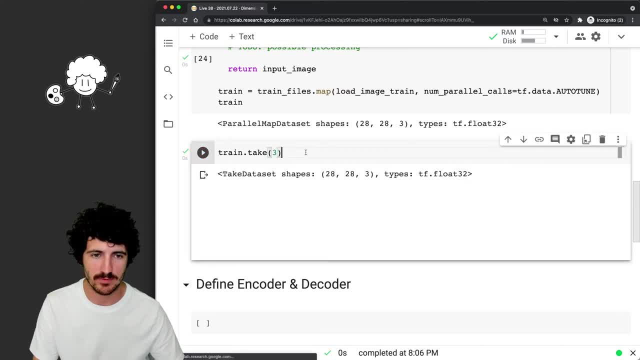 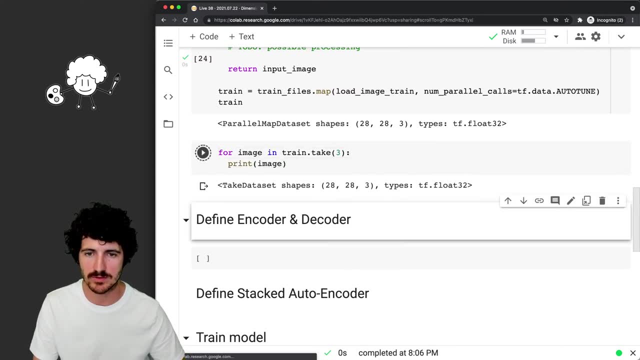 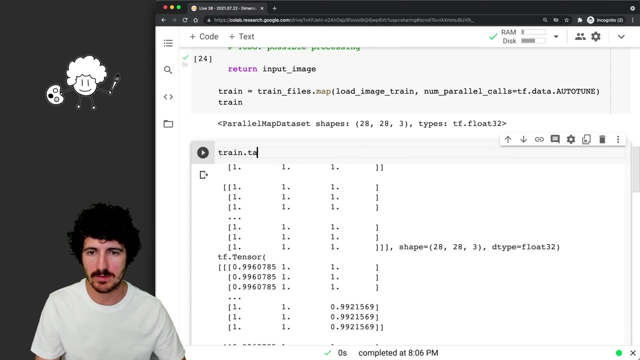 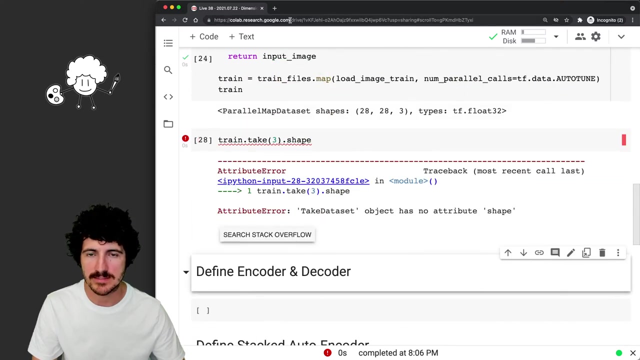 So we can do train. take two, three, for example, for image in blah, blah, blah, Print image: All right, So we actually get the shapes and maybe we can even print here the shape. No, Hmm, Parallel. take two. 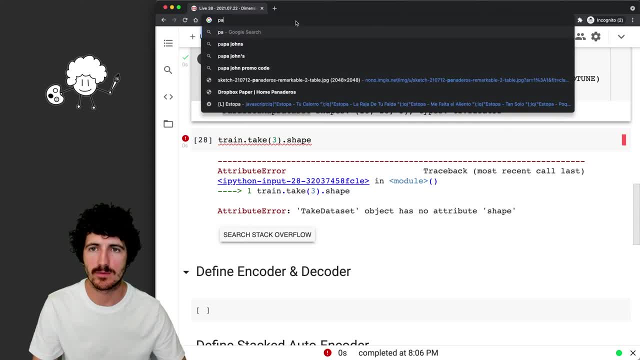 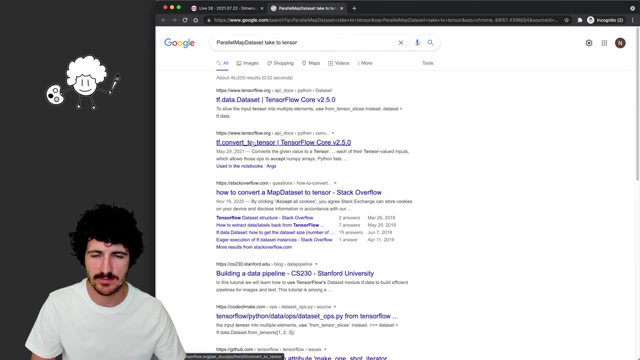 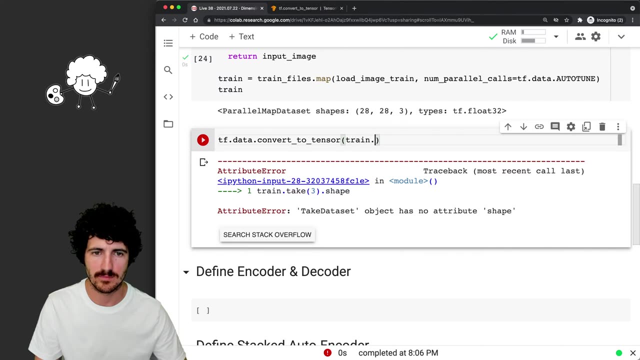 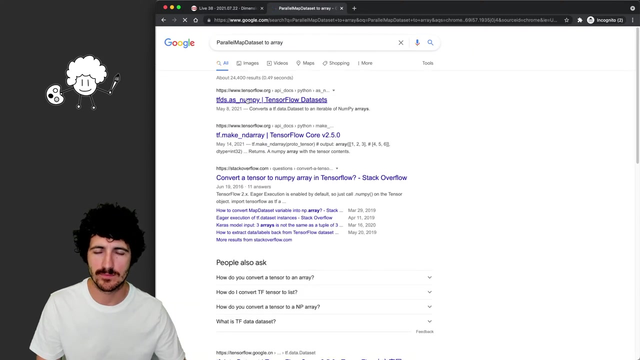 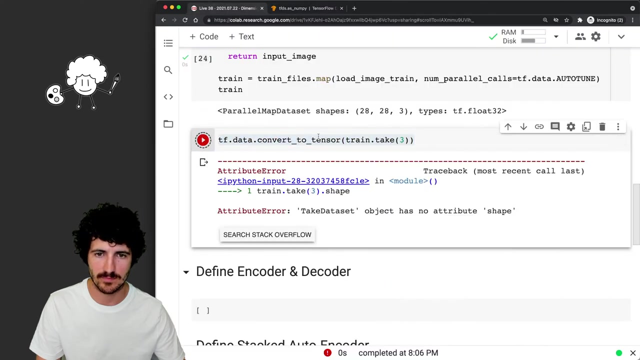 Then, Sure, Let's see- I'm not sure- if this works. All right, Um cool, All right. So Okay, No, I'm gonna, I'm gonna. It's kind of a good long�, All right. 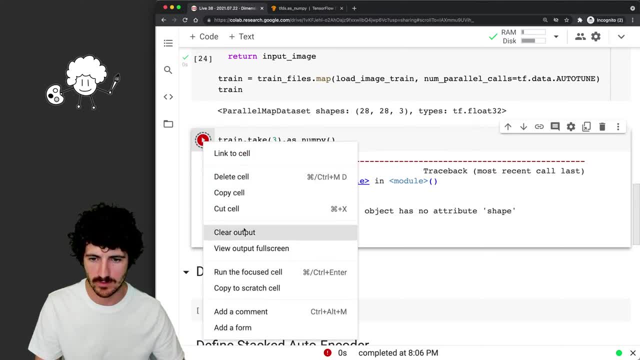 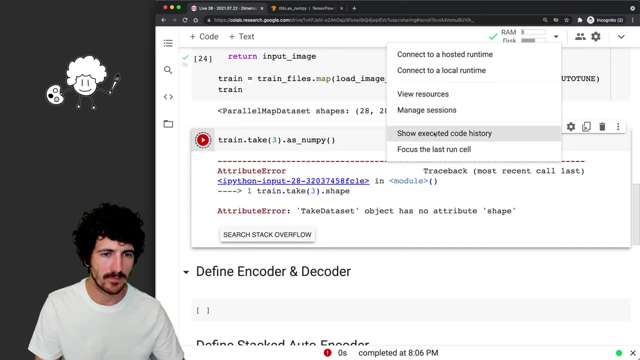 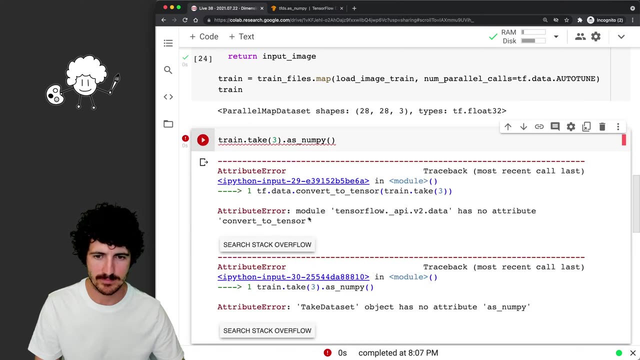 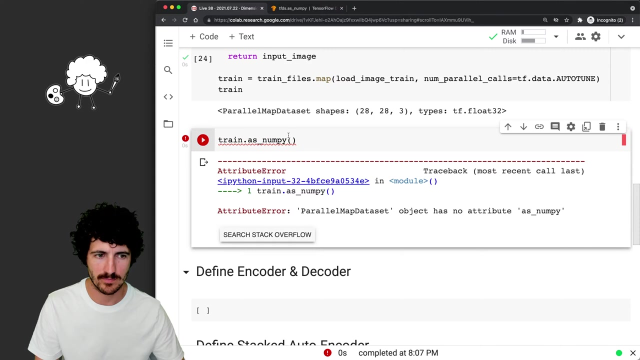 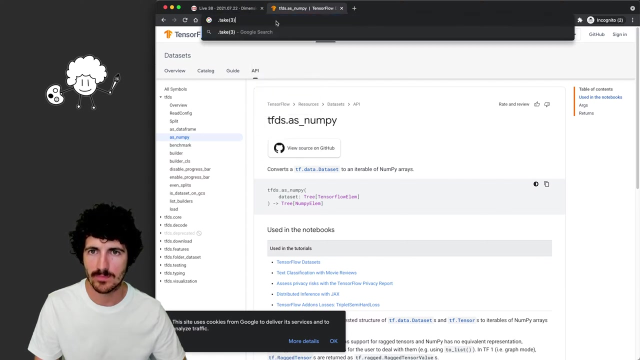 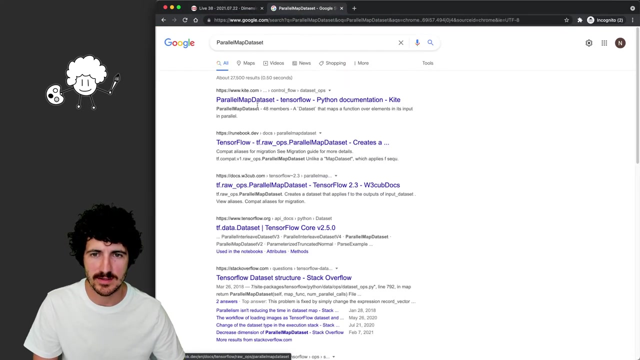 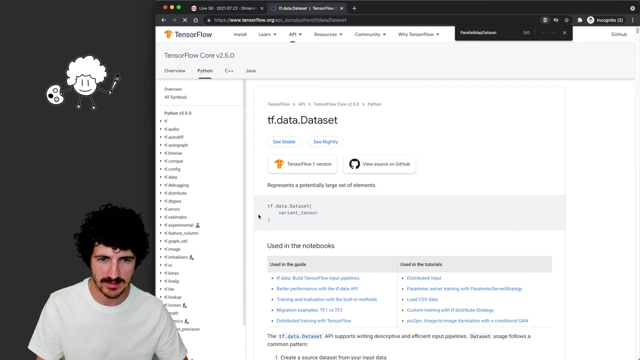 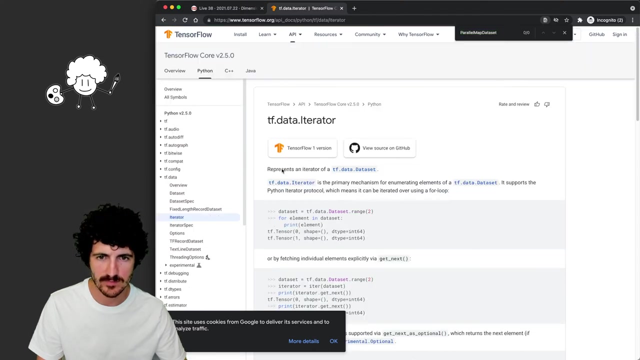 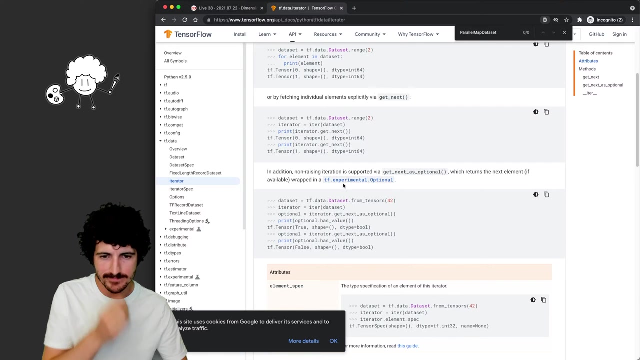 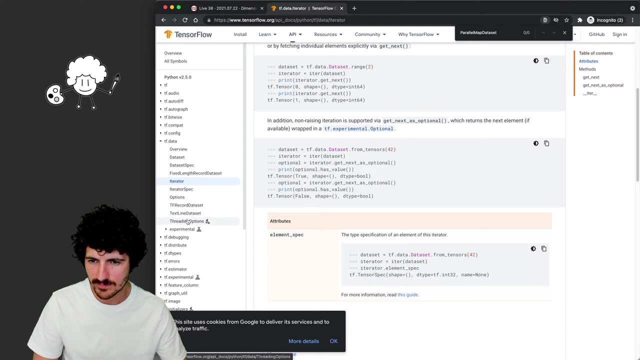 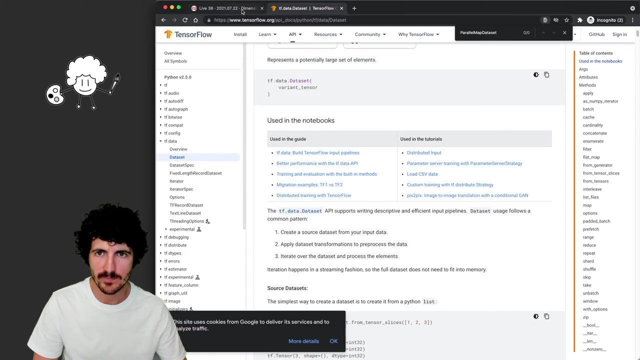 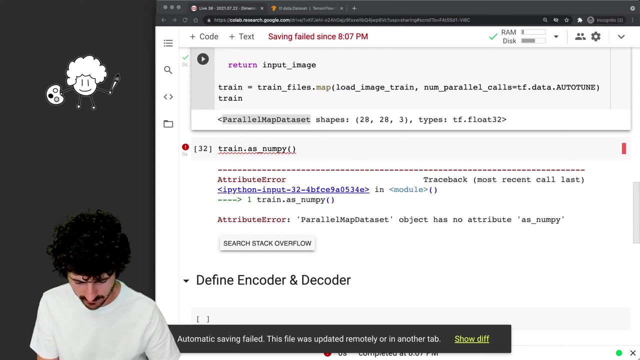 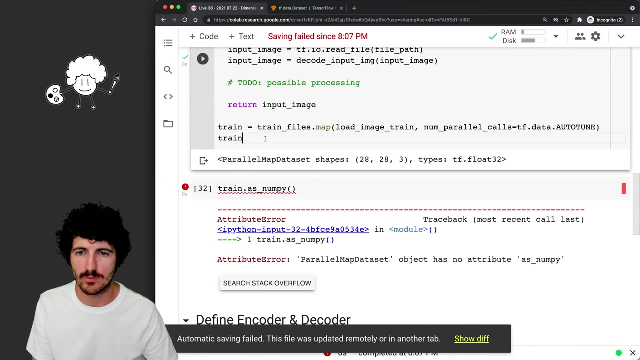 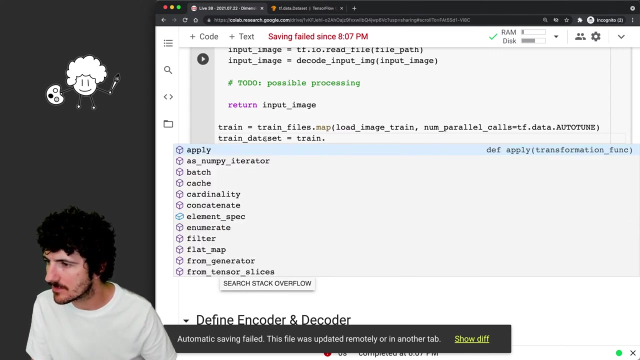 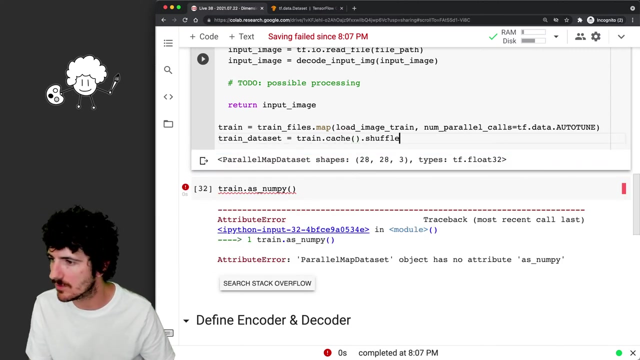 Not sure. Um ah, Yeah, Okay, So these, these are the brand I've seen before as well And I never know how to properly work with this data set objects. Thank you, All right, But what if we do a train data set and we run train cache, shuffle buffer size, which we need to decide hatch. 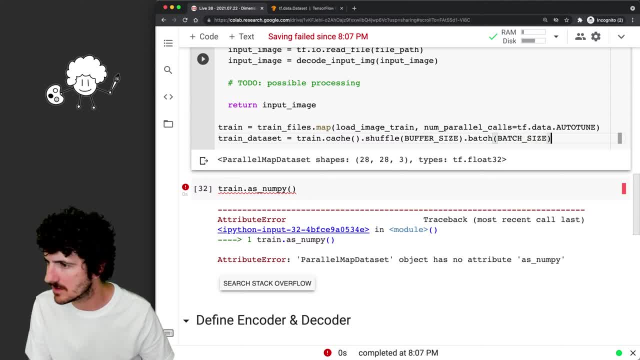 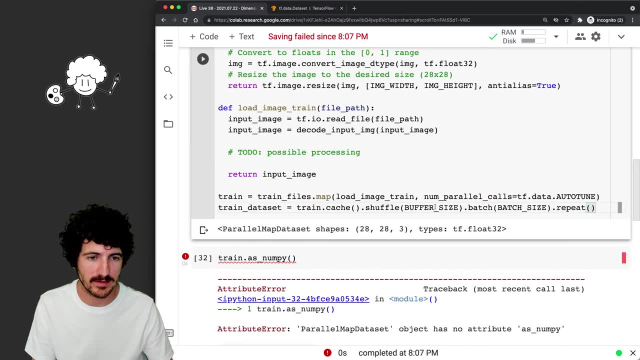 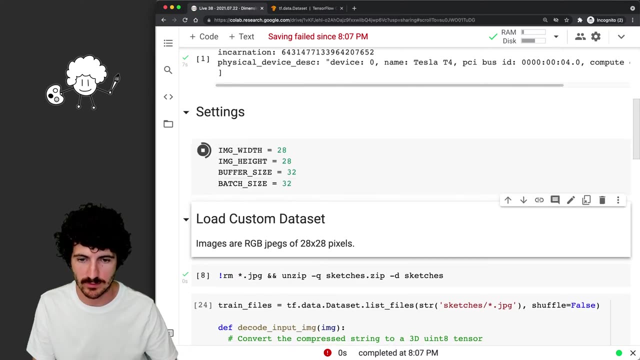 That's size B, All right. So he's going to ensure that we have more data samples and we now need to define these two hyper parameters. So let's say, our batches are 32 and we're going to see now if this gives us something different. 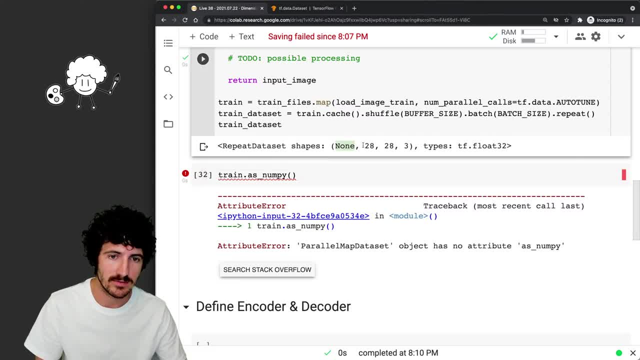 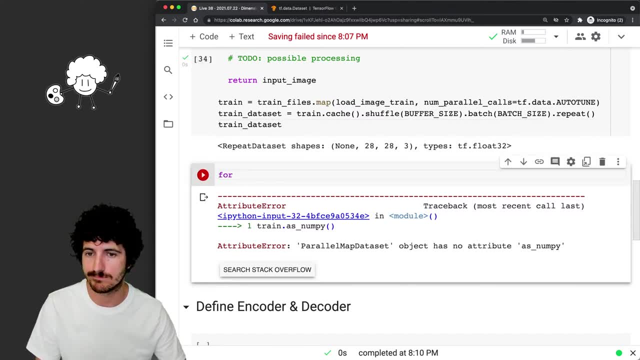 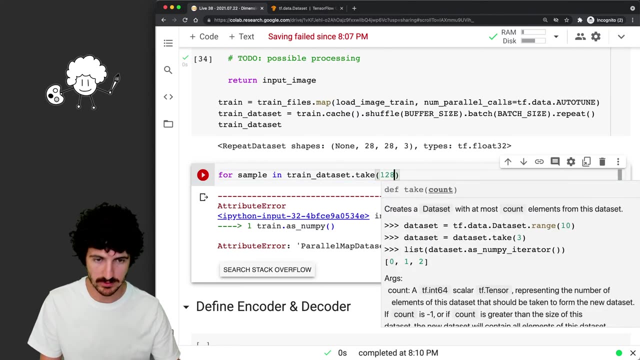 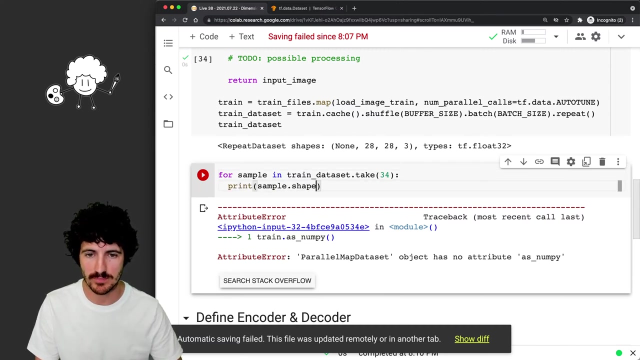 All right, So repeat data set shapes: non, blah, blah, blah. So this means We have as many as we want. so we can now do for sample in train data set: take 128.. Well, let's, let's do just 34 green sample shape. 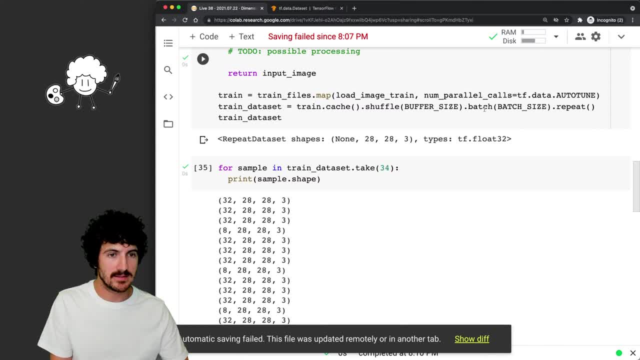 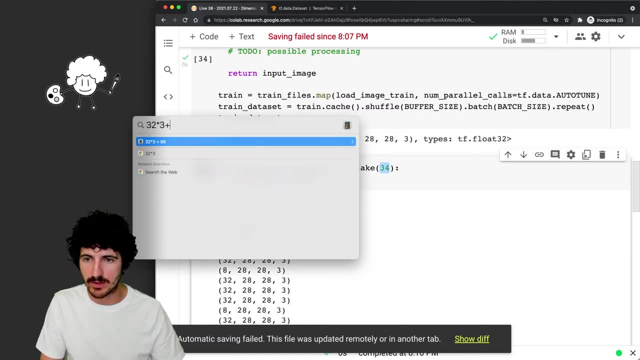 All right, So we're getting batches, so we're batching these things, And, uh, so let's say we just Right, So 32 multiplied by three plus eight, uh, that is 104, right, So all we can get here is um these four batches. 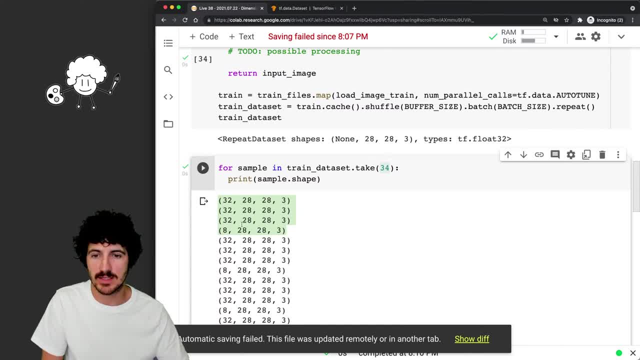 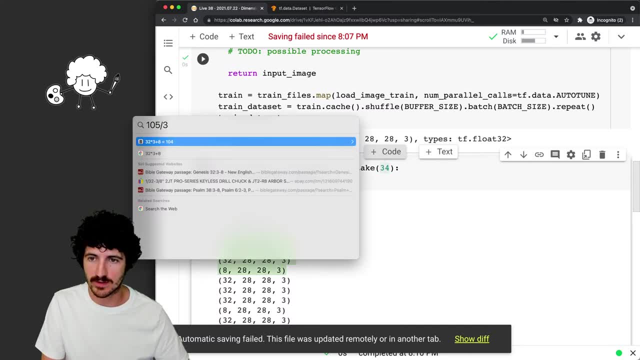 And then we reset because we only have 105 samples from the data set. So they shuffle and then they start again here. So because 105,, uh, we can not really well 35. So our batch would be, for example, 35.. 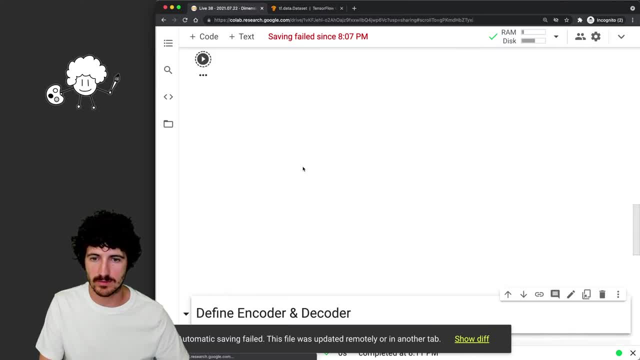 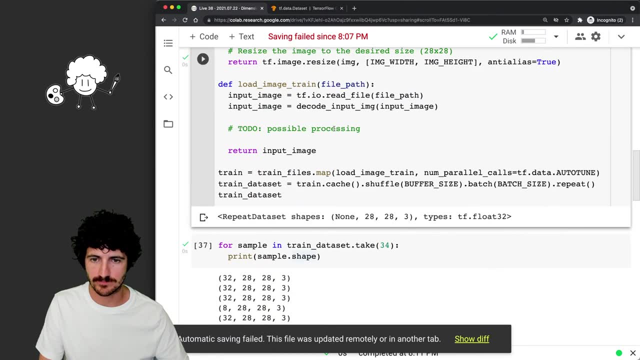 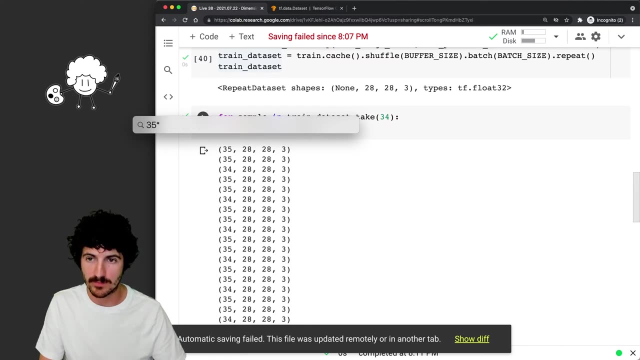 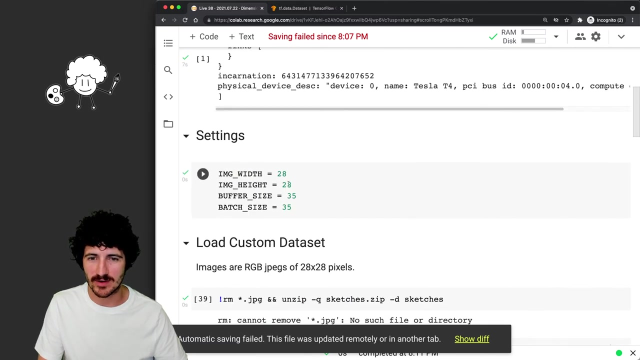 And now maybe, but we still get, oh, because of the buffer size, 35. Right now we, uh, we still get 34.. All right, Let's actually leave it here. So this way, we can, we can get um. 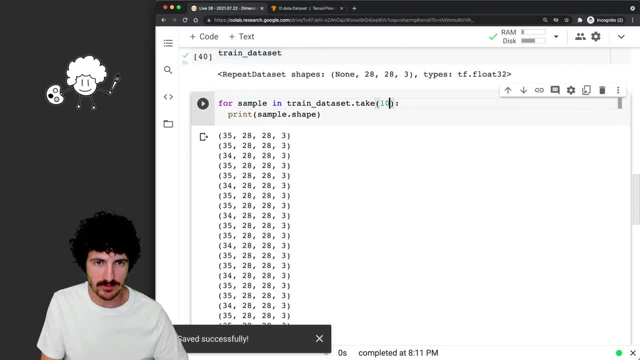 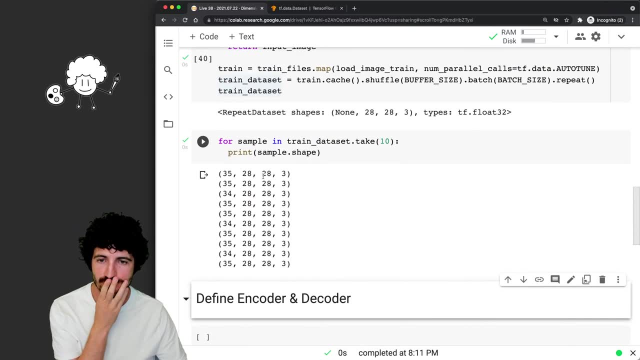 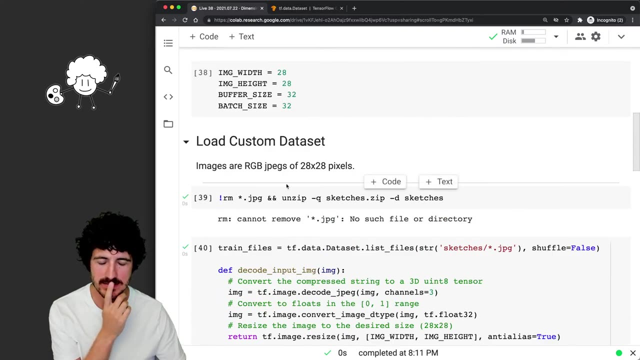 many different um batches, so we can say 10 batches and we'll have more, uh, more samples here and um. we don't really need these data batch, but uh, what we can do is that we can put here the possible processing that I mentioned. 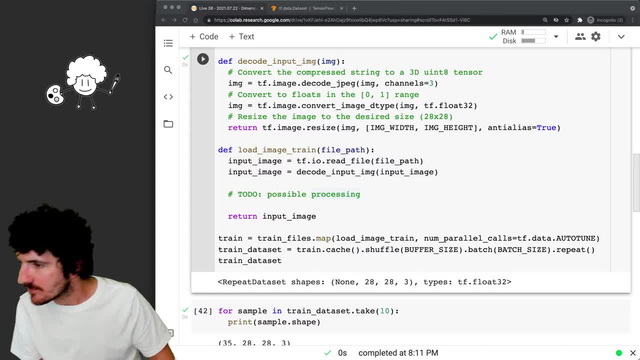 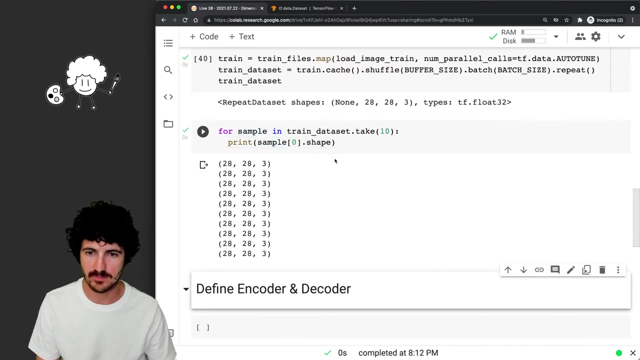 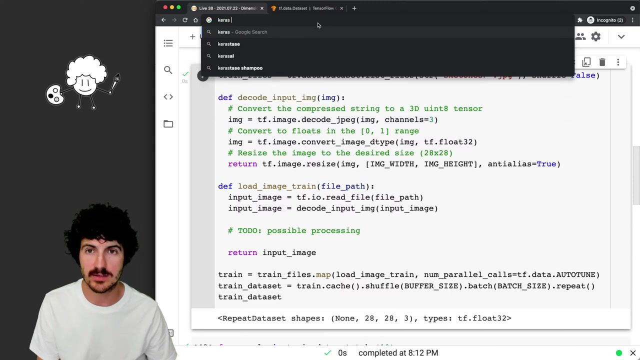 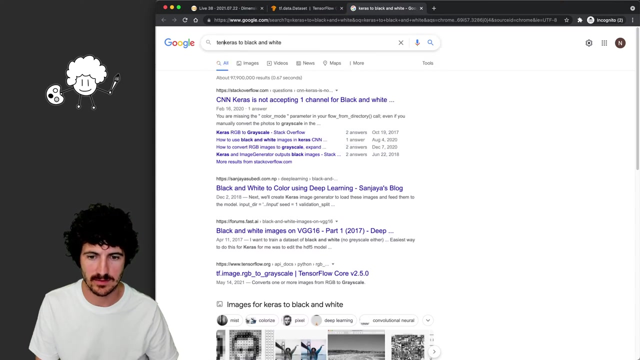 before. Hmm, Hmm, Hmm, Hmm, Hmm, Hmm, Hmm. So we had for each of these. all right, So we have an RGB image, Um, one thing that we can do here Here is so Keras, uh, to black and white, RGB to gray scale. 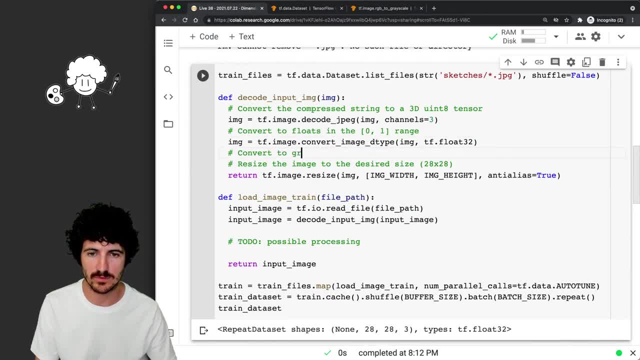 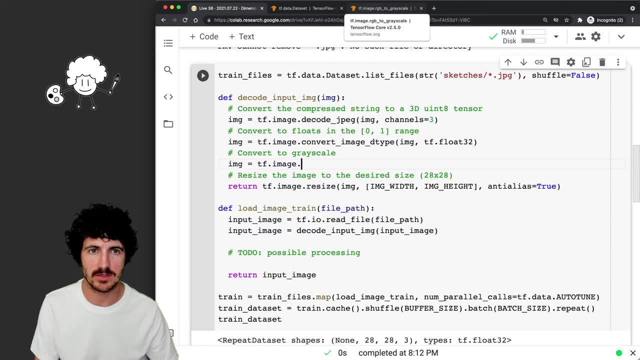 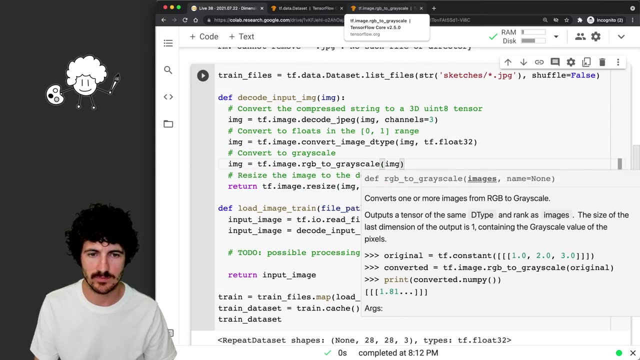 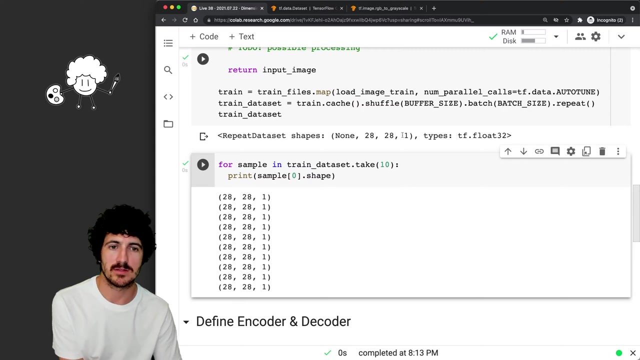 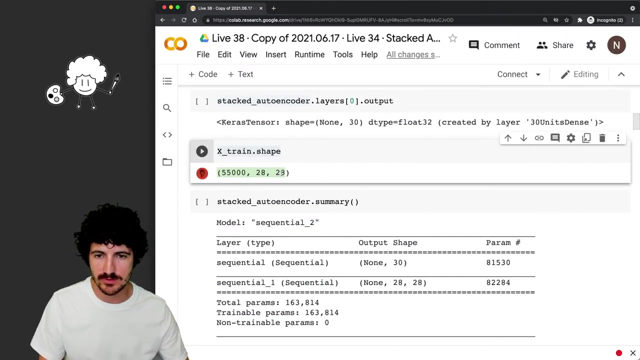 So we can actually, uh, convert to gray scale. So TF Keras image RGB to gray scale image. All right, Let's try that out. Now we do have the, the shape that we wanted, So now these are going to be um the same proportions. 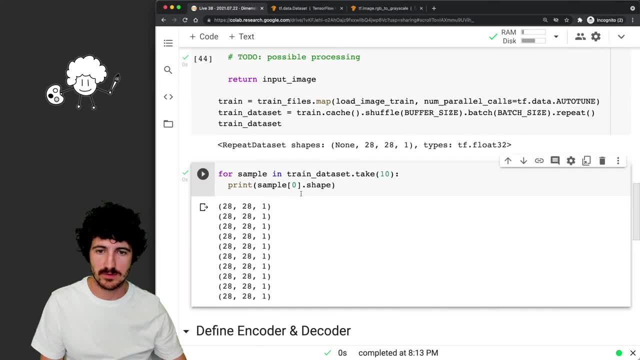 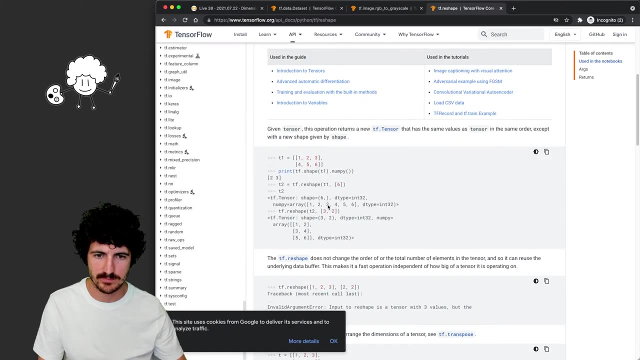 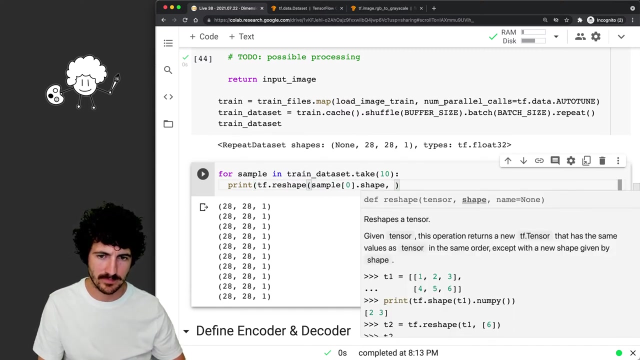 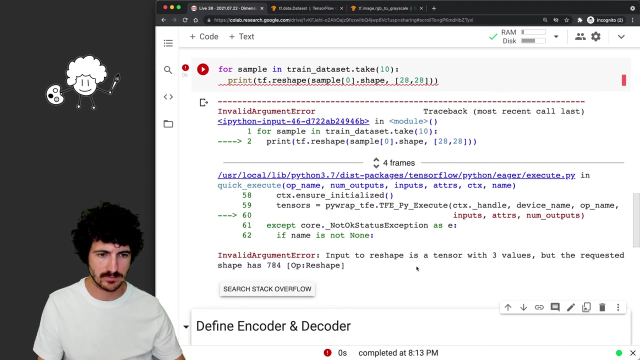 So 28 by 28,. uh, let me see, can we do this, Can we? Oh, we finished it with a longer far angle. Alright, All right, Good job, Dan. Fantastic. Very good, Yep, Great job. 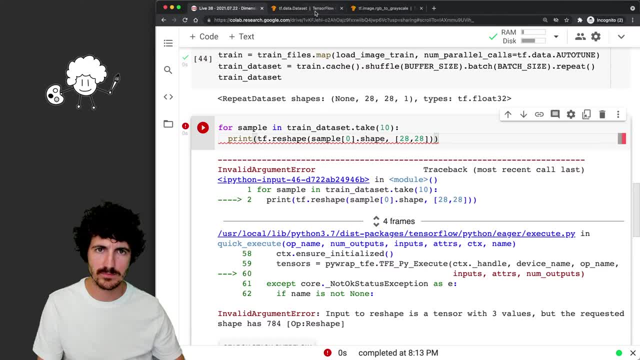 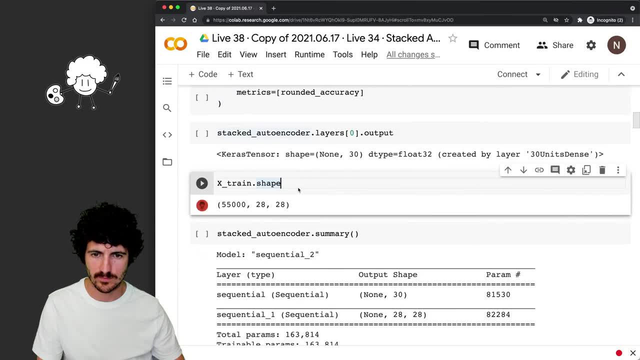 Check out more stuff. Be sure to troop a separate video conference for the today's conversation. The same thing with respect to taste systems: Fantastic, Okay, Uh-huh, Thank you. Thank you, Let's run, run before, All right. 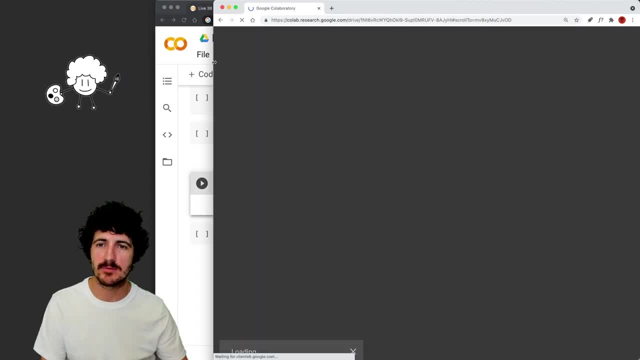 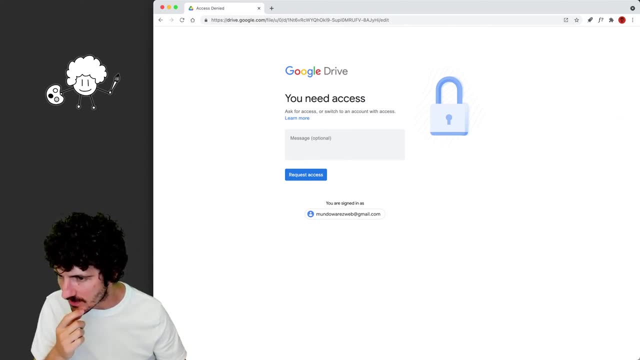 Ah, can do this with same session. I'm not sure if the sessions are via IP or I want to use coffee model. how I can use it in Google call up class. I started playing with color produce mall and it is worth every penny. 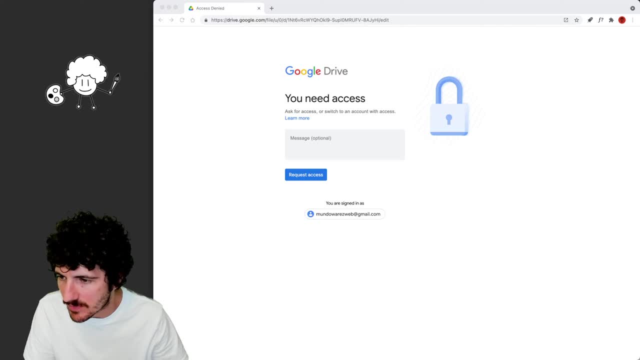 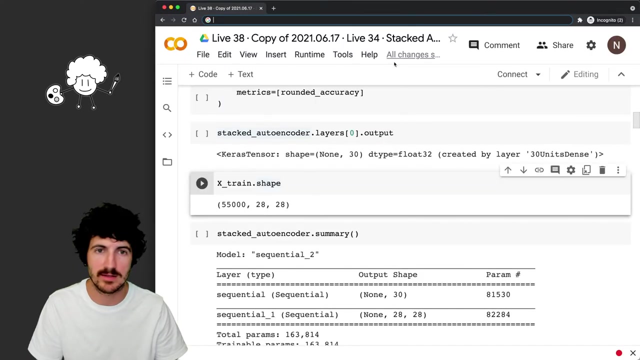 Highly recommend. last run I could train a model on P five 16 days for 24 hours, No stopping. Yeah, So cafe model. I'm pretty sure that you can- well, I don't know- run cafe model. call that. 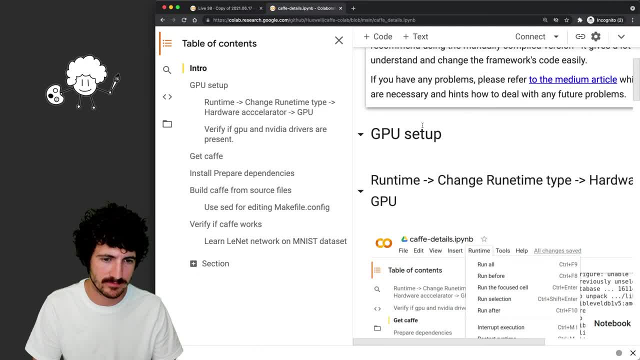 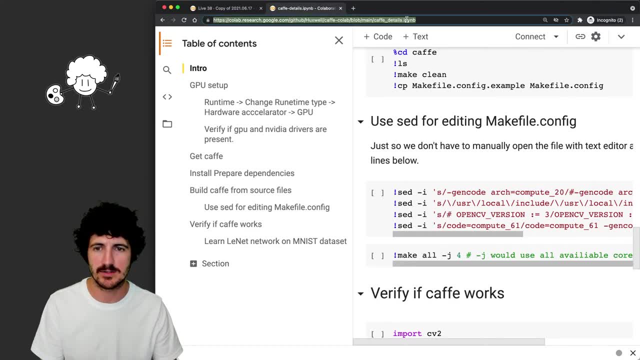 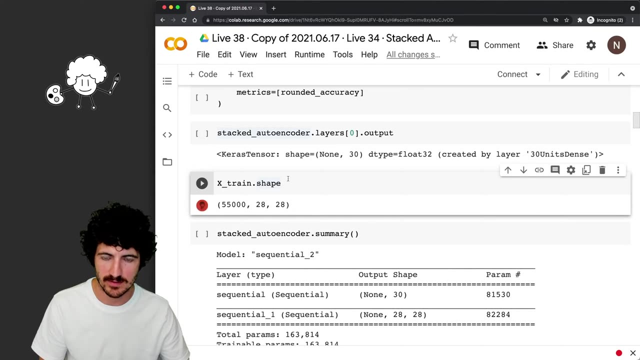 Well, it seems like here is a way to do that, but I'm not sure. I've never done it myself. Um, okay, Let's see what these data is all about. Um okay, Actually, I just thought we can. just we're testing, we can bring this. 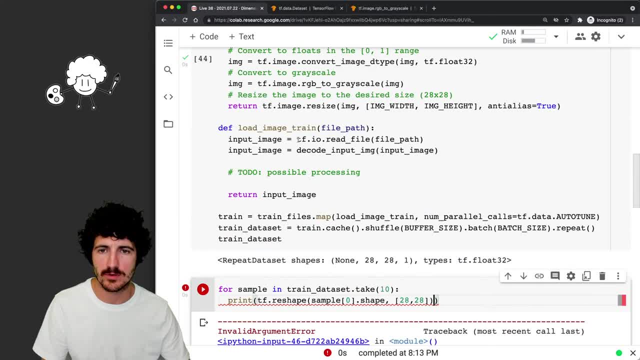 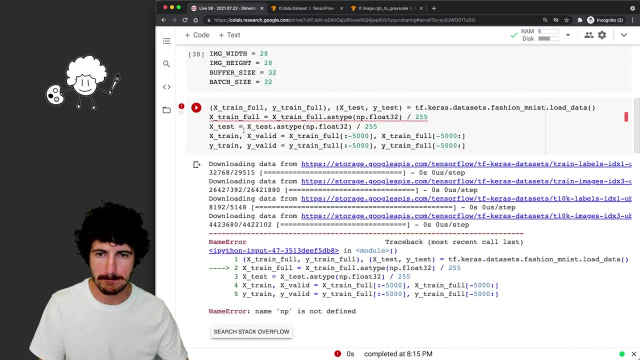 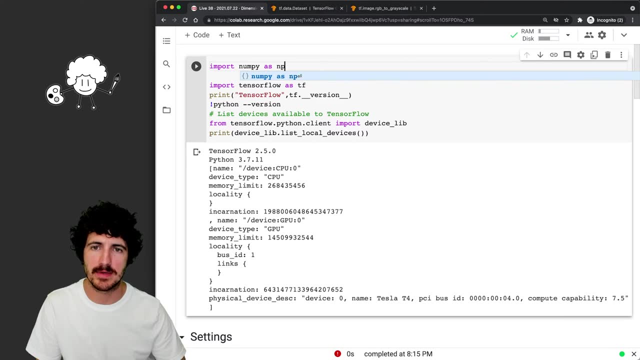 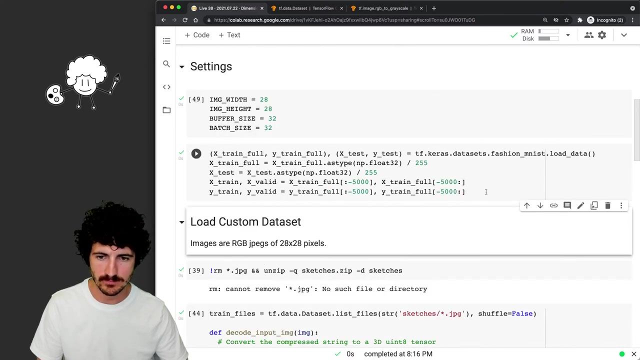 All to all the other notebook. Let's just try to be back with this. All right, So we have this here. Um, okay, Import, maybe import, non bias, MP, Great. And here we have, for example, X train full shape. 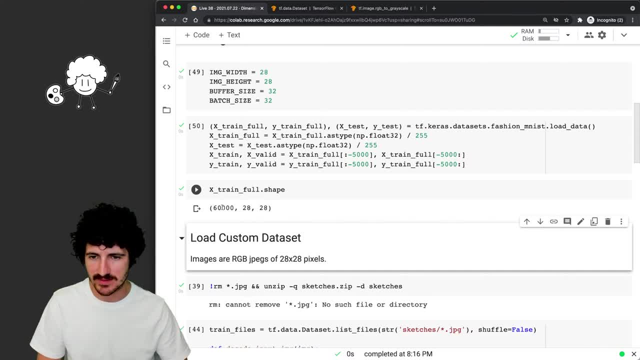 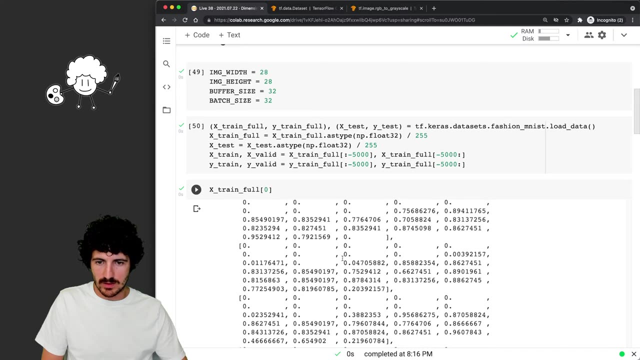 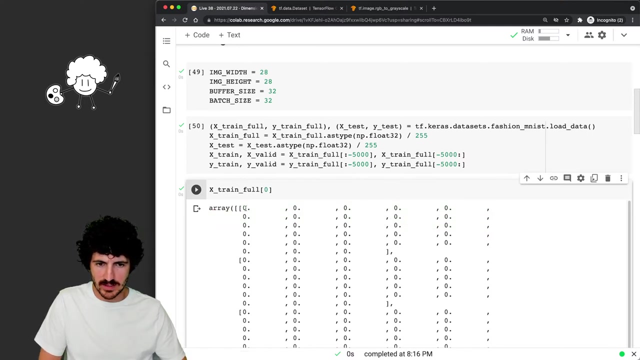 Okay, What is this like? So this is a 6,000 or 28 by 28.. So we get the first one. What's the shape? 28 by 28.. And if we print it 28 by 28,, so there's like 28 items of 28 digits, right? 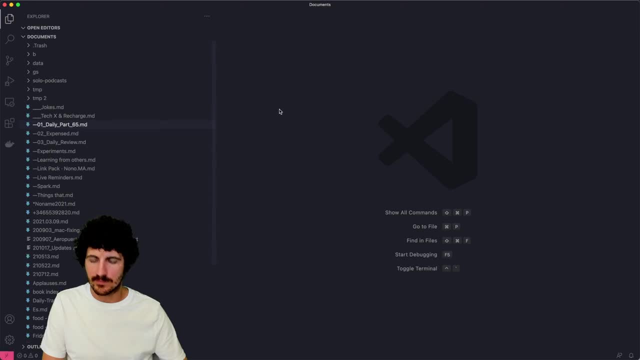 Okay. So again, it's pretty easy to do with a simple way. with that, I'll just say a motion. Okay So, and then this is how we're going to do it with this one. All right, So we're going to do: we're going to use an empty cell and we're going to do a. 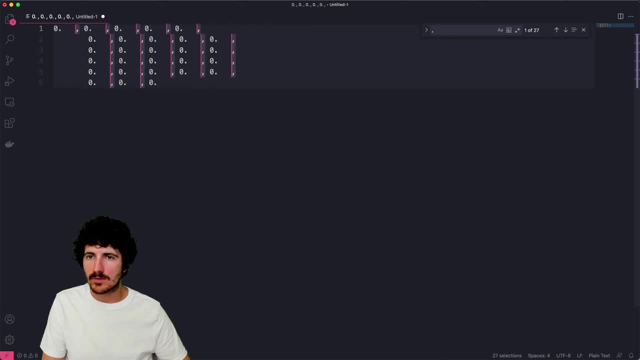 simple way with that. Okay, Let's go to. let's go back to our simulator and do some tests. So this is a simple way to do this, So let's do. we're going to do a sample failure test, Okay. 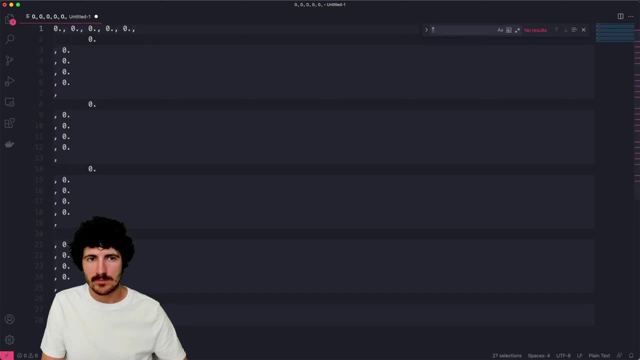 So this is the expression here. Oh, I want to do the best thing for this, All right. So let's go back to this one and let's see, let's do a sample failure test. Here we go, All right. 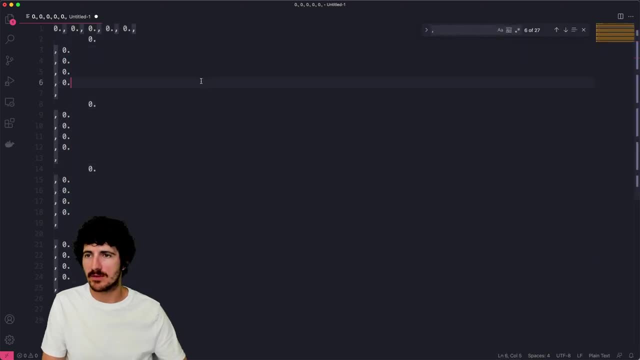 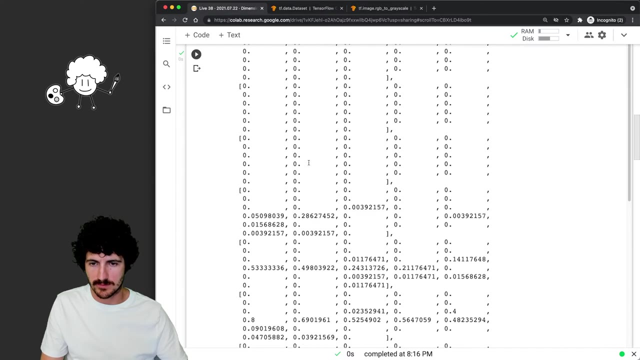 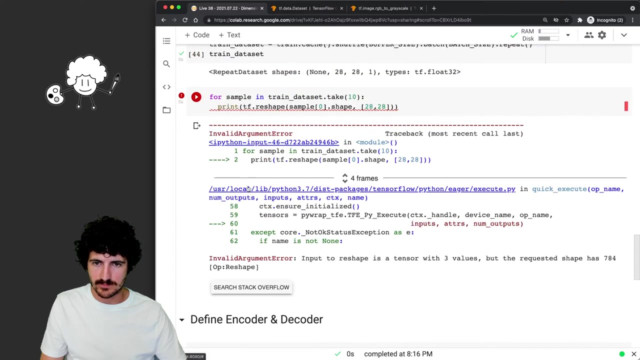 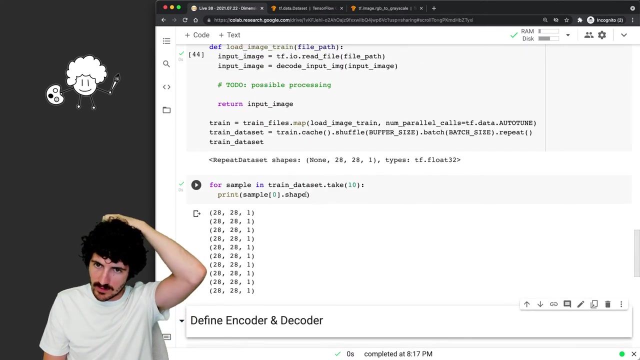 So So you're on a day: Okay, us 27,. yeah, they're 28 digits. All right, How can we reshape if we do have something that is like our data, right? So we have here the sample: 28,, 28, one. 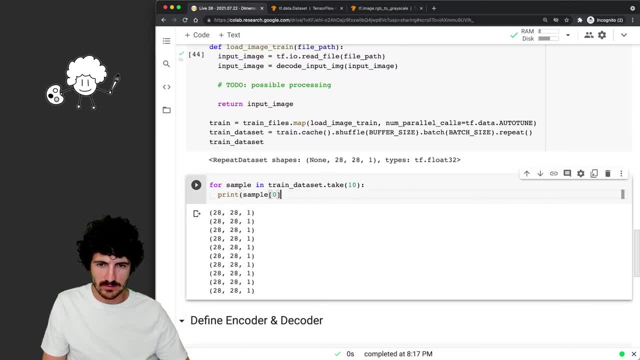 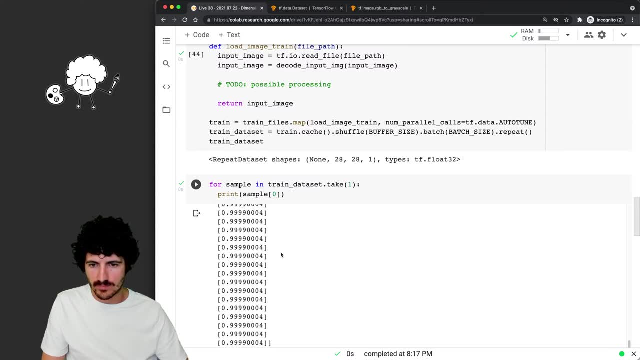 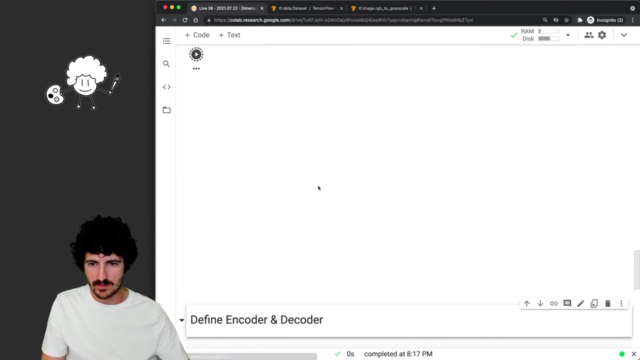 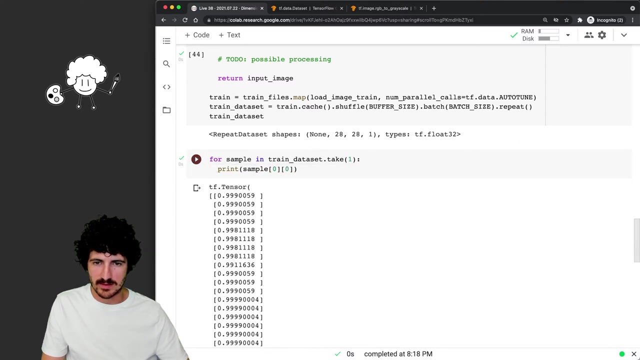 So these means let's, let's just print it, So let's take is one batch, Hmm, Okay, So this is the opposite: of expand them. Okay, That's all right. So we're going to. you need to speed this by persuasion. 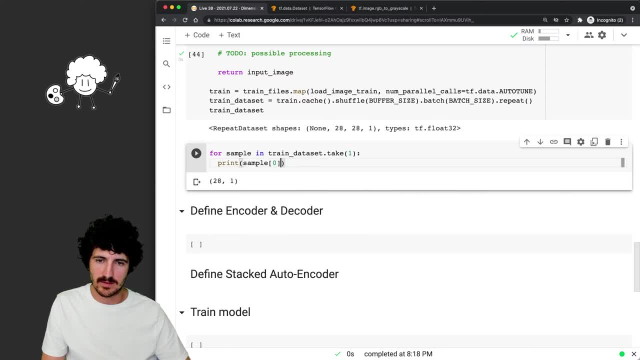 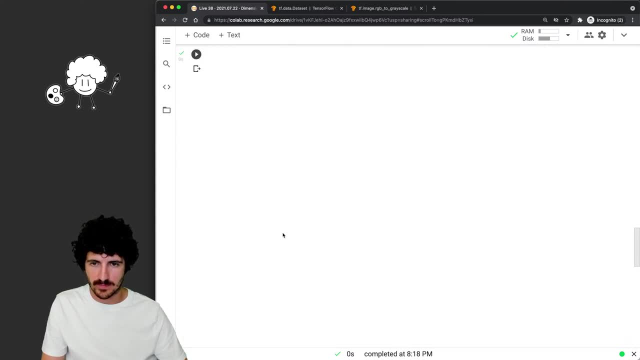 why you mess with the, the data. Okay, Okay, So let's review this by guys. Yes, Let me check. So, so, yeah, I can YouTube site. it's going to make it happen. You will get emails from everyone that I'm talking to. 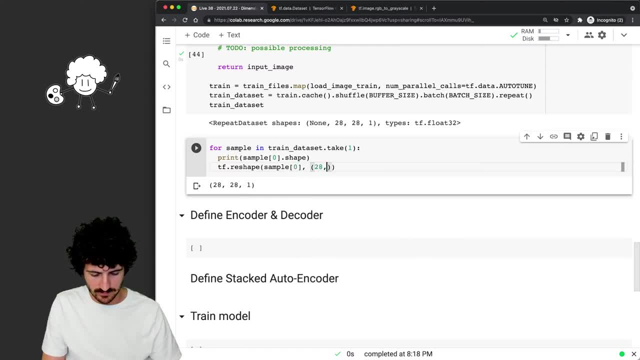 they will send you emails. that's very coming in straightaway. Um, I can share. I can share the requests and the commendations. they'll also want to go back and do the settings, everything Excellent, Thank you Okay. 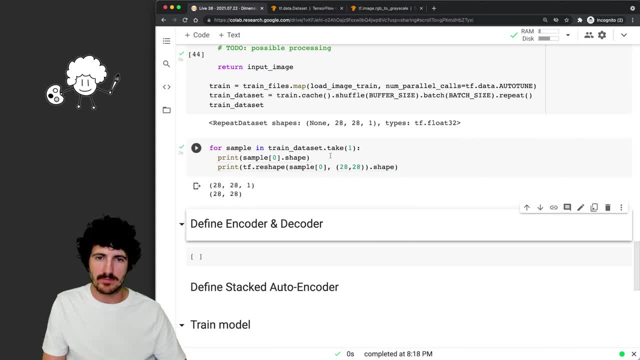 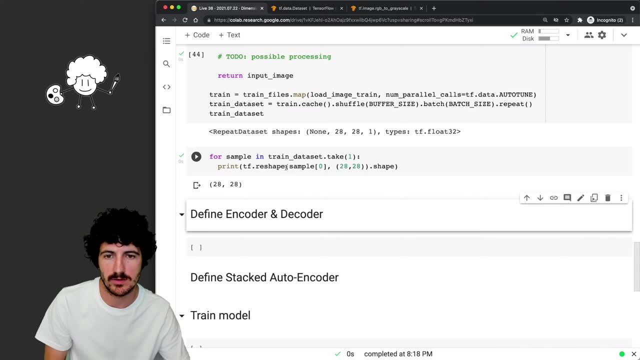 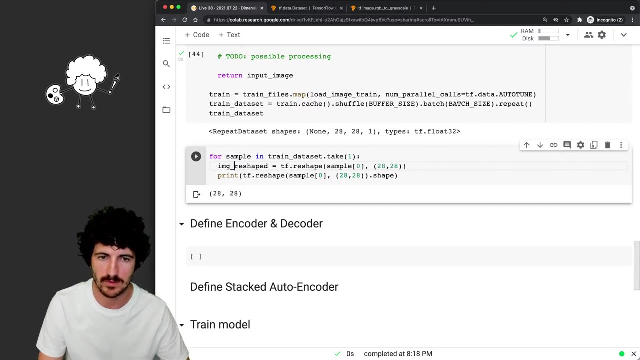 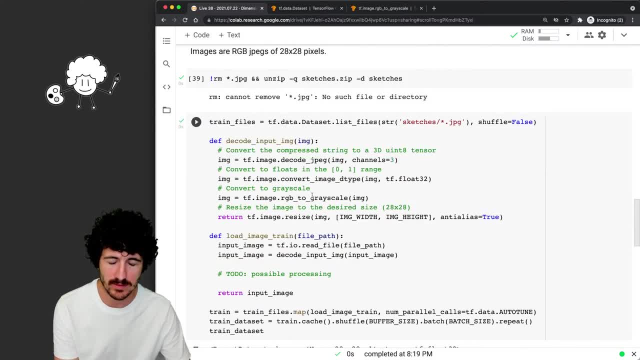 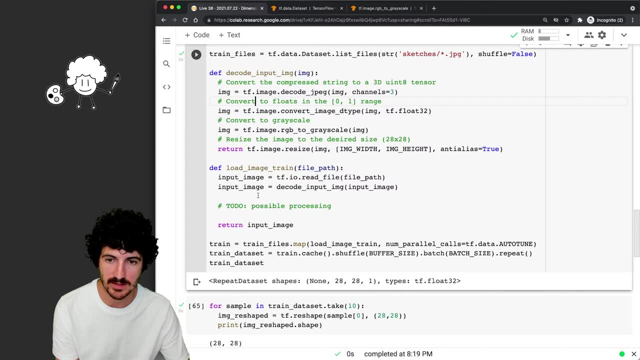 A way in which we can do that. So we probably want to, because this is: this is returning the images and here we're decoding the input. So maybe input image, here we do the reshape and we say that our input image is going to be reshaped. 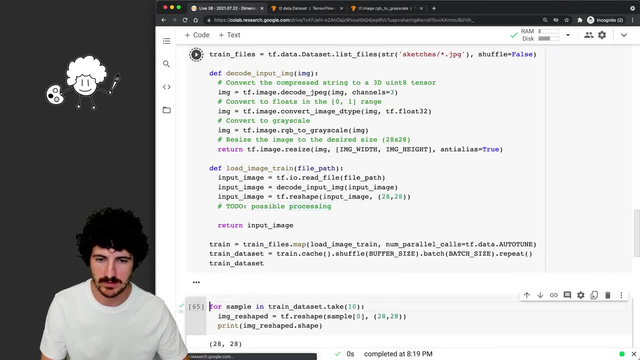 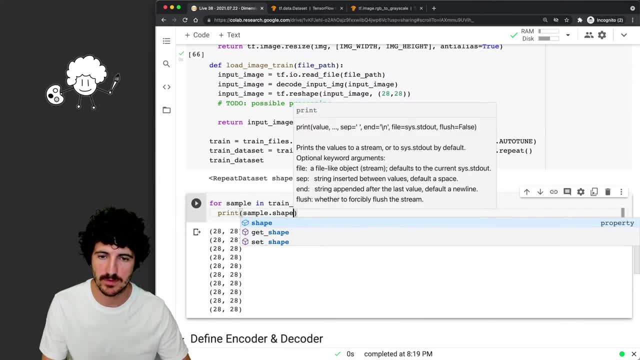 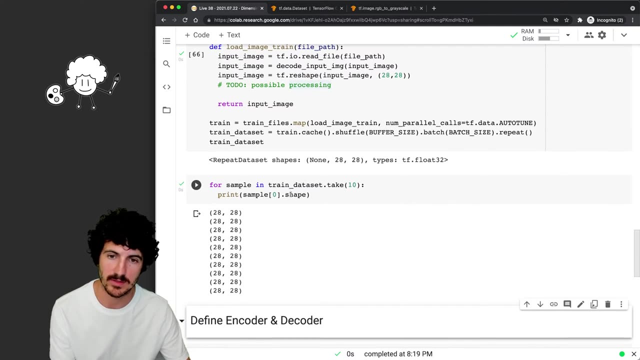 228. By 28,. let's see if this works. All right, nice. So now we don't need to do any reshaping, So we just print the sample shape and our dataset has a set of images that are 28 by 28.. 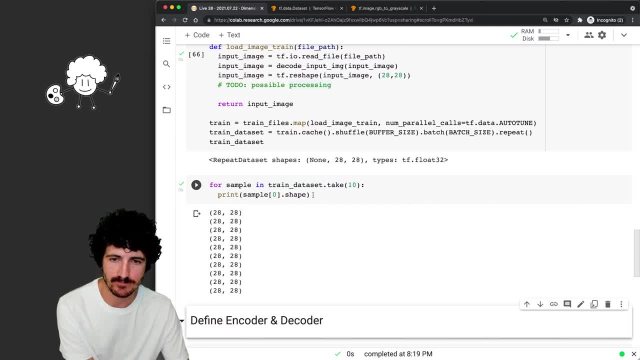 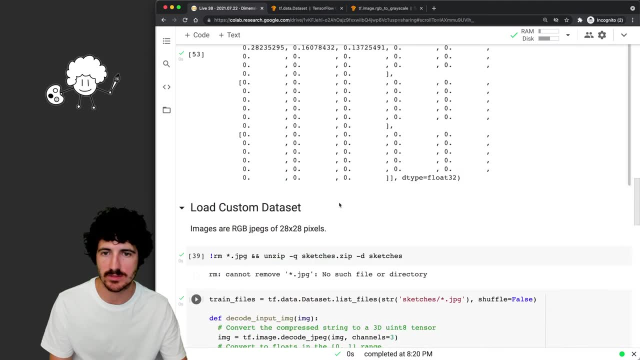 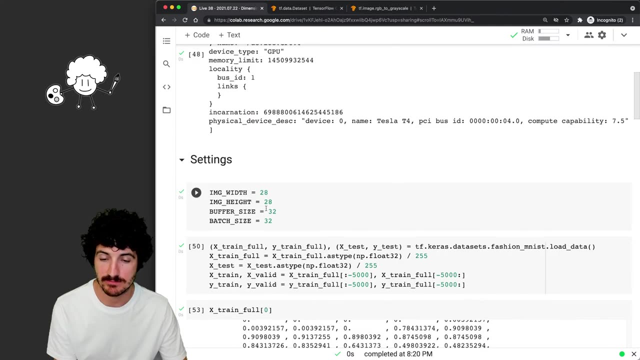 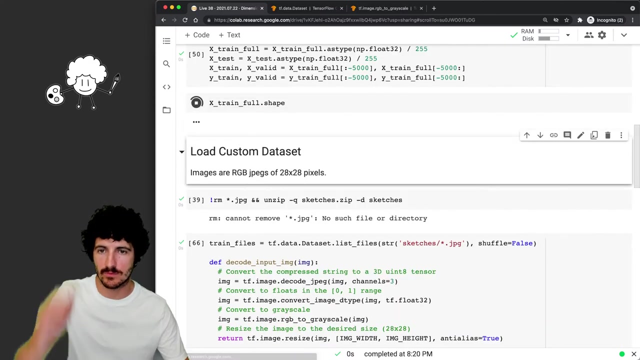 And I guess um. individually, each of these is 32 by 28,, 28, which we saw. Okay, There was um. what's the shape of this? 28 by 28 and the full is 6,000.. 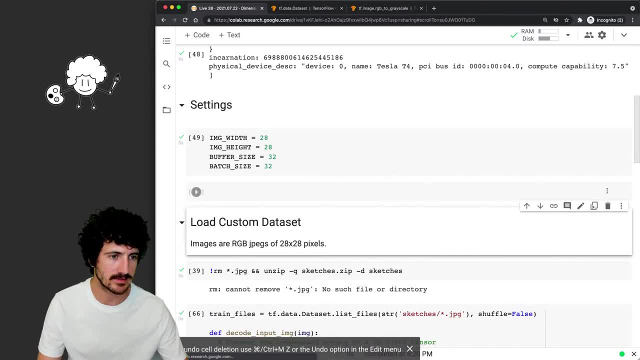 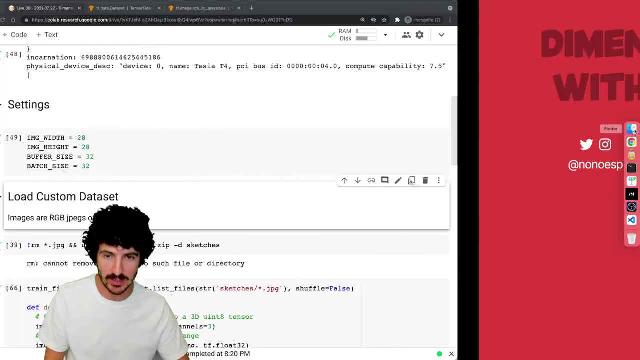 All right, Awesome. So we're loading our dataset. That's good. So we're loading our dataset in a good way that we can now use it. Um, just as a recap for those of you who just connected, we're trying to. 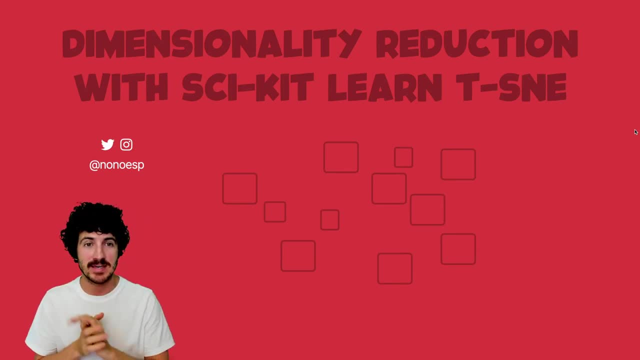 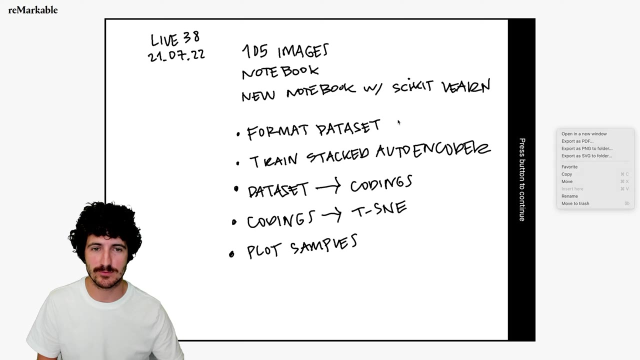 Load a dataset to do a dimensionality reduction exercise with the t-SNE implementation that comes with scikit-learn And you know we've gone. uh, we're trying to be here, So we're on on these. um, Oh, push button to connect. 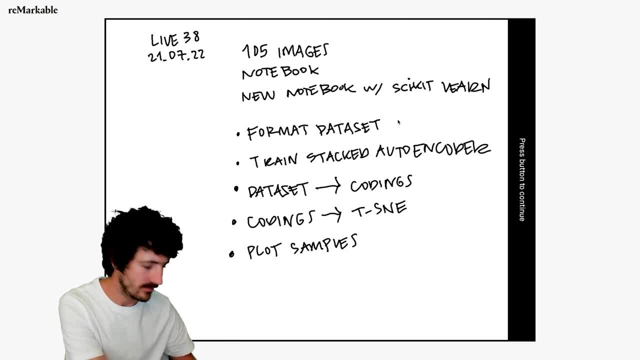 Okay, So we're trying. um Hmm, Not sure These might have got 10 disconnected. Okay, So we're trying to um, Hmm, Let's see. Okay, So we've got a little bit of a delay here. 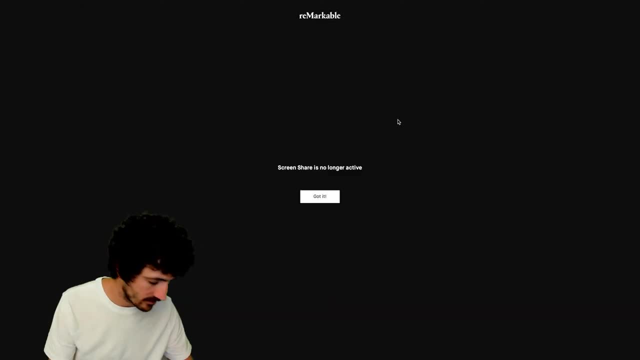 So we're trying to do a dimensionality reduction exercise with the t-SNE implementation And we're trying to do a dimensionality reduction exercise with the t-SNE implementation. So we're trying to do a dimensionality reduction exercise with the t-SNE implementation. 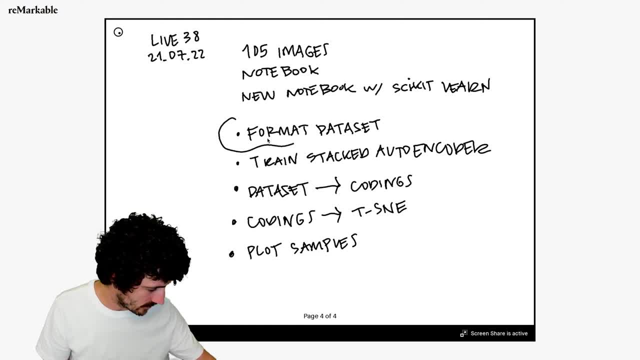 Okay, Back now. Great, So we're trying to do this right. So format the dataset and later we get time, we'll be there, but We'll have to continue with this series. I don't know how to make sure that. 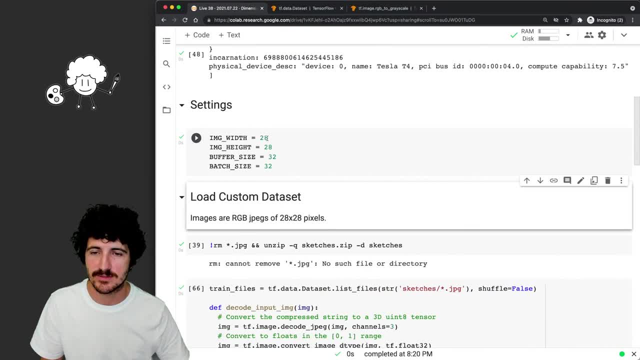 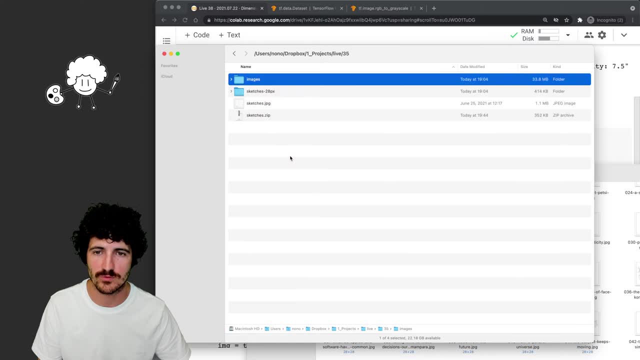 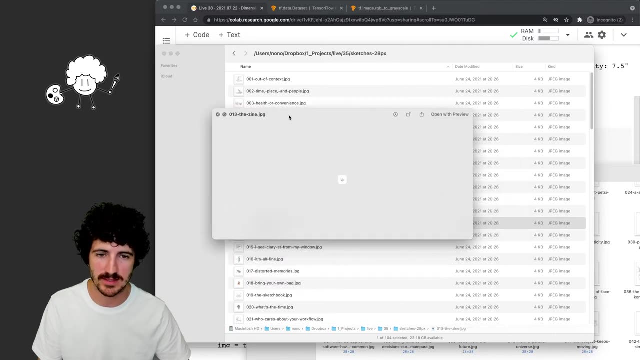 Uh, this is something that we can finish, All right, So we're loading these images in 28 by 28 size, So two really small to see with your eyes, right? These are super, super, um small images that are pixelated. 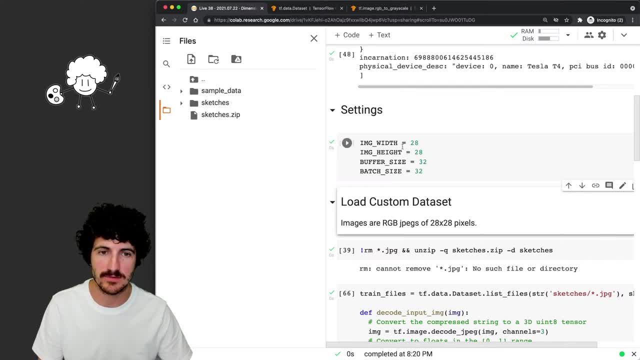 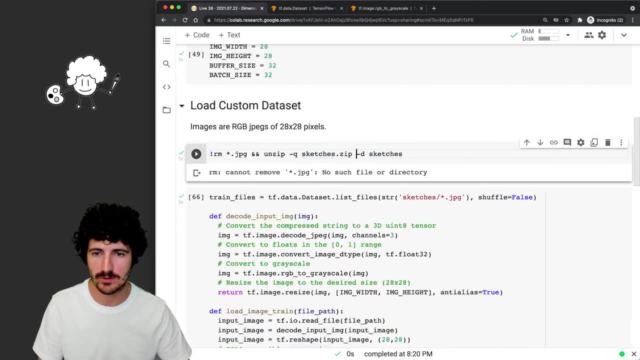 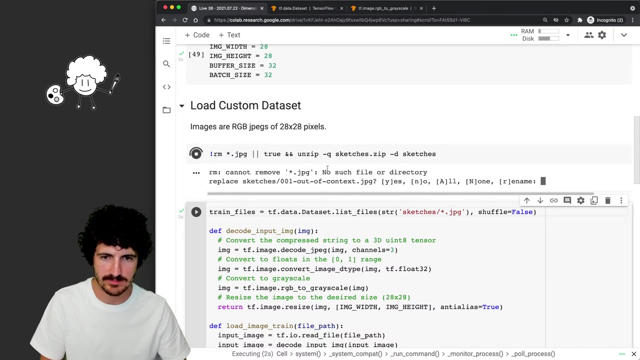 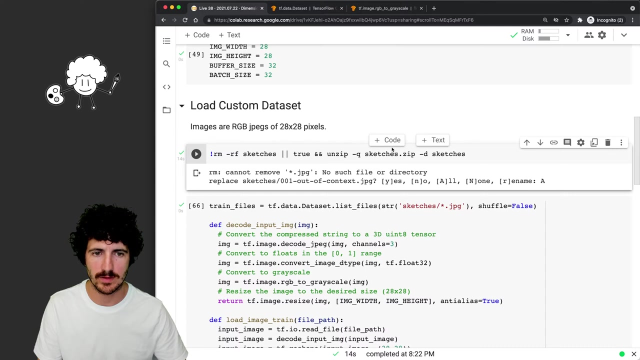 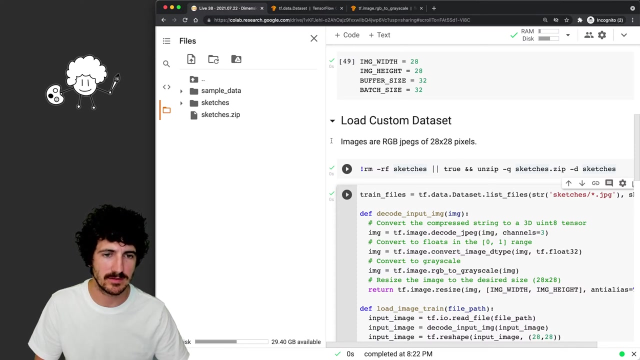 Um, we drag and drop those two here as a zip file. So we, you know we unzip that with um with here, So we unzip those files. All right. So probably we can run this now. So these removes the folder and then unzips, right. 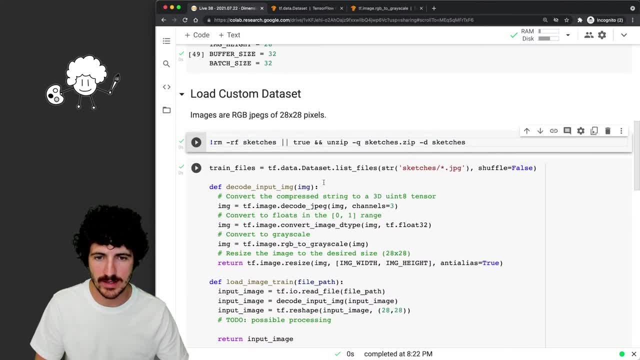 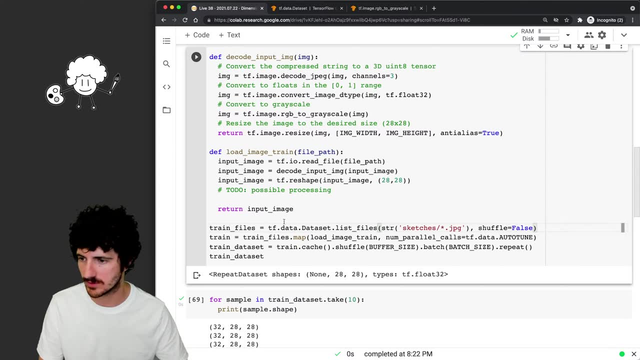 All right, So great So we load the data set here. Uh, we actually don't need to do this year. We can put these functions: Hello Lourdes, Nice, to see some familiar faces online. Um, great, So we have the data set here. 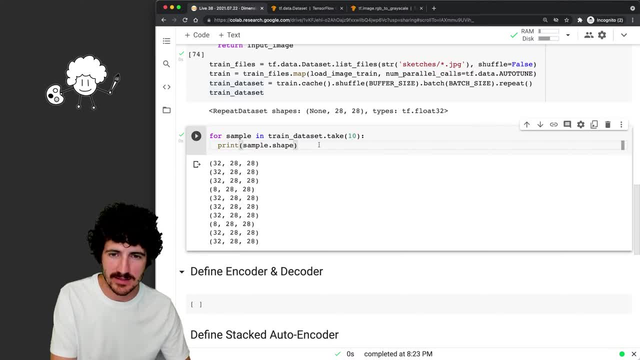 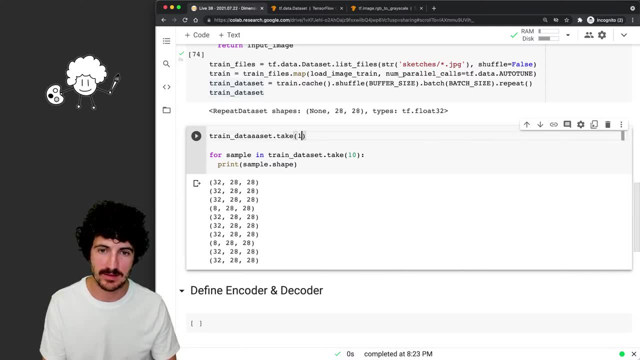 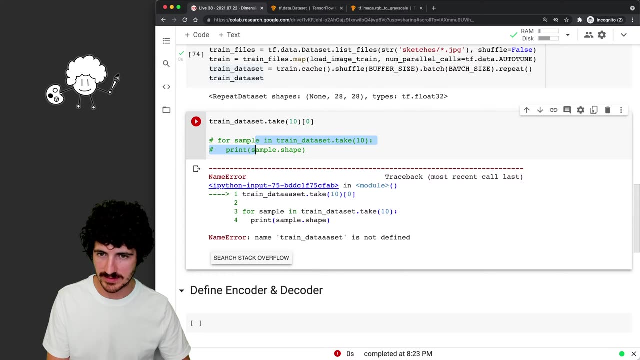 So We're loading that data set in here We can load a set of uh things. So if I do train data set, take 10 and I get the first one. let's come in this out. Take that to say it's not so scriptable. 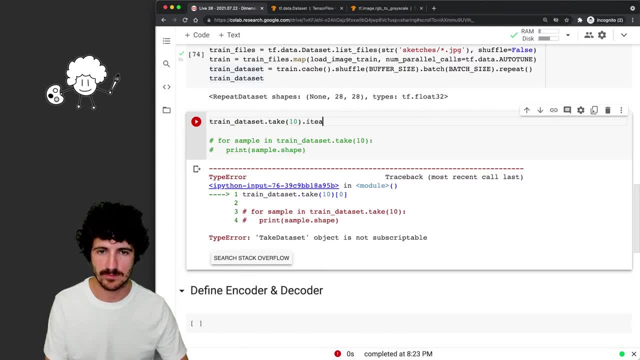 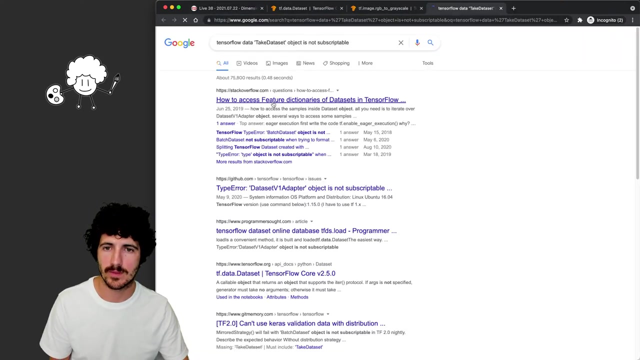 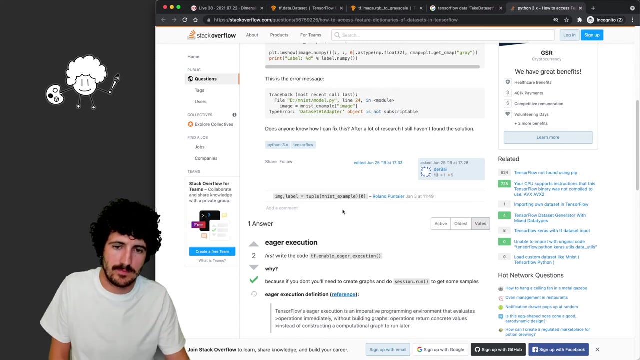 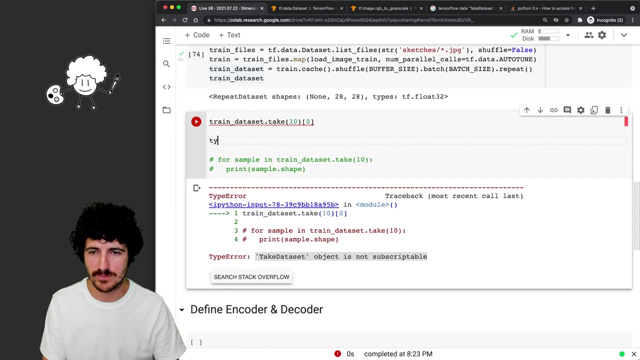 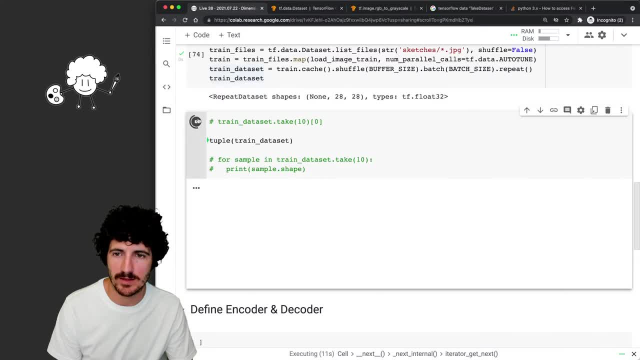 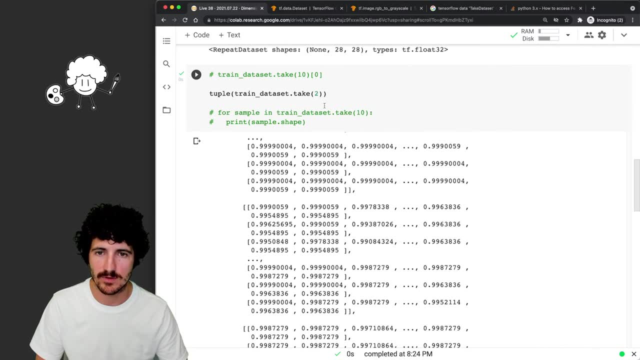 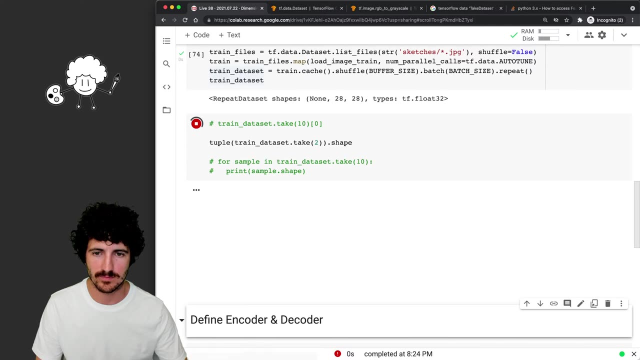 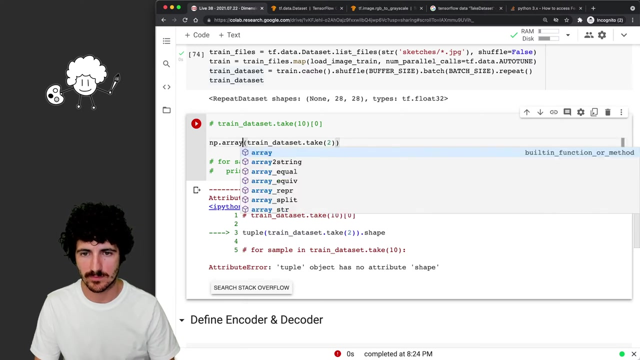 All right. So, or maybe we made that on an object that is not going to end up any time, So maybe just make it into Awesome. So let's see shape. Ah Okay, Let's make it. Conversion set is working in a way that it would not have chopped off. 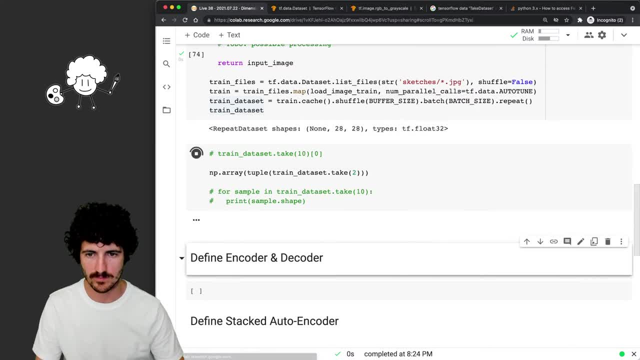 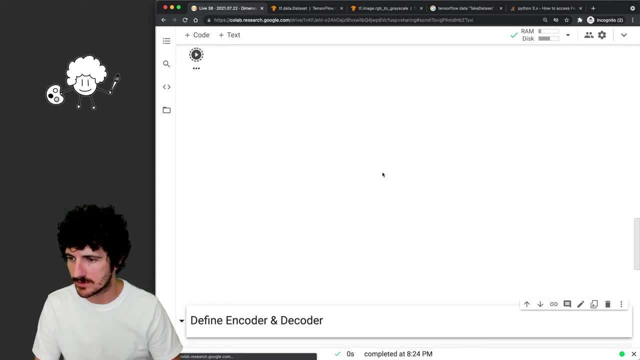 So practicing that Pronounает sort of error andgeordient relationships or whatever. that's what we're getting. is it wanting to change that space? Okay, Yeah, Awesome. So let's see shape convert to tensor, Right? I don't know this. 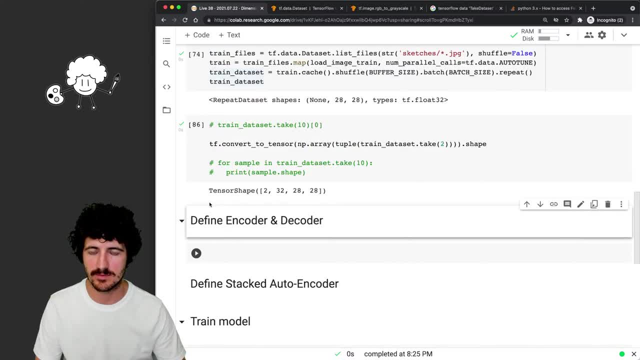 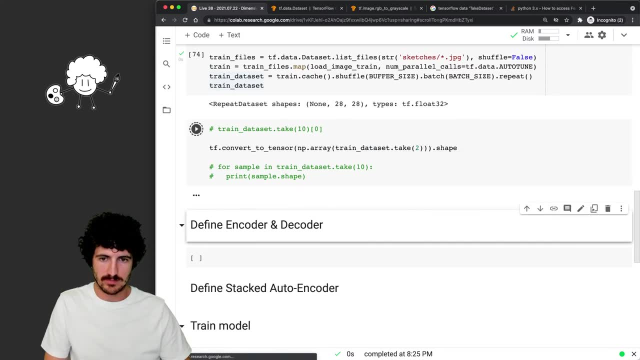 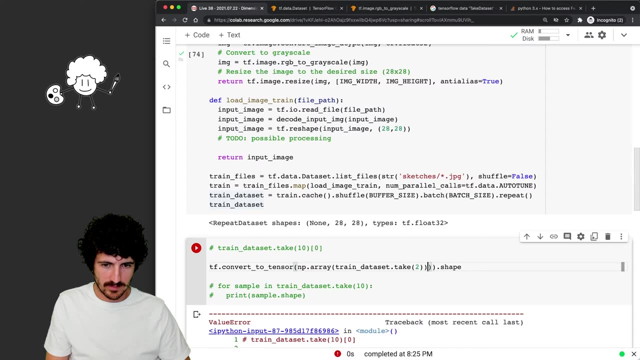 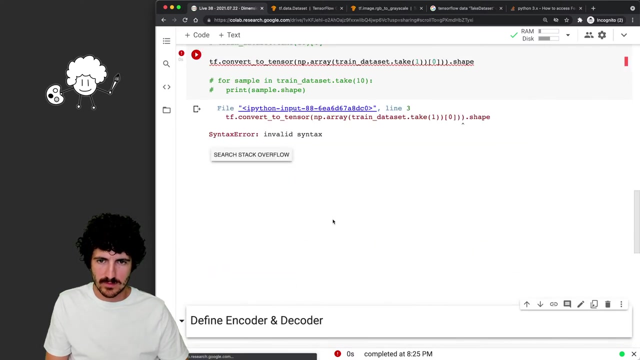 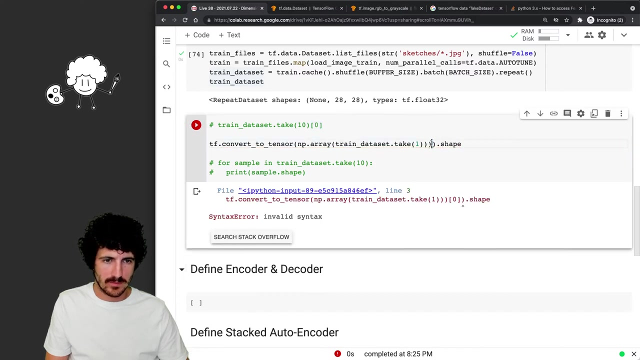 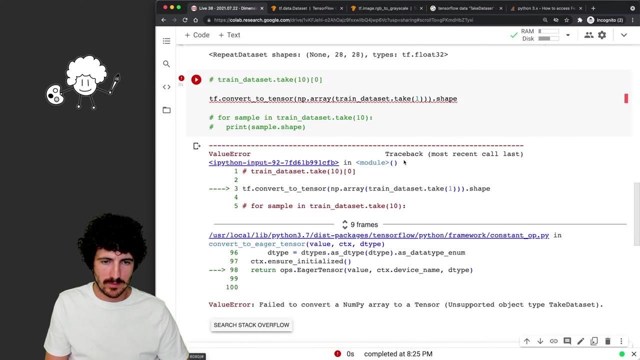 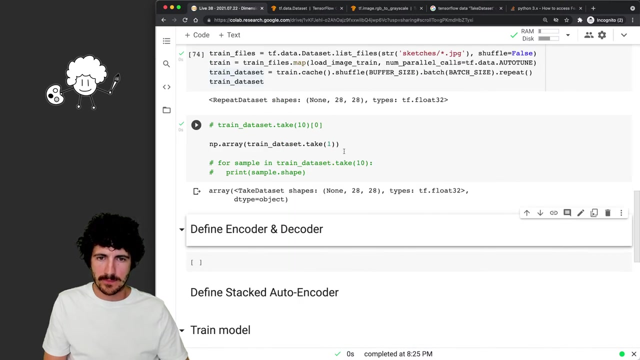 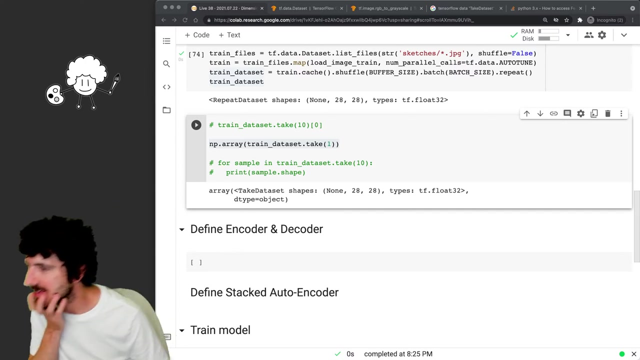 This seems a bit like a hack, but I might get there to, maybe not. Yeah, All right, All I'm trying to do is get the, the, the, the two items. Thank you, п impacto. Okay, wait for that. 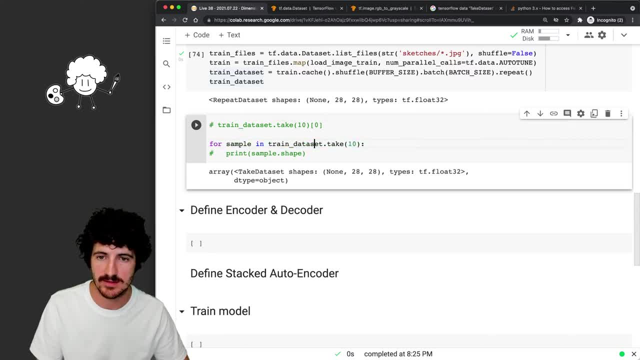 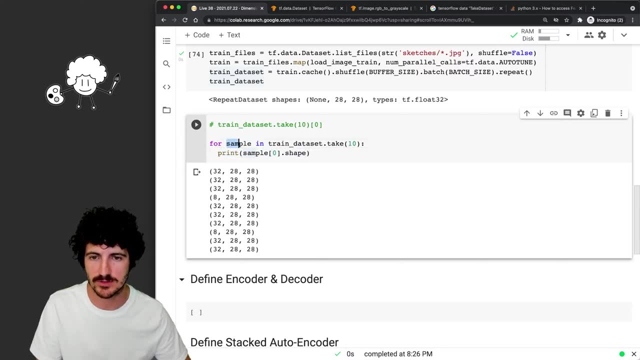 Yeah, All right, data set that we have here, right. So we have a data set and, um, you know, if we get the, let's say the. so let's say so this is, this is actually a batch on our data set. 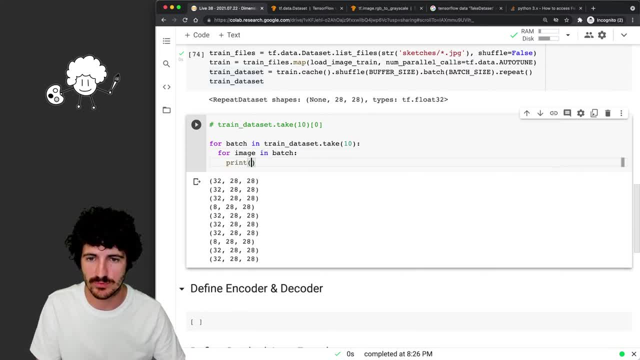 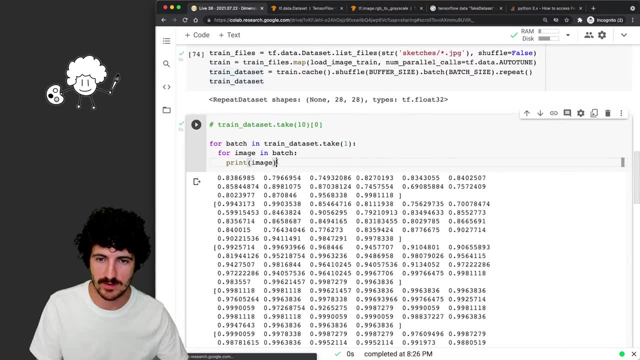 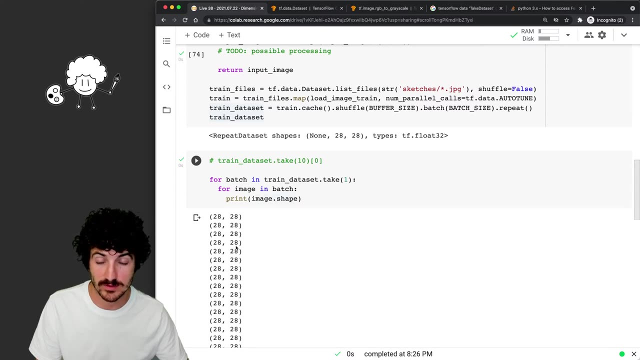 So for image in batch, we can print the image and maybe we just take one batch, Right, So we have the image. shape is 28 by 28.. Um and uh, we could actually plot this, So just to visualize it, but we're not going to do that right now. 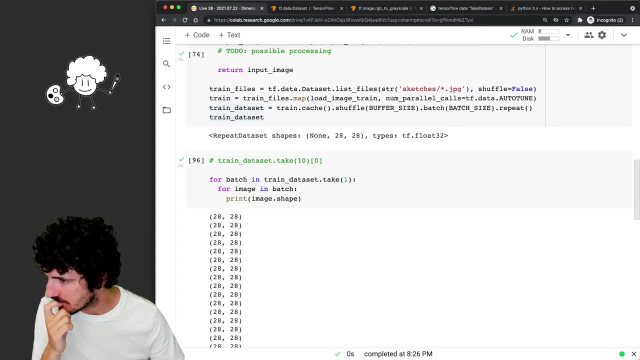 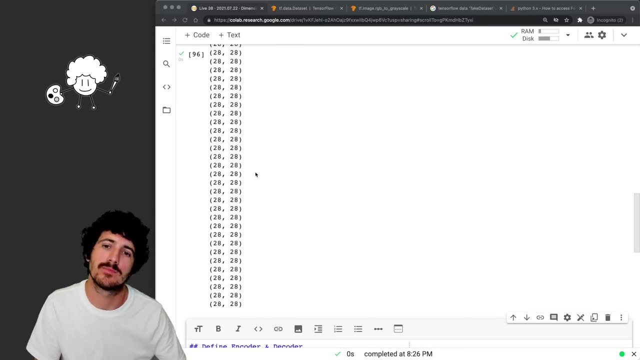 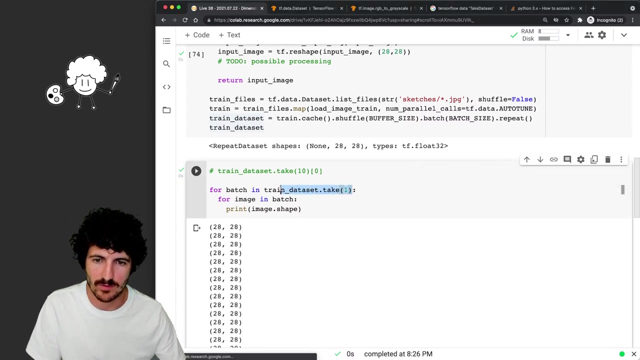 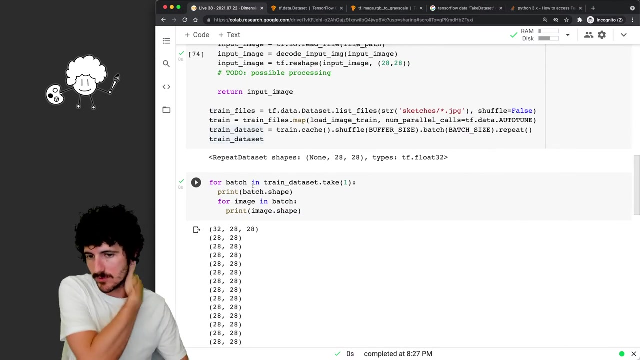 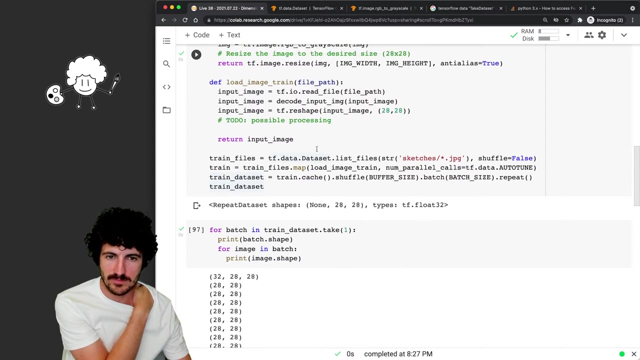 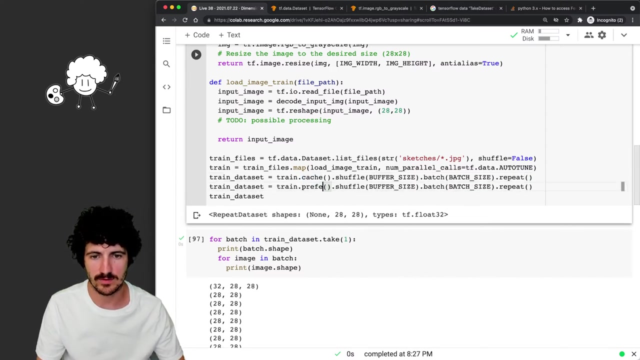 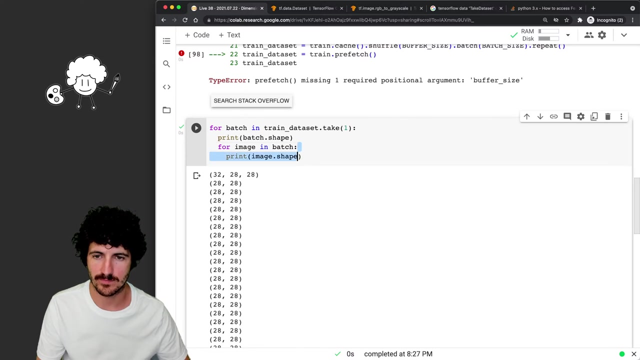 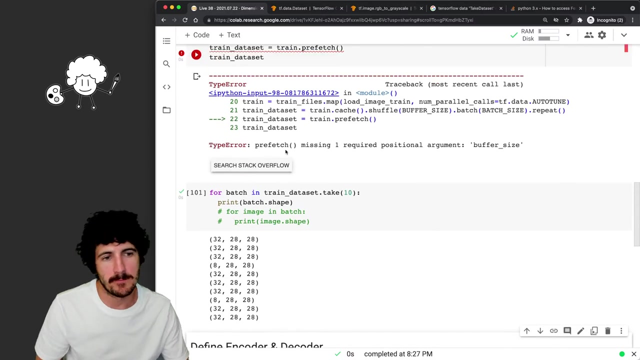 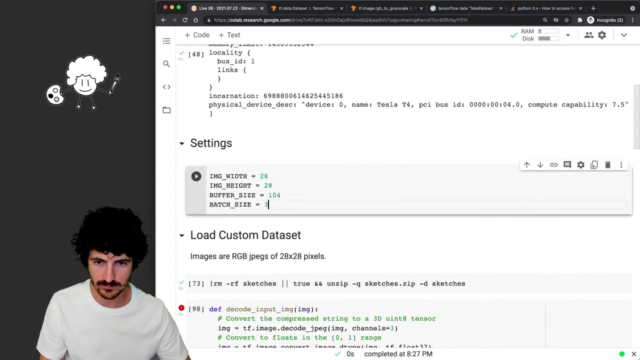 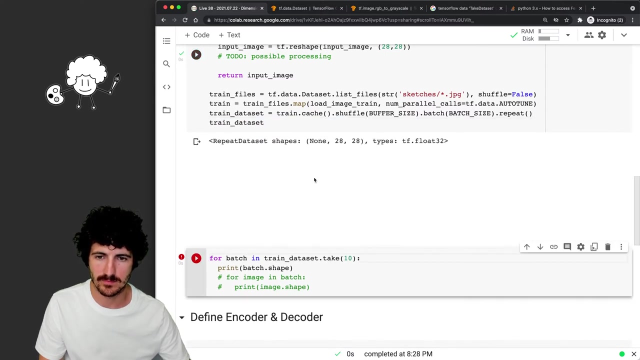 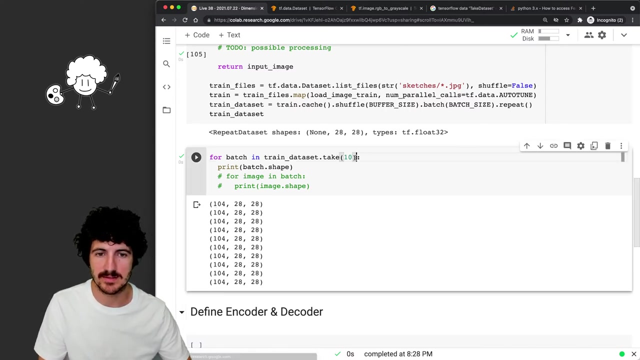 Um, Okay, All right, Let's see. Let's see what we can get. So, Right, All right. Um, I'm not sure if I can do here a prefetch. Okay, so here I'm getting at least a batch, so we can say: can I get just the first batch? 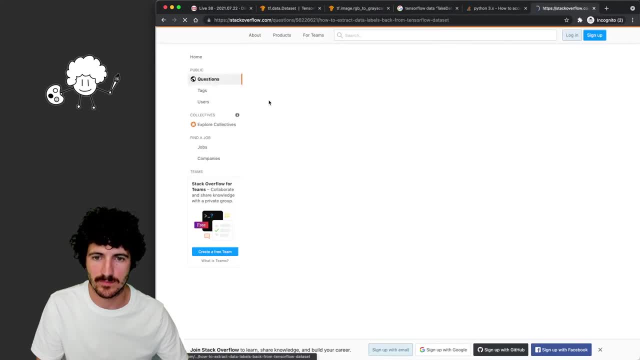 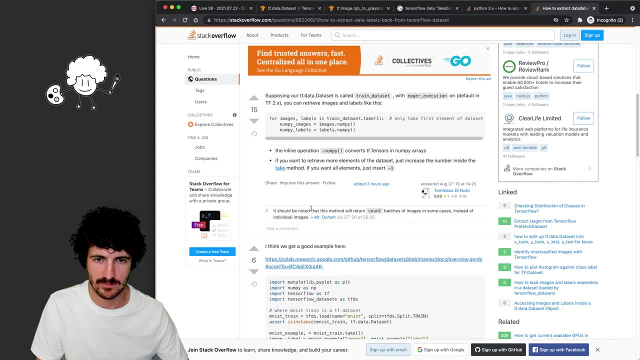 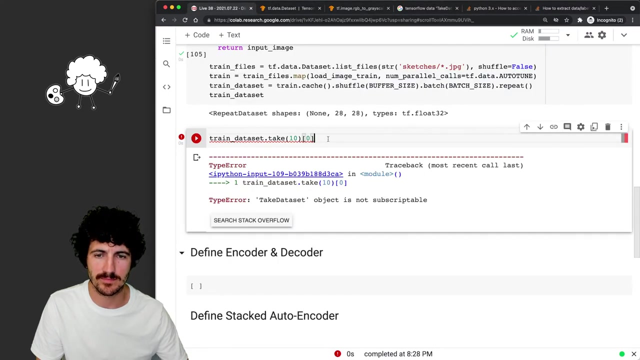 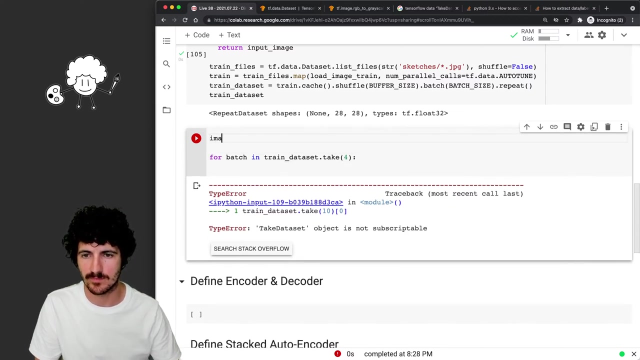 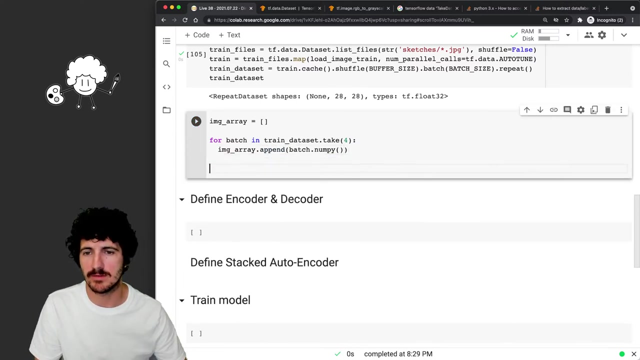 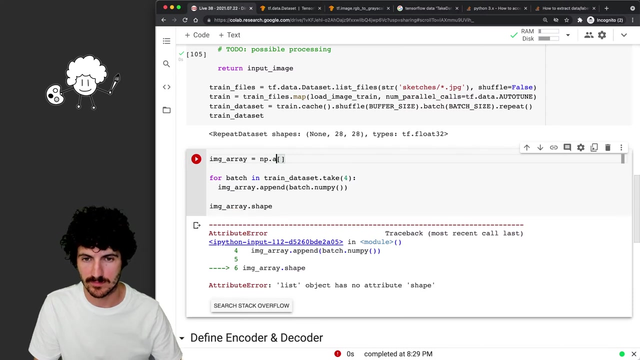 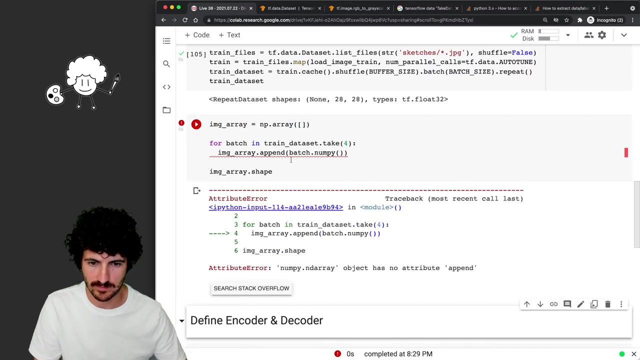 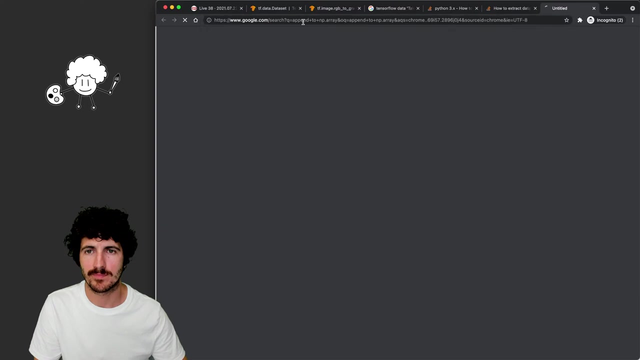 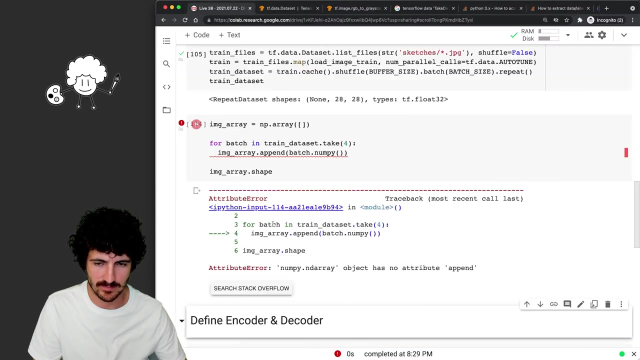 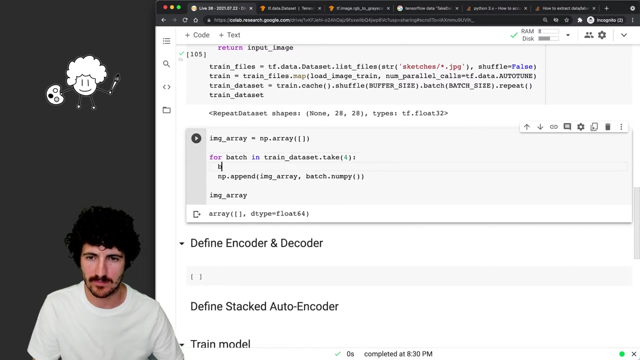 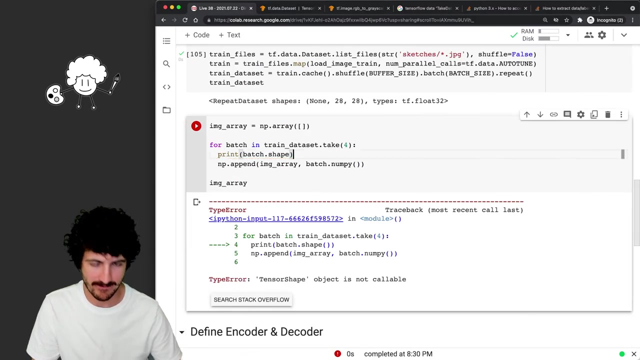 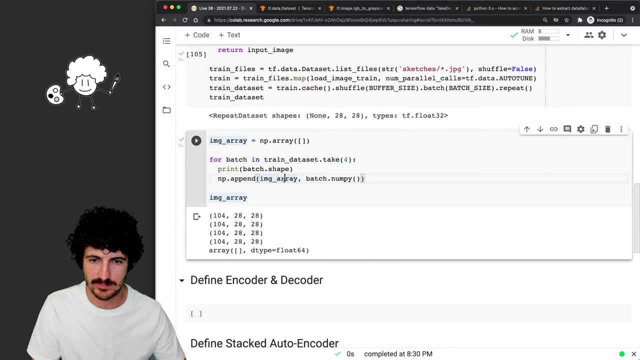 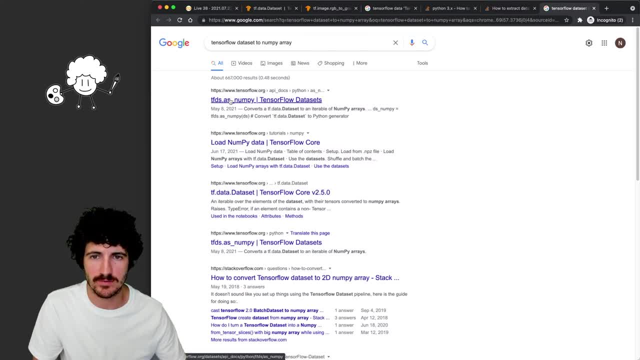 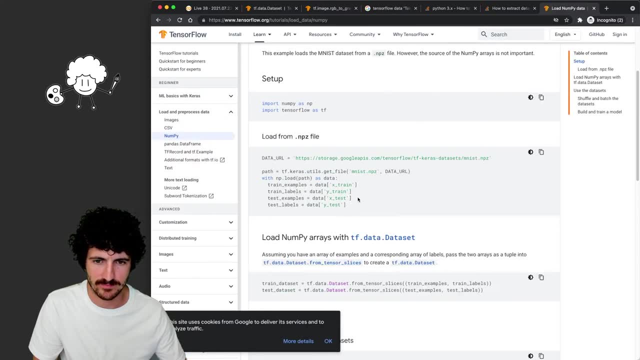 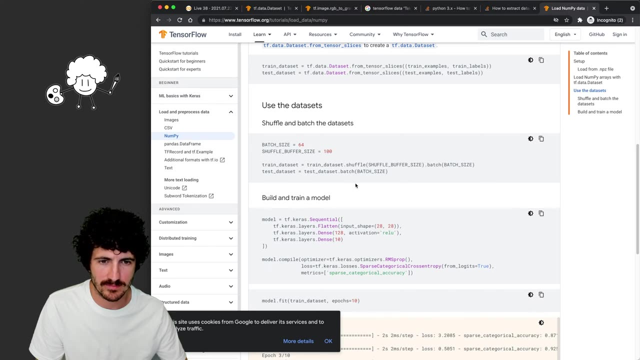 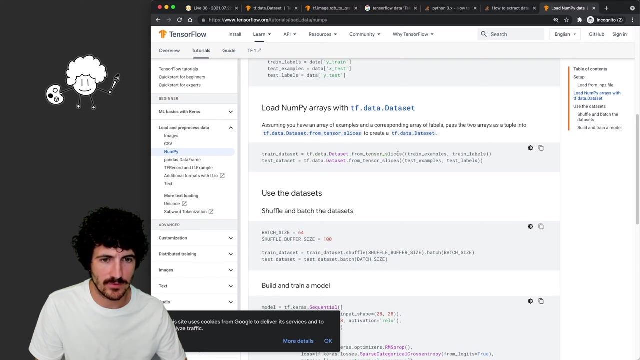 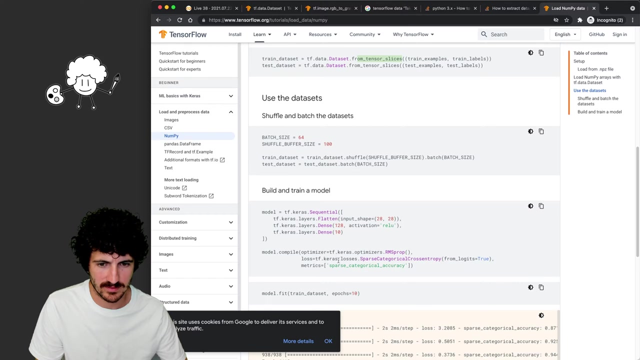 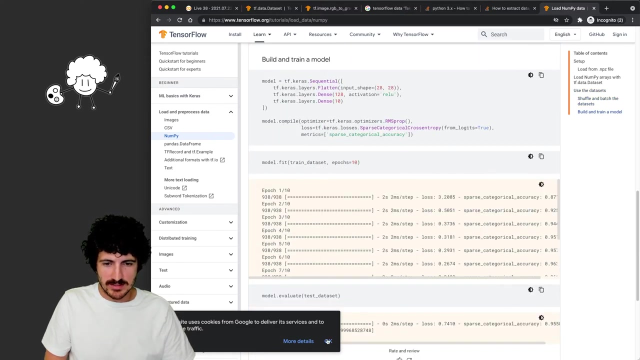 I'm really always confused why all this doesn't really work. but non-py data, Intentious laces, train data set shuffle, but I don't know. I don't really understand. I mean, we were probably able to simply use that. 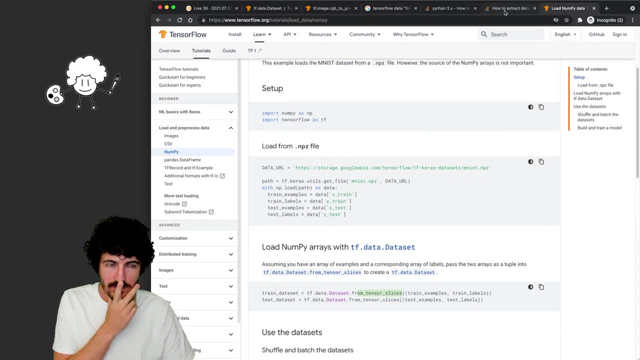 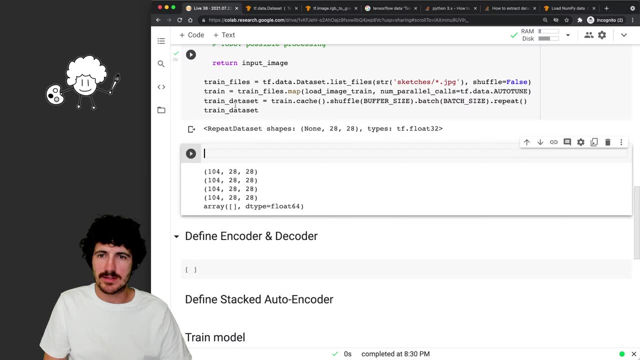 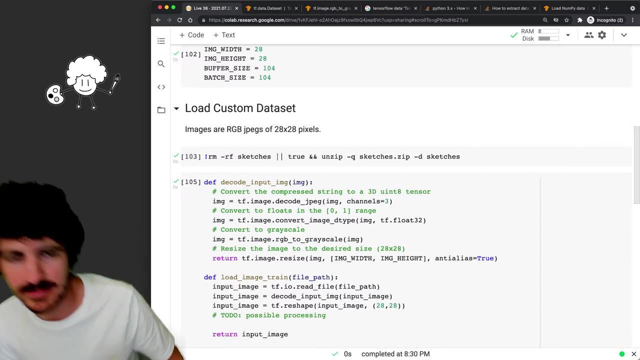 All right. So we have the data sets, We have the train data set. We can train with that and it seems like that's going to be okay. Um, let's take a look. So where are we? So we have, we have to so format the data set. 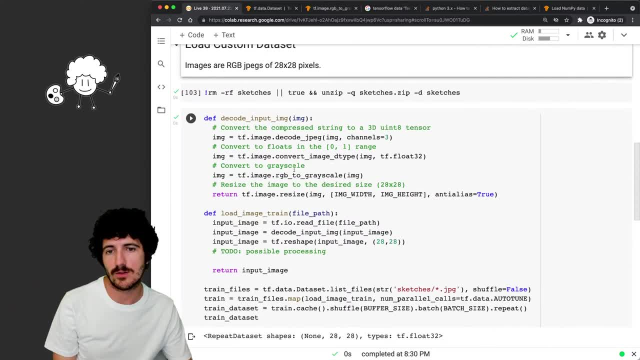 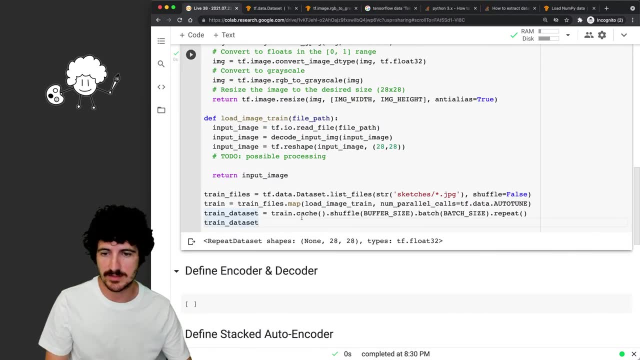 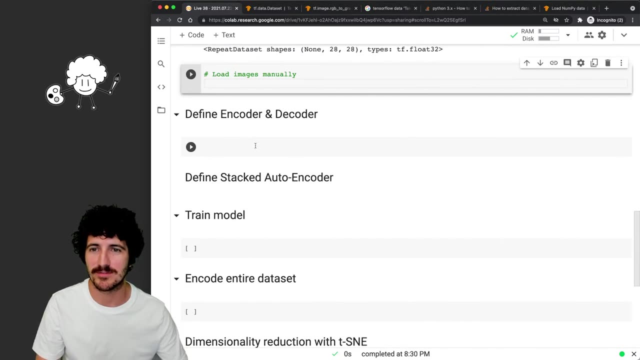 I want to get at least a few inputs loaded manually. So I would say: Load image train. Um so let's say we just load the data manually, So load images manually. We've been here for half an hour trying to do in a different way. 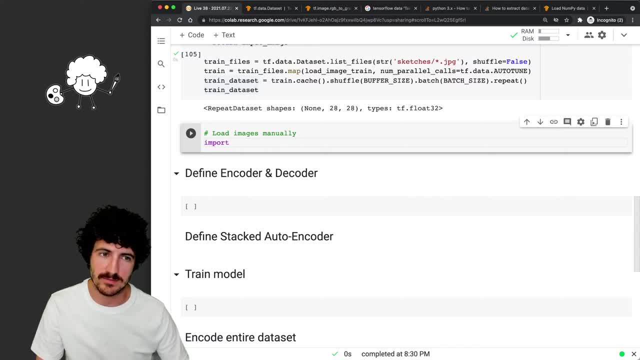 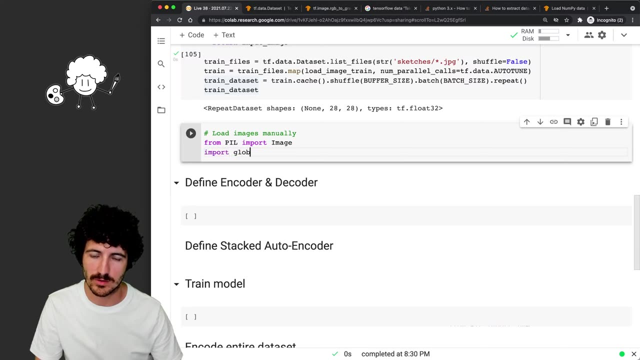 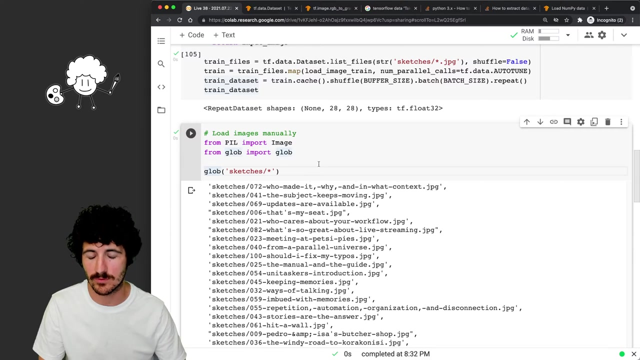 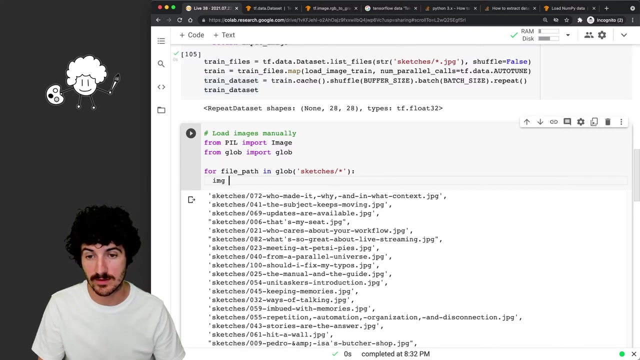 So I can say: import um so import. so from pill, import image. so we can do: Uh, import glove, from glove, import glove, I think. so We do glove sketches. We get all the paths right. So for file path, in this we can say our image is going to be image, open file path. 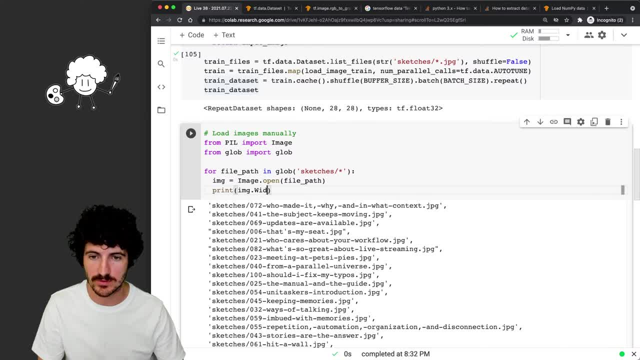 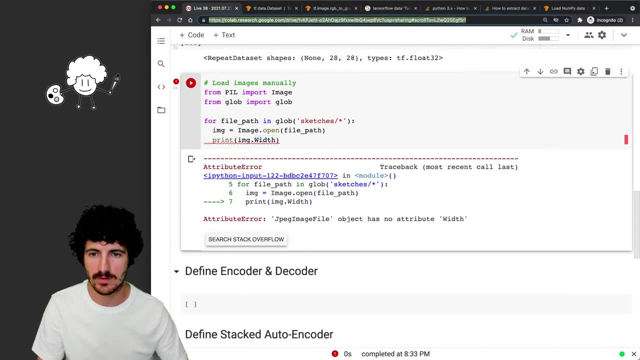 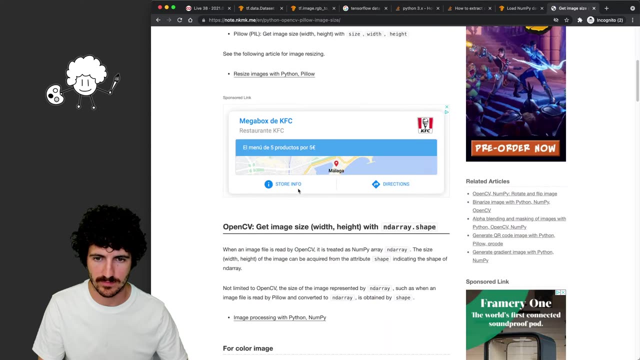 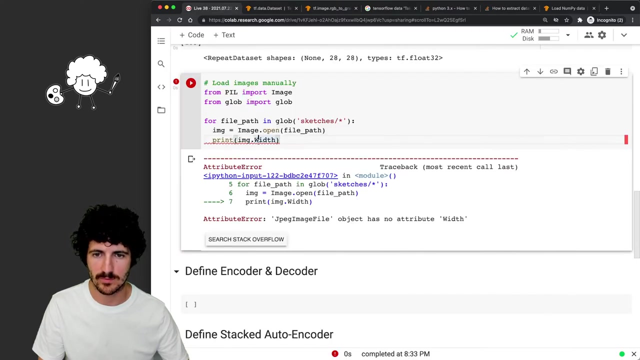 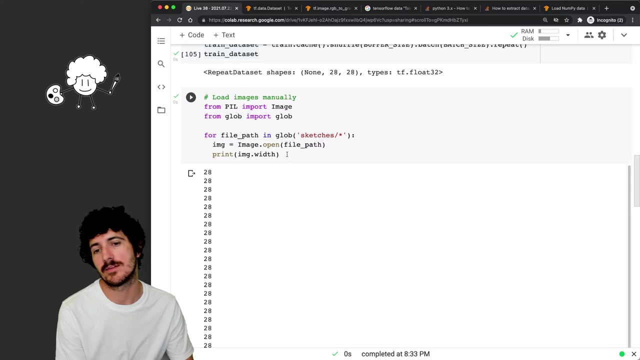 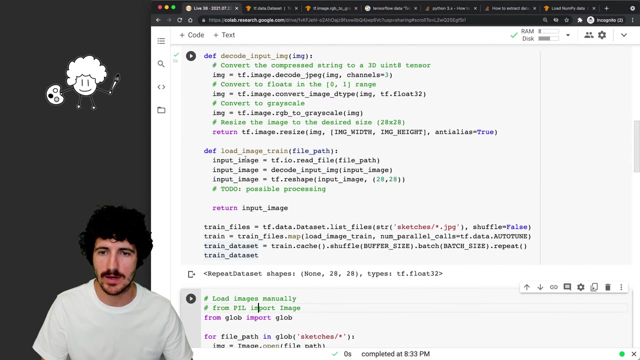 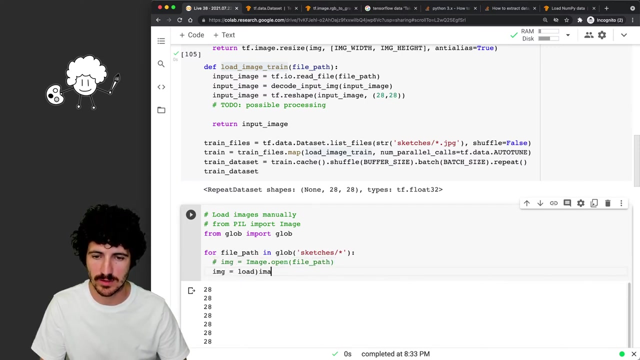 Okay, And we can print, for example, the image with image size. Okay, So maybe just lowercase, All right, So it's 28 by 20.. That, that seems to be Right. Um, well, once we have the bath, actually, even if we don't use bill, we do have this load image train, so we can do um image equals, load image train, and then we put here the, the file path, and then we can say: print image shape, right. 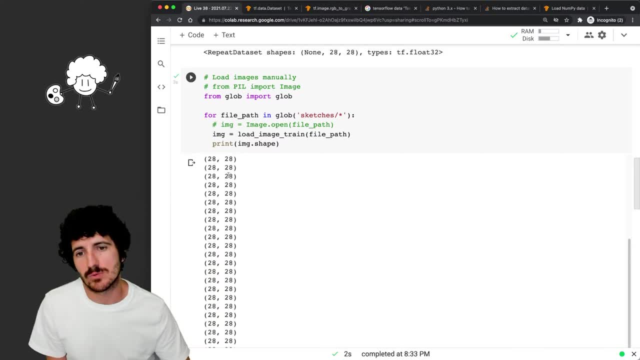 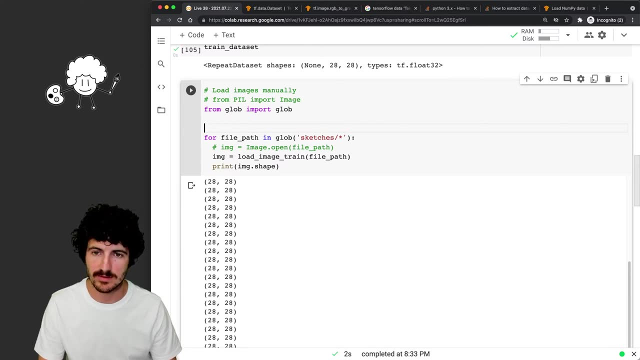 So we get images that are 28 by 28.. That's well, so, um, we could say, okay, our like, let's say X train full, could be that, And we just do: um X train full, append and this image, and then we print X train for. 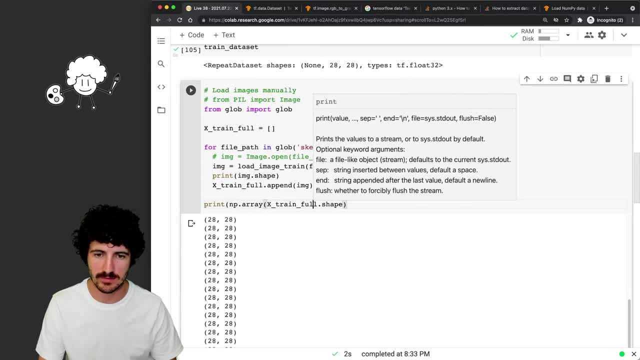 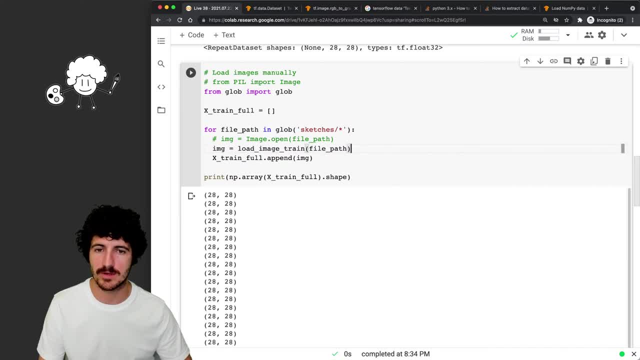 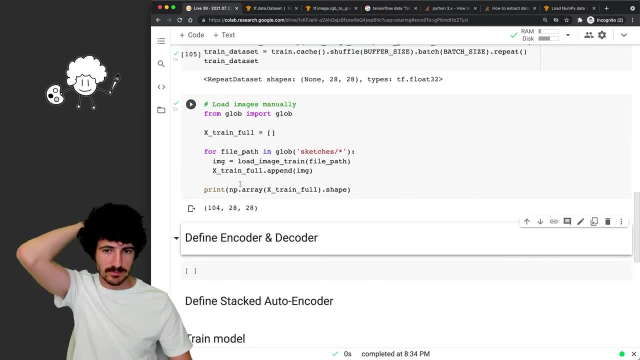 We don't need to to print here, So we're just appending. We don't need pill, Right? So this is what I wanted to do. I didn't want it. I wanted to try to do it with um, with the TF data library. 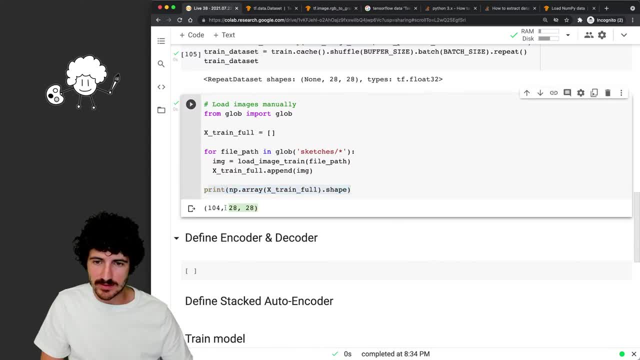 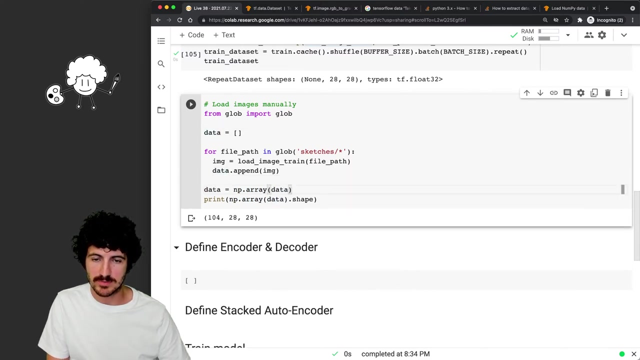 And once we have these, these are also black and white. These are the the type that we want it And, uh, so we could say: um data, So DCs, so our data is going to be this right. 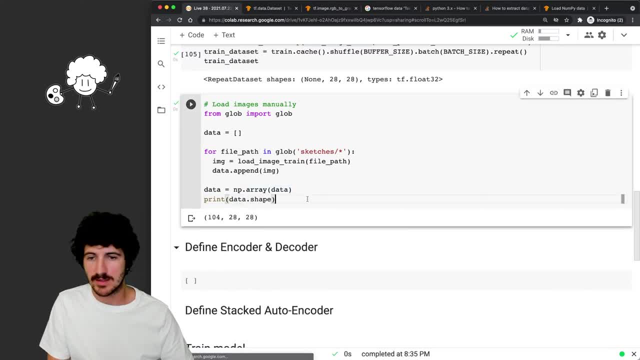 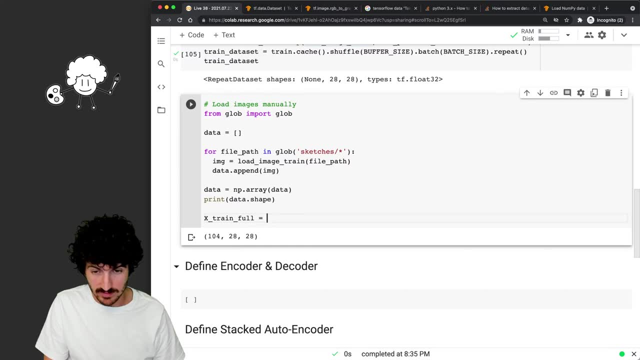 And then we can say, okay, we have data on the shape of this And, uh, because we don't have more data, we're going to have to say X train full is going to be um, so a hundred and five, 104.. 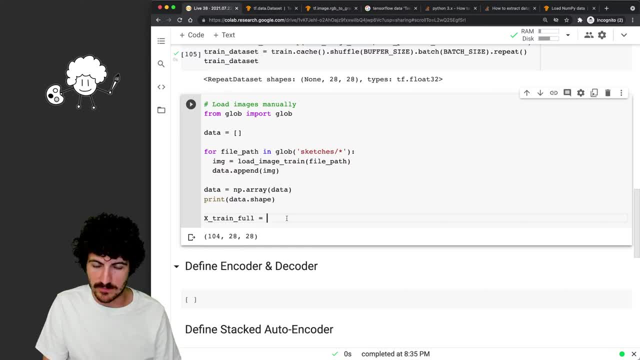 I'm not sure why it is a hundred and four, Yep, Yeah. So um, we do here data and we get the first, so 104 multiplied by 80. So let's do 80%, So 80,, 84,, for example. 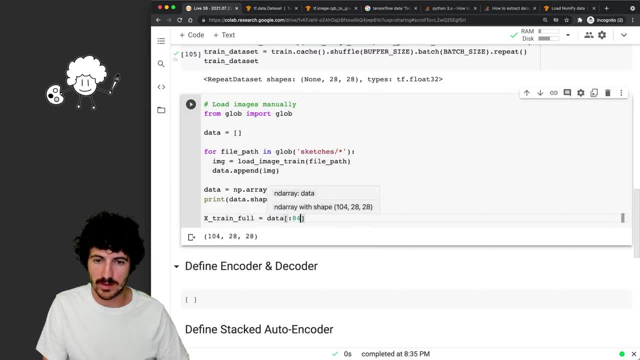 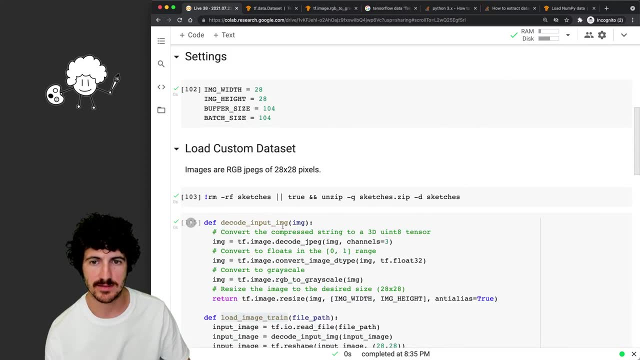 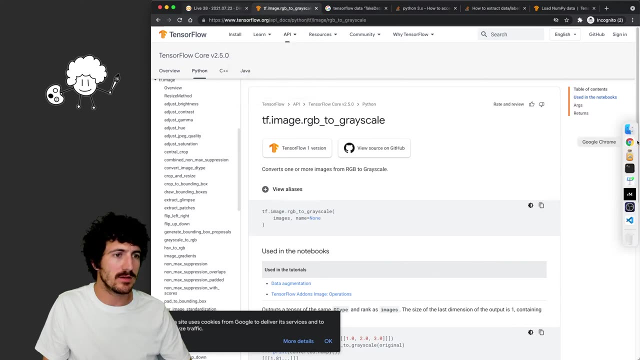 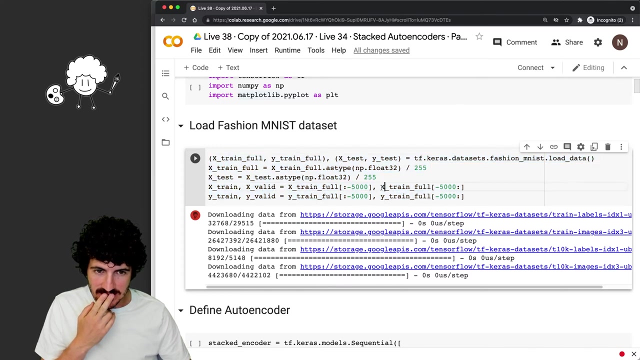 And do like minus 84. So we leave 20 X, Bob, and, and we just want to see the- let me just close everything here. We just want to see the validation. It's the same, Okay, So, um, therefore, we need to say okay. 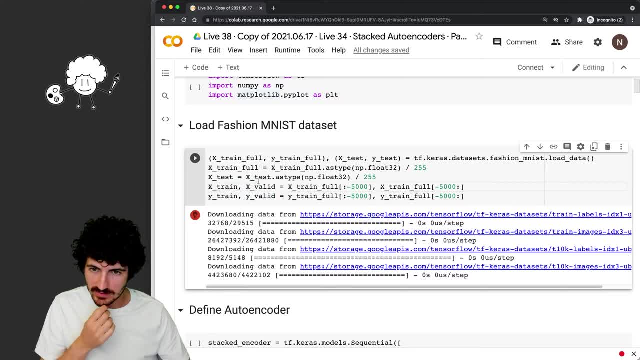 So, no, I'm left doing a communique, right, I'm leaving, but I think we do have a trade law which you could hit, like all of the, within the control option. All right, So X train full is going to be. just is the data. 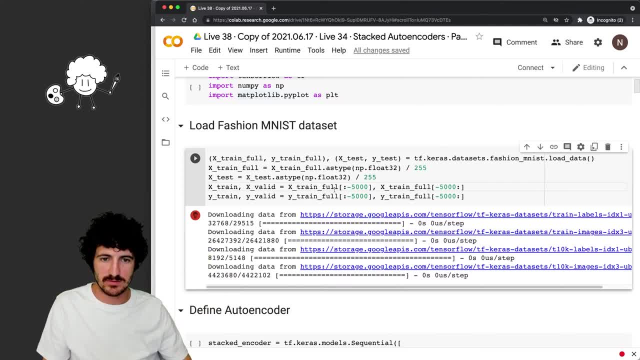 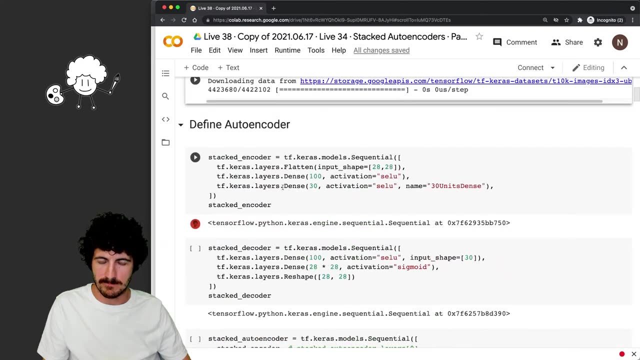 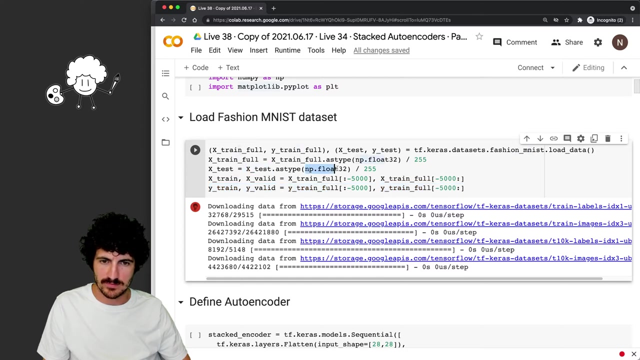 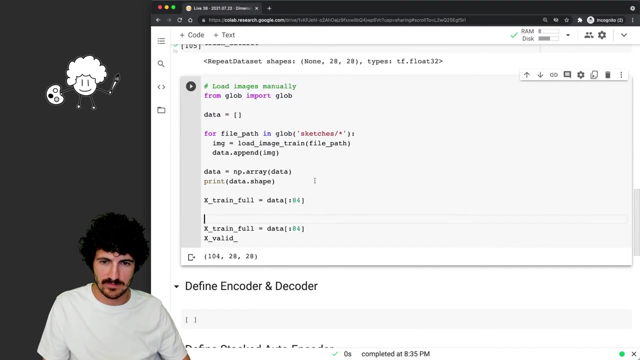 And why train for? Why does that? Oh, I'm Christine, I'm sure what the Y is here. Hmm, All right, So X test type. Okay, That's important. So we get here, we get the X train for zero. 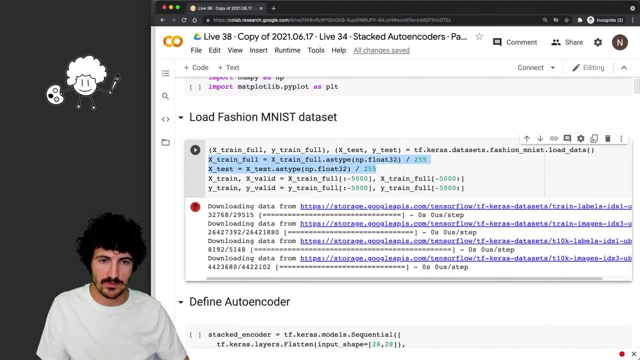 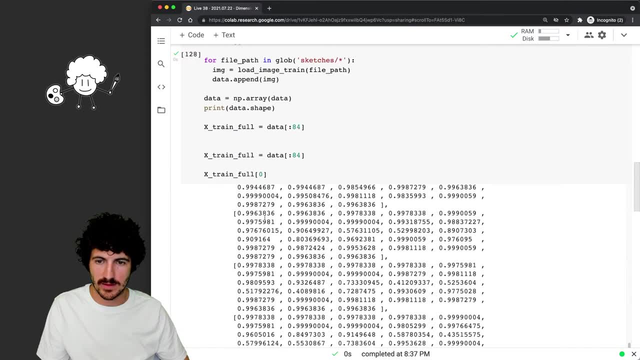 They're already converted to D type. That is what they're doing here to flow: 32 divided by two, 55. That's what we were doing here, So we don't need to do that. So all the data is all the data. 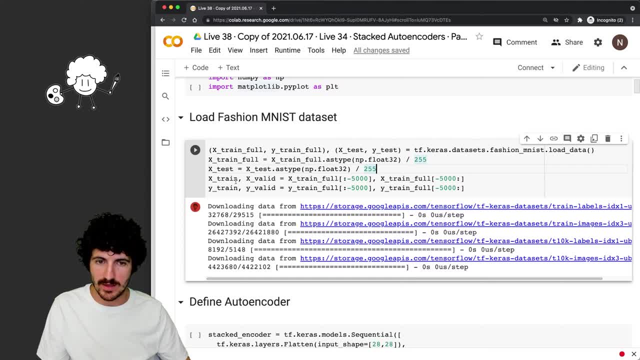 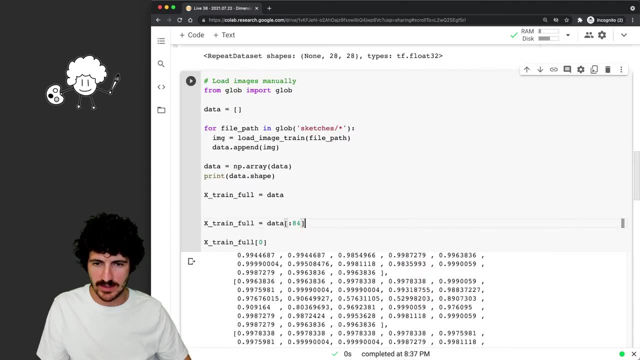 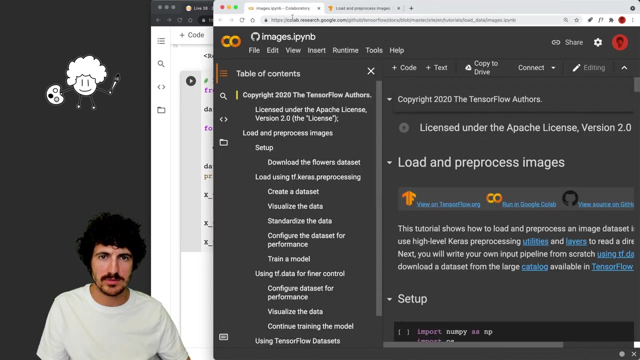 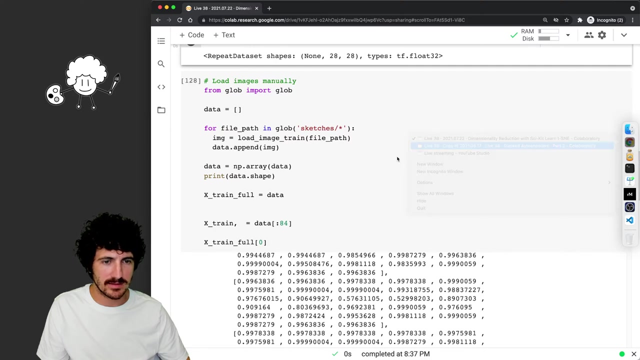 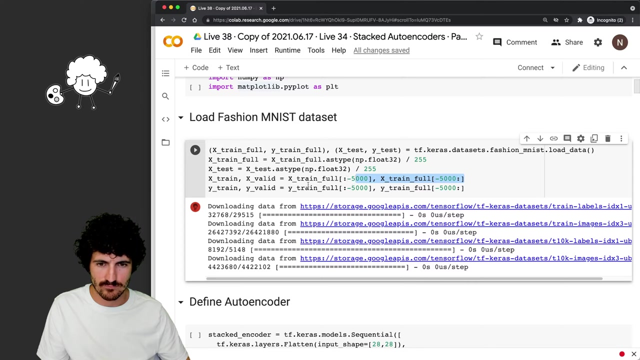 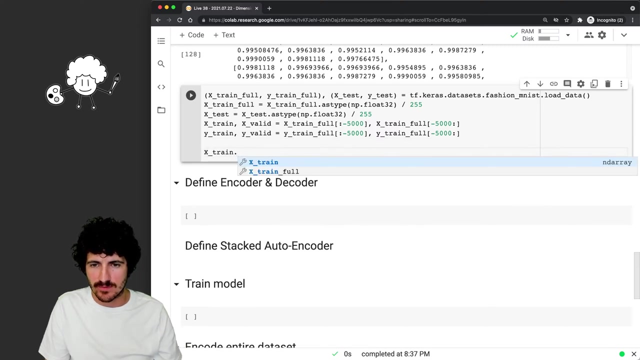 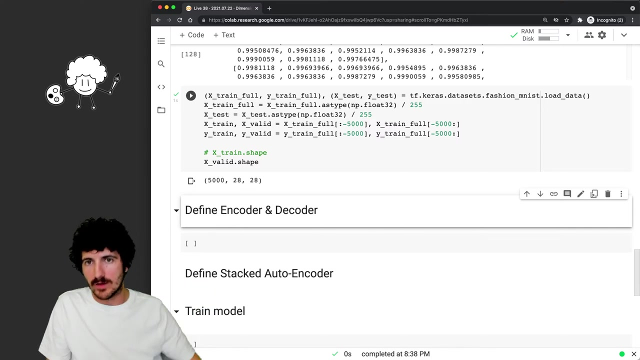 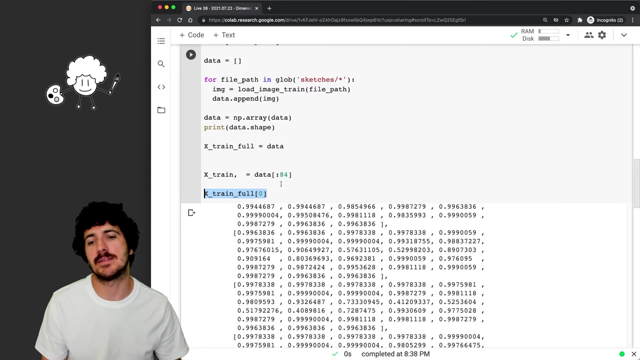 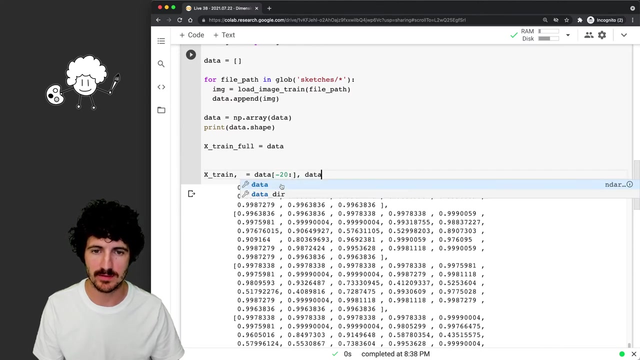 And now we have X-train, white train. so we get here X-train, and are all these notebooks right, Okay, All right. X-train, full Test, this, Yeah, Okay, Okay. So let's see. So we're going to get here um minus 20, eight, uh, six. 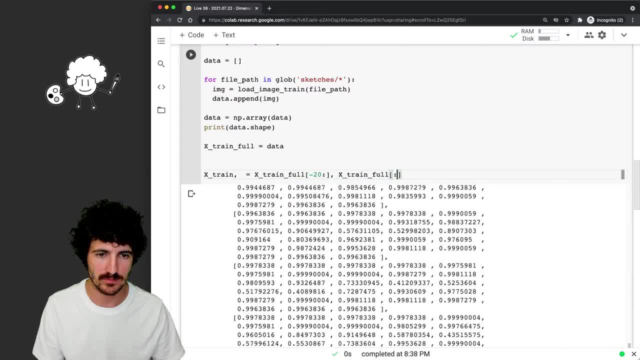 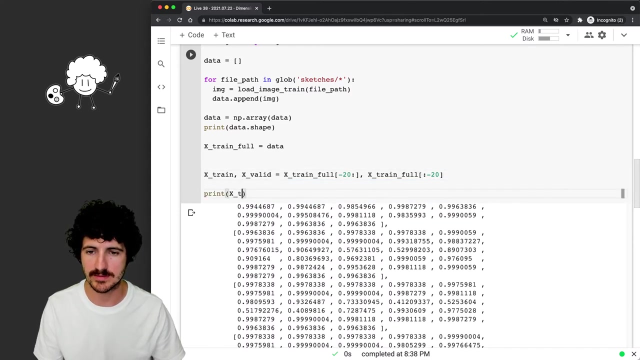 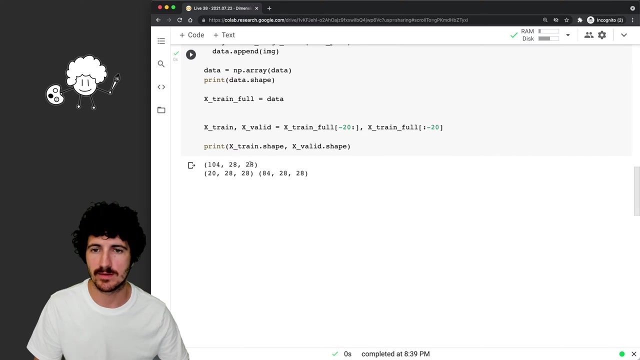 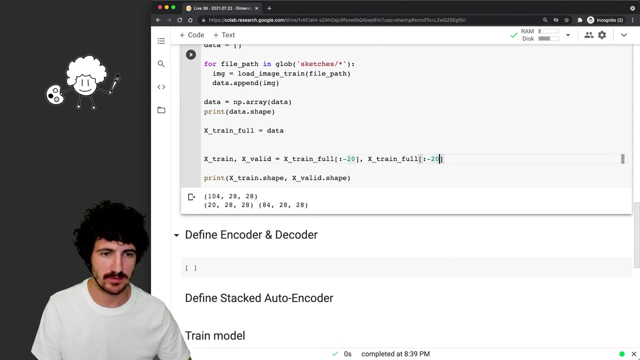 train for X, train for minus 20.. And this would be X ballot And we'll print here: X train, X value, shapes, shape, All right. Hmm, Train probably the other way around, All right, So we got the entire data set. is this shape? 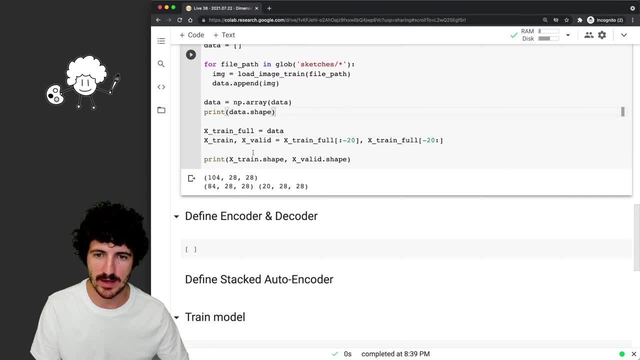 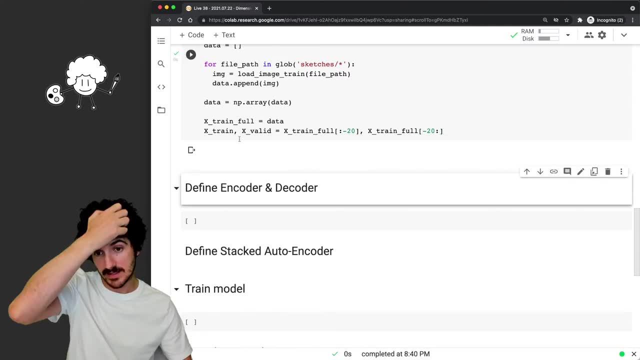 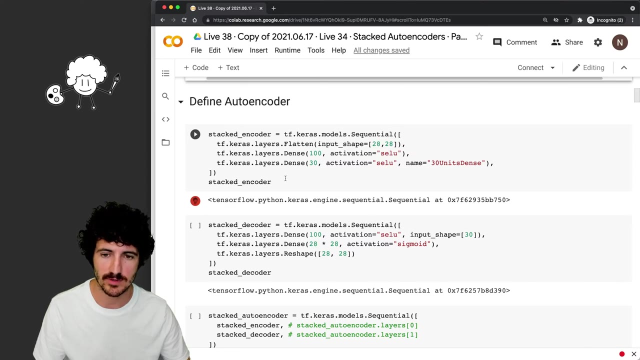 Then we have all the, so the data, and then we have the training and the validation data set. Cool, Right, So we have a data set now and that we can get the encoder decoder. Okay, Cool Um architecture. So we're going to copy and paste here for expediency. 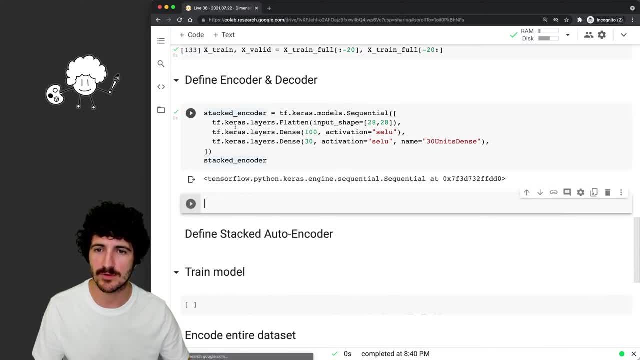 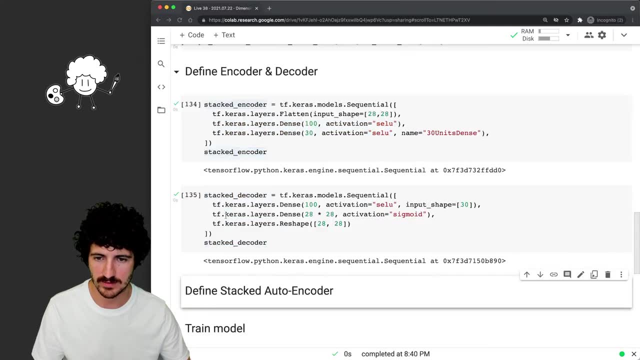 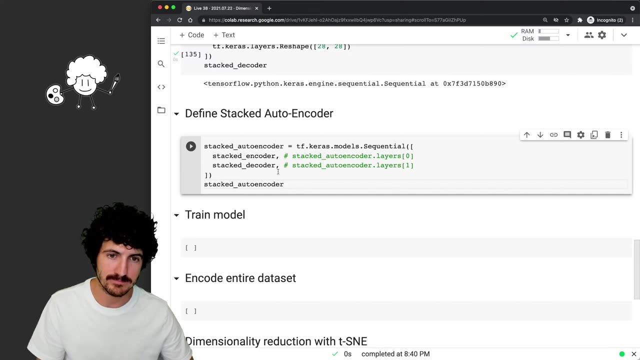 Otherwise we're not going to get there. Uh, we have the encoder and we have the decoder, and uh, we have the stacked out encoder which we're going to paste here. We can go probably another day a bit slower, Um, awesome. 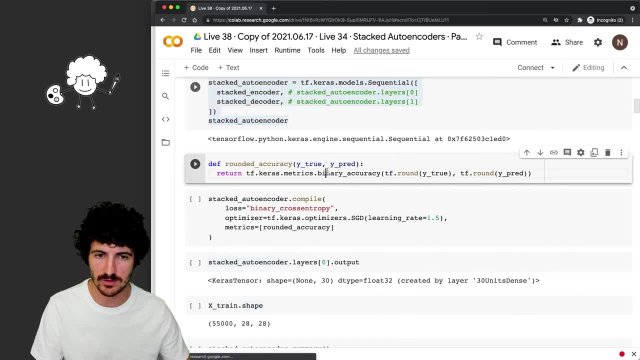 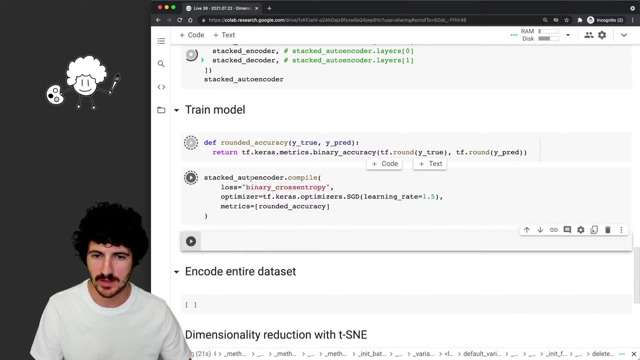 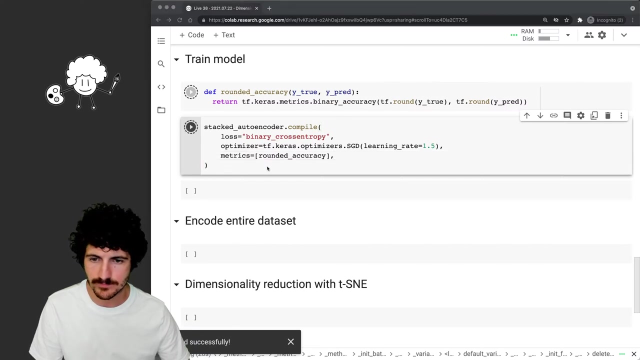 So we have our stocked out, Okay, And now here we define that uh, rounded accuracy, which is our custom metric. We compile the model with a binary cross entropy and this learning rate and our custom run that accuracy metric and um, And I'm going to make sure that this. 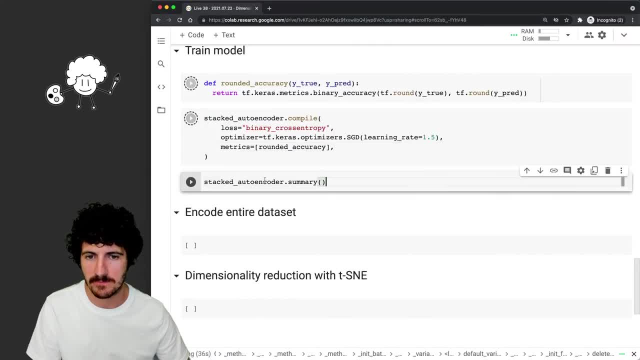 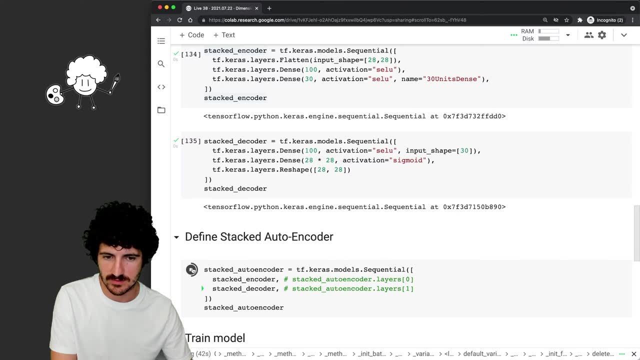 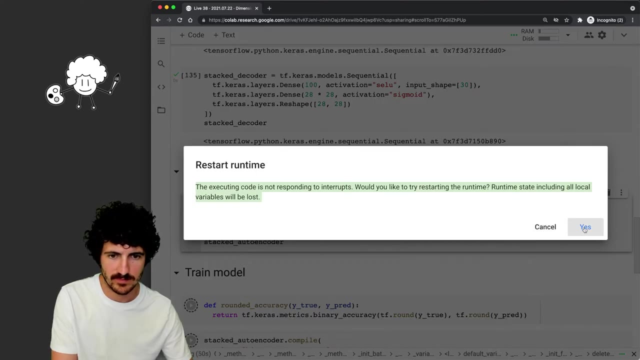 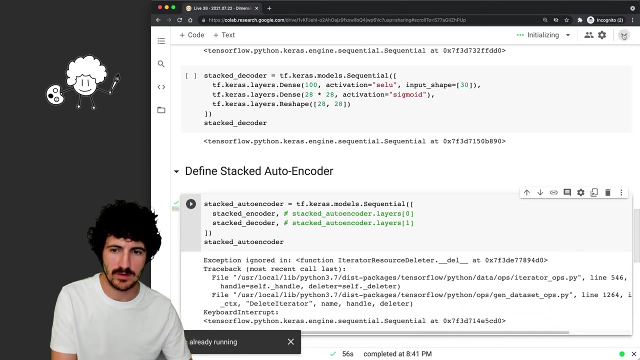 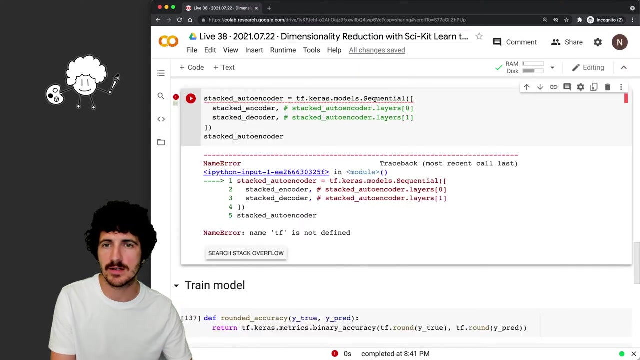 working. Shay summary. Okay, We can bring the summary And, uh, let's see what's hanging in there, What's going on. Uh, okay, We can. actually something is weird. TF is not different. Okay, So we could run everything above the cell. 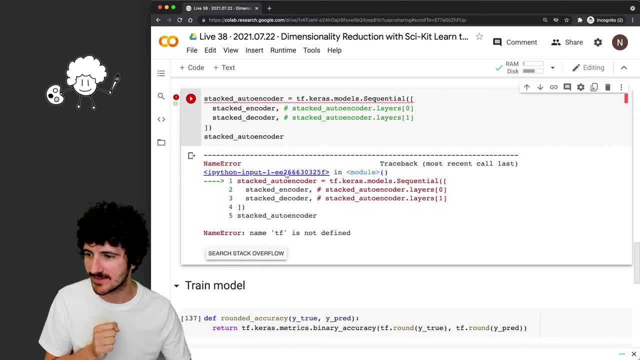 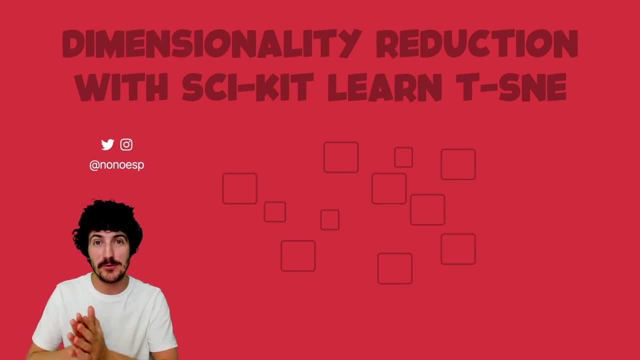 So I see some, some people are connecting now. So, for those of you who are new, or those of you who weren't here before, we're going through a dimensionality reduction exercise. uh, with Disney, this an algorithm, an implementation of this algorithm in scikit-learn- we're trying to get there. 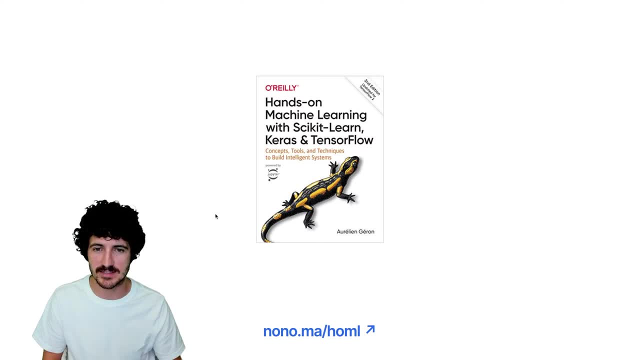 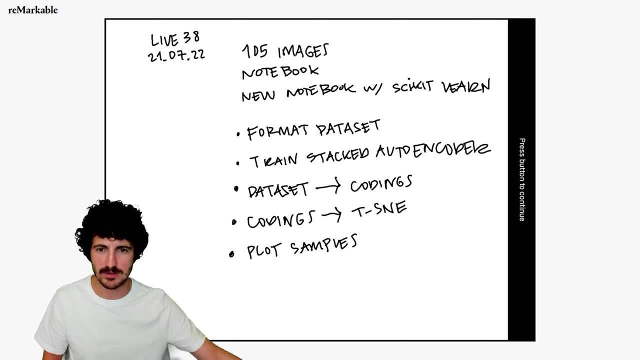 We have to, uh, to do a few um stages to get there. So one was To to format, to format our data set Um. another one was to to train a stack out in quarter, which we're doing now. 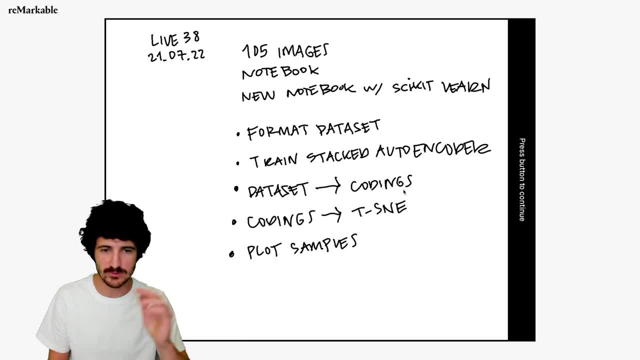 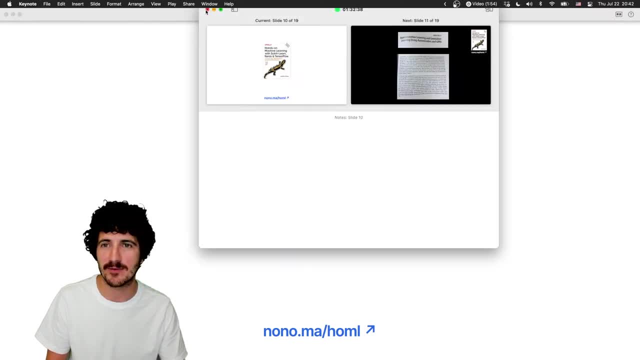 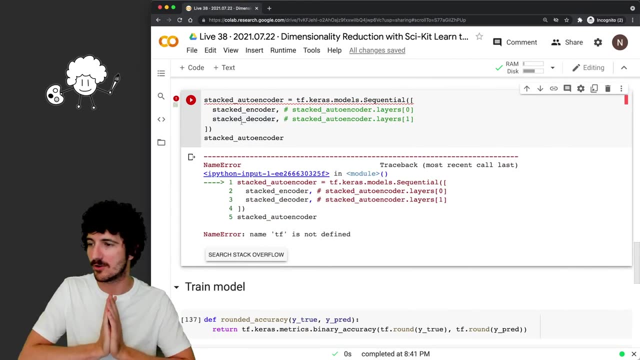 And then later we'll see how to convert our data set into coatings, those coatings into Disney, and then plot the samples. And we seem to be running a bit out of time, All right, So let's leave this here, and, yeah, I would encourage you to say hi on the chat to tell us where. 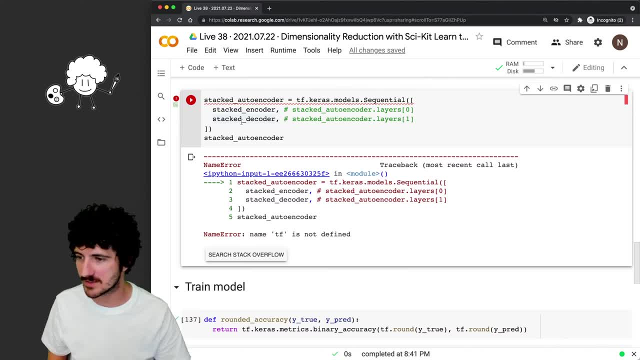 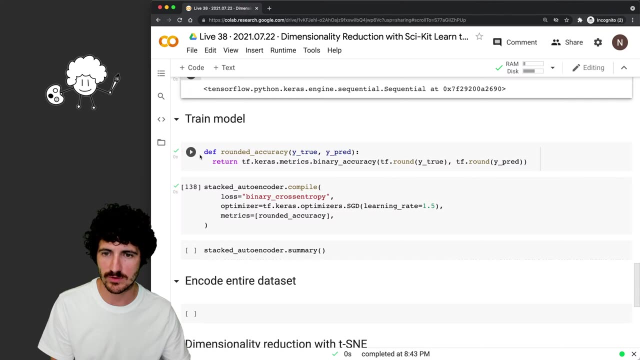 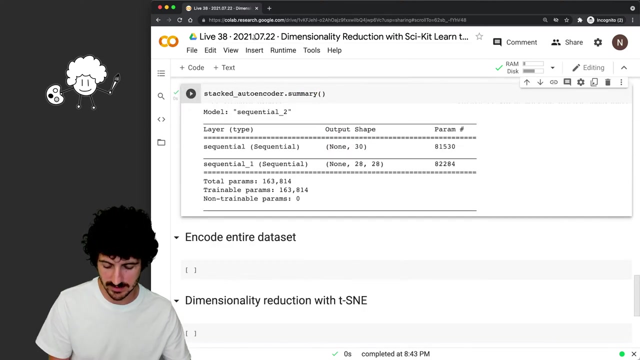 You're connecting from and what you're looking for to learn from, uh, from this channel. Um, all right, So TF is not found. So let's um execute this cell. So we have our autoencoder, We define our metric, compile this, we get a summary of the model and we have to train now. 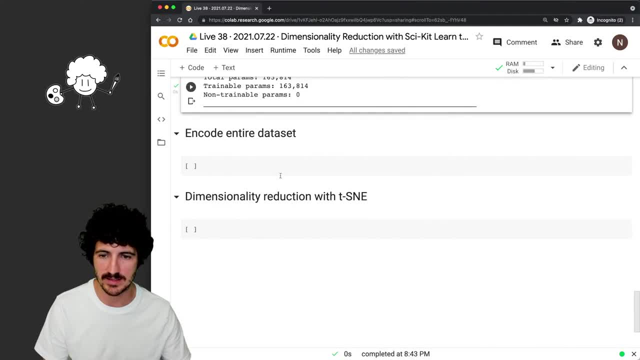 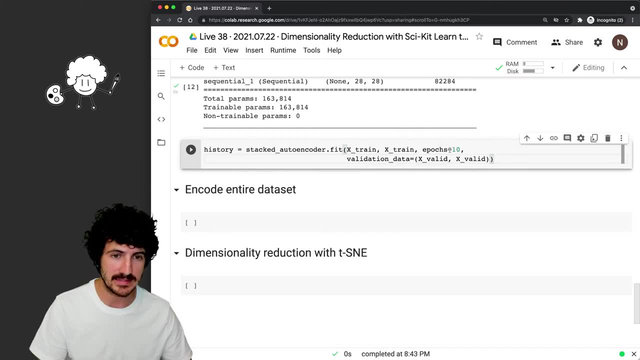 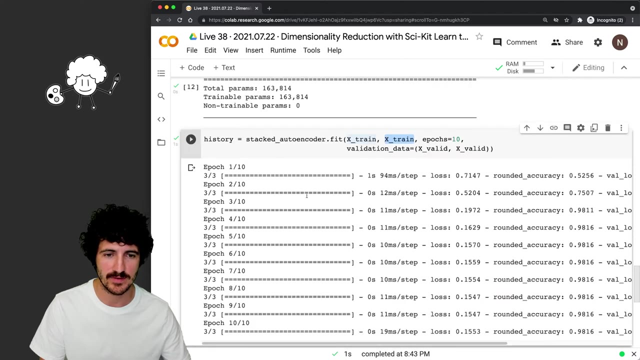 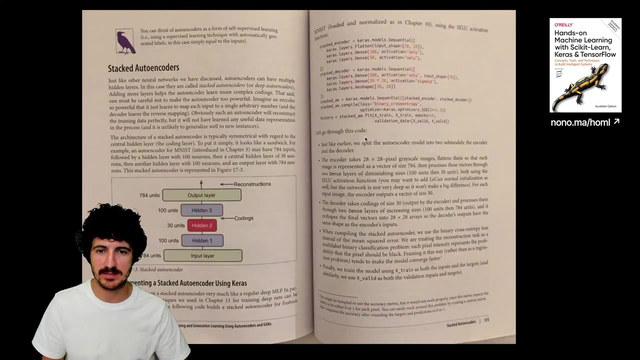 So now we can train with our data. So this is the actual cell that trains when train for 10 epochs, and you see that the input and the output data is the same because we don't have um. you know we're trying to. if we're looking at this image right, the input and the output are the same. 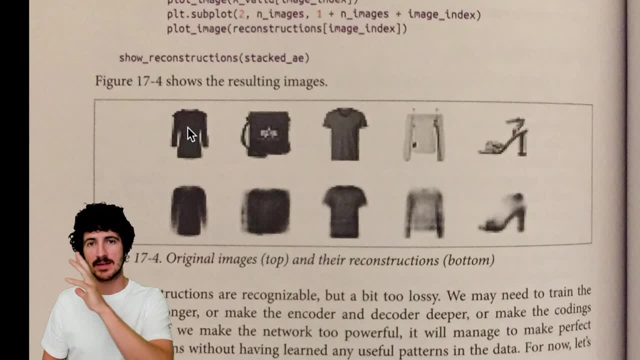 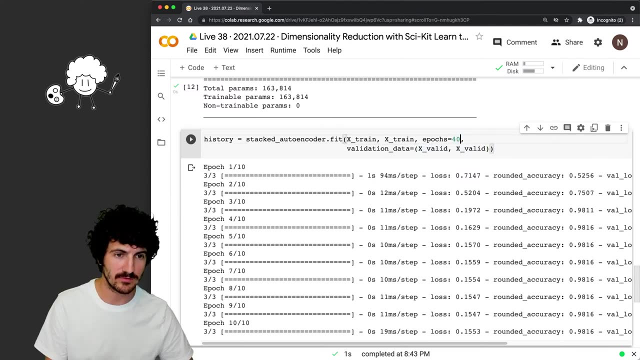 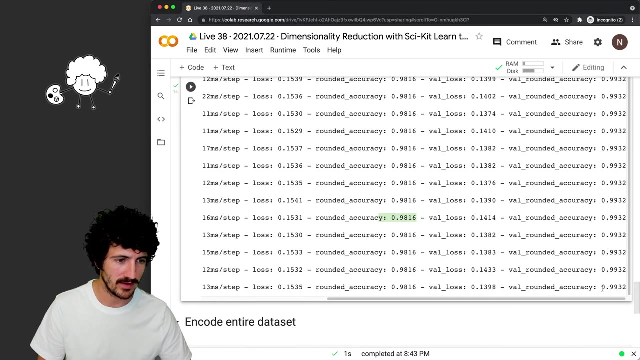 So the goal that we're trying to reach is the same, So we use the same input and output The data set on one training. All right, So these super fast, so maybe we can train for more epochs. Yeah, it seems we might be overfitting there because we don't really have too many samples. 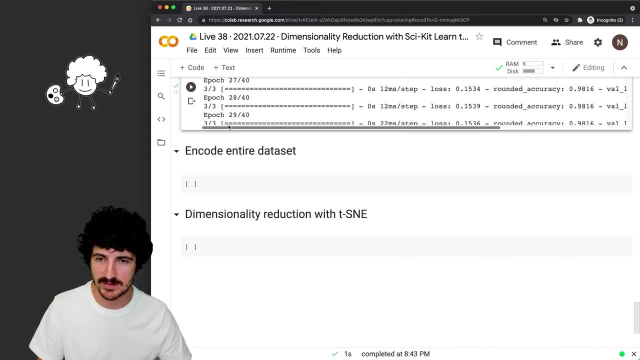 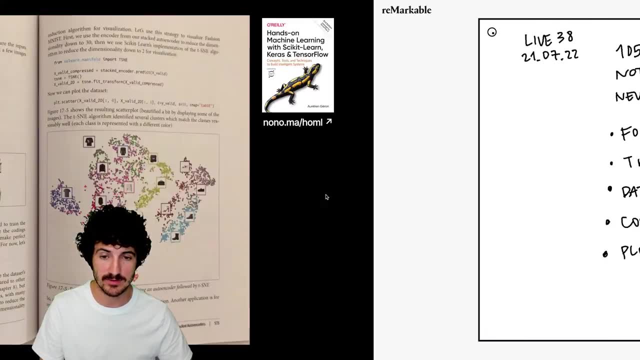 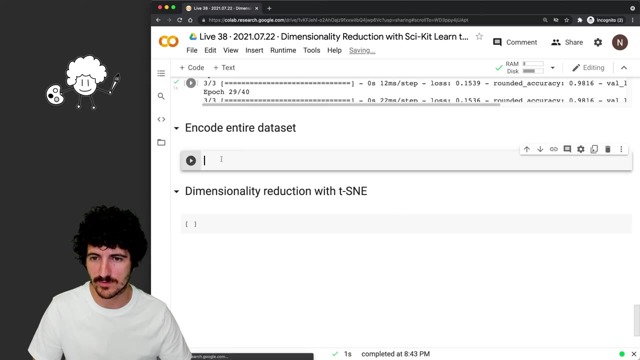 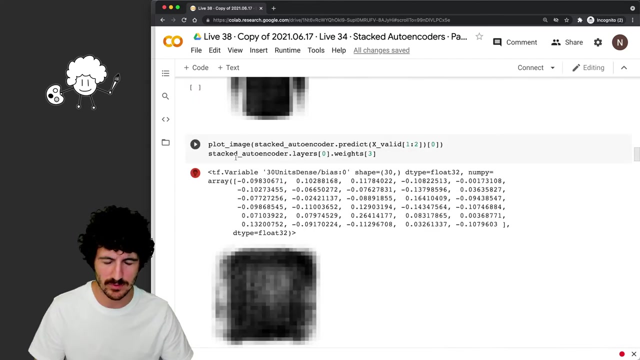 We just have 104 images, but, you know, maybe we get somewhere. Um, okay, So we have gone through this and this and now we need to see we can get the coatings. This is a bit hard, So for me to understand, the other day was was a bit hard so we could, uh, get a soup network of what we had before we. we have our encoder and 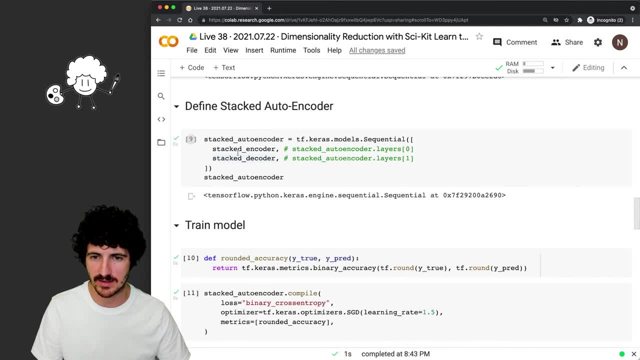 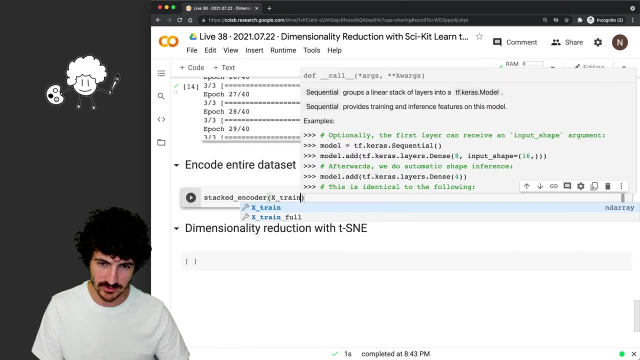 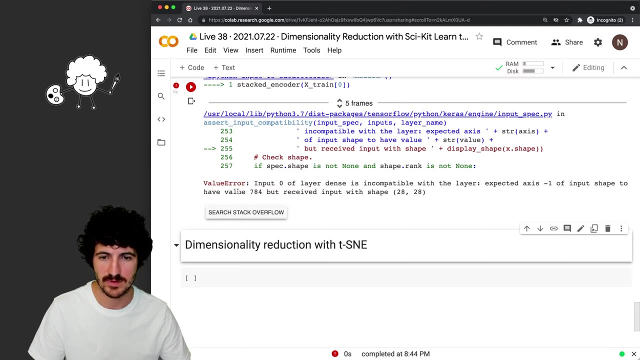 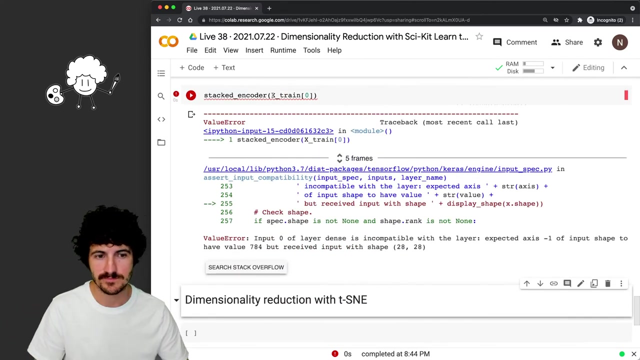 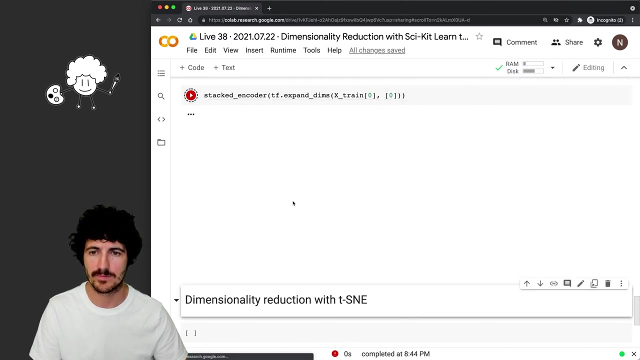 So I believe we can. Uh, as a an email there are stacked out on our stack and coder So we could pass X train, zero D, zero layer is incompatible. Yeah, See expanding. Yeah, Yeah, Yeah, All right. 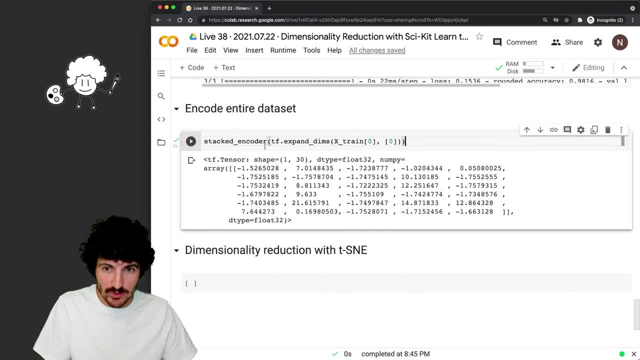 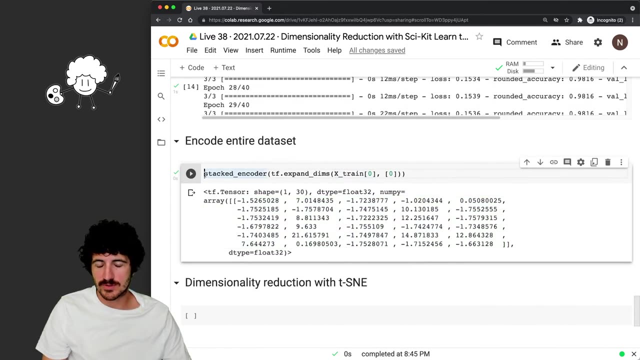 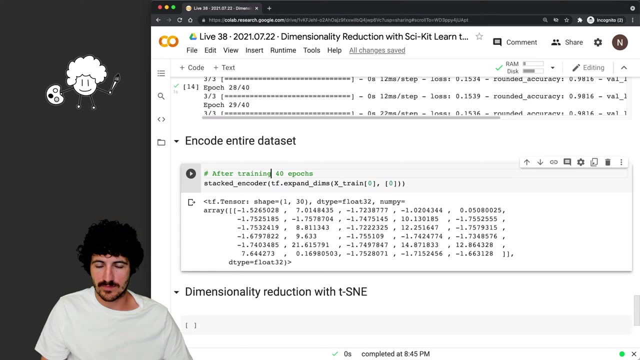 So if we pass the image through the stack encoder, right, we're passing, uh, the first image on our dataset. here we're getting the codings, which are 30 digits, um and what I'm not completely sure. So this is um, after training, 40 epochs, let's say, if we retrain. 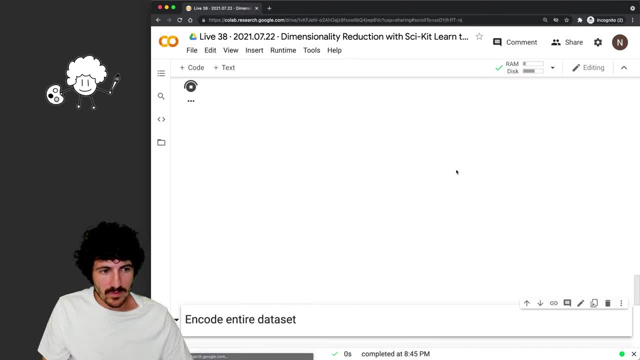 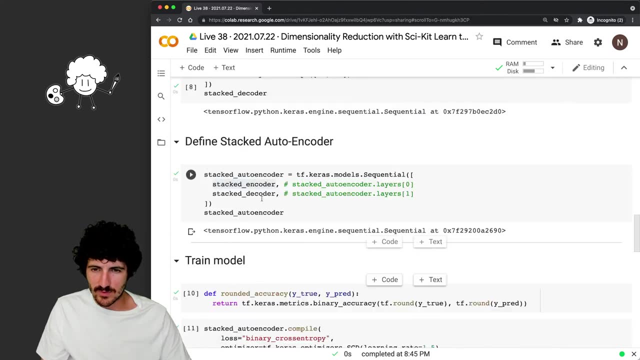 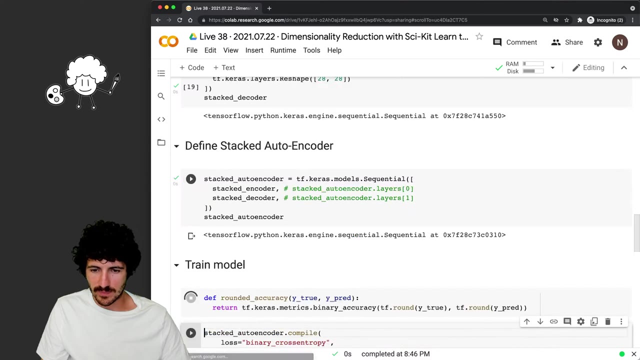 let's say we retrain, for well, if I retrain now, I think continue from where we were, so we have the same accuracy. so we might need to reset our model here and train And again. right, Let's train again. 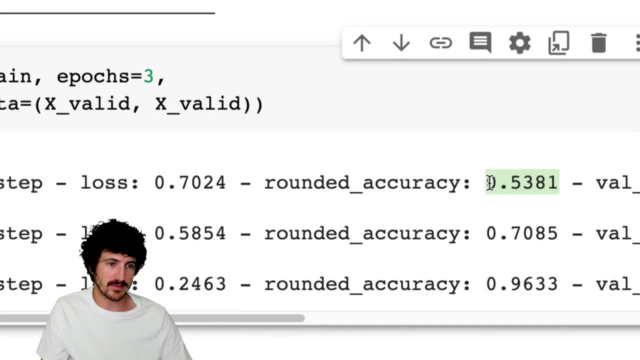 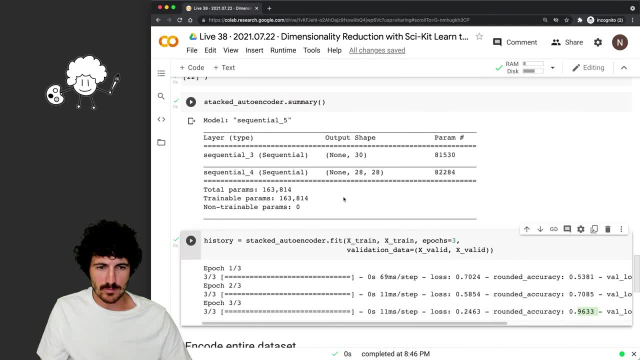 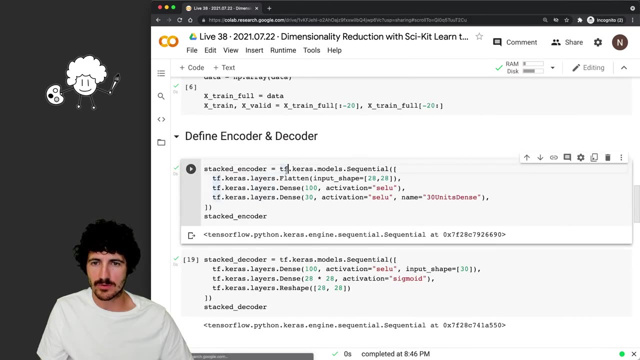 So you see the, the accuracy starting from, or if the render accuracy starts from 53,, 70 and 96, we get really fast, We get really high. So I'm just going to put here one. So we get just to this step and I'm going to go through all the cells again. 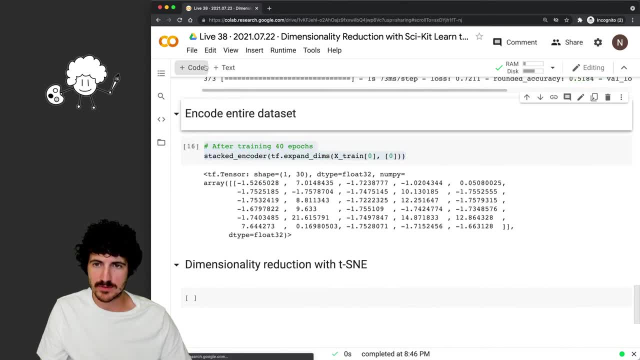 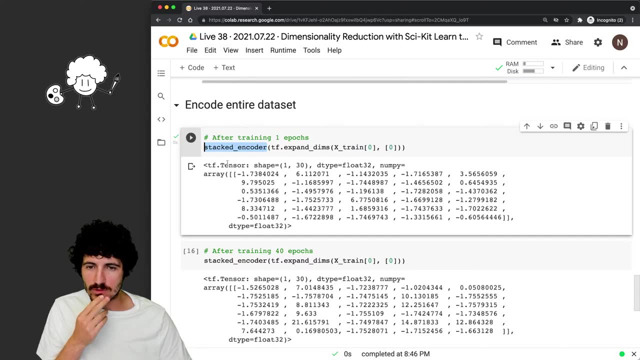 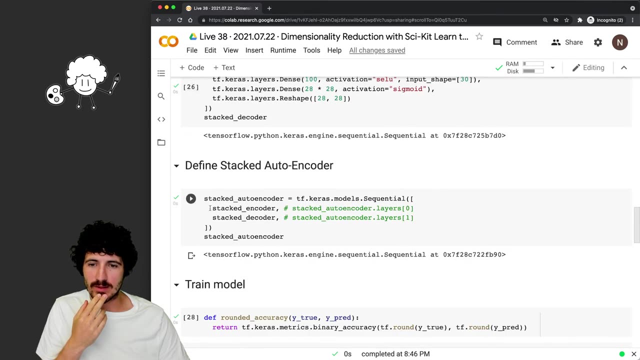 All right. So we have this model here, and this was with 40. Epochs. We're going to try to do it now just with one epoch, All right. So the encoder network right, which we defined here and we included here in 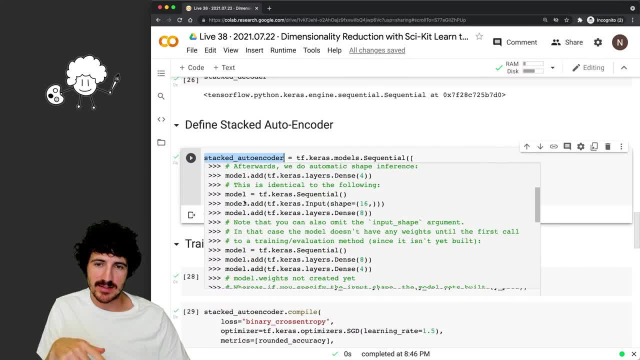 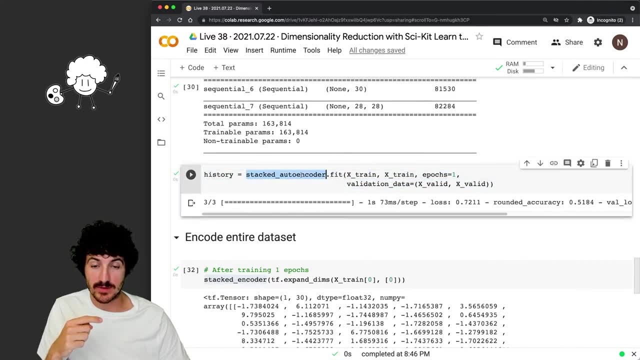 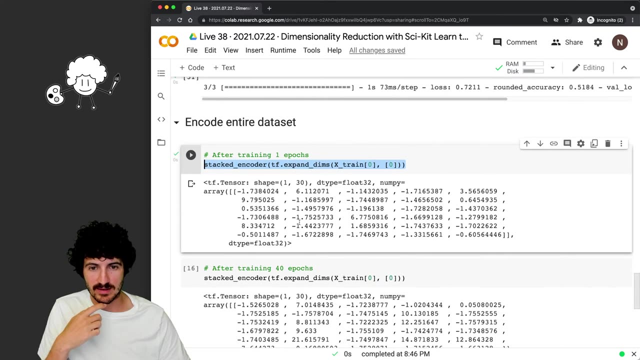 the autoencoder has actually been trained and its weights have changed. So we, um, when we run this feet method, the autoencoder has inside the encoder in. We actually have this network here that can, um get these, uh image right. 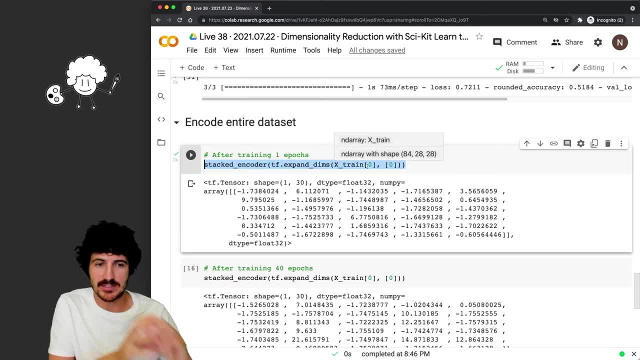 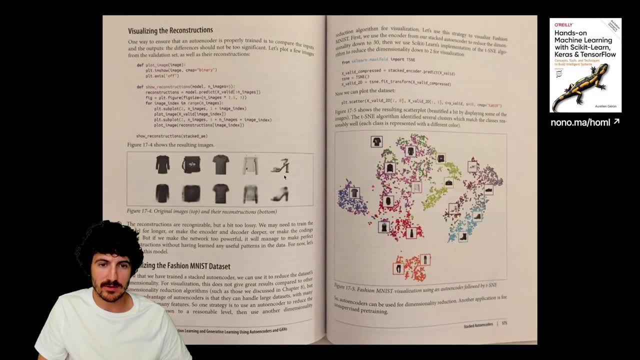 This input image says 28 by 28 image, and then generate the coatings And what we have here now are 30 coatings, right, Like what we talked about before. Let me see if I can, if I can reconnect, Yeah. 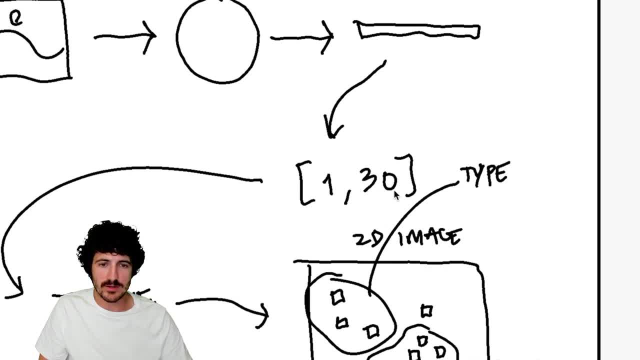 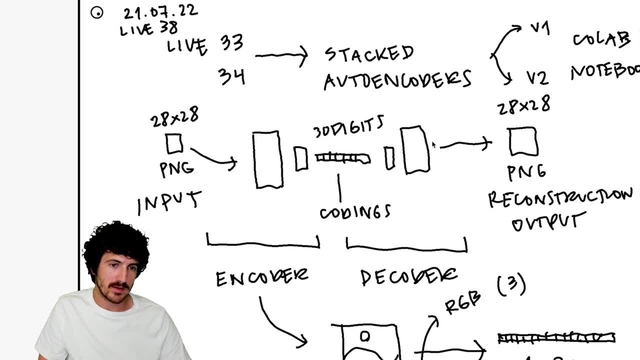 So we reconnecting here. So these are those 30 coatings. right, We were talking about Um a 28 by 28 image that was passing through a network. So we were training in this loop of encoder, decoder and in the middle, 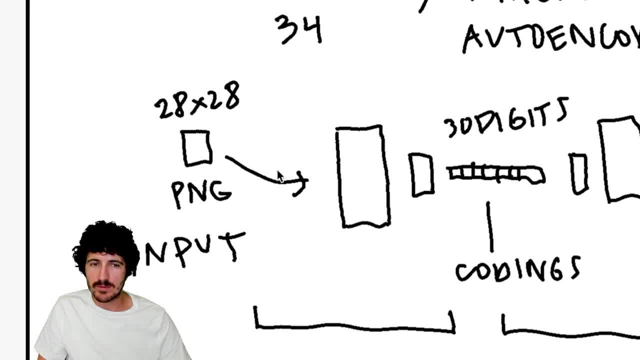 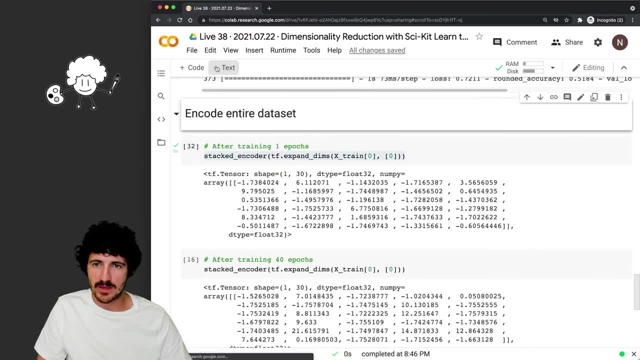 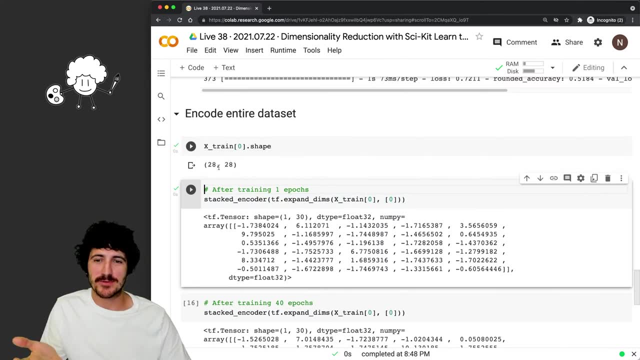 these encoder part ends up with um 28 by 28 on the left and then 30 on the right, Right, And we are actually seeing that here. So we, uh, if we look at the shape of X-train, so we look here is 28 by 28.. 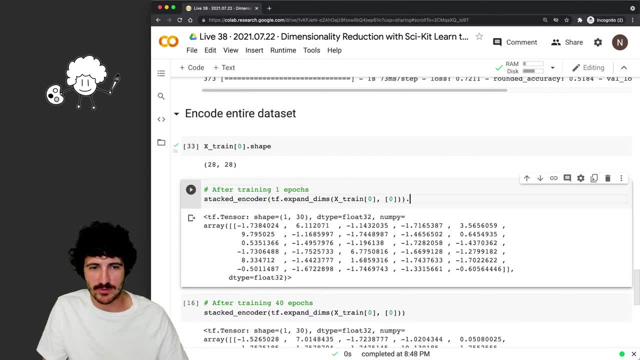 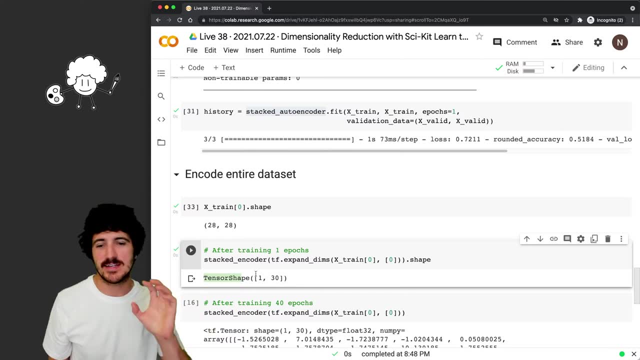 I put it through the encoder And, as promised, if we get the shape of this- I'm not sure we can do that yet It's one by 30. So it's a linear tensor that has 30 digits inside of it. 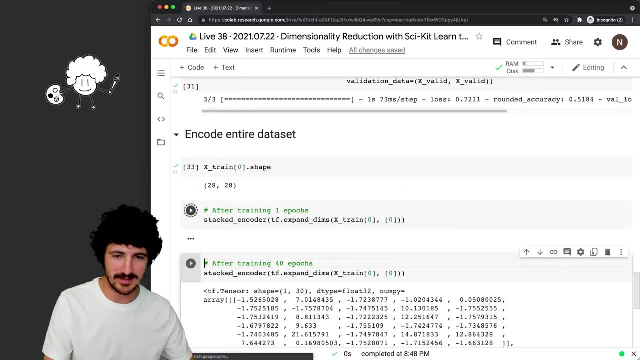 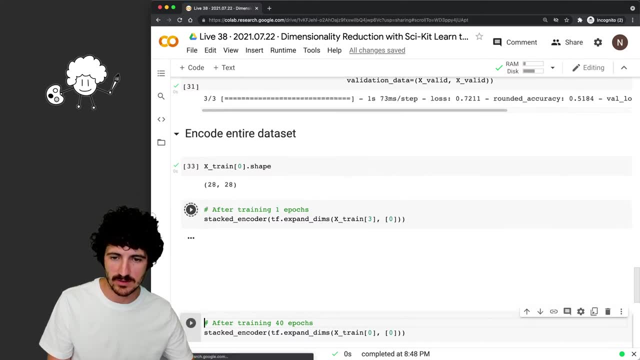 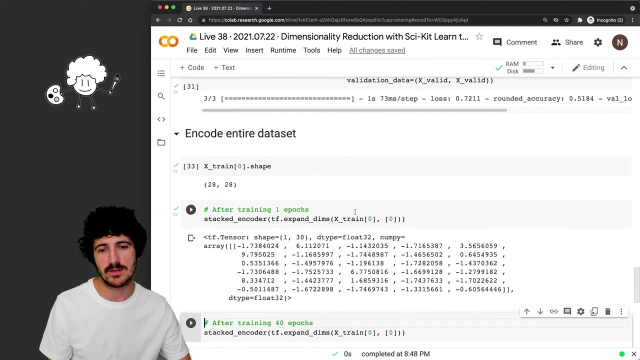 And you know, promise achieved, right. Um, if we change the um, the input, so I'm taking different images here- The coatings on the bottom slightly change, right, They change a bit because the input is a different image. 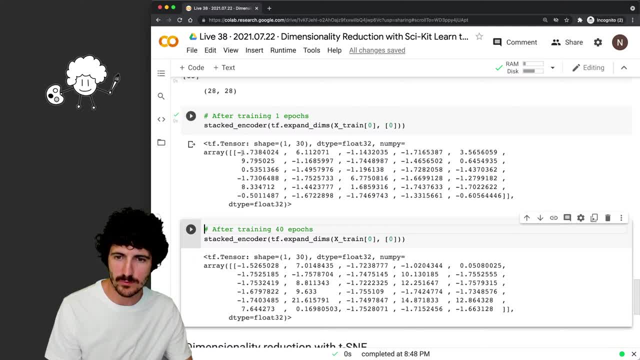 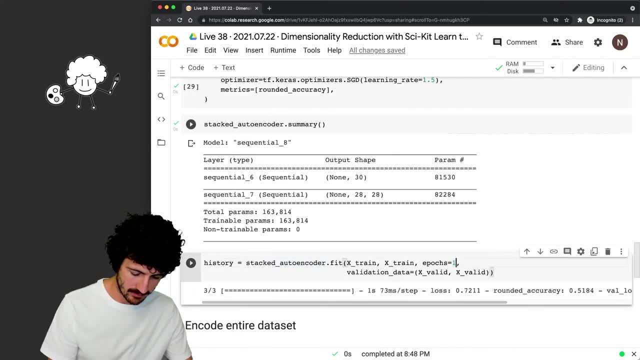 Um, they're different, right? So one 73 and one 52. So what we're going to do now, just to prove that that's true, is that I'm going to go to 15 epics and I'm going to rerun the cells and retrain. 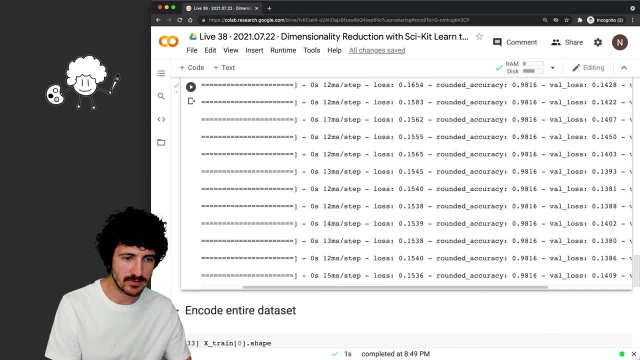 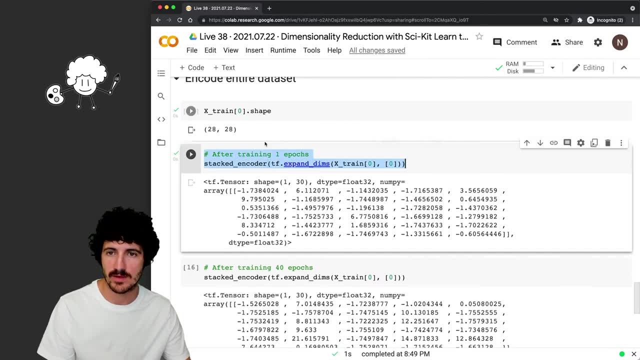 Right, So we retrain there. now our render accuracy is again at 98.16, which I believe is the same that we'll get if we go to 48 books, And that What I'm going to do is that I'm going to put here 15 epics, but I expect to see 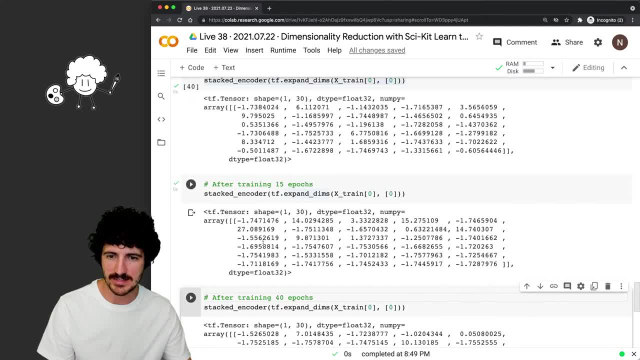 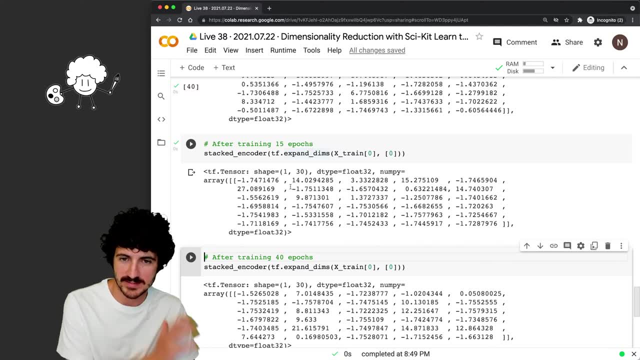 something similar to be low, Um, and I don't let me see why that is. I'm not, I'm not really sure um that all of these things that I'm saying is are true or not, but uh, I'm. 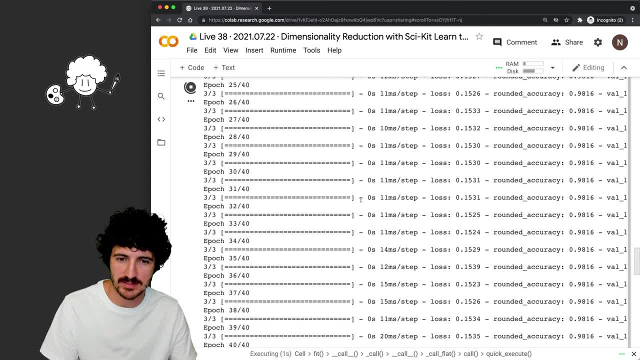 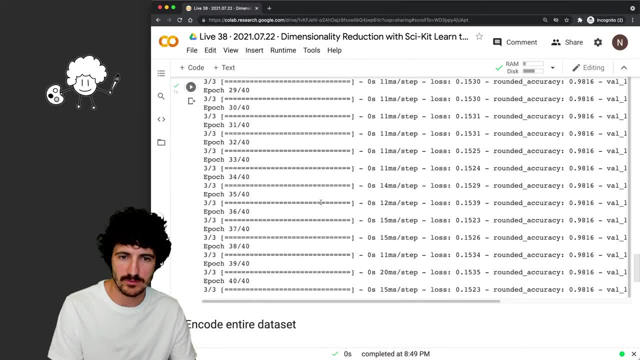 trying to get there to understand everything. Okay, Let's train again- because I said 40 epics, but that wasn't really true- and rerun this. All right, Not really Getting there? Okay, Let's do actually. So 48 books. 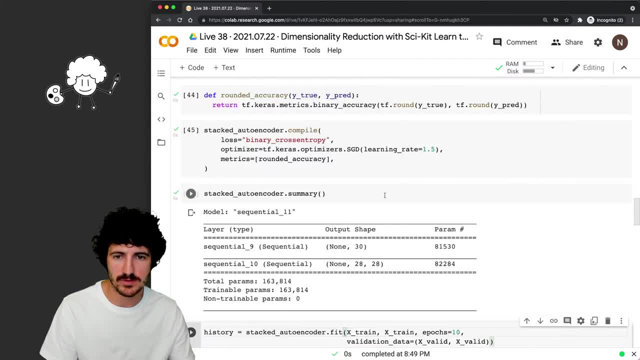 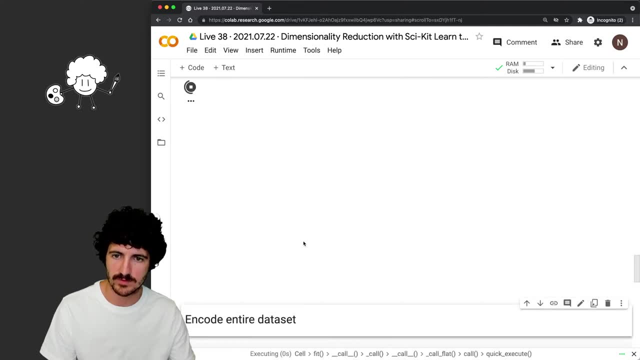 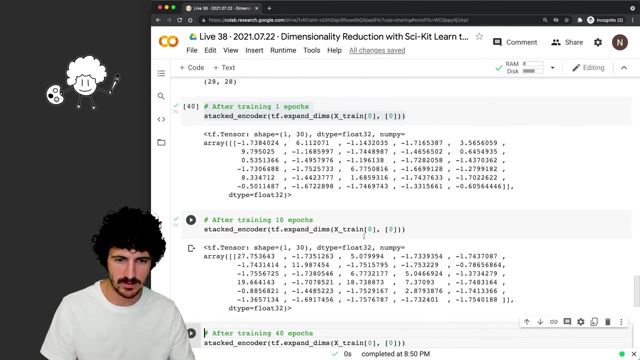 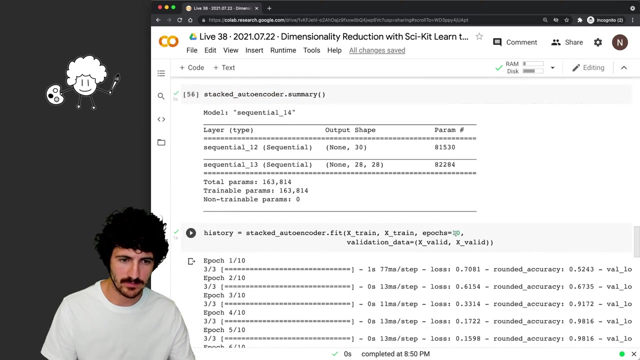 So let's do, actually, uh, 10 epics and redefine everything from scratch here, Right? So that's 10 books, and we're going to put here 10 books, Right? And now we're going to put 40 books. 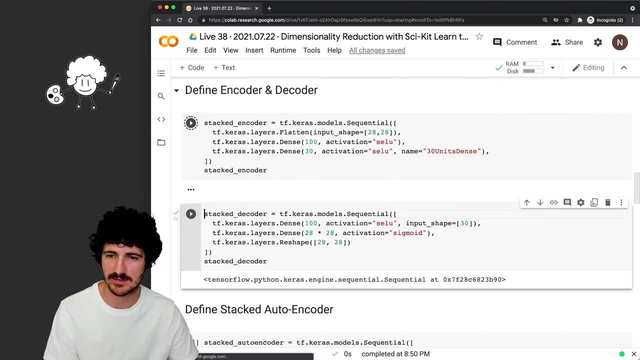 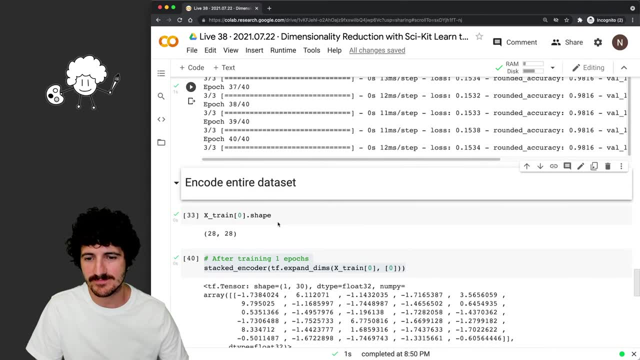 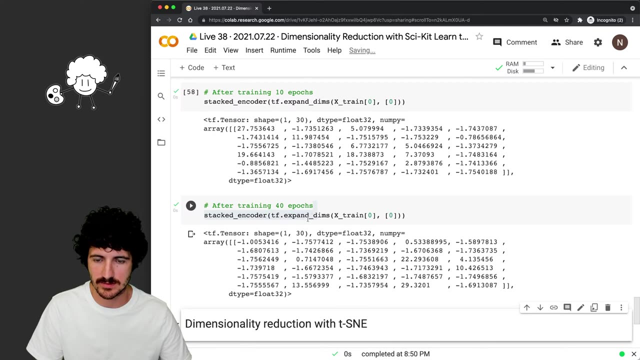 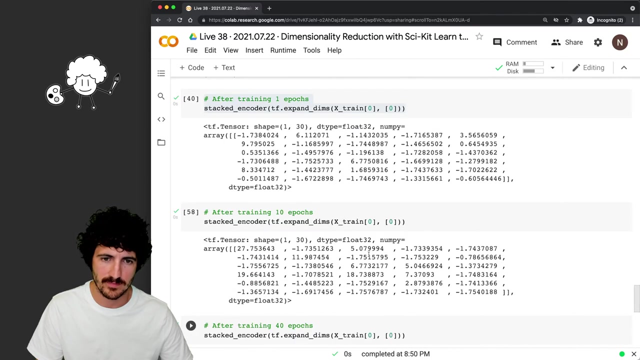 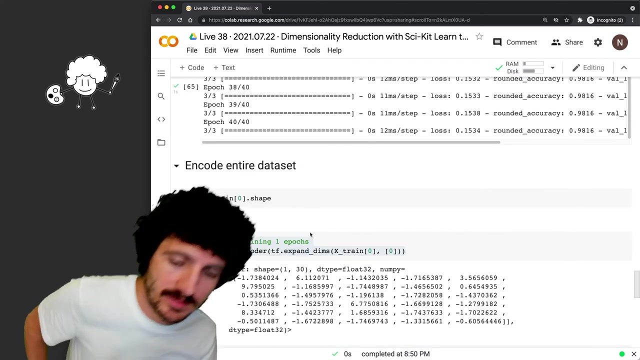 And I do think we need a larger data set. All right, So 40 epics around this, minus one everything. Hmm, I'm unsure what's going on. So how we can, how can we see the weights on the layers here? 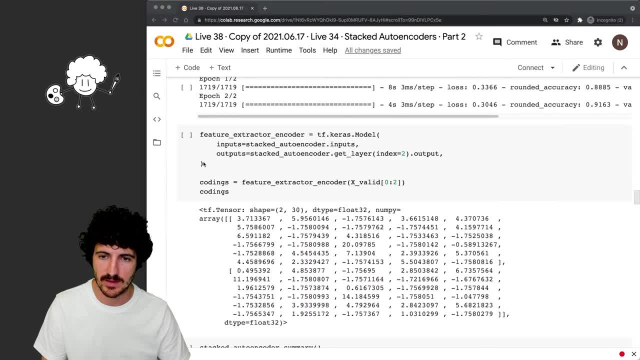 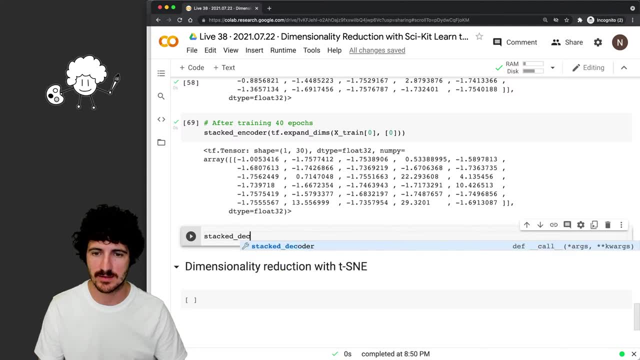 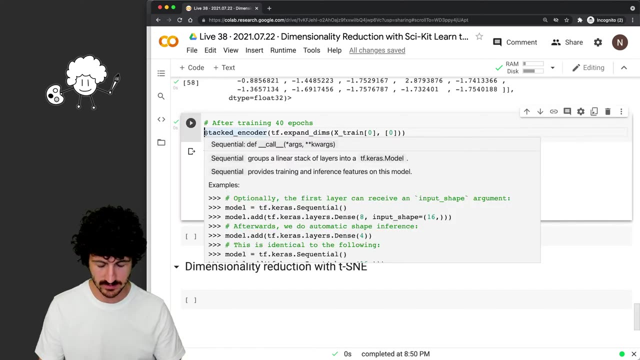 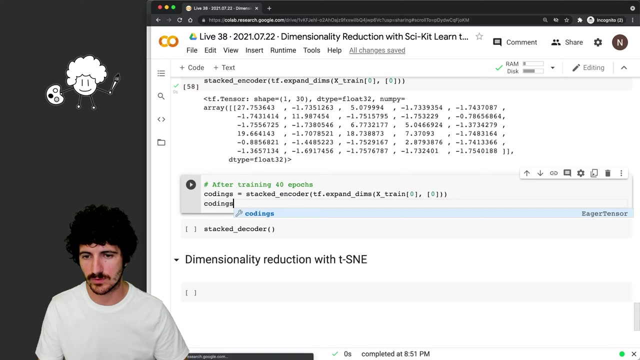 All right, So I have a way to plot the coatings and well, one thing that we can do is that if we run this by the stock decoder, right? So if I now get This output from here, So let's say that the coatings and I run this, my print coatings. do you see them? 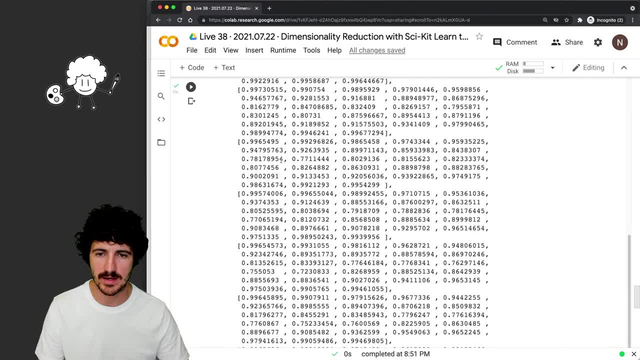 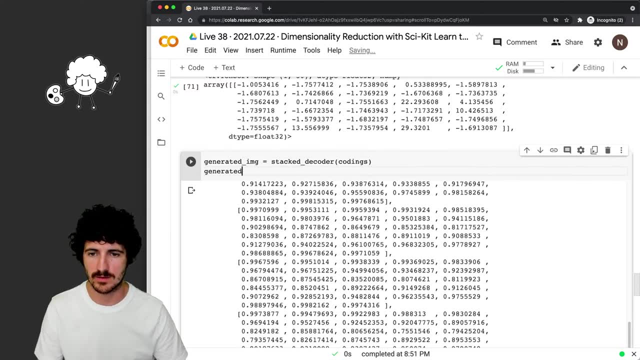 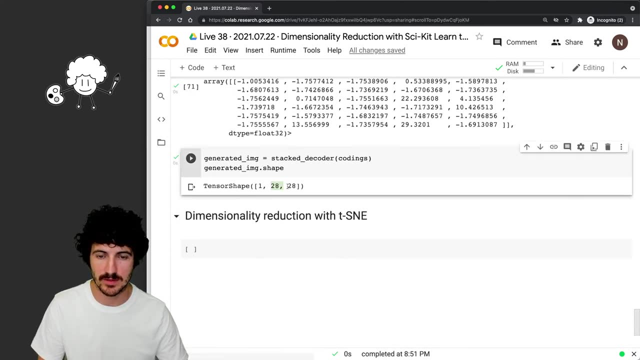 So now I can pass the coatings back here and we get back, Uh, so this is a generated image, generated image shape, right, So that's again Uh, 20 by 28 image that is black and white, And, um, if we get the first one of that batch, we get an image. 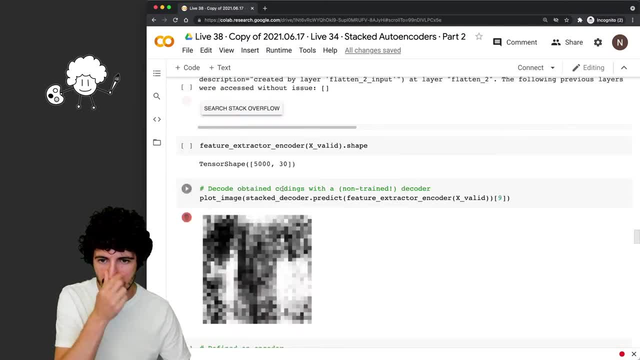 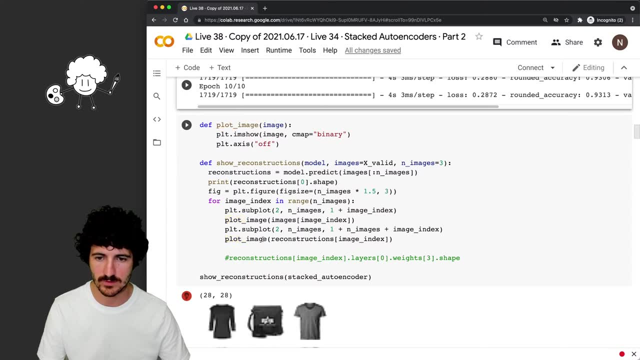 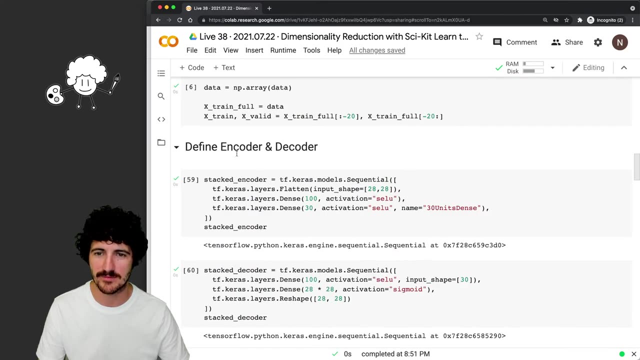 So let's take a look at how to uh plot those, because I have the code here. So, plot image- we have a helper method. plot image show reconstructions. All right, We just need to put these helper and we'll have to do some cleanup. 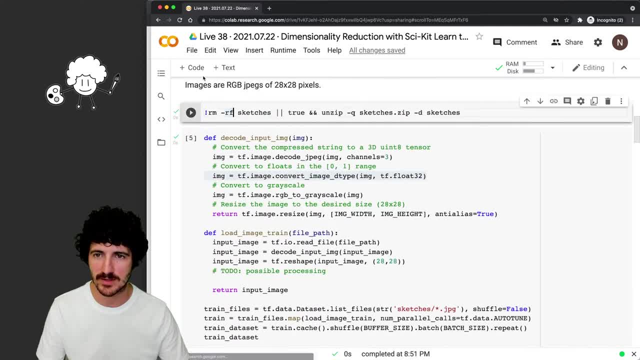 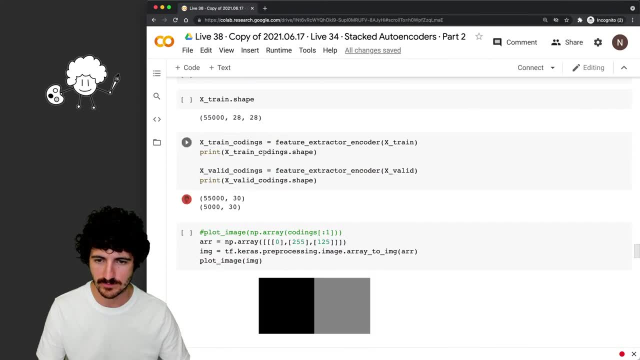 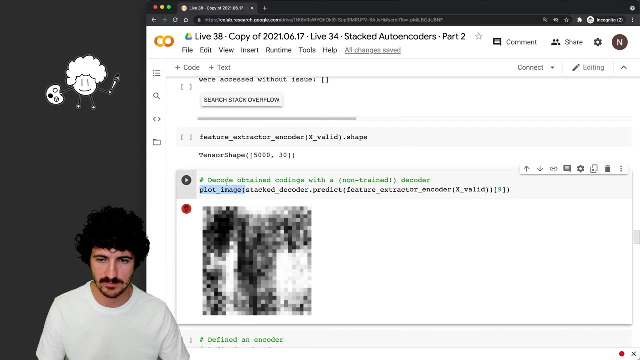 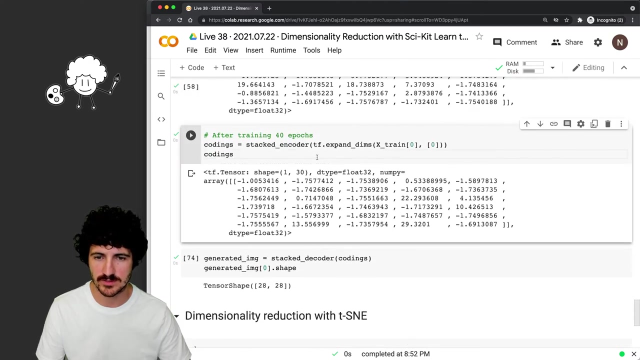 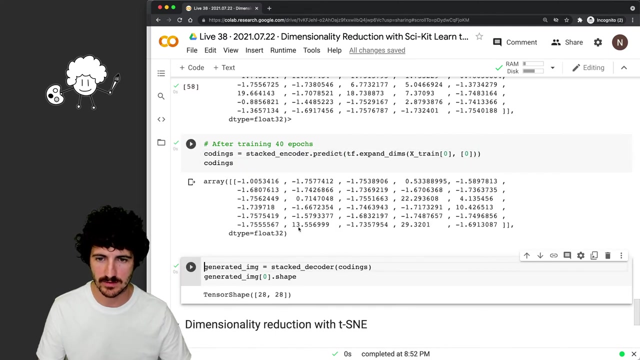 I'm not going to do it in today, but we'll have to do some cleanup. All right, Helper here. So we can plot the image And I'm not sure if these changes anything. if I do here predict I get a tensor, and then if I do predict I get something different, but it's, at the end of the day is the same result. 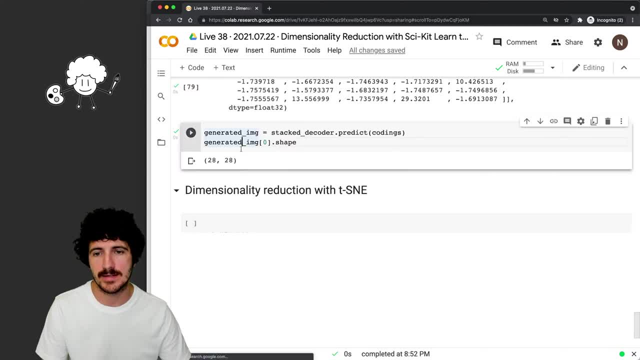 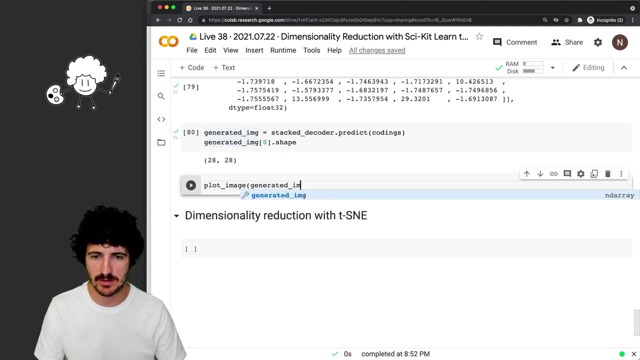 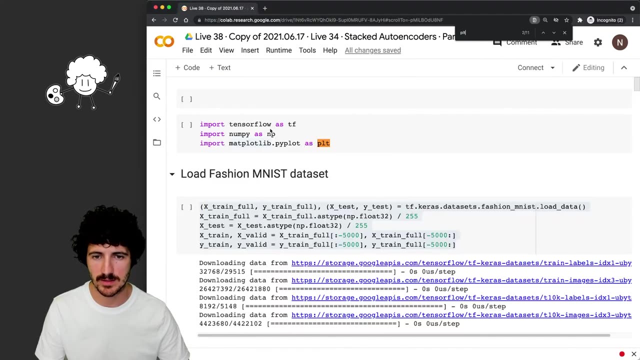 And then I get an array as well, All right, So, um, we wanted to plot this image right, So we're going to applaud the generated image. Let's see what that does. Plot is not defined. All right, PLT. 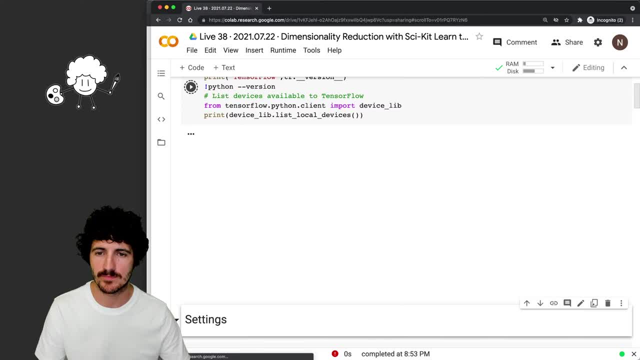 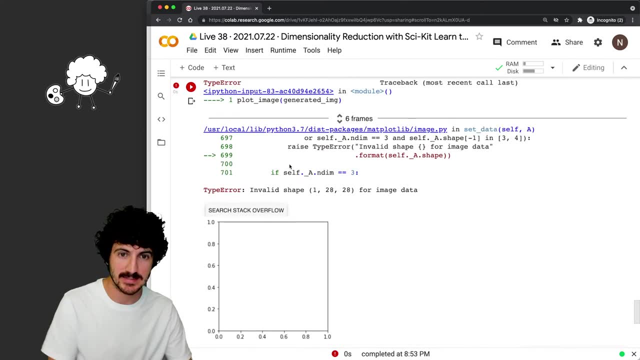 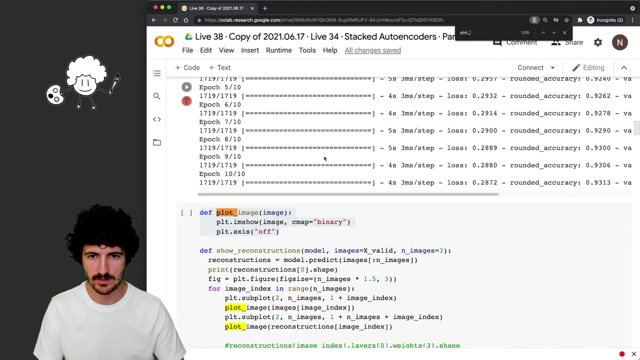 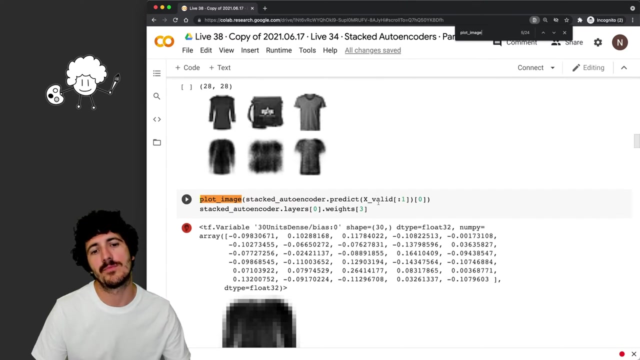 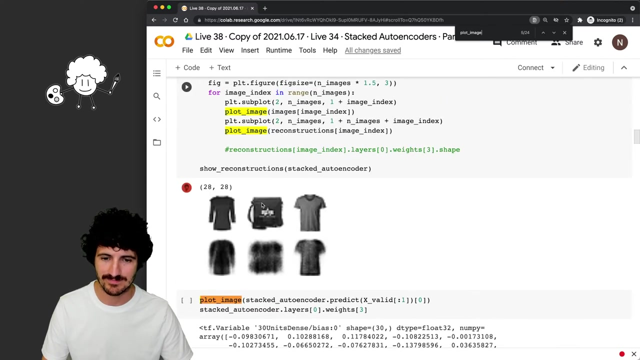 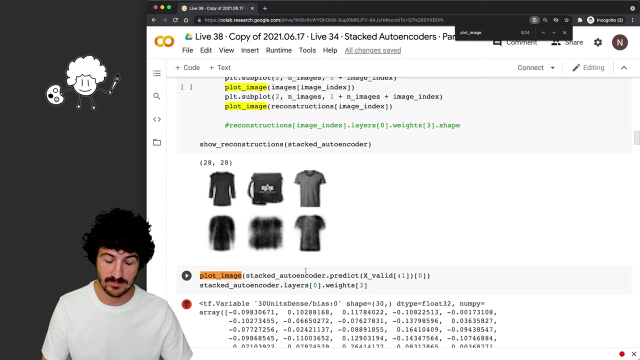 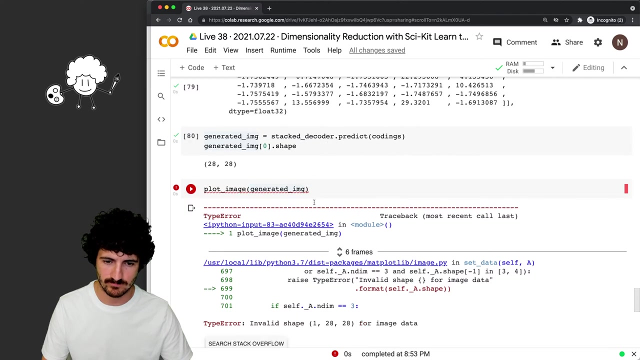 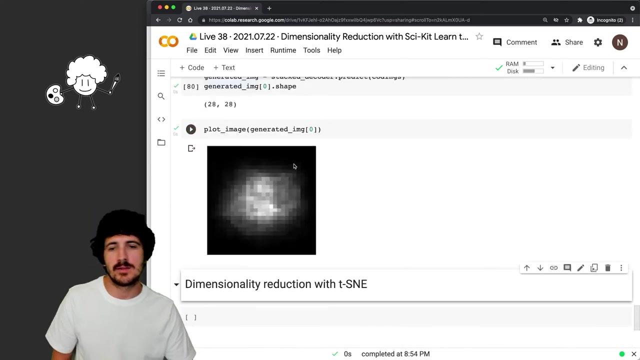 We have another dependency and then we go back and, uh, we got our plot image All right, So it doesn't really have Predict valid zero. Um plot image. Hmm, All right, So it seems like it's learning. 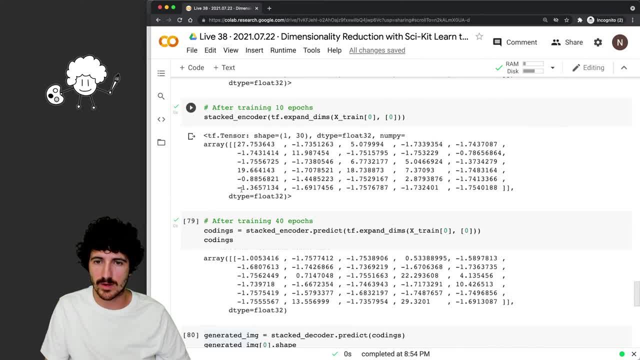 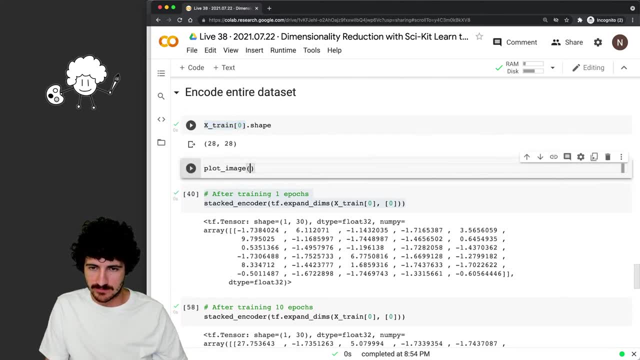 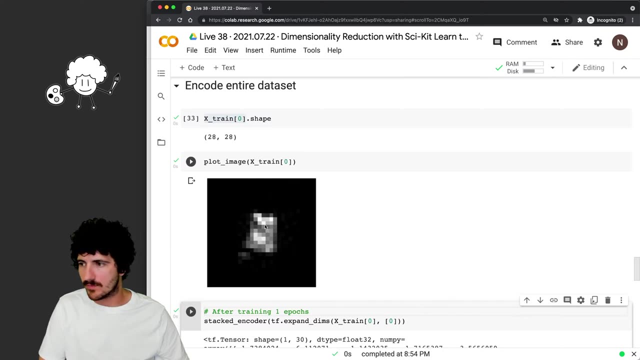 Something right. So it's learning something. We got the um, the input that we're using here. We can also plot it Right. This is one of the. this is the input that we're um, that we're inputting to the network. 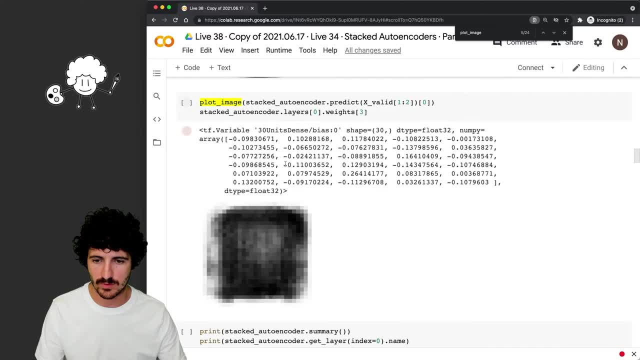 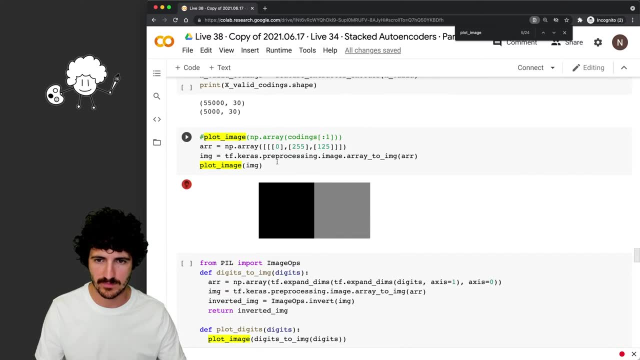 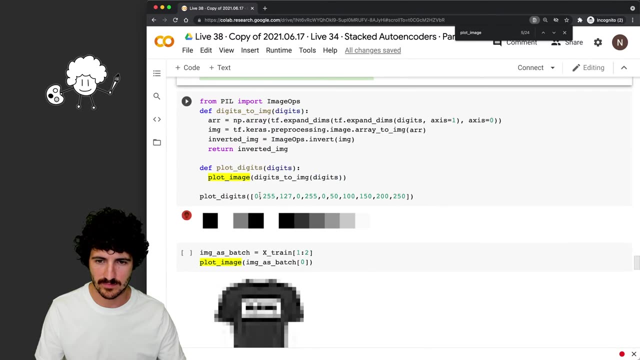 And, uh, I think we also have something to plot: the digits. Maybe, maybe not. I'm going to say, okay, Let's start with this one And then we are going to plot it. So let's start with, uh, say, we have an input that is in the system. 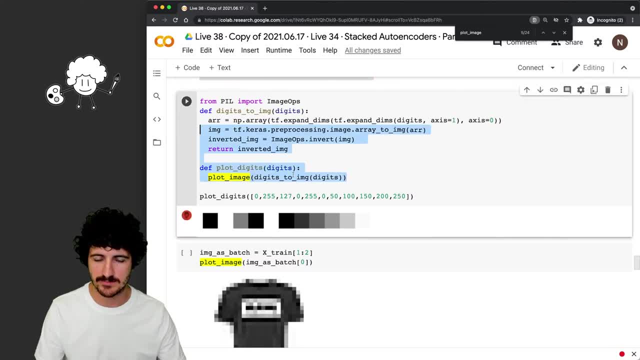 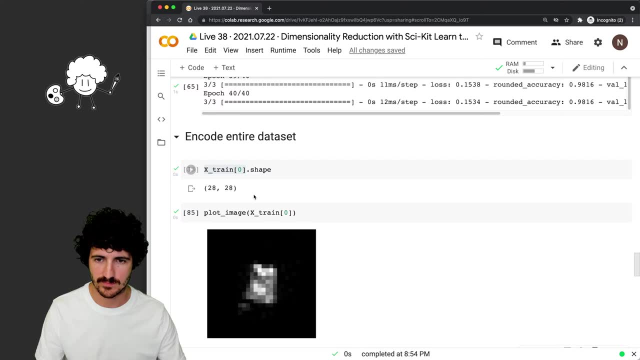 We are going to, let's say, the input, I'm going to design the input and we are going to sort by the input. Let's say that I would like to use this input value. I'm going to apply the input value, So my input value is zero to zero. 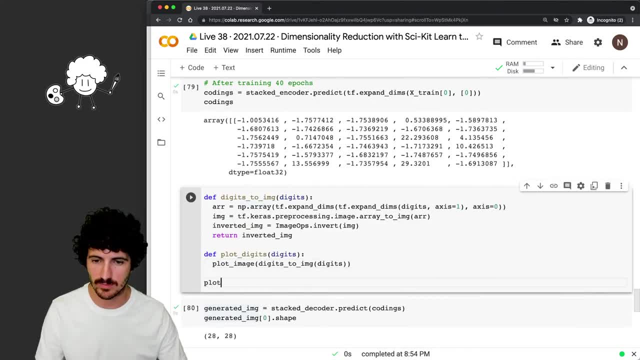 And then we can see it. So if it is zero to zero, Right, So Yes, We're going to change it All, right. So let's say plot. so let me see plot digits. where's plot digits? Yeah, 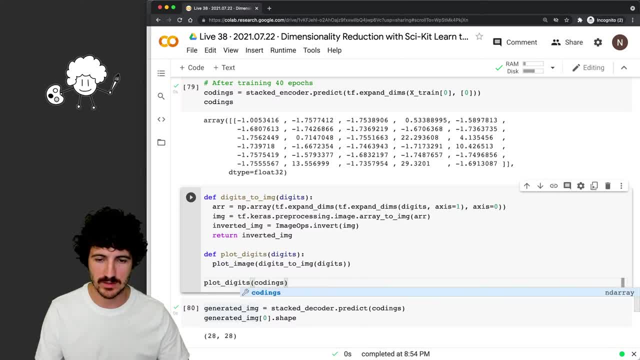 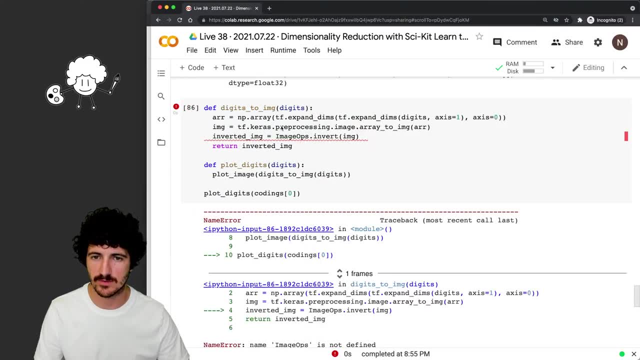 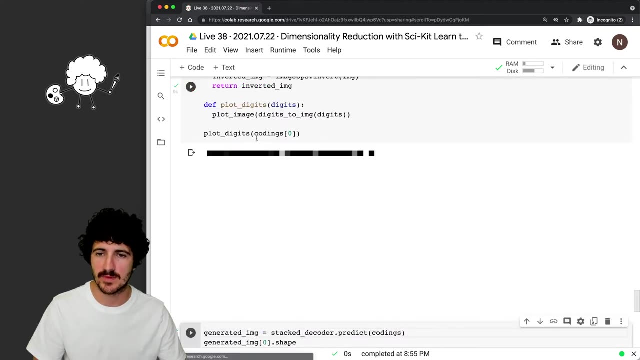 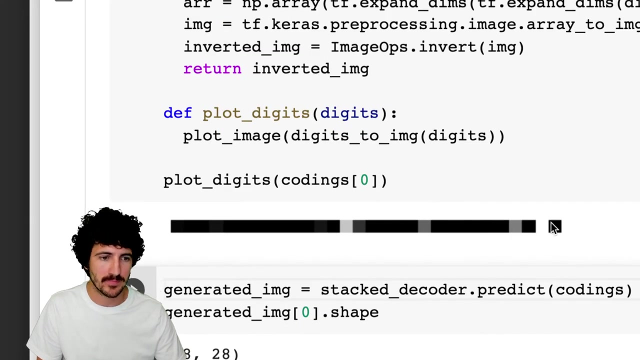 Plot digits And we do those codings. zero image ops is not defined, All right, And we'll probably have to put all of these dependencies, um, in the same place, All right, Right, So those are my coatings, So they go from. there are 30 digits, from zero to one, and they're 30.. 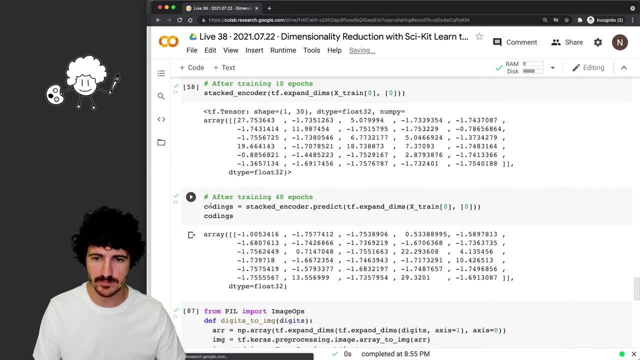 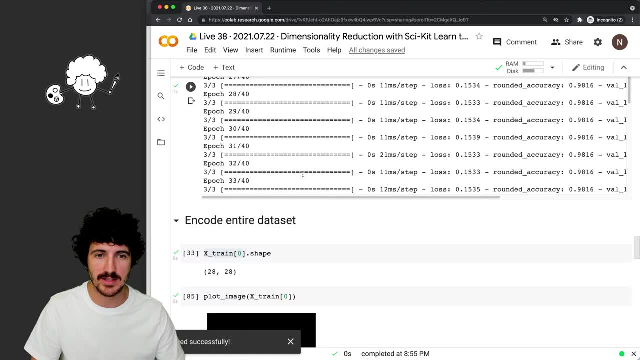 And depending on when you load them- So like at what point or after what training they- they change All right. So let's actually just do one thing: I don't really know how these will affect or overfeed or whatever, but let's say we 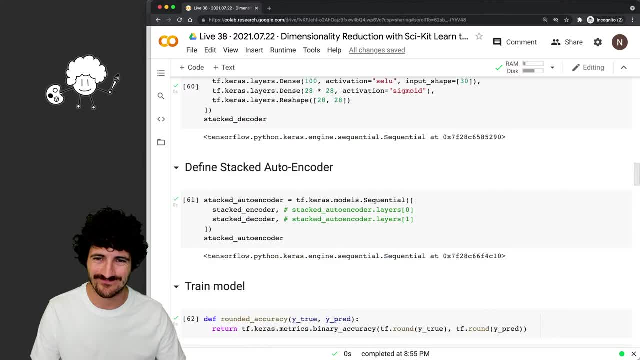 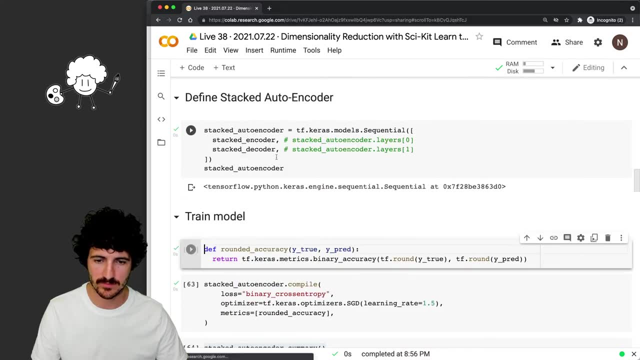 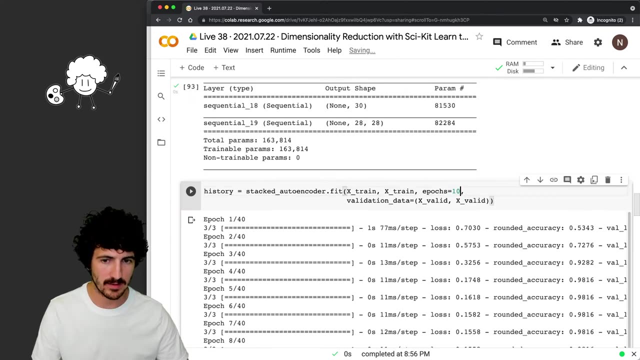 because this is pretty fast. um, we define the model, Boom, We do these definition here, We train summary, and then we're going to train for 10 bucks, Right? So still, the model always gets to the same place, right? 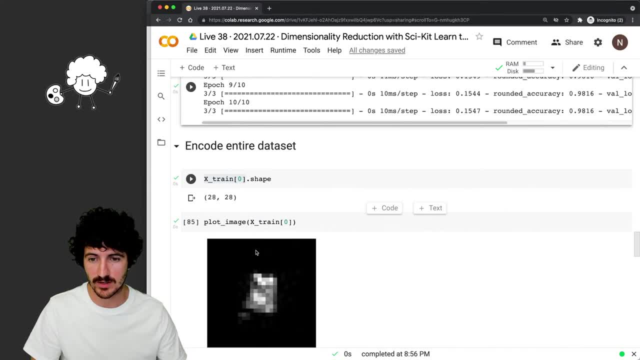 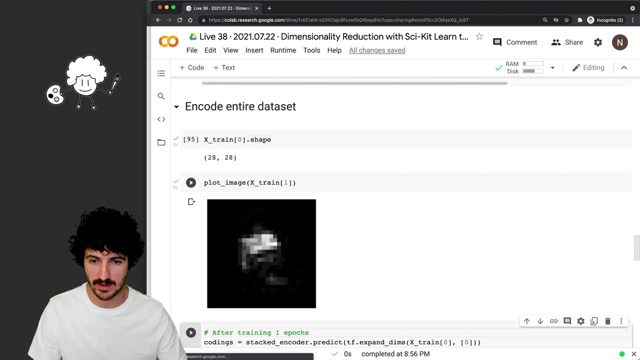 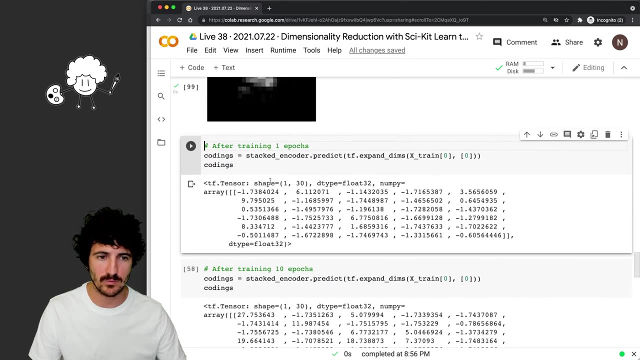 Um 99, 32 accuracy, and that's 10 epochs. So we still have the same input. We could maybe take this one or This one right. These are different sketches And we pass that through: this one that says there wasn't 10 epochs. 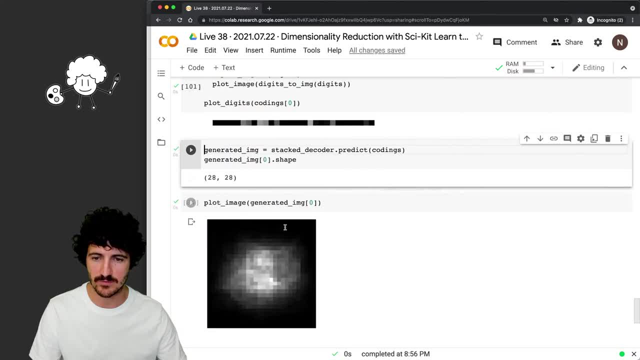 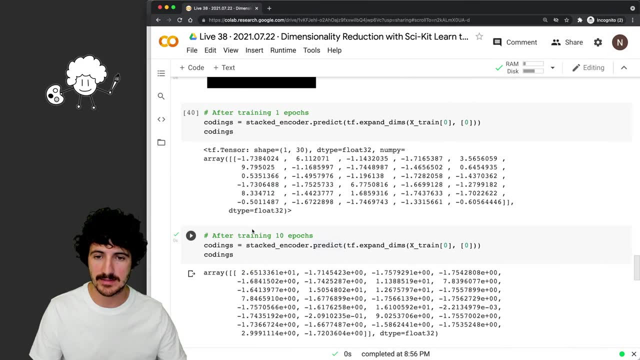 And now we can plot our digits right. It's slightly different than before: we generate an image and now we predict. So this is a slightly different than before, And you know we could actually just comment this out and we're going to take another image. 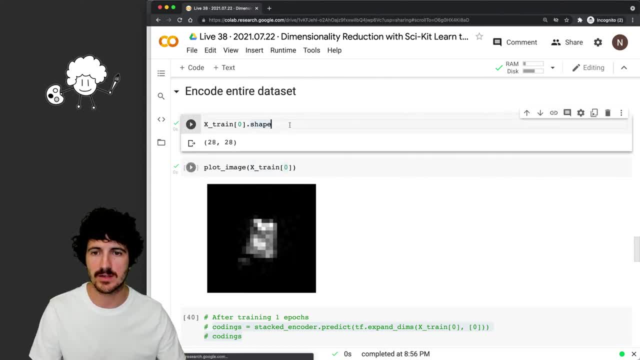 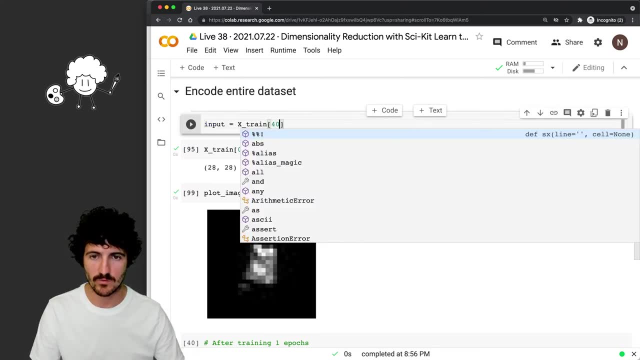 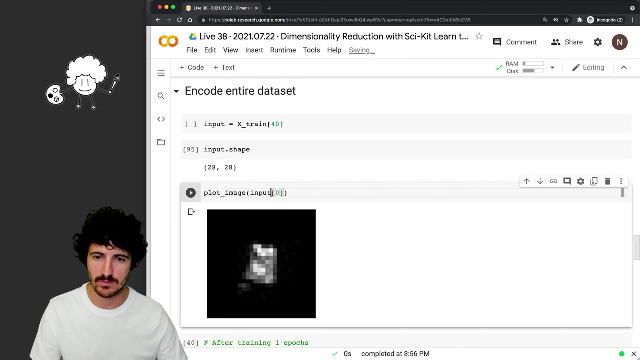 So let's say image, image 80. So let's say Um input is going to be X, train 40. Right, So now we just do this, So you just get the input. Please don't need to do a lot more input. 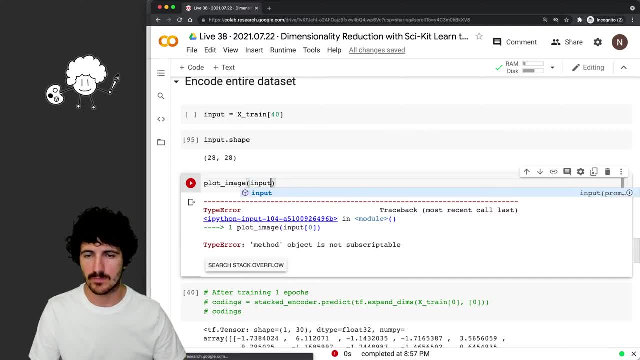 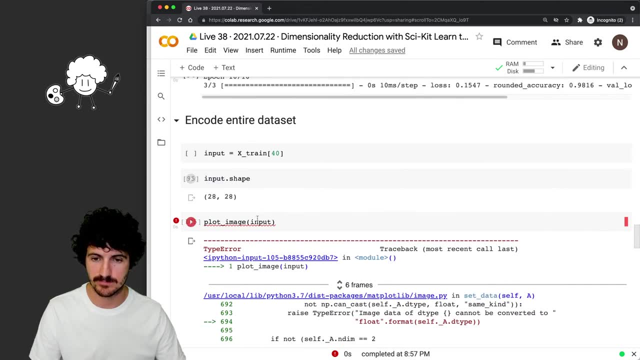 Now Give me a minute. Yeah, I'll try. I'll try. Okay, So let me just you know if I hit it in the hole like this. Oh, it's the same thing, I'm just going to copy and paste it in an image. 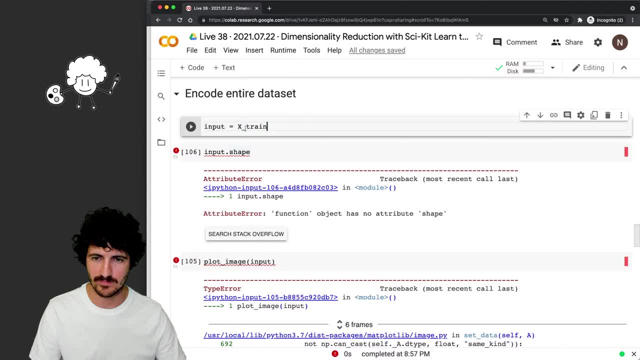 You can see it as the same thing. It's the same, It's the same. If I see I'm going to hold it up here And then I'm going to do like, oh, it's the same, but it's right here on the edge. 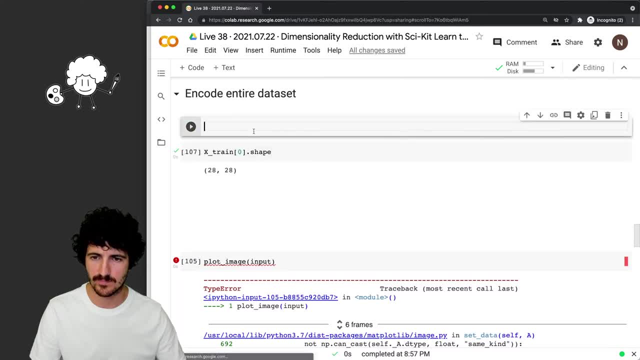 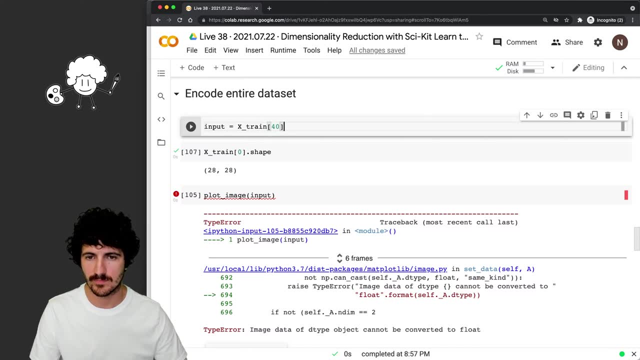 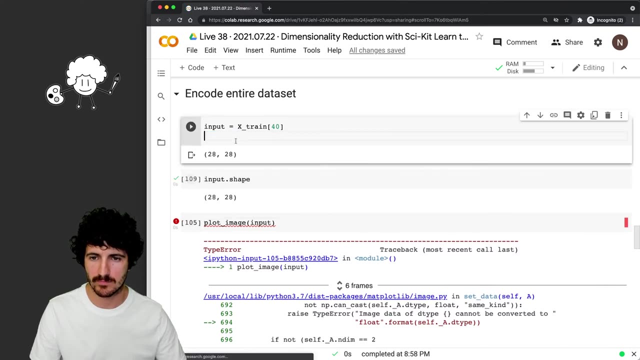 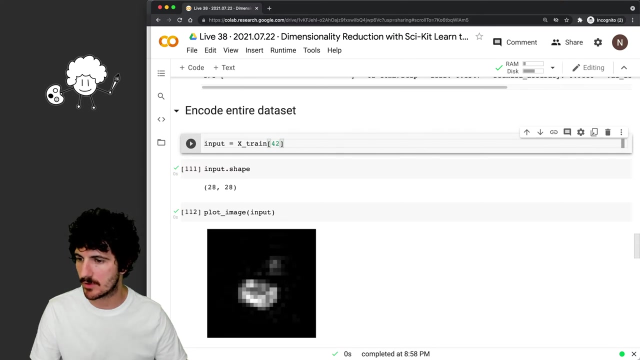 You'll see that it's the same, It's like that. So I've got like you've got to put that in that box right now and you're just going to kind ofling it. Okay, All right, So this is our input and now we can choose from here with a number. 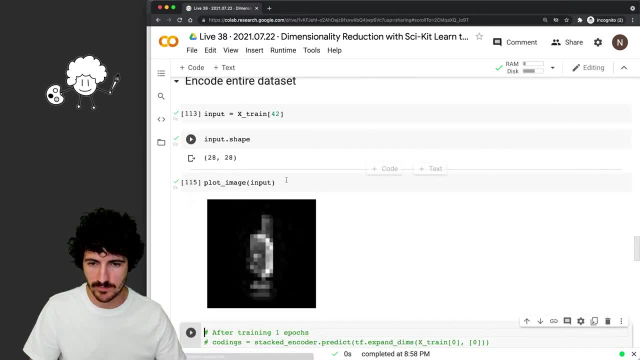 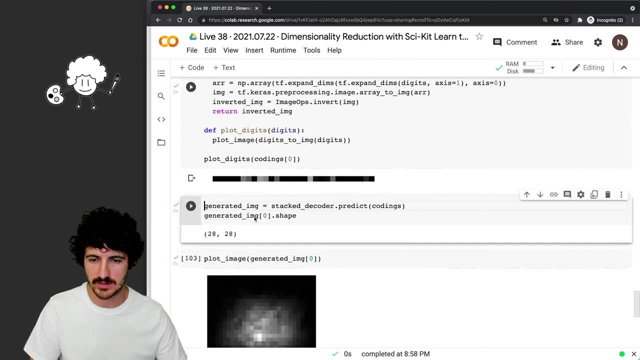 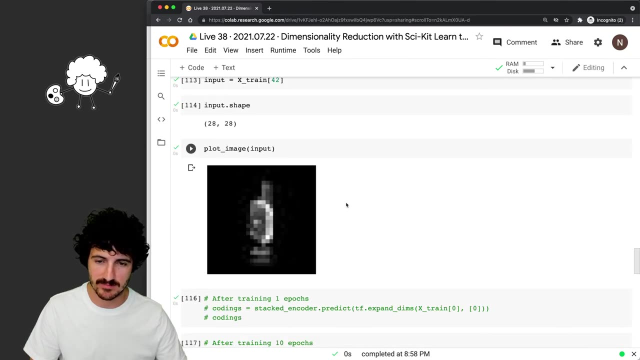 So we say the input is a sketch 42. We have that And this doesn't do anything. This does any something. Now we plot our digits and now we reconstruct our image, which doesn't look anything like this at all. So I don't really understand what's going on with um, with the data, say. 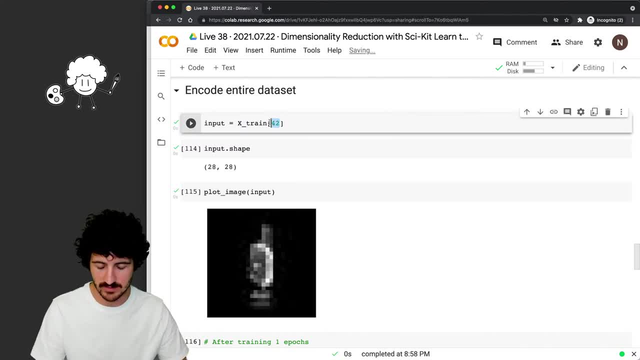 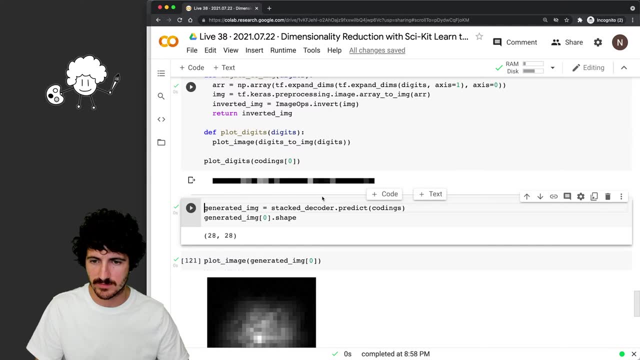 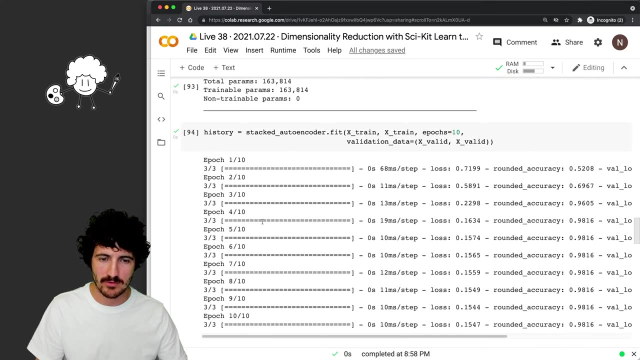 it might be. it might be that it's overfitting and it's just like learning something, that it does something really similar for everything, for all the images. Yeah, So it doesn't seem like it's doing much, All right. So one thing, one easy thing that we can do here is because we've used the 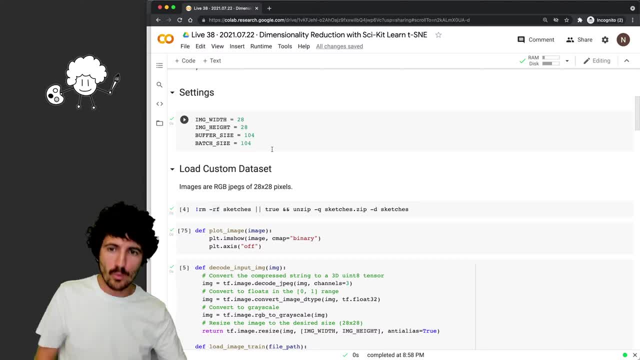 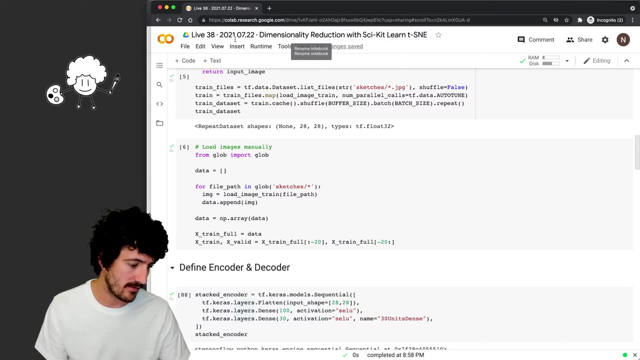 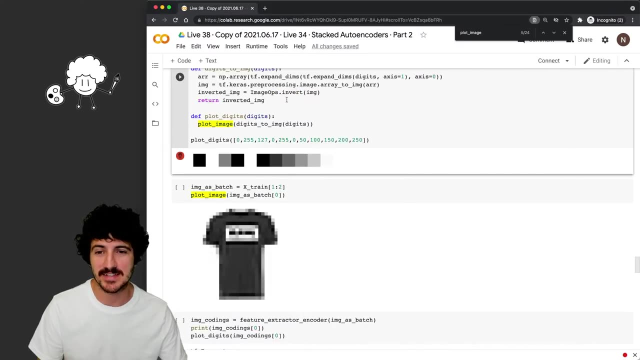 same, the same variable names. right, We can? um- uh, you, you have to think about this. right, We have 104, um sketches in the the. the fashion MNs data set has 60,000.. 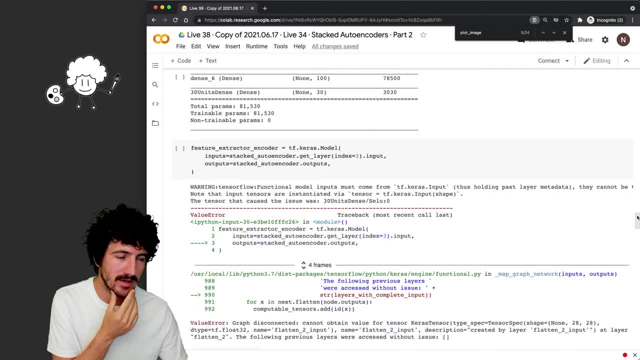 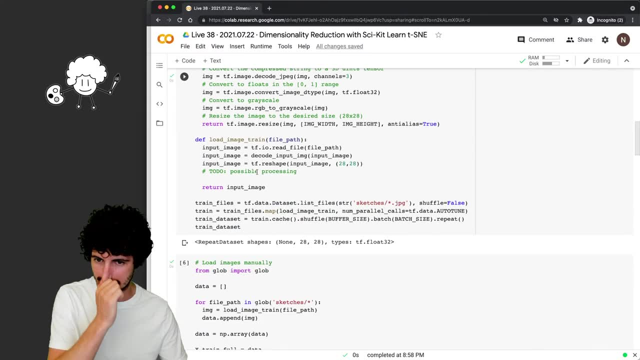 So That's Probably one of the things why eat uh is performing so much better, Right? So what we're going to do is we're going to load that data set. Now we're going, after all this effort, to load our custom data set. uh, we're. 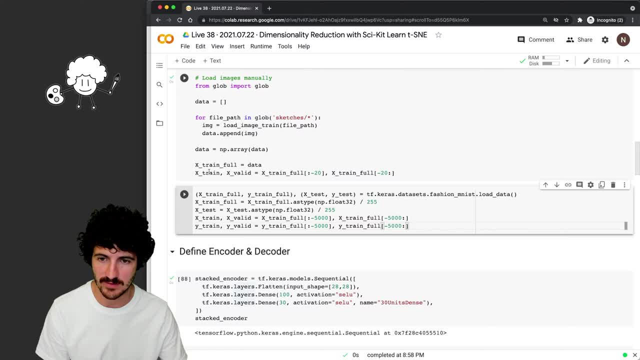 going to define here their data set. So the we're going to have the same X train X valid um data set. I don't think we need this part and we do need this one, So we're going to load that. 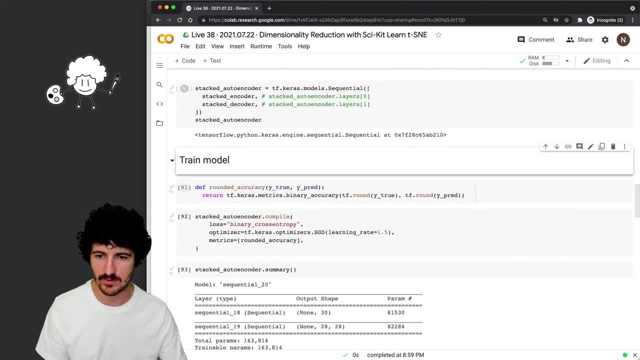 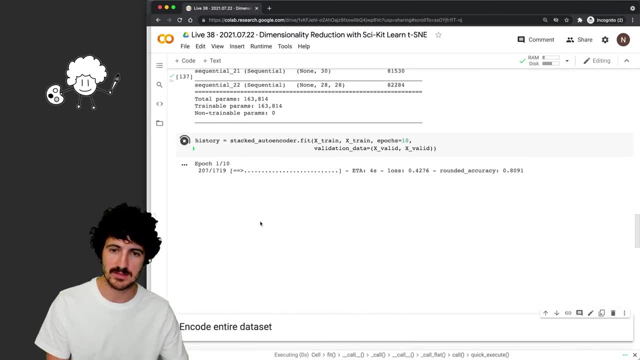 We're going to Load our model, We're going to define everything the same way And we're going to train for tenant books. Let's see how long this takes. This takes a bit longer now because we have a bunch more images. 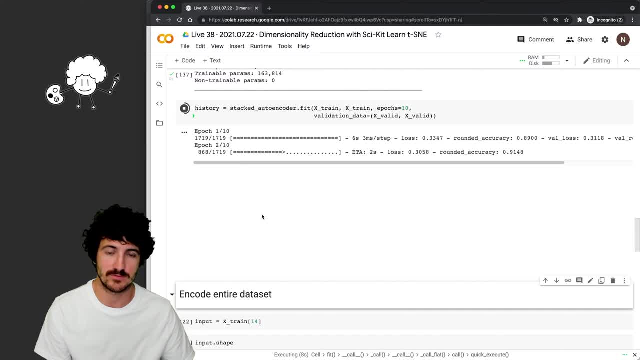 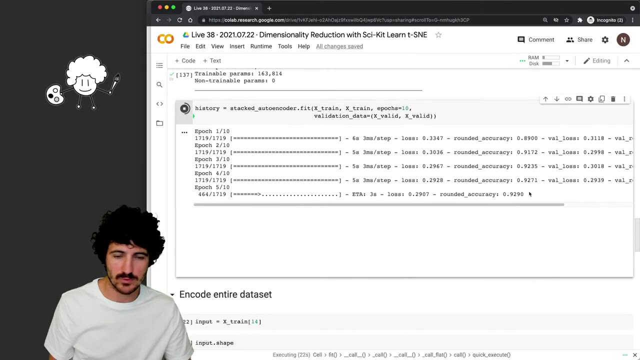 We have um 55,000 images for for training and 5,000 for validation. And uh, you should be uh thinking right now. the accuracy is slowly going up. It's not as fast As it was going up before. 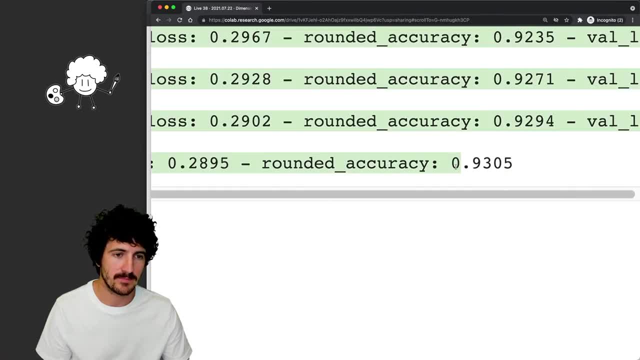 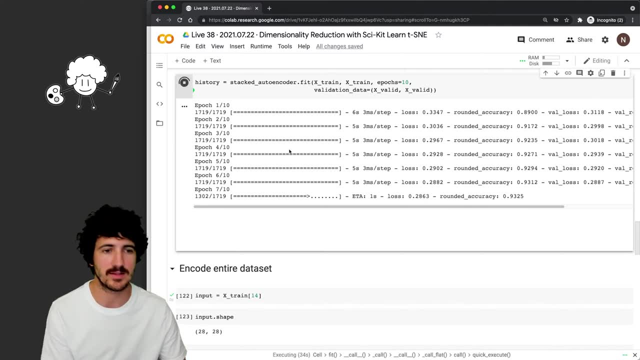 Right. So we can see here: this number keeps changing and, uh, that's good, Right. This means that there is some actual learning that is happening, not just that we're overfitting on a data set and learning a few things. 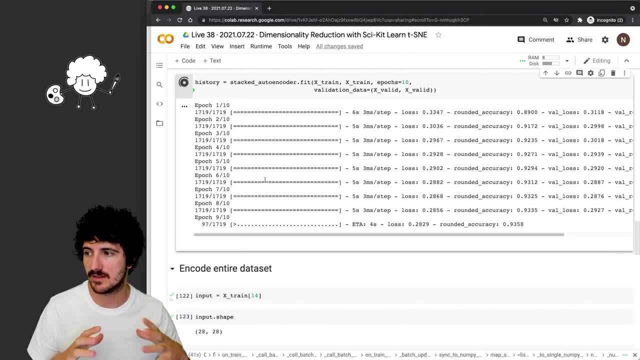 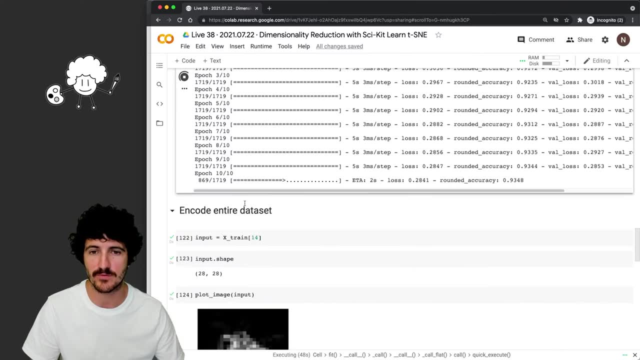 And uh, yeah, I would be interested in seeing this network how many data points it needs to to give any like some information that makes sense. Let's try it. I mean, I I'm not sure if this is going to work, but all right. 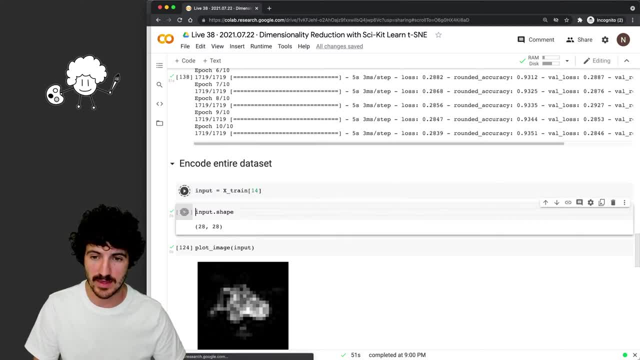 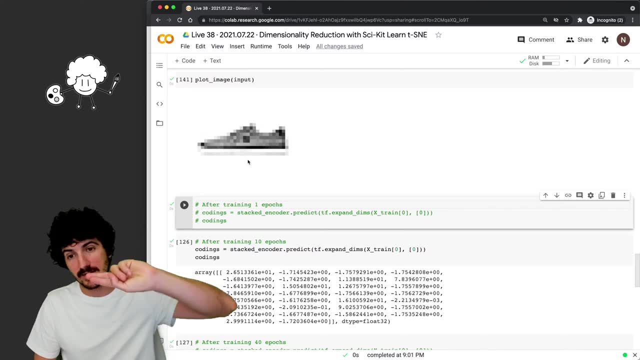 So the model is trained. Now we can put a input 14 here, but is this? that looks like a shoe? I also look that the data set is inverted, So that also might make it learn in a different way. So we get the coatings. 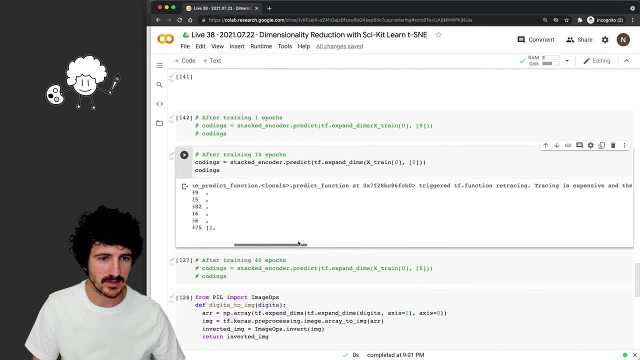 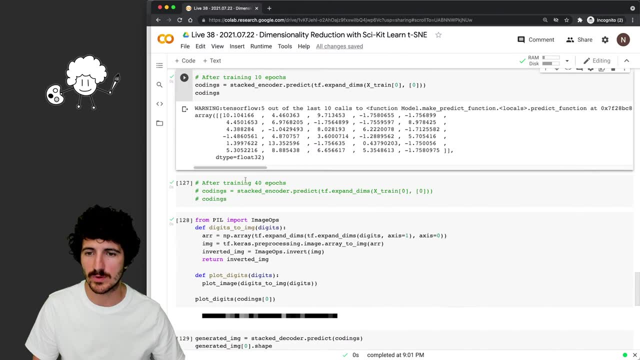 We still get Oh, five out of the last 10 calls triggered to function. Retracing is expensive. If I'm here repeatedly, blah, blah, blah, All right, But we get our data and now we get our coatings right. 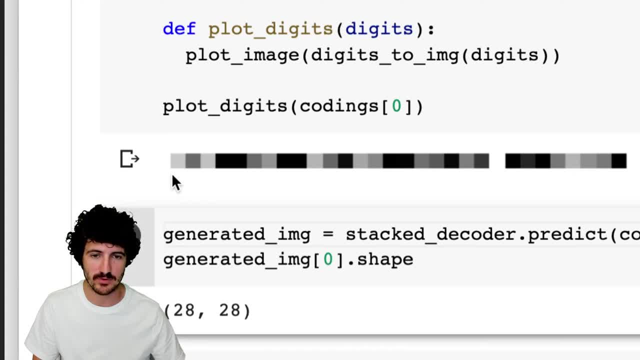 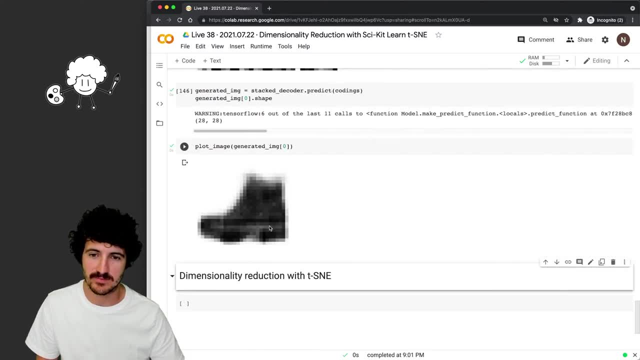 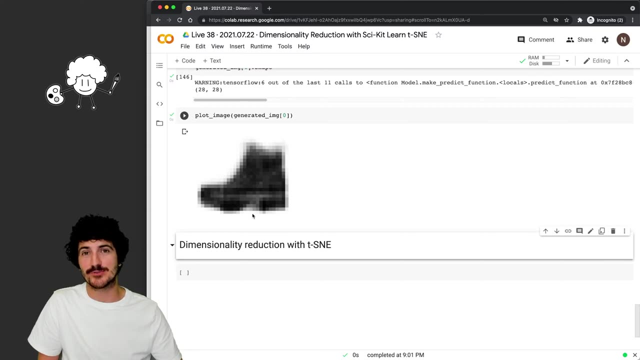 These coatings may a lot more sense. It's it's a bit more granular, It's not just like a lot of black and uh, we get our generated image here All right. So it doesn't look anything like it, but at least it's a shoe, right. 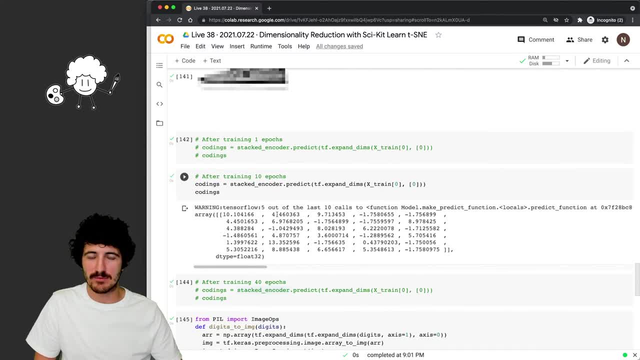 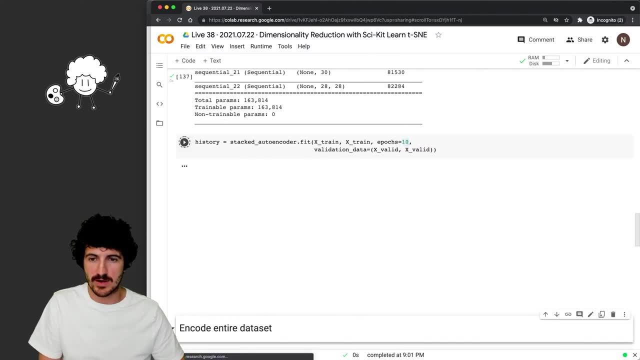 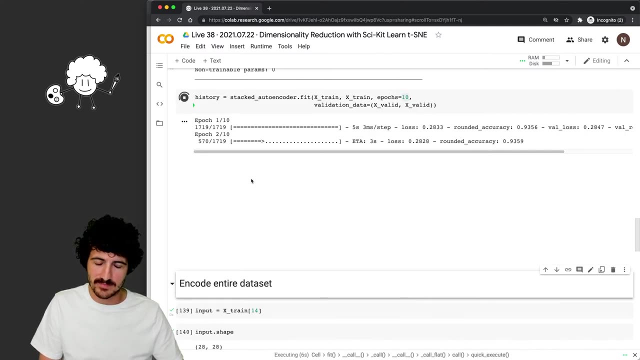 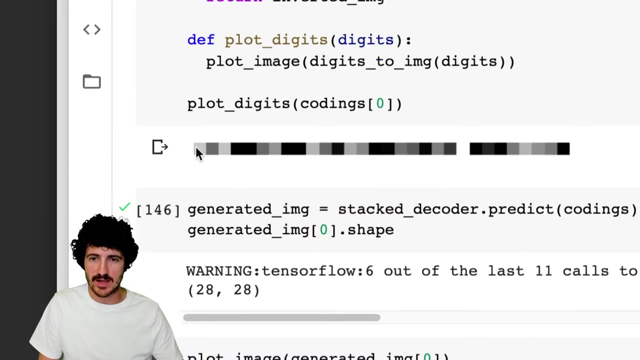 So it's learned something and it seems like we're able to reconstruct the output from What we have. uh, let's actually just train for for 10 more epochs and um, and see where we get Just to. to let you know. while that's training, these coatings here actually represent the issue. 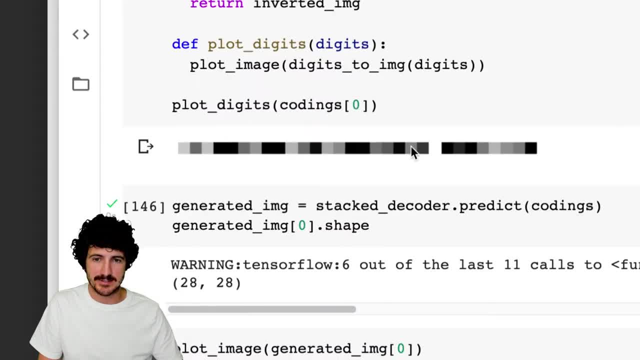 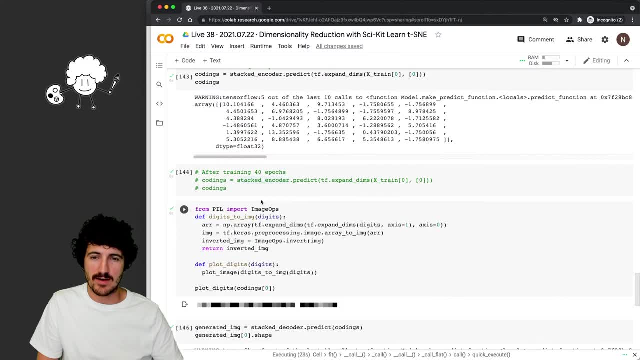 If we modify these um coatings, we're going to get a different image right. That's kind of like: Uh, puppeteer, Like we, we have an image, we're encoding it into this image and then we decode it back. 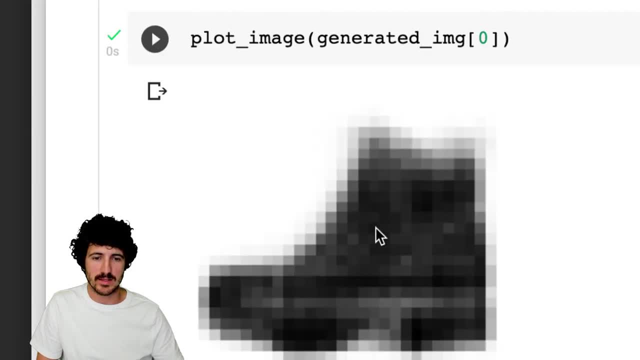 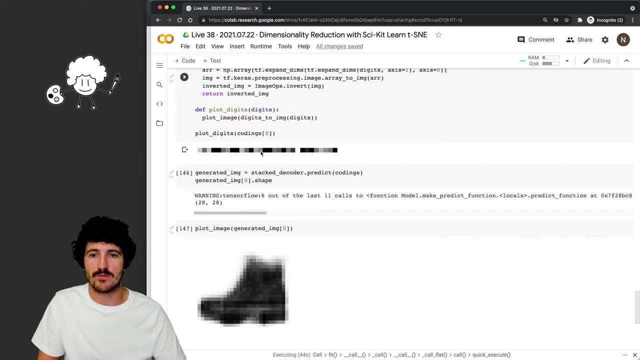 So if we generate images like this one, we will get images like this, And there is a correlation, of course, because of the weights that the neural network has learned from the coatings to the output. All right, So it seems like we're almost done. 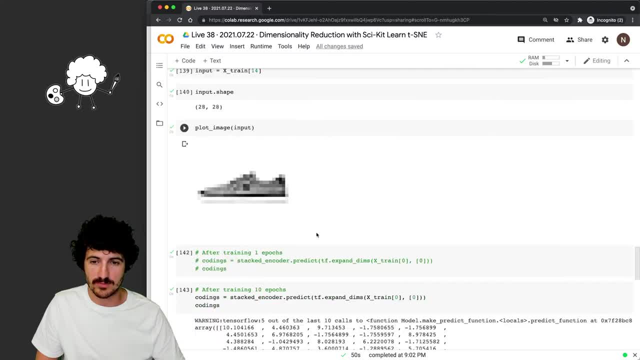 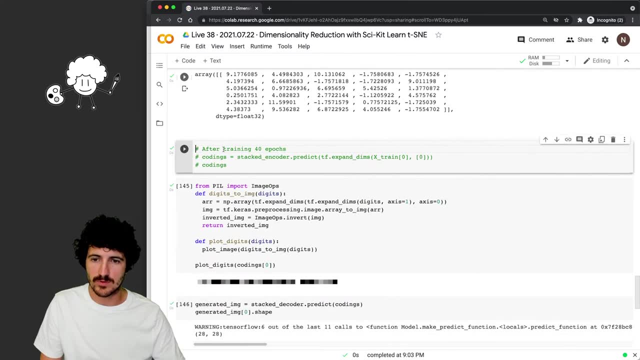 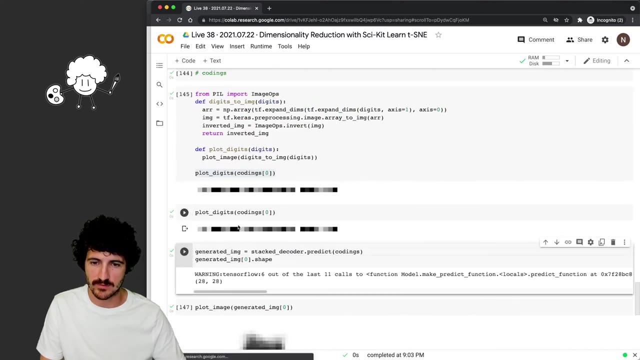 We have a bit more accuracy- Not too much more- And uh, we are going to use the same input. Uh, I'm going to do one thing: I'm going to leave this here and I'm going to compare, So, how the coatings are different. 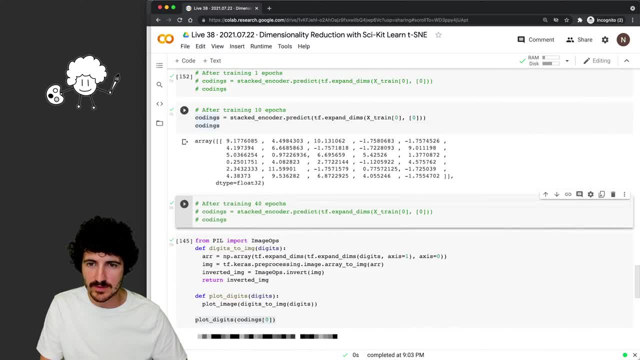 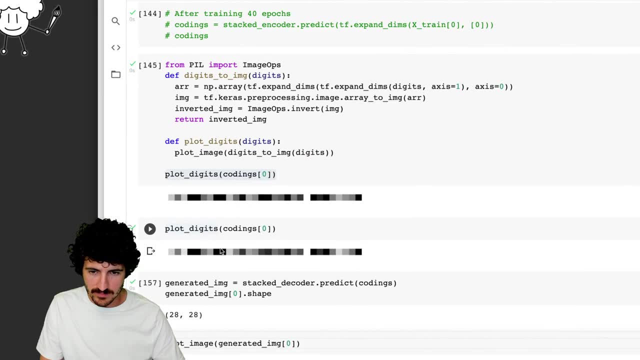 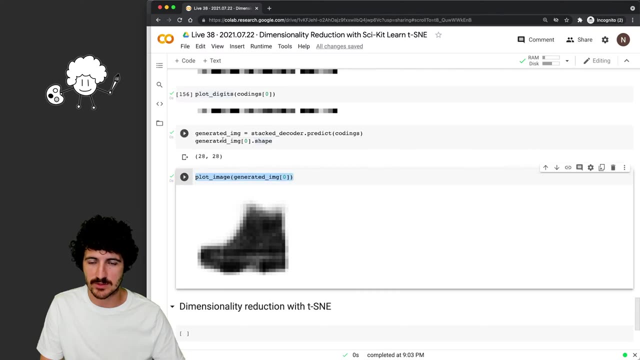 They are almost the same. So I would say, let's regenerate this as in case, uh, generate the coatings. They seem to be almost the same. Let's see If the decoder has learned anything else. right? So we have the image here we're going to predict and now. so I'm going to put it here. 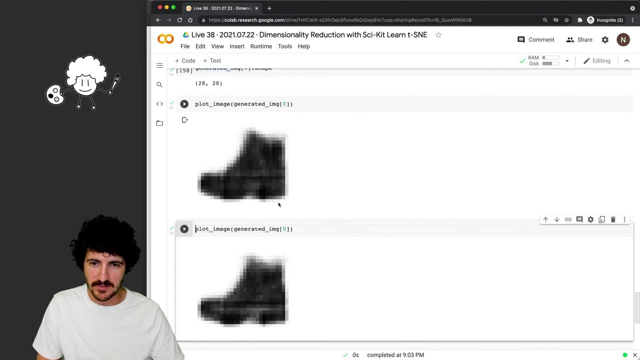 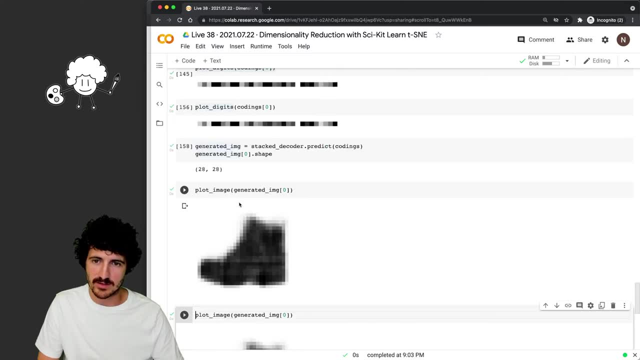 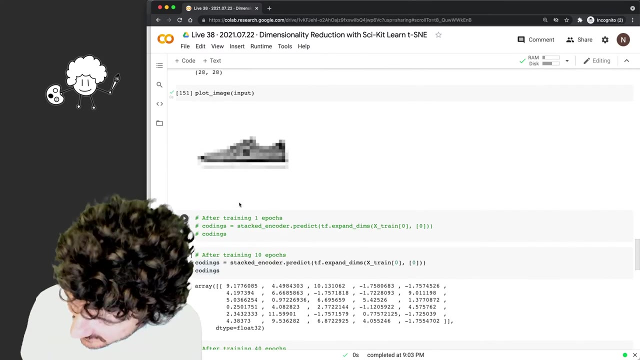 So I'm going to regenerate a new image and you see, I mean I can already see some, some changes in there. so it's not okay And let me just double check something. Okay, cool, There is a slight change. 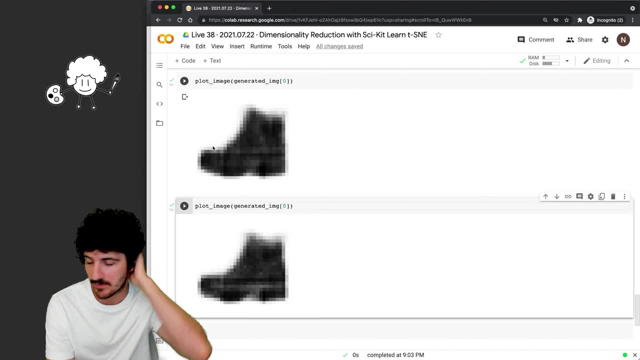 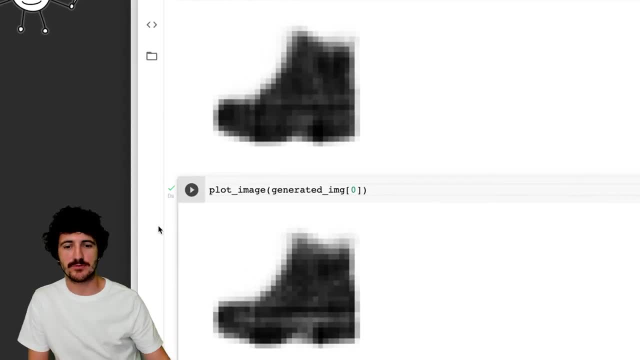 I'm going to say: Right, Uh, I made an errors, I made a mistake, So this has changed. right, So we can compare these two images and they're different. So there is something else that the network is learning while we're retraining, right. 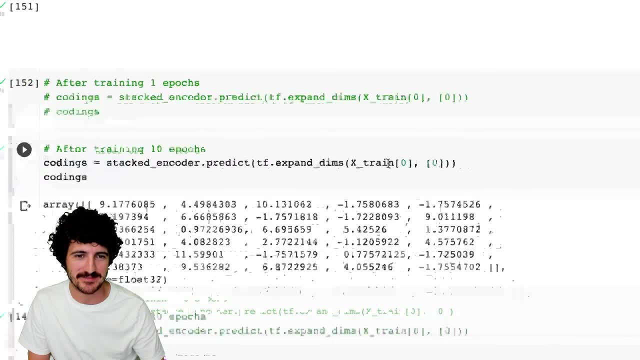 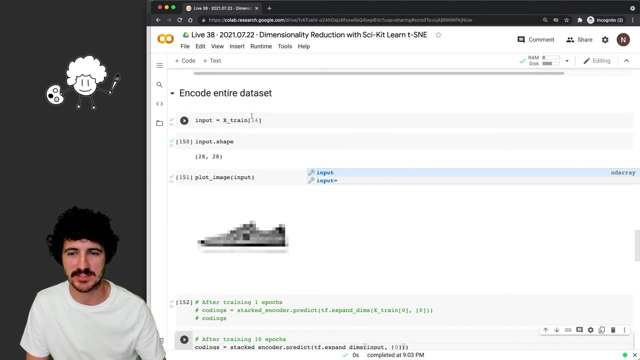 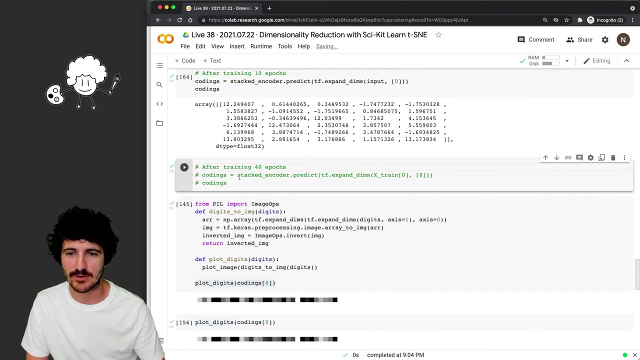 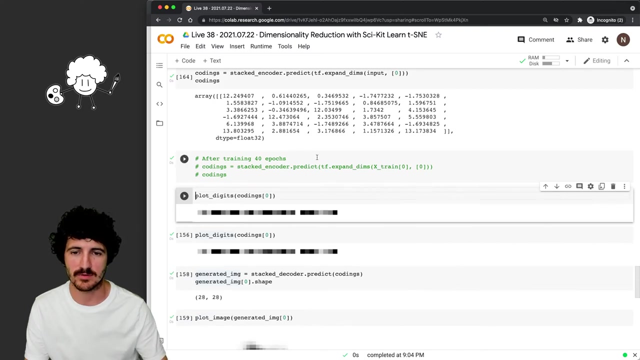 What is funny is that I forgot to change these variable here, So these should actually say input, because we were continuously using um extra in zero while we were visualizing here the number 14.. So if I actually Do this right now, you're going to see how the the coatings that we get- and I'm going to take this helper functions above the coatings that we get- are going to be super different, right. 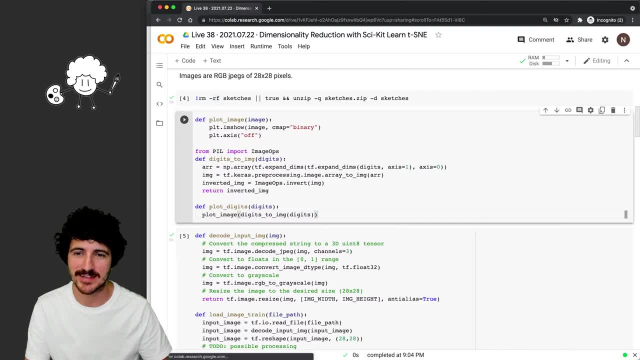 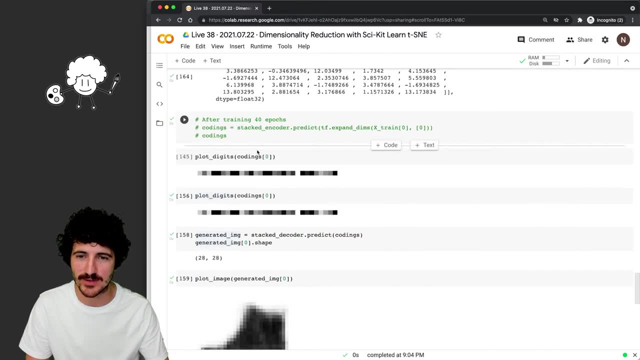 That's something that I've even realized and nobody realized, because nobody told me. So you should have told me. and, uh, that's going to change, All right. So look at the coatings now. So these coatings here are super different, right? 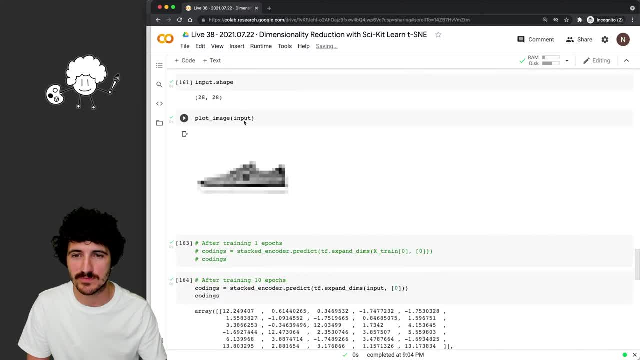 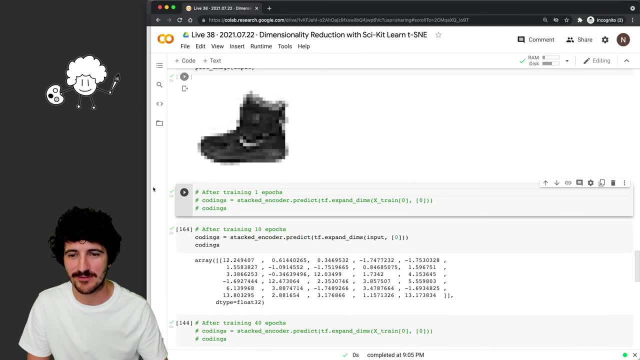 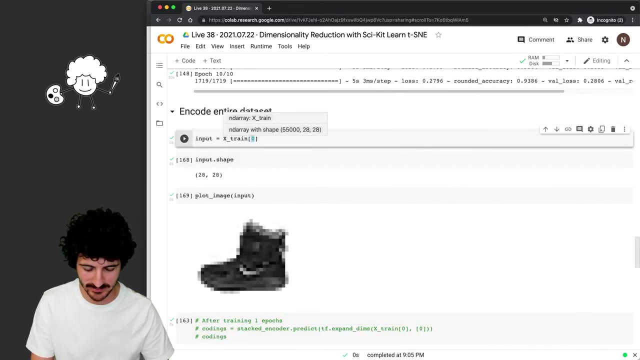 These Now Doing code D shoe right. Well, we can see, is that we'll go to zero and we plot that image. We indeed have something super similar to that boot that we were generating before, Right, Uh, which is, you know, it's super, it's super funny. 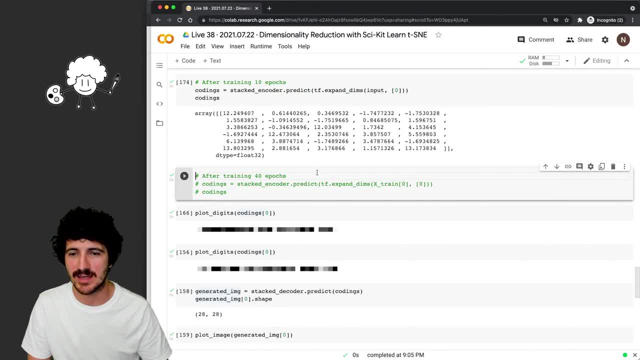 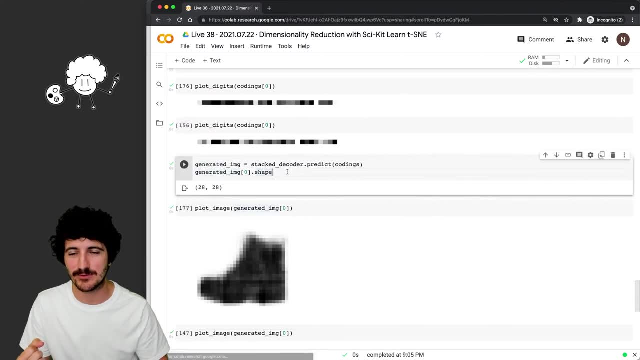 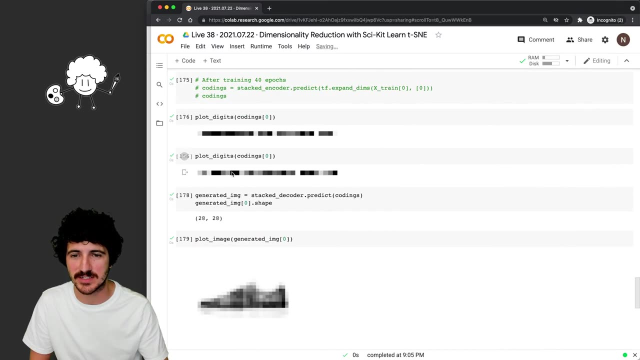 So we're going to go back to the, to the shoe. I'm going to go back and generate the coatings in Now. I'm going to generate that shoe and I need to predict before. So predict and generate that shoe. Awesome. So now our decoder knows how to generate a shoe that looks a lot more like that one and not- you know not what we saw before. 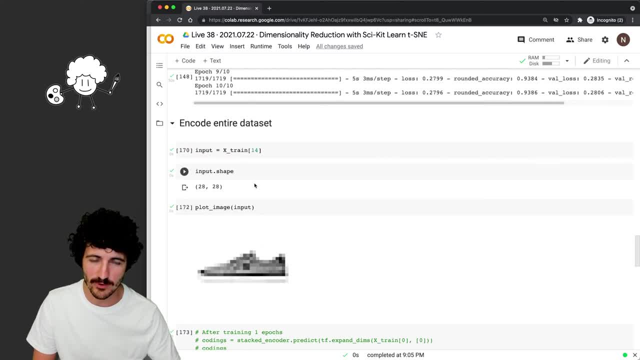 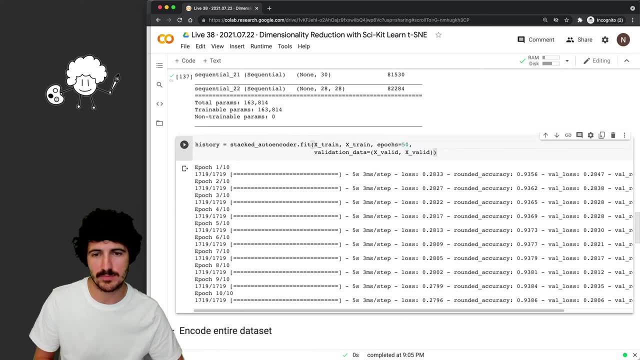 That was, uh, an error, right? So what these brings us, uh, or where these brings us, is like it's actually trained for like 50 more episodes, something that is going to take a bit, And, uh, let's try to take the rounded accuracy up. 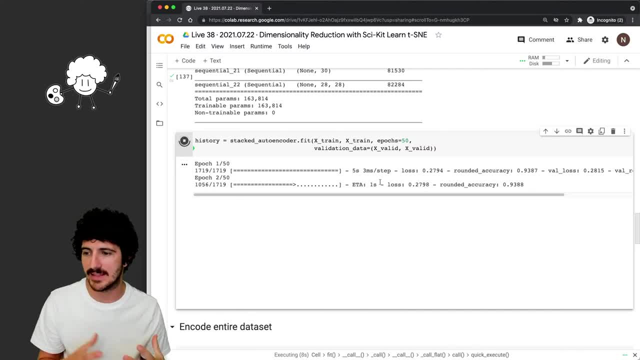 Let's see how the network learns differently. Okay, And later we're going to go back, We're going to use the data set of the sketches and actually verify if there is something that is being learned, because before, even though we were training, we were not changing the actual input that we were predicting with on the encoder. 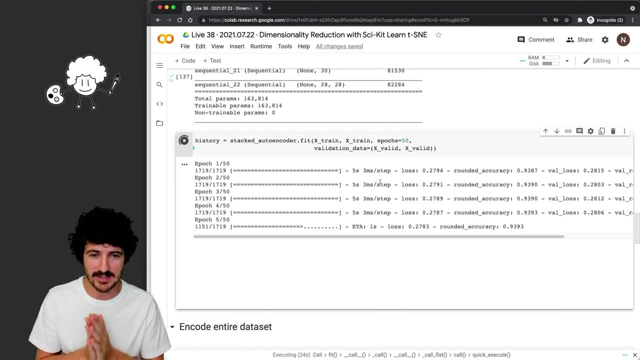 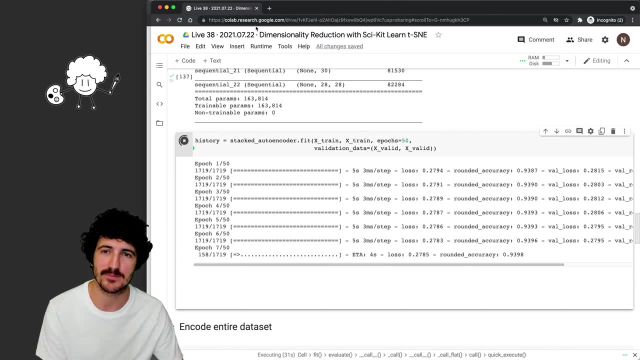 Right, So the the codings were not really changing, So I I do still have hope that we are going to see some, uh, some things there and and that this is going to improve a bit. All right, So um. 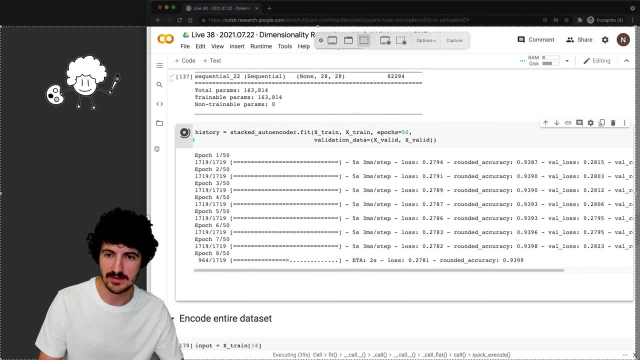 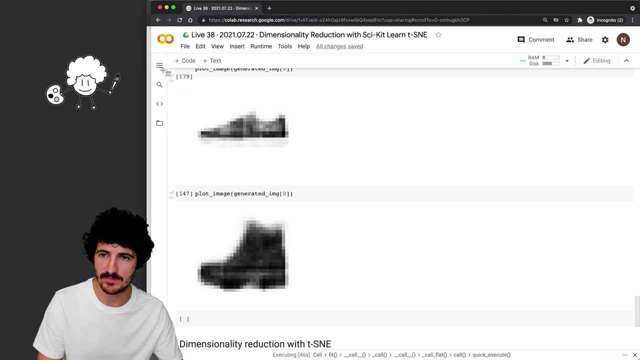 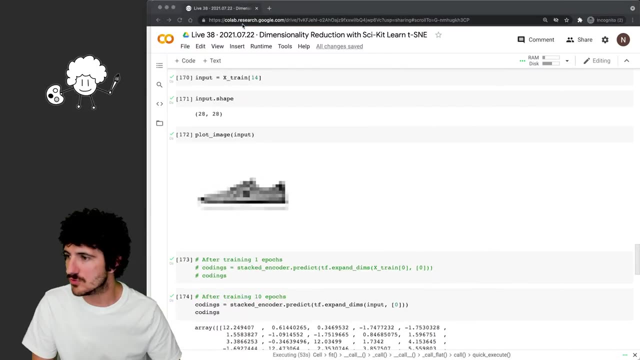 maybe I can. yeah, no, I'm not going to do that. All right. So yeah, maybe I can. maybe I can share an image or something on um. all right, Okay. So hello, Who. who's online? 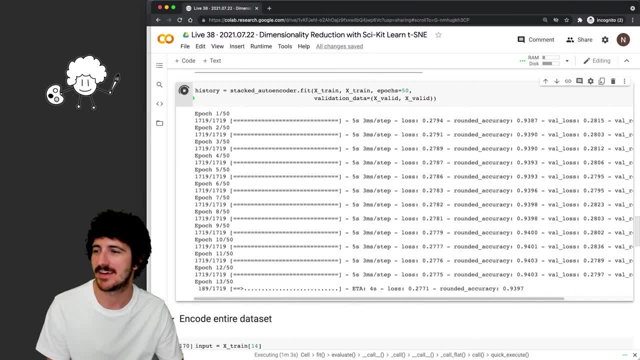 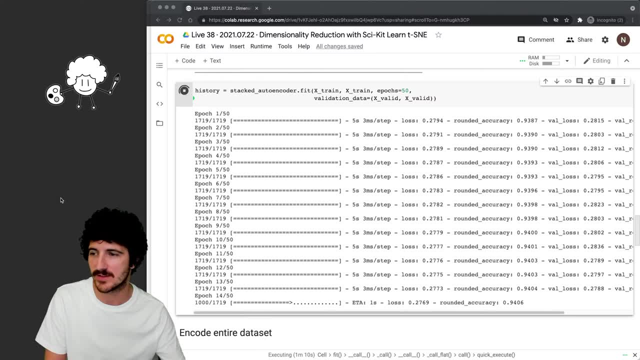 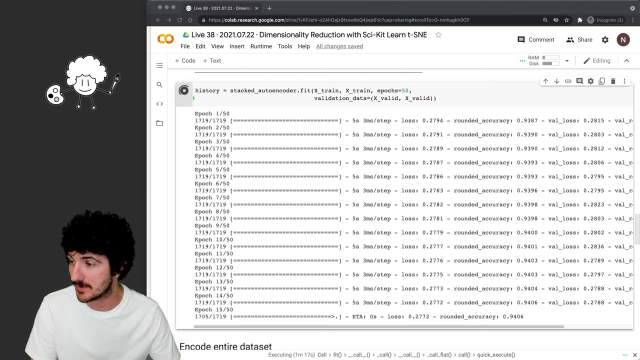 I'd like to ask, like, if you're online, let me know, Like I, I want to know more or less, Uh, if these uh pace that we're going through is interesting, or or you can grasp something if it's too slow, if this is something that you're interested on on seeing, um, yeah, because these you know the the fact of doing this online is mainly for you to be able to to ask questions and to to tell me what you would like to see more off, or um, like any comments that you have. 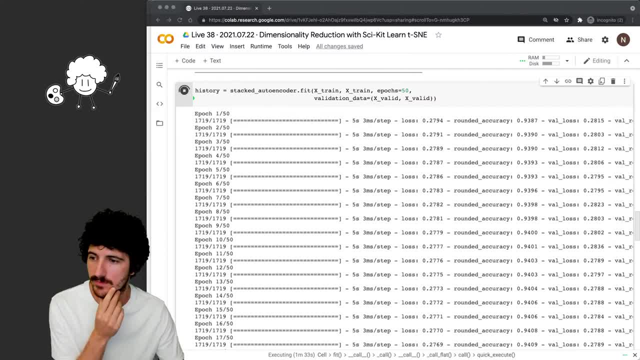 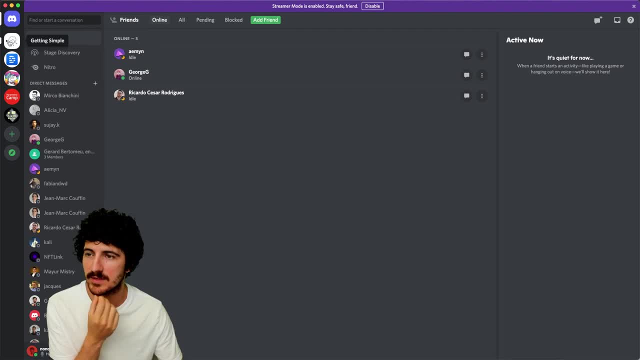 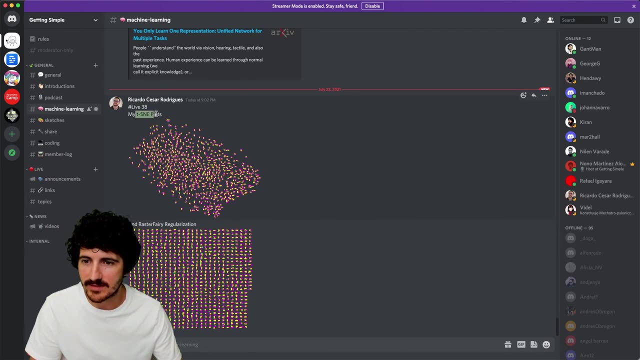 Okay, So let's see if there's any activity on the um, on the discord Server. So I I showed it before and you know we've seen him many, many times. Uh, it seems like on the machine learning channel. uh, life 38, my Disney's plots. 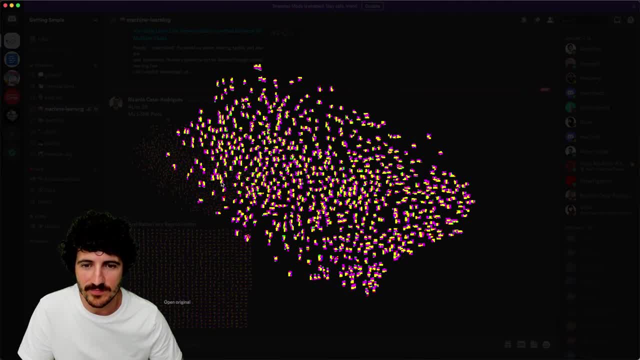 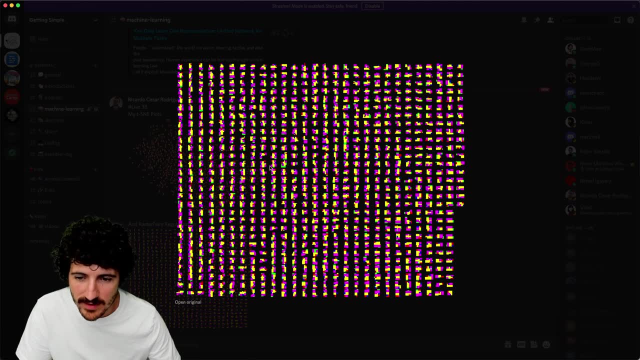 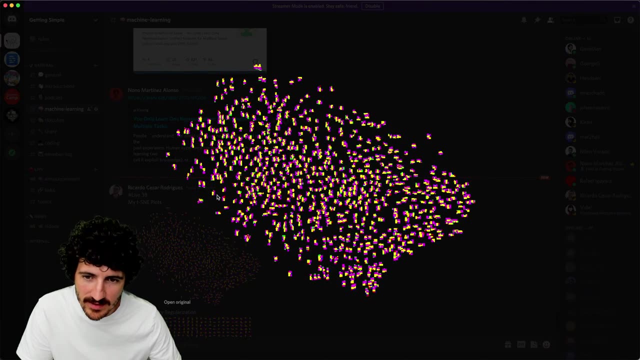 Whoa Awesome Is this? um, is this something that you've done today? I'm just curious, uh, or or is this something, um, that you had from before? This is, this is super cool. Um, these seem to be grouped by similarity, right. 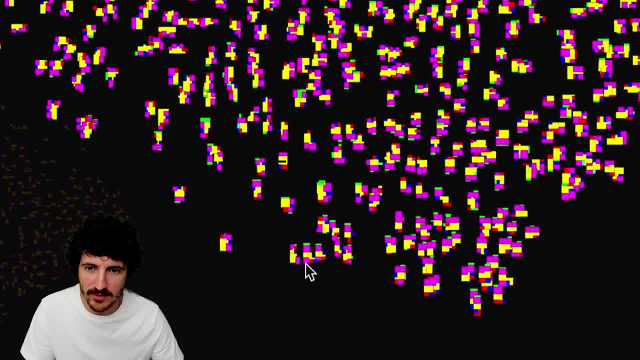 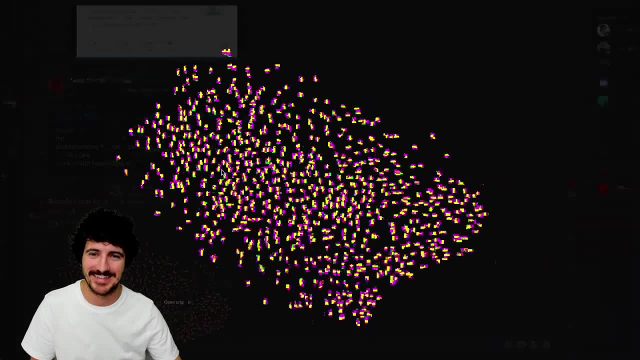 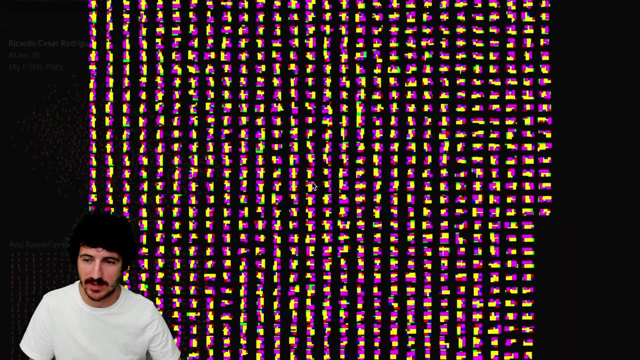 At least these are all like um vertical. Yeah, I mean, I can see some, some similarity. right, This is a really nice background. Um, yeah, So, um raster fairy regularization- Okay, Yeah, I would definitely like. 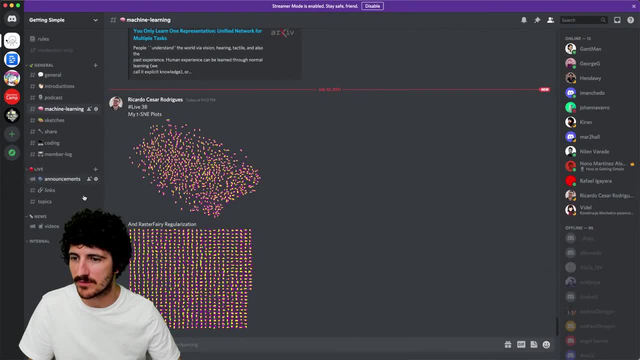 I'd like to learn more about these methods. I, I mean, I don't know if this is a different method I, I don't know anything about. great, I love this. Thanks for sharing. I just realized you shared a few minutes back. 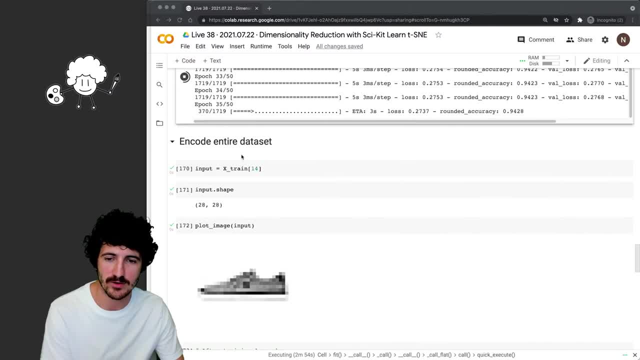 Uh, okay, So we are. uh, Epoch 34 out of 50. I'm going to grab some. um, okay, no, no, I sent a Disney plot on this court channel and regularized version of the Same images. 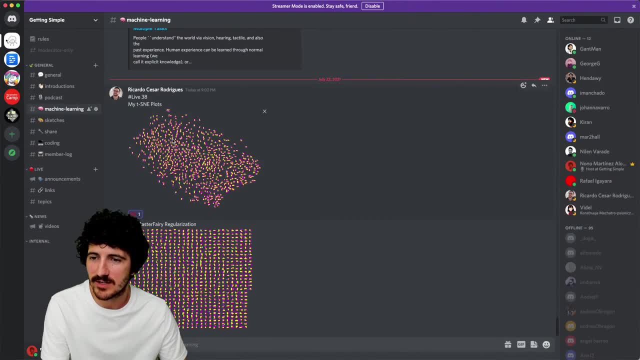 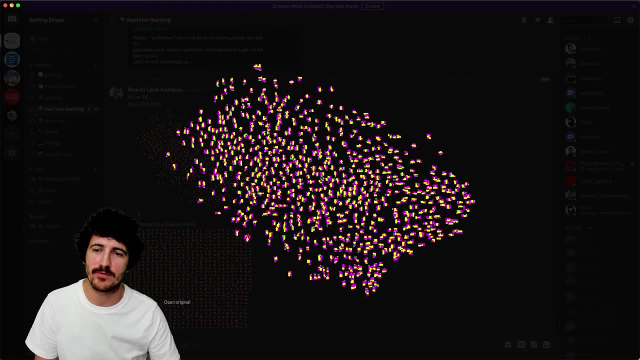 Check it out. Yeah, So I I'm checking it out here, So I I shared it. Um, is this something you've done following the life into there? You had this from before and you were showing us. this is really awesome. 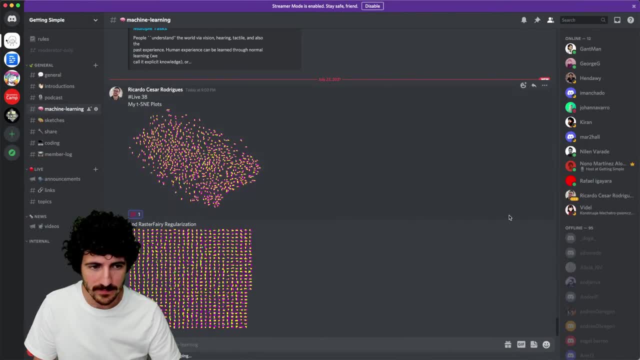 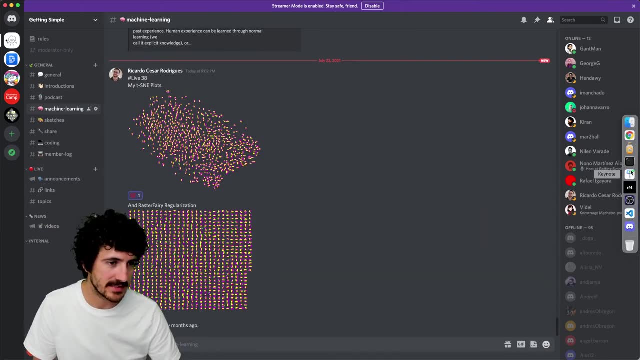 I really, really like it. All right, And while Ricardo is texting us, I'm going to go back here. I'm going to take. Uh well, let, let me see, I've done it a few months ago. Yeah, this is. this is really cool. 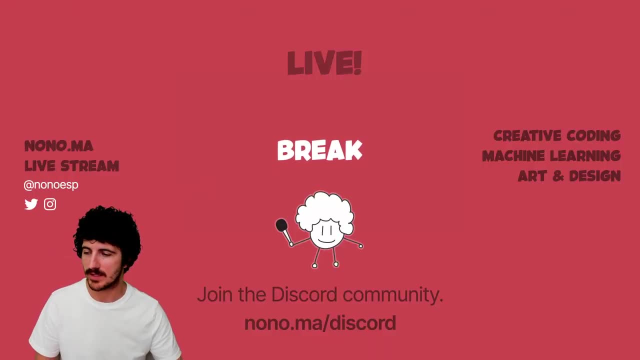 I'm going to leave you with this while this is training really quickly And I'm going to be back in a few moments and, um, we're going to continue. uh, looking at the at the Alton quarter. Okay, Let's go. 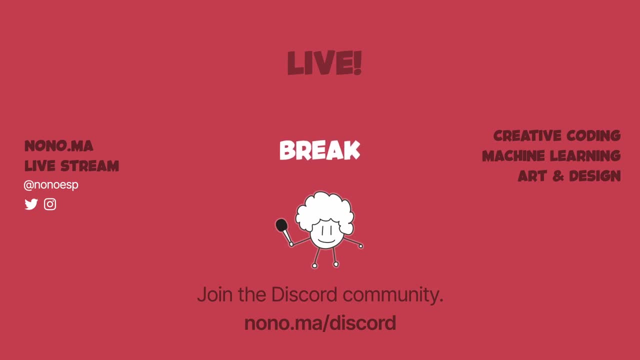 Okay, All right, you guys, We've got this, Okay. So the police officer finds out what happened to the man in his white van And he's like, yeah, I think the man in his white van took the car. The guy in his white van took the car. The man in his white van took the car And he's like: no, no, no, I don't believe you. He says yeah, Okay. So he's like: oh my God. Uh, they're like that's quite a bit more than you. 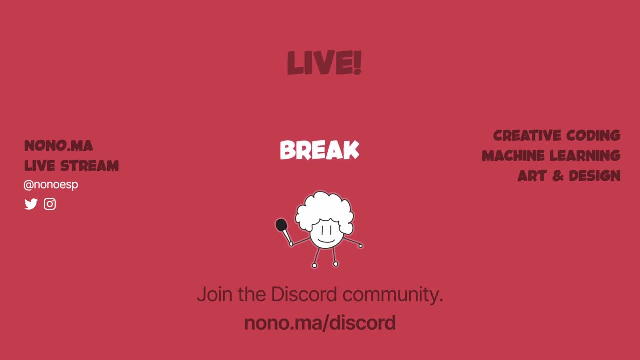 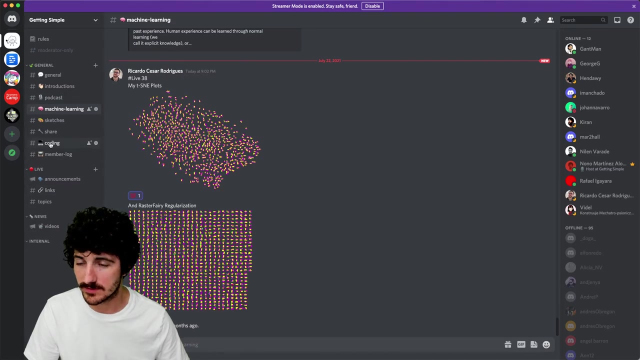 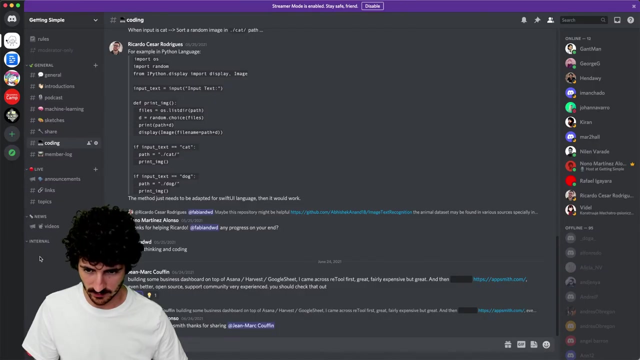 It's a little bit, Yeah, Something like that. you, you, you all right, we're back and we're gonna keep going cool, okay, so this is the discord channel. so I was mentioning before on the. on the coding channel, you can ask a general coding questions. that was for class, a class. 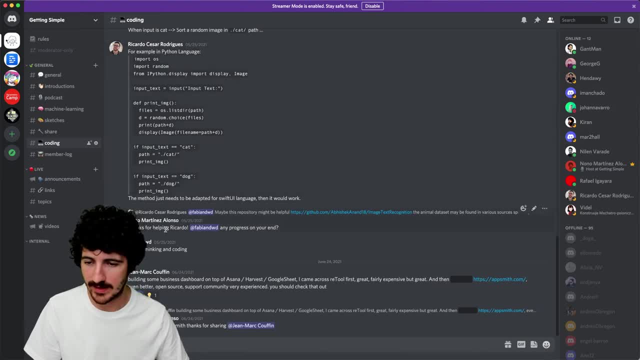 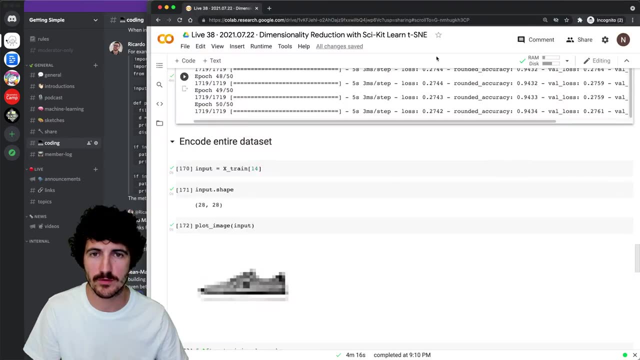 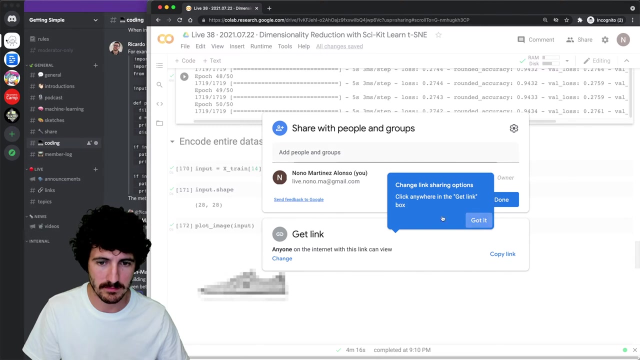 clues, I don't know how to pronounce up and yeah, so really cool, so whoever wants to go there. okay, one thing before I forget, so you can play with this if you're watching this. later I'm going to make this one to anyone on the internet can view, so we're gonna copy this and we're gonna put this on the links on the. 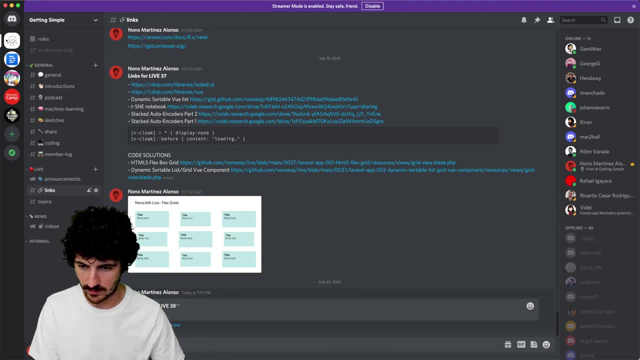 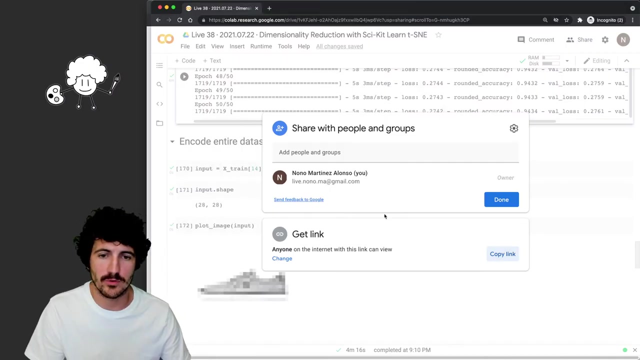 on this episode. so this is call that notebook and this is Disney. load data, start out, encoder, but no, but cool. and Ricardo, do you have a link that I can share there as well for for some of the projects that you've done? Ricardo, do you have a link that I can share there as well for for some of the 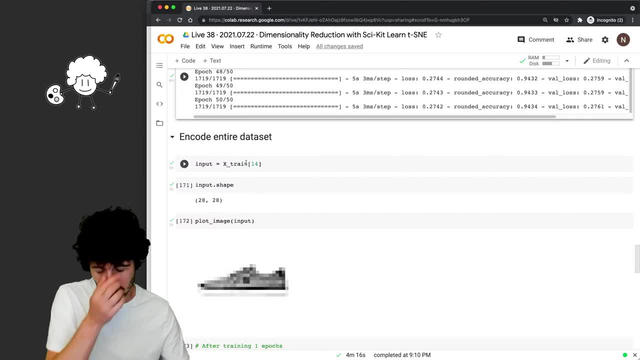 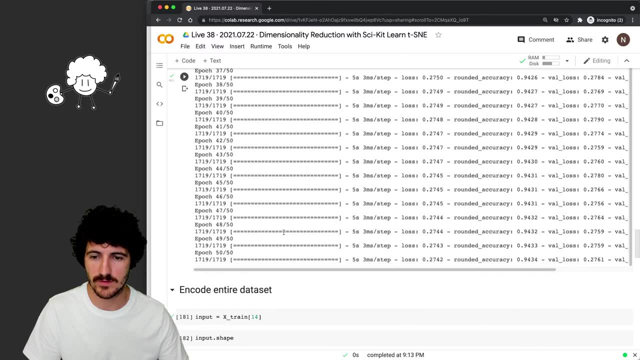 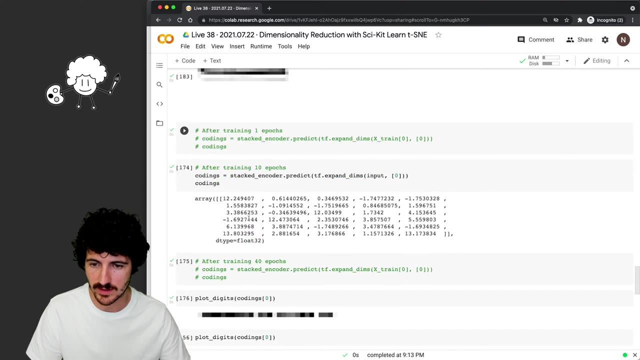 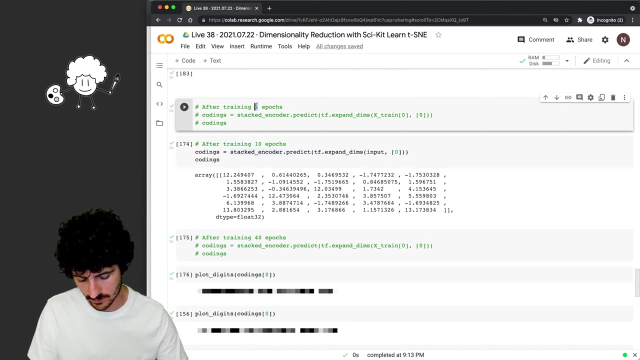 projects that you've done. okay, so let's go and see, we're loading. we've trained for, I believe, 50 more epochs, right? so we get an accuracy of like 94, 34, 94 percent, I think, and we're going to now. so here we get the coatings for I think, I don't know- maybe 10 plus 50. so 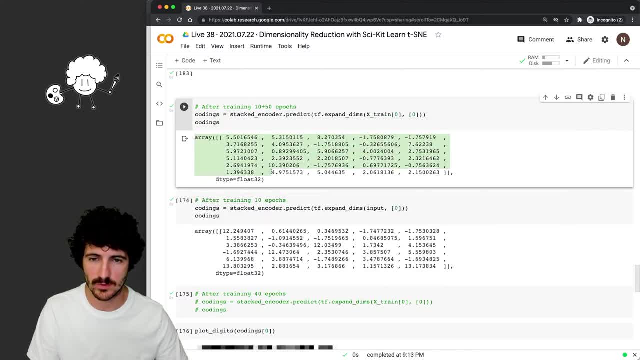 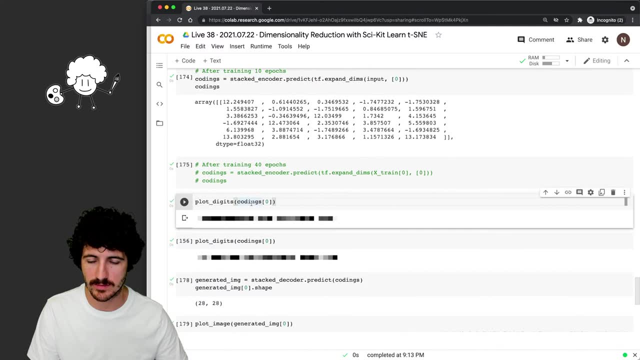 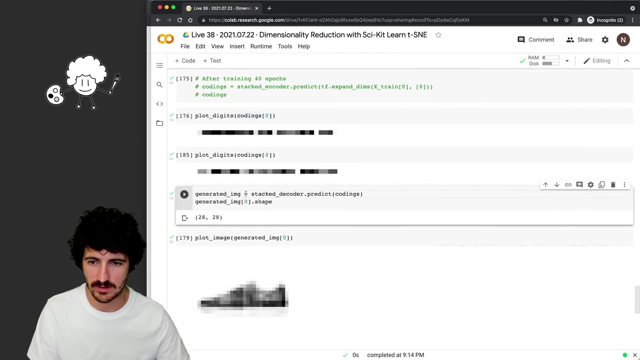 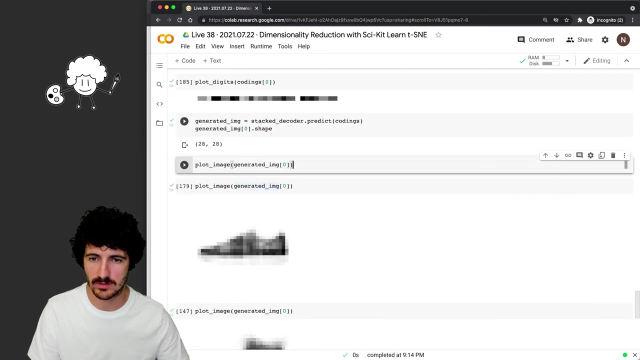 we can see those here, right, so the coatings do change a bit. and now when we plot them, right, so these were the ones from before. so when we plot them, they're really different, and let's see what the generated image looks like now. so we put a block in here, okay. 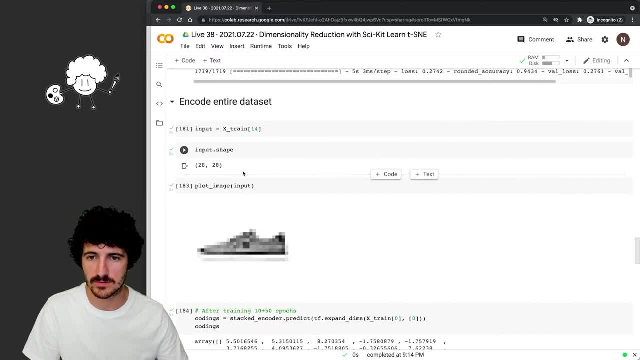 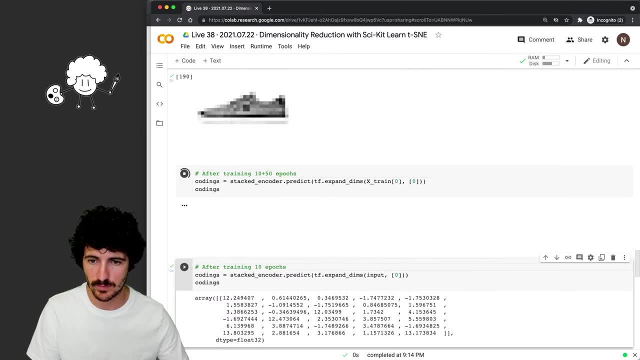 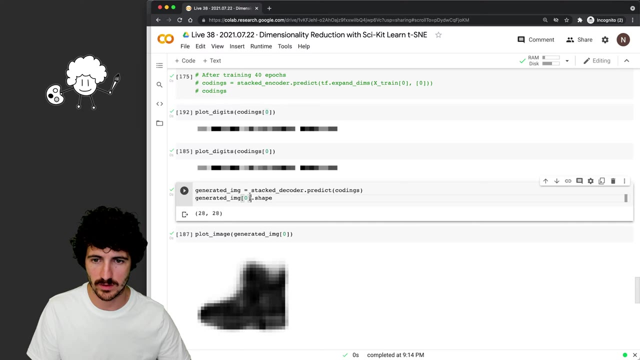 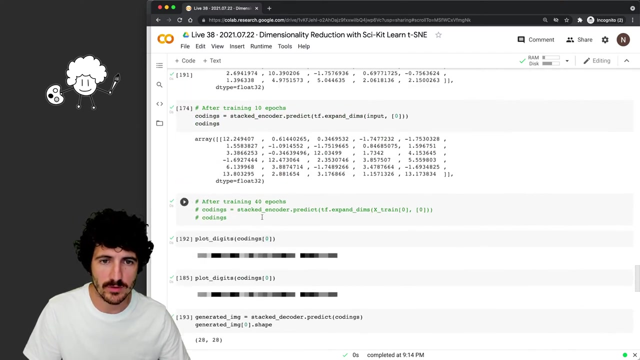 so this is because it's for the other image. so okay, so this is because it's for the other image. so we put this here. we need to define this here. 14. we put this here. we plot our coatings, we this- huh, what am I doing wrong now? input? 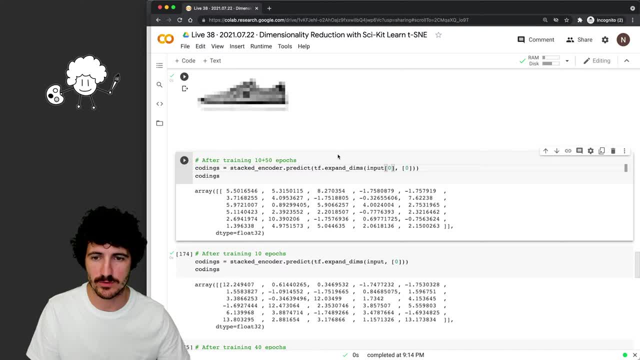 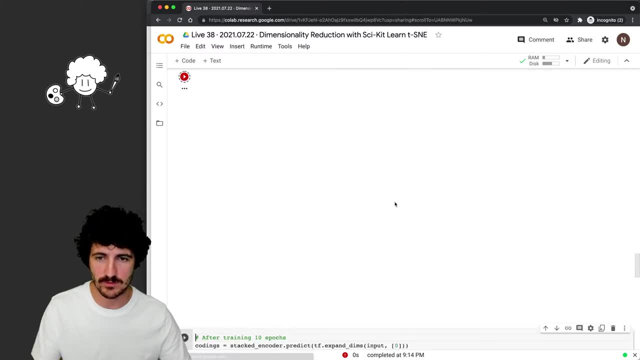 oh okay, so same error as before. so we left this on the old code, so that's why we have to define this instead. I, okay, that's why we we were erroring here, Right, So we put the input. um, so we get the coatings. 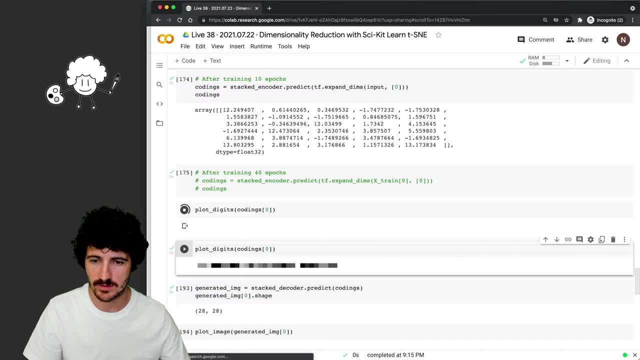 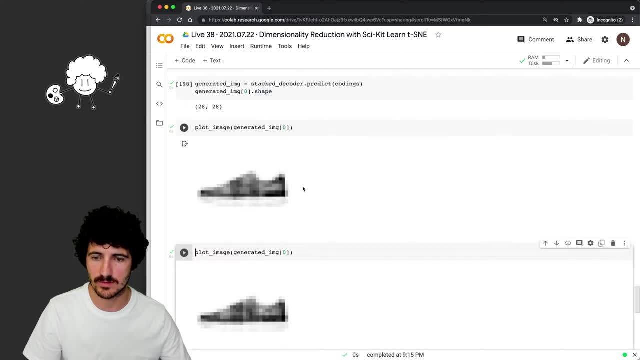 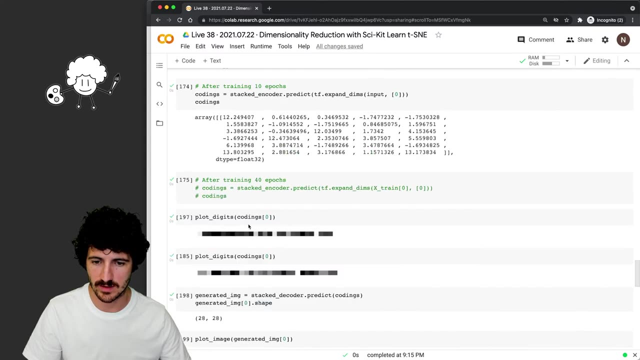 Did this look a bit more like the ones below this, look back again differently, And now we predict and now we plot. Okay, So we're getting you know. you see here, Stripe and I would, yeah, I would say it's hard to notice which one looks more similar, but you know this. 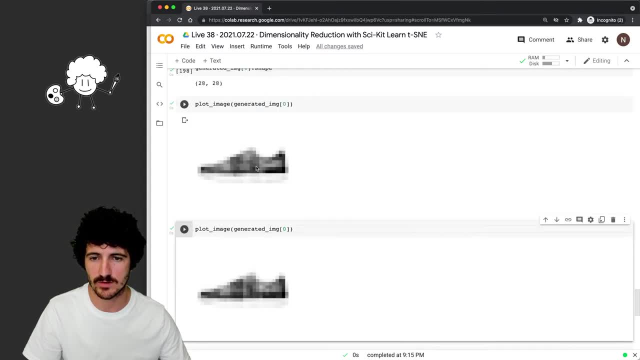 is a bit more refined because we've trained for longer, so I would say maybe this one. so this is like a 10, this is a 10 plus 50.. Let me show you here, And this is the input, is the original. 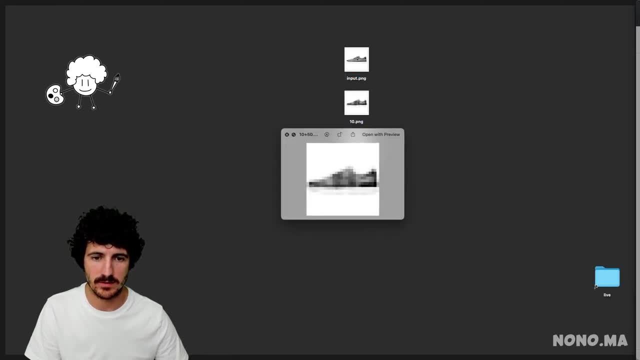 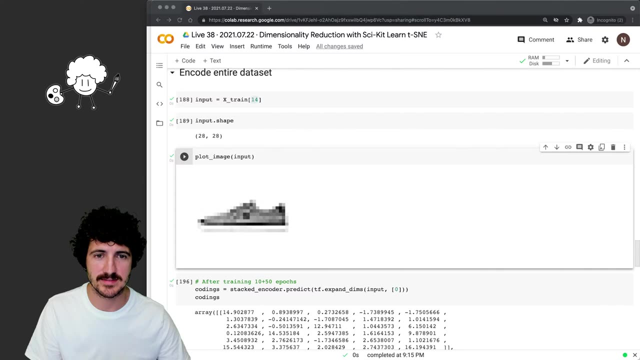 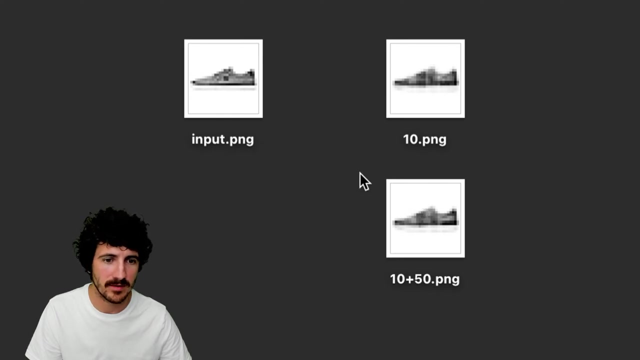 So this is the actual input. So Which one looks more Similar? I'm not sure, Right. So I guess, um, they're more or less the same. They don't really look that much similar, but yeah, I don't know that that's kind. 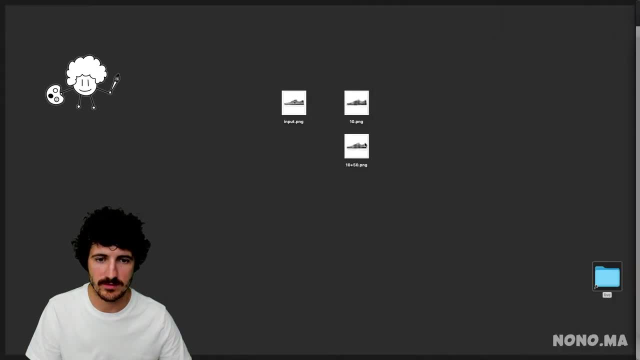 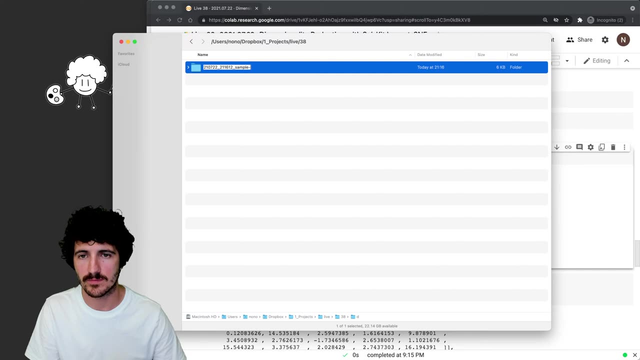 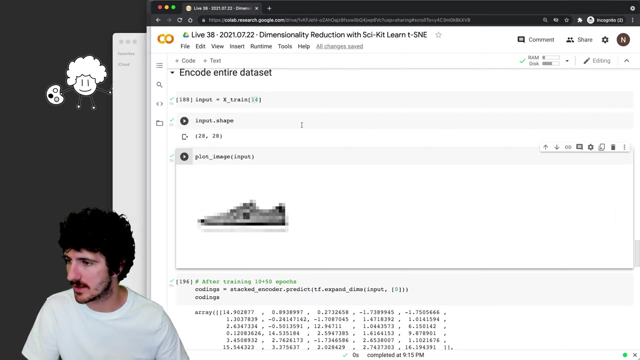 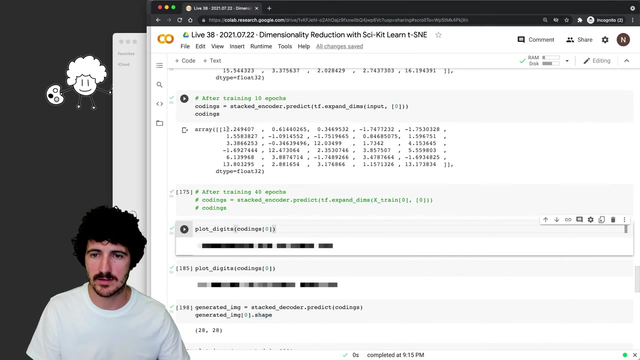 of one of the outcomes of today, Right, So let's just put here, All right, So, what I was mentioning before. Sure, So we, we try. what I said is that these coatings right, If, if we look at the coatings what they really are, they're not more than 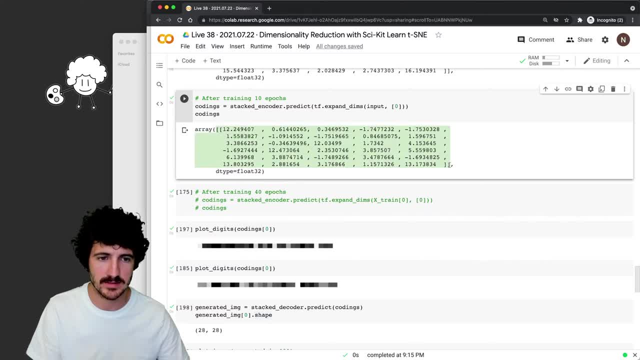 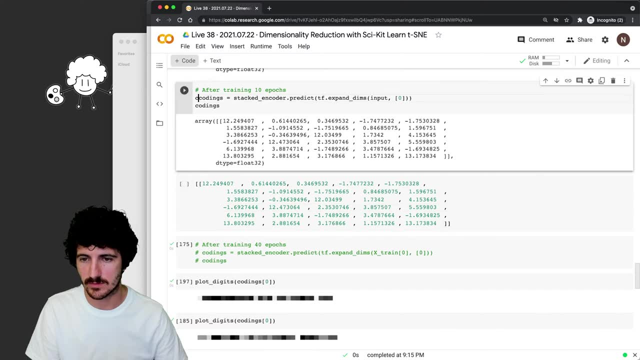 an array contained inside of an array. So we could get this here and we could say: okay, I want my coatings to be, for example, um ouch. So my coatings could be an MP array with these data. And now we bring the coatings. 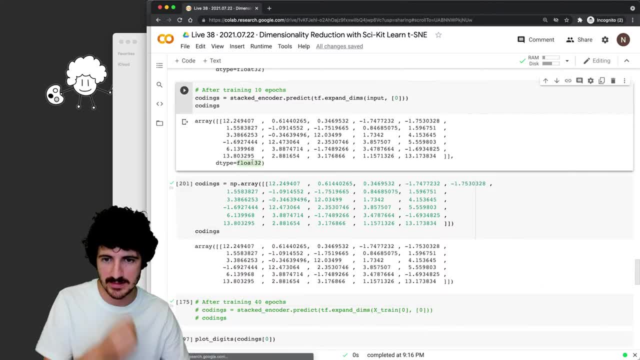 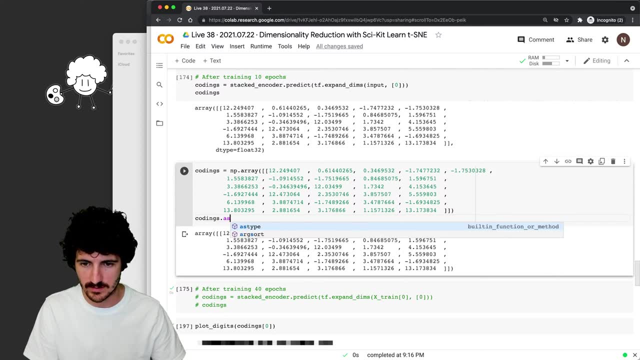 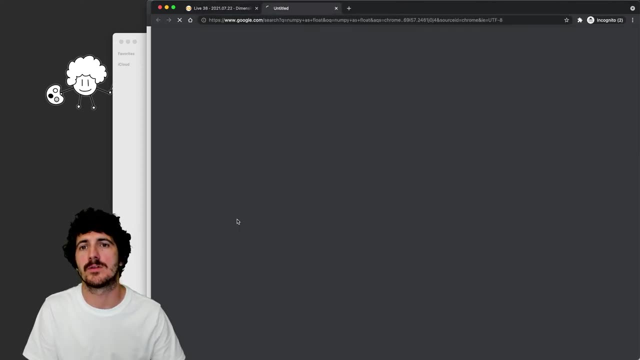 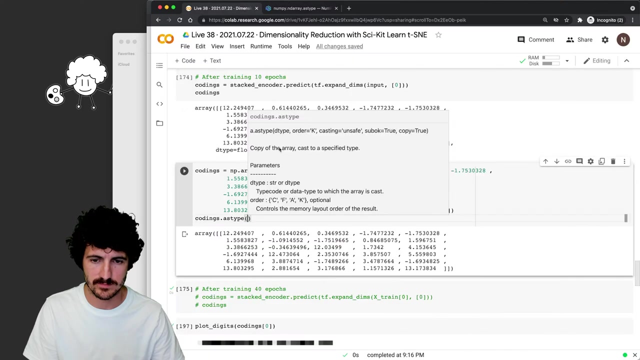 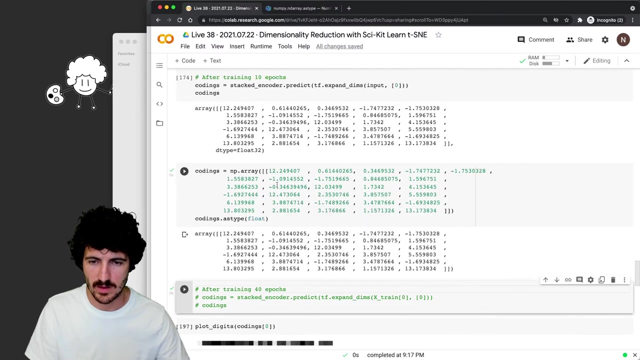 And now we get exactly the same. but this is float 32 type and we could probably do that as Type NumPy, as float See, as type. Um, Well, never do that, Let's just try out. So I get the coatings this way. 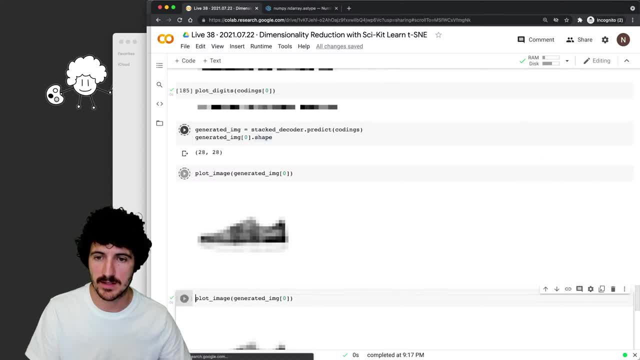 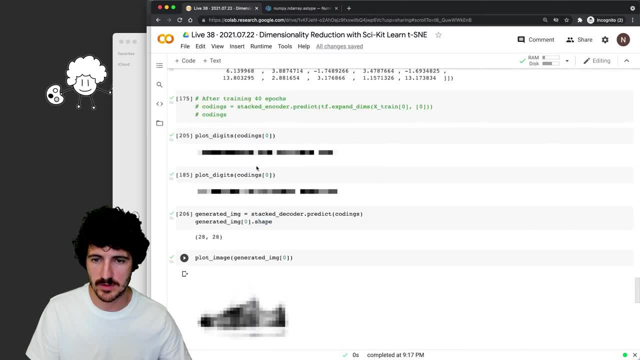 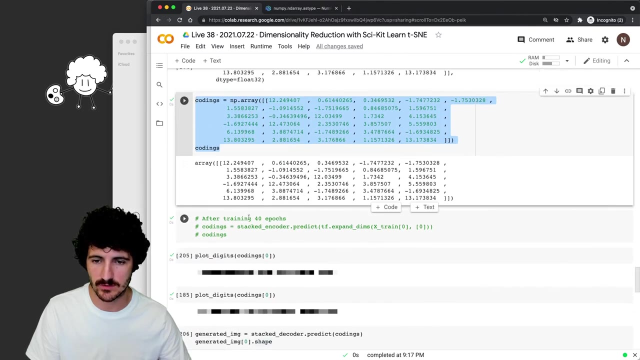 I plot them. They're the same because I just copied and then we predict we get the image right. So let's put that image below. So those are the same image and, uh, I'm going to bring these. well, we'll, we'll leave them here. 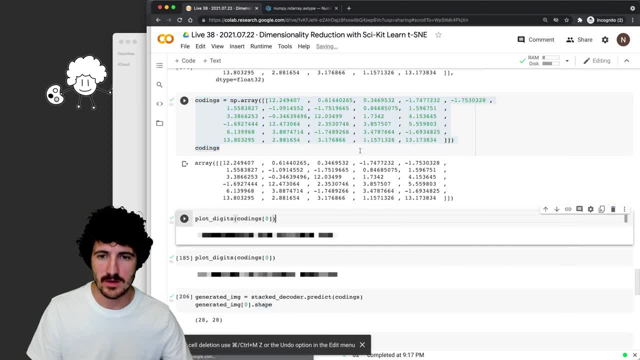 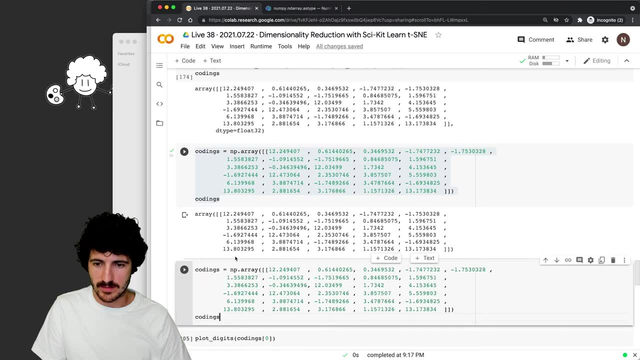 So we get, we can probably remove this part. So now what I'm going to do is I have these coatings here and I'm going to copy them, So I'm going to change them slightly. So let's say, here we put: well, not slightly, let's change them a lot. 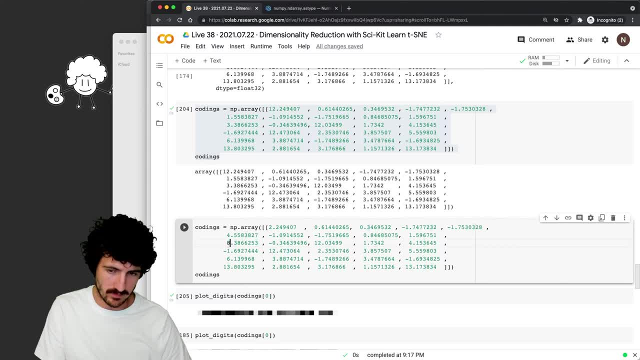 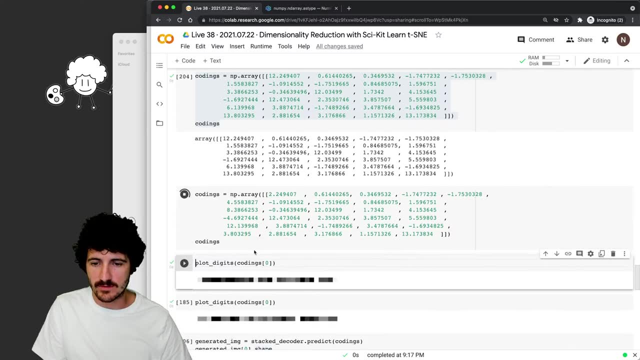 So maybe we put here: a four is going to be an eight is going to be minus four, It's going to be 13 is going to be one, right. So we change those coatings and now, instead of the one we have above, we have the one below. 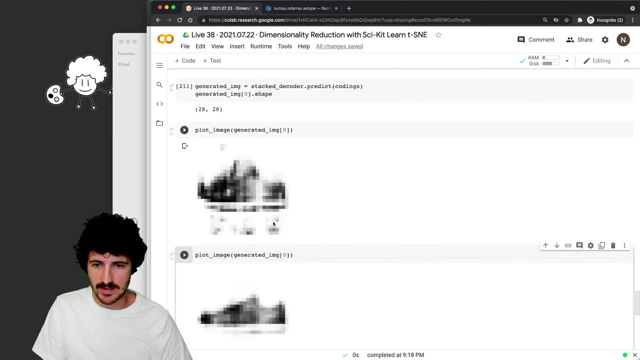 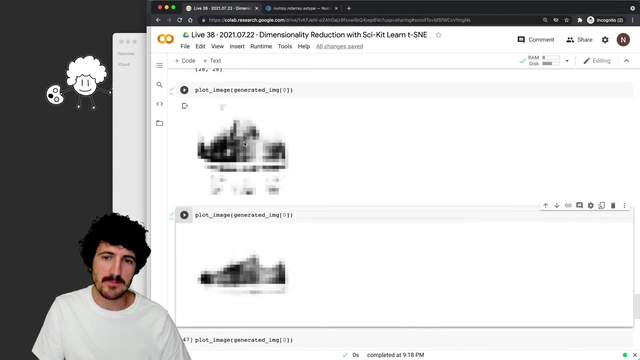 And, uh, when I generate the image, That is what happens. right, We've changed the things and there are some parts of the image that I still look the same, but by changing numbers we're changing different features on this image. 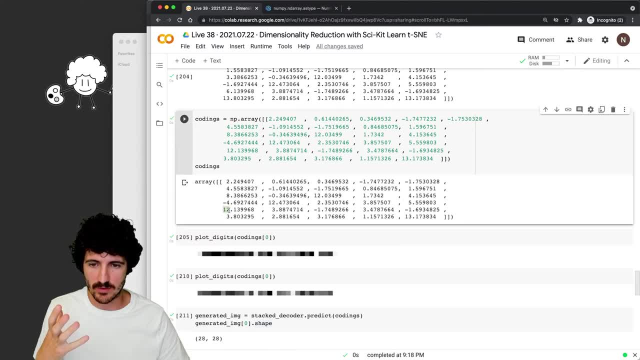 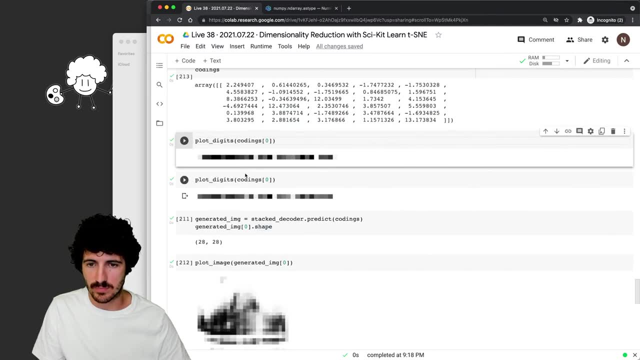 And uh, you know, one can imagine that now, if I do put this one uh here to zero, and uh, I, I plot again. Now we have just changed slightly Something here, right? So instead of white we get this gray. 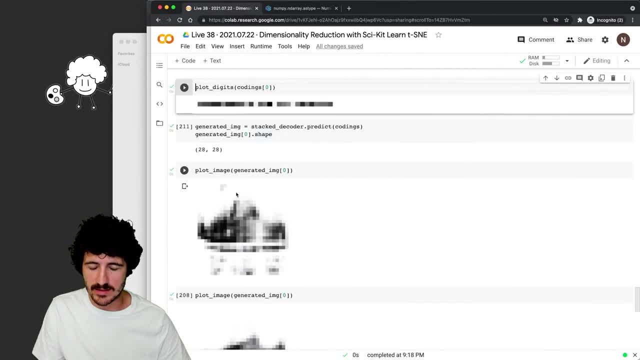 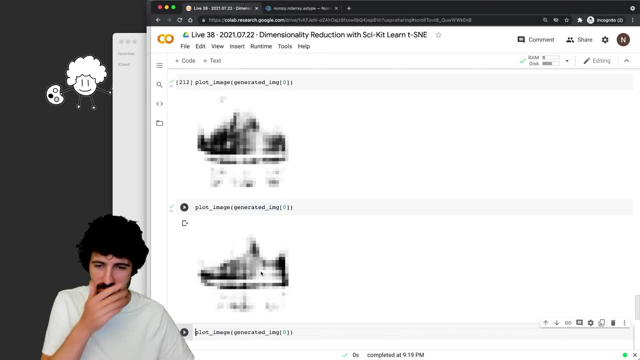 Well, instead of this gray we get this white. and uh, now I can predict again and generate the image And now that changes back again and looks again more like a shoe. just changing one number like changes the output a lot. 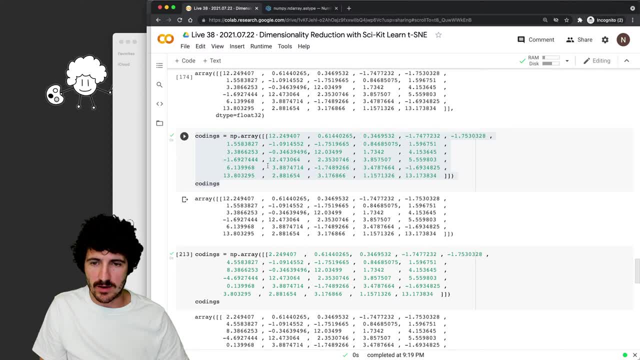 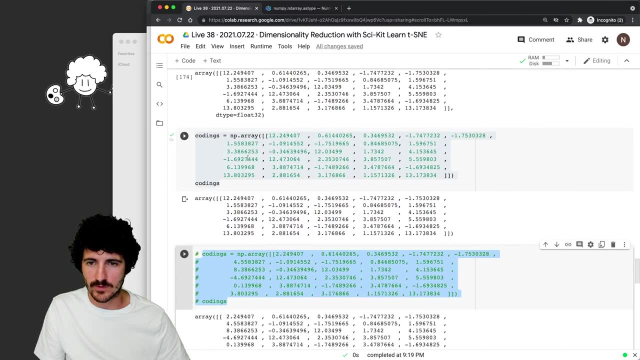 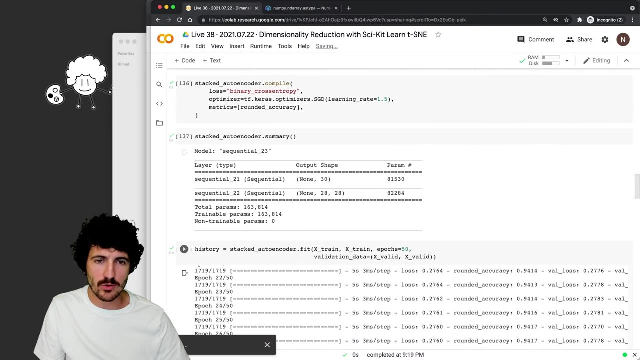 And okay. So what we're going to do now, we're going to leave these ones commented, just to to make sure that We don't get confused later, and we just use the, the actual prediction function, and we're going to go back. 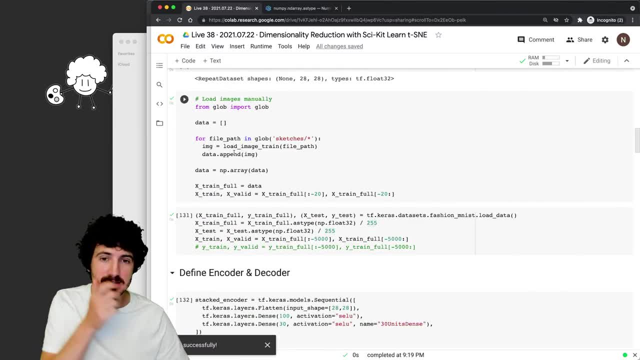 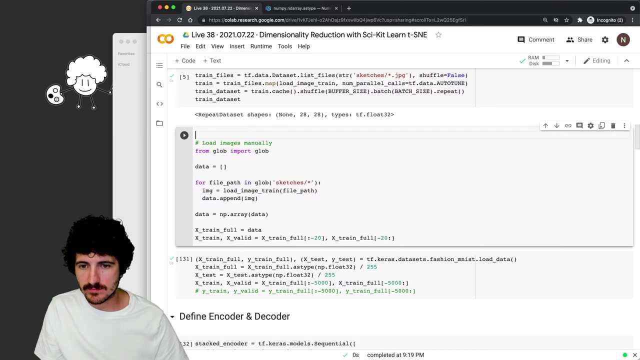 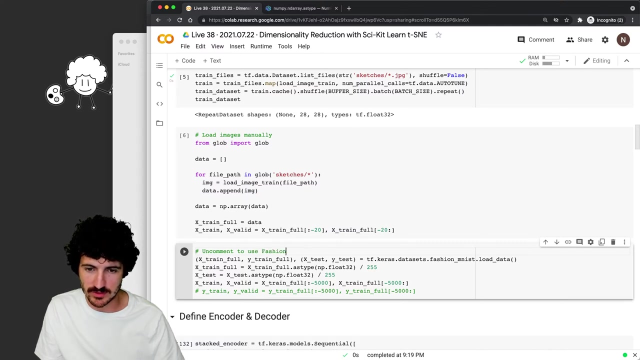 Um, I'm hesitant to duplicate this, So maybe maybe let's leave this um part one, fashion MNIST- and duplicate this one. Um, maybe not. Let's, let's just see Uh, um and comment to use fashion MNIST data set instead. 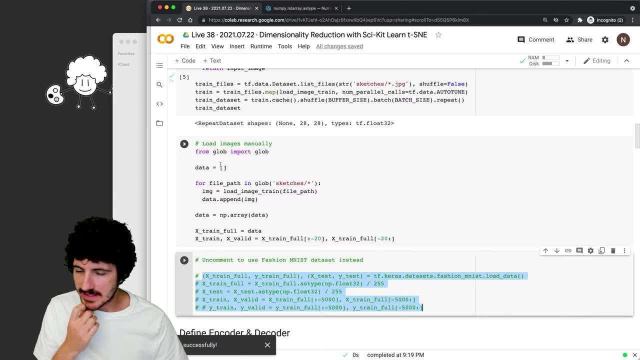 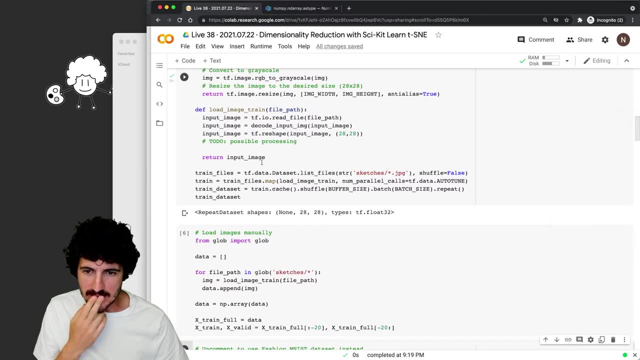 Right, So we come in this out and, uh, now what we do is okay, I'm going to take out a few things that are open. So we comment that out And we just want to go back to where we are. 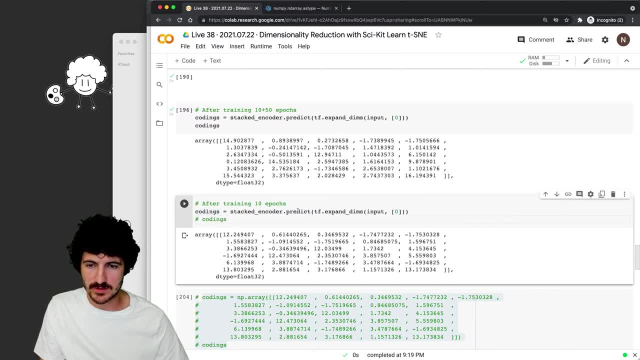 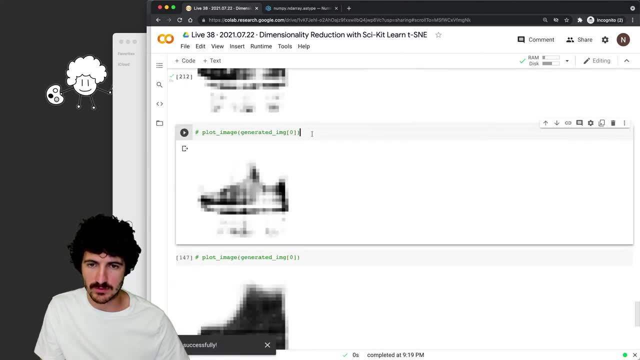 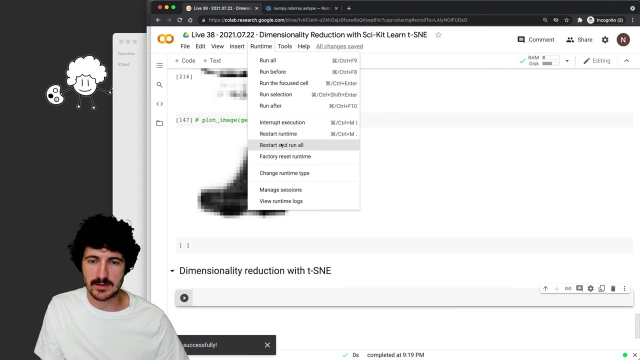 I think everything right. So we don't really need to expand twice here and we don't really need two coatings and we don't really need three visualizations. So we're going to do is that we're going to go back here, We're going to run restart and run all. 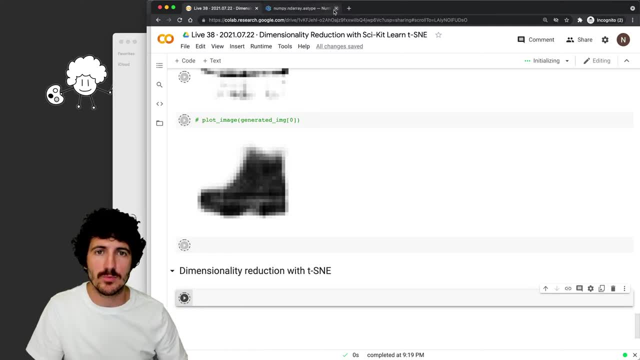 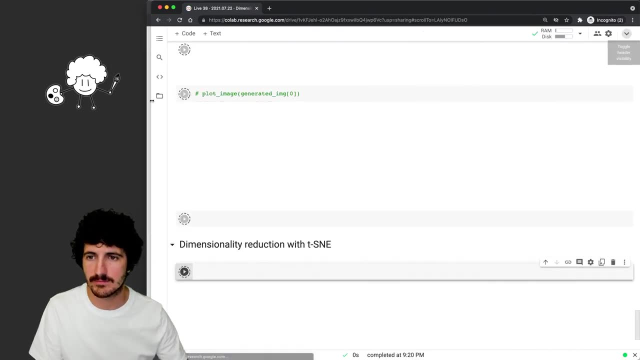 So this is going to restart the runtime of our uh Jupiter notebook and call that, And it's going to execute all of our cells once again And, yeah, hopefully we can see something with our data set right, With our real data set. 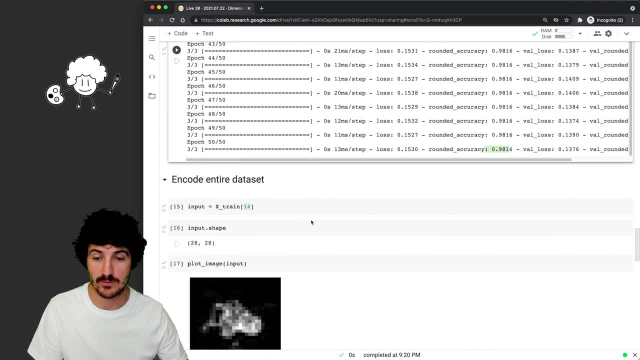 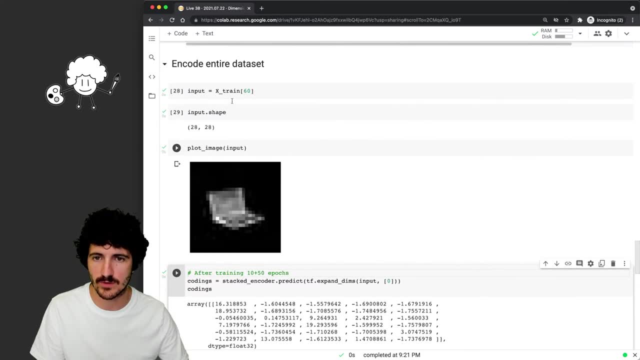 Okay, So these are strained. We're at the same um accuracy that we were able to get before, but now we have an image that if I said here 60, right, We can see a different um input. So maybe we can just um merge these ones. 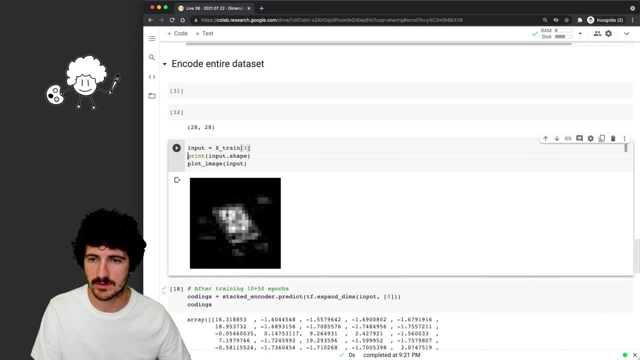 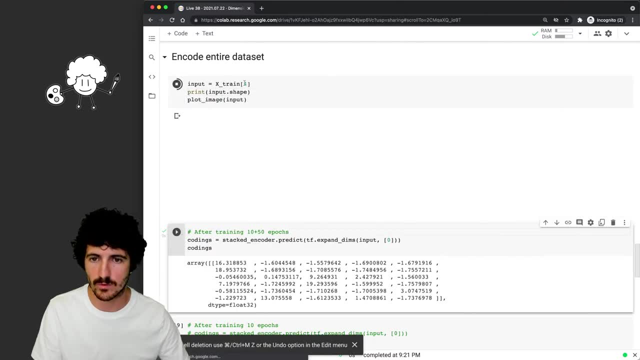 Because it doesn't. you know, we don't really care that these are just one cell, So we're going to remove these other two, Right? So let's see four, five, six, Okay, So this is kind of different, right. 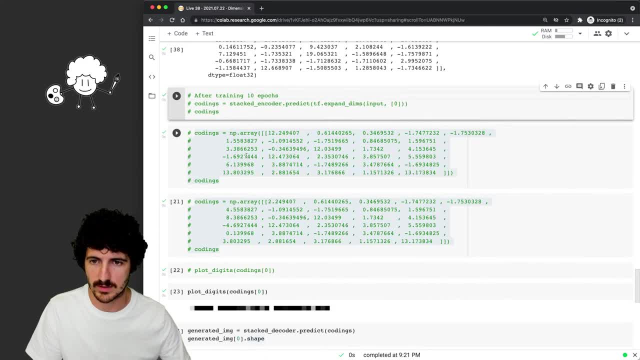 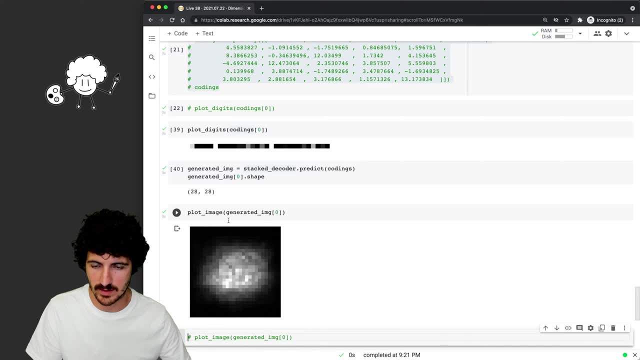 From everything else. So we're going to go and run that, We're going to run the coatings, which are different. We're going to do that, And then that, okay, Is there anything Wrong? Okay, Wrong here that we've done. 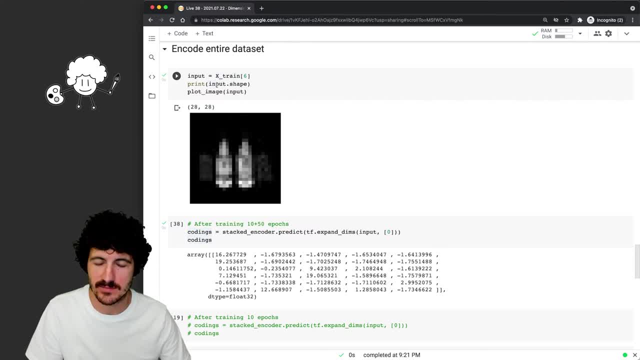 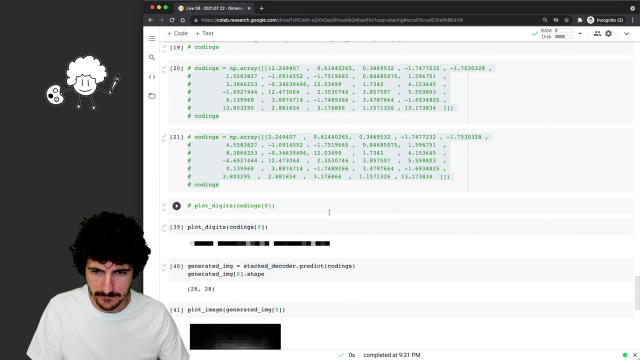 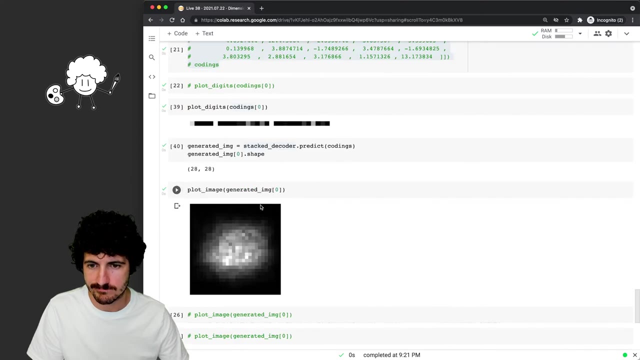 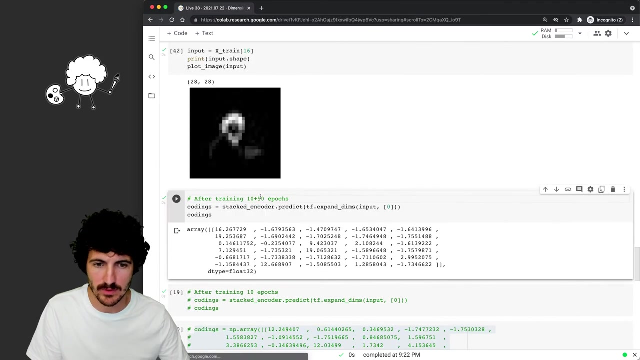 So input X, train six um input shape, expand them's input: Zero coding, zero coatings, coatings. No, this doesn't seem like it's changing a lot, right? So we go now with 16, we have the input. we're actually predicting on the input. 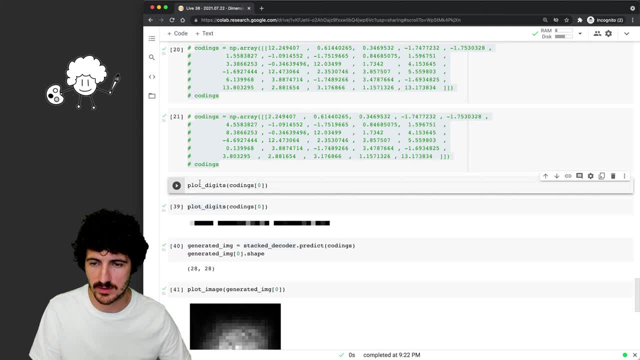 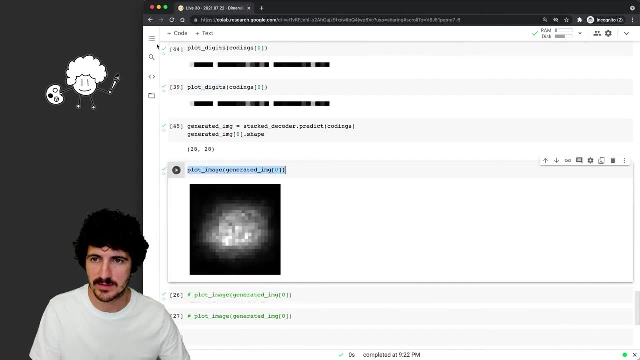 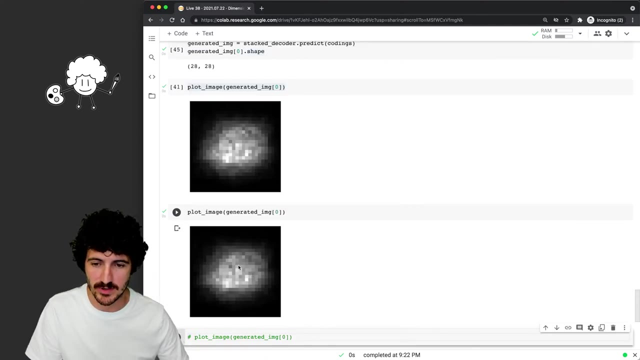 We plot the digits here, So we're going to plot the digits again and they barely barely change. So we do this and we do this. Yeah, So this is changing, but it's barely changing, It's just learning like a real weird mapping. 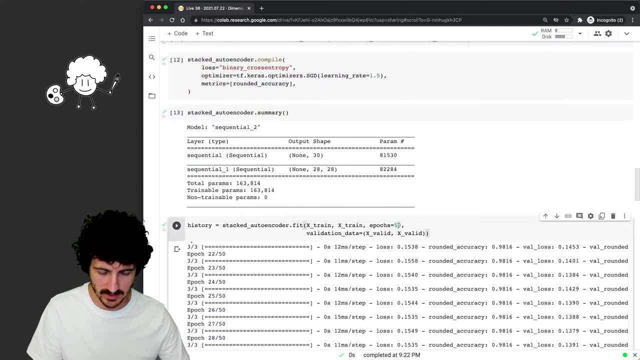 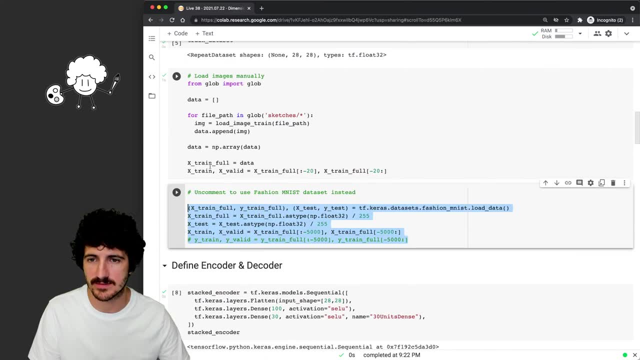 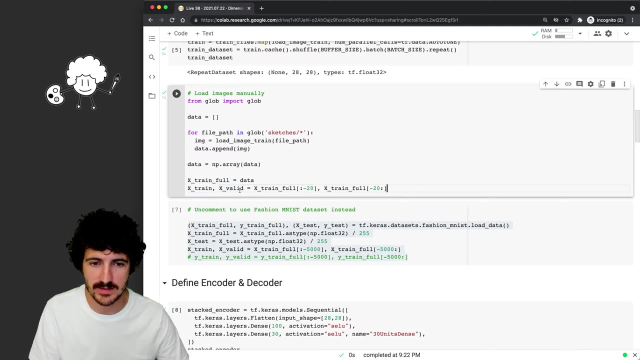 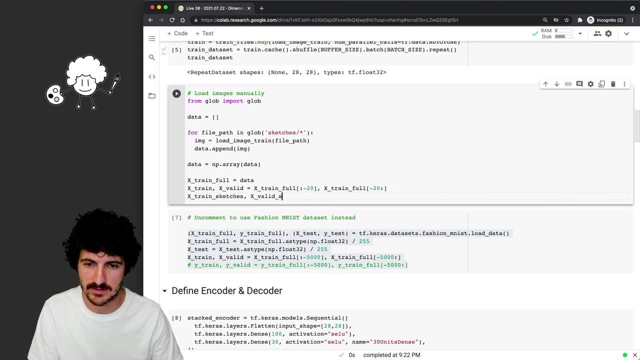 Um, maybe one thing that we can do here is so we can actually train for for 10 epochs once again with the Other data set and see, let's just make a cool experiment. So this would be X train. um, let's do here. save this as X train sketches. um X value sketches. 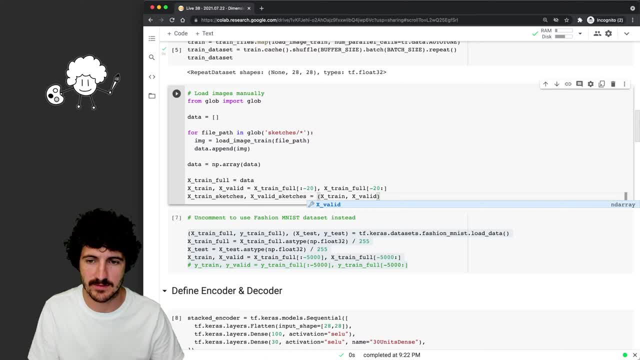 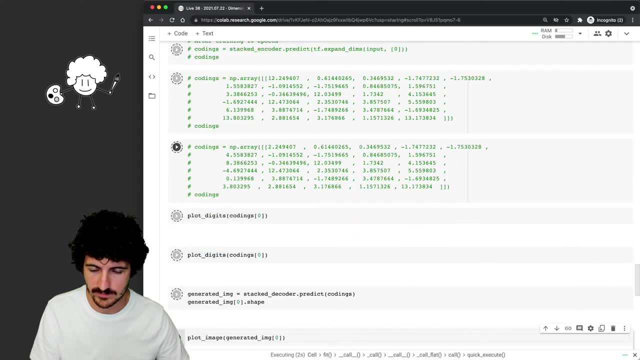 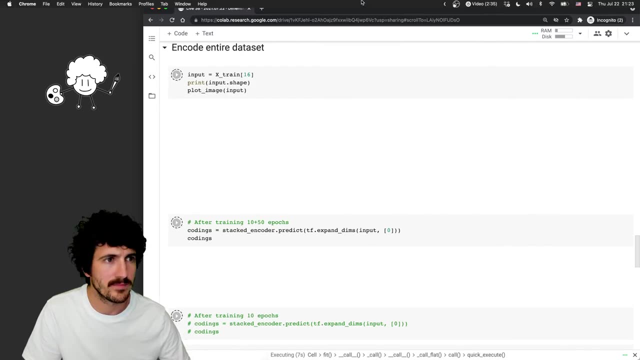 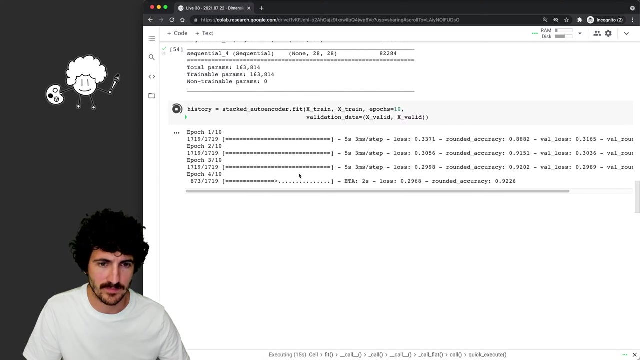 Equals, X, train, X, value, All right, So we're going to rerun everything. So we're going to retrain now, Um, and regenerate the images, All right, So we're training here, um, on the meanwhile. So let's actually look at what we need to do. 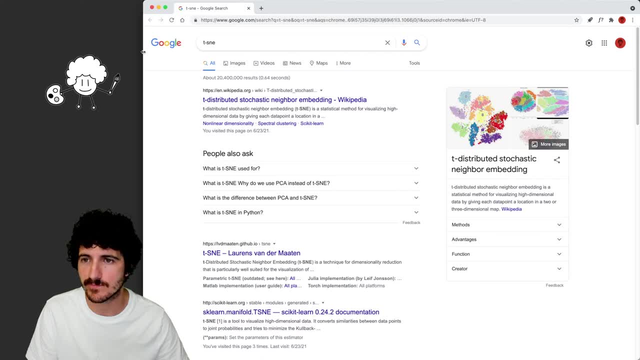 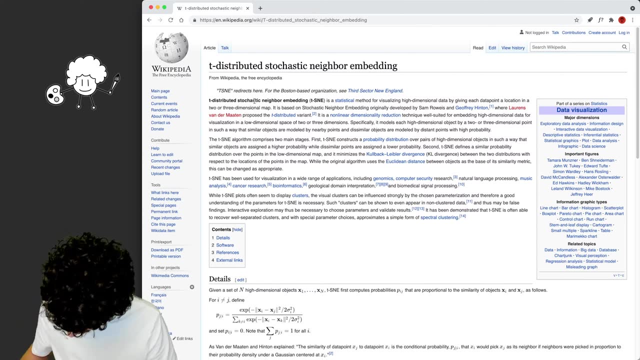 The, the Disney, um, the Disney algorithm. Right, I'm going to take a look here at the book. All right, So we're、 let's see, this is basically just taking a look. I'm going to take a look here at the book. 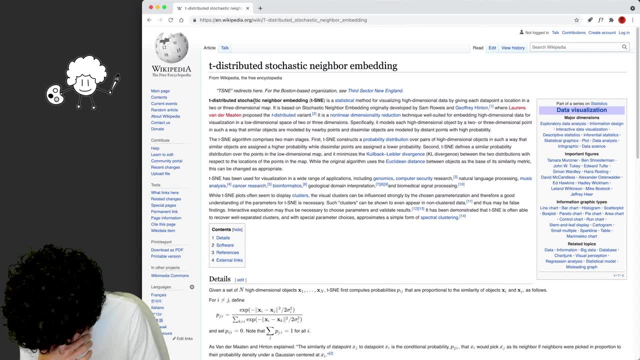 Um, and I'm going to do this, See we, uh, we're just going to take a look here. Uh, these things are going to repeat. This is the. this is the same thing as we just did, Right? 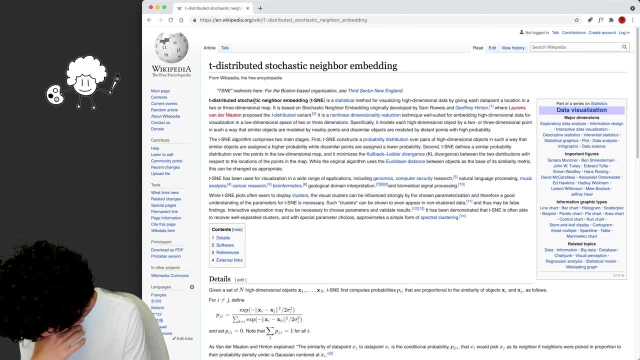 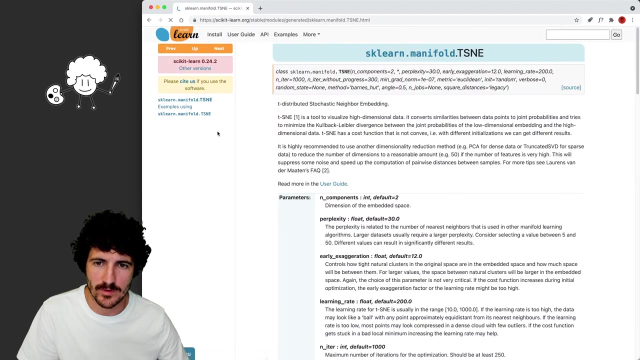 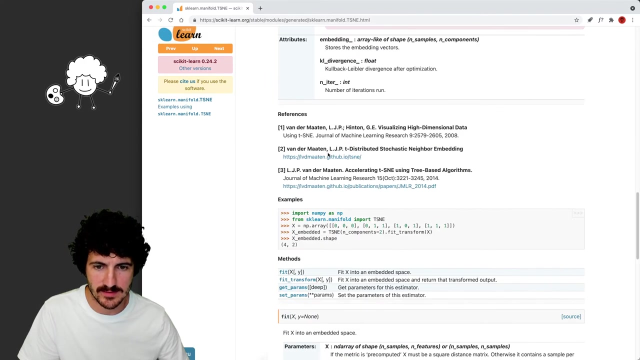 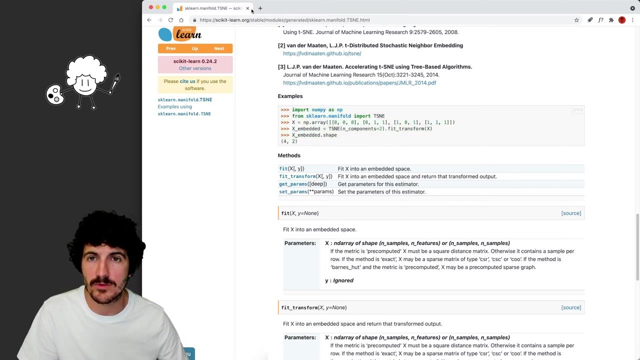 So we're just going to do this, All right. So it seems fairly simple. So we have a Disney um the psychic learning implementation, which is including a scalar manifold Disney, And uh, all we need to do is uh, something like this, more or less: uh. 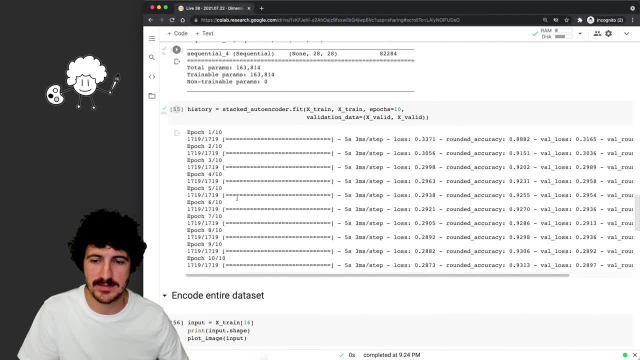 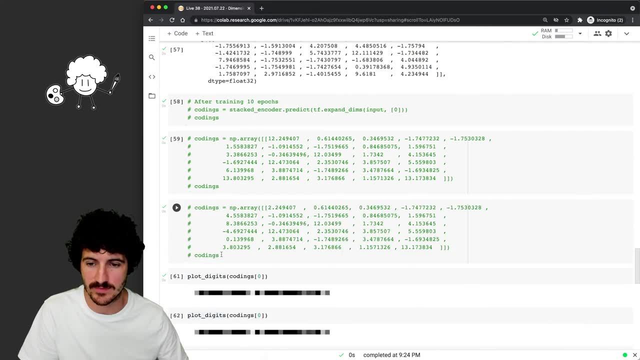 we're going to do that coding before we go today and, uh, let's see how this went. Okay, So we have these fans and we get pants, which is pretty good. I mean, we have a lot of Involved in in this experiment, right? 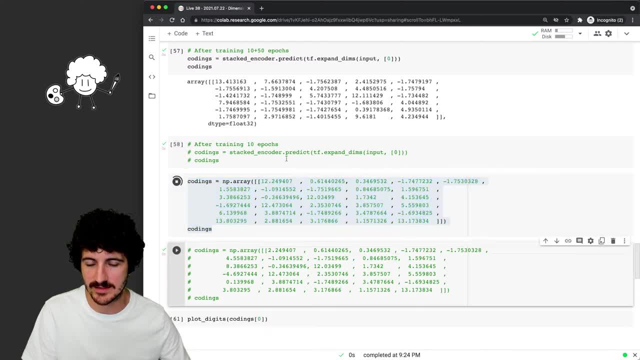 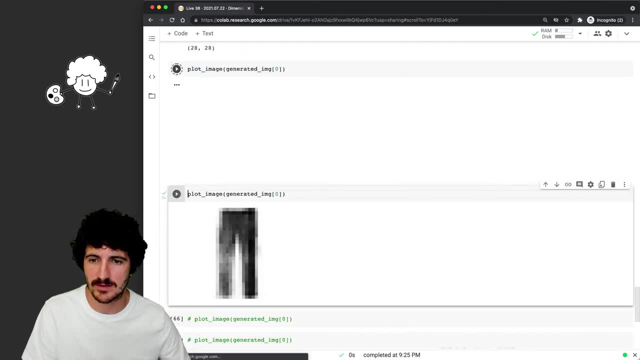 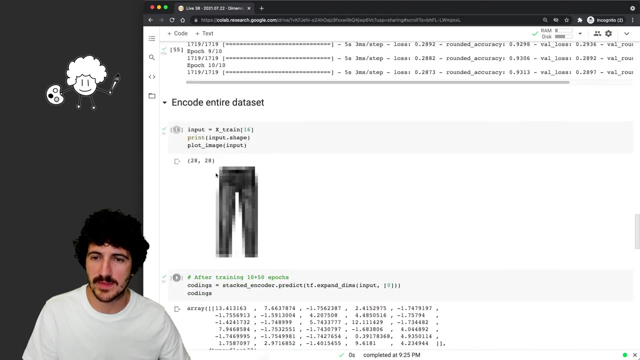 We could get, uh, these again like hand generated coatings which match- and this one's here pretty similar, And uh, we get this, which is a completely different output, right? Well, again, let's comment that out. 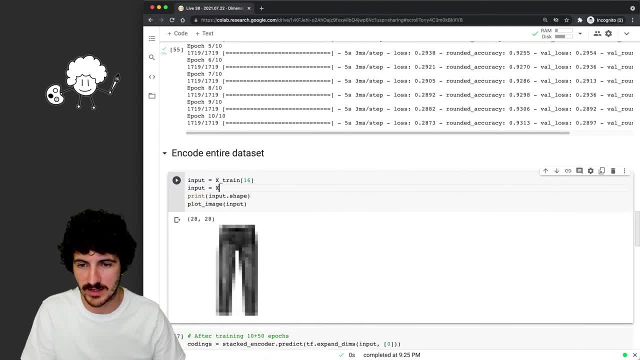 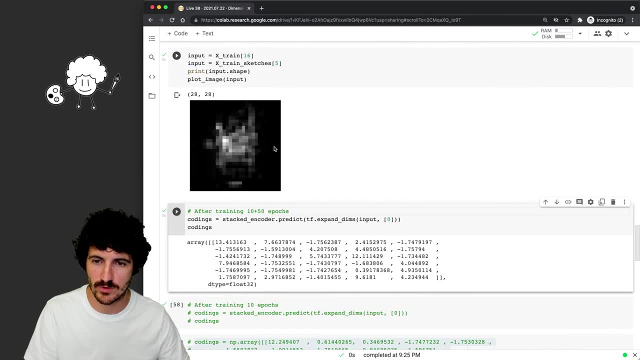 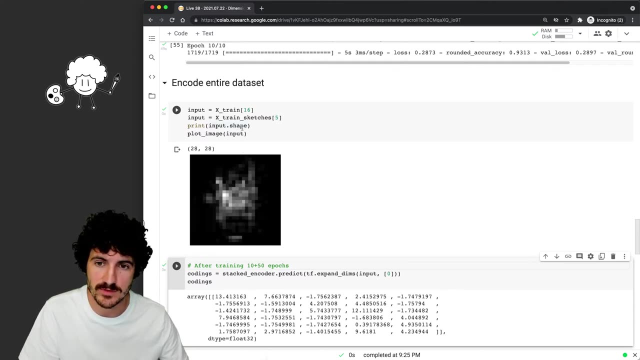 And uh, instead of getting an input X train, so we're going to get an input X train sketches and we're going to get the fifth Right. So now we're talking about this one And uh, one thing that I mentioned before is the, the inversion of those. 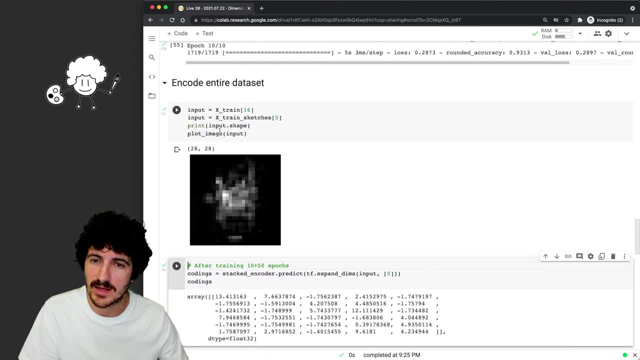 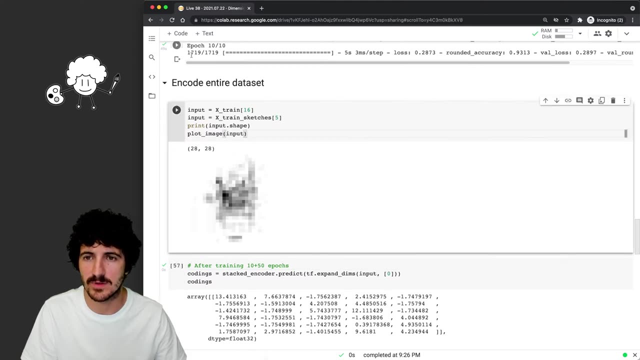 So maybe, um, I'm not sure if we can uh to, to, to, um, if we can do something like this, yeah, we can invert the image, right, Uh, okay, So let's actually put this separate. 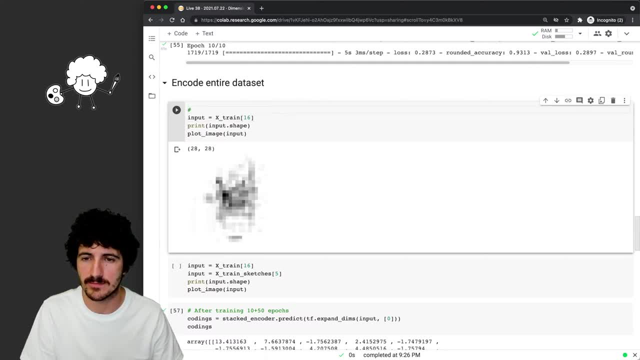 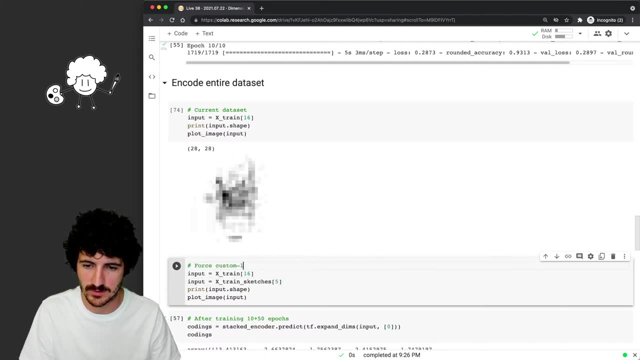 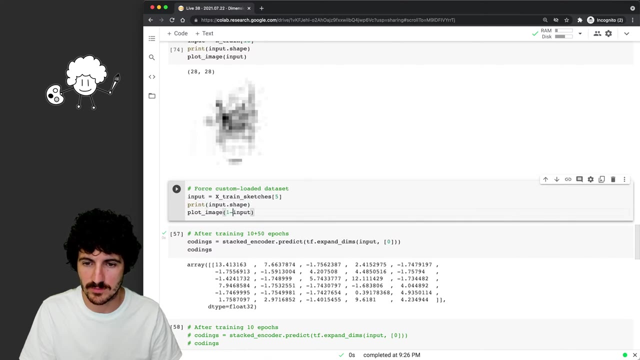 So we put All their logic here um: current data set or uh, force custom loaded data set, All right, So we are going to load that and we're going to plot. So the input minus one, uh. so these would load the original image and this one. 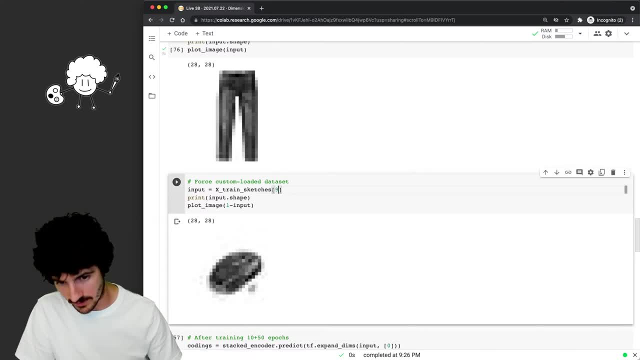 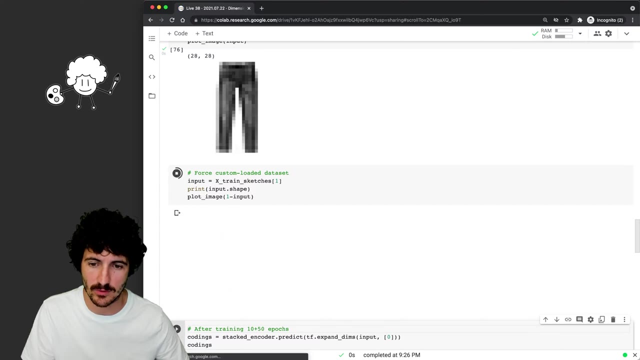 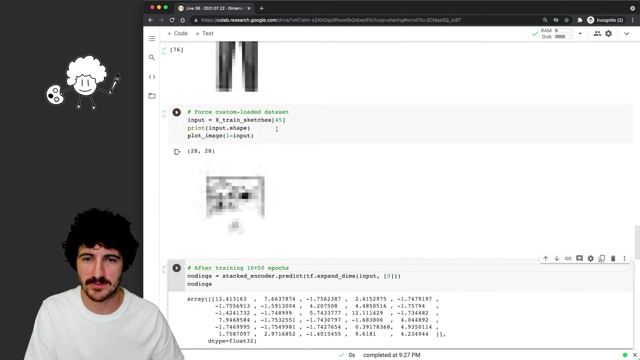 would load, uh, like a separate sketch, Right? So Yeah, The interesting part here is that we have images that correspond to my drawings and not to clothing. We want to see if we obtain the coatings of one of my sketches. What is the um, the corresponding image from from the decoder that we're going to obtain? 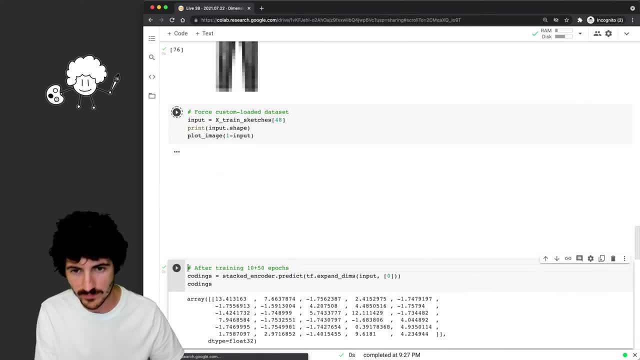 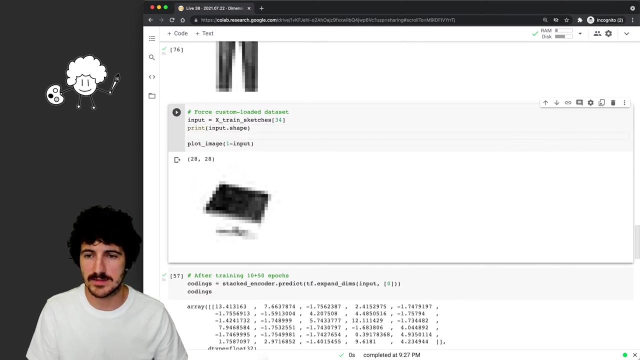 right, What type of clothing? Okay, So I'm trying to get here something that has a bit more contrast. all right, This one, for example. So I think what we need to do is say here: input equals one minus input, to get it negative. 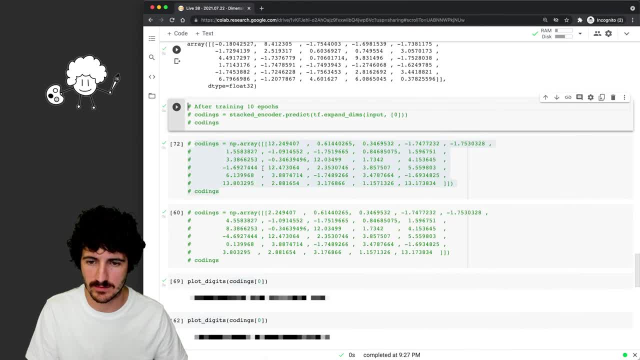 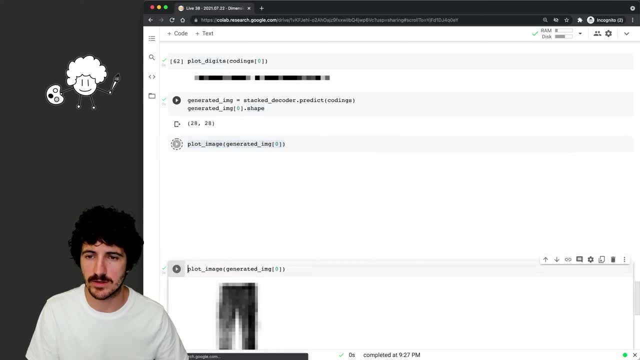 So we don't have to do this here And now. we can Do this. We can extract the coatings once again and we generate the image and then we plot it All right, So you can see right Like it's activating that part here. 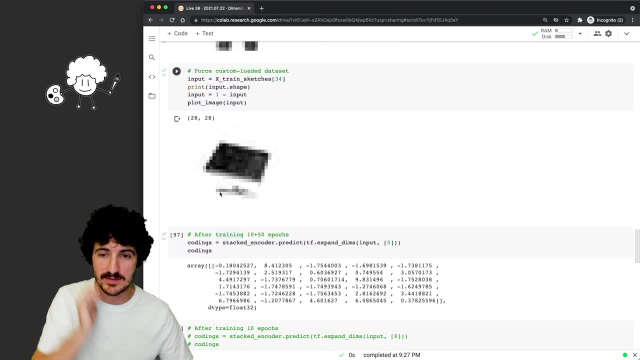 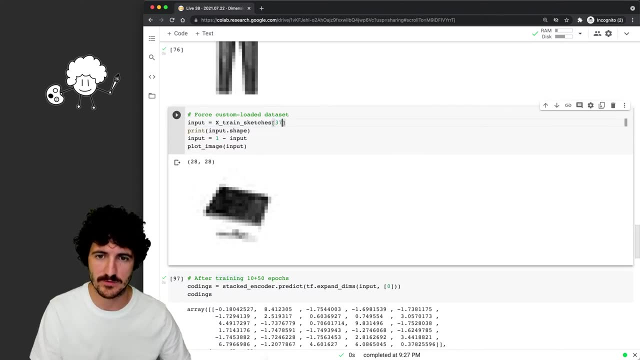 So he's trying to make it into a shirt and, um, yeah, I don't know, not the best, but it's a good experiment. It's kind of activating or like encoding, uh, with one data set and then obtaining with. 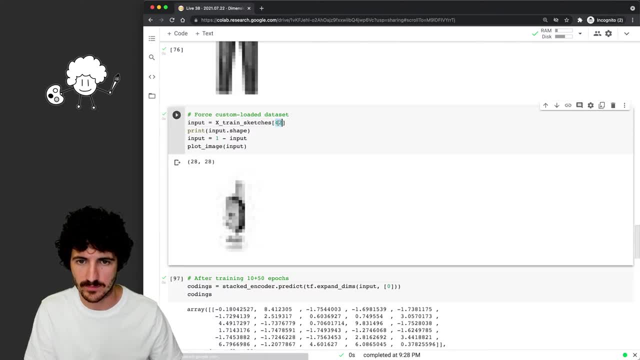 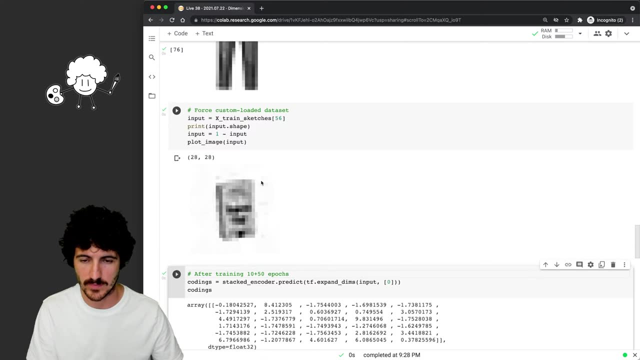 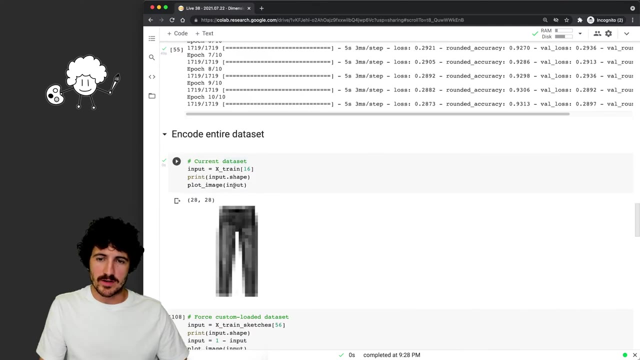 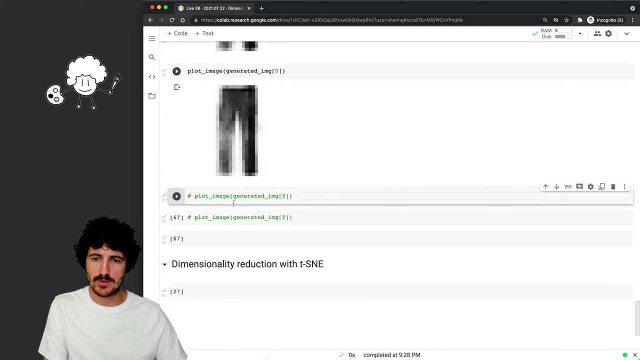 Another one. Okay, Let's see. Yeah, I don't know, It's a bit a bit of a weird experiment, but good thing is you know, if we just comment this out, we still have the proper data that we need it. 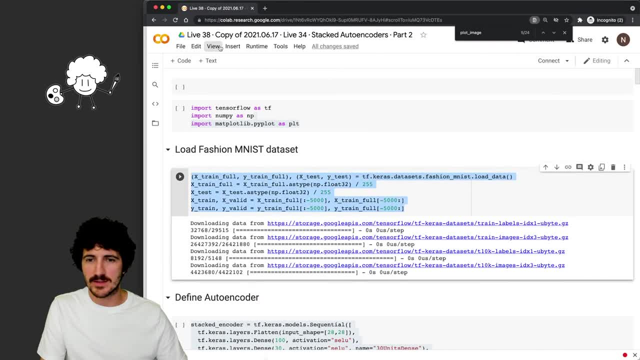 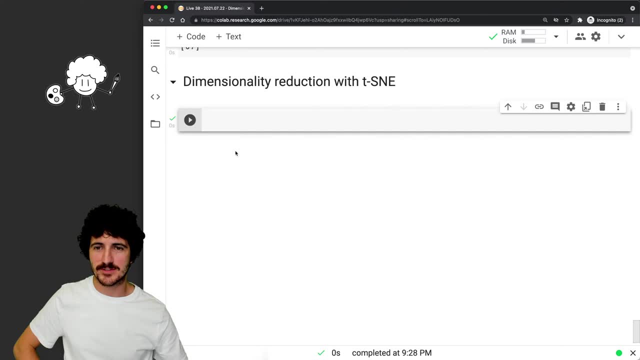 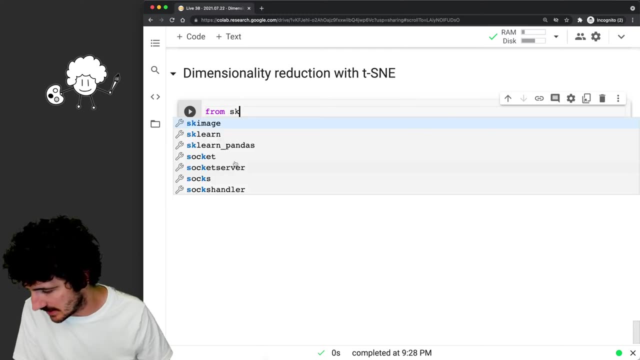 So we have the shoes And all that we need to do in order it to uh account with um or to use the Disney algorithm which we've been waiting for so long. Uh, we just need to say: okay, from SK, learn manifold, right. 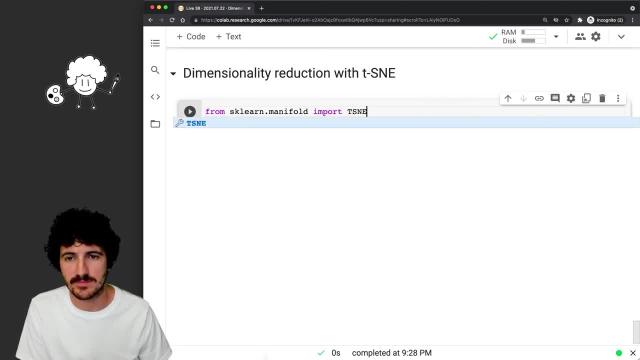 What we saw before: import Disney, Right, So we import that library. and now we say, okay, our X valid, or like X, let's say X valid, or X train compressed, because we don't. well, let's actually do X valid, because otherwise we're going to have too many, we say stacked. 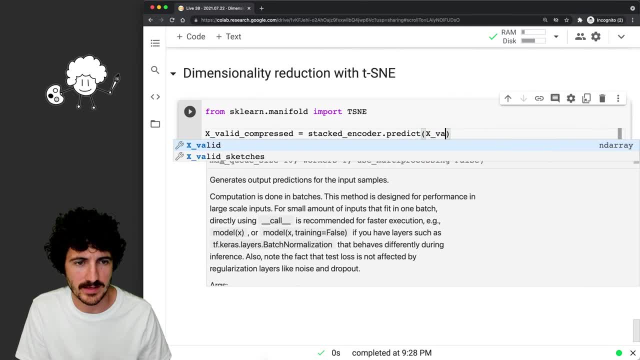 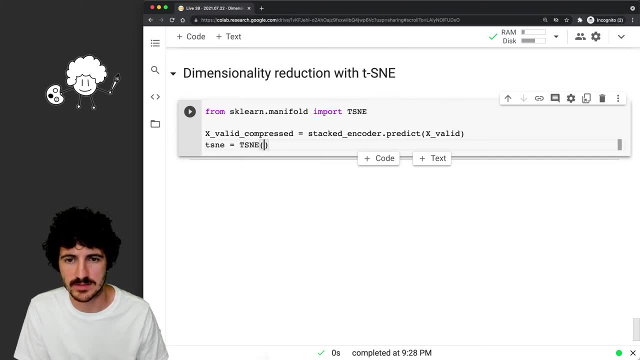 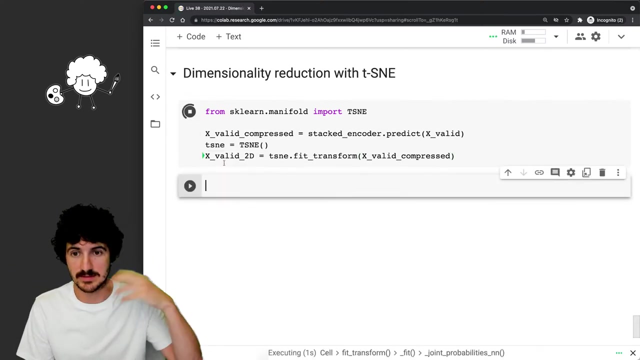 encoder, predict X valid, and uh, we do Disney equals Disney. So we instantiate this library and then we do X value to be equals Disney Fit, transform X valid, compressed, All right. So I'm going to run this and this is. you know, this is processing. 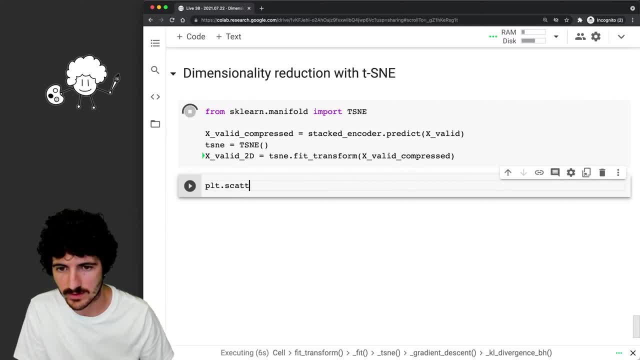 And the next thing that we're going to do is that we'll plot, make a scatter plot with the X valid to the everything and the zero X valid to the Everything. on the one, C, Y valid. Um, do we have Y valid? 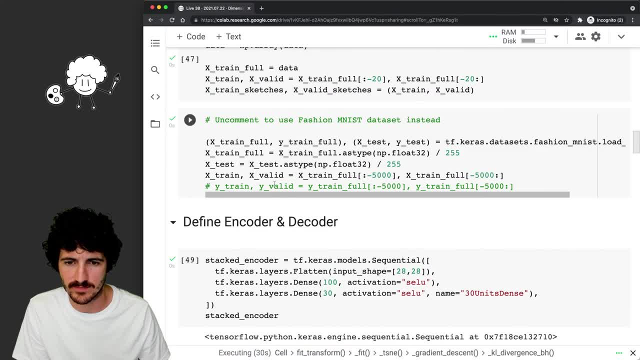 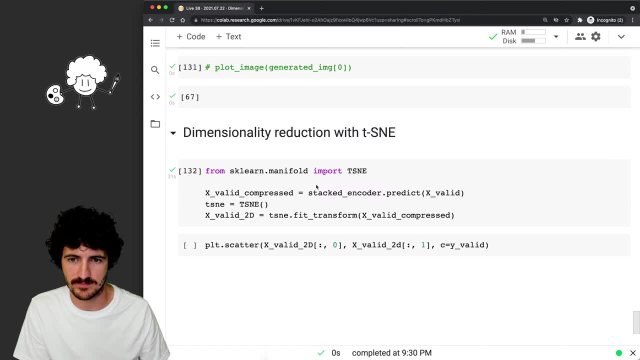 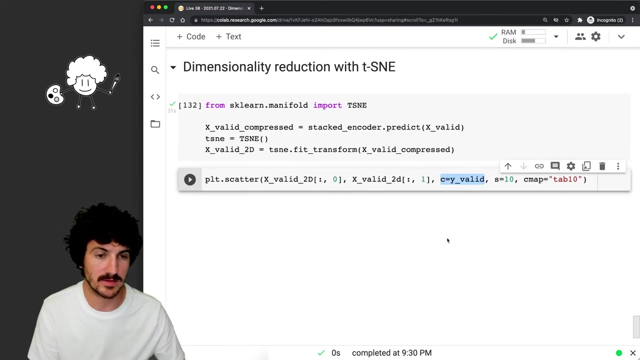 I don't know if I removed that for okay, So we need that now for some reason And, uh, we just need here as 10 C map, top 10.. Yeah, And these are the categories. uh, because we know the categories and we 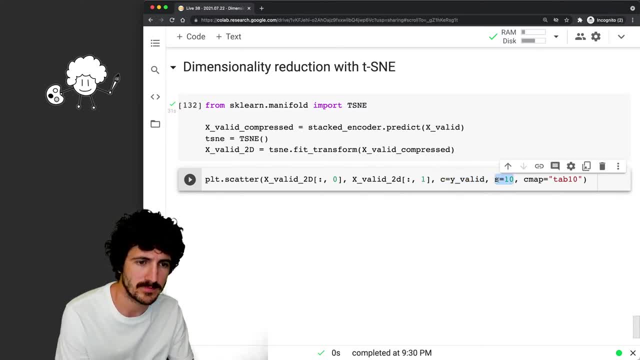 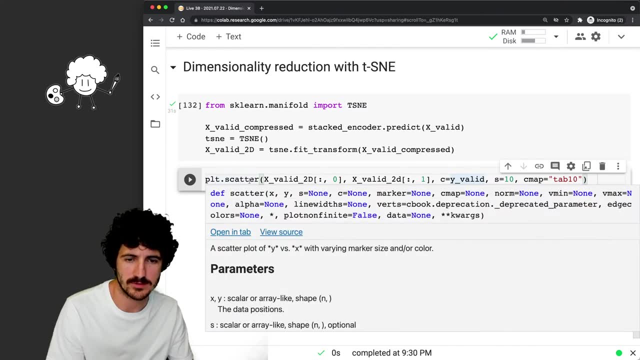 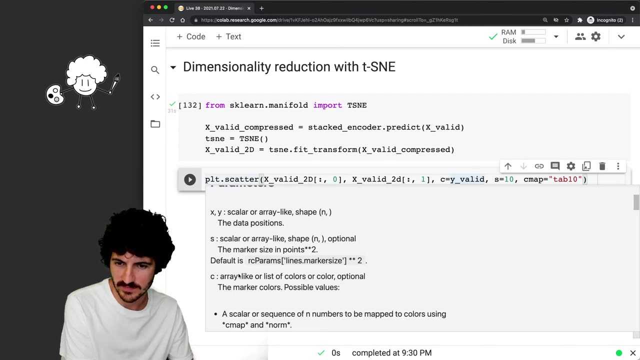 know that there are 10, um different classes, so I'm not sure. Yeah, So Scala, shape array of list of colors or color optional: uh, Scala. uh, Scala array like shape option. the marker size in point. 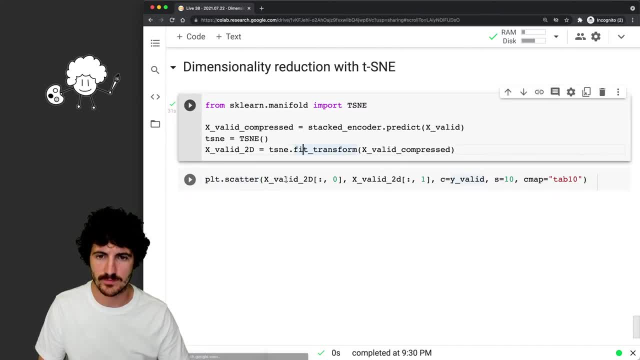 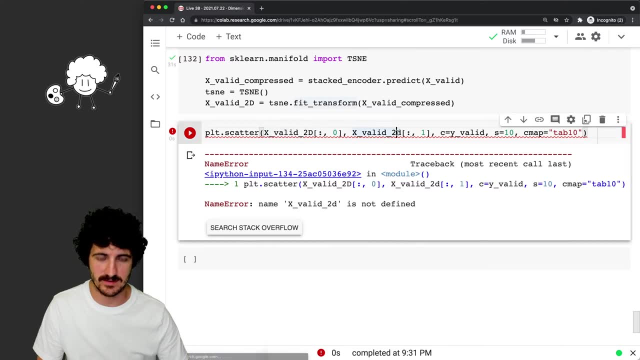 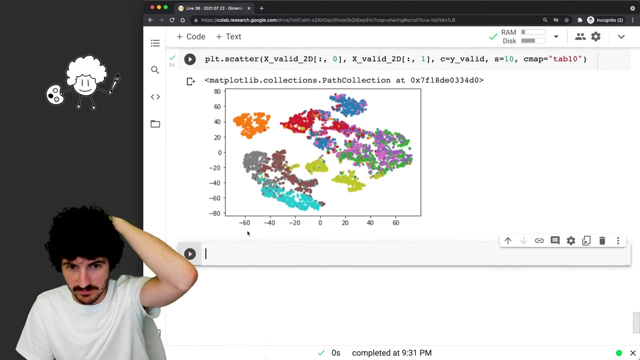 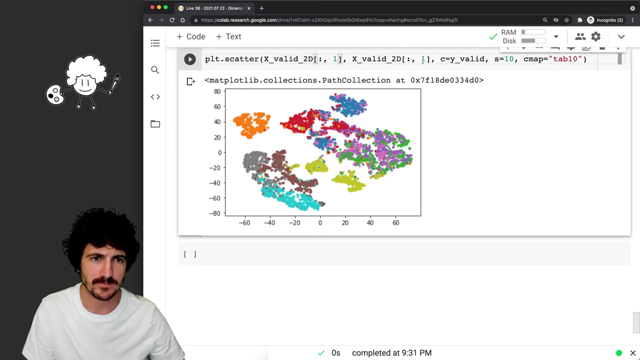 It's all right Cool, Let's try this. X valid is not defined. All right Cool, All right. So these actually matches in some ways, kind of changing the axis- what I have on the um, on the book. 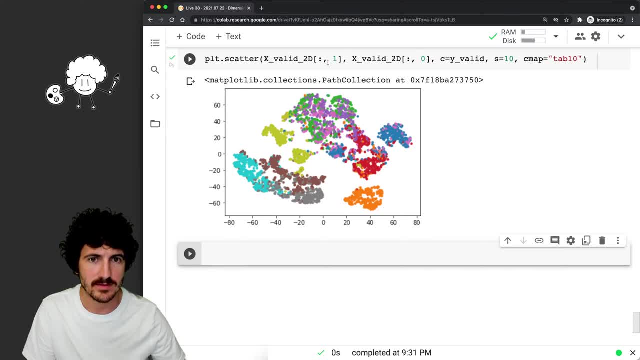 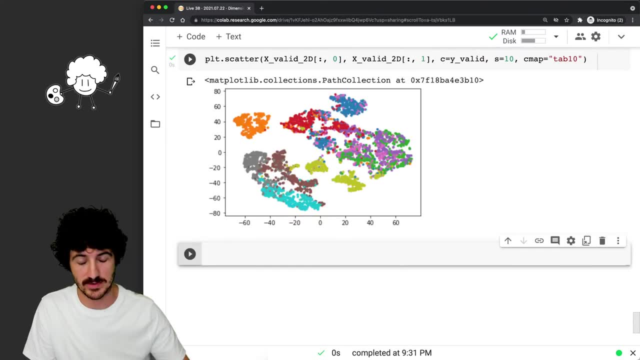 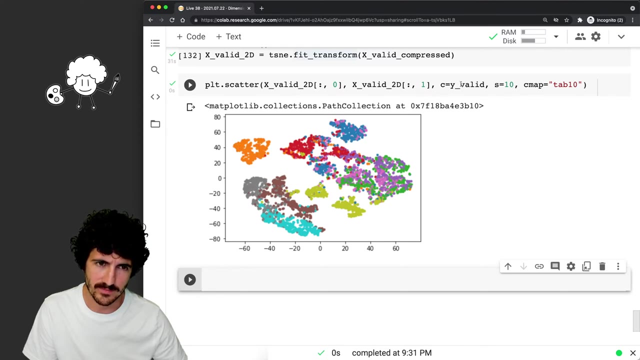 So I think maybe if I changed- Um, yeah, it's changing something on the axis, I don't know why, but it matches what I have on the book. Um, yeah, So if we didn't, if we didn't really have the um the car, so the the valid right. 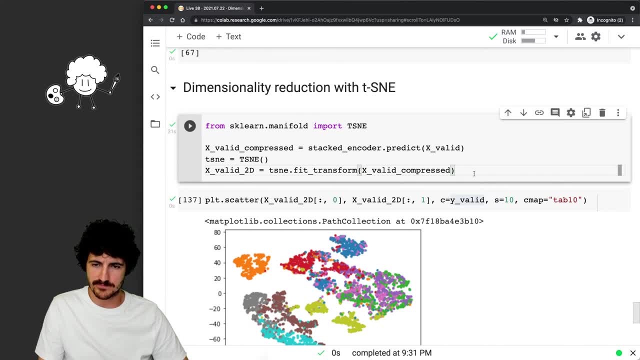 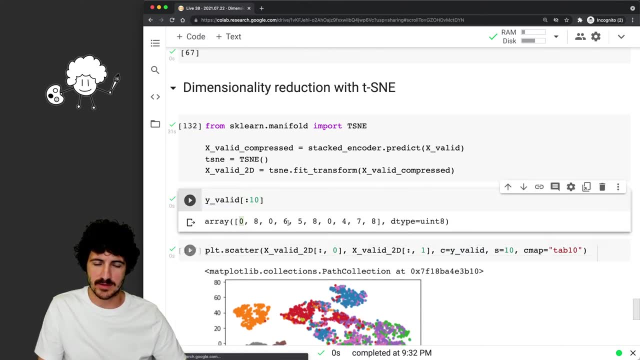 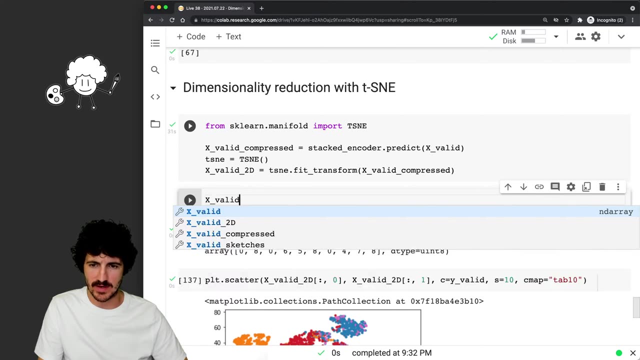 So if we print here Um, just so you see why valid- and I take like maybe 10, right, These are the classes of the data, right? So we have here X um valid And if I take 10, you actually have the images, right? 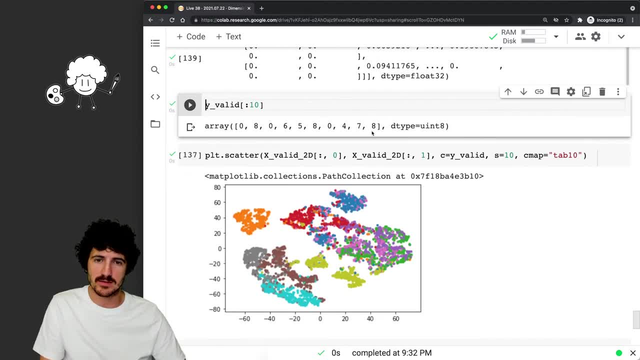 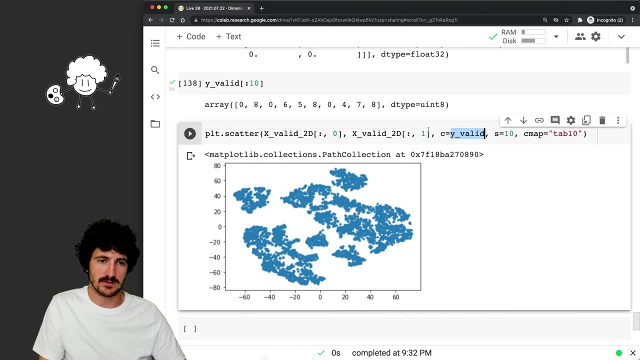 These are the images that we're supposedly plotting there, And then here we have the colors. If I were not to provide that, We'll just get a set of Of um lots Right, And you have to think that those have um similarities among them. 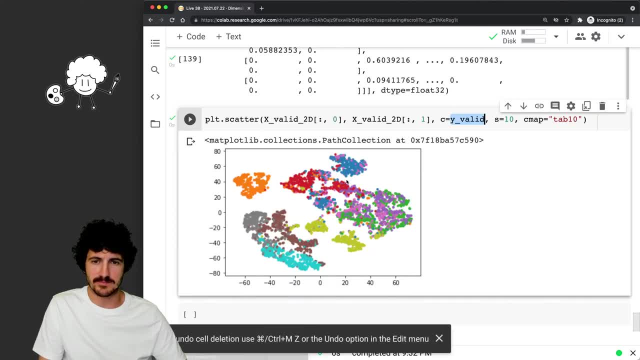 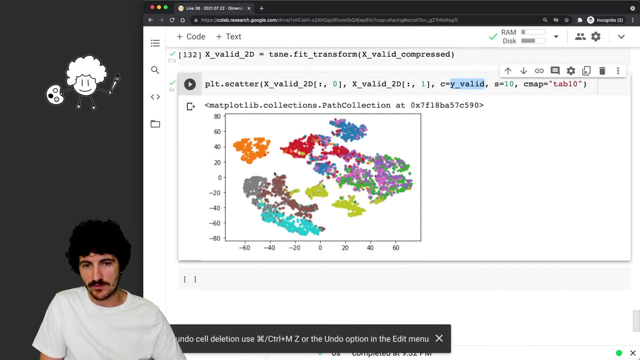 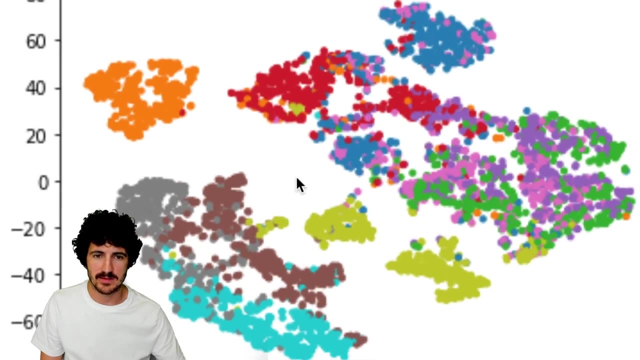 So, yeah, this is, this is Disney, right, This is, um, uh, the basis of what, uh, we were looking at. I want to continue farther with this, So continue um looking at this a bit more and um developing these. 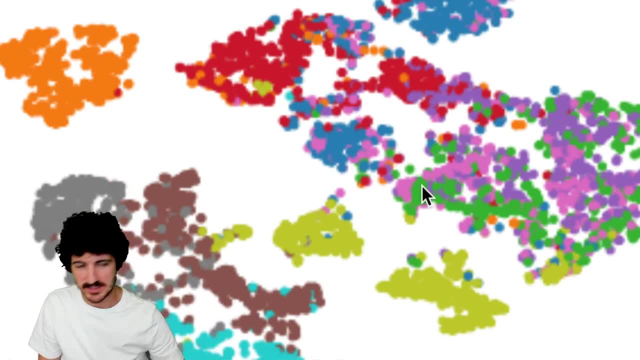 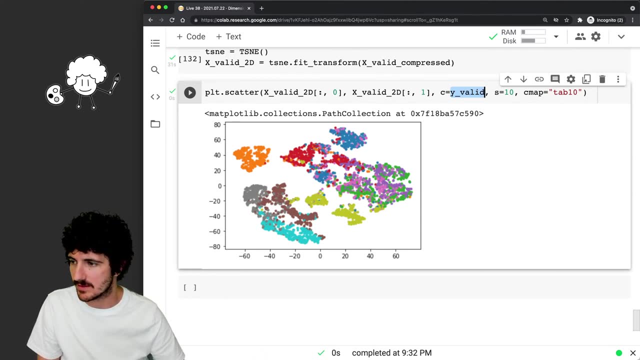 farther, because right now we just see them, We just see like Plots here. We don't even see images or anything. And it would be good to like plot some images here or like even have an interactive board where we display the um, the samples and um, yeah, 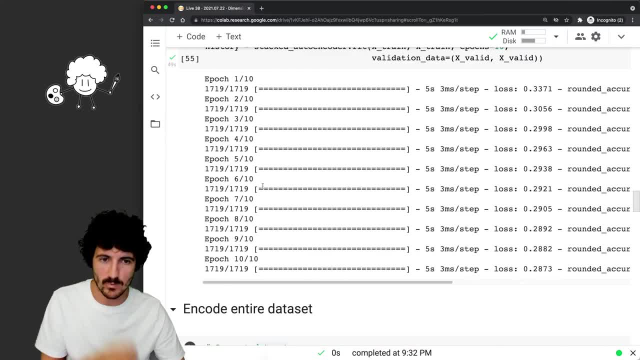 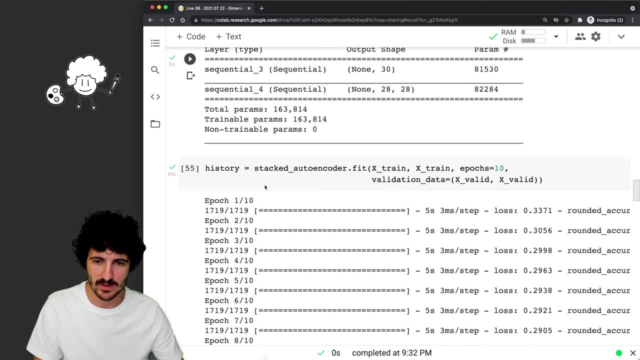 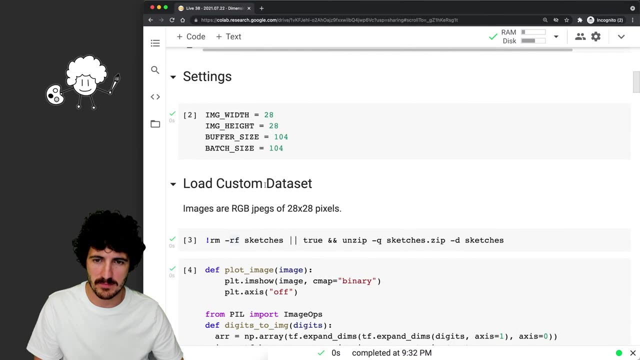 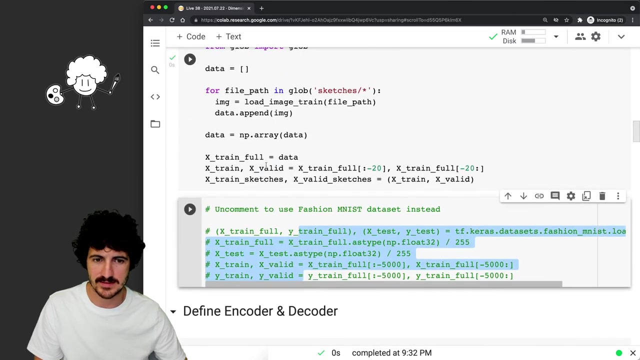 What else? what else can we do? Can I try once more? I don't really know if we're like overfitting or what, but um, yeah, Yeah, Yeah, Yeah, Yeah, Yeah, Yeah. Let me comment this out once again and try with our other data set. 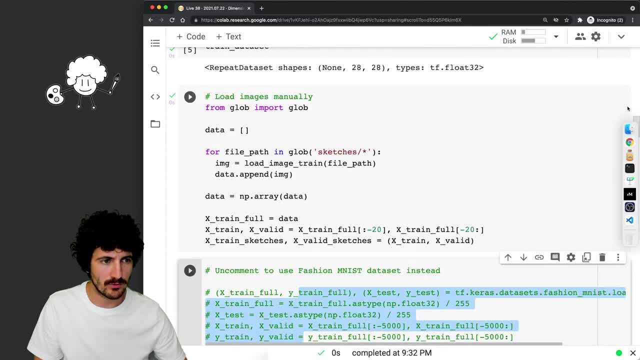 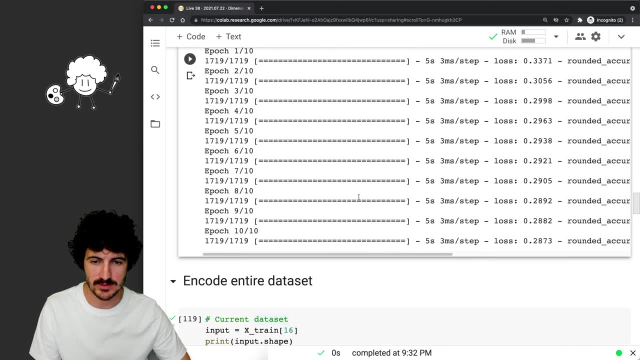 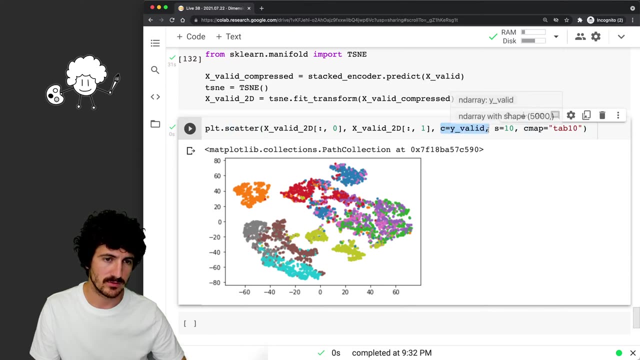 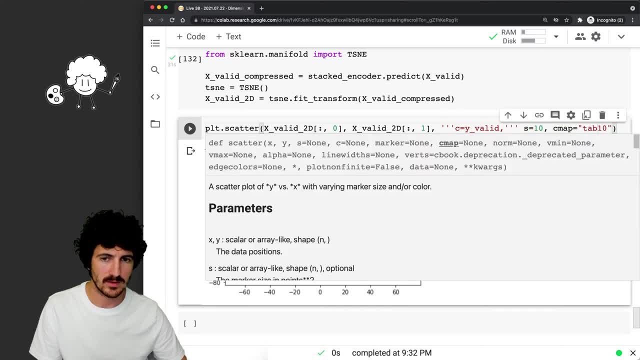 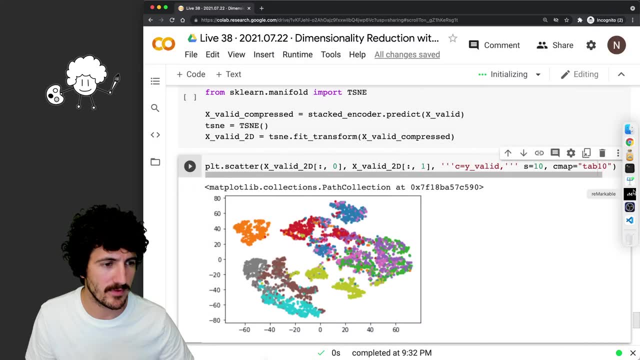 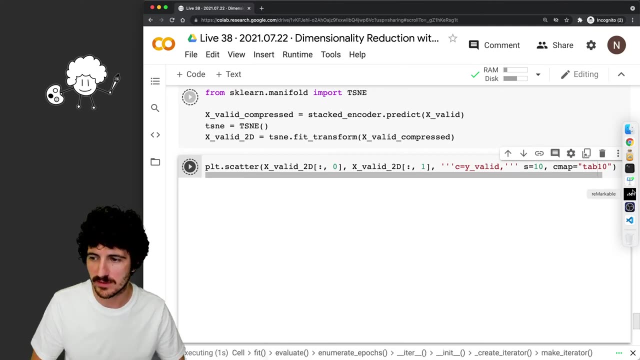 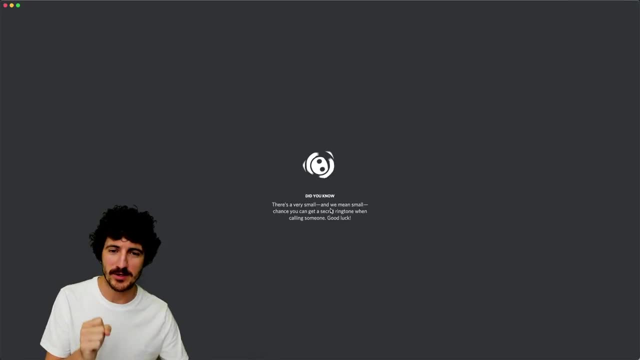 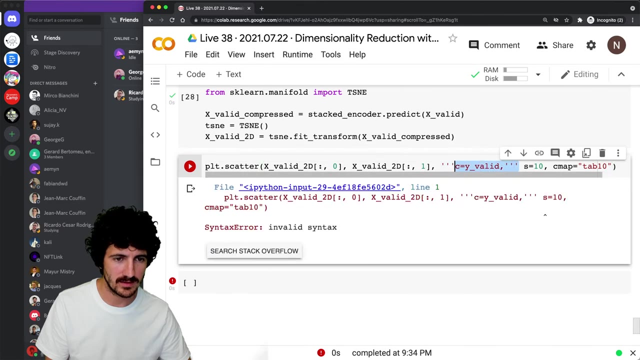 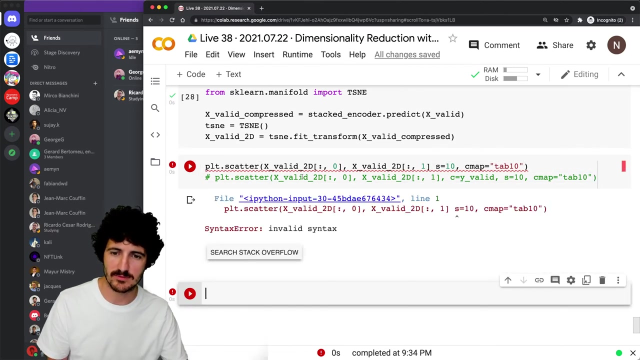 I think we're almost done with this. I'm happy that we go to where we got today and uh, yeah, we'll be. Yeah, Let me see. Well, maybe I don't, but yeah, we're going to be looking at more dimensionality reduction algorithms. 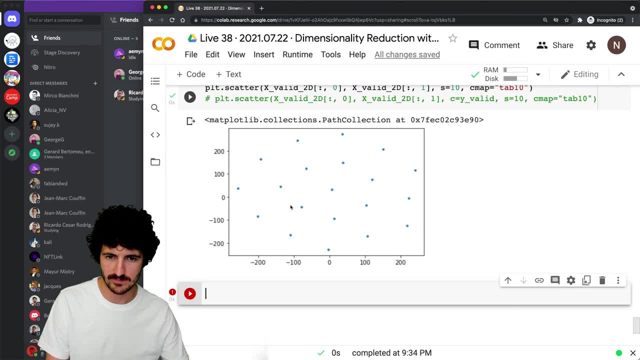 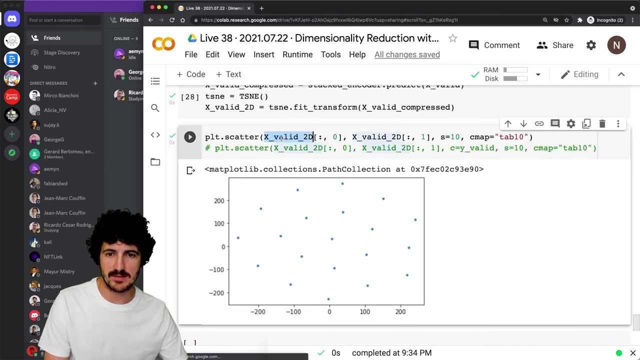 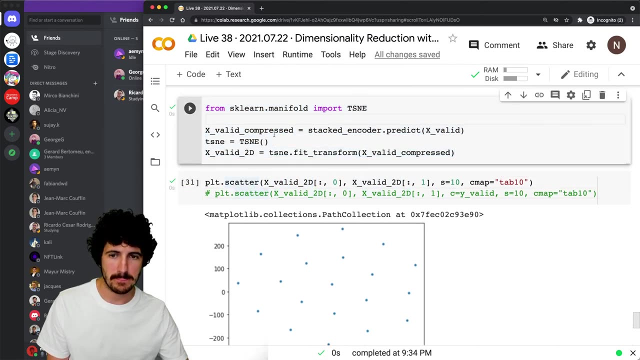 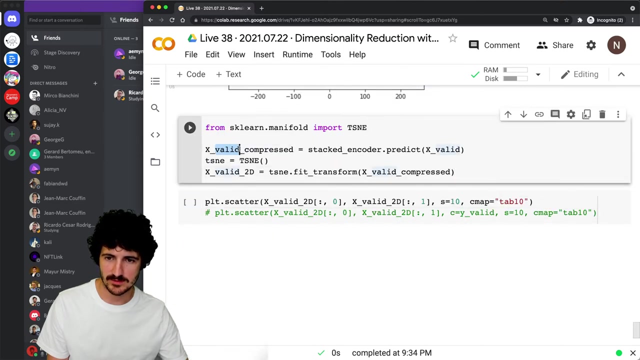 All right, So this goes here. Okay, So what does this mean? So X valid? I don't really want X valid here, We want the actual thing which is: um, yeah, So let's actually do here: X train, compressed X train to the. 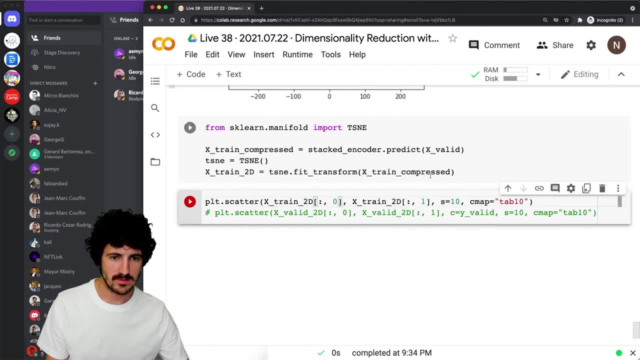 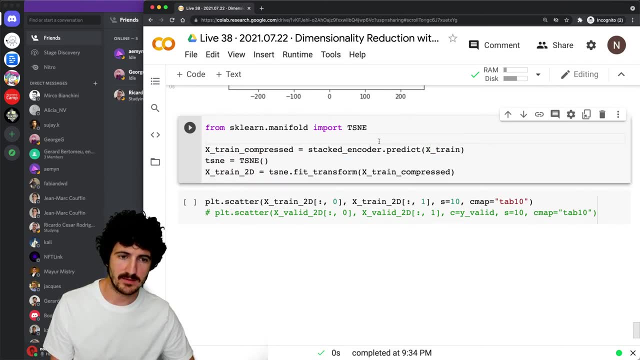 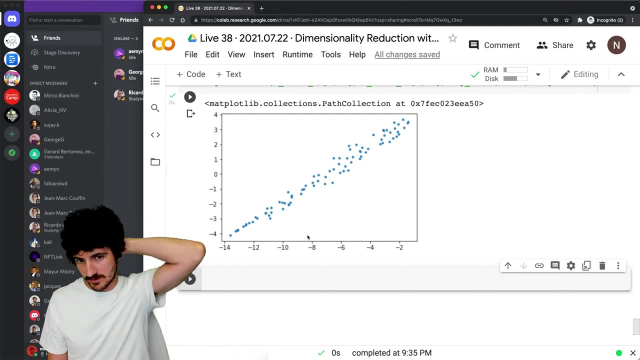 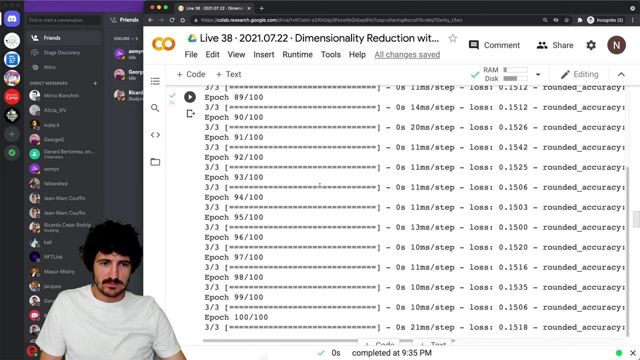 Um, X train, and that should be it, Right, All right. So it seems like it's still is fitting some in some way. these, uh, these drawings by similarity, I don't know that they're that Different for them to to learn any other things, but you know, they're spread on on space. let's say, 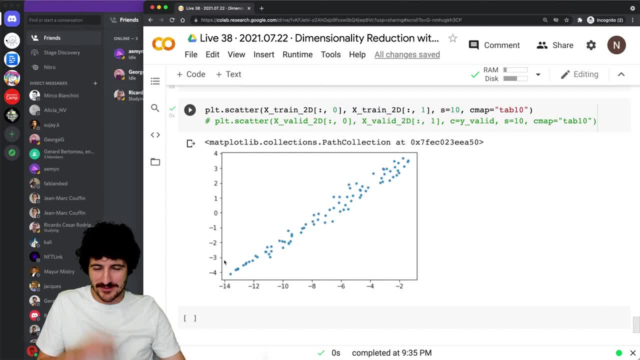 And um, and I really want to now see the plots in in this individual sketches and see which ones they are. Hmm, How can I, um, sorry, you've never seen it before. Yeah, In this, in this, in this end, I'm going to go ahead and, uh, just read it here. 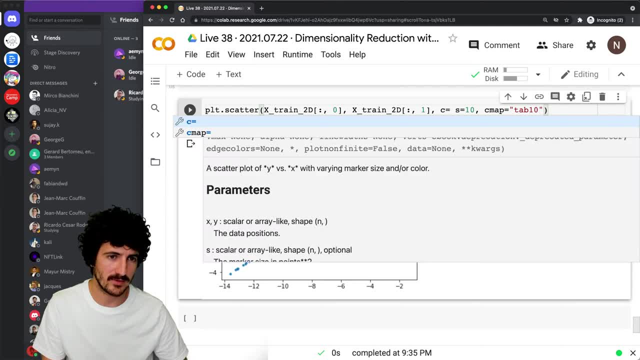 You want to write the plot of the plot here, the plot of the plot, and make, and then you can do the plot like a nothing. Okay, So you start out by saying, Hey, okay, So we have the plot, the plot of the plot. 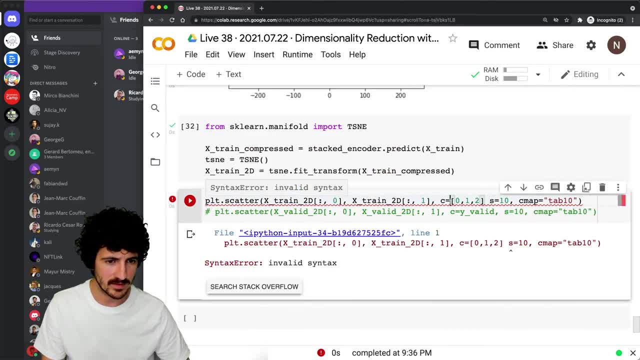 And you're going to go to a particular plot. you're going to write in the plot: Okay, You make a straight line. You make: make a straight line, Okay. So the plot is like this: You make a straight line. 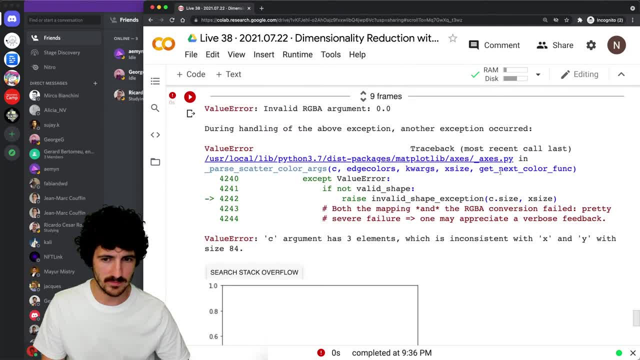 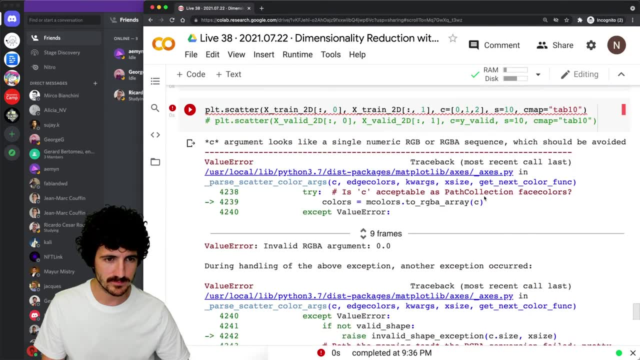 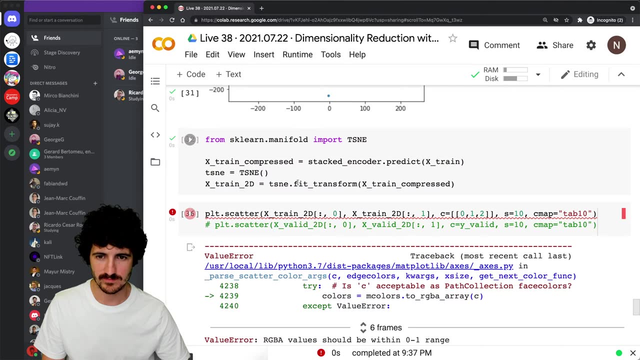 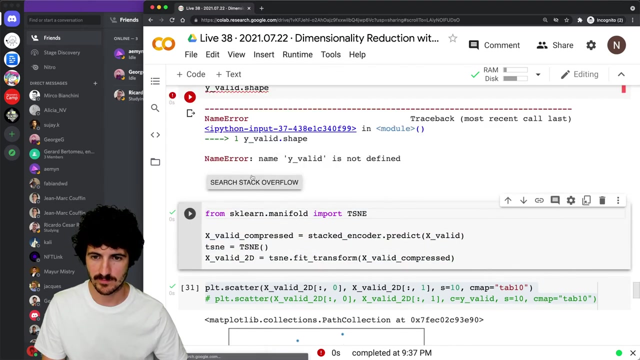 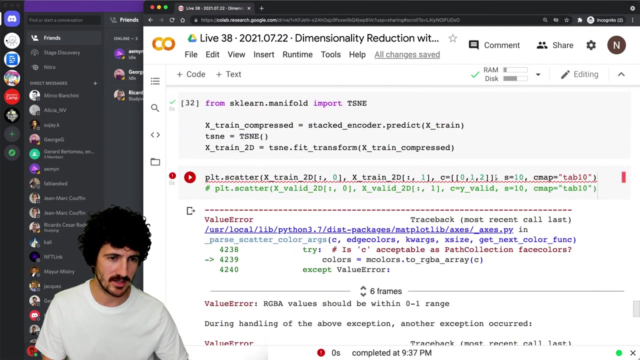 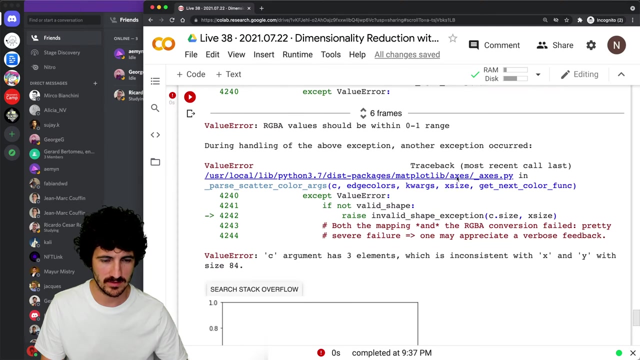 Okay, So that's nice, You make a straight line here. Okay, What's the plot of this plot? You make a straight line here, Here, Hmm, I don't remember now what the shape of this was: 84 with X and Y. it's size 84.. 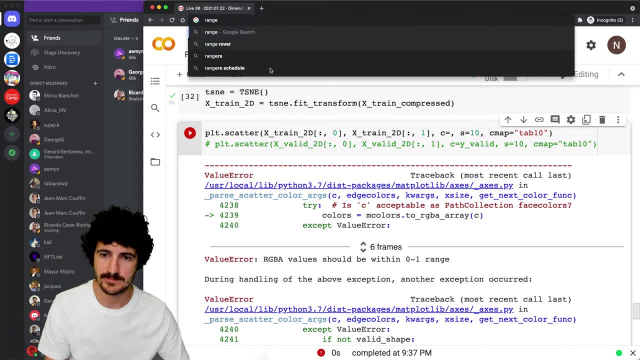 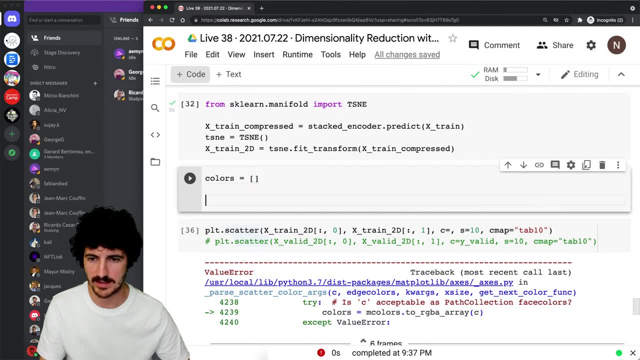 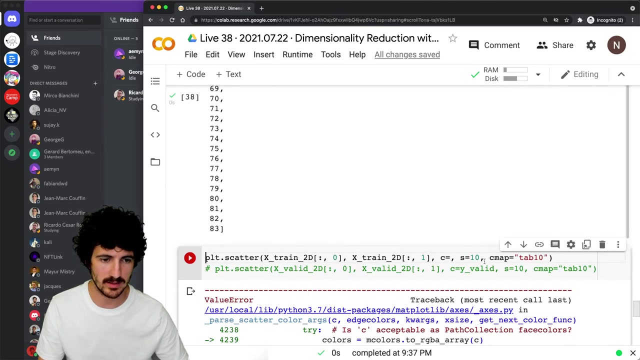 All right, So range: um. well, let's actually make a list manually. So colors equal that. And for E in range 84, um colors, append I Colors, Let's see All right, So we get 83 and then we can put that here. 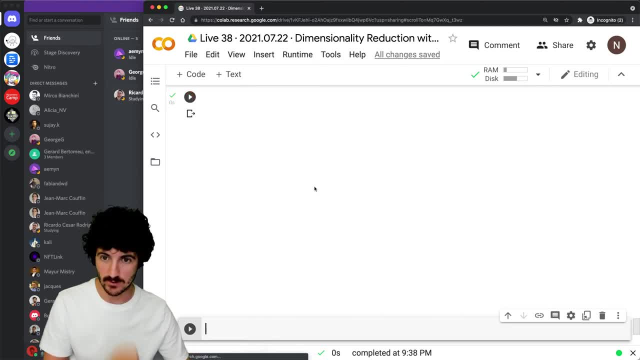 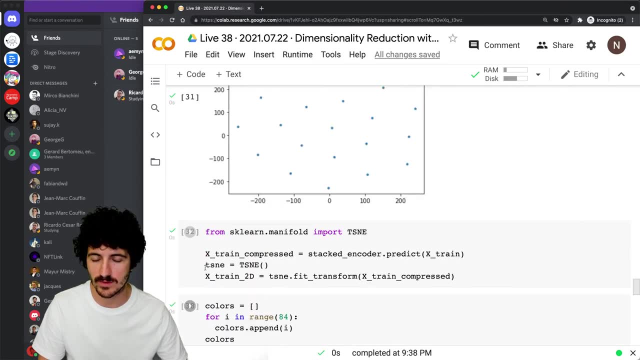 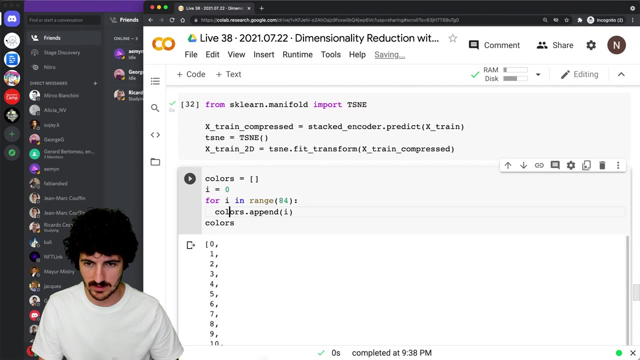 Colors. We get 84 colors and that plots. All right, That is useless, right, But we're going to do something, just at least to cluster them. So we're going to say: equals zero and E plus one, And then when? 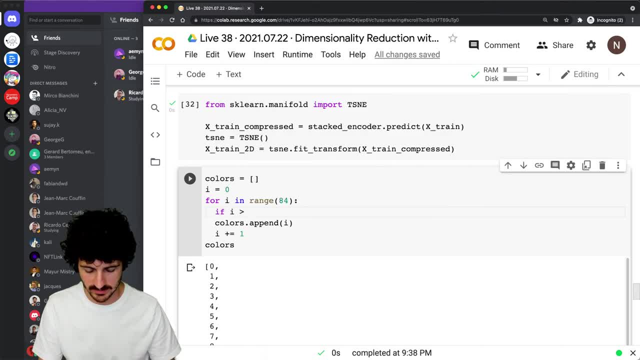 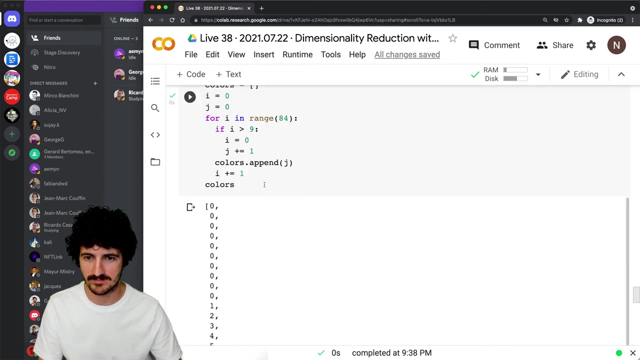 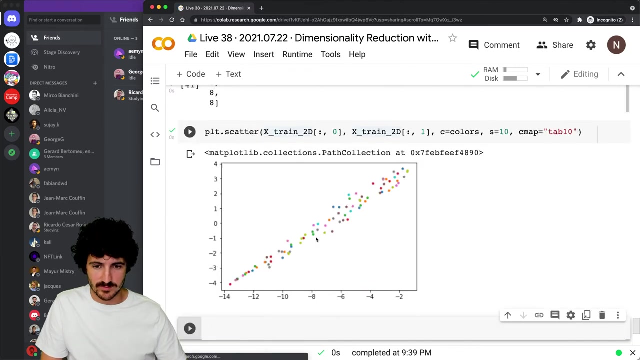 I, if I is greater than nine, I is going to be zero and J is going to go up. So J plus one. So we have less colors. No, not really I. oh no, All right, So let's see how those colors play out. 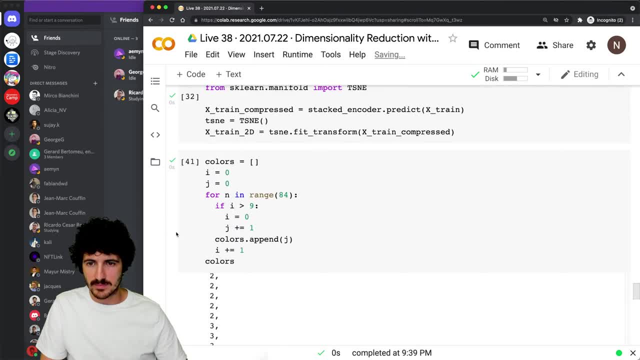 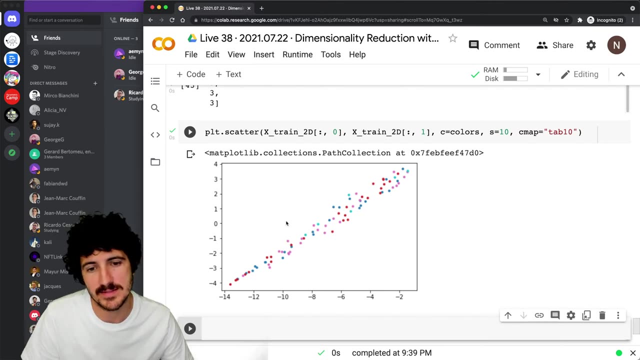 Great, We have too many colors still, so we might just need, let's say we just have three clusters, so 84 divided by three, that's 28,, 25,. right, We have not three colors. So it means that DC's telling us that drawings that are not initially um. 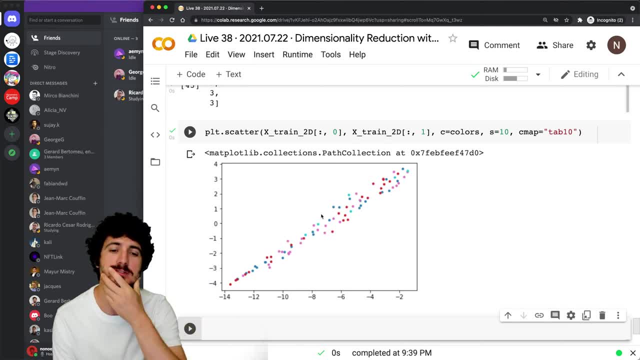 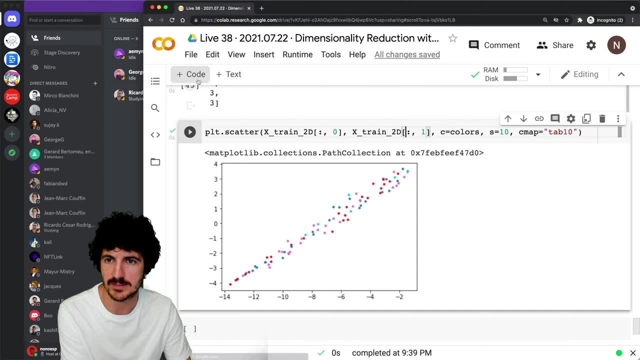 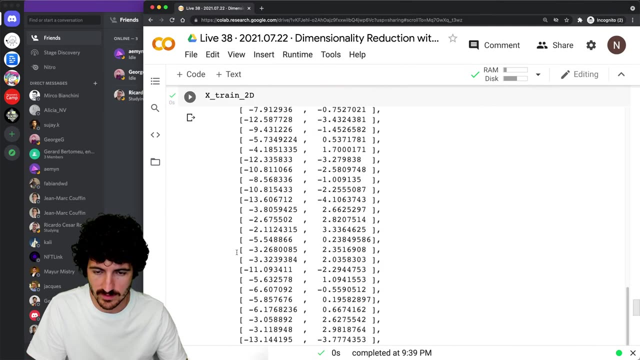 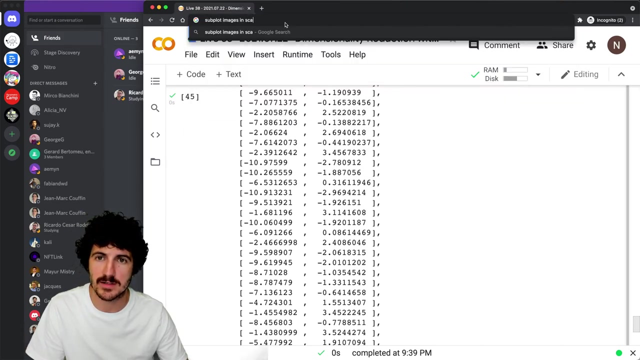 together. right That this is not the order. they're like being clusters, clustered in different ways. Um so maybe Uh to, to, to to. let's inspect now that X train to be So uh soup plot images in scatter. 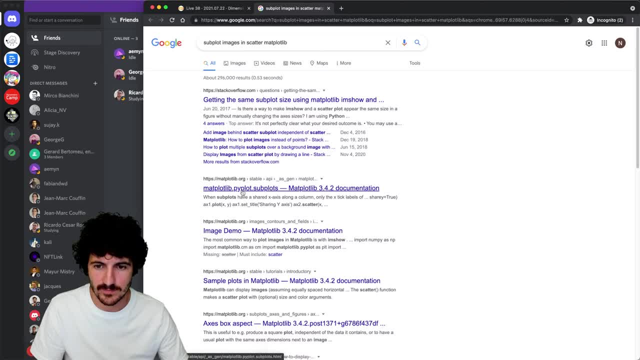 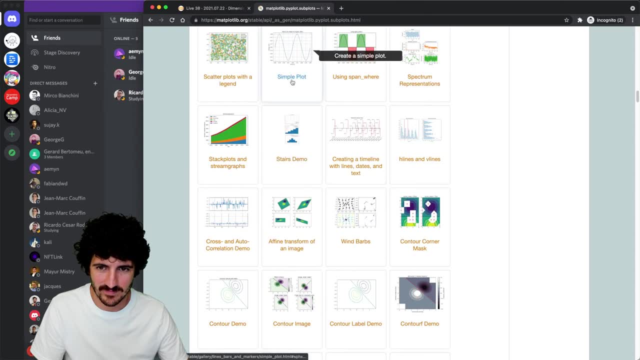 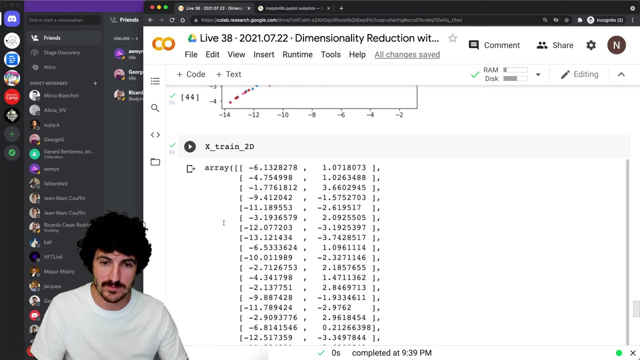 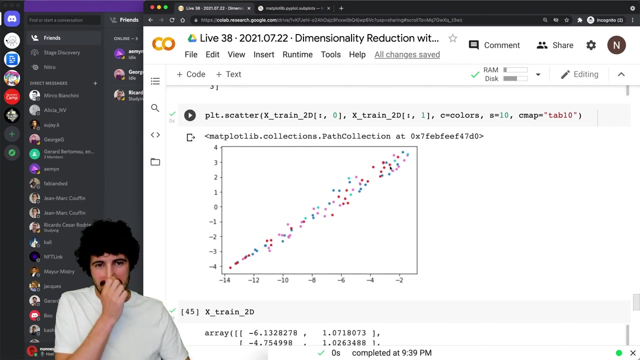 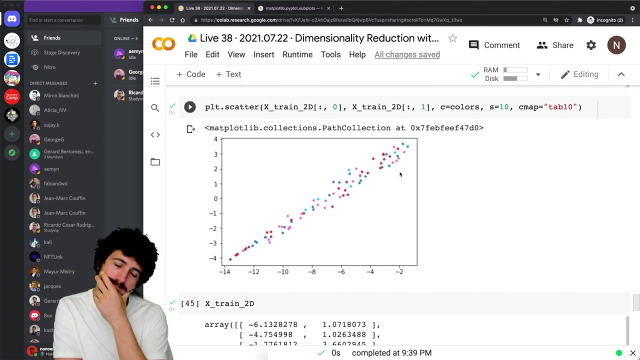 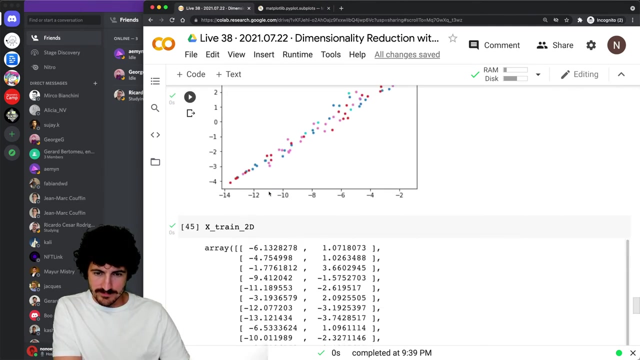 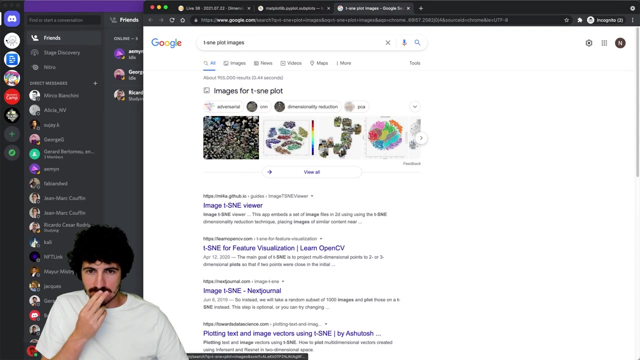 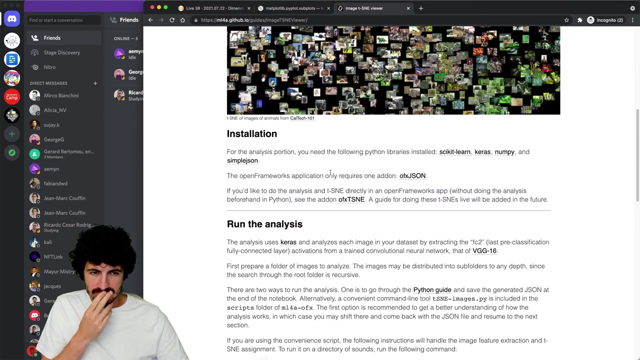 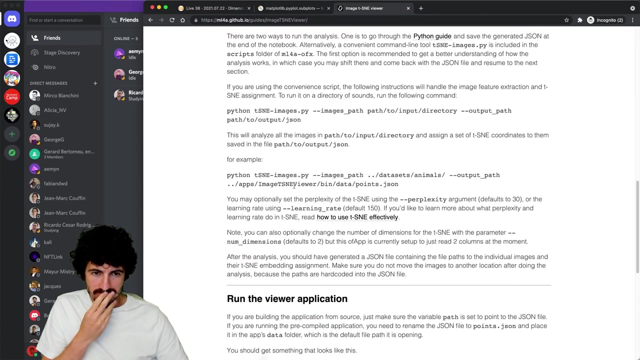 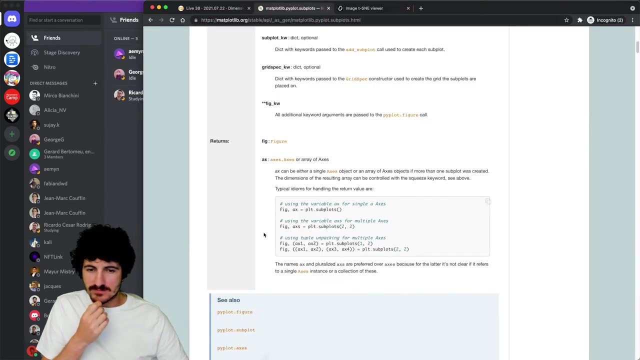 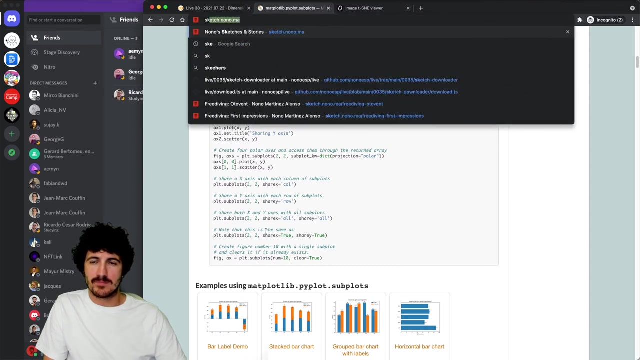 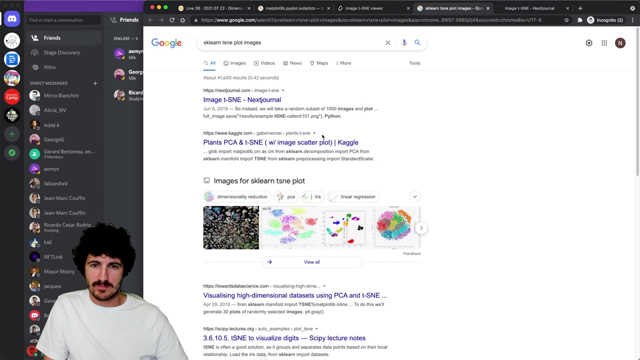 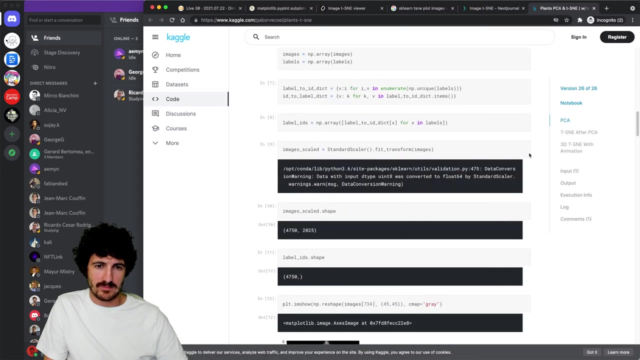 Can we do this? Okay, that's another challenge, okay. so, hmm, I wish I could just grab what images were these ones. I wish I could just grab what images were these ones. I wish I could just grab what images were these ones. 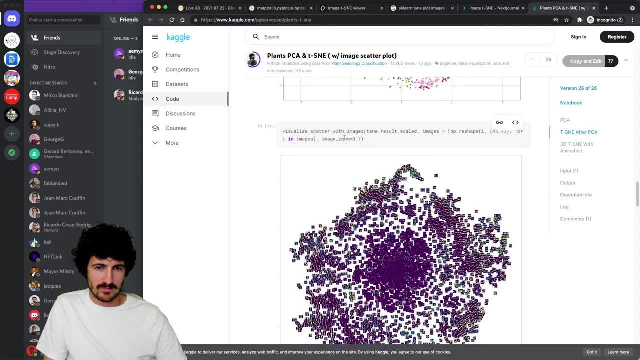 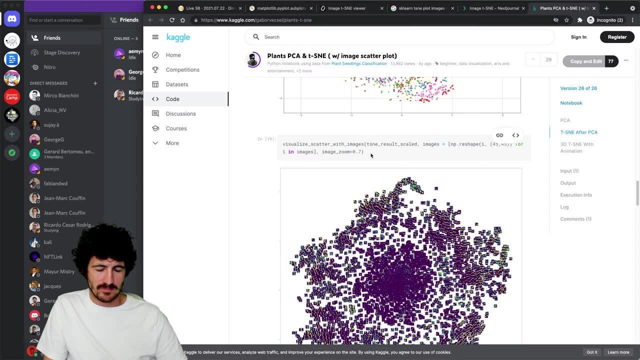 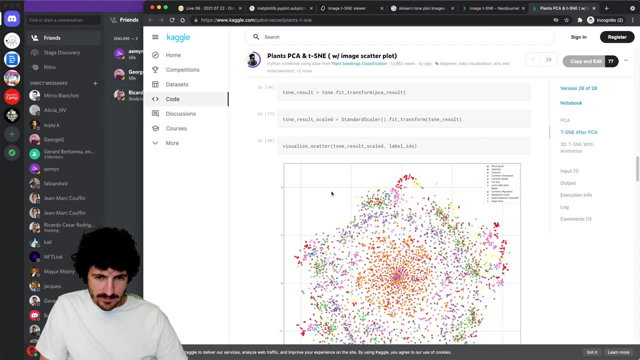 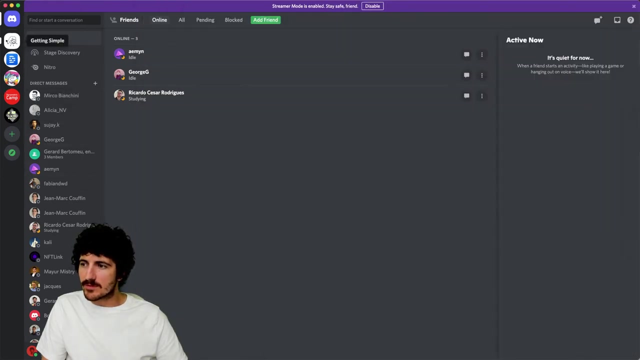 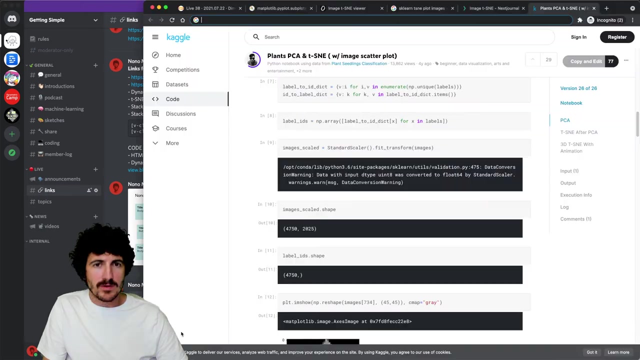 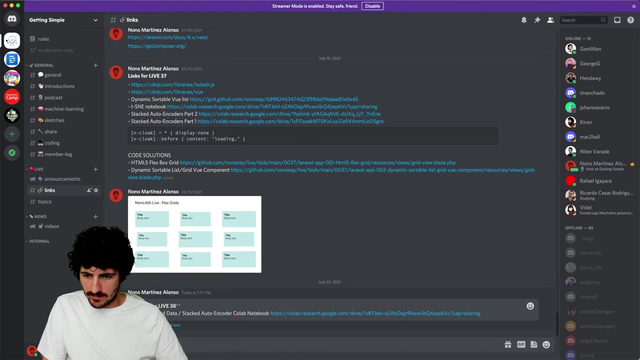 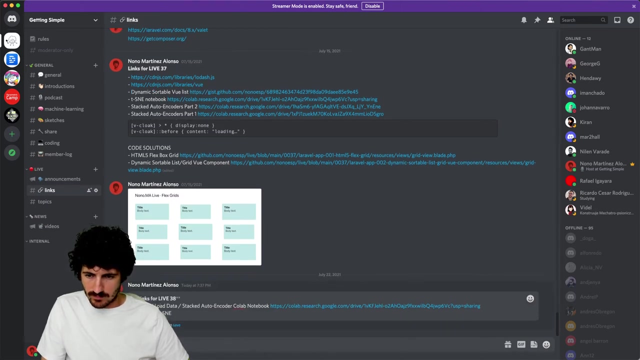 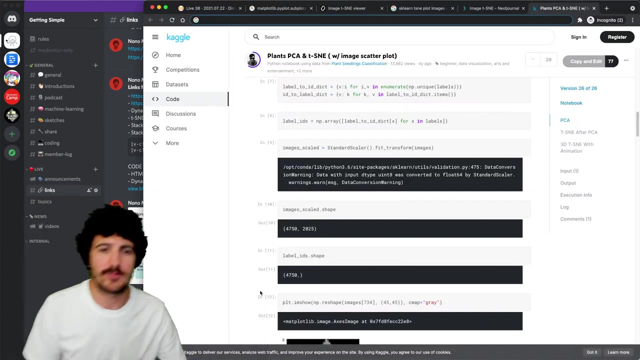 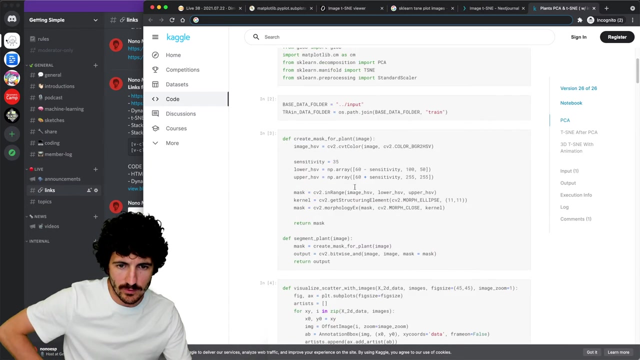 okay, I'm going to paste this link because it's pretty cool and we can probably continue with this one, and we can probably continue with this one, all right. so what do we have here here? manifold from t-SNE. 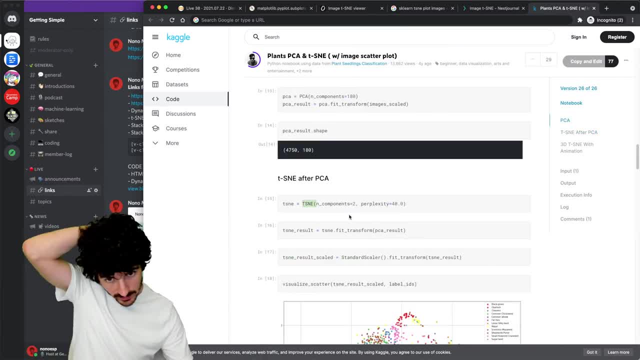 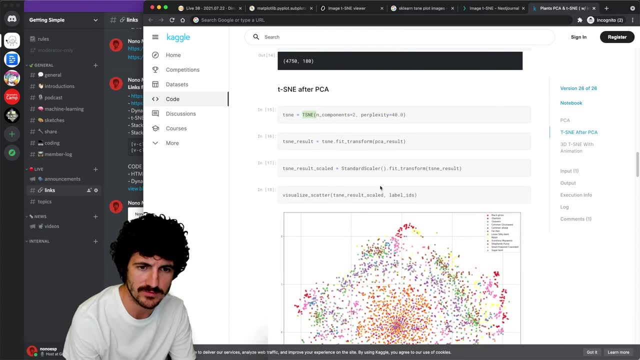 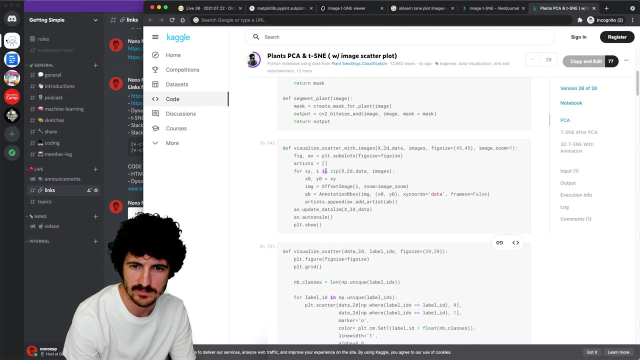 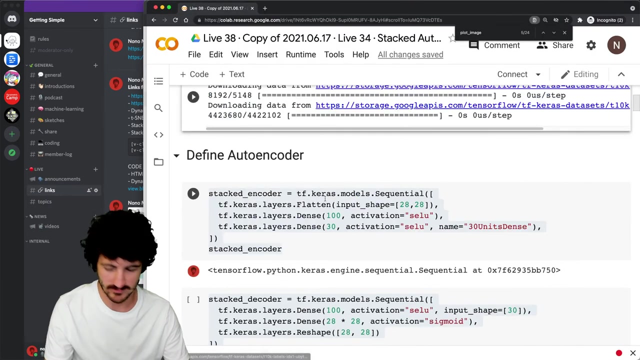 from t-SNE, from t-SNE components to perplexity 40, feed transform results. scaled feed transform visualize: scatter with images. let's try to just copy paste this one, which you shouldn't really copy and paste code. 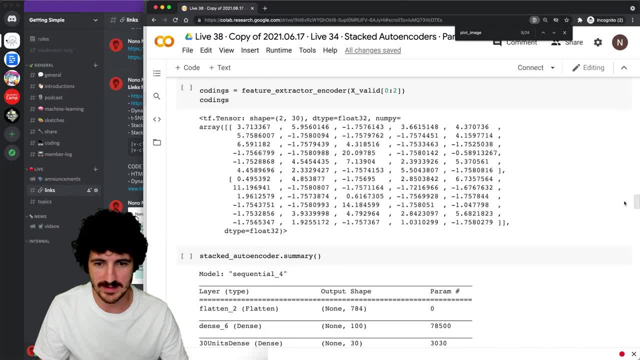 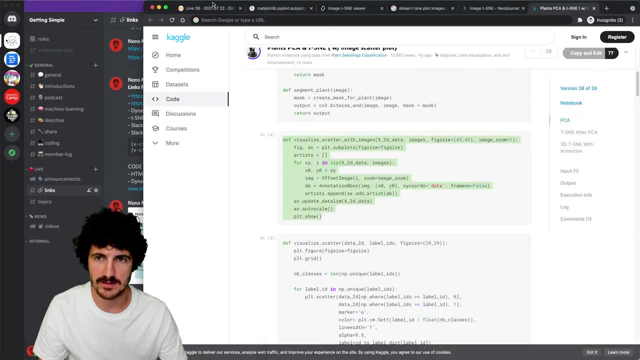 but because we're finishing up, but because we're finishing up, let's see what we have. let's see what we have, let's see what we have, let's see if we get that stretch goal. all right, so we got this here. 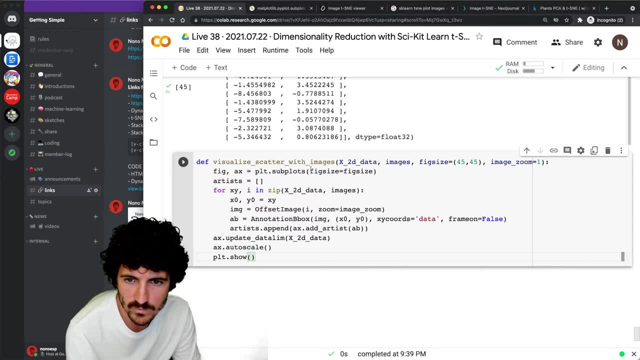 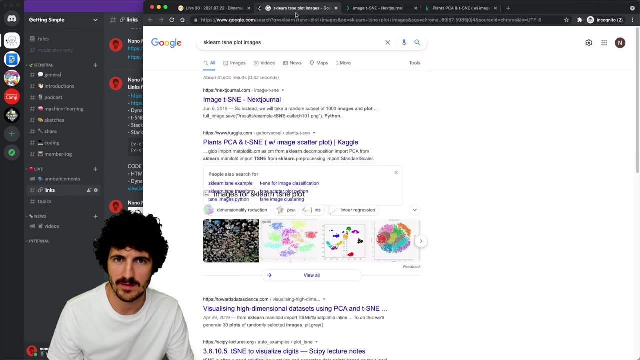 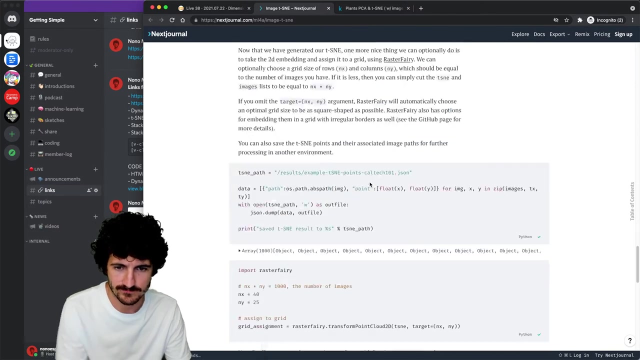 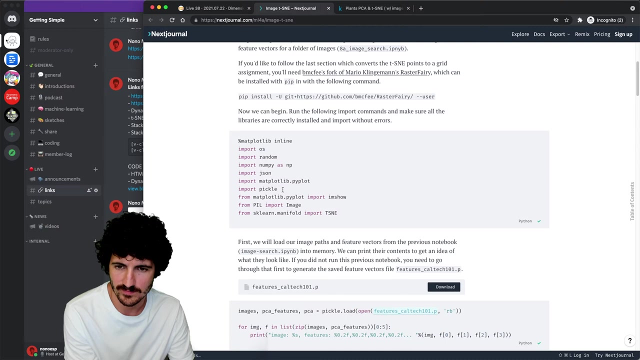 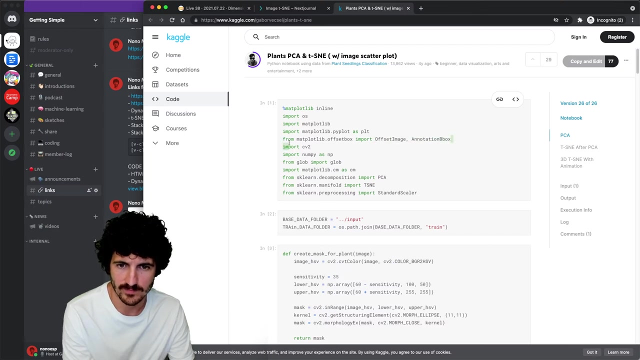 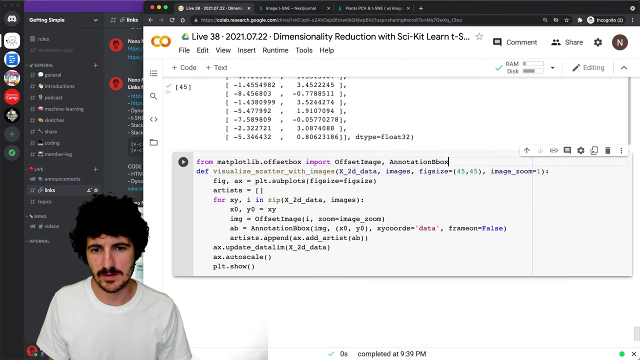 and we have this. so plot annotation. bounding box- offset image. what are these helpers from? what are these helpers from? what are these helpers from? oh, here comes a couple. alright, alright, all right, all right, okay. 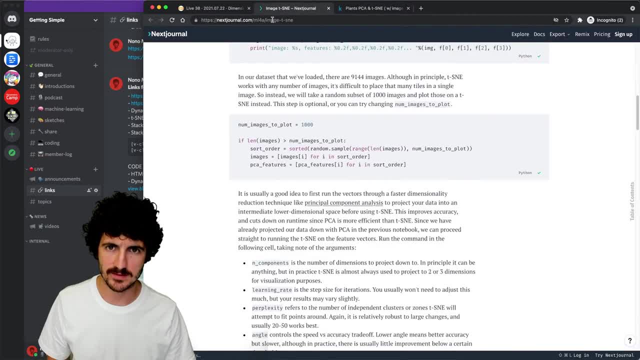 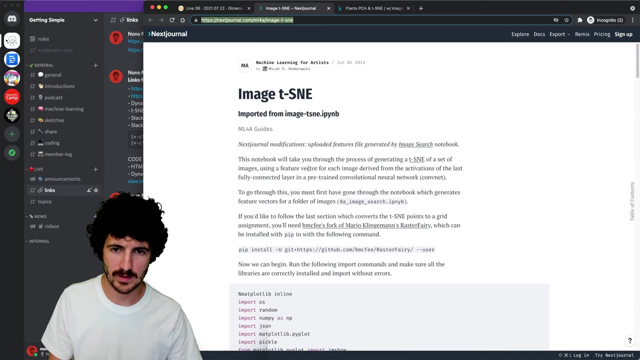 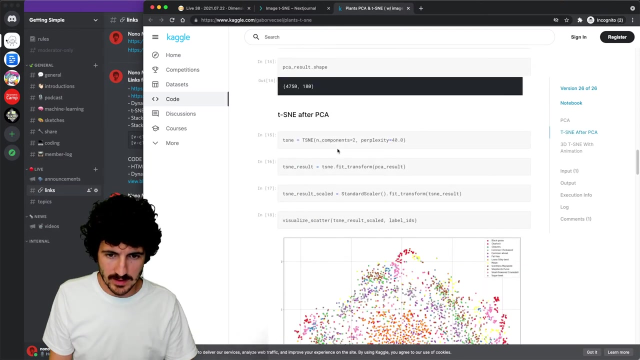 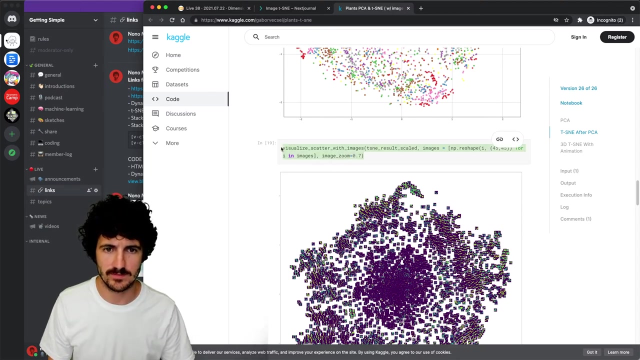 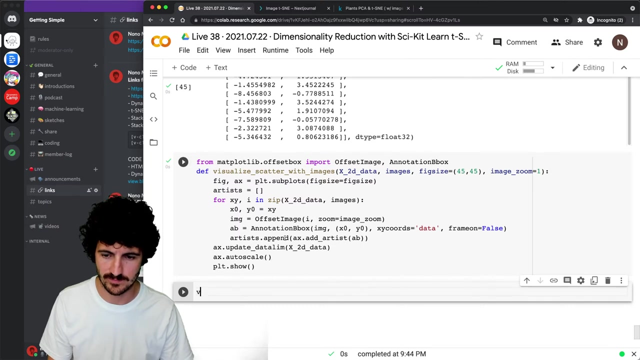 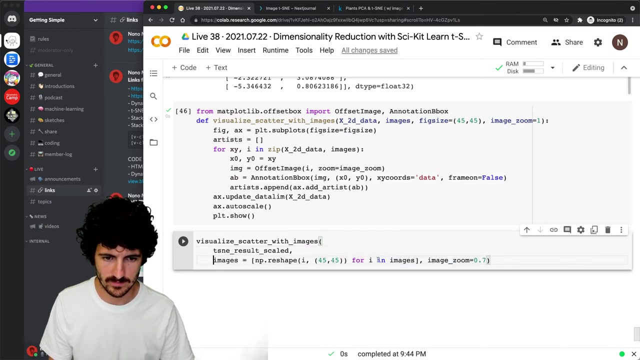 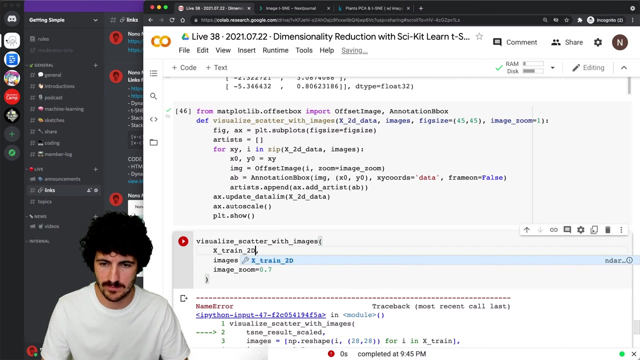 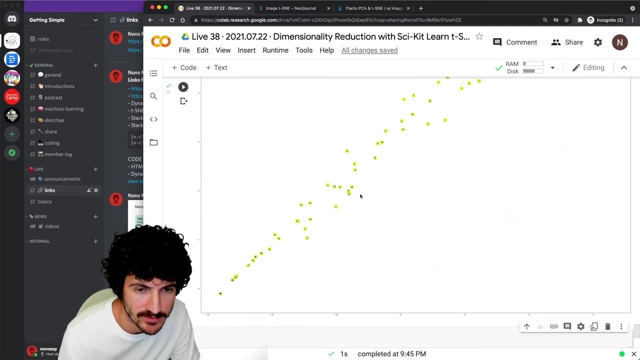 let's see. okay, okay, let's see, We can define this as another one. that might be good. So visualize, scatter with images. Let's see. Oh, that is awesome, All right, So copy pasting. that goes for the web. 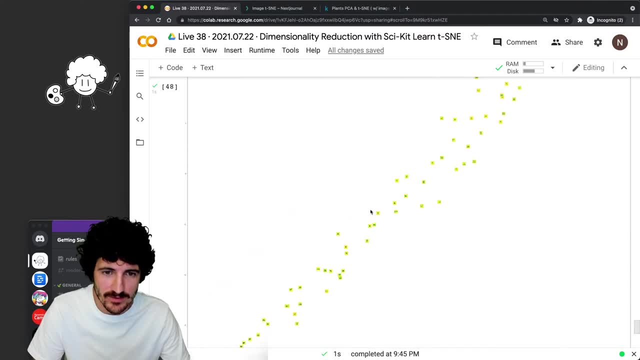 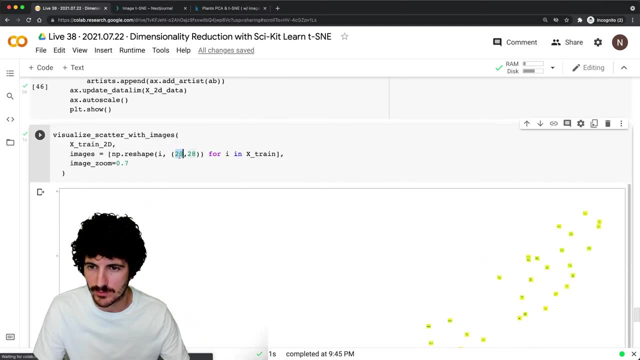 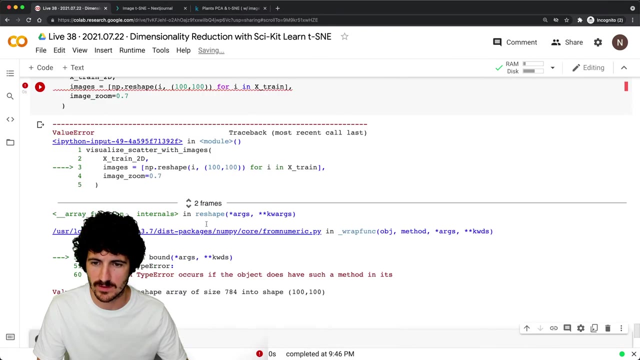 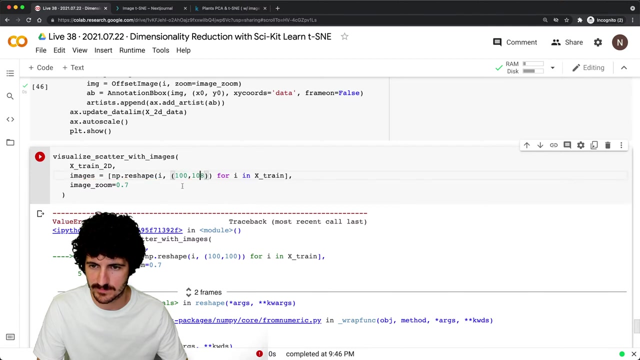 All right, That's awesome. Okay, So we got A pretty good resolution image, I think, And I might be able to maybe pump this up. Can I reshape array into shape? Oh, reshape, not rescale. Okay, Image soon. 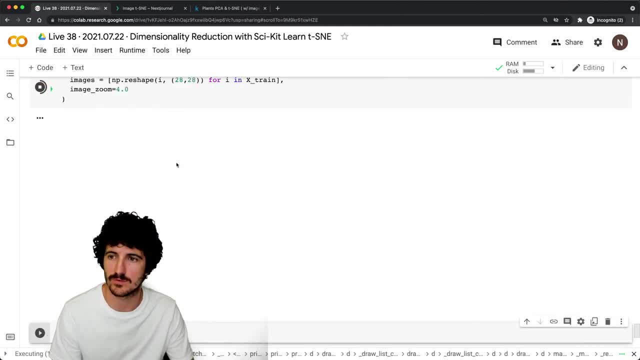 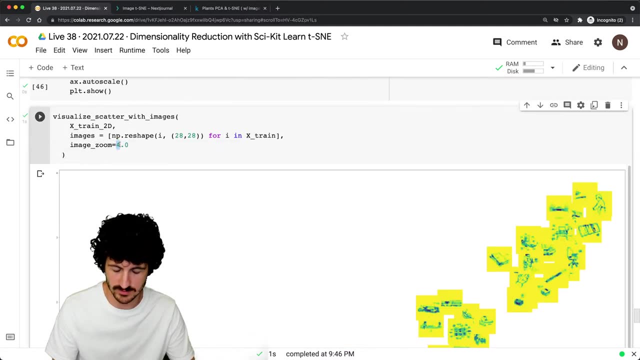 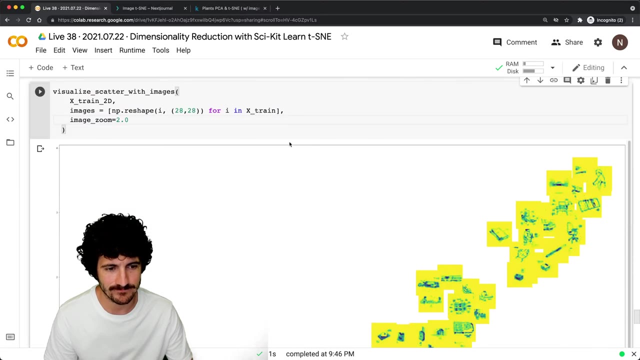 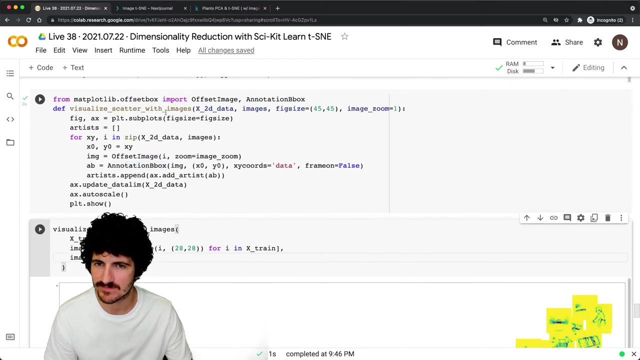 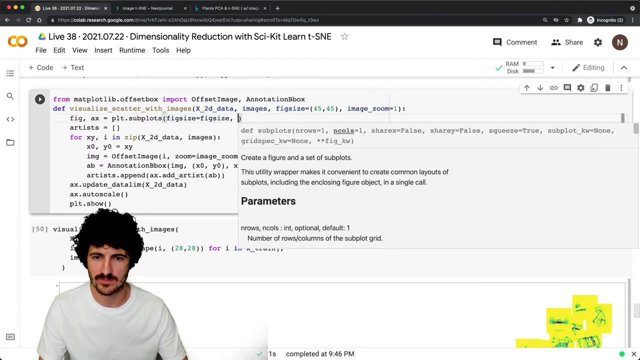 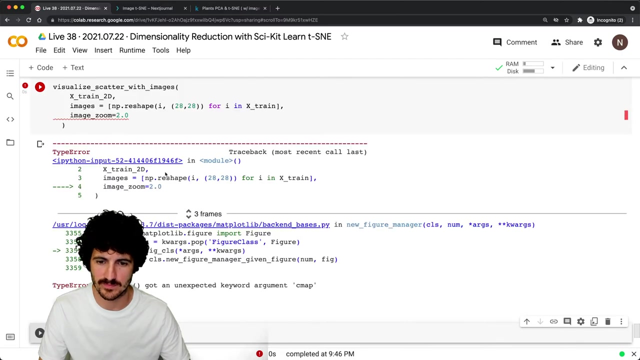 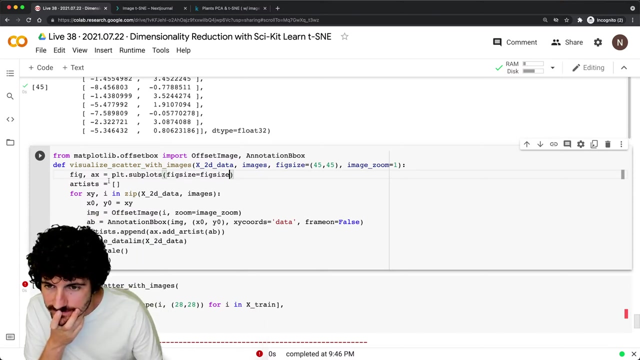 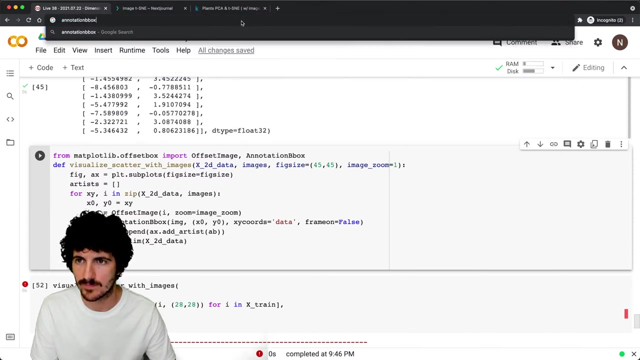 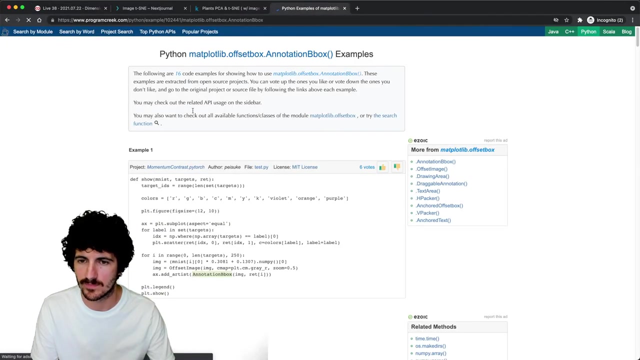 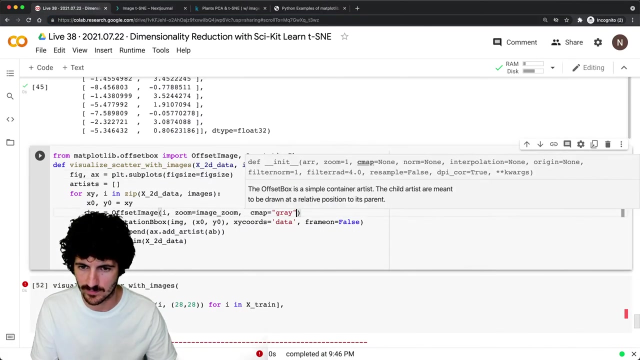 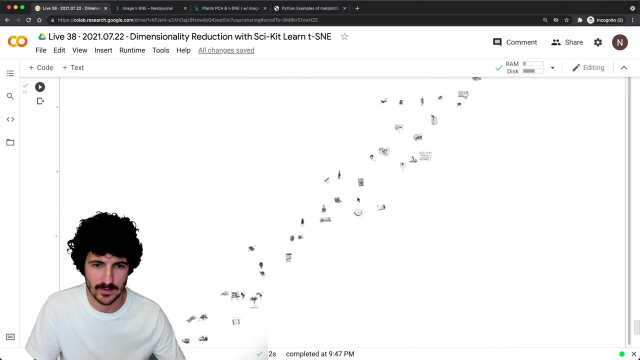 Let's do maybe four, because this is, these are too small. Great, This is awesome. Okay, So maybe let's just do two. I don't know why it is coloring with that. Hmm, Okay, Okay, Thank you, Thank you. 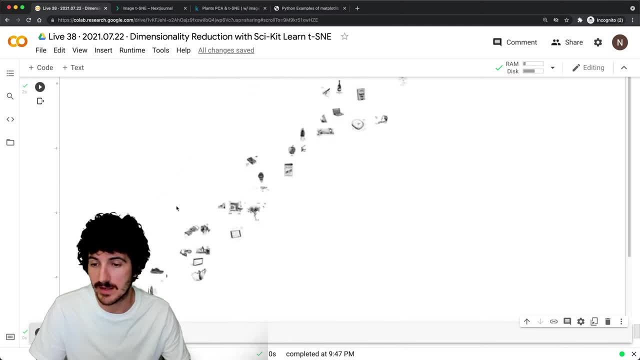 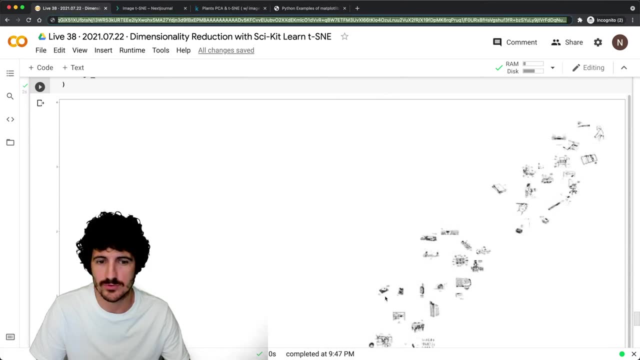 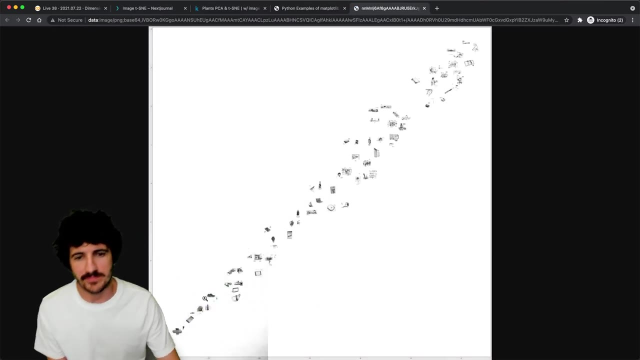 We got it. So, um, I don't, I don't think we're gonna. you know we're going to get too far with this. but long story short, I think we got it. We got what we wanted. So it seems, in some way it doesn't seem like it learned too many different features. 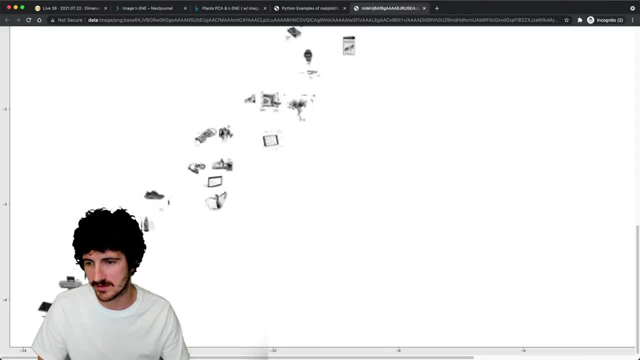 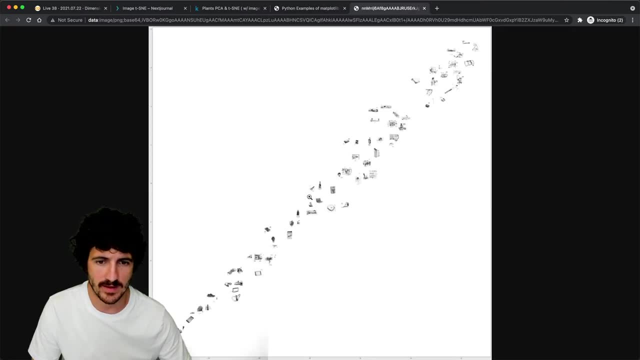 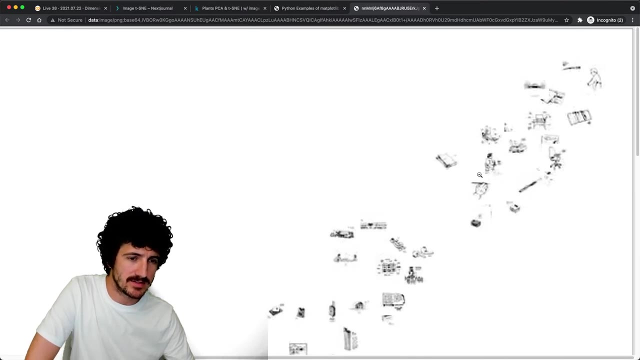 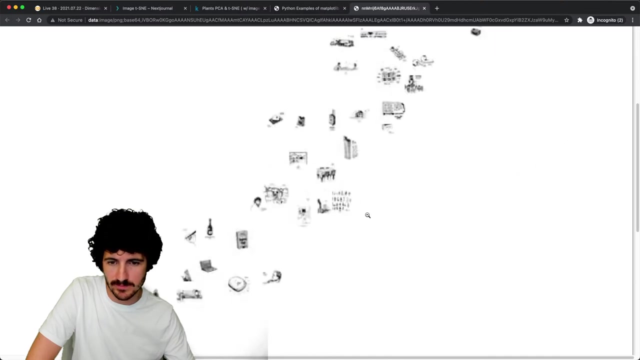 Hmm, It just seems like the darkest ones are, or like the more infield ones from the bottom left. Yeah, I don't know, I wouldn't, I wouldn't say there is anything specific that well, I mean, these ones are the ones that are from some like people, I'm here. 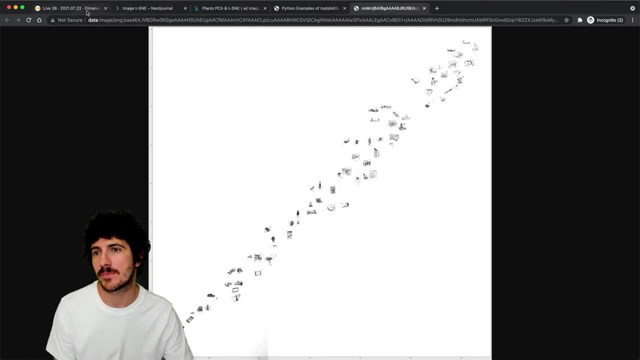 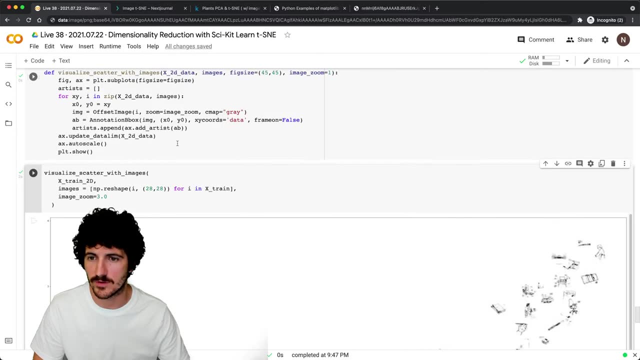 Yeah, I'm not sure I mean, but these, these sort of work, And, uh, if we, I think it would be a bit crazy if we do that with a segment of of the other ones. So this is pretty cool. 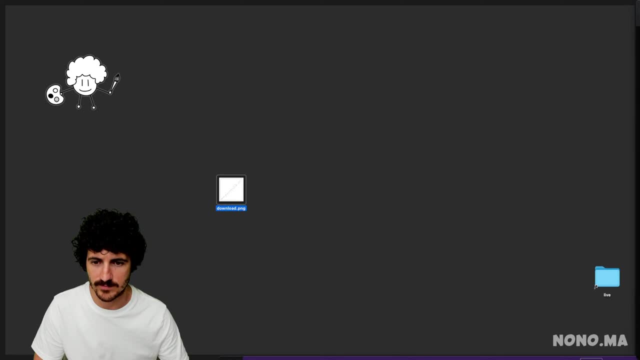 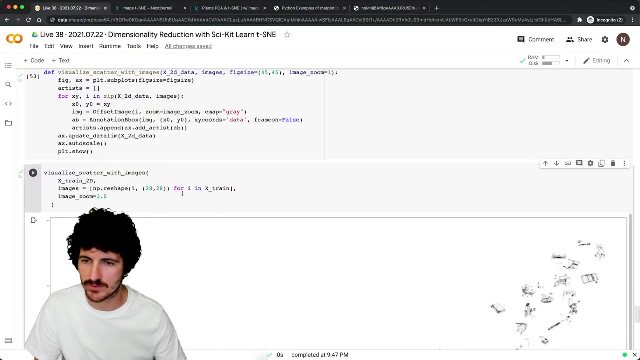 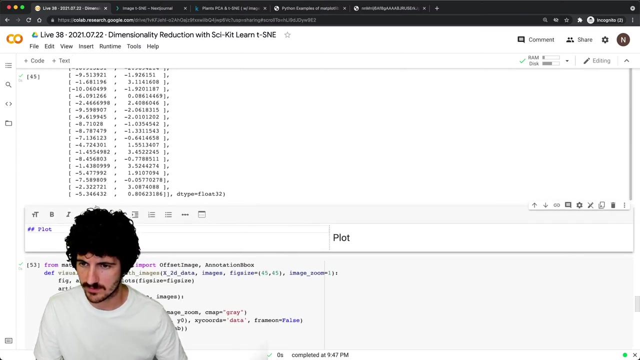 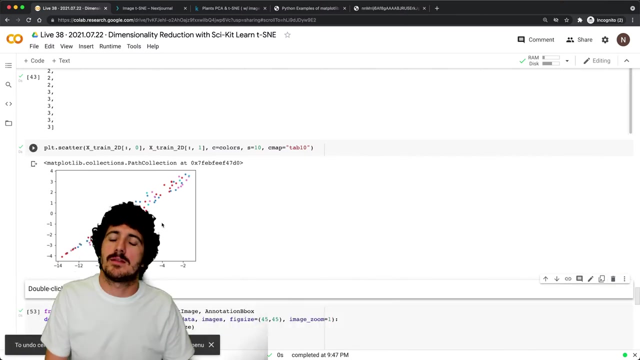 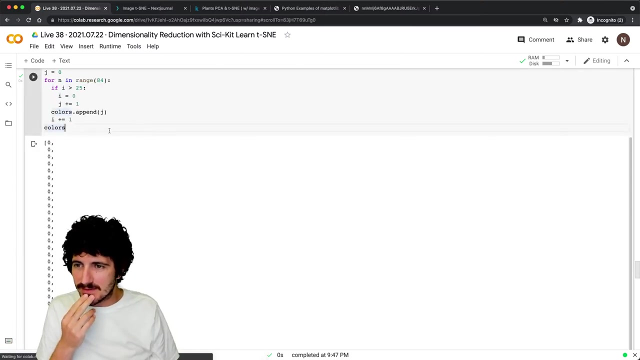 I'm going to save this image. Um, we can plot that share it. And, uh, I think it would be cool to get a subset before we go get a subset. And, um, so let's do a plot, I'm going to remove that one and, uh, maybe you know, I want to make sure this doesn't bump when I go with the full other full data set. but I think it's okay. 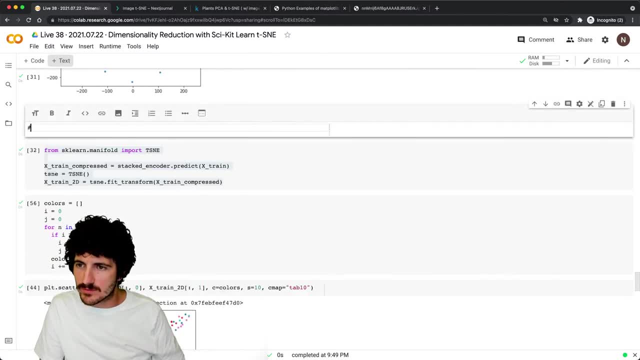 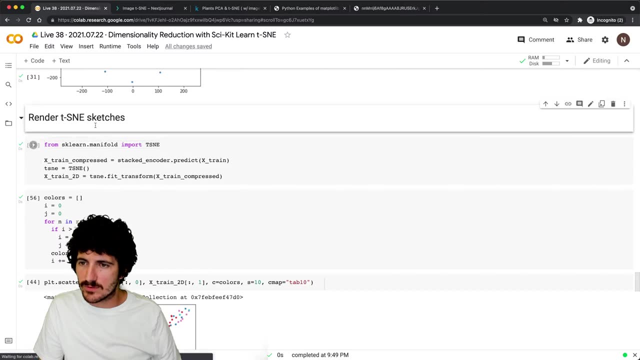 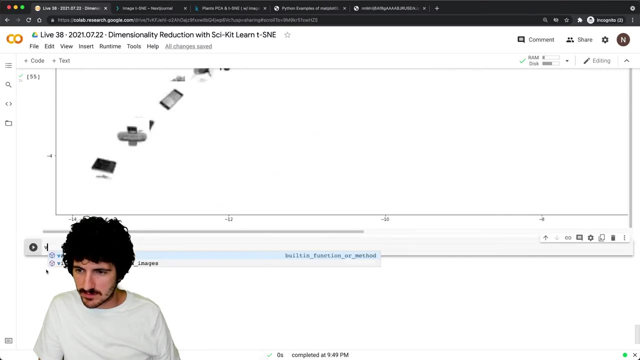 So let's try to just copy. Okay, So this uh render Disney sketches. Um, uh, we're now going to Copy these and paste them. I don't know if I can pay them here. I did paste, Um. 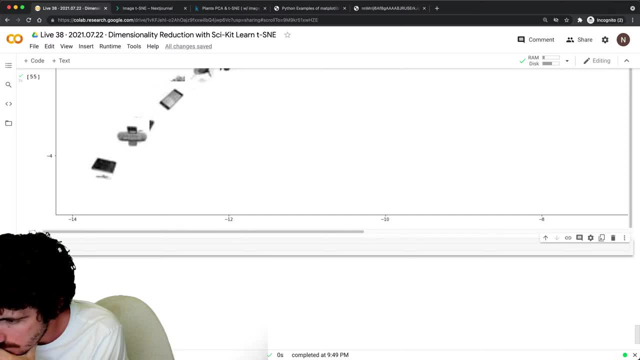 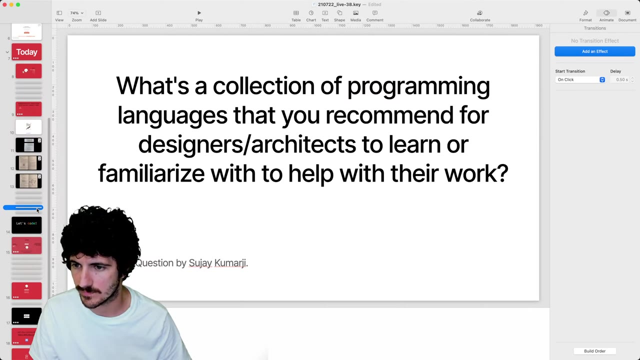 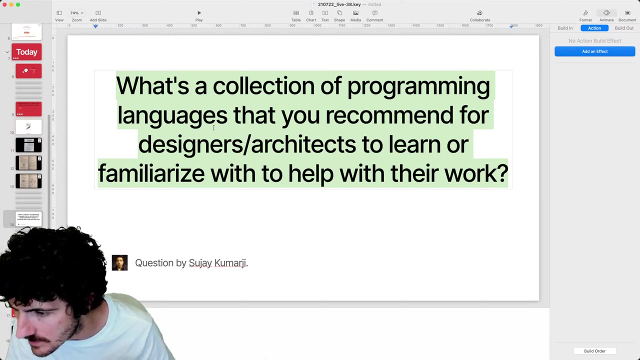 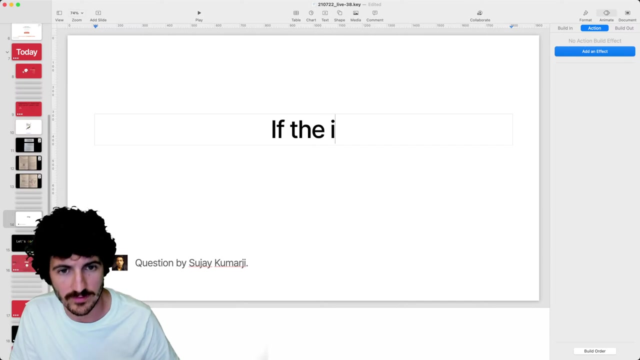 Oh, Um, okay, So the, um, the question that is being asked- and I'm going to put it here because I think this is super relevant- So yet, um, so on, skip slide, uh. these would say: If the, if the images, if the. 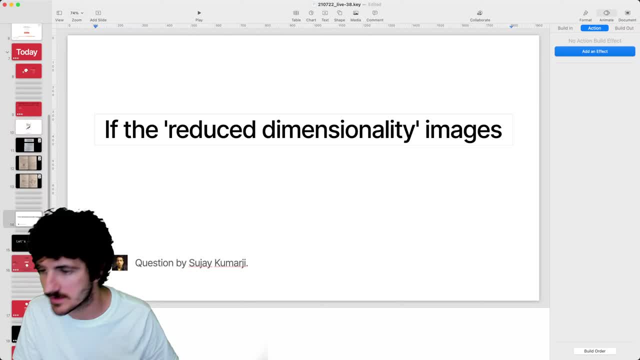 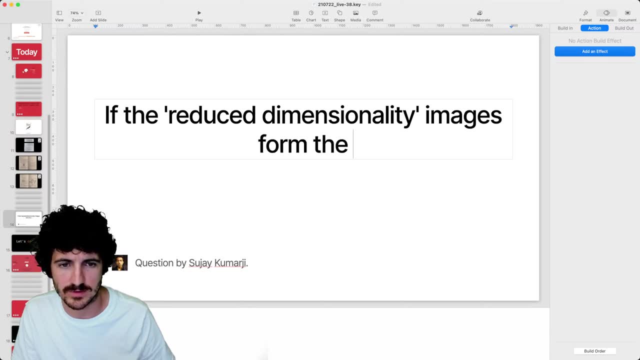 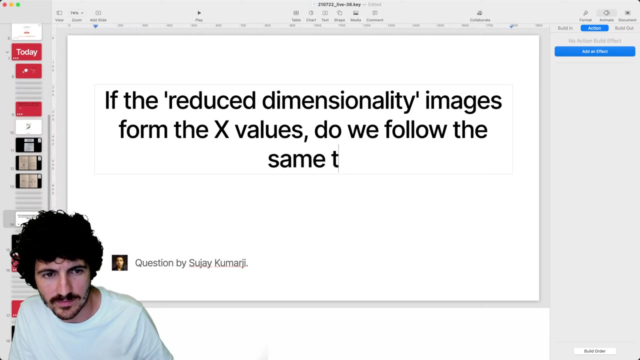 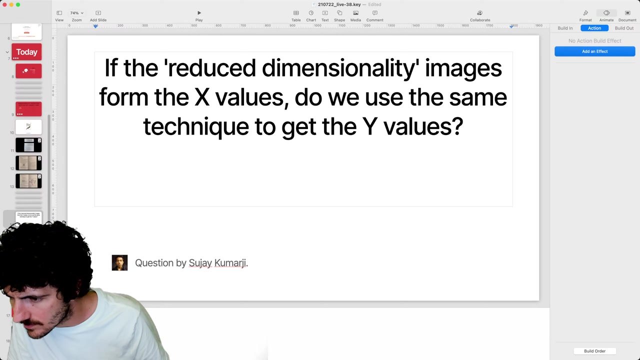 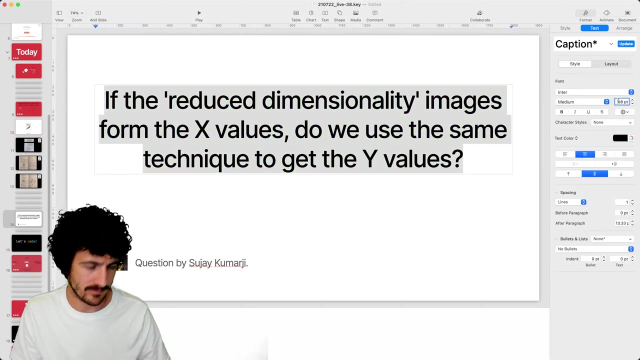 reduce dimensionality. images form the X value of, like the X bar. Well, yeah, let's do the X values. Do we follow the same? Do we use the same technique to get the Y values? Yeah, All right, There is a bit of a family's understanding or like a like, maybe lack of clarity. 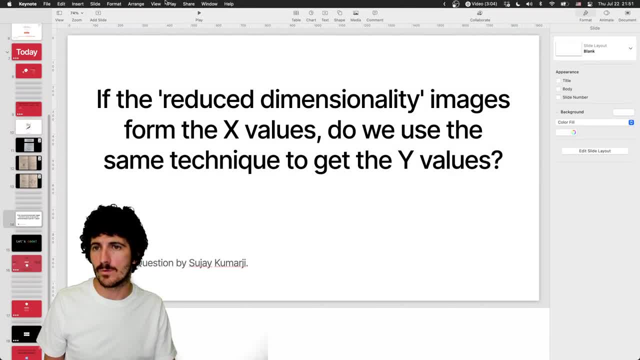 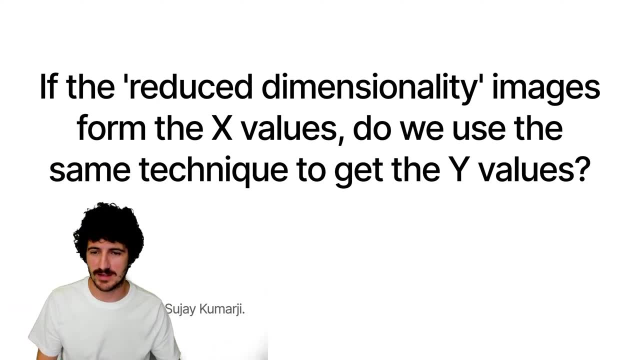 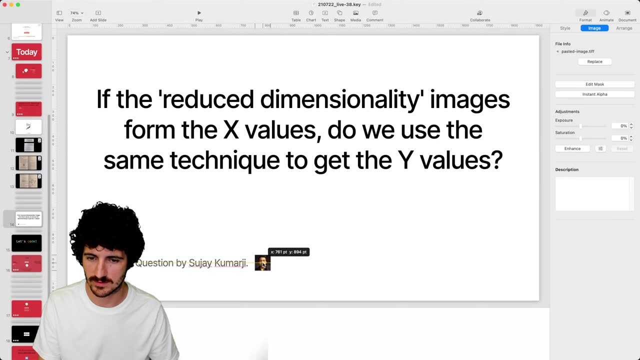 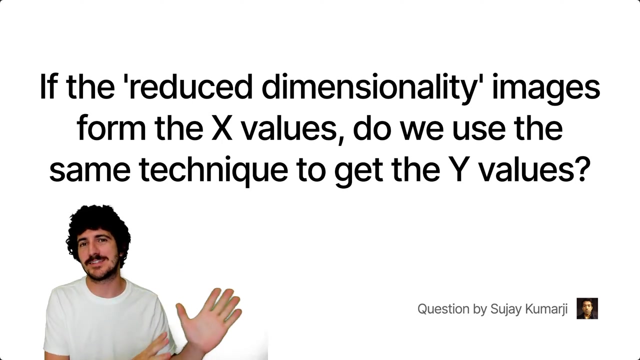 that I that I explained here. So, okay, Just trying to reiterate the question and maybe, maybe I need To move this, Okay. So, looking at this question: if the reduce dimensionality images from the X values, do we use the same technique to get the Y values? 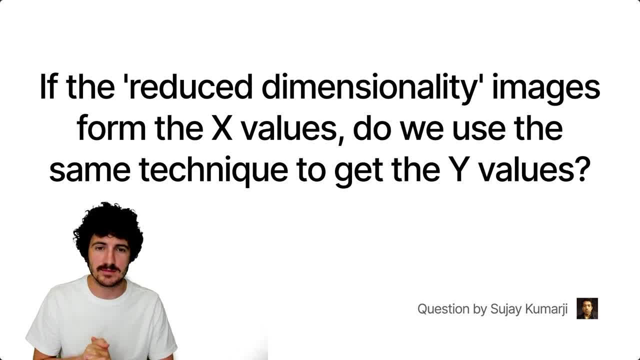 So I don't think. so we're not getting the Y values. There are two Y values that we're mentioning here in. in the In stacked out on coder world, There is one X value and one Y value, and in any other neural network we're using 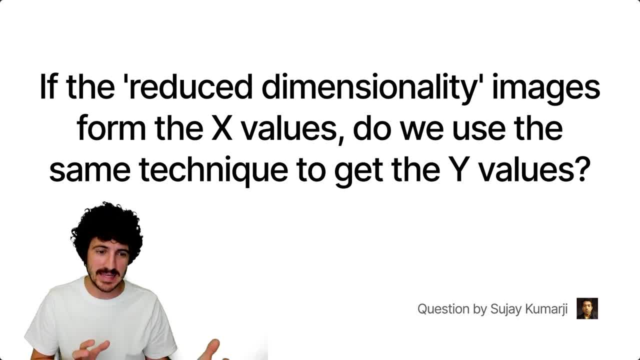 Yeah, Yeah, Um yeah, a neural network that we're using for training and then later in the These knee dimension ID reduction algorithm. There's also X and Y. The first ones that come from the fashion MNIST dataset are the X and Y values. 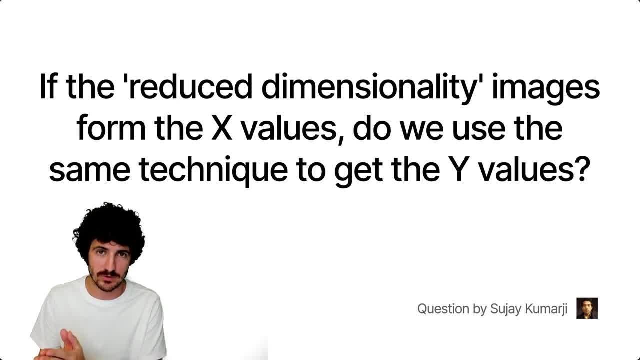 from the inputs to a training neural network and the outputs when they're classified right. So if you input a shoe, maybe the class is number five. If you input a shirt, maybe class is number eight. So you have inputs or images and outputs are the classified images in the specific. 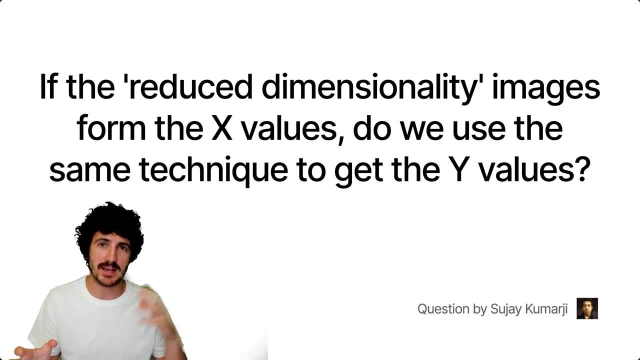 case of stacked out encoders, we're inputting the image and outputting the image. That's why, throughout the workshop, we didn't use the Y values. We were using the Y values as the colors for which to plot the data with. 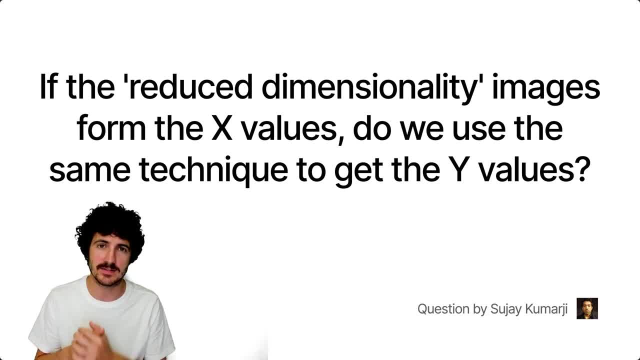 Right, And that's sort of like a validation that the Disney dimension ID reduction and the coatings with the stacked out encoders that we're obtaining make sense for these data set. right That they're actually being distributed by similarity. Disney is only reducing those 30 digits to two dimensions, right? 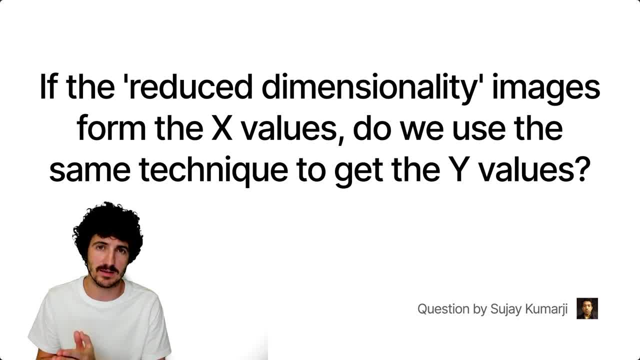 So those 30 digits already represent similarity. If we could sort those um 30 digit coatings by similarity in a row, right To the human eye they wouldn't make sense, but if we plot the images they would. What? 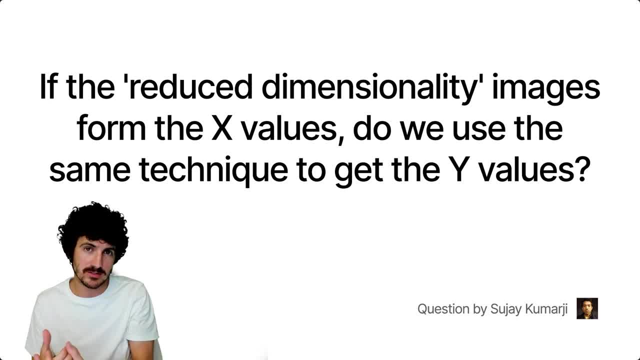 Uh, Disney does is that instead of having 30 dimensions, so they're not visible to the human eye, you go and try to plot them right, So you squeeze those 30 digits, So 30 dimensional um space, into a 2d space which is X and Y. 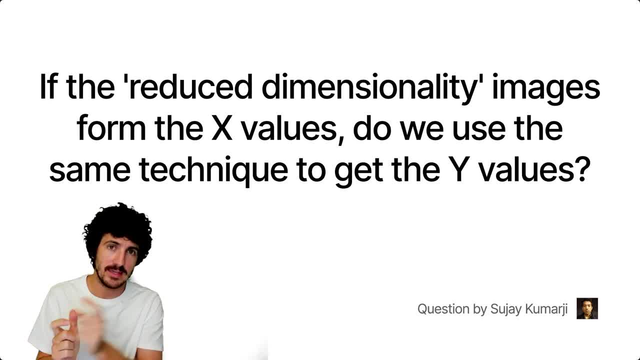 So we get those 30 numbers from the coatings into 2d, that is X and Y. So the same method brings the coatings from 30 digits to two digits, that is X and Y. the X train that we named before are the images. We don't have anything to do with a T-SNE um dimension ID reduction algorithm. 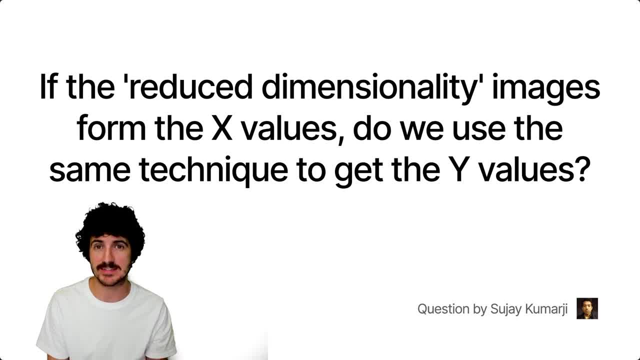 And the Y values that we were mentioning before, where the categories of the data samples that we were plotting. that only served, as I mentioned before, to color the dots for each of the individual samples. in the case of the fashion MNIST right, the data set is really segmented into shoes um shirts. 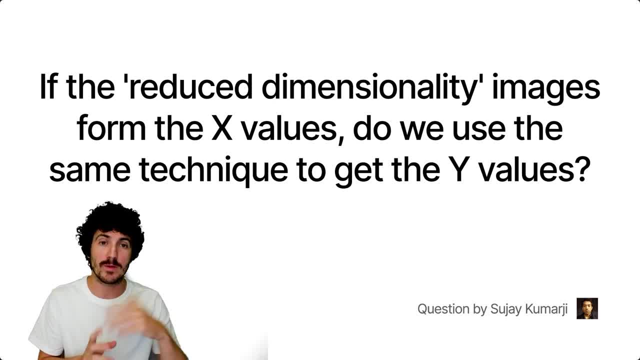 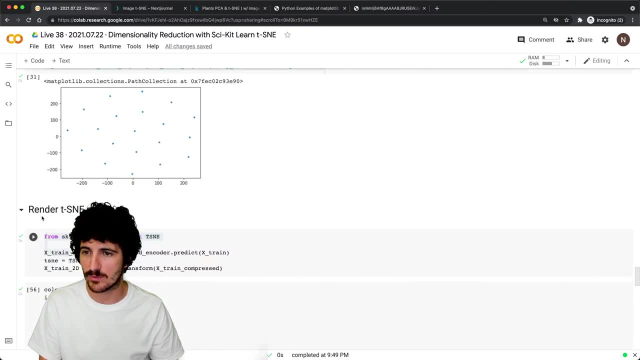 uh, boots and and many other things, And then when we plot them as we saw before, we can actually see that the um, that the actual classes that are being rendered right, They- if I go here and scroll up uh w- we don't have it right now, but we saw. 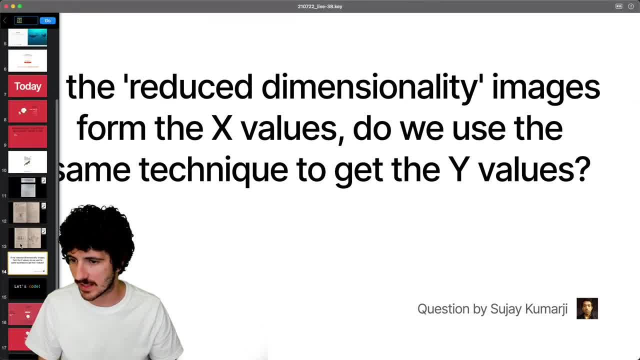 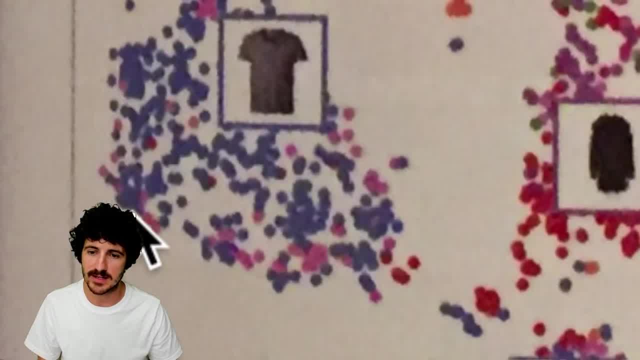 it before, where the um, the classes, actually match more or less the colors, Right, But you can see that it's not exact, right? They're like colors, Right, Right? Colors here, like the blue and the pink, only, uh, correspond to shirt or 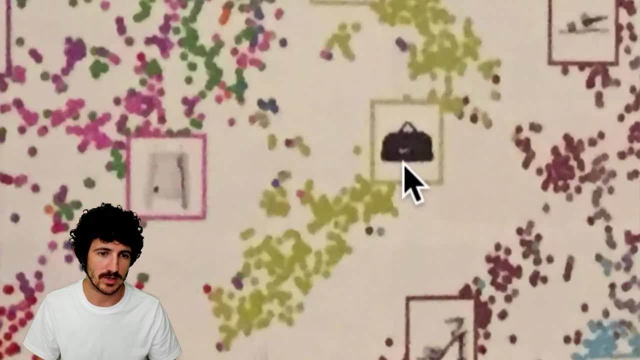 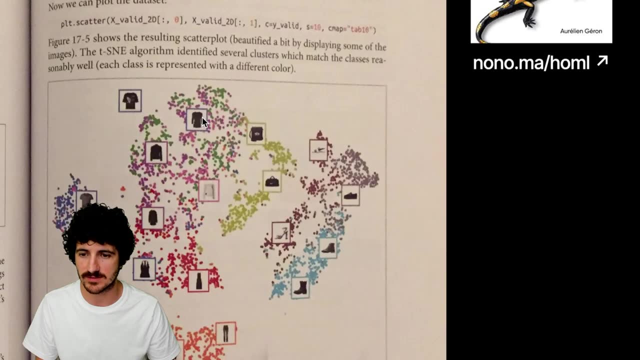 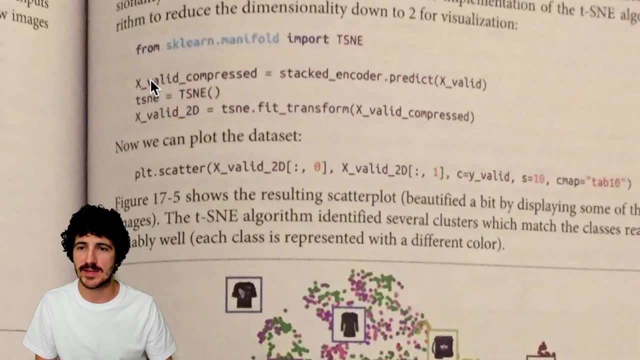 um, I think maybe these other type of shirt- right, We're like these green, yellow ones- are purses, uh, but still, their purses are getting mixed with these dresses, Right, So? and even here, right, So, yeah, there are two different X, uh, X and Y, right. 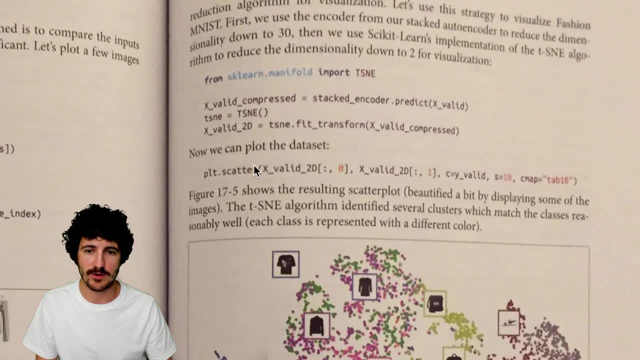 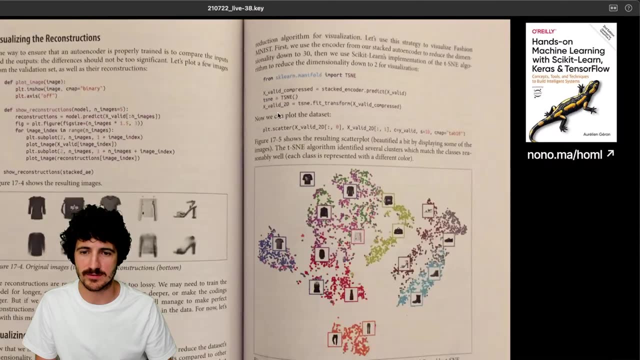 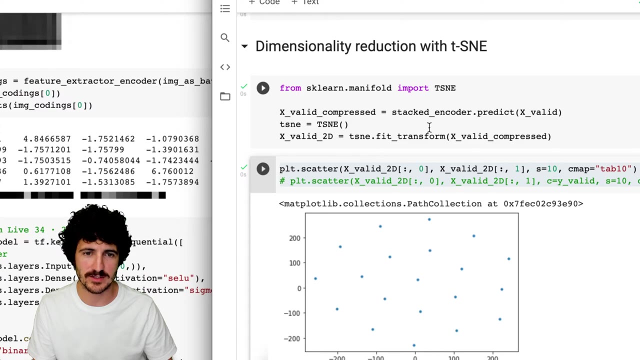 So X and these Y are different from, uh, the X and Y of the X value to be these variable here. X value to the. that we can actually see with more resolution here. Uh, it's actually, it's actually so this one here, this is actually to the values. 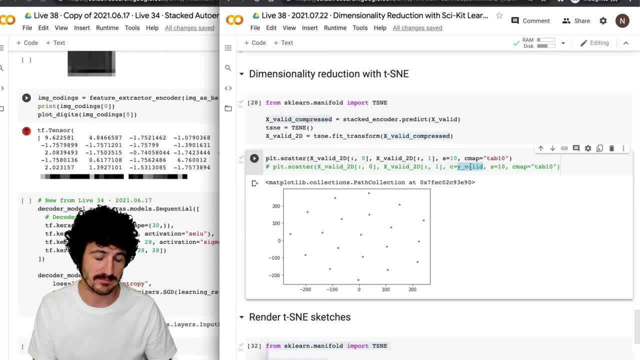 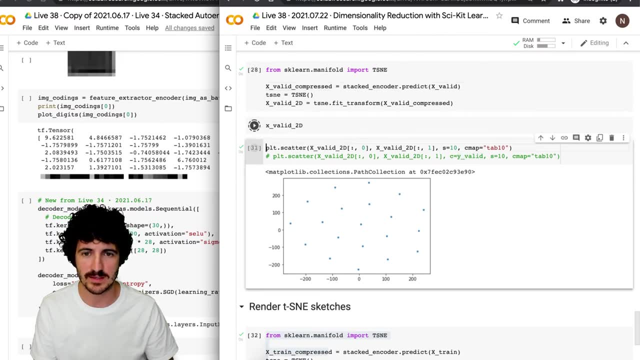 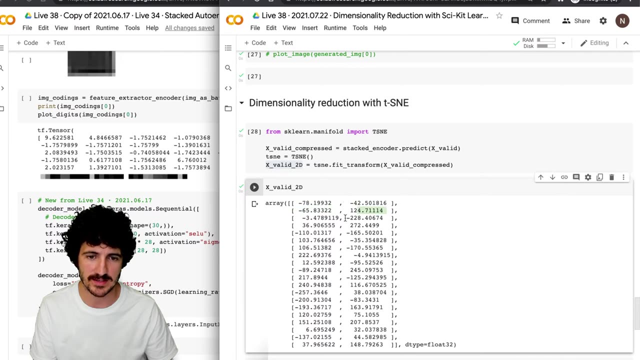 This are images and these are just labels, right? So if we plot, as we were doing before, the X valid to D, what we get is just um and the notebook. yeah, we just get X and Y, X and Y, X and Y, and that's just to plot the values. 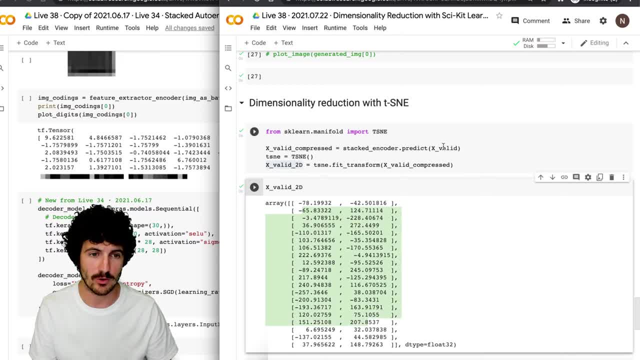 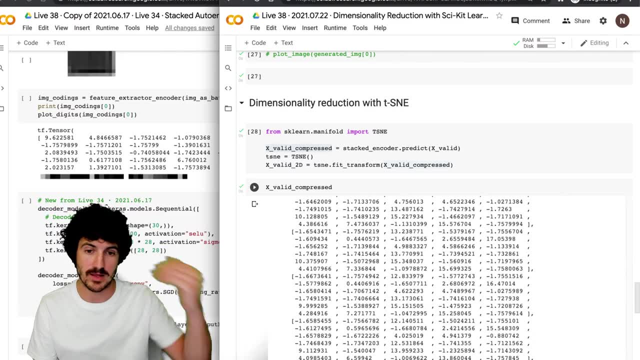 And these come from the coatings right. We've um encoded the X valid into compress, which this is like a, like an array of coatings, And if we bring this one, we're going to get like an array of 30 digit um coatings. 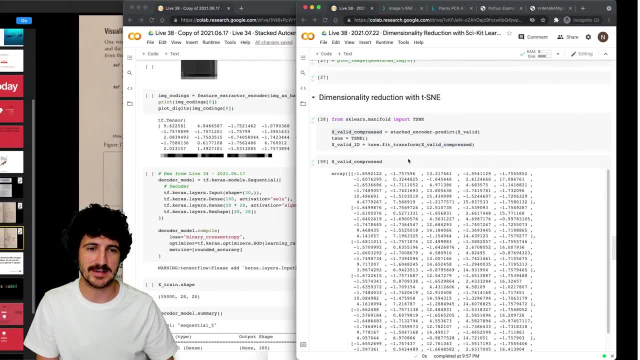 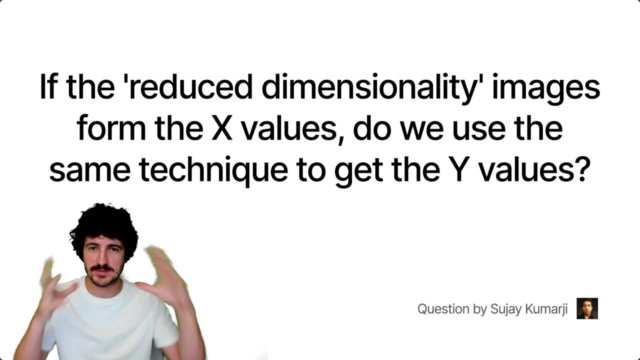 Right And yeah, so that I hope that, um, that answers suggest a question and things. Thanks a lot for asking. I think this kind of Wraps up conceptually a bit, uh, the last part of what we've done. 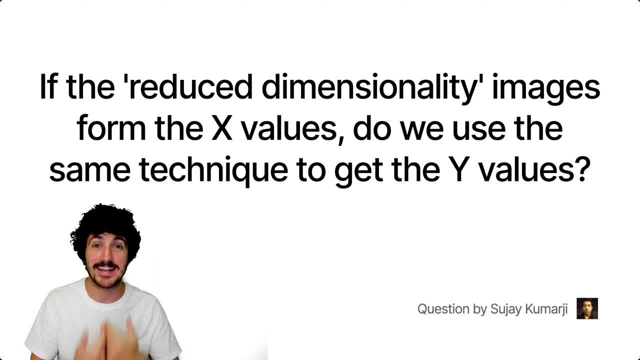 Thank you And for anyone who's watched, thanks a lot for watching and I'll see you next time. It was not a market, I don't, So here. you can check out more of the machine learning videos on my YouTube channel. All right, 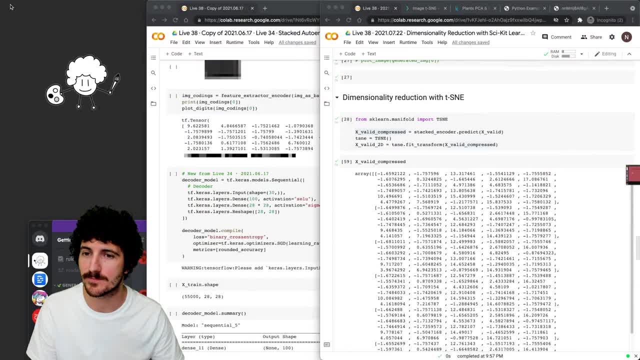 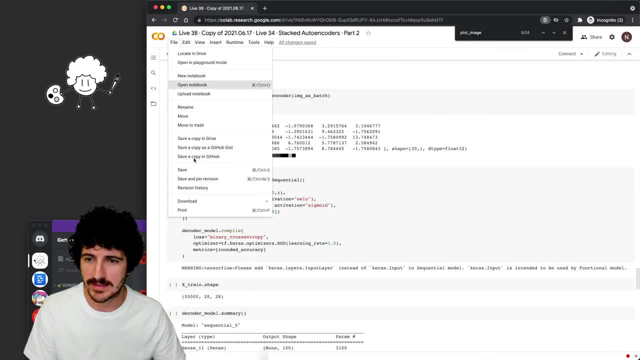 So just to wrap up, thanks for the questions. So yeah, that was super useful And, uh, the last thing that I want to do, probably I can delete this one. Can I delete this one? Move to trash, Uh. 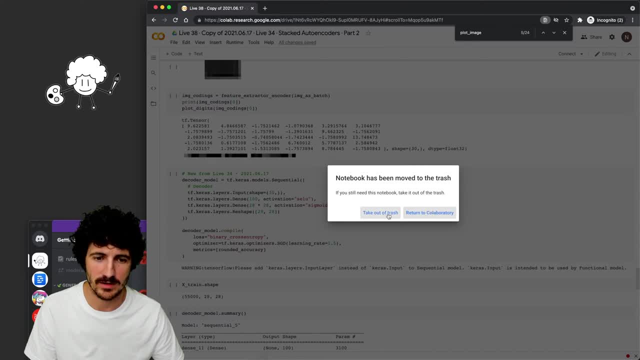 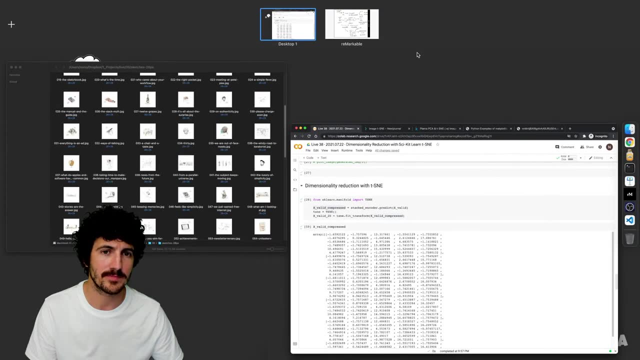 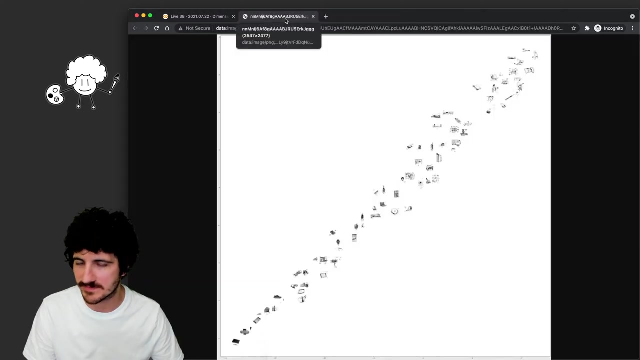 copy: Yeah, All right, So we what we want to do, and I'm going to close things here. I'm falling asleep now. Uh, we're going to close these things. Um, yeah, Thank you for the question. 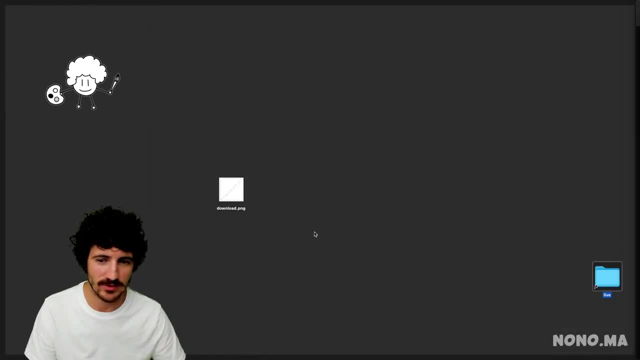 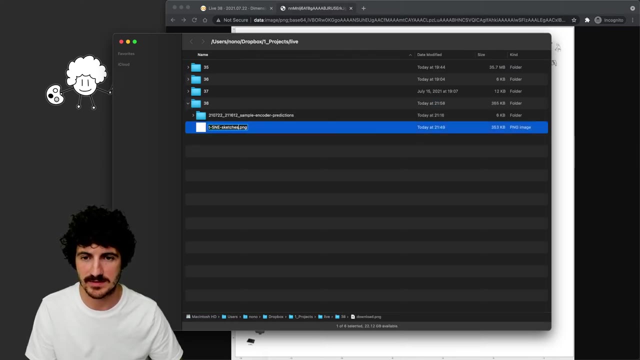 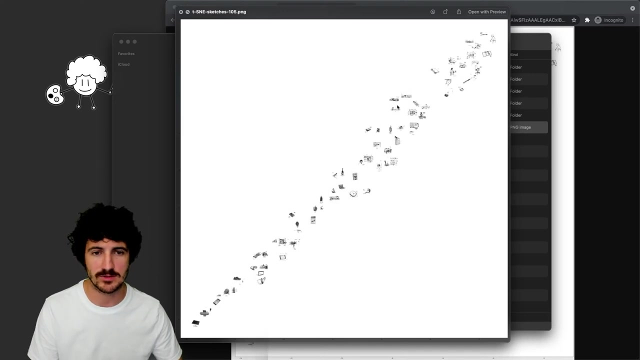 Really, That was really useful And we're going to come here to live. This is, uh, Disney sketches under five. Yeah, So that is here. And the fact that they're linear- I'm not sure that might be because they're not more dimensions to separate them, more features for the data set to learn from. 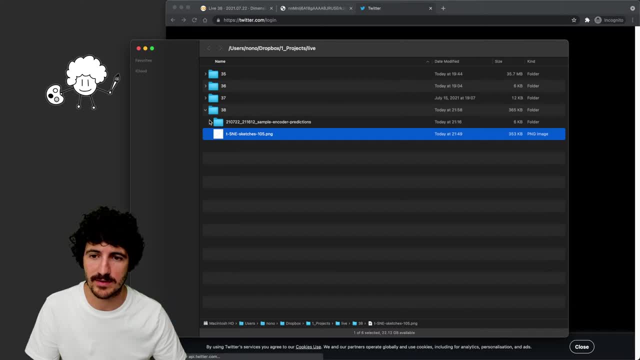 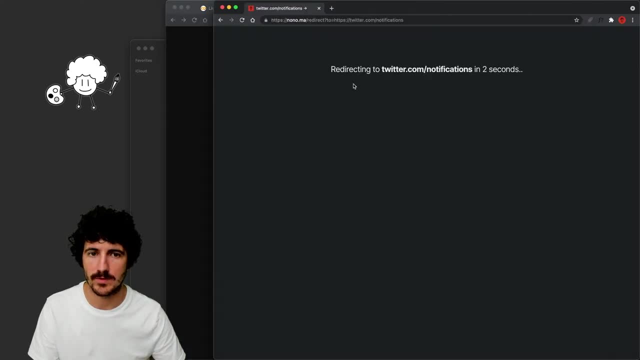 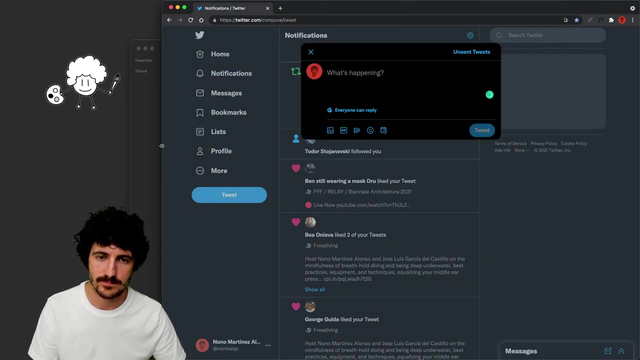 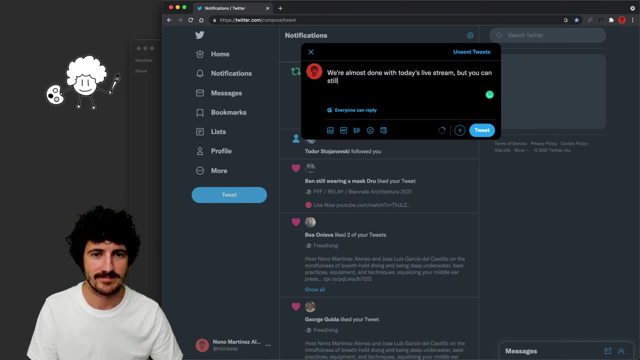 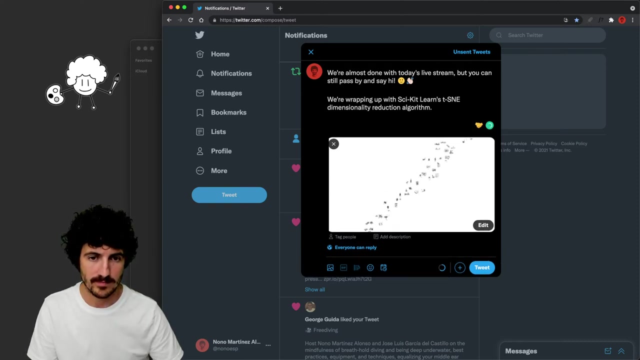 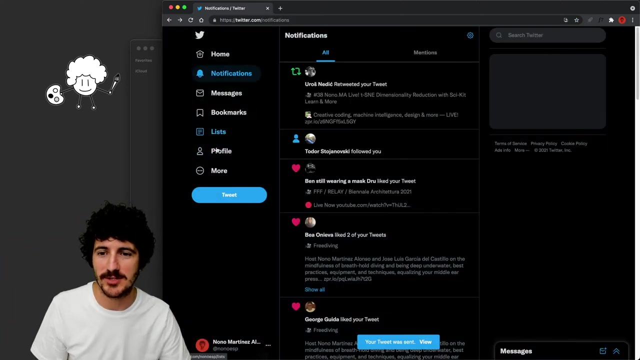 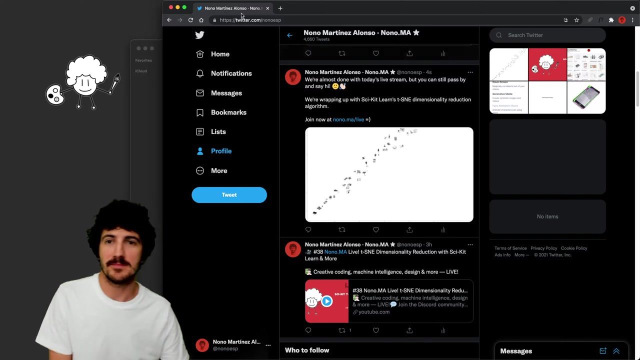 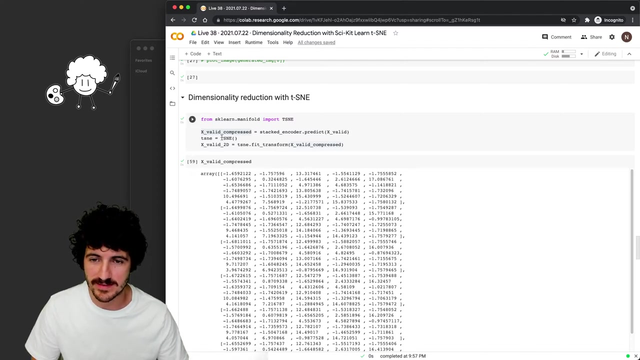 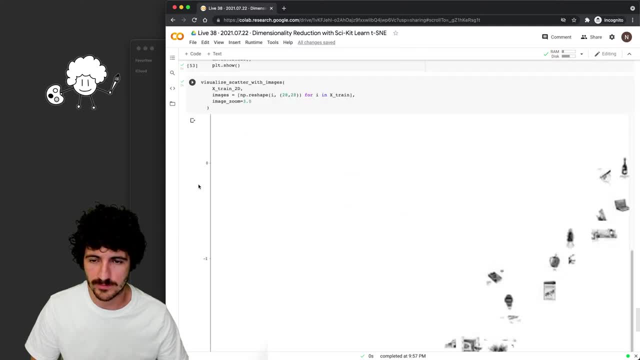 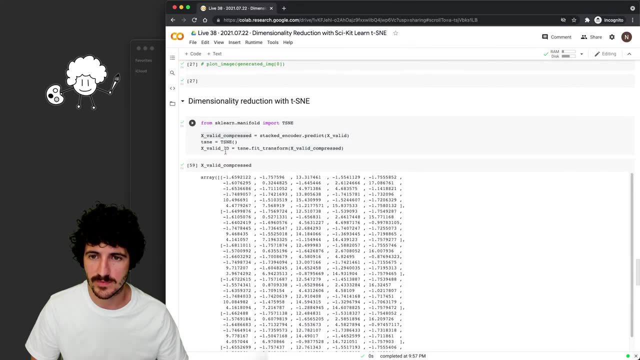 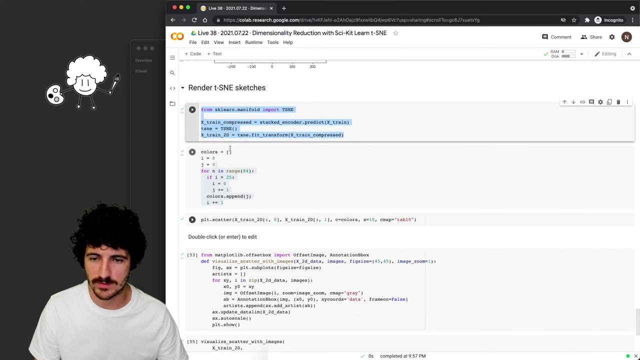 Let's see. So we're- um, we're going to close this thing, We're going to hide this as well. Reduction with Disney rendered. She's in sketches, All right. So we're just going to copy all of this, and I probably don't need the colors yet. 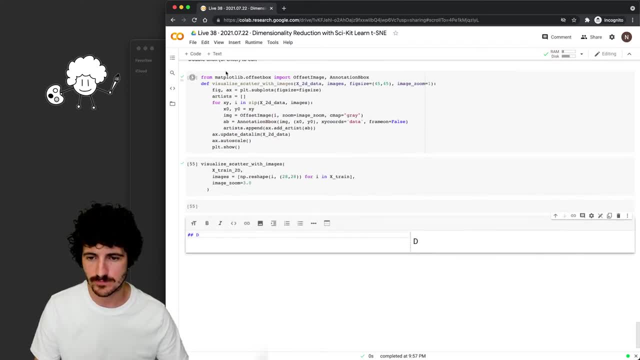 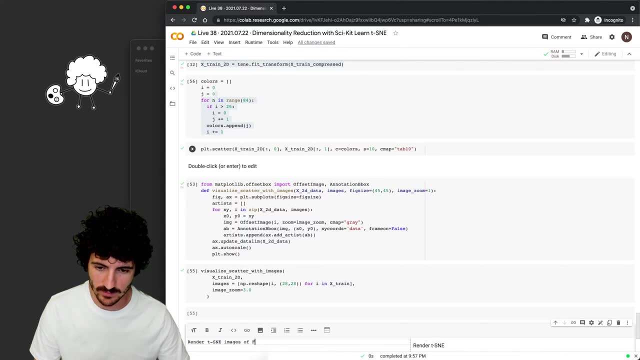 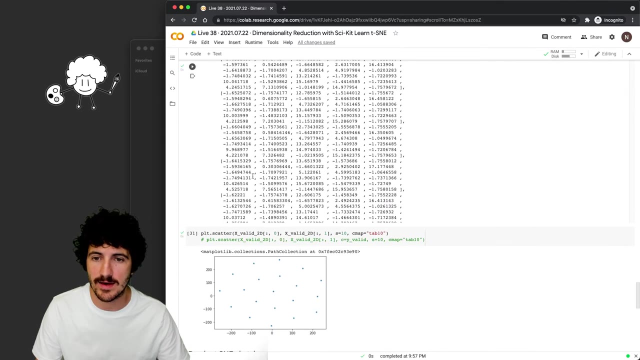 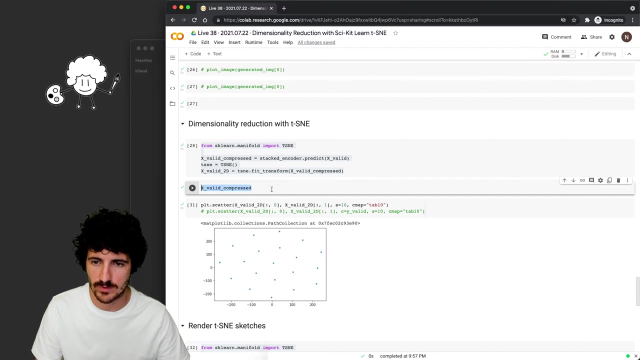 I don't think so. Um, Render Disney images of fashion MNIST. Okay, All right. So how are we going to do this? We do have up there, so I can remove this. We do have This. um, we don't really need to bring this anymore. 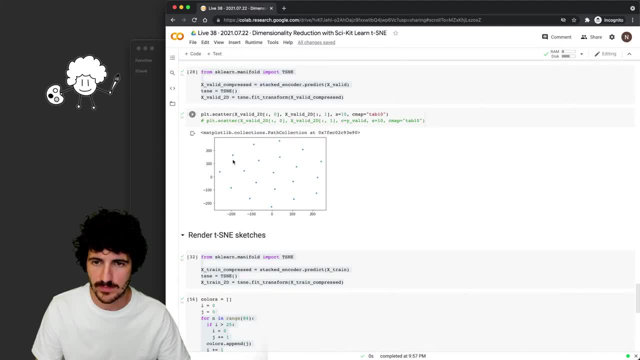 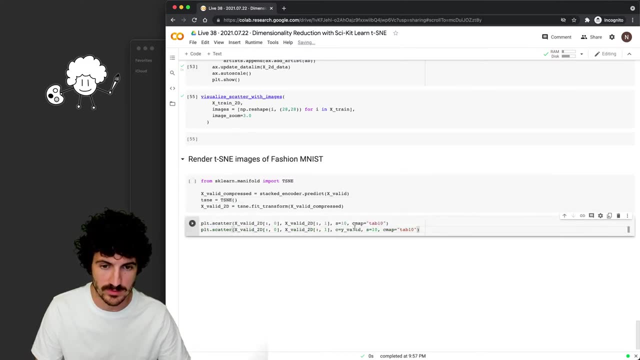 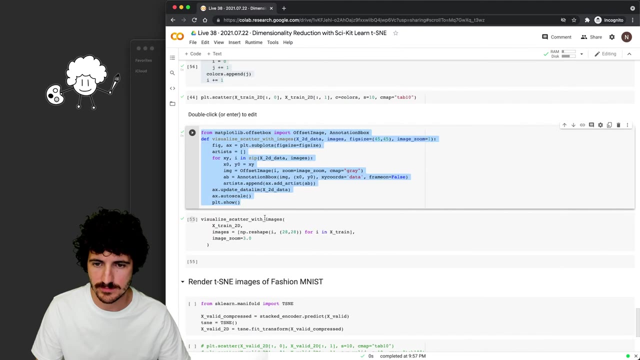 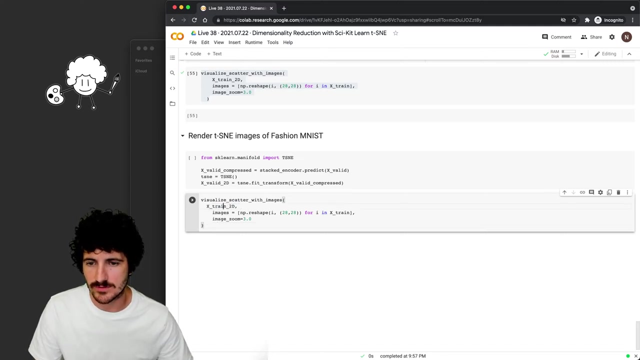 We do have this, but the here this year and we do want the colors. Um, well, we don't really need this anymore. We just need um, we just need this really. And uh X Train to the and uh, extreme. maybe we're going to have more images. 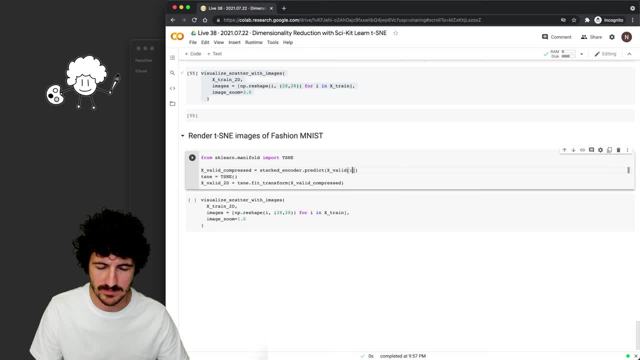 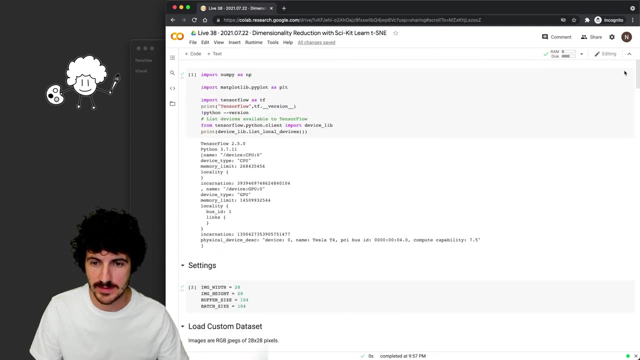 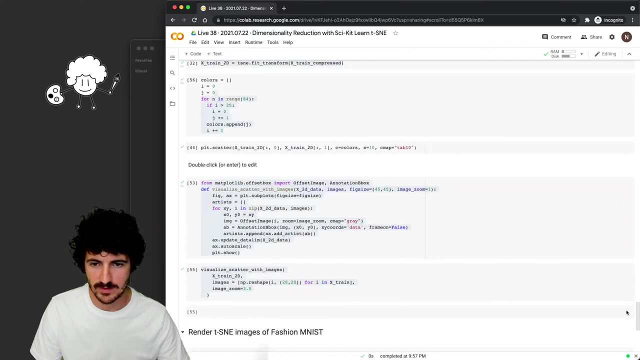 Exvalid. uh, maybe let's just pick um 500 images for now And uh, what else? we need to train the model And that's going to take a bit of time, So let's put this back. Um, we start and run off. 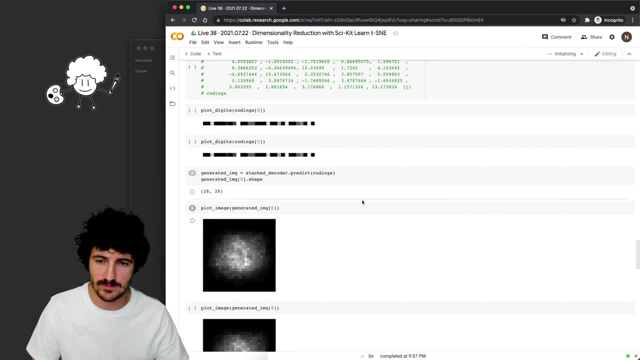 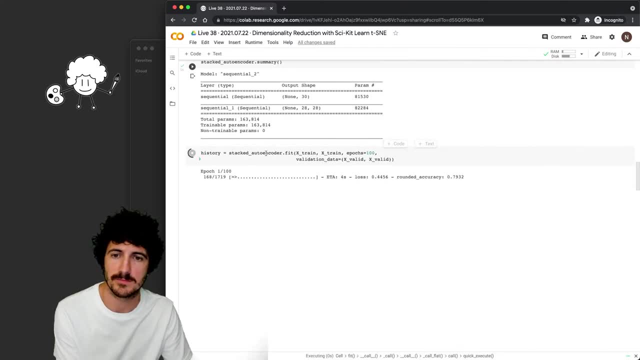 There'll be things that are not going to work, but, uh, we'll get there. And these- probably the thing that's going to take the longest- is going to be training, which we're going to take like maybe 10 or 15 seconds. 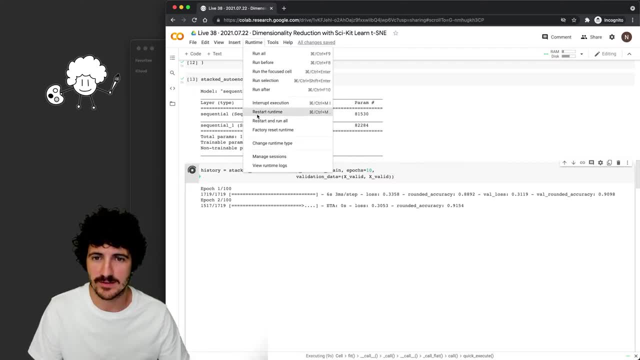 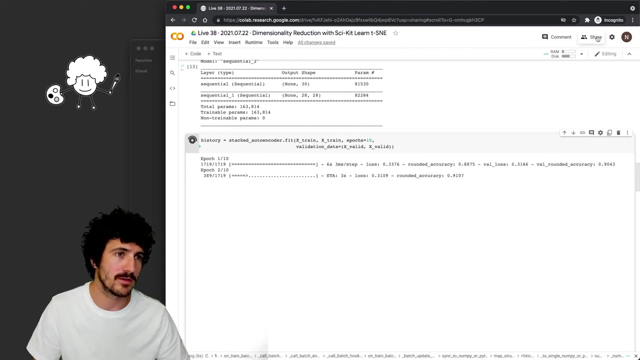 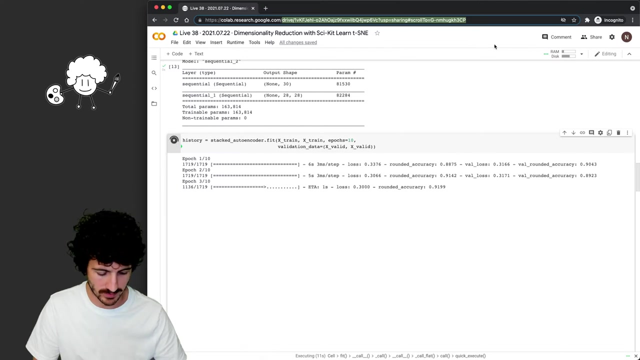 Oh, a hundred, Maybe not. No time for that. All right, So we're starting again. All right, So we're running again. I think we're still using a GPU and yeah, And as um Ricardo mentioned before, you should get a call-up pro if you're going to, if you're going to be. 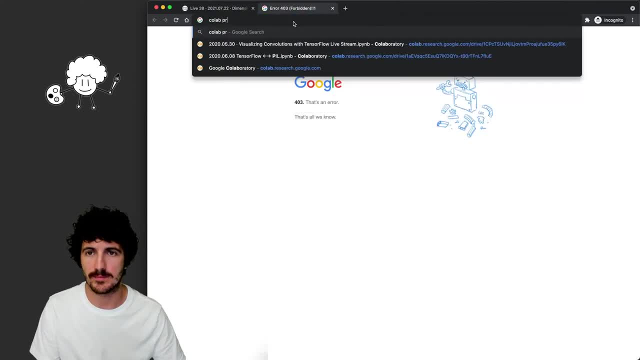 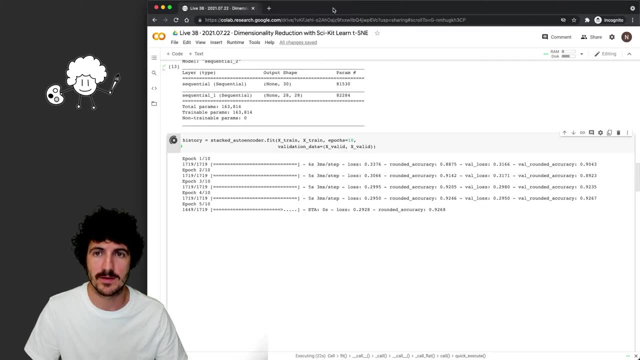 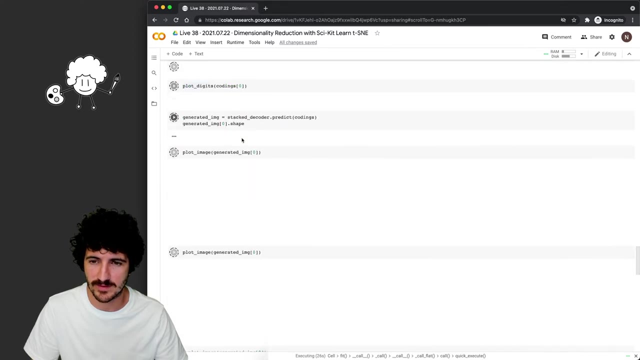 training models for long call-up pro it's like 10 bucks a month, So definitely worth it, All right. So we're training five, six out of 10.. We're almost there, All right. I'll ask for whoever is online. 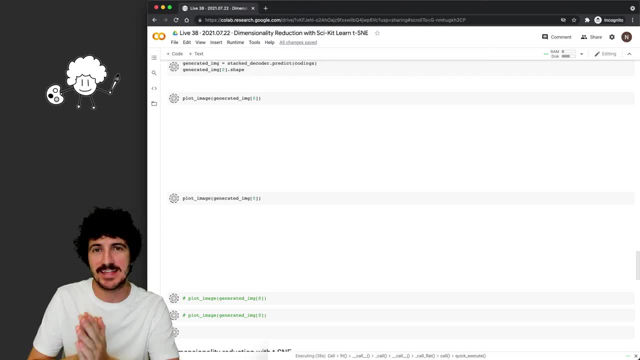 Do you want to let me know on the chat what you want to see next time? So next Thursday we are not going to have live streams. On August, or the most part, I don't think we'll have any. So next week is maybe going to be the last one, unless I do others during the week. 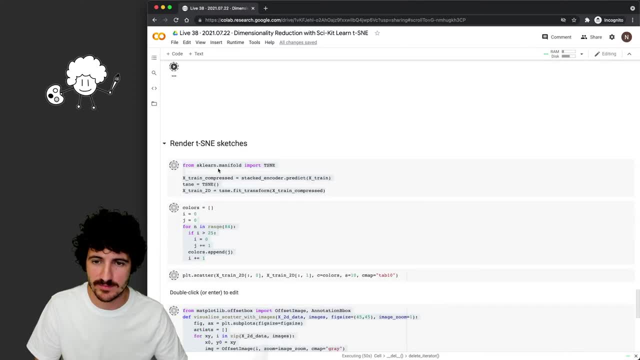 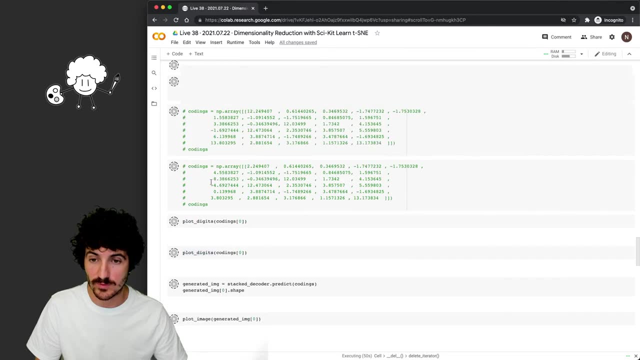 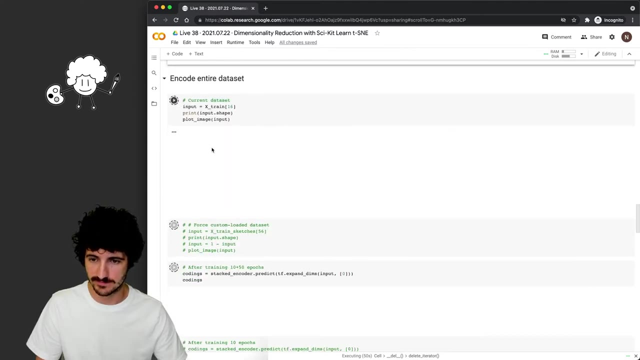 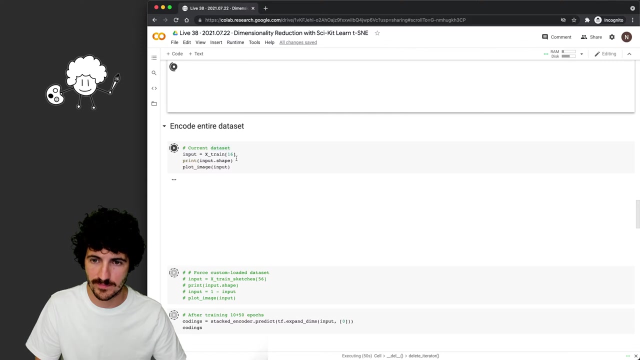 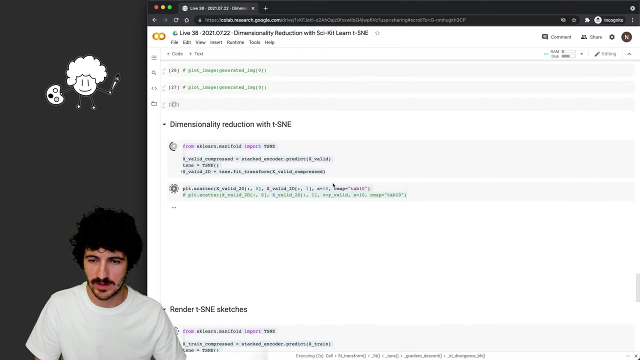 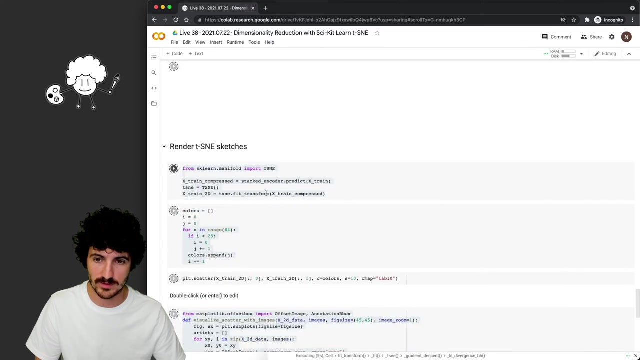 So, yeah, Let me know, Let me know. All right, So we should be now done with training. We are, Hmm, Great, And we probably going to see some error below, but let's see, Well, probably not, Oh yeah. 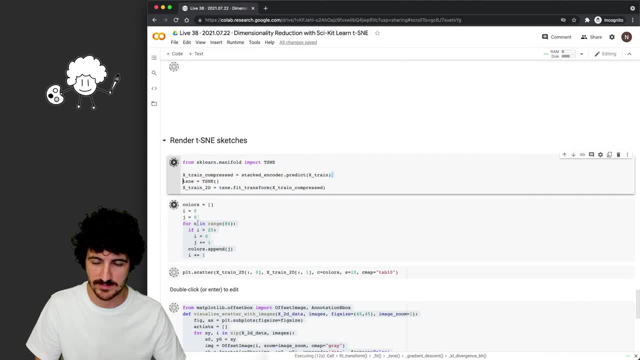 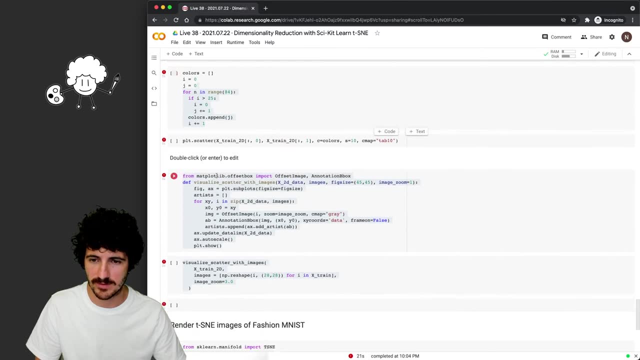 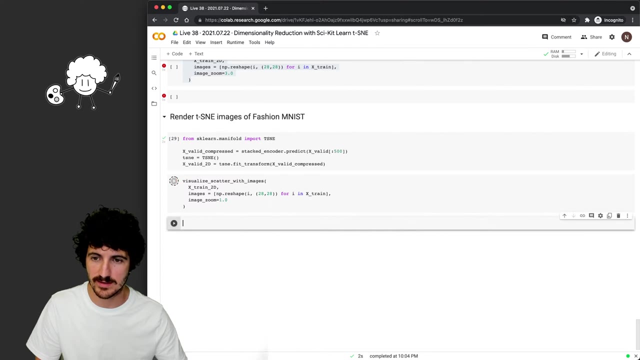 I don't think this is going to get completed. This is too much to be plotted. Okay, All right. All right, So I'm going to interrupt that one because, uh, where I want to really get is here. So we do that and then visualize. 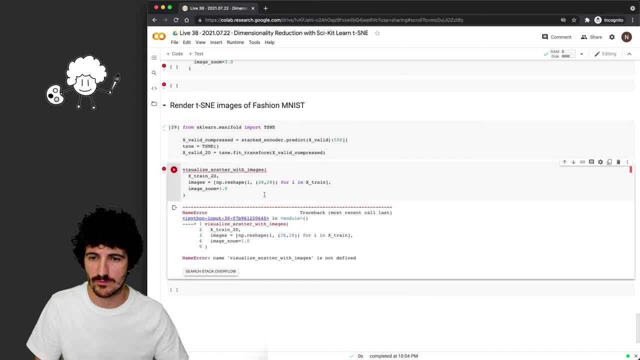 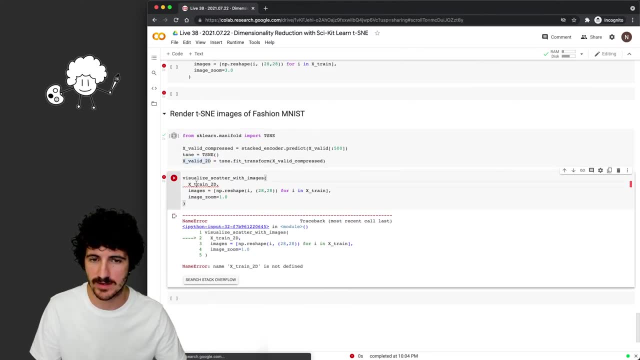 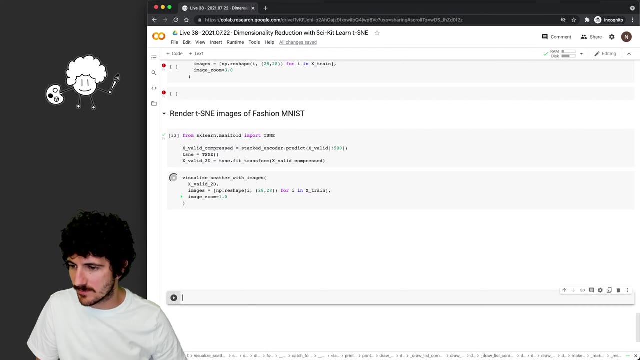 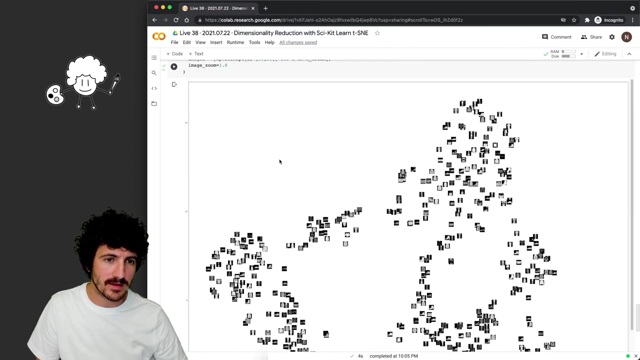 Okay, And we run this helper and then we run the cell once again: X train to the X valley, to the all right, Whatever, All right. And yeah, we should now get an image generated Here. Great, And maybe it's, maybe. 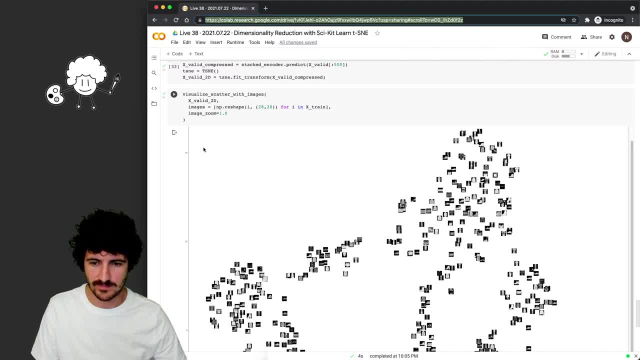 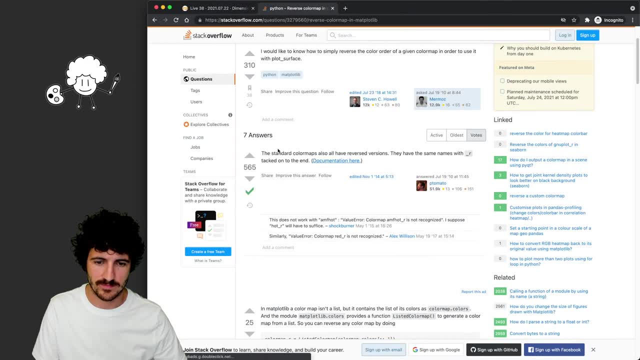 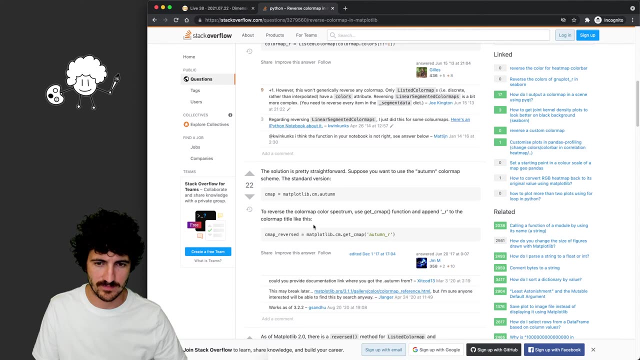 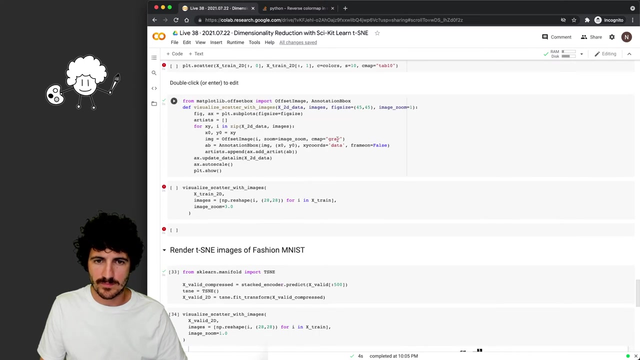 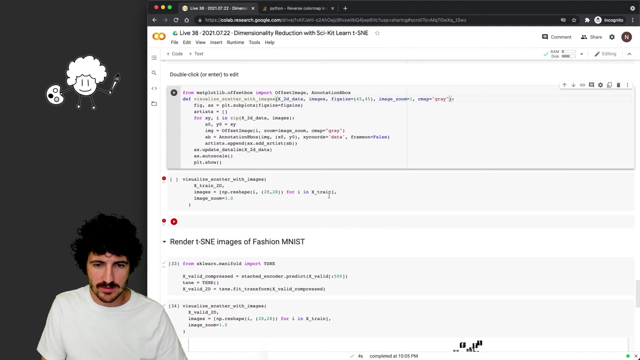 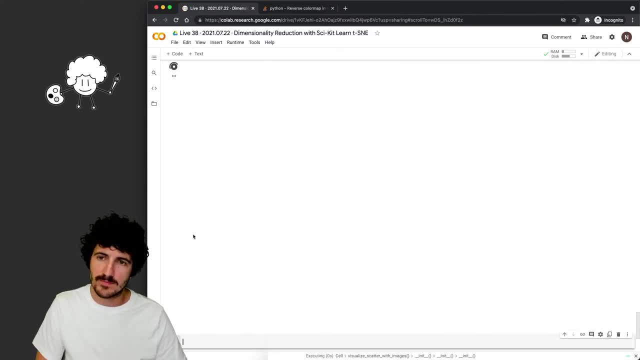 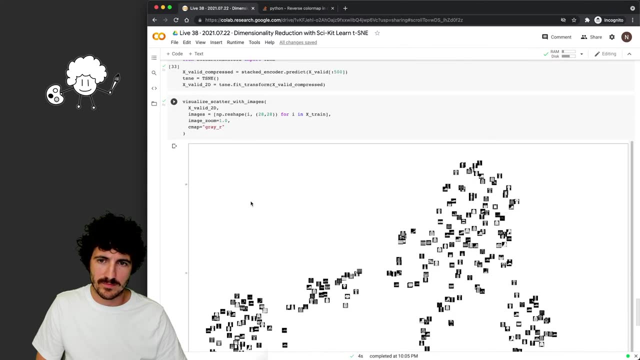 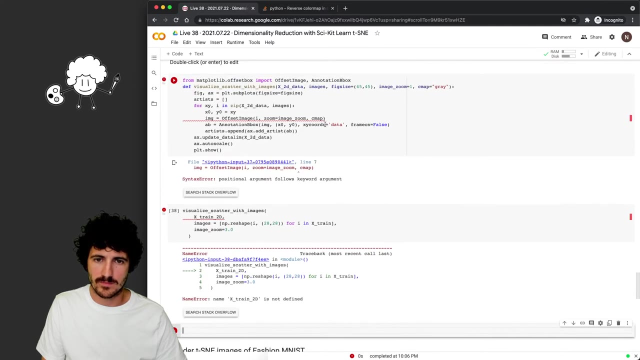 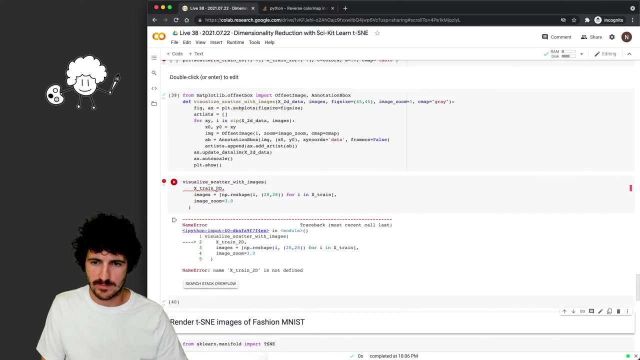 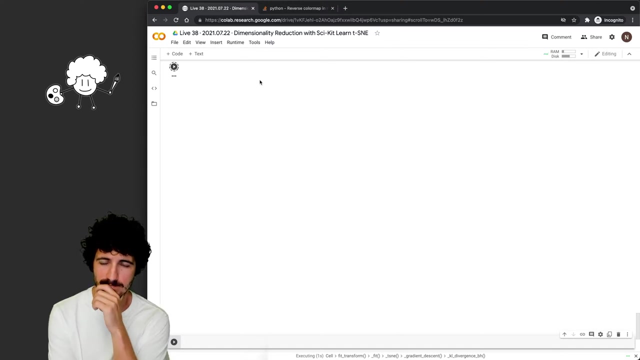 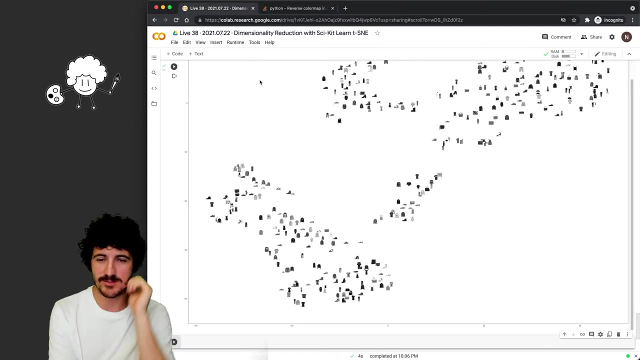 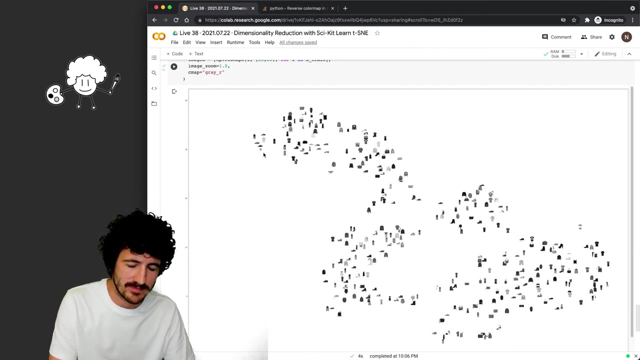 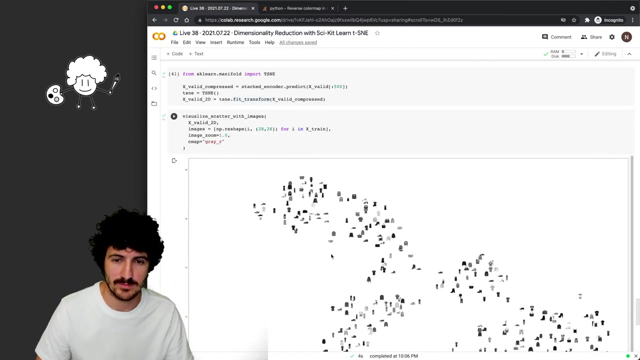 See, my gray are Awesome. Great, This is indeed a pretty pretty cool Okay. What this tells me is that you know, we haven't trained for long enough, Probably. Um, I'm going to get more samples, so I'm going to take 2,500. 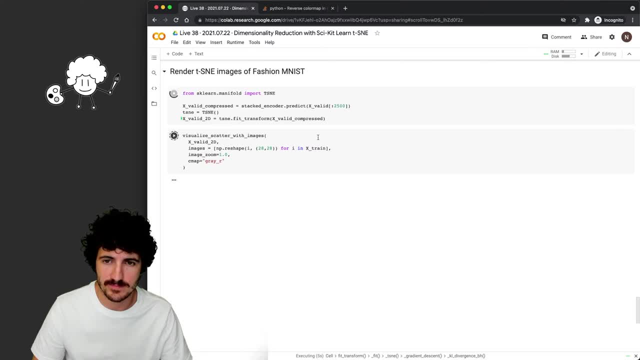 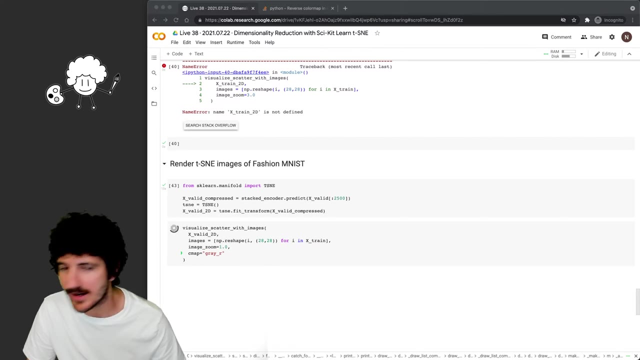 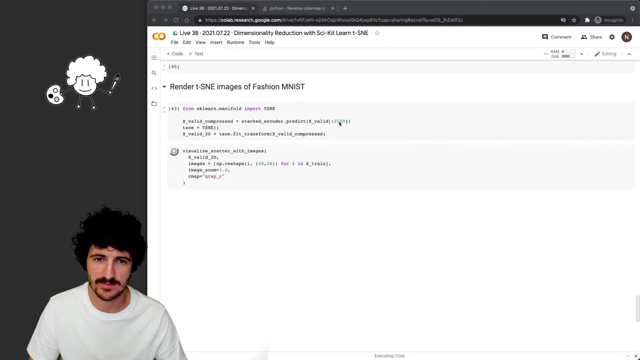 Uh, but yeah. so, uh, we can train for longer. It's already really late. I don't know for how long we've been going. 30 hours, Okay. So let's see, Maybe it's a bit too much. 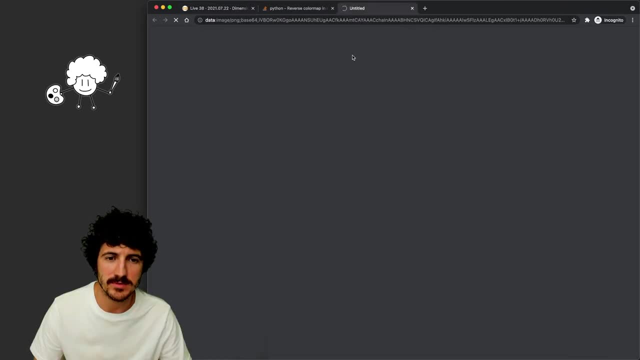 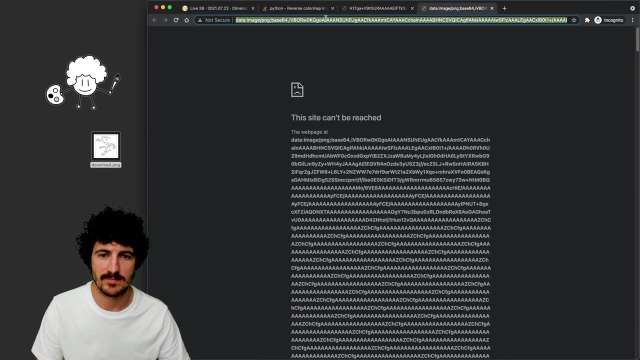 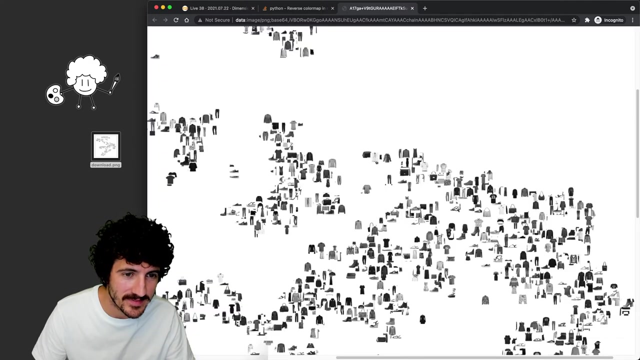 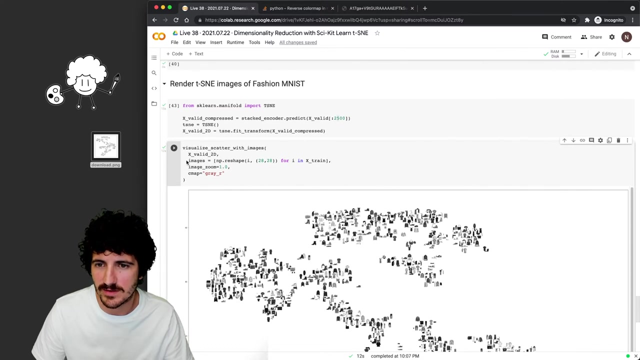 Okay, No works. That's a cool image, right? I don't think these ones are similar. Not sure if we're doing anything wrong here. Let me see if there's anything. So X valid- X valid. fixed valid. compressed X valid. 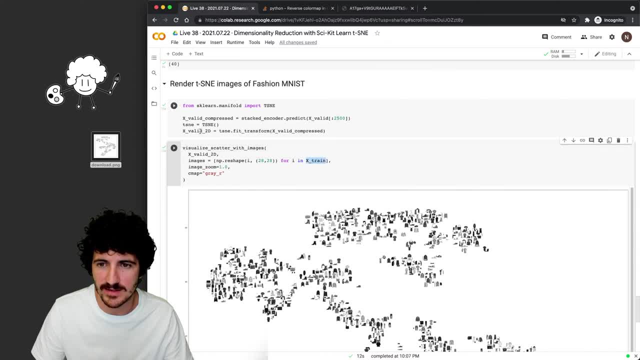 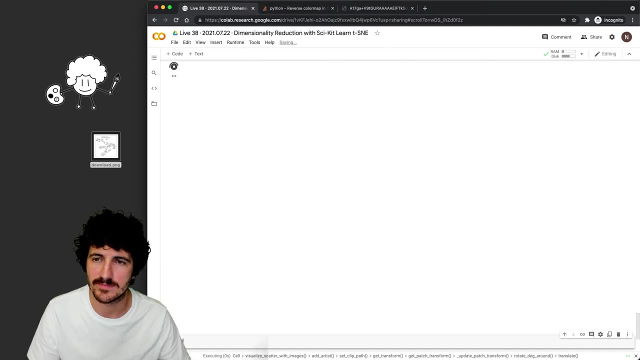 It X Train. All right, X valid Images. Okay, So we're X valid to 500.. Right, Right, Let's see. Yeah, this is like looks wrong, Definitely, Okay, Okay, Okay, Okay. 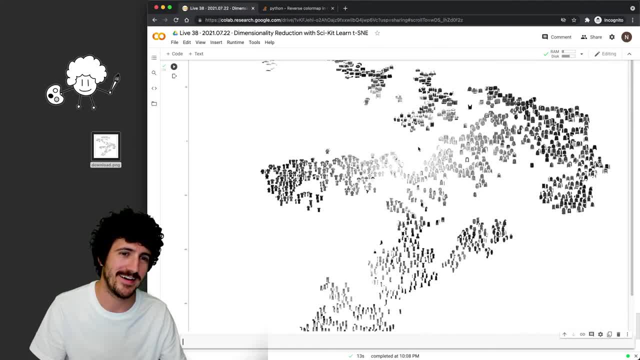 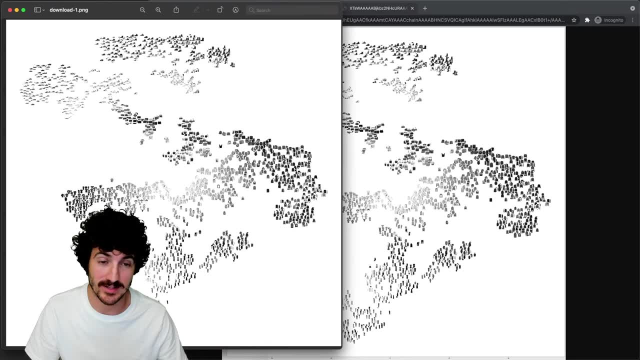 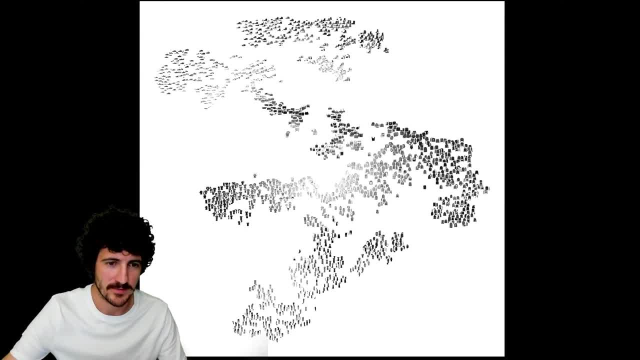 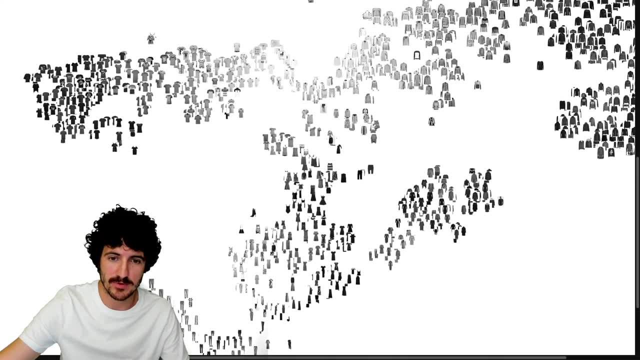 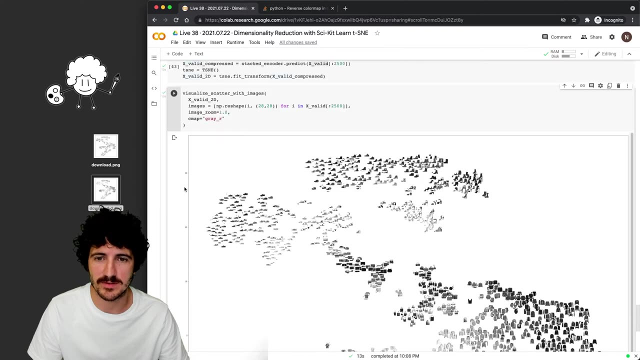 This is something more similar to what Ricardo was showing before. So this is awesome That just with 10, um, 10 epochs, these looks so good, Okay, So let's prioritize this then, because this may we can do even better. 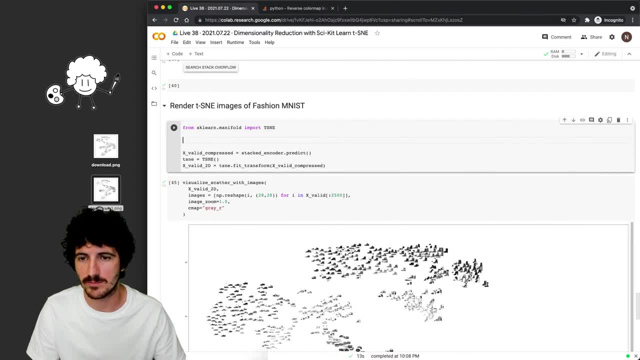 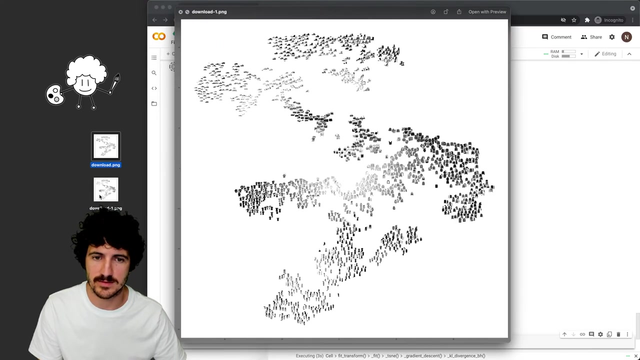 So we'll do: Uh, input is going to be this and we'll just predict on the input. Um, maybe just put the inputs All right. So, um, what do you want to do? Okay, I'm going to generate this just to make sure that we're getting the same. 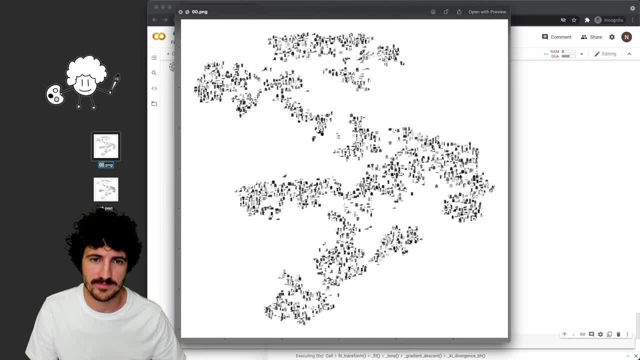 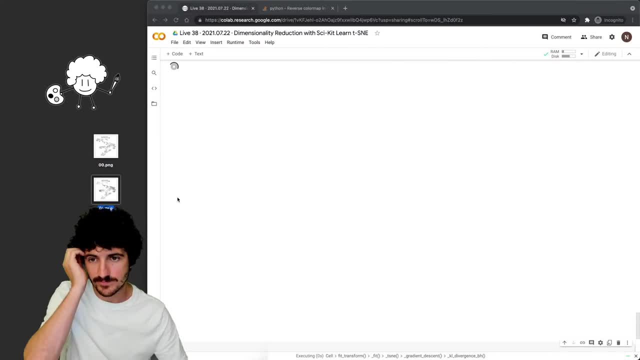 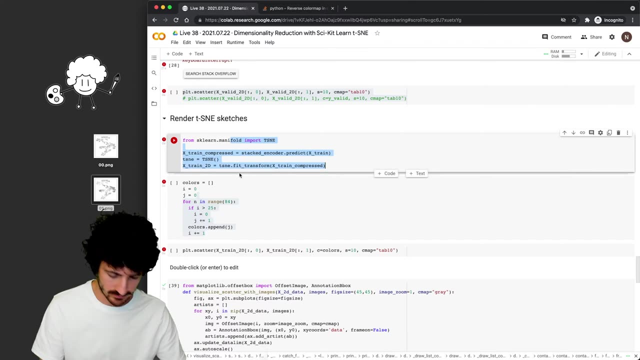 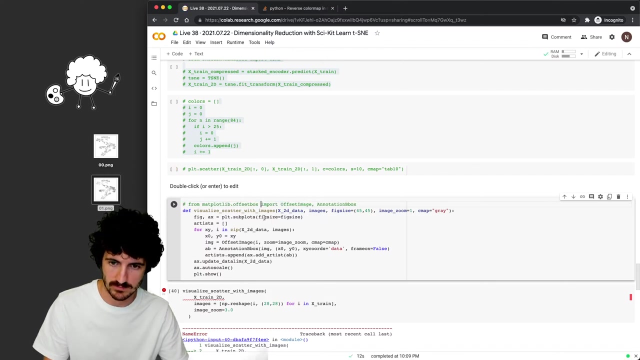 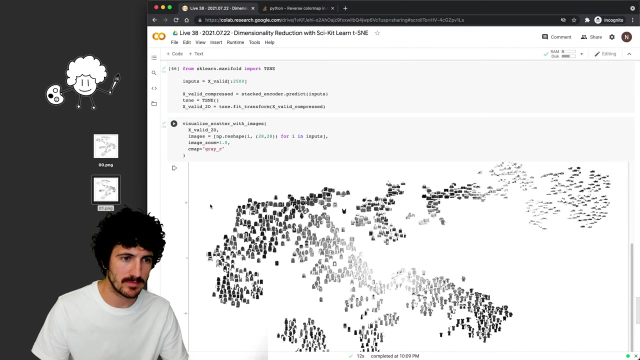 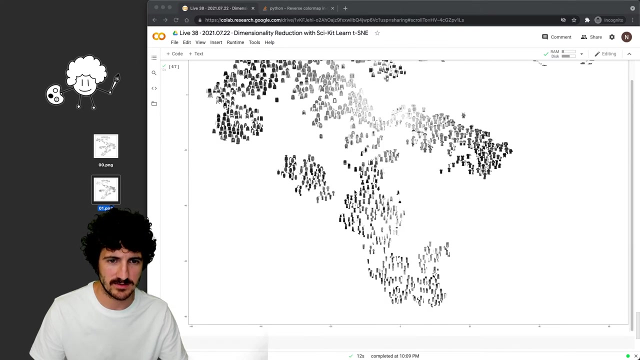 So zero, zero, zero one, And uh, what we're going to do right now is I'm going to close this thing. So comment this out: This is being plotted, which is pretty cool. This has not changed. I'm sure why it changed. 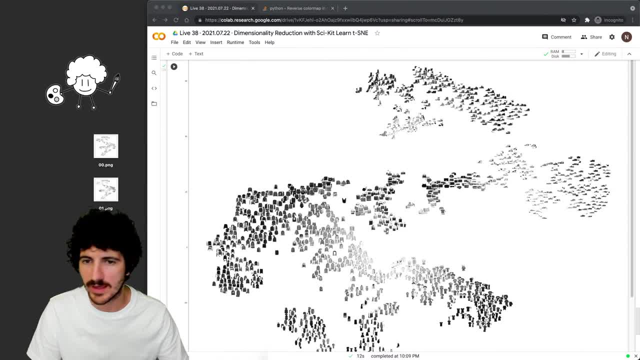 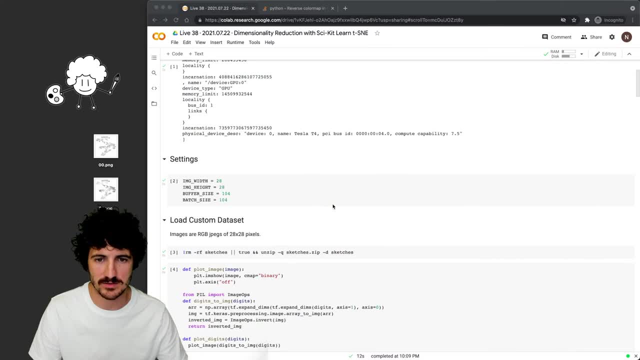 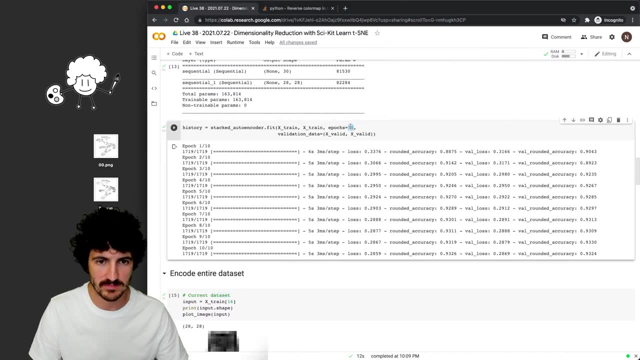 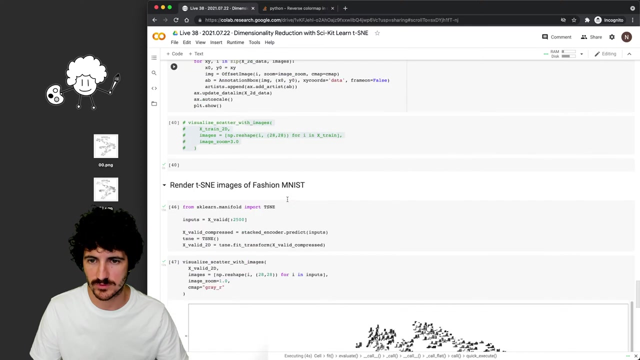 For some weird reason And, um, we're just going to train for longer just to see how that image actually changes, how this works, Sorting changes. So we're going to train here for 20 epochs And when we have the model trained, these will be trained, uh, for 30. 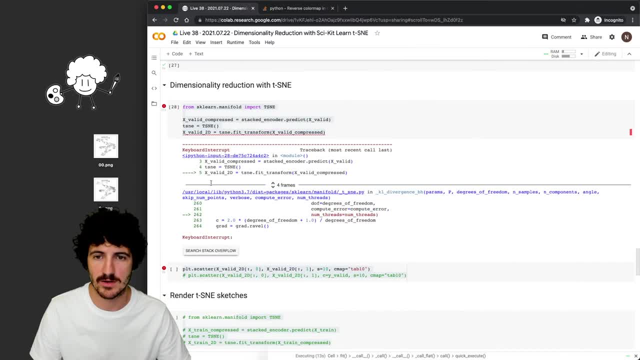 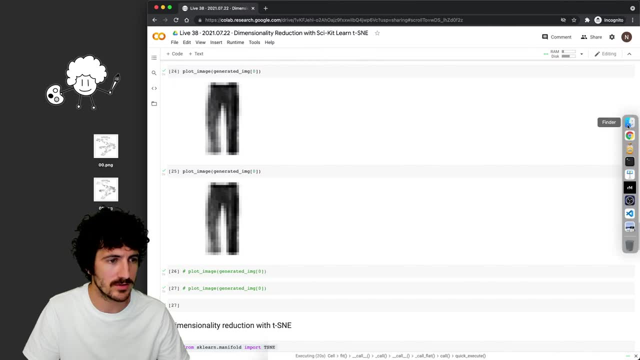 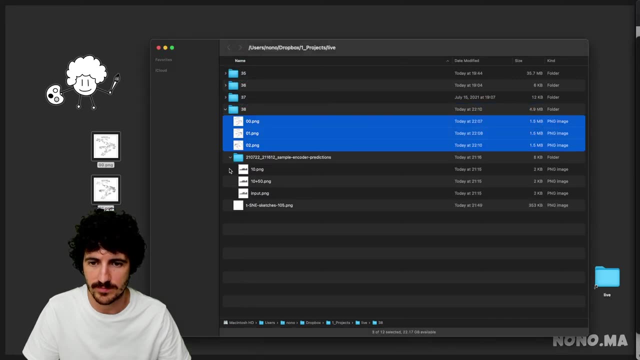 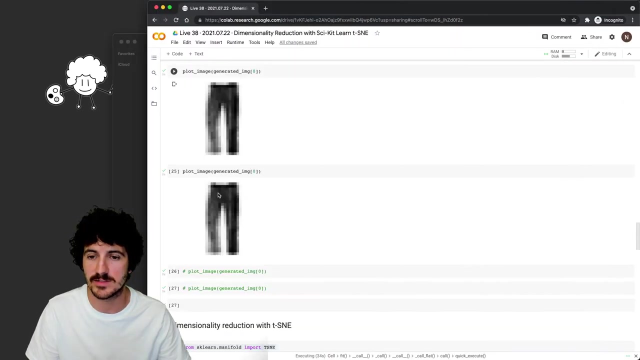 epochs total, and then we'll be able to get this thing All right. Uh, let's start archiving a bit. So we have that on this cord. This Images are going to go into today's folder. Hmm, Let's check that. the images on the other data set at also right. 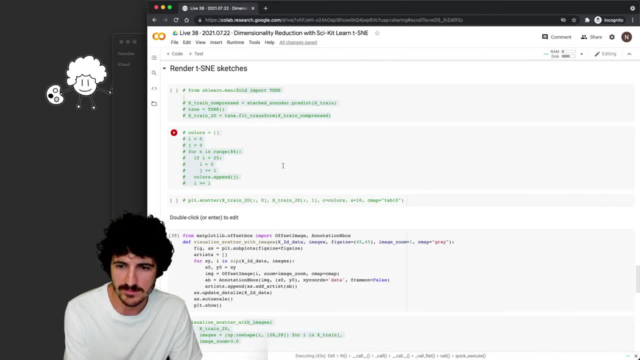 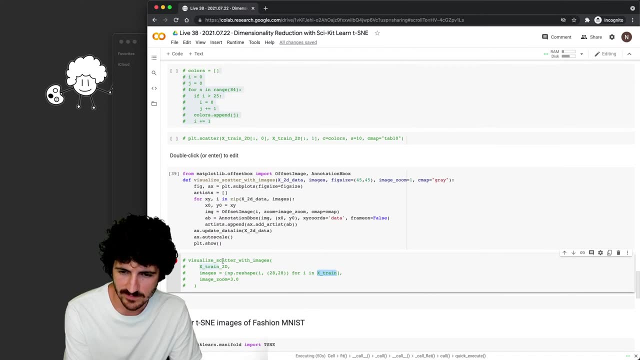 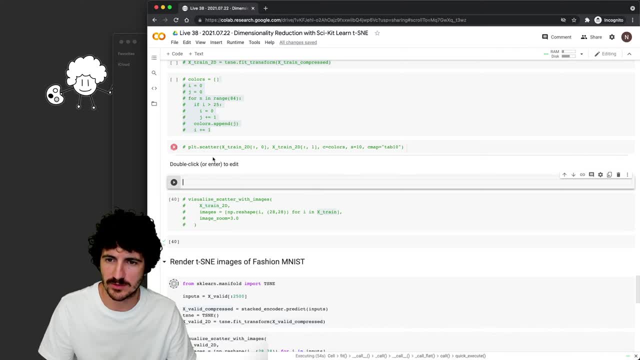 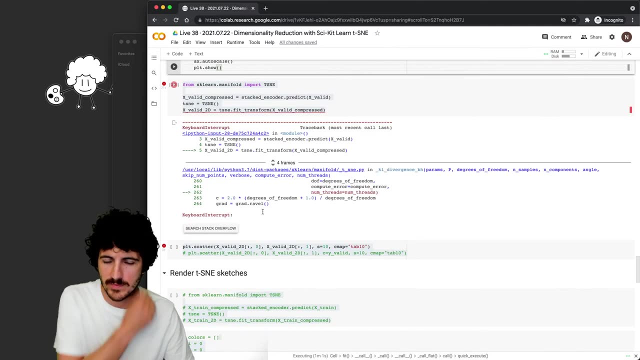 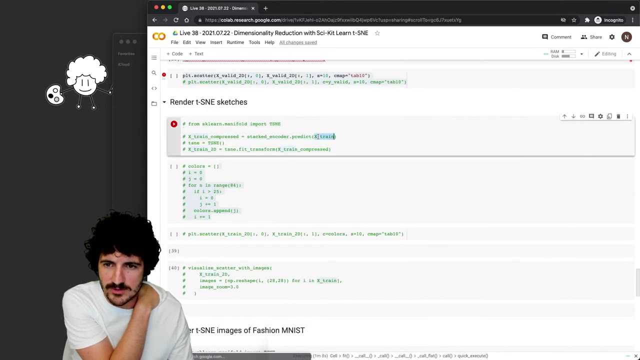 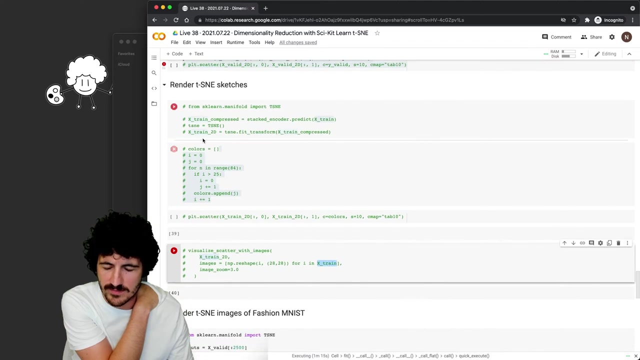 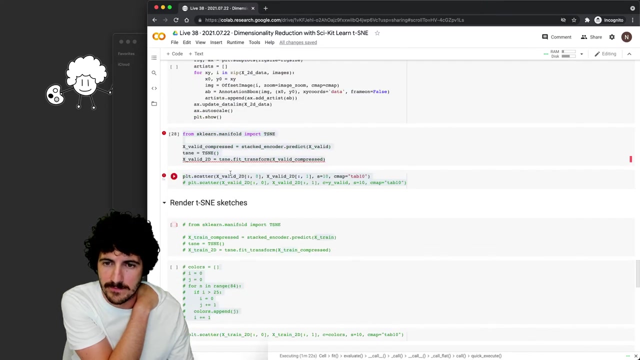 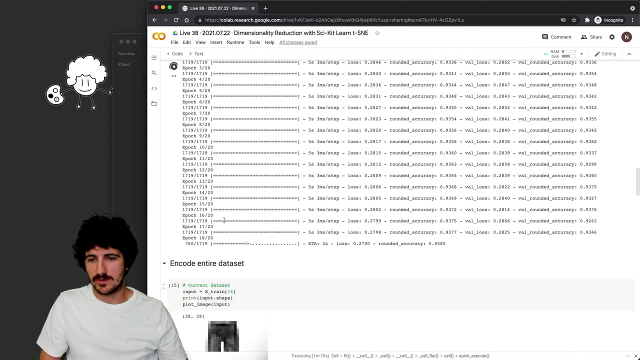 Yeah, Yeah, Yeah, Yeah, And we can put these helper function above. Yeah, So I think this was okay. So we have the extreme, an extreme here. Okay, Yeah, Okay, Okay, Yeah, Yeah, All right, So we are at um six, 17 epochs out of 20.. 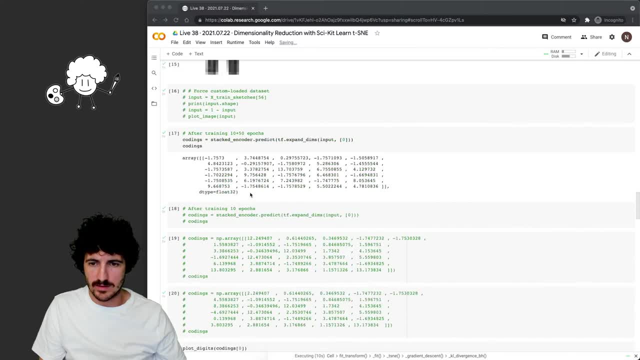 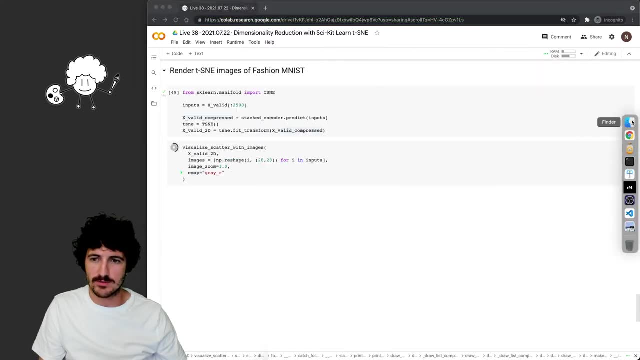 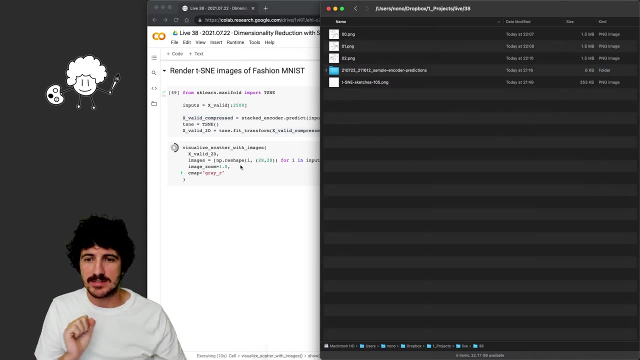 All right, And now this should be running. So this is run, and now it's going to run, All right. So this is the comparison moment. So we're going to take a look at whether training for 20 more epochs is improving anything of our um result. 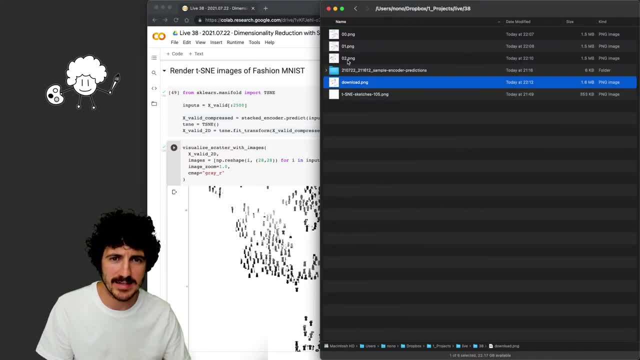 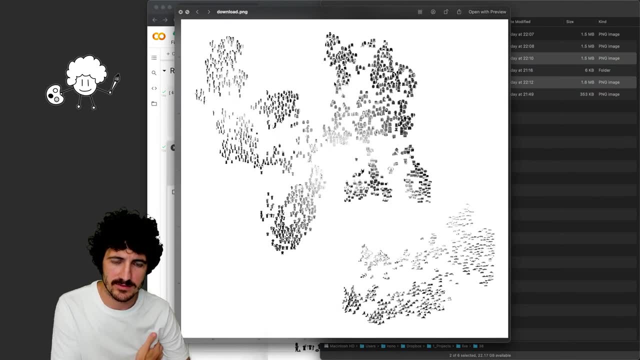 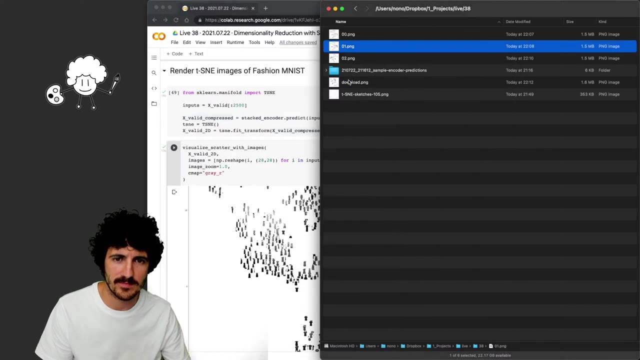 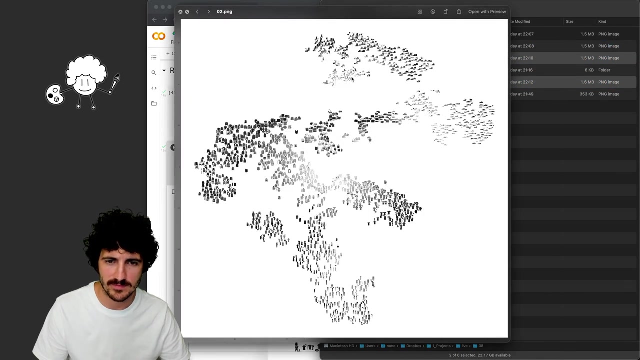 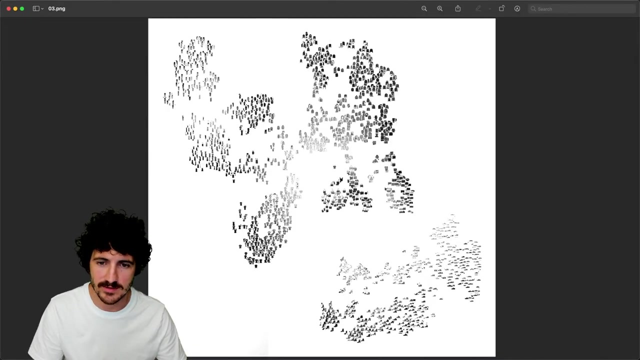 And maybe we have the axis changed again. I don't understand why. Okay, Uh, all right, So Disney doesn't um give us the same access all the time, which sucks. Hmm, So I can not compare, but anyhow, for some reason, this is not um doing that. 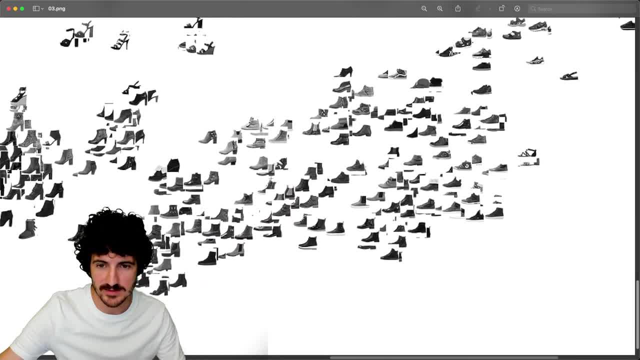 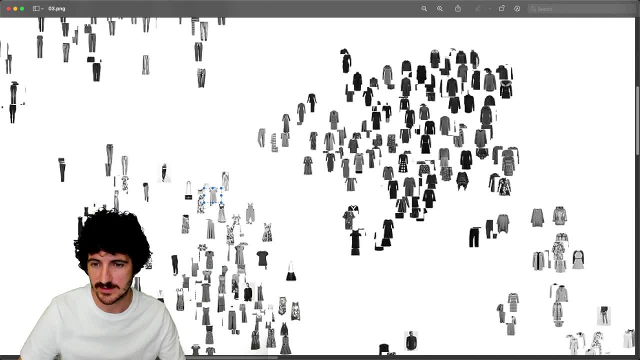 but yeah, this is great. So we're sorting shoes by similarity. So now You know, we could create a recommendation system just with these images, where, if you pick this dress, you could um propose a few other things that are around it. 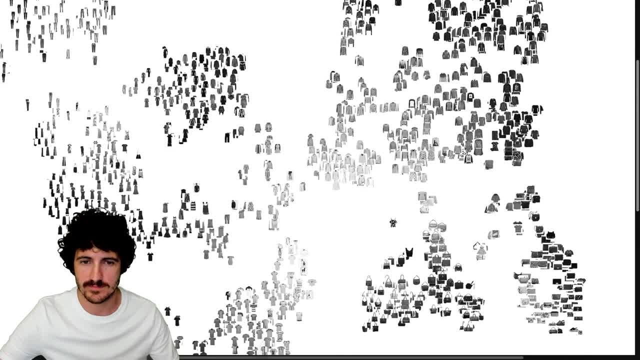 Great, All right, So this was live stream 38.. I always start thinking that I don't want to go for so long, but then we ended up getting into these things. Yeah, Yeah, Yeah, Yeah, Yeah, Yeah Yeah. 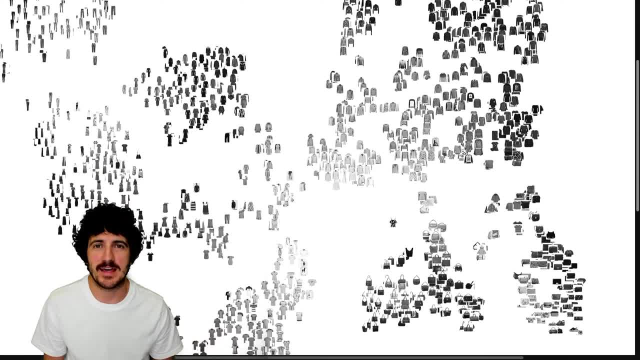 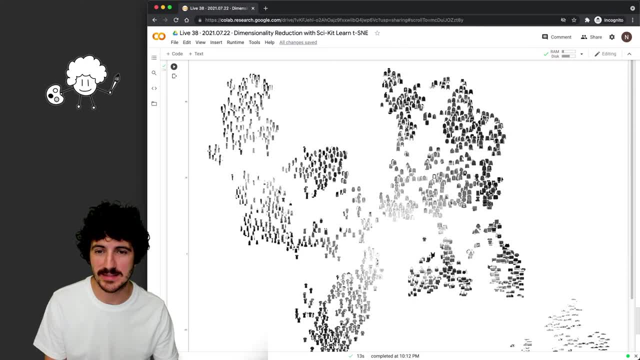 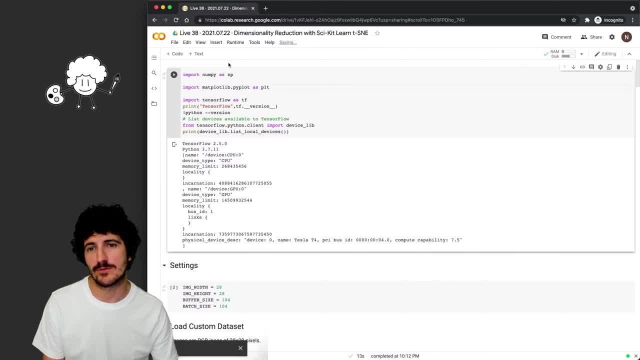 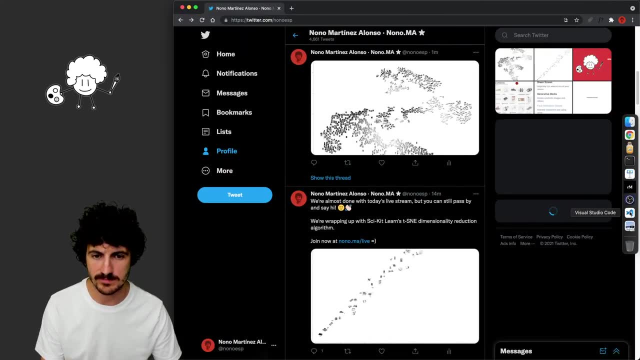 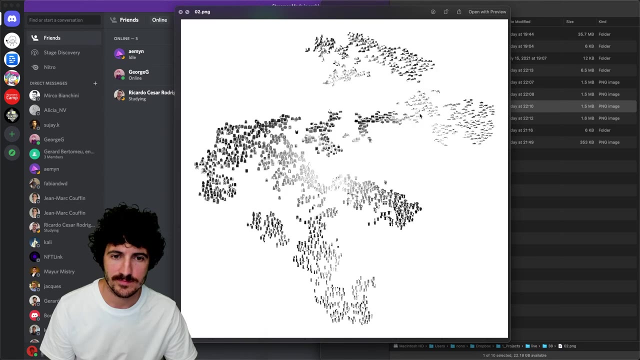 This has been awesome. We have the notebook there to check for everything that we've done. and and yeah, I'll do one thing- I'm just going to put the um- the outputs that we've obtained on the um- on. 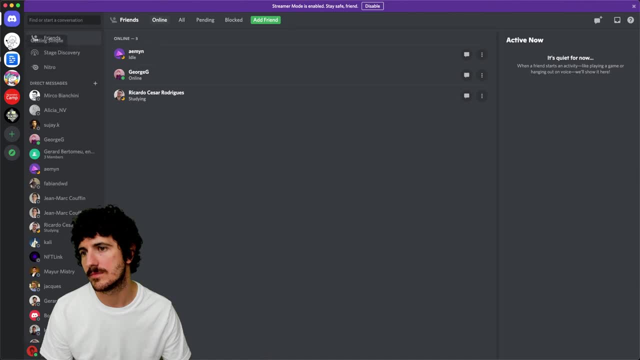 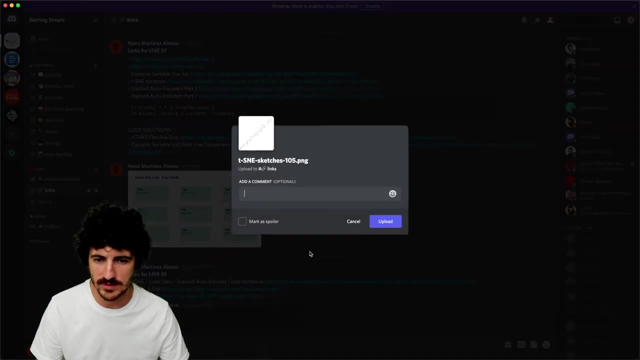 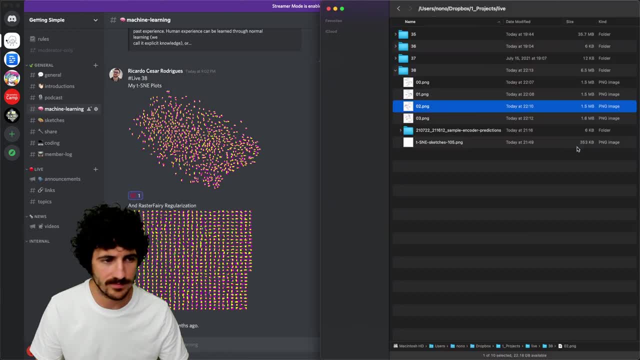 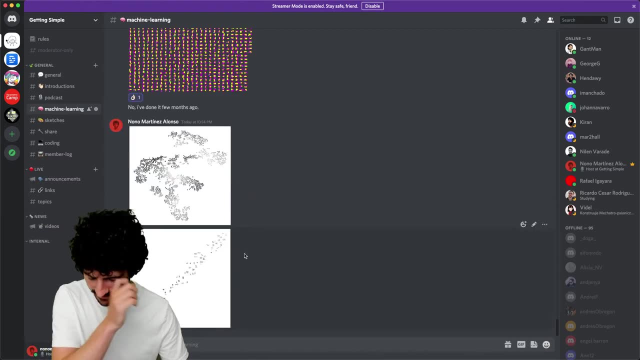 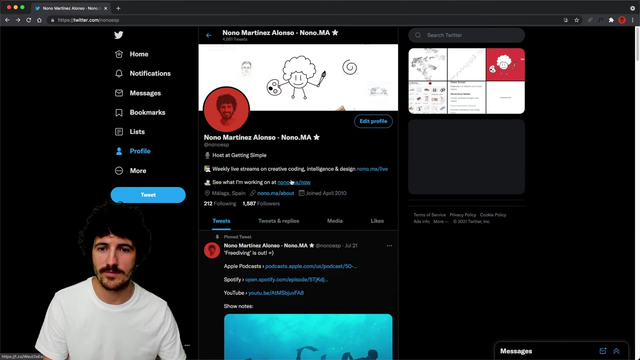 I hope you have a him. This concludes the keynote session. I hope everybody enjoyed it and I'll see you. That, Okay, Yeah, All right, And with all of that, if there's anyone who just connected, say hi. 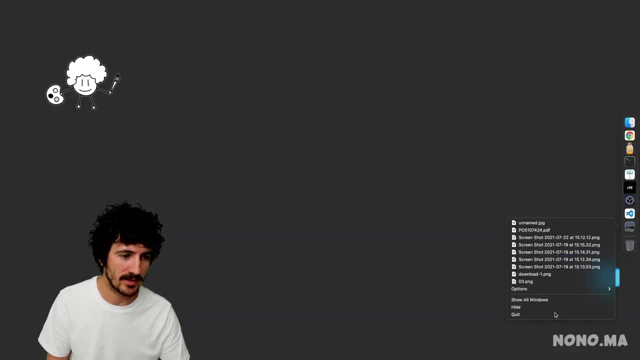 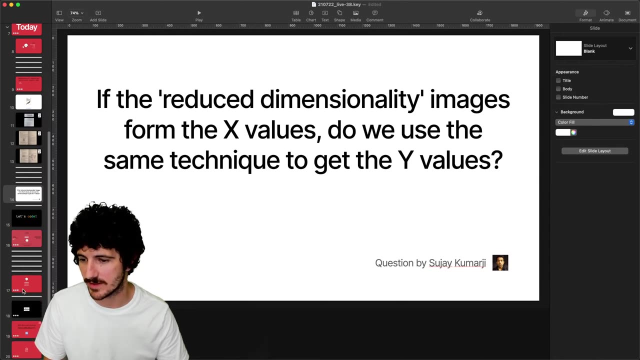 tell us where you're connecting from And, if you want to, you know if. if you want to ask anything, otherwise, um, we're done here. Uh, it's going to be. you know, it's going to be like um. 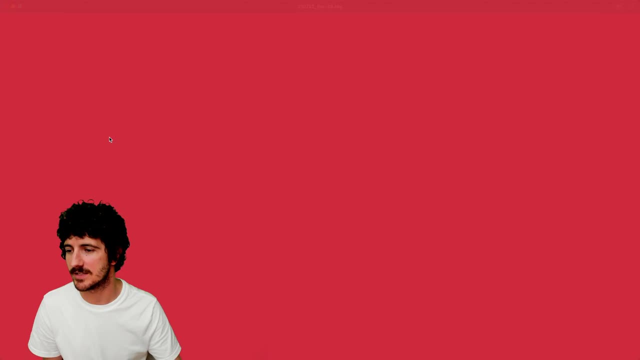 I mean it was a pleasure. I have enjoyed this session a lot. Thanks for everyone's participation. I really hope that you're learning something, as I am, So I didn't know any of like. I mean, I knew what we learned on previous. 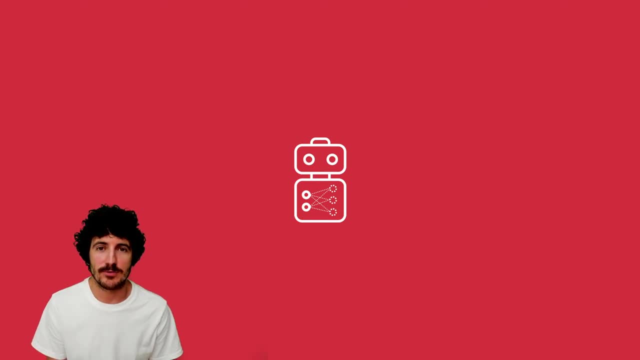 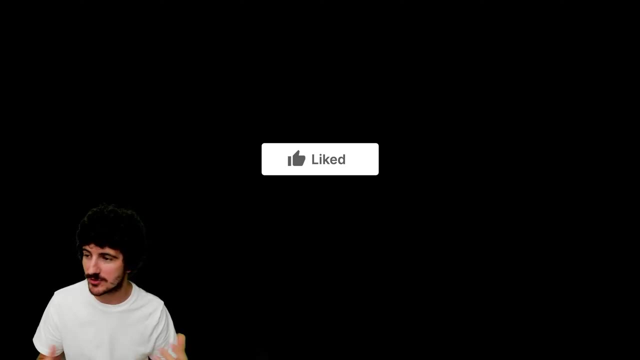 live streams. but I keep learning. So, yeah, call to action. support the channel by liking the video if you're enjoying or if you just want to support the work I'm doing here, And subscribe if you want to get notified when I go live next. 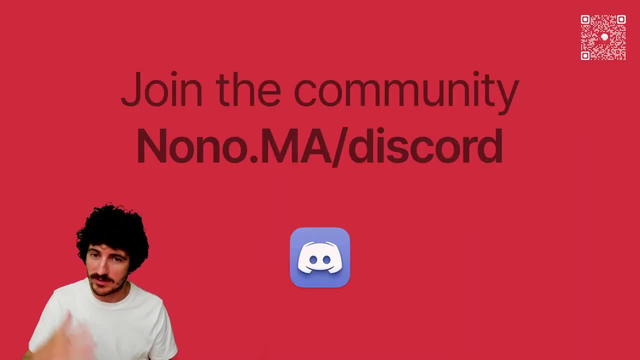 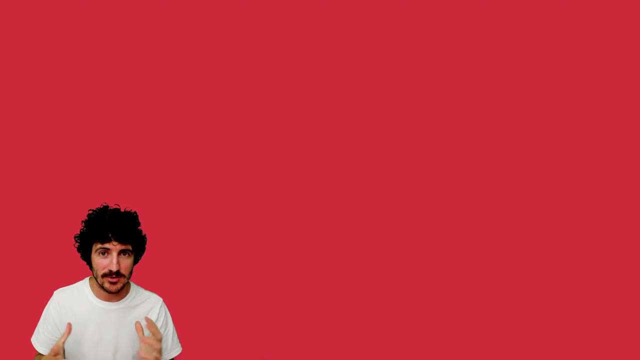 or when I upload new videos. you can join the community There is. you know I've repeated a bunch today. Um, I want to thank you for watching and I'll hopefully see you next time. On the meanwhile, you can go watch. um, many, many, many, many videos. 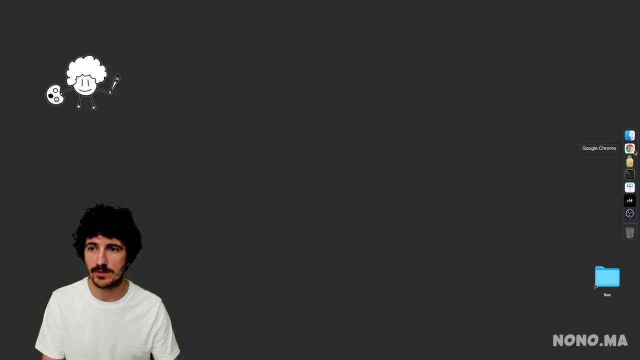 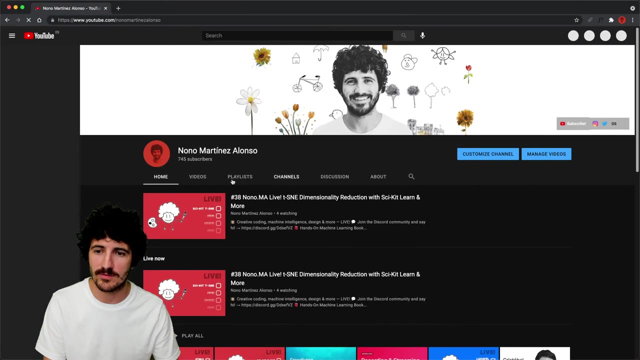 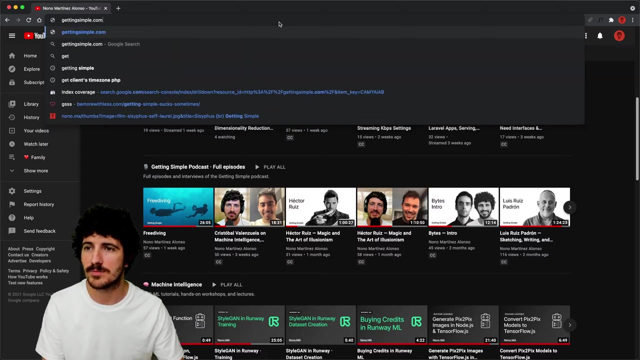 that are already online on on the um, on the YouTube channel. So we can see that, uh, none of the masters YouTube I, I have plenty of material, plenty of videos. also have um, um, so the the getting simple. 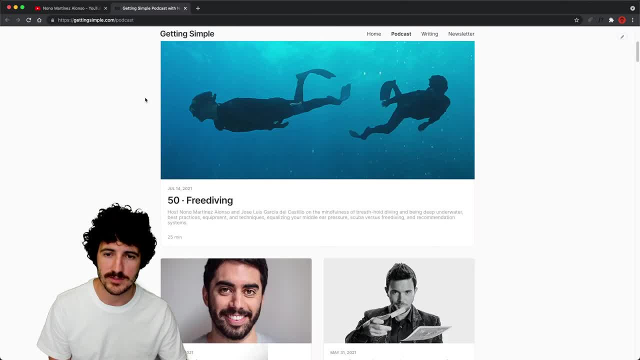 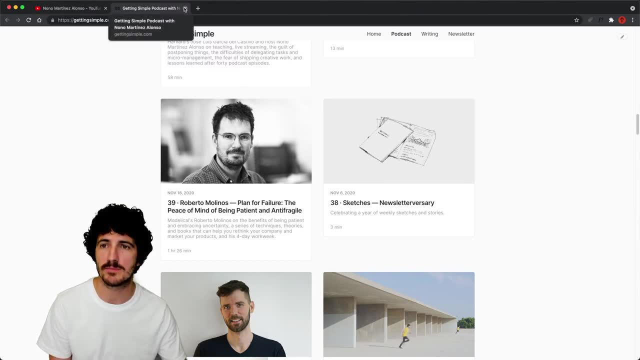 podcast that you can take a look at, getting simplecom. there is like 50 episodes already, many related with machine learning, others with design, art, creativity and more and more things, And I'll give a shout out to parametric camp. 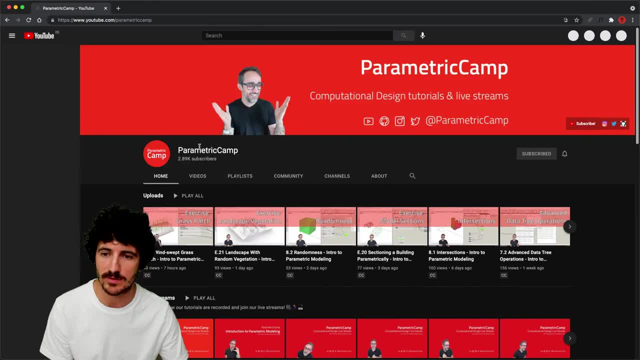 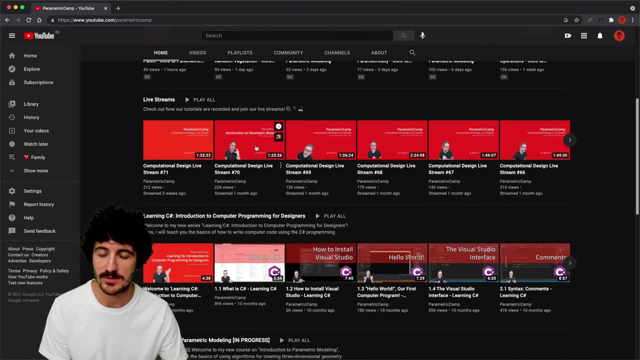 If you want to learn how to do parametric design with a grasshopper, uh, this is the place to go. also, a lot of C sharp, a lot of Um things. the computational design live stream by by Jose Luis is something. 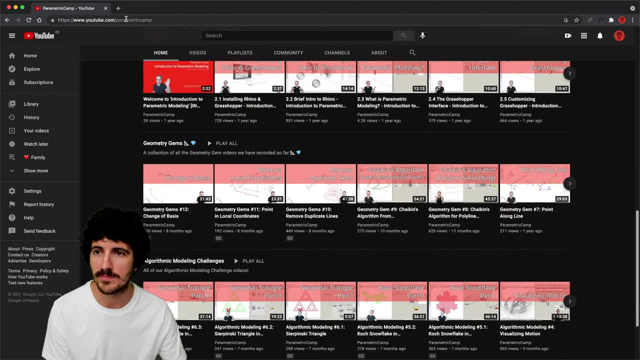 that, um, you can uh learn a lot from. I'll give also a shout out to, um, my, your mystery. I never find your channel, Uh, but I always look for it, So let's open Cognito here. 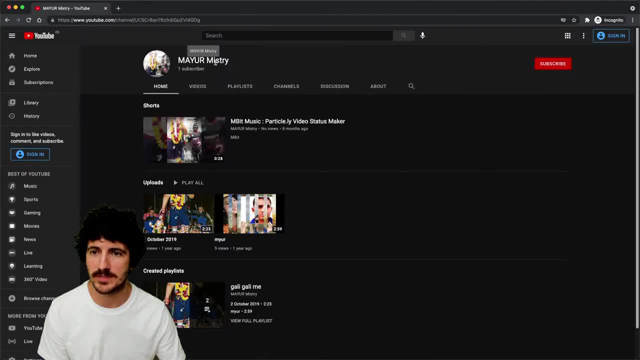 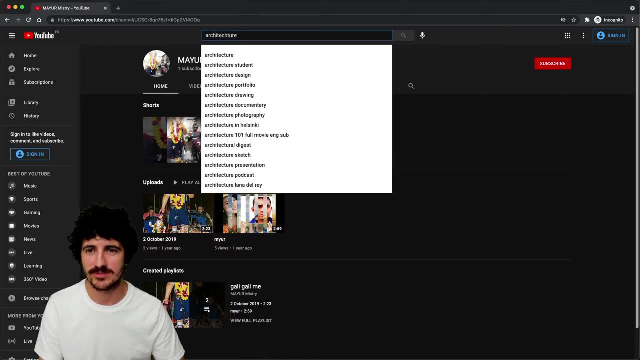 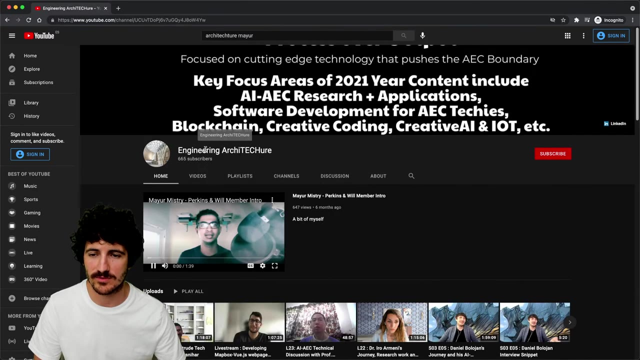 Um, you can look for my, your mystery. Well, this is not the one. Hey, I keep Sure. Yes, Engineering architecture. You can go follow his channel as well. Um, and yeah, I don't know a lot more to come check out. uh, Ricardo Ricardo's. 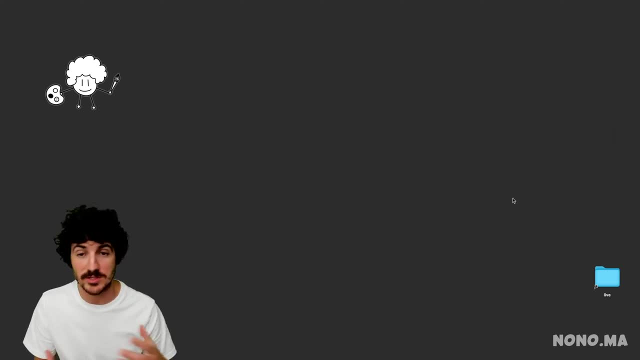 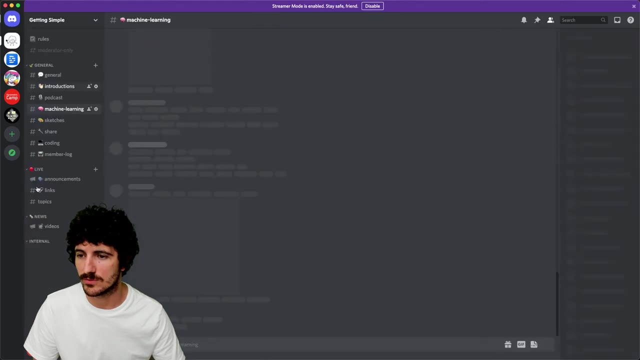 work as well. Um, you know if you're watching or if you're watching after the fact and you want to share your work? uh, join the community, go to The um, go to the shared channel, and people are already doing that here. 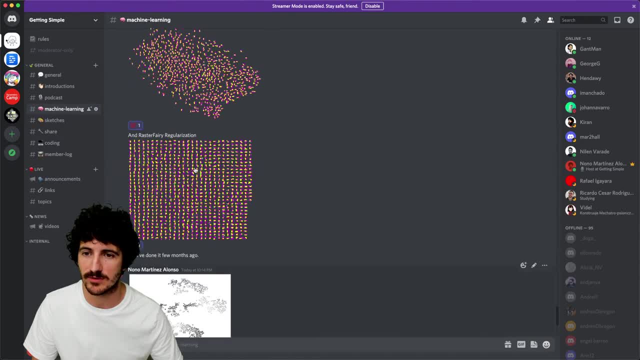 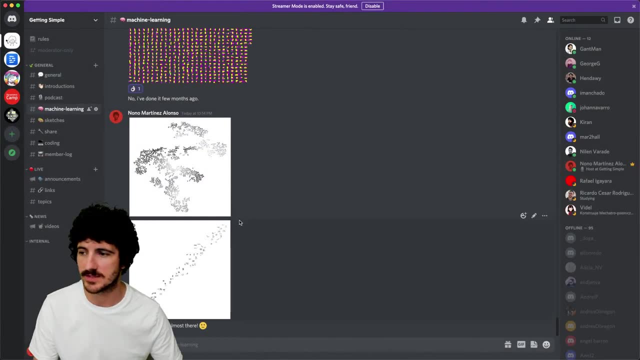 They're sharing things. If there is something really specific, for example, as Ricardo did today, to share, maybe you can share on the machine learning channel. or as I did with some of the outcomes of this life. Sure, Once again, it was not a market. 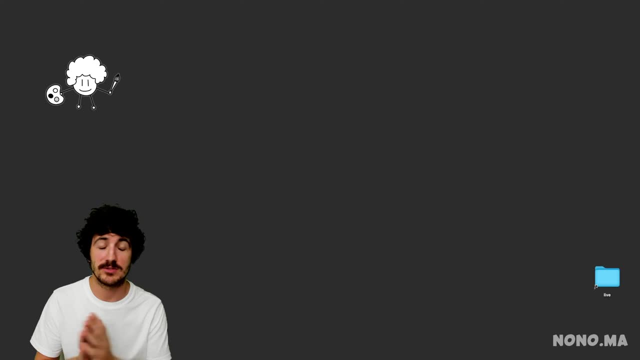 I'll answer here. Thanks a lot for being there. I would appreciate your comments. Uh, if you have any questions, any suggestions, leave them on the video comments And, um yeah, I'll see you next time. Bye.